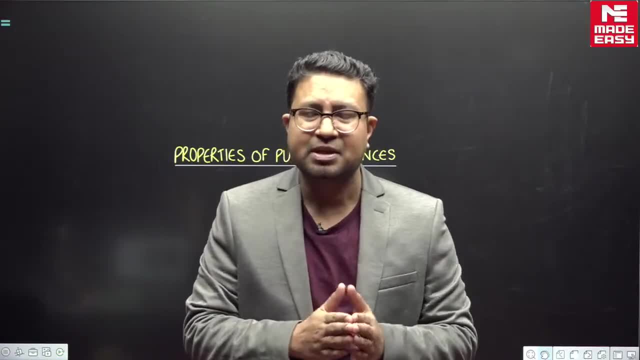 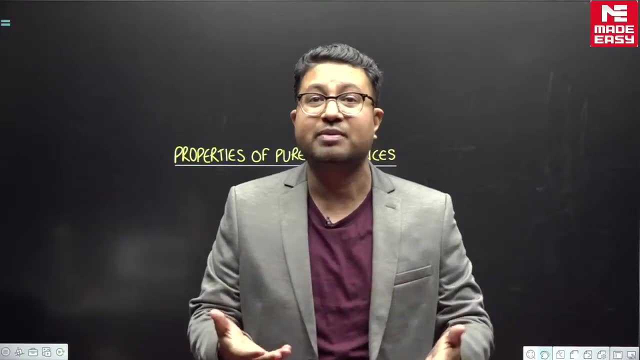 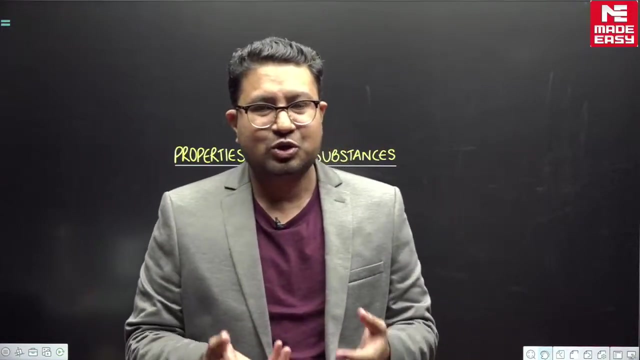 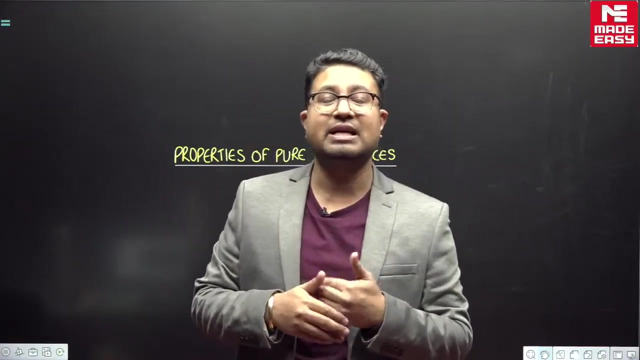 Thank you, though, and when you give the test, that is not something to demotivate you, because the test is actually showing you those areas where you need to work again. So test is not the final result, but once you give the test, you get to know whatever areas are weak Now. 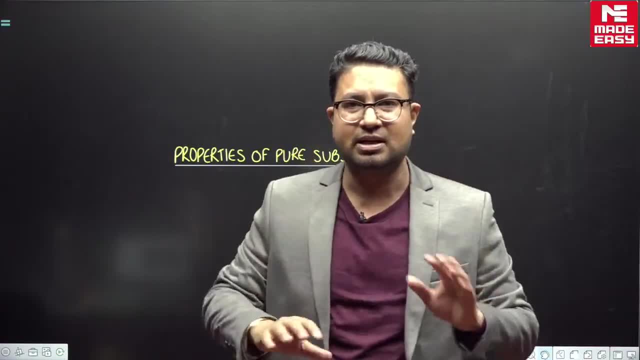 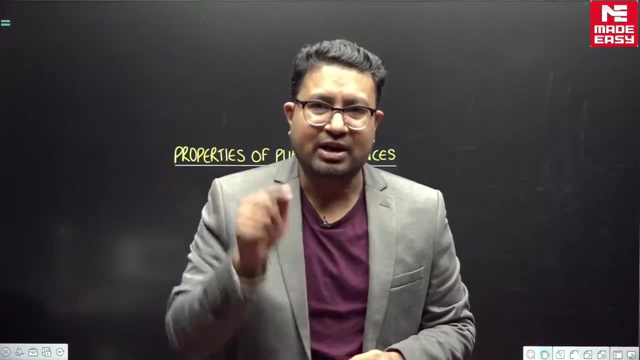 some people what they do. they give the test, they get the marks and that is done. then they move on to the another test. that should not be done. I think What you should do is, when you have given the test, whatever questions you are not able to solve, revise that part. try to understand why you are not able to solve those questions. 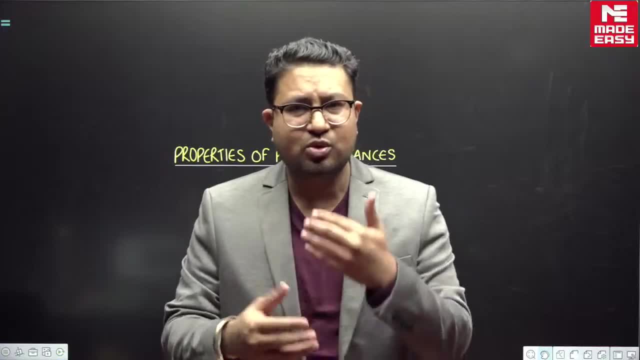 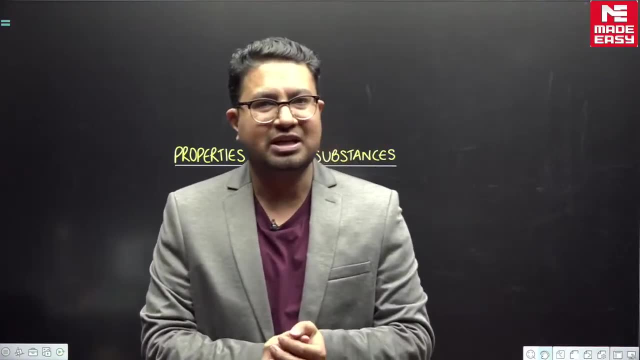 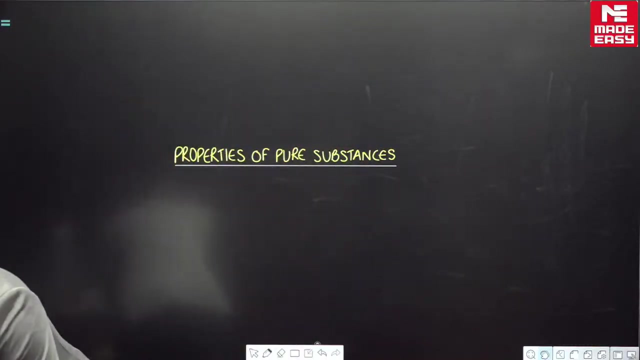 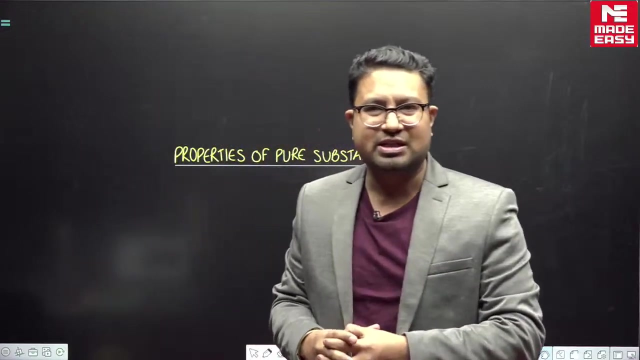 So that is how you will get best, which that test has to give it to you. fine, So let us start with the discussion, today's discussion. we will start, and so, yes, good evening, very good evening and happy new year To all of you. So let us start with the today's discussion. properties of pure substance. ok, 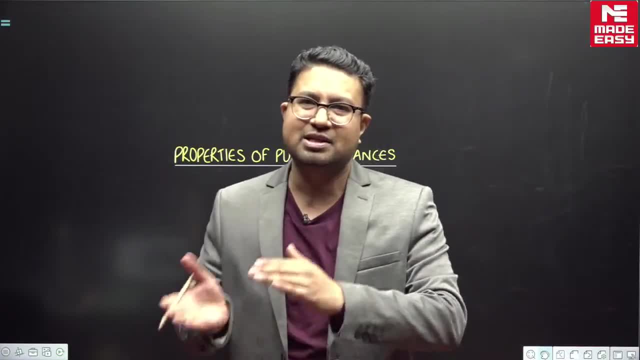 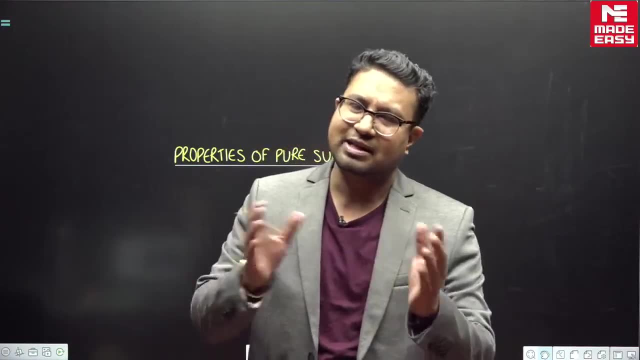 I have, whatever discussion I will be doing, I will be doing the discussion in Hindi as well as English. So anybody who is watching with ah, I mean who is not comfortable in Hindi, then also there is no problem. and who is only comfortable in Hindi, then also there is no. 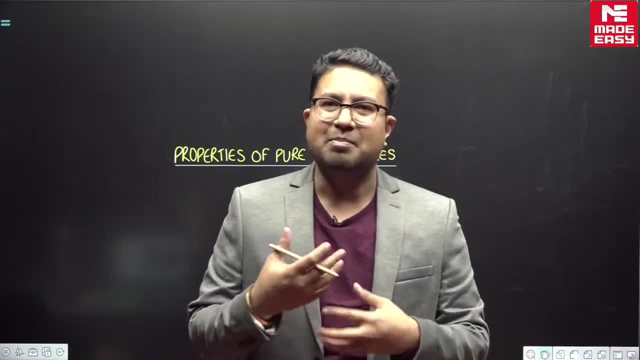 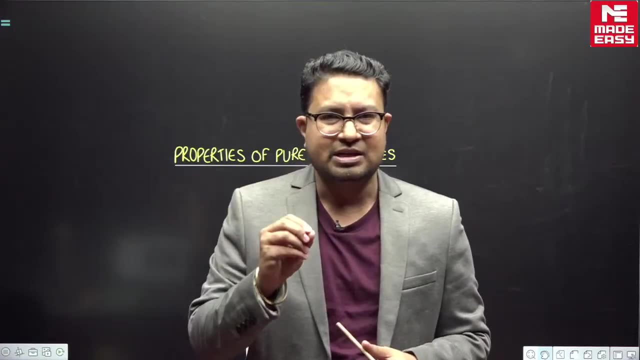 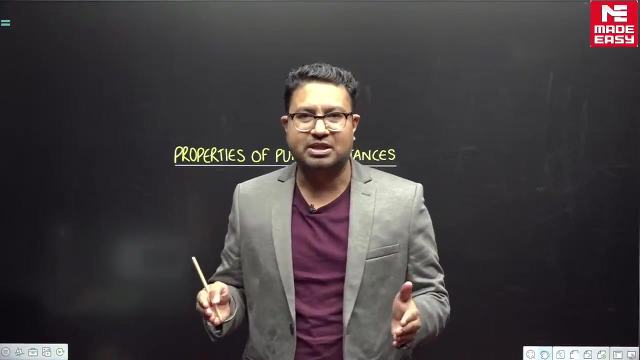 problem? no problem, because whatever I will tell you, I will mix both the languages, So you do not have to worry about it. ok, So we do not have to worry, we will do it. So let us start. Just focus on whatever the discussion is going on Now. ah, if we see pure substance, 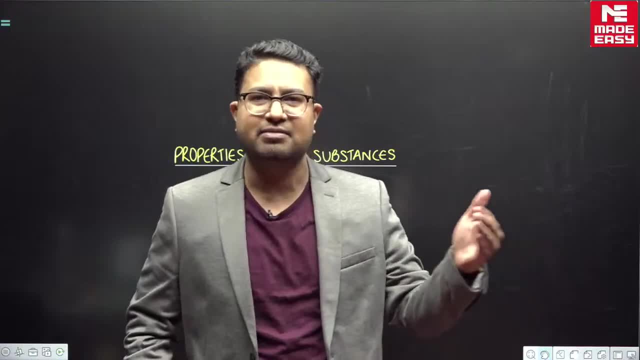 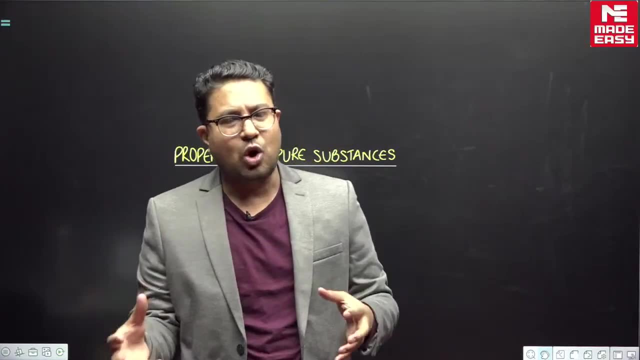 so pure substance questions that are asked in the gait exam. recently they have ah. in the last 3, 4 years They have continuously asked question on this. it is there, continuously, question is asked, Or they will combine it with the questions of first law, first law. 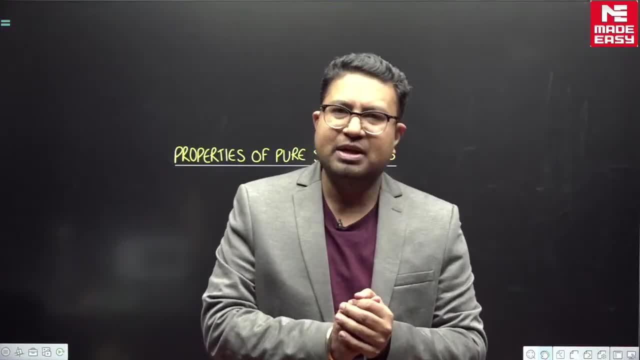 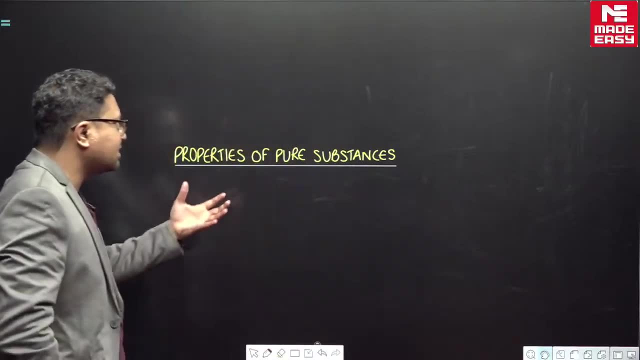 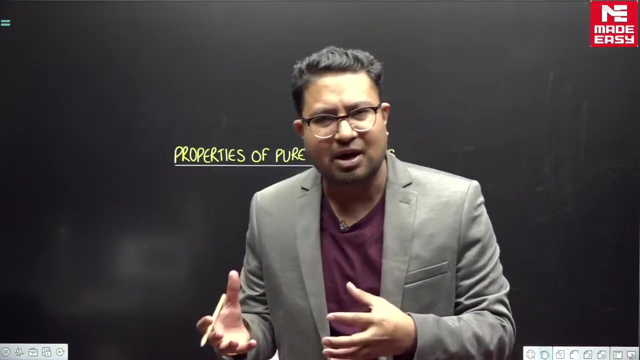 combinations also take. So if we are comfortable with this topic, we will be easily able to answer the questions. ü. So properties of pure substance. now, what is a pure substance? pure substance, what is a pure substance? So when we talk about a pure substance, when we talk about pure substance in the very basic, 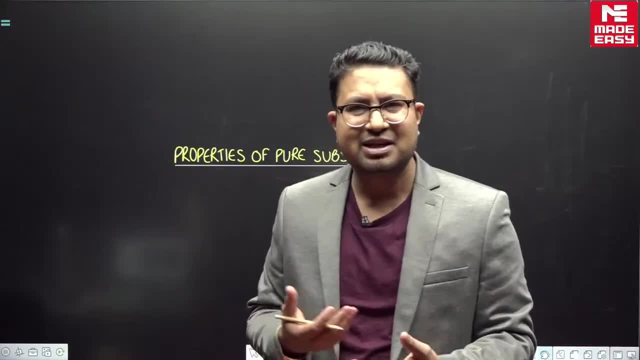 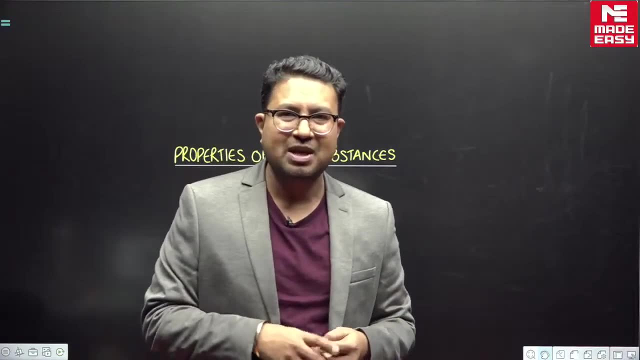 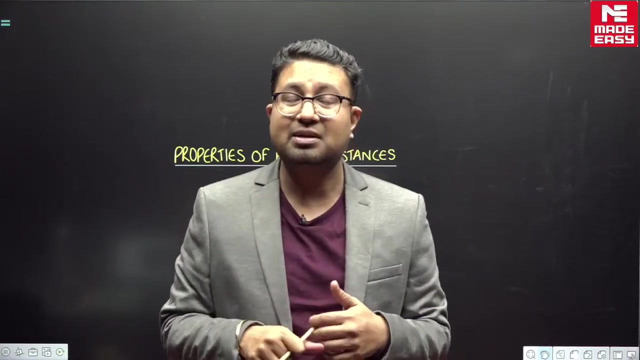 beginning of the thermodynamics, there is a definition which we give right. we give a definition As such pure substance should mean as such pure substance should mean. I will tell you the physical essence of it. pure substance means one substance, But sometimes, sometimes, whether it can be in the liquid phase or liquid plus vapor phase, 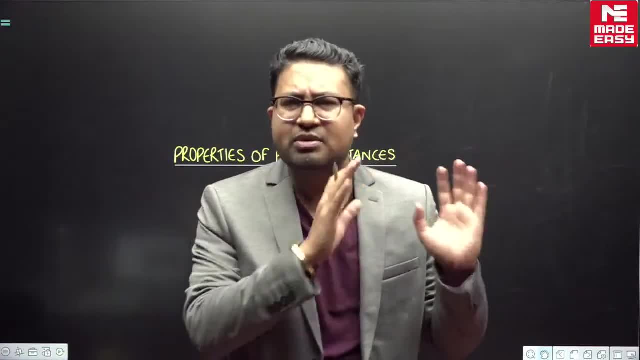 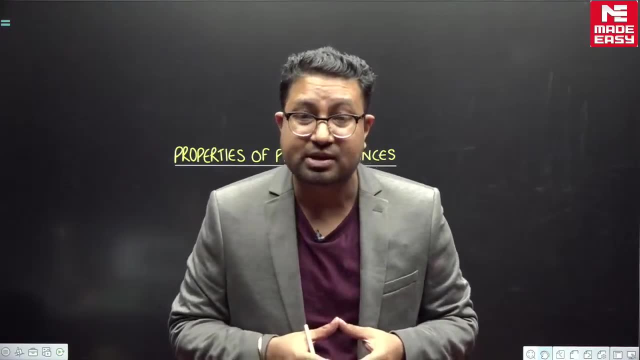 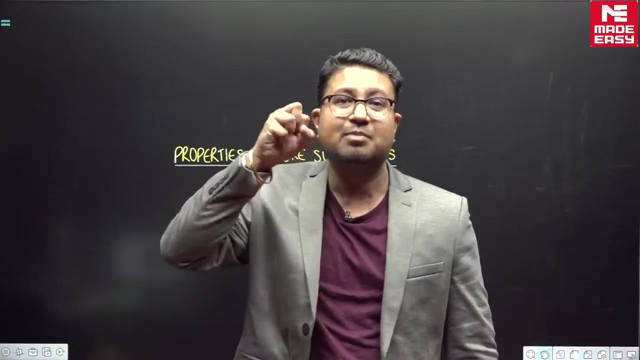 or liquid, vapor or solid phase, but only one chemical compound, only one chemical compound. But even if there are multiple chemical compound mixed together, even if there are multiple chemical compound mixed together, sometimes we can treat them as a single component of the substance. 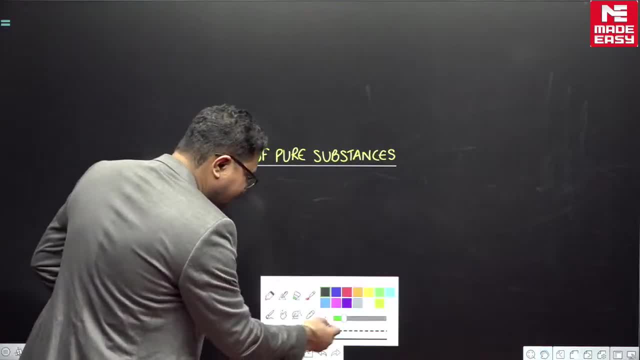 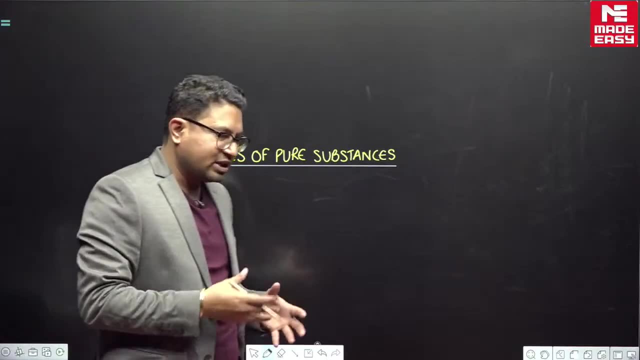 So if we talk about the water, if we talk about the water, H2O. if you talk about H2O, so when we talk about the H2O it can be in the liquid phase. suppose there is H2O in the. 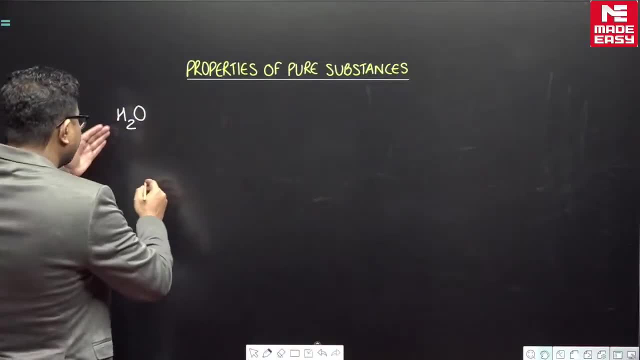 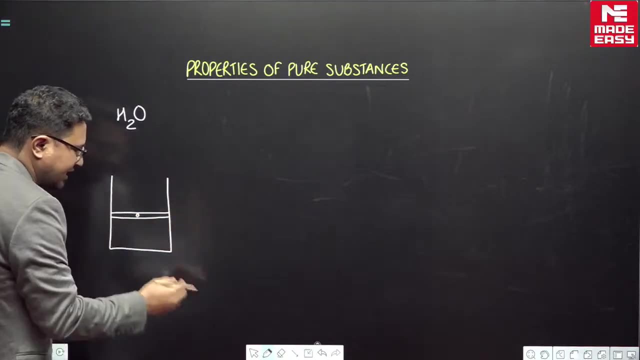 liquid phase. So we will say, we will say that if there is H2O in the liquid phase, suppose it is kept in a container. kept in a container and we have H2O kept in it, H2O is there, in which. 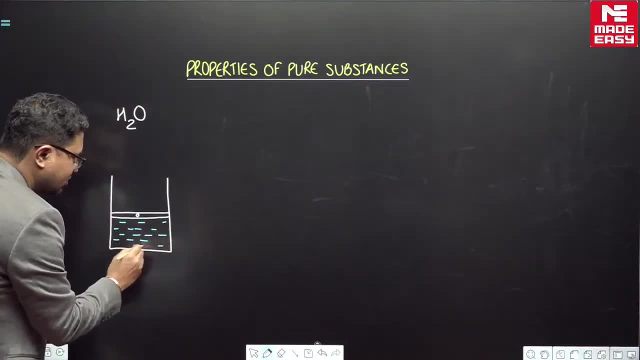 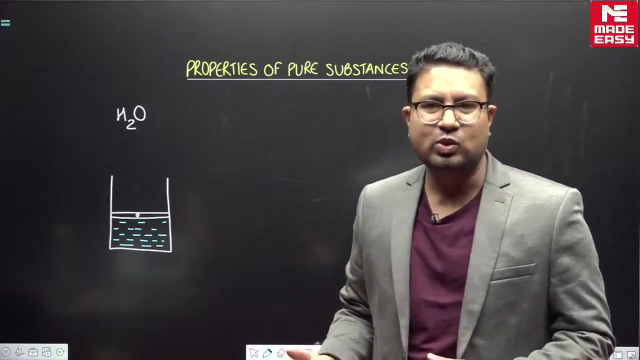 state there is H2O, In which state The H2O is? in which state is H2O in the liquid state? So we have a container. there is a container in which the H2O has been kept. H2O is kept. 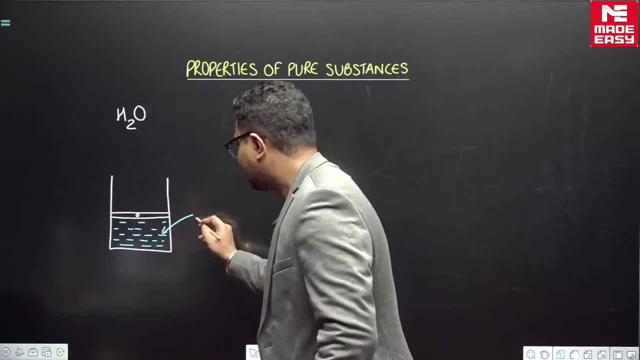 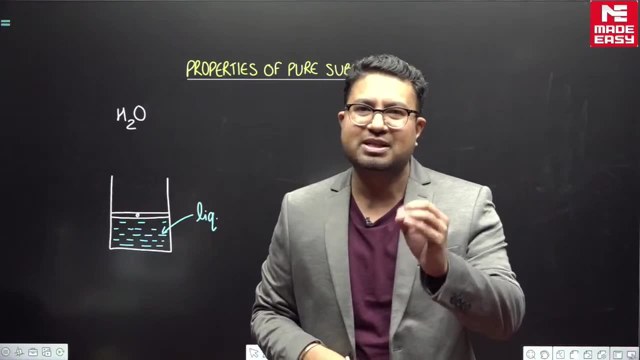 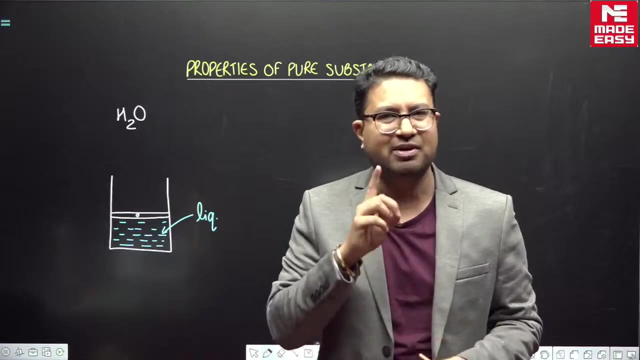 water is there in the liquid state, in the liquid state. So we have the water in the liquid state. in the liquid state. Now it is a single chemical compound, so pure substance if we see physically. so it should be a single substance. there should be one chemical compound. it should be one. 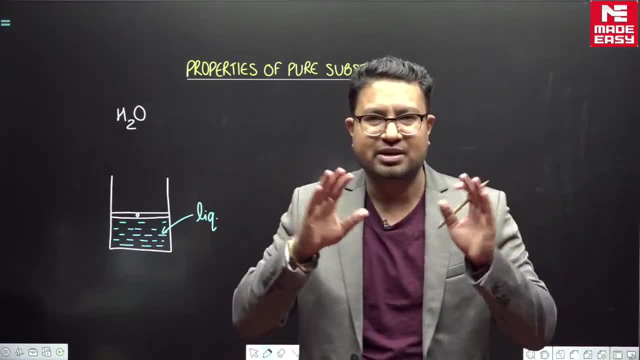 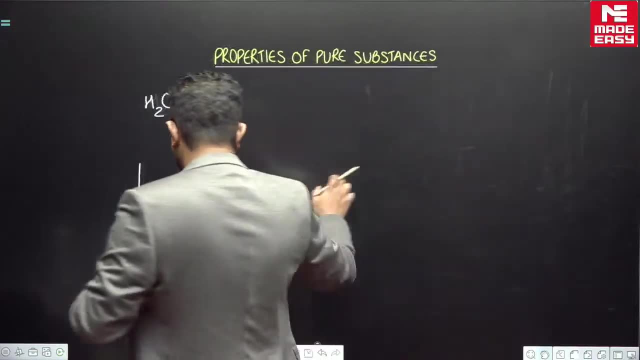 chemical compound, But the definition of pure substance. according to that, if we see, if we see what is the definition of the pure substance, what is the definition? A substance is said to be a pure substance. A substance, a substance, a substance is said to be, we will say said to be said to be. 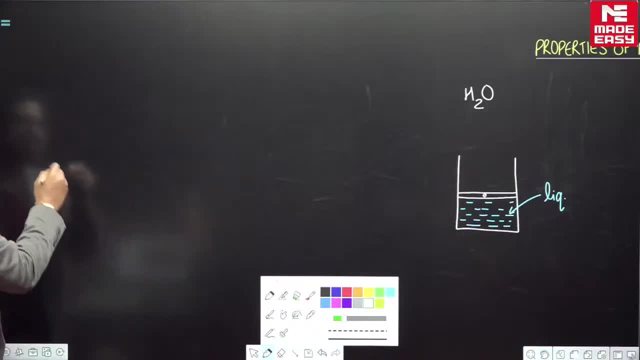 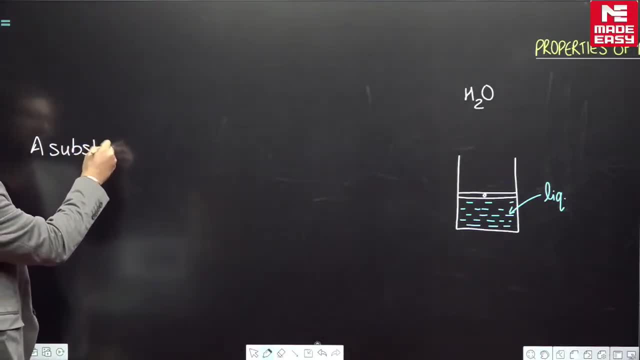 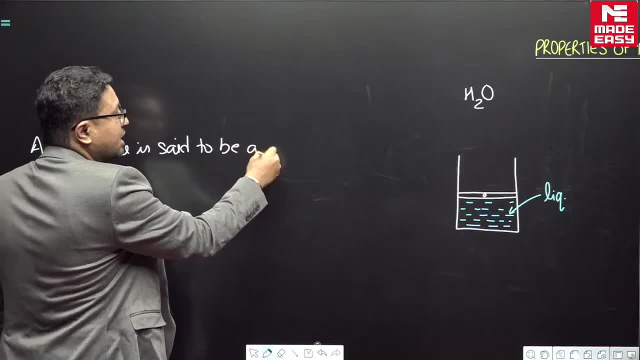 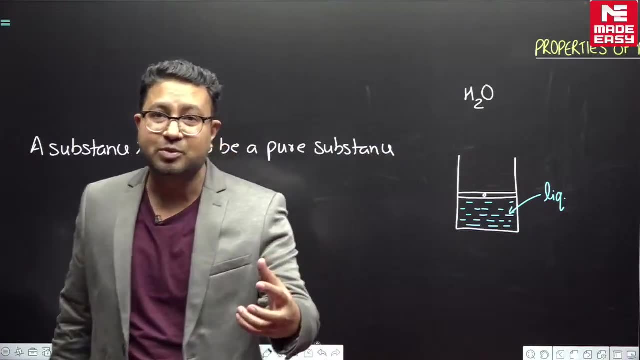 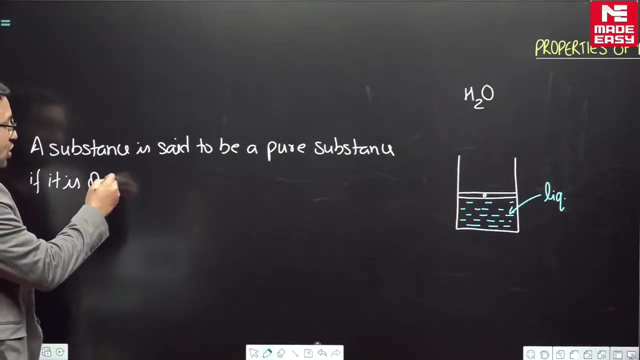 A substance is said to be a pure substance, said to be said to be a pure substance, a pure substance, a substance is said to be a pure substance. we will say that a substance is a pure substance. a substance is said to be a pure substance if it is, if it is of homogeneous, homogeneous, homogeneous chemical composition. 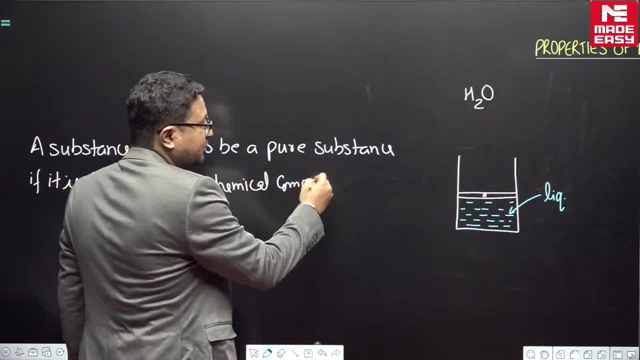 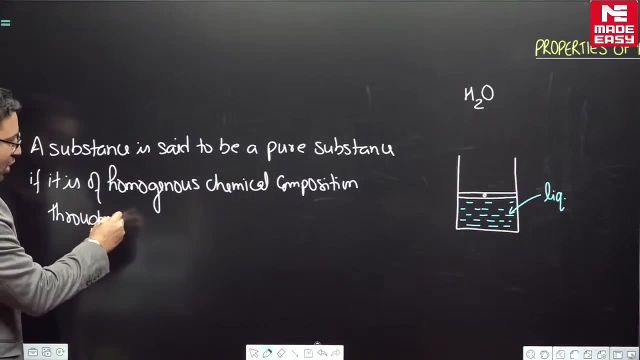 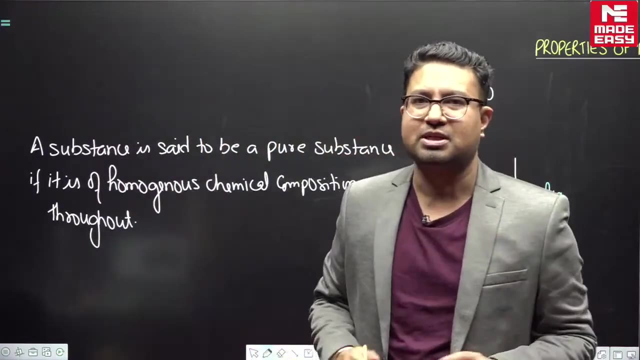 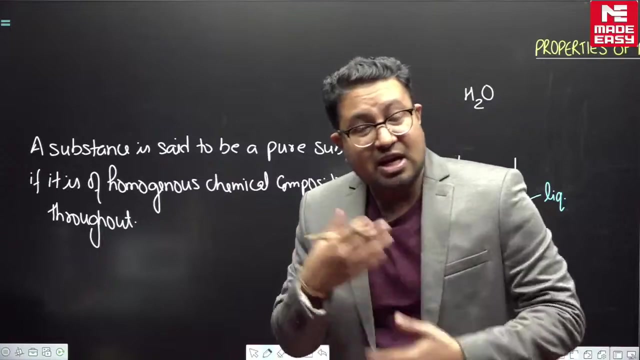 chemical composition: composition throughout, throughout. homogeneous chemical composition throughout. any chemical composition is the same throughout. So if the chemical composition is same throughout, we will call it as a pure substance. pure substance means pure substance means having one component, chemical compound, but even if it is not a single chemical compound, 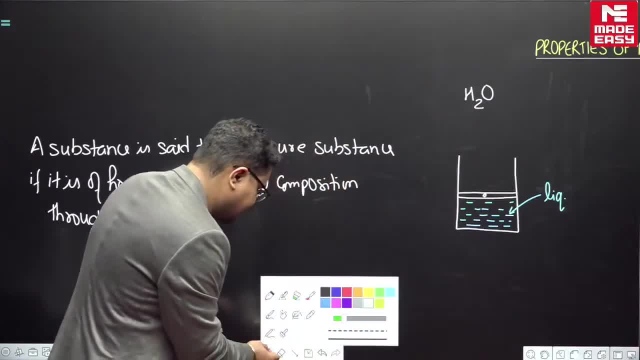 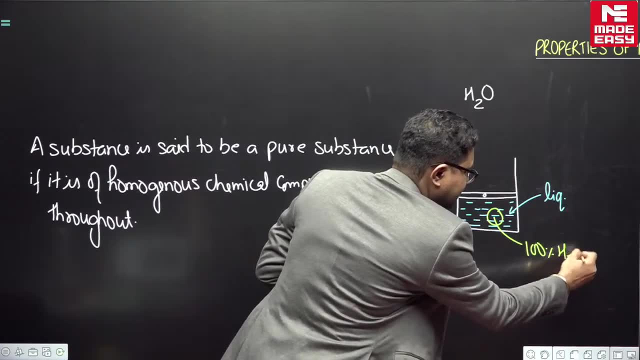 If there is no chemical compound like air. suppose, in this case, if you take a sample here, what will you get? 100% H2O? What you will get 100% H2O? There is one chemical compound and that chemical compound is H2O. 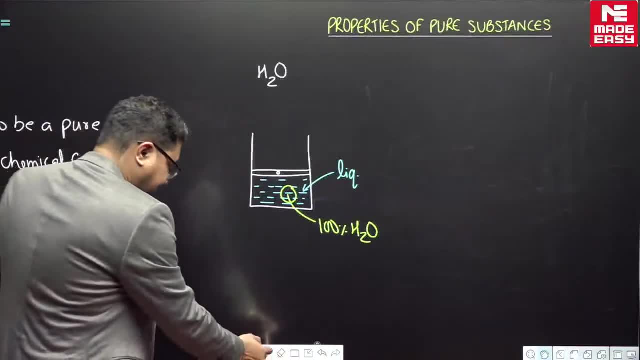 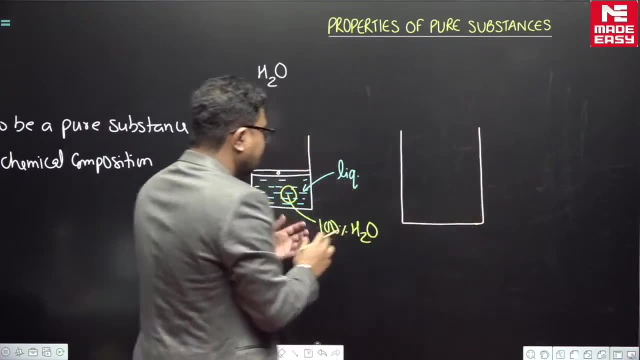 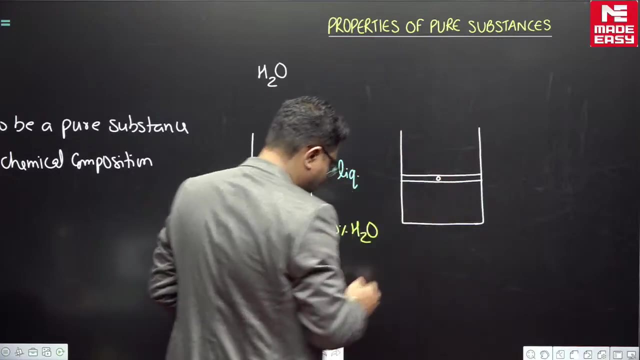 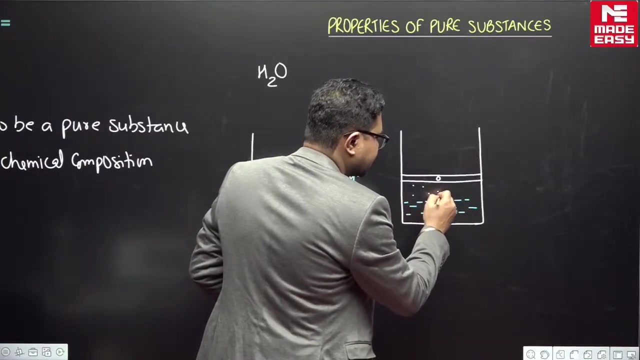 There is only H2O. Now suppose we have. I will talk about the air also. Suppose we have a piston cylinder element and in this H2O is present. H2O is present in liquid state and H2O is also present in the vapor state. 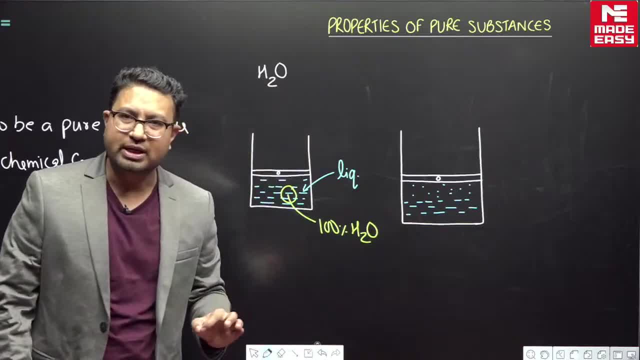 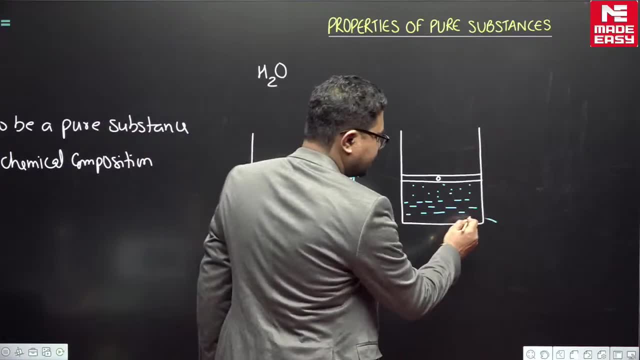 H2O is present in vapor state. H2O is present. Chemical compound is H2O, H2O. it is present in the liquid state. It is present in the liquid state. H2O is present in the liquid state and H2O is present in the vapor state. 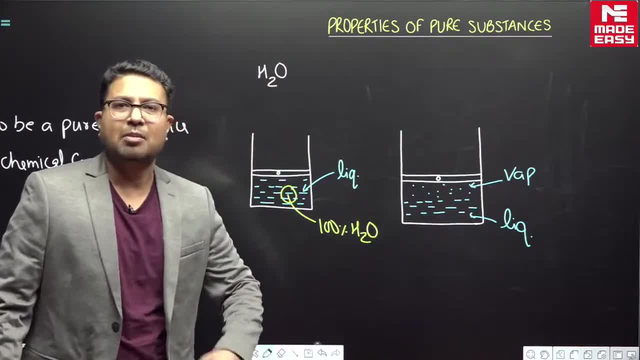 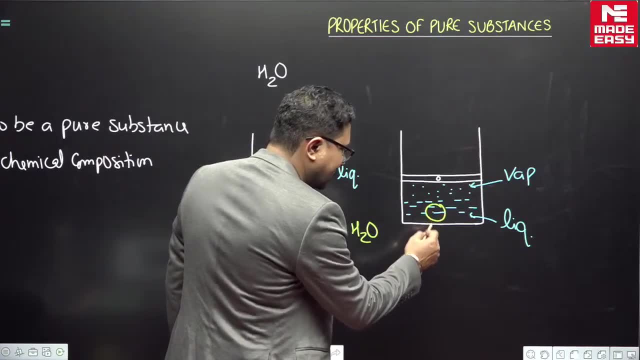 And H2O is present in vapor state too. Okay, Now I have to decide whether it is a pure substance or not. So see, when I take a sample here, what will I get? I will get 100% H2O. 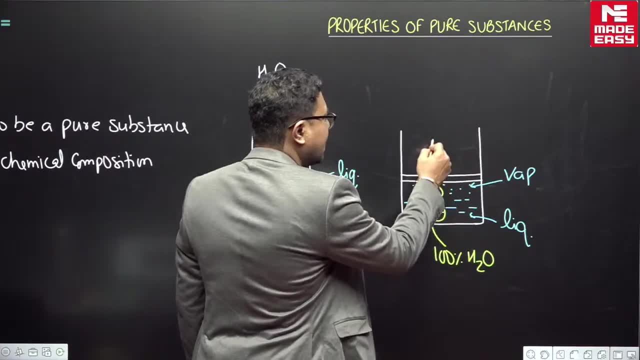 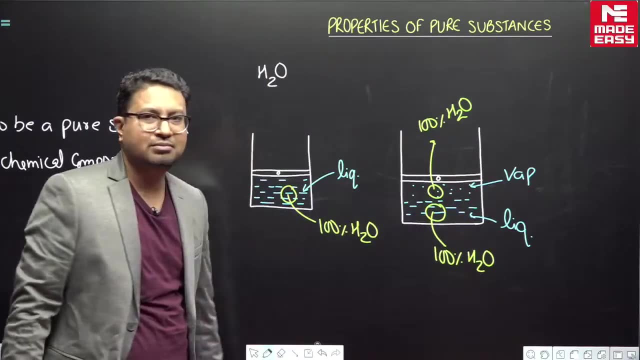 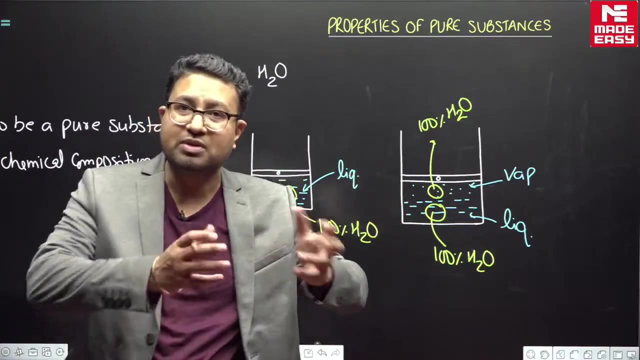 100% H2O. And if I take a sample here, what will I get? I will get 100% H2O, 100% H2O, 100% H2O. Yes, So H2O, whether it is in liquid phase or vapor phase, or both the phases or any other compound. 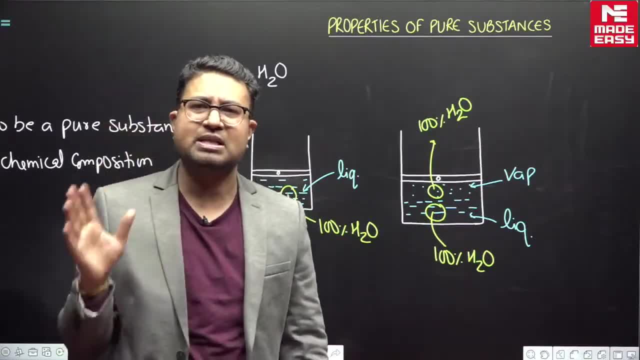 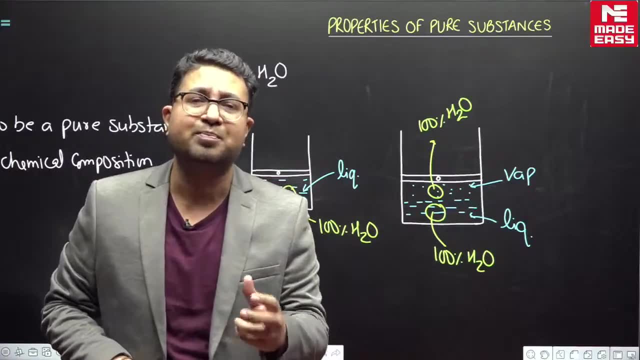 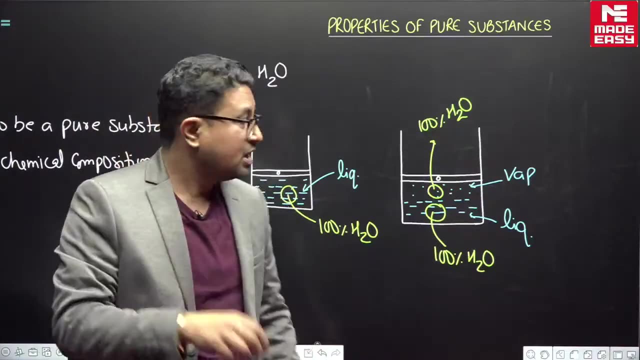 if there is only one chemical compound, no matter how many phases are present, it is always a pure substance. It is always only one chemical compound. So when we have to think whether we should treat it as a single compound or not, See. so if there is only one chemical compound, then always, always, it is one compound there. 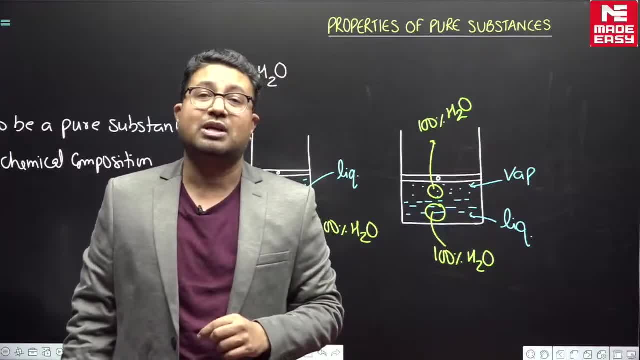 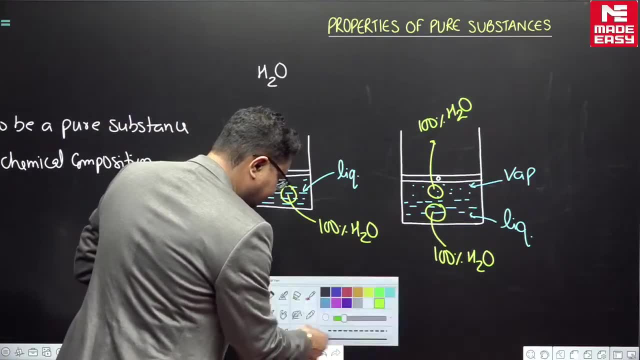 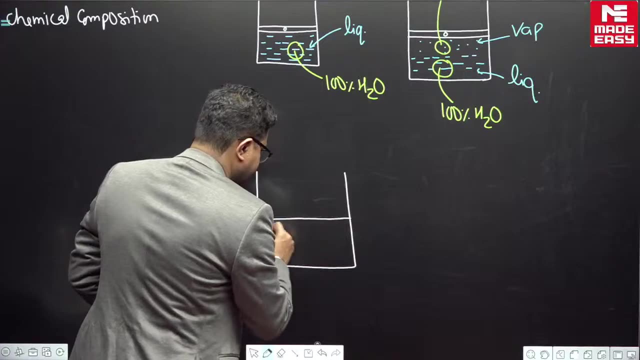 is no doubt about it. there is no doubt about it. but what happens is that when it is not a single chemical compound, one chemical compound like gaseous air, if we talk about gaseous air, so if we talk about the gaseous air, if we talk about gaseous gaseous air, 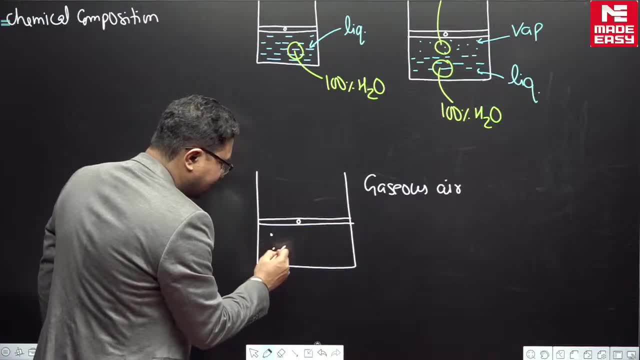 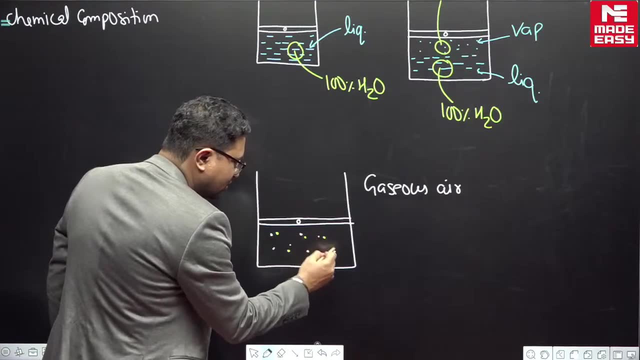 So gaseous air? if we talk about gaseous air, then what is there in air O2 N2 mix? there is mixture of O2 N2 water vapor mixture. there is a mixture in gaseous air O2 N2 water vapor. 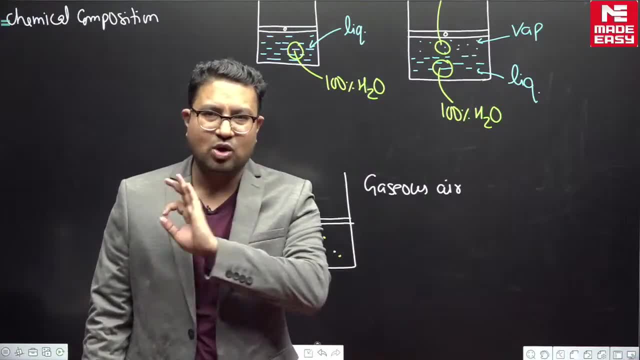 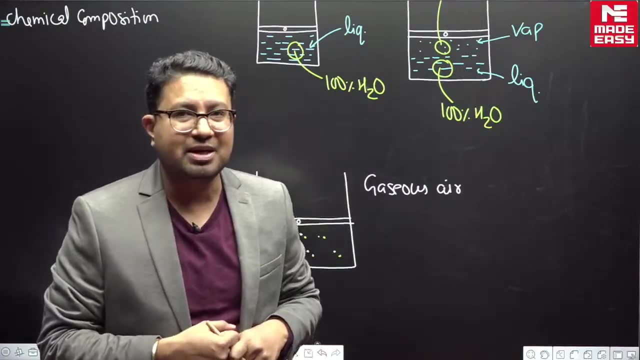 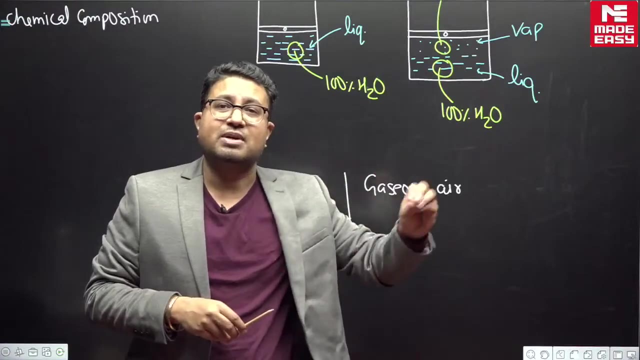 mixture is there in gaseous air. now one component is not there, it is not directly one component. so we say, we say that even if you are not a single component, even if you are not a single component, even if you are not a single component, then also for some of our study we may be able to treat you. 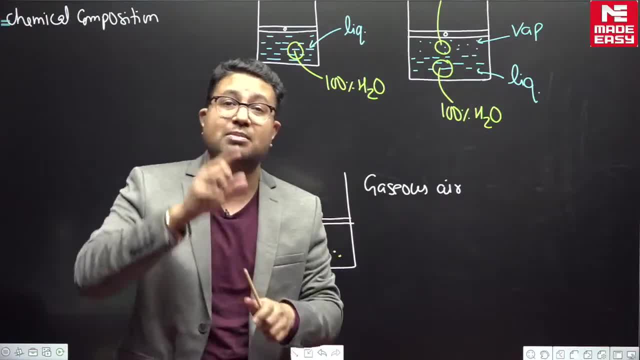 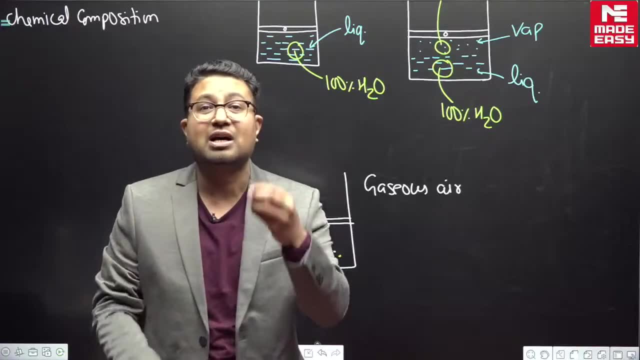 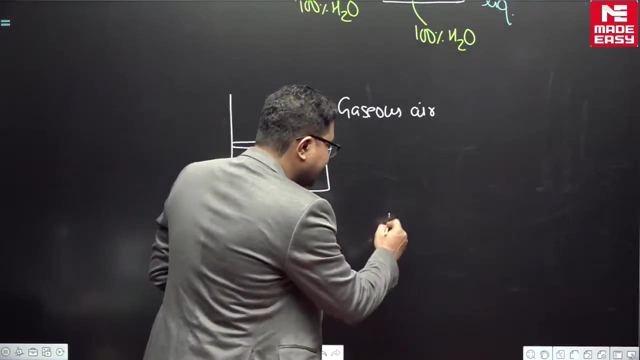 as a single component. Pure substance means one chemical component, but even if it is a single, even if it is not a single component, then in some cases we are able to treat it as one component. We write PV equal to MRT. so when we write PV equal to MRT, we use it as a single component. 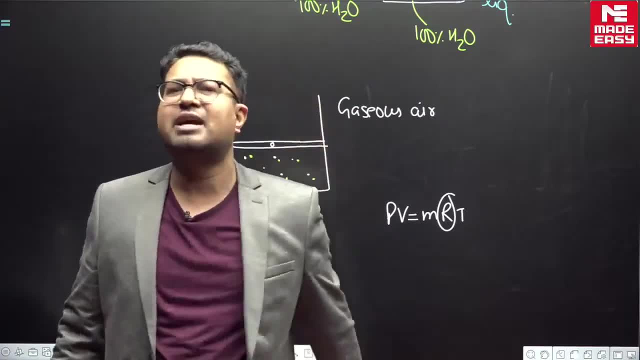 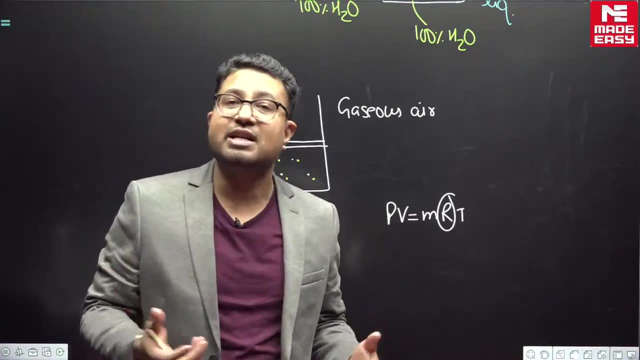 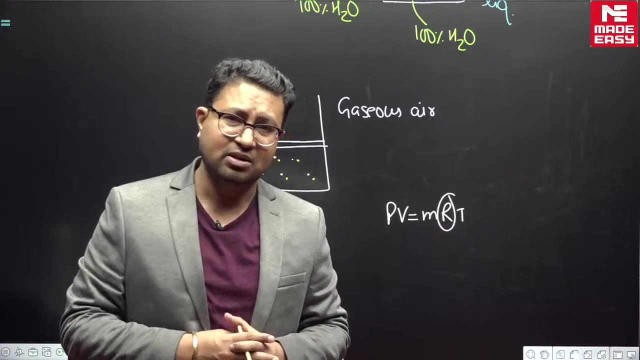 We write 1R for the entire mixture. For the whole mixture, we write 1R. So we treat the gaseous air as a pure substance. We treat the gaseous air as a pure substance. We treat the air as one component. 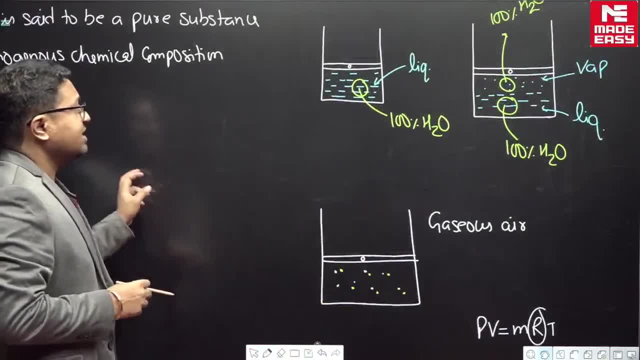 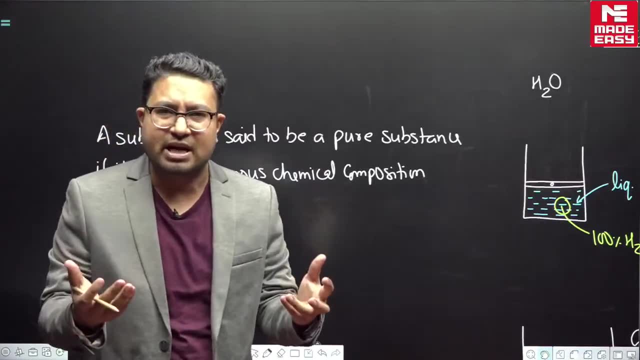 We treat the air as one component. Now you see, Here, here, here, what we are going to study. Here. we are not going to study the definitions of pure substance. I just gave you an idea. I just gave you an idea. What is a pure substance? So, pure substance means a single chemical compound. 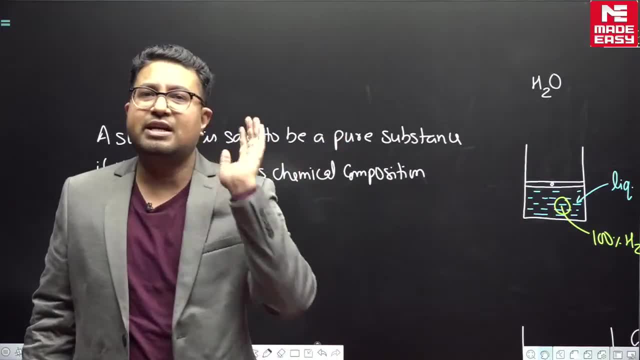 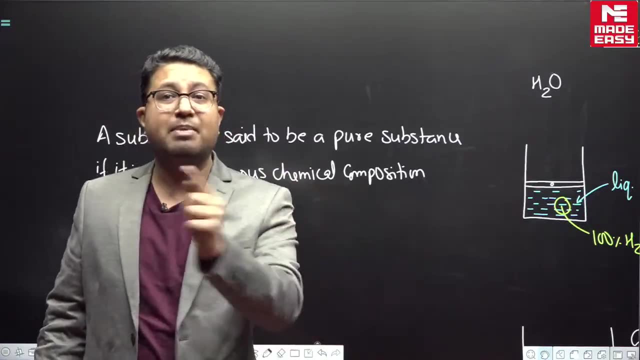 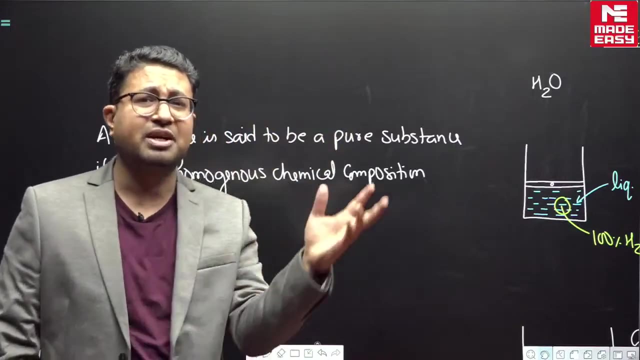 but even if it is a multiple compound mixture, If it is a mixture of multiple compounds, then also we may be able to treat it as a single component. We consider it as one compound and think about it. just in our mind We think that it is a single component and we can study. 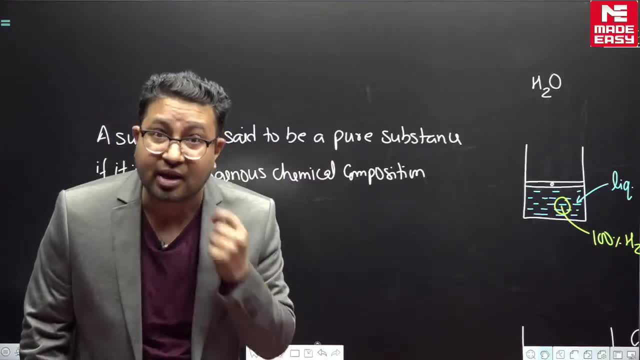 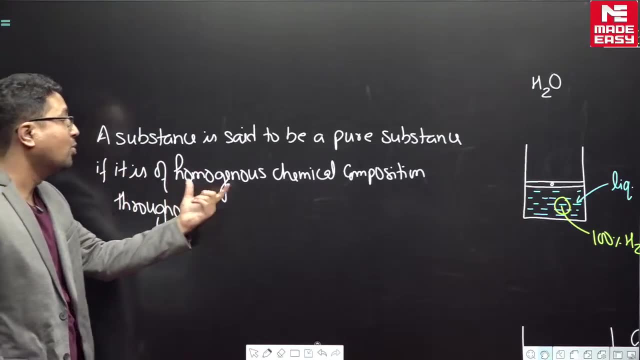 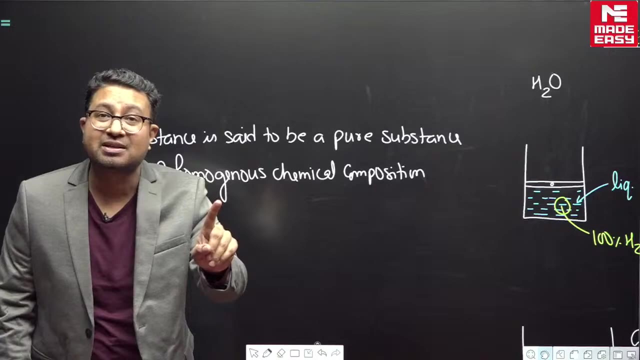 We can consider it as a single chemical compound and study it. Does this definition tell you A substance is said to be a pure substance if it is of homogenous. Homogenous means the same, Not in every aspect. Not in every aspect. 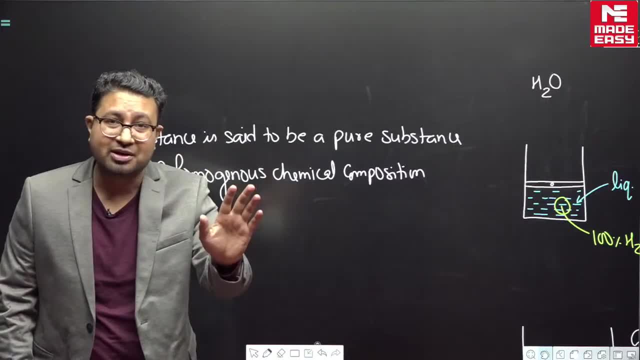 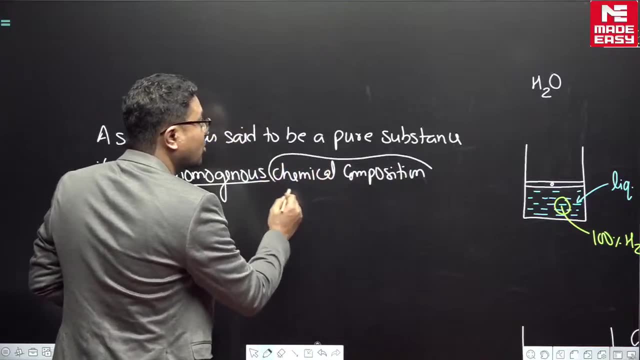 Not in every aspect. Density should not be same, Density should not be same. It is not said like this: What should be homogenous, In what sense In the chemical composition? Homogeneity in what aspect? In which aspect In the chemical composition. 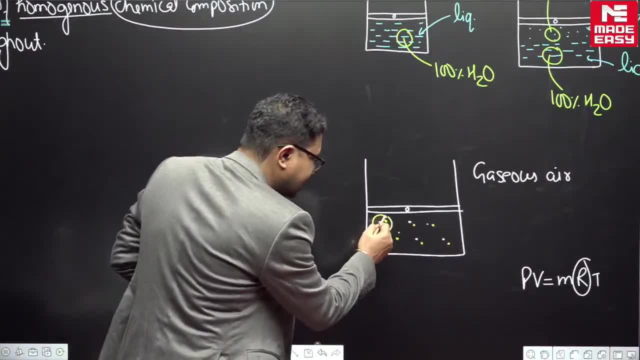 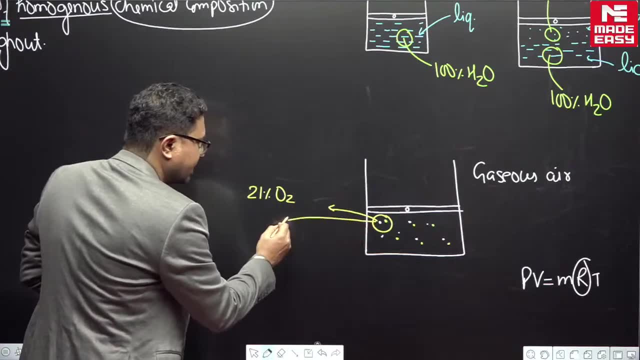 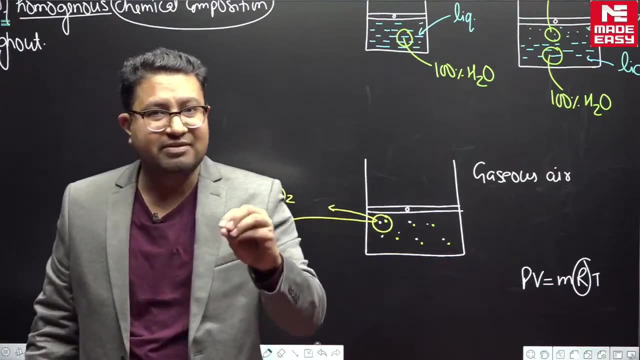 What does it mean to say? So if you have mixture here? Suppose, here you have a mixture which is 21% O2.. If it is 21% O2 and 79% N2.. We have 21% O2 and 79% N2.. 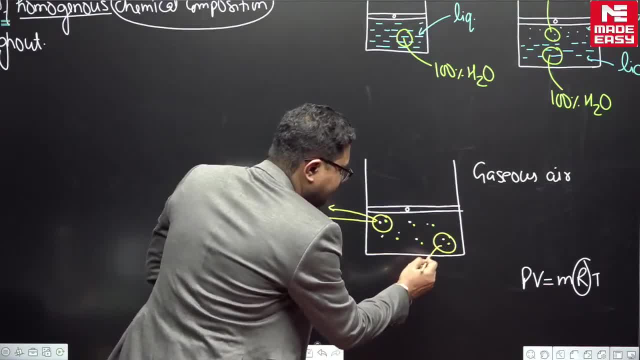 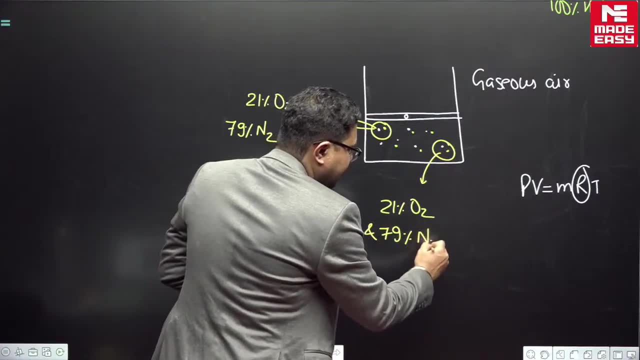 We took a sample from here. So if we take a sample here, If we take a sample from here, We will have same: 21% O2 and 79% N2.. We have same here. So if the mixture is in the gaseous form, 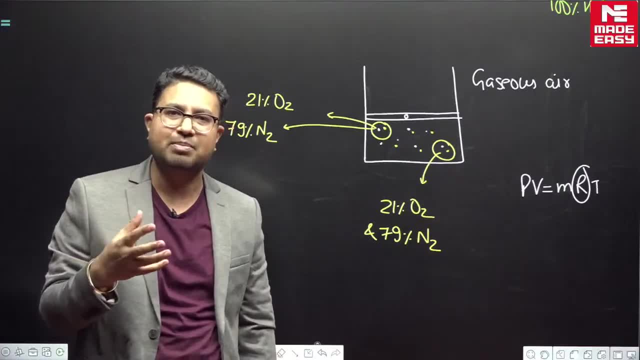 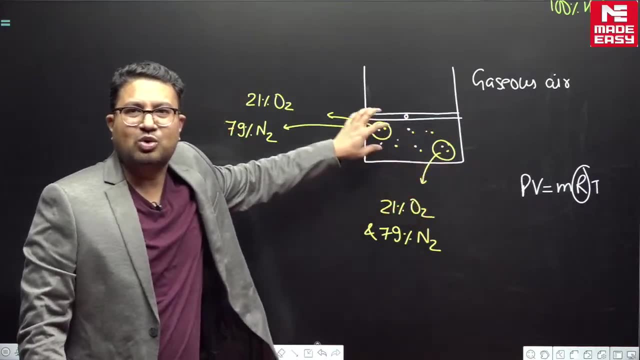 No matter wherever you take the sample from. You can take the sample from anywhere. No matter wherever you take the sample from, If the percentage in the mixture is same, Suppose major components are O2 and N2.. There are CO2 also. 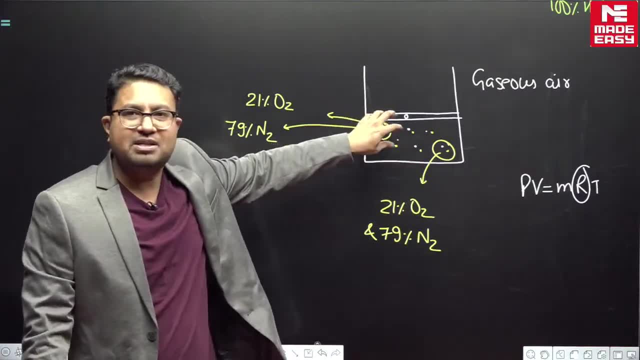 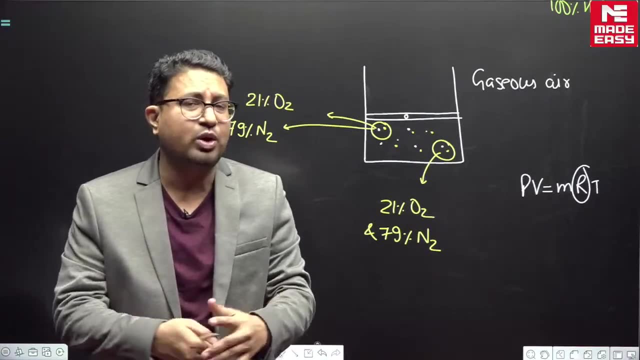 There is vapor of H2O also If the percentage composition is same. So whatever study you are doing, Whatever study you are doing, Whatever study you are doing, You may be able to treat them. You can consider it as one component and study it. 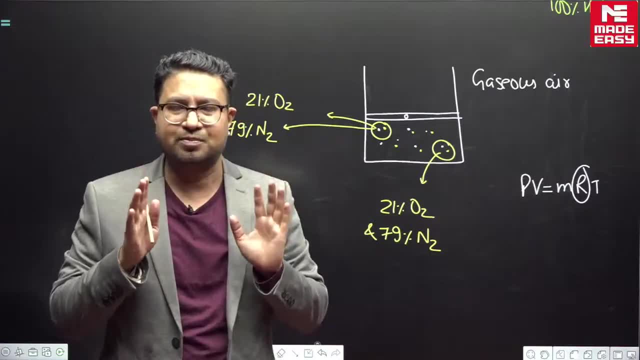 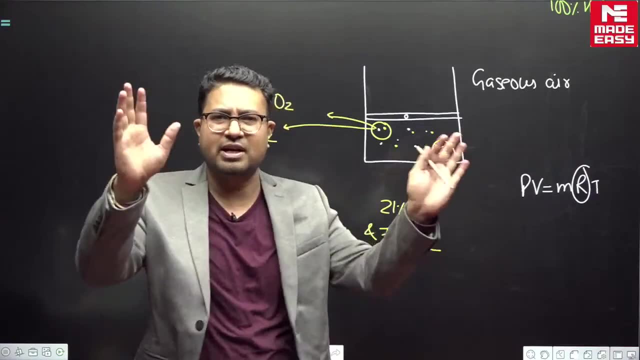 Even though it is not a single component, But you can study it. So definition of pure substance. If you see basic, It means a single chemical compound. But no matter, it can exist in many phases. It should be a single chemical compound. 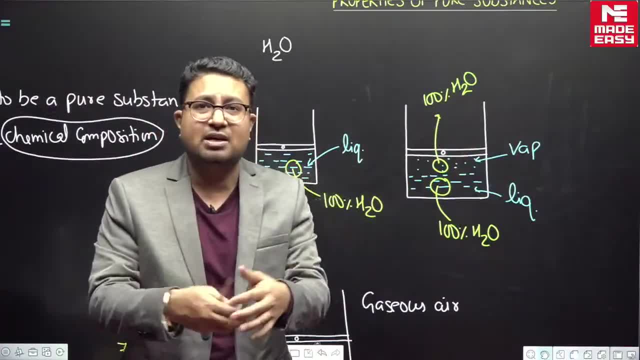 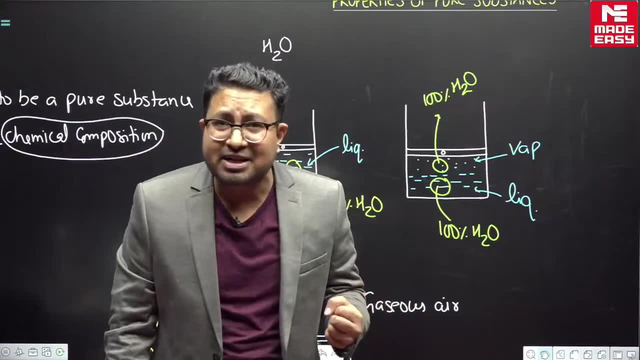 It can exist in many phases. But if we have to decide, If we have to decide whether it is a single component or not, It is not a single component, But still, I don't want to complicate my study. I don't want to complicate my study. 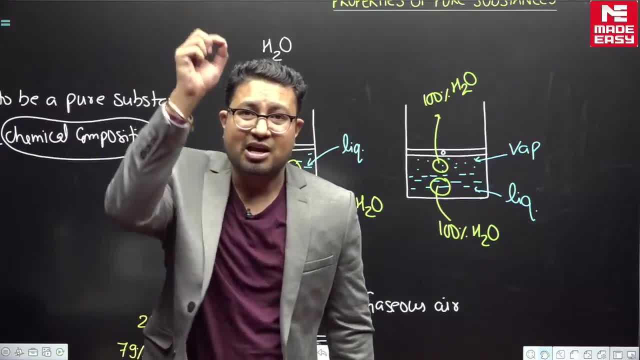 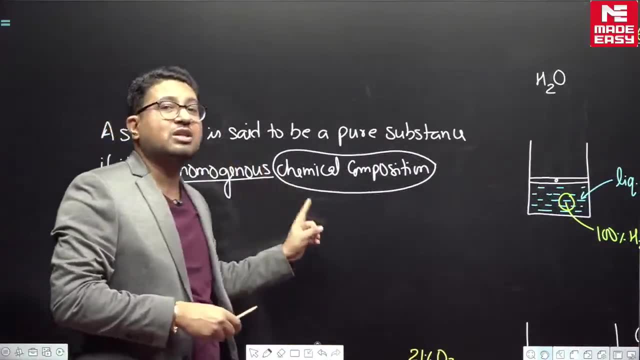 I don't want to complicate my study- Then, If it is possible, If it satisfies this, If it satisfies, Even if it is not a single component, Even if it is not a single component, We can treat it as one component and study. 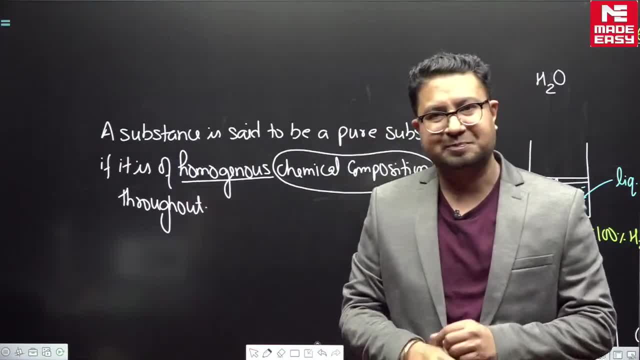 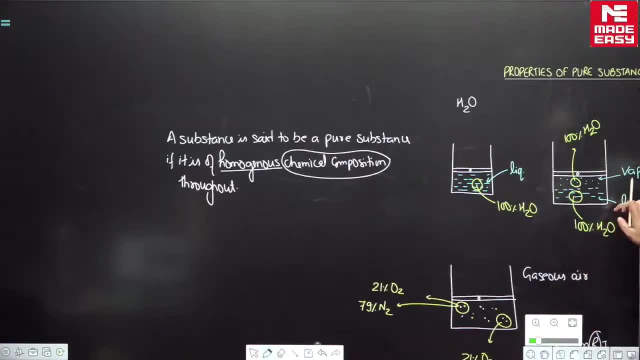 We can treat it as one component and study. This is about the pure substance. This is about the pure substance. This is about the pure substance Which I just discussed. So, basically, here what we are going to discuss, We are going to discuss properties. 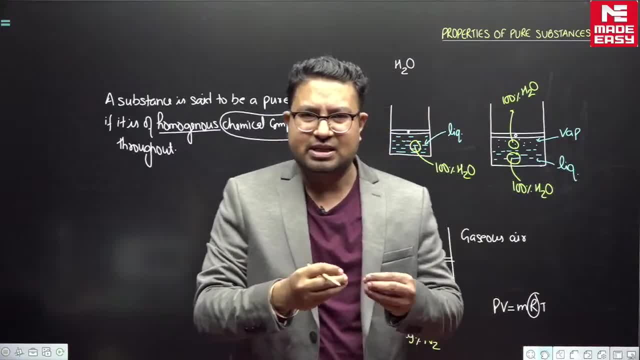 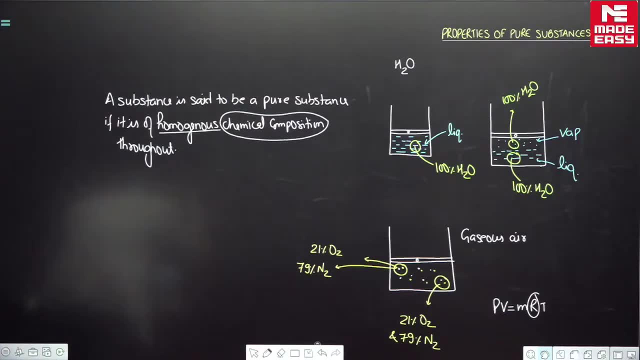 We are going to discuss the properties. So there is a just brief information I gave you. So there is a just brief information I gave you. I gave you a brief information. I will just move aside Any people who want to Just take a screenshot. 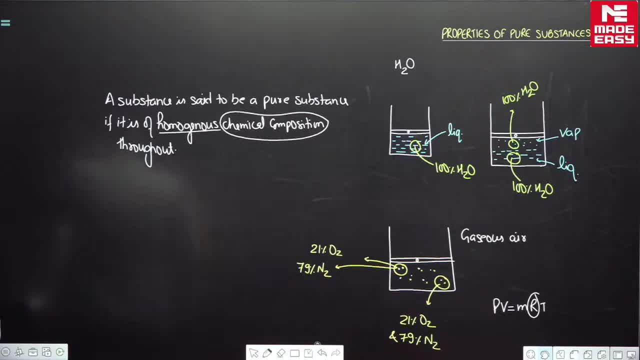 Any people who want to, I will just move aside. I will just move aside. Fine, so Language in English. I will always keep. I will always keep. Don't worry, Our language will be Hindi and English. Our language will be Hindi and English. 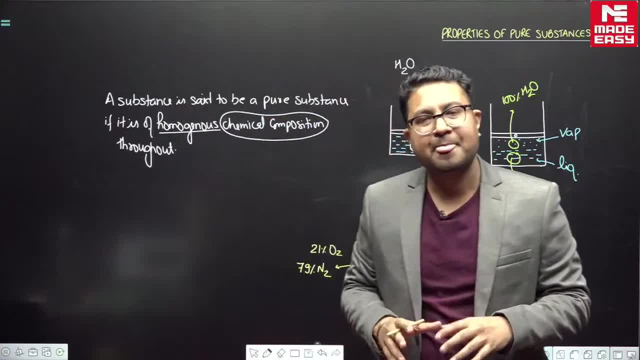 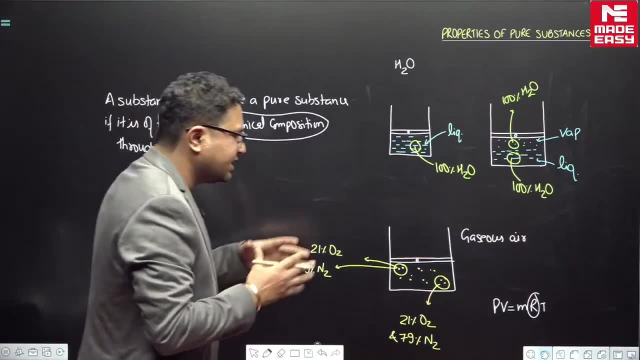 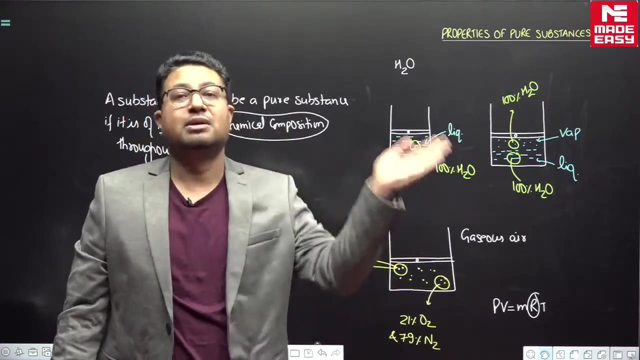 So Now, fine, Now what? What further We will be discussing? We will be discussing: We take something As a pure substance If it is a single chemical compound, But we may treat a mixture So as a single chemical compound. 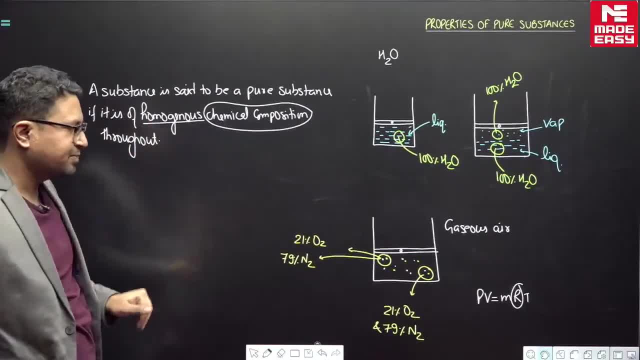 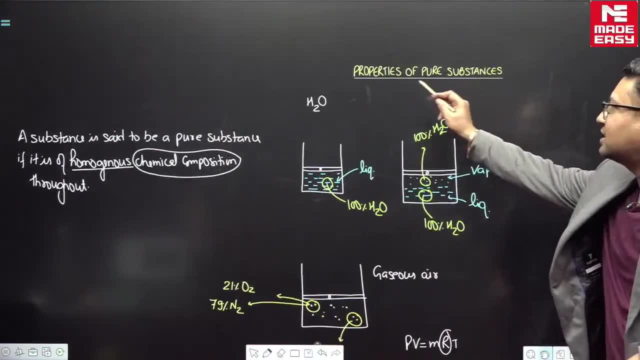 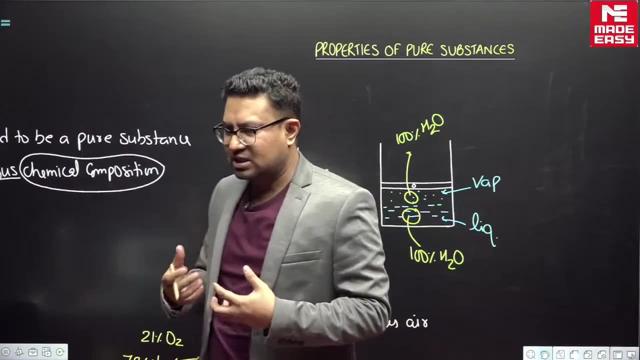 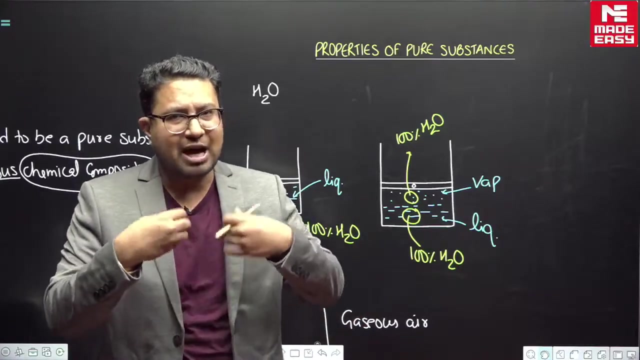 And study. But here today Our discussion Is about the properties Of pure substance, That is, the properties Of pure substance. So let us try to Understand the various Things, properties of the pure substances- and we will also see its application related to it, We will see how. 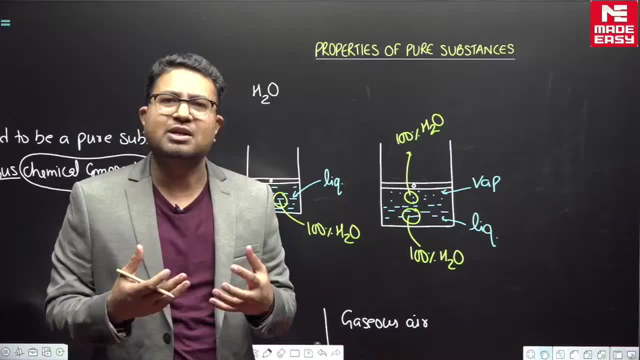 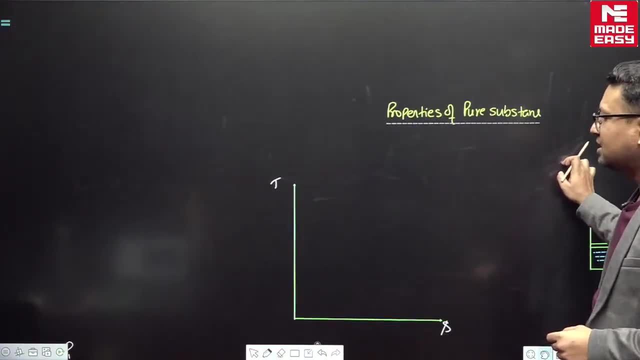 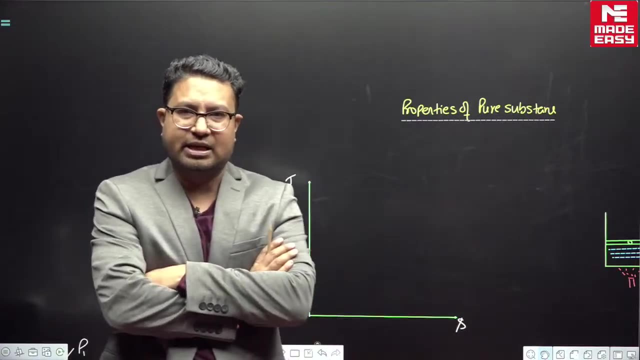 we can apply the understanding. How can we apply what we understand? So, first of all, I will discuss a diagram, that is the TS diagram. First of all, I will discuss a diagram whose name is TS diagram. Our main discussion is starting from here. That was a brief introduction which I gave. 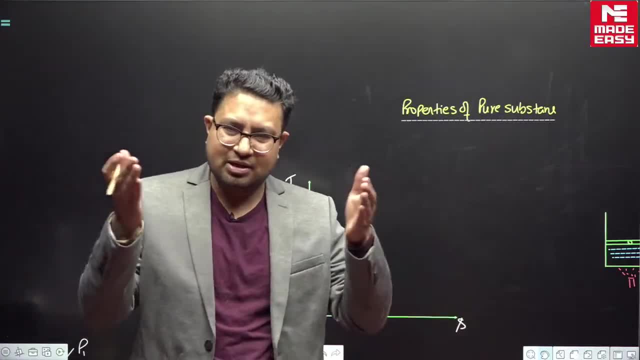 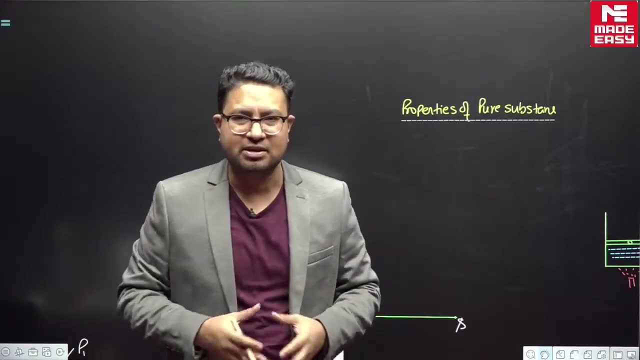 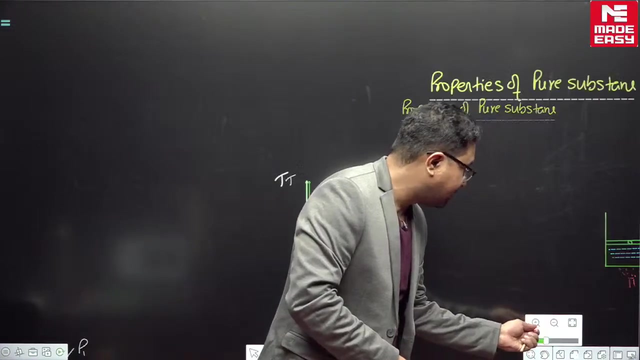 you, Anybody who has joined just now, just for your information. the main discussion is starting from here, whatever we are going to discuss now. So we are going to discuss the properties of the pure substance. We are talking about the properties of pure substance, Even if there are 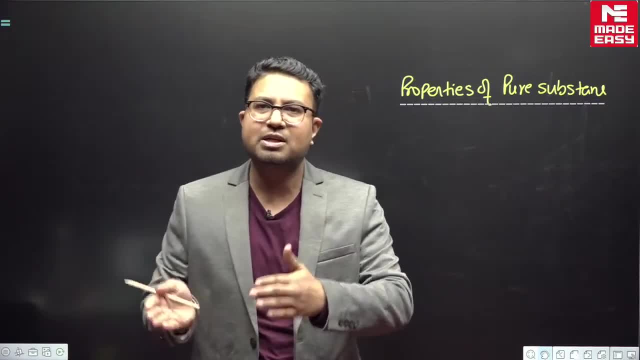 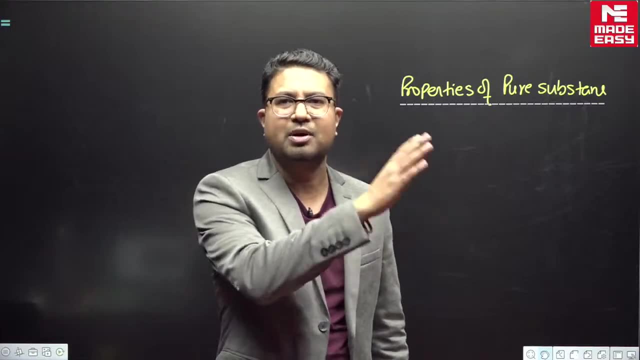 many things you may not have studied in detail, if you have not studied thermodynamics in detail. even if you have not studied thermodynamics in detail, if you start watching from here, you will be able to continue. There may be one or few things which you will have. 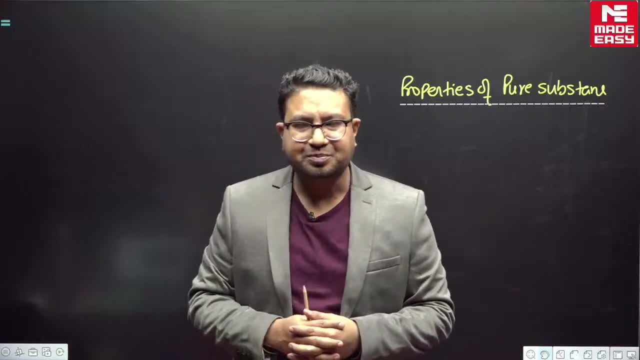 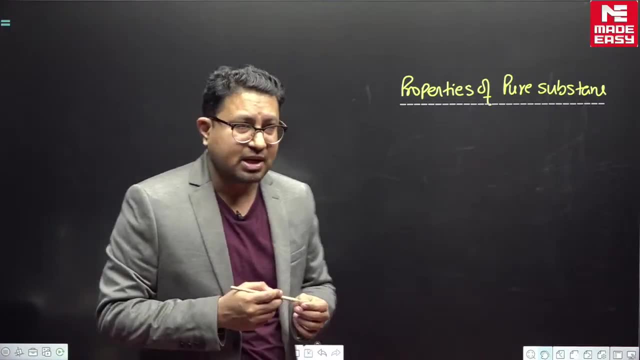 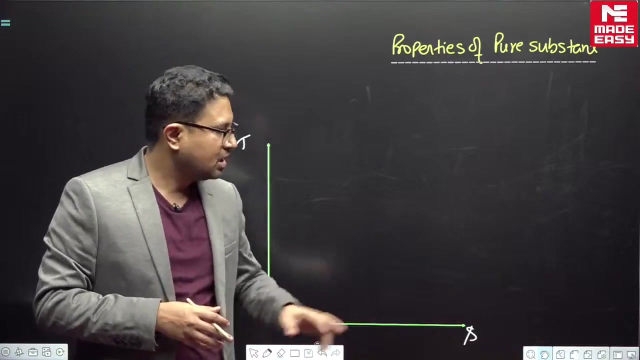 to understand. just otherwise we will be able to continue. Now I want to discuss the TS diagram. I want to make a diagram of temperature entropy and I will take water as the substance. I will take water as the substance. Fine, So here I have shown. 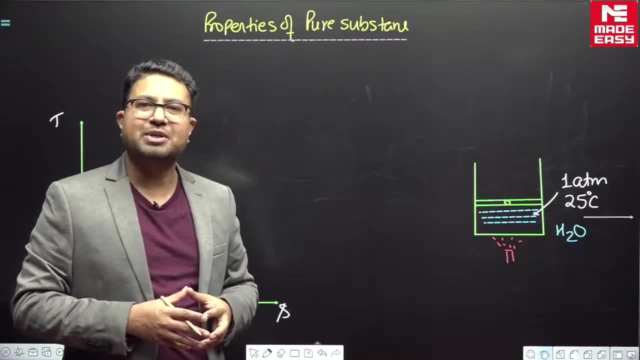 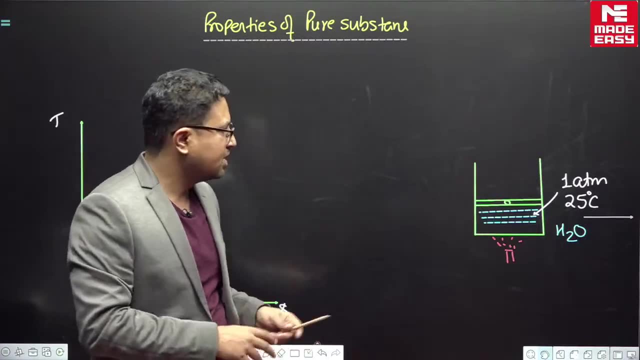 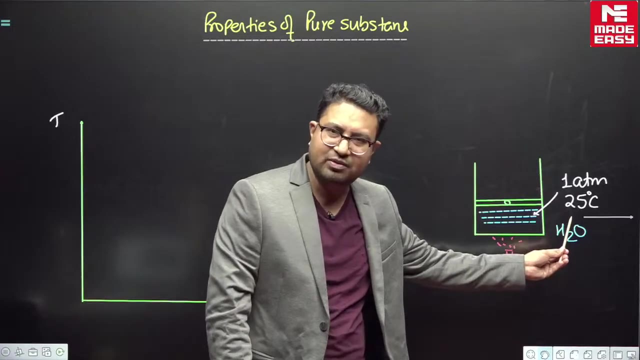 I have shown a piston cylinder arrangement. I have shown a piston cylinder arrangement. Piston cylinder arrangement contains water. There is water in it. The water is at one atmosphere. The water is at one atmosphere. 25 degree Celsius is the temperature of the water and I am going to. 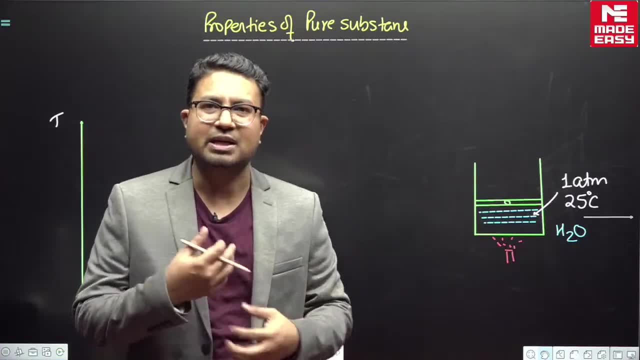 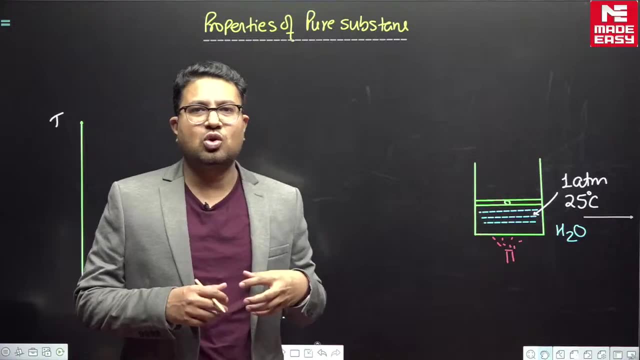 heat it. I am going to heat it. I will be heating it. In the piston cylinder arrangement. piston is free for movement, The piston is free to move, so I will assume the pressure will remain constant. I will assume that the pressure will remain constant. 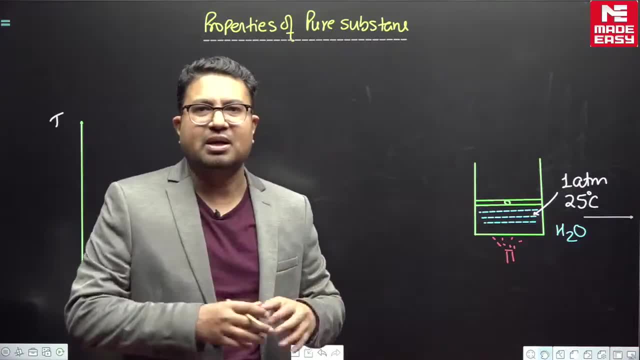 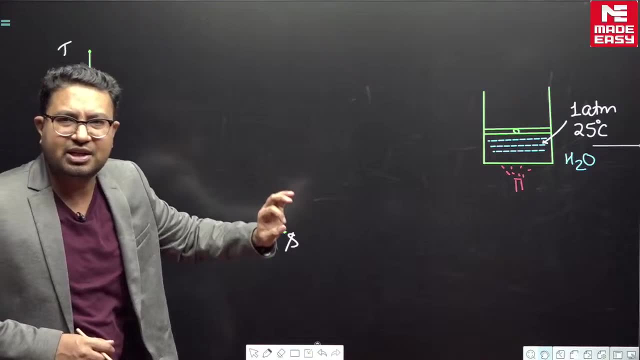 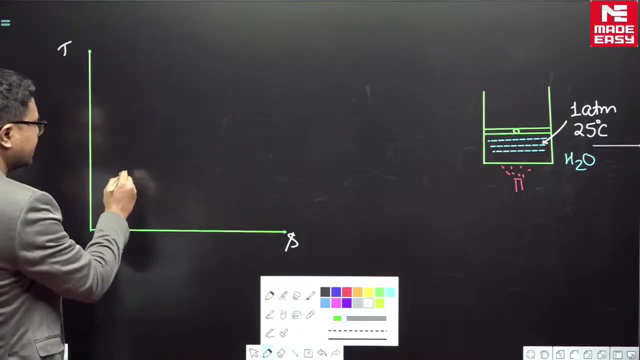 so, on constant pressure, we are heating the water. so, at its initial condition, according to its initial condition: 1 atmosphere and 25 degree Celsius. according to that it is having some temperature. so let us say this is the value of the temperature and accordingly it will have some entropy. 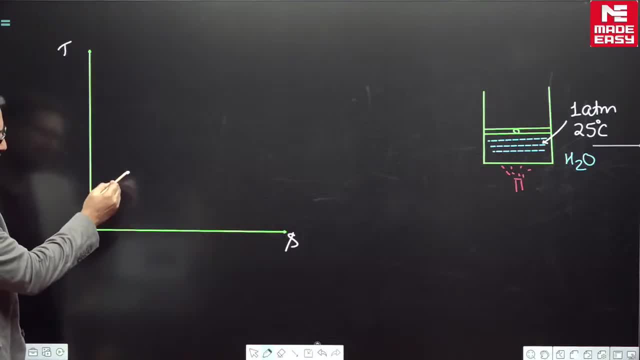 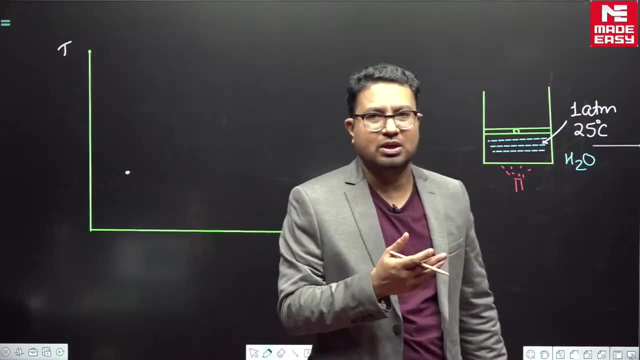 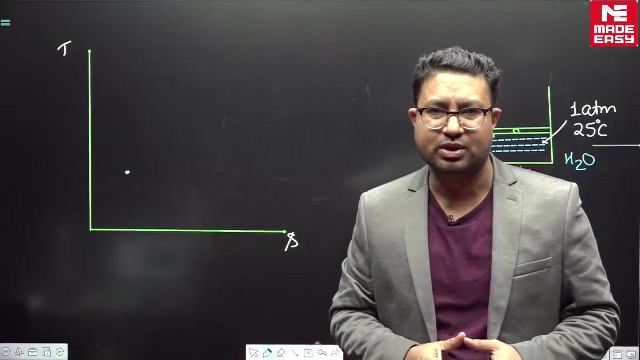 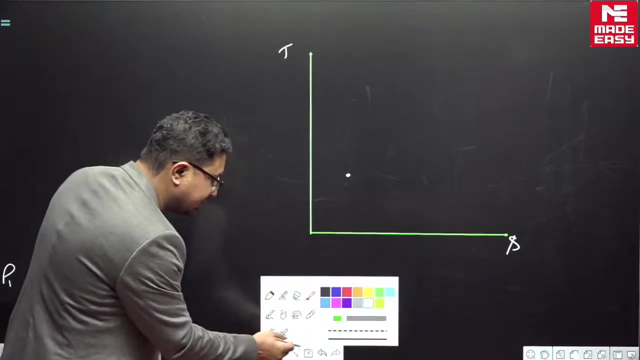 so I have located the point here. I have located the point here. now I will supply heat. as the heat will be supplied, pressure will remain constant. constant pressure heating process is happening now. constant pressure curve: how it looks on the TS diagram. how the curve of constant pressure looks on the TS diagram. 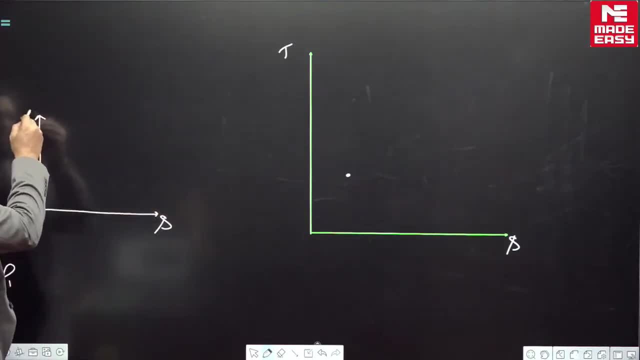 see as the curve of constant pressure looks on the TS diagram. If we see the constant pressure curve on the TS diagram, suppose, starting from a single point, if we start from a single point and we draw two curves, one curve is constant volume and one curve is constant pressure, 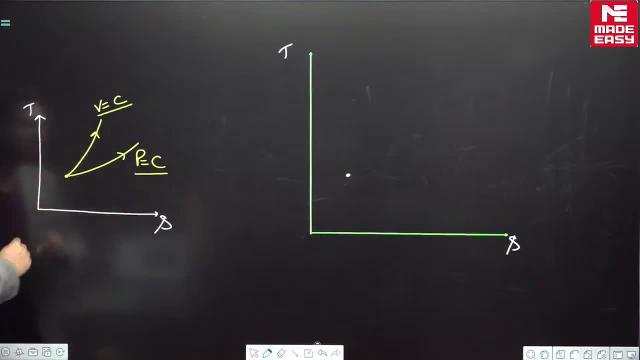 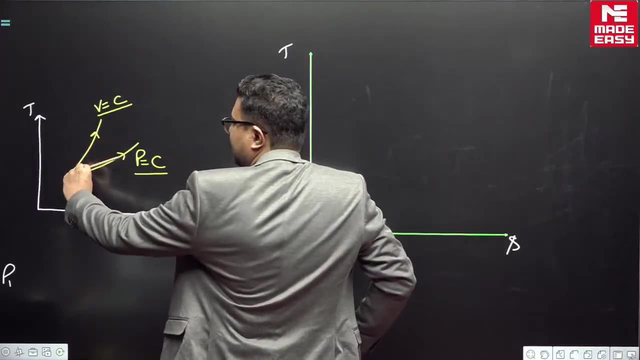 One curve is constant volume and one curve is constant pressure. So the constant pressure curve will be that curve which is less steep. It is less steep. it is such a curve that you will heat on constant pressure. temperature will also increase. temperature will also increase. entropy will also increase the 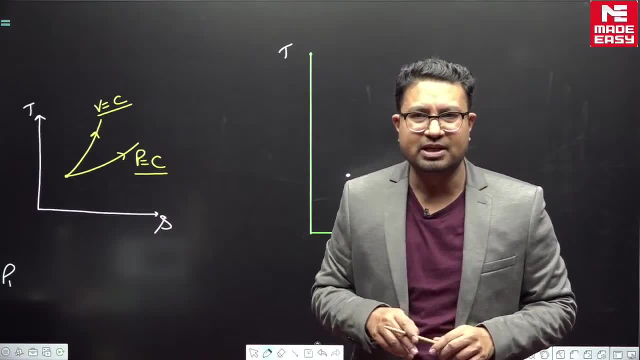 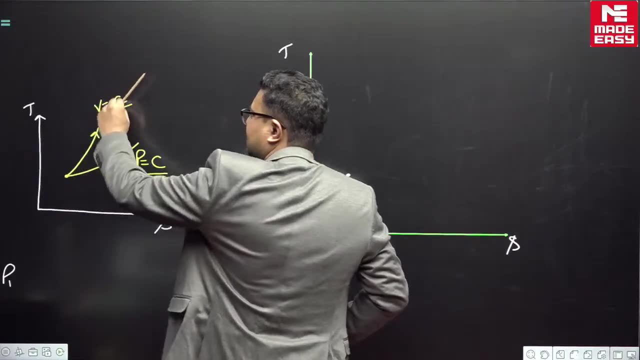 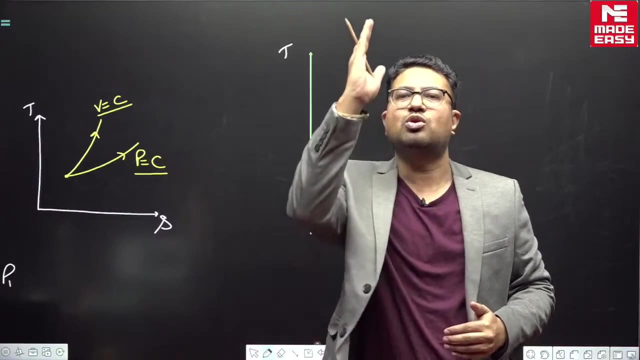 entropy will increase, temperature will increase. entropy will increase, but the constant pressure curve is less steep. it is less steep compared to constant volume curve. Constant volume curve is more steep compared to constant pressure curve. Constant volume curve is more steep. more steep means more closer to being vertical. 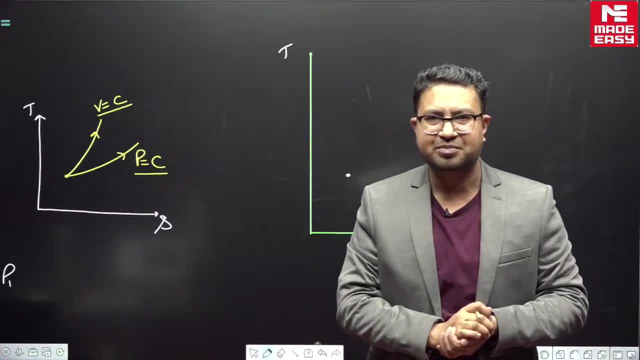 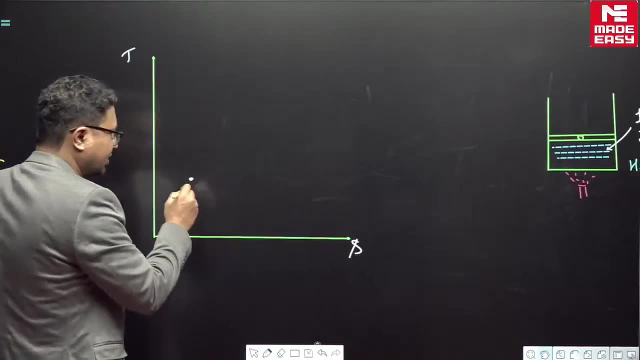 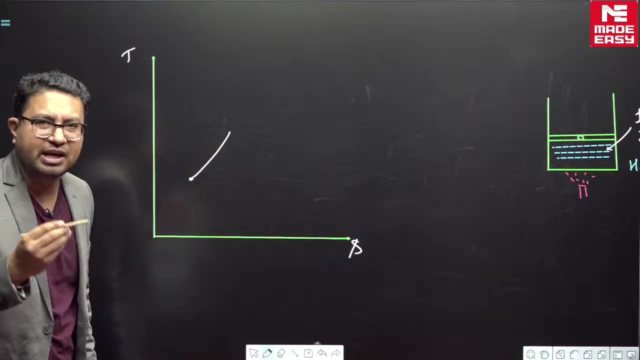 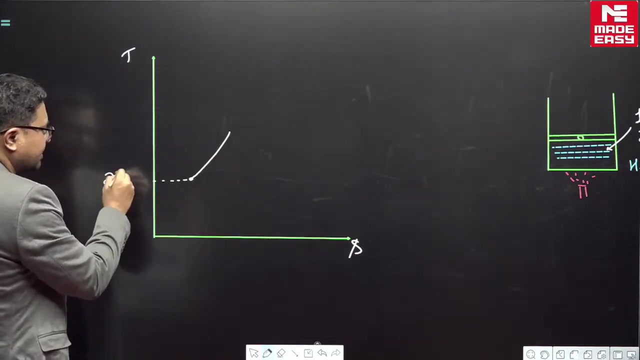 it is more closer to being vertical. So when I will heat this water, the temperature will increase, the entropy will increase. Temperature will increase. entropy will increase. Initial temperature was 25 degree Celsius. Initial temperature was 25 degree Celsius. 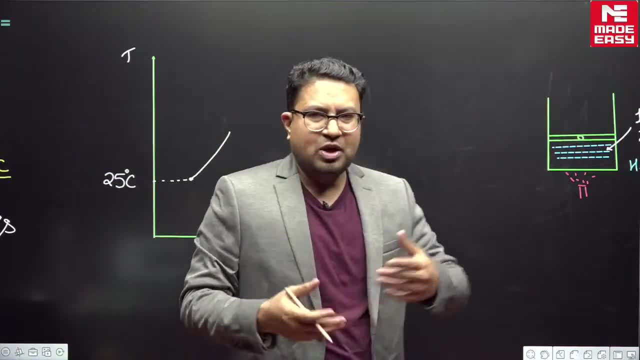 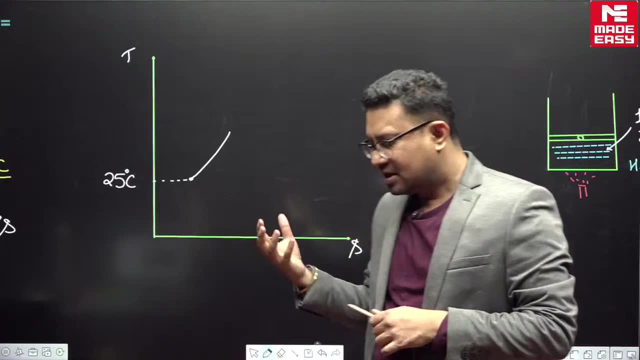 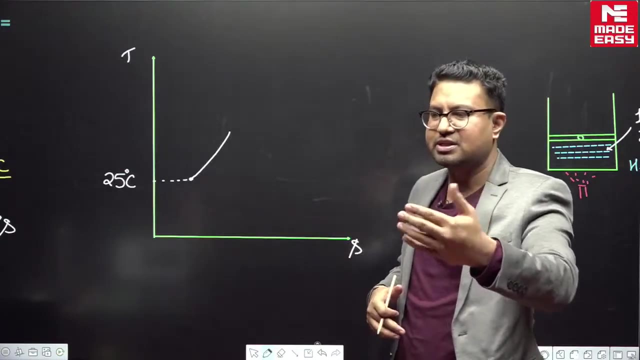 This was the initial temperature. So we observed. Suppose you have put a sensor inside and that sensor is giving you the data as you are going on. heating temperature is increasing. temperature is increasing. pressure is constant because piston cylinder arrangement is here and the piston is free to move piston movement. 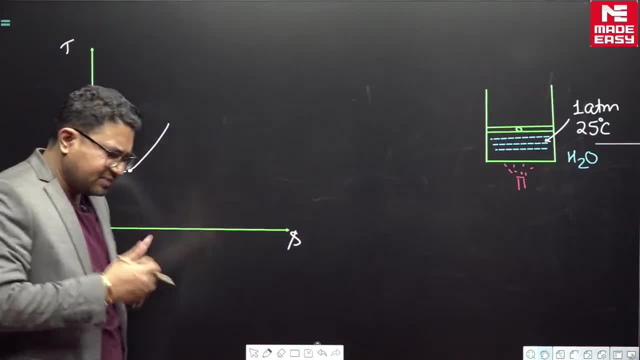 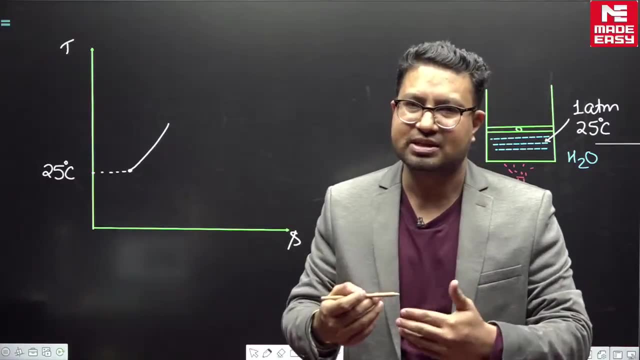 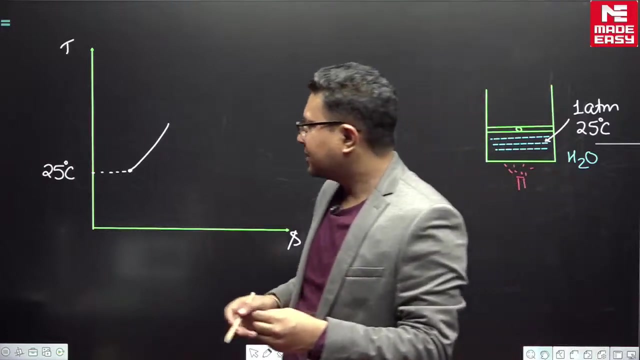 is free, pressure is constant. So, as we continue heating, as we continue heating after some time, after some time, temperature reaches 100 degree Celsius. temperature reaches 100 degree Celsius. I am conducting an experiment. I am conducting an experiment. temperature reaches 100 degree Celsius. 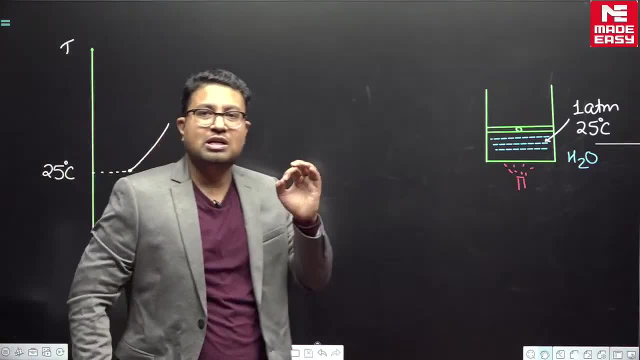 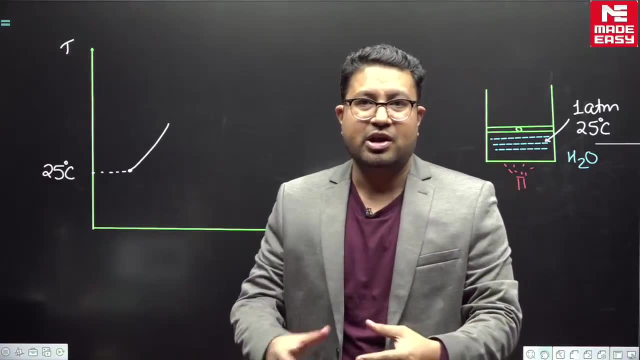 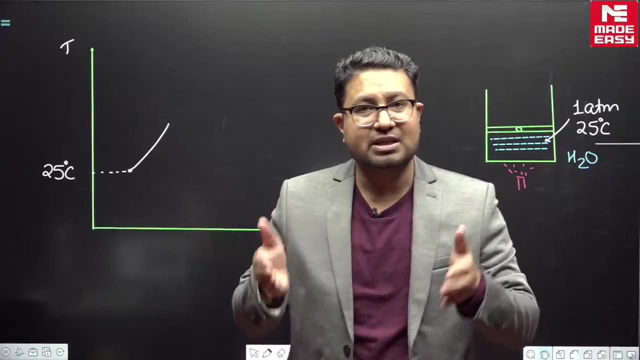 So this is the observation. see, understand this. there is no reason for properties. we try to know what are the properties. Now, water boils at 100 degree Celsius. one atmosphere boils. you cannot explain it logically. this is the property. this is how the substance is. 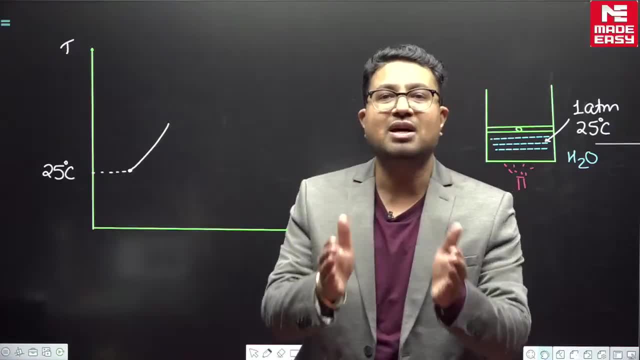 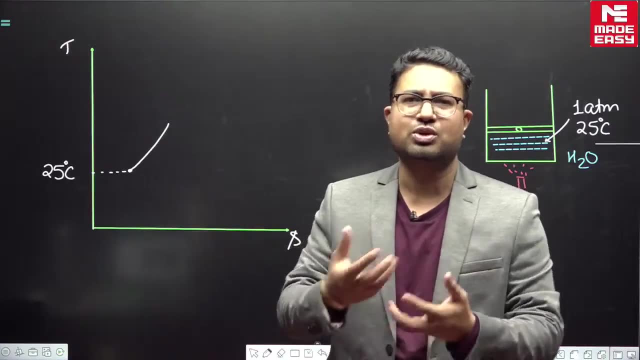 We have not made it. we have not made it. this is how the substance is. we are trying to understand. we are just trying to understand. we are trying to know. we are just trying to know about it, we are trying to know about it. we have not made it like this it was. 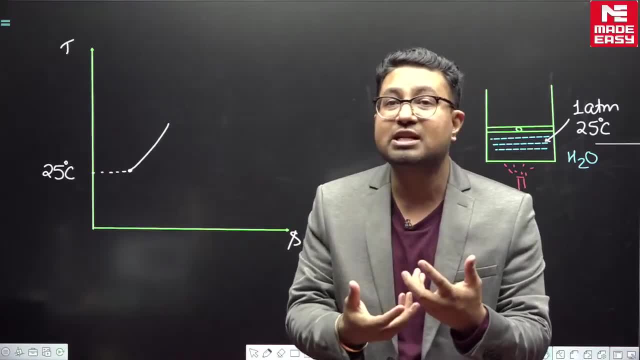 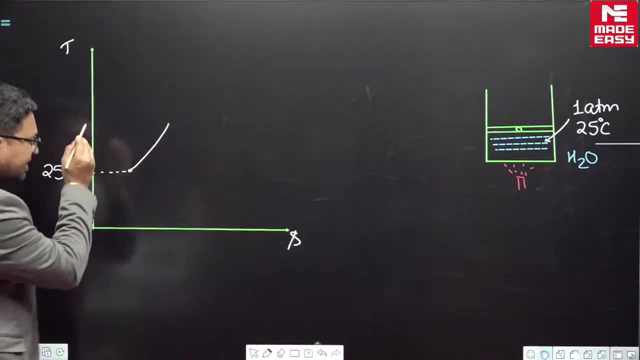 already like this. it was already like this. we are just trying to understand its properties so that we can use it for our benefit. So we are doing an experiment. so now here we started heating at 25 degree Celsius. temperature is increasing, pressure is constant. 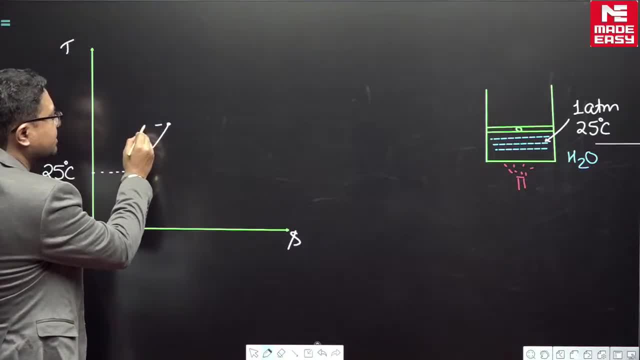 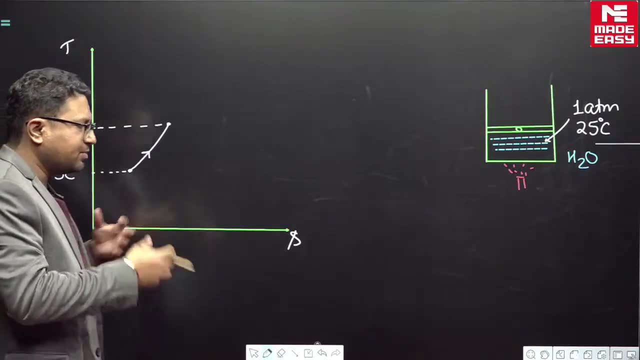 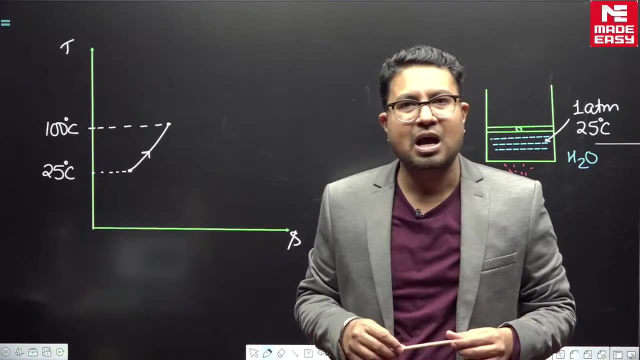 What we have noticed here: when we reach 100 degree Celsius, when we reached 100 degree range, we reached 100 degree Celsius. When we reached 100 degree Celsius, we noticed, we noticed that the temperature has stopped increasing. Temperature has stopped increasing. now, temperature has stopped increasing. but what we observed? 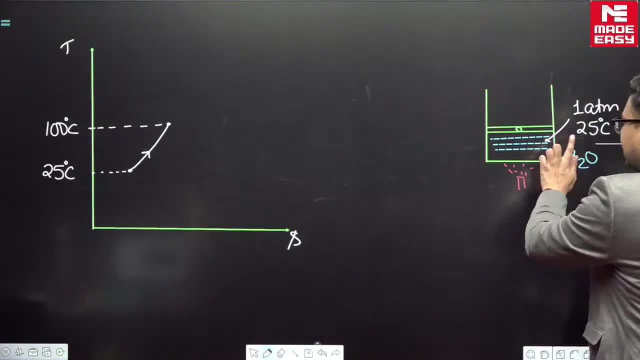 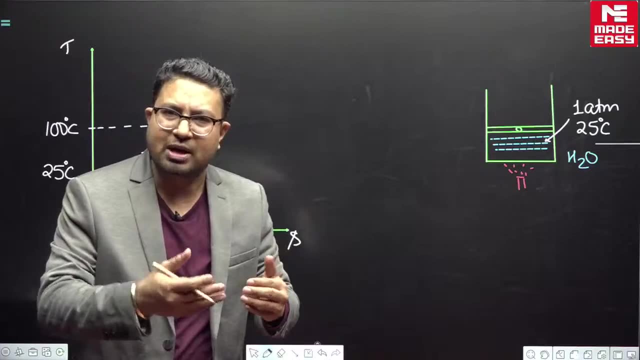 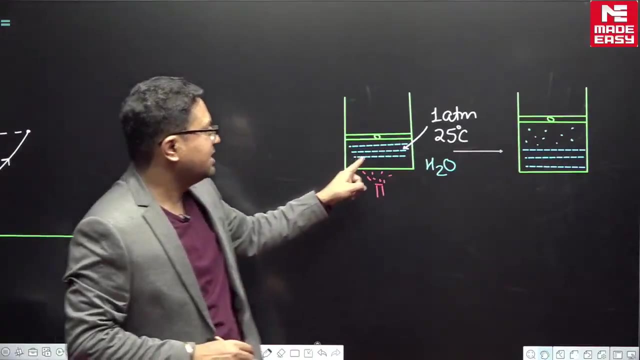 what we observed. suppose this is a transparent cylinder. suppose it is transparent cylinder. you heat it. Here we used constant heat. We had kept constant balance. temperature change is stopped, but heat supply is continuing. heat supply is continuing. you observed inside the cylinder. you observed that some of the h2o is becoming vapor. 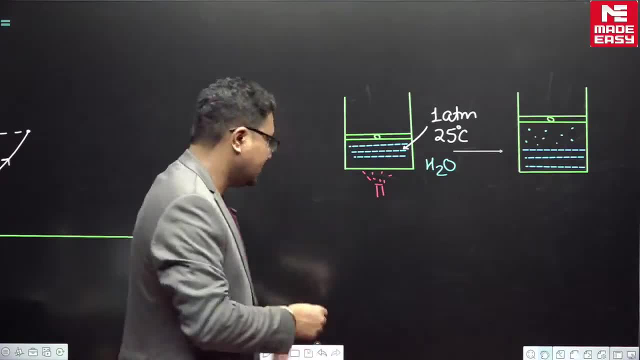 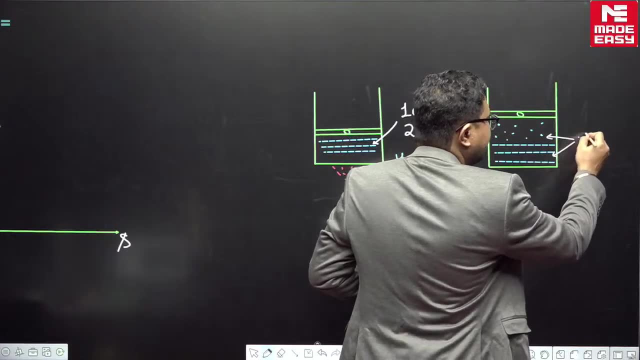 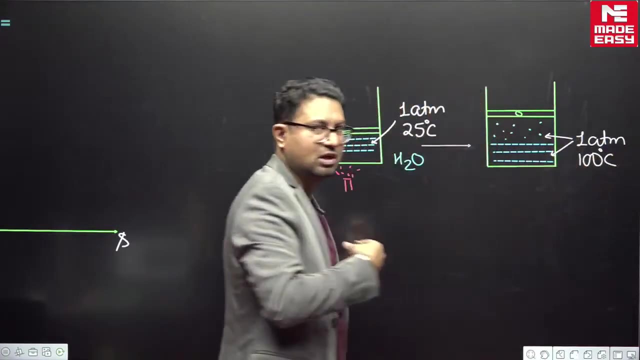 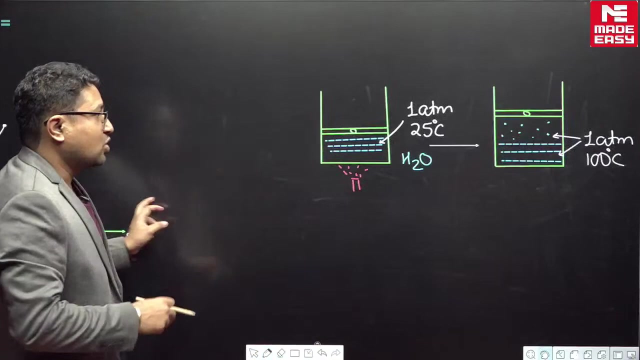 so there is vapor also. there is vapor also, and when this happened, this happened: pressure is constant, one atmosphere and temperature reached 100 degree celsius. we observed this, that this happened when the temperature reached 100 degree celsius. then we saw, once the temperature reached 100 degree celsius, 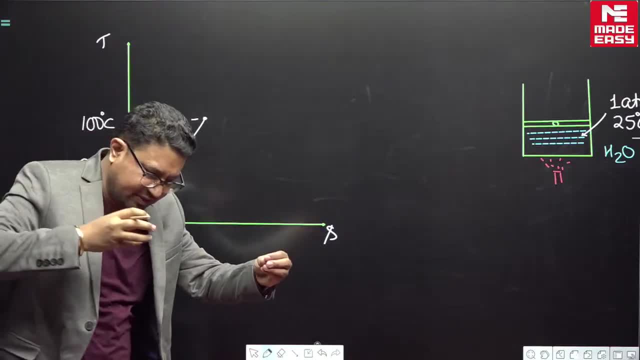 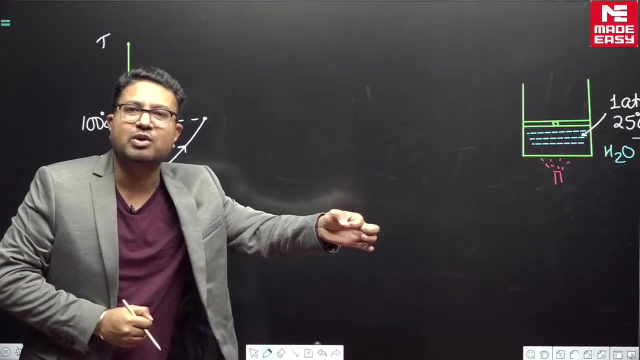 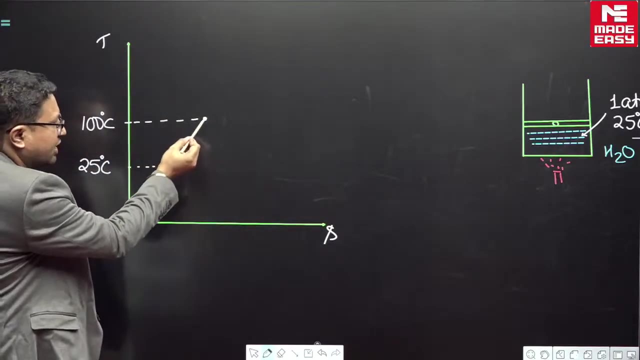 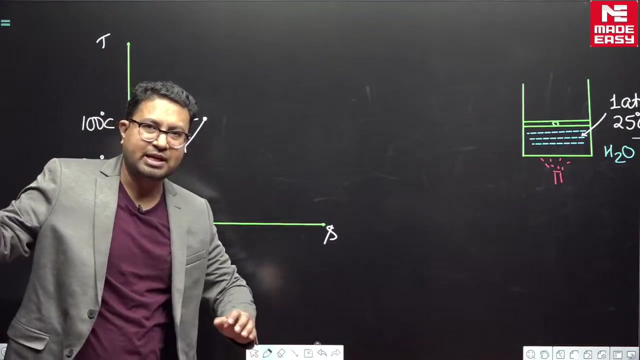 then whatever heat we are supplying, corresponding to that, there is some mass which is converting from liquid to vapor. so, whatever is the liquid, the liquid is, whatever is the liquid, it is having this entropy. but when it is absorbing heat, when it is converting into vapor, when it is converting into vapor, 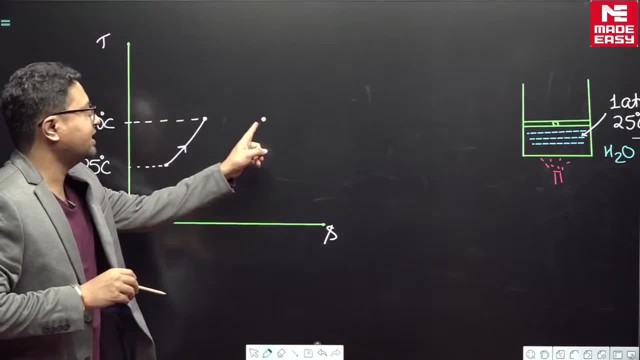 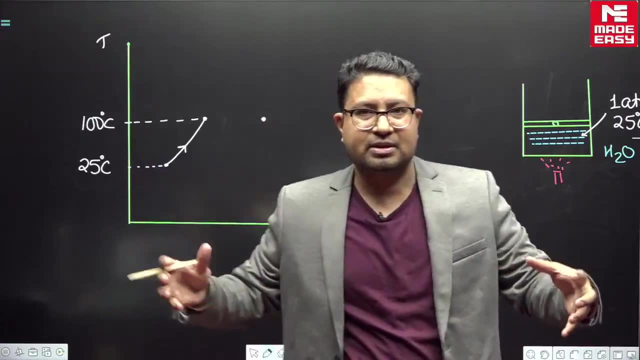 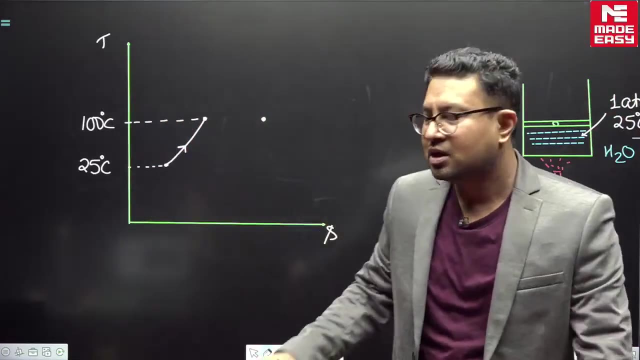 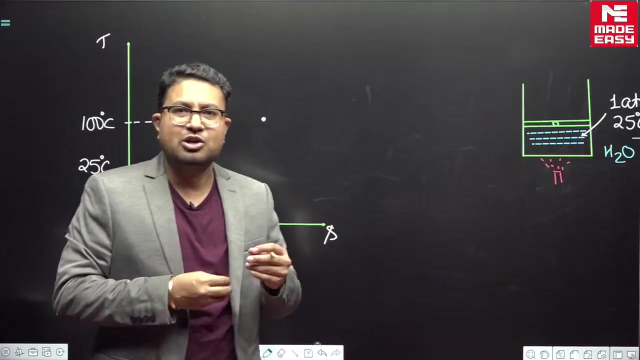 let us say it is having this entropy, the temperature is same, but the volume increases. the same mass gets scattered in a larger space. so now, but initially let us say 1 kg liquid. you supplied some heat. 100 degree Celsius, you supplied some heat out of 1 kg. 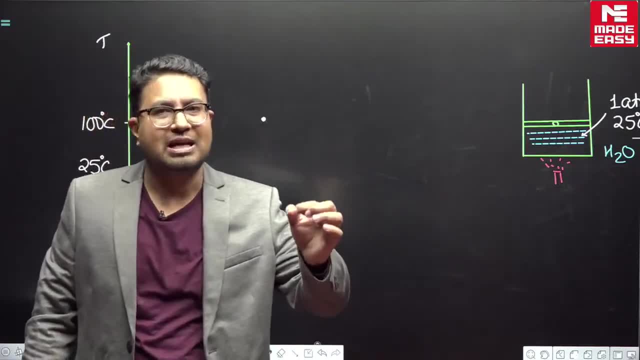 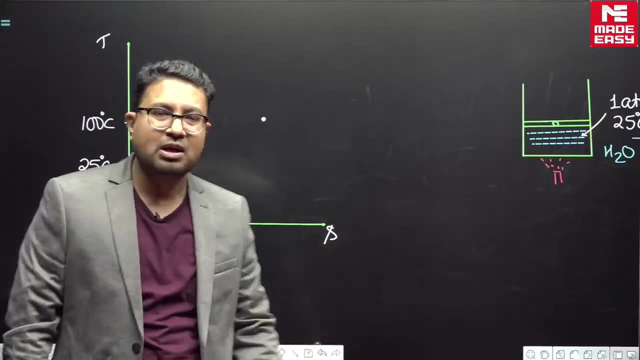 let us say, out of 1 kg, let us say 0.1 kg converted into vapor, 0.1 kg converted into vapor and 0.1 kg converted into vapor, and 0.1 kg converted into vapor and 0.9 kg, which is 0.9 kg, it is still liquid. 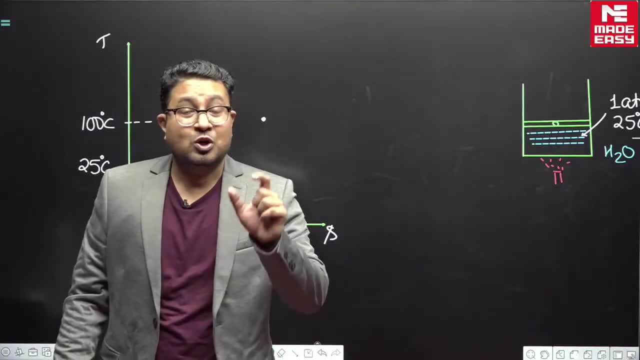 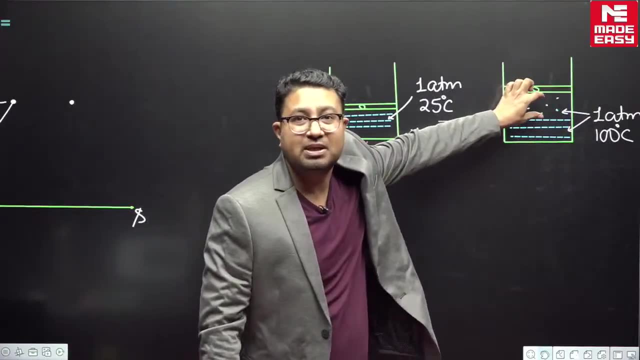 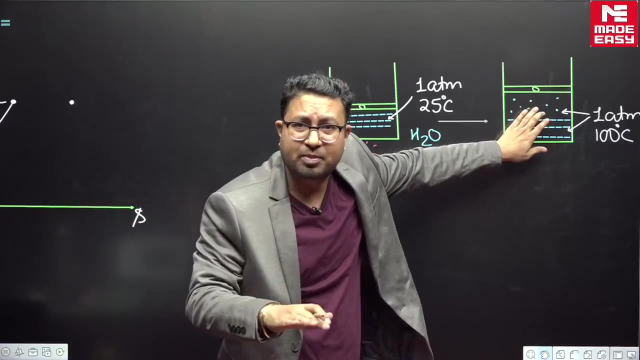 0.9 kg is still liquid. so you will see that the average property average because you have some vapor. vapor is having high entropy. it has absorbed heat during its conversion. heat is absorbed during conversion. liquid is having lower entropy. so when it has absorbed heat it has converted from liquid to vapor. 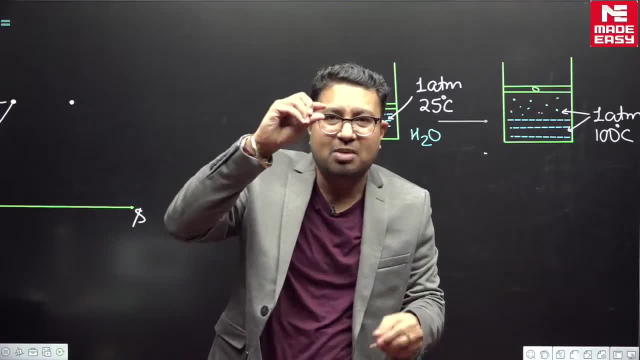 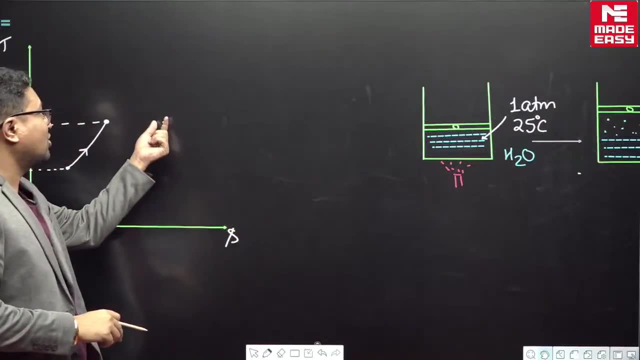 entropy which has increased. so we have a small mass which is having a higher entropy and bigger mass which is having a lower entropy. so entropy of 0.1 kg: is this much? entropy of 0.9 kg: is this much? suppose a class test took place. 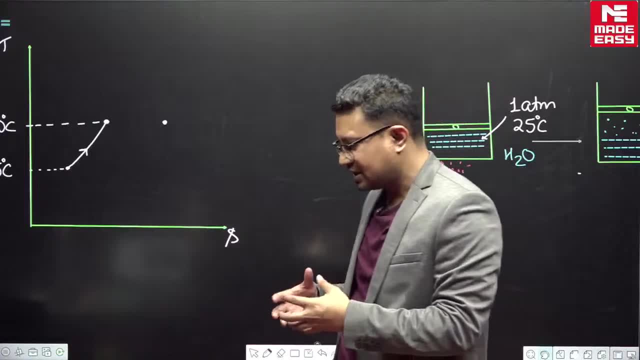 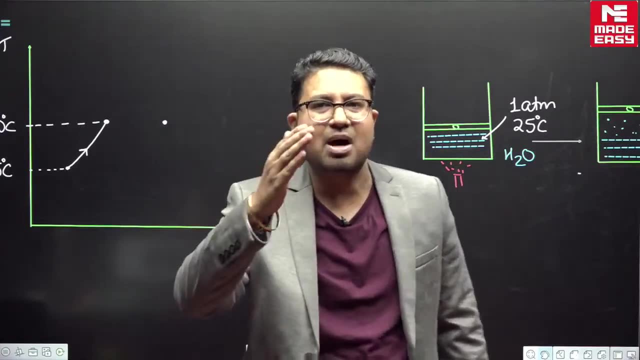 let us say, a class test took place and in that class test, in that class test, there are two types of students, only only two types of students. one of the students got 90 marks out of 100. some people got 90 marks out of 100. 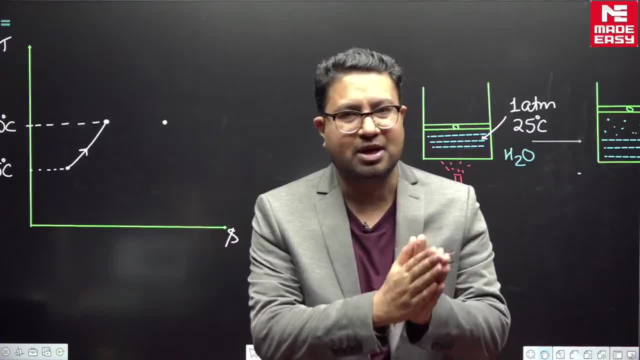 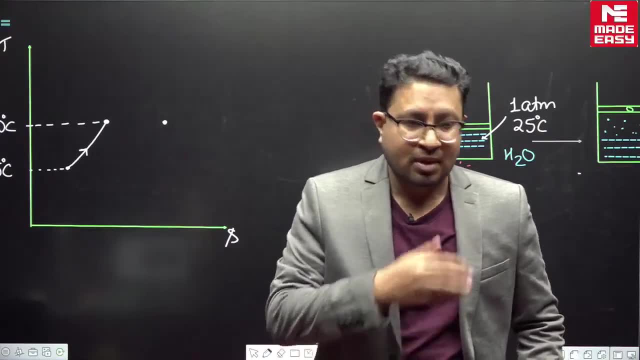 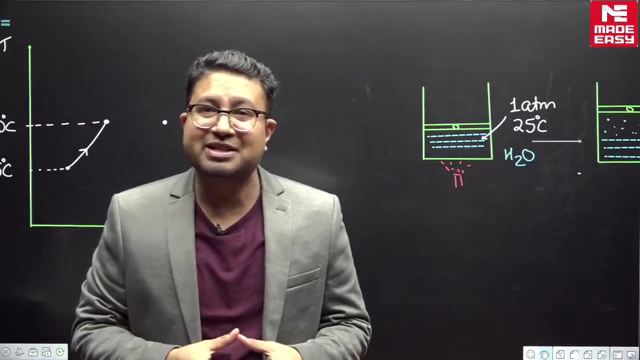 and some of the people got 10 marks out of 100,. some people got 10 marks. Now, if I calculate the average, if I calculate the average and it comes out to be 20,, if I calculate the average and the average comes out to be 20, if the average comes out to be 20, then that means that means. 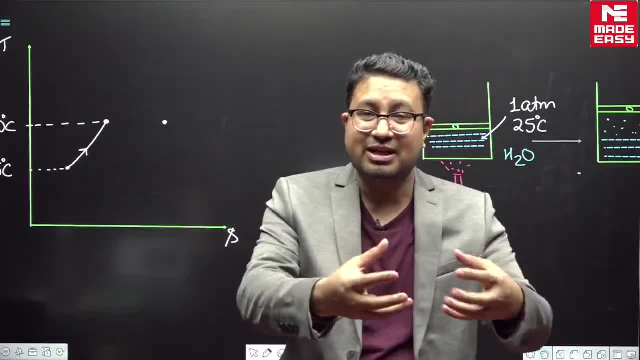 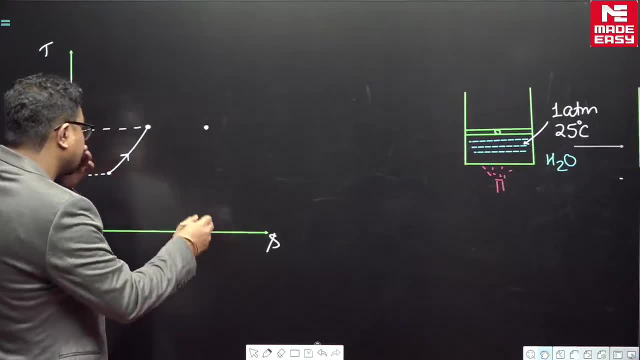 people having 10 marks were higher number whose 10 numbers came. these people were more compared to the people who got 90. So when there is more liquid, when there is more liquid compared to vapour, the average entropy will be. this average entropy will come. So you. 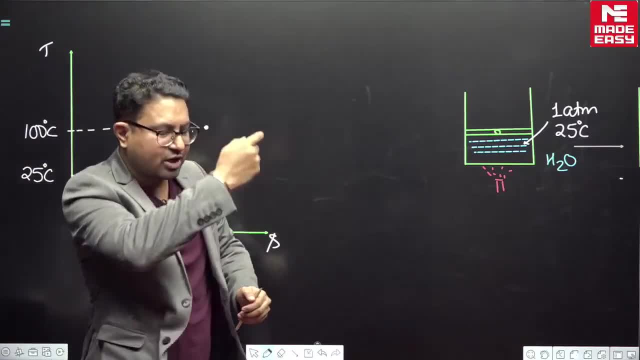 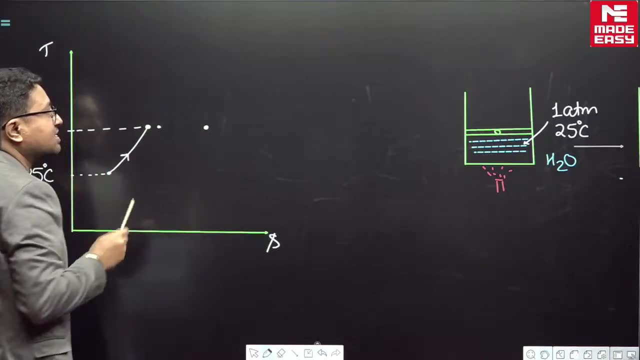 are heating. you are continuing heating. some liquid is continuously converting into vapour, So the mass which is in the vapour state is increasing. vapour state's mass is increasing. liquid state's mass is decreasing. entropy- entropy average average average is increasing. 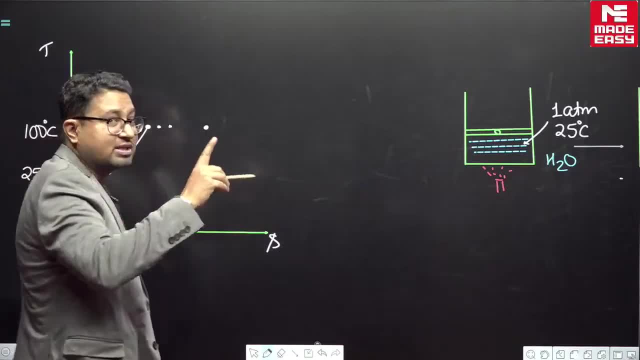 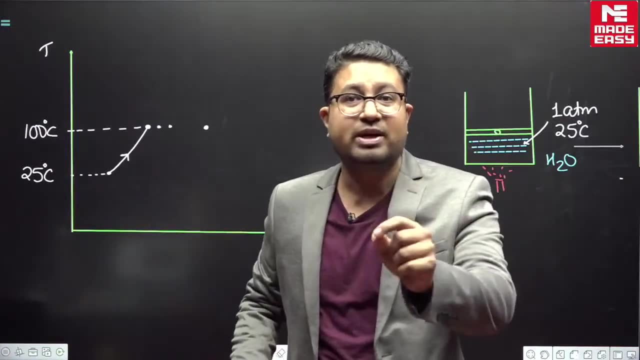 it is increasing. average entropy is increasing. Try to understand. Try to understand this. try to understand this. when a class test was carried out, some people got 10,, some people got 90, average 20 came, but nobody is having 20 marks- nobody. 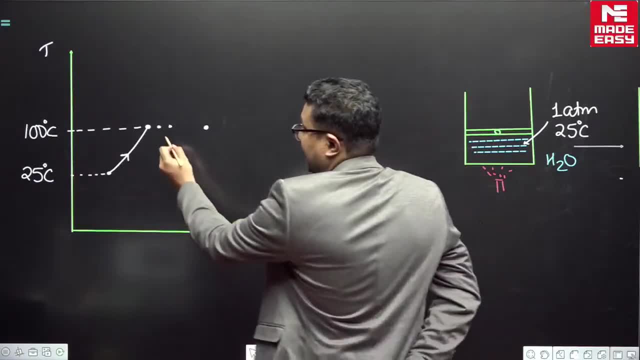 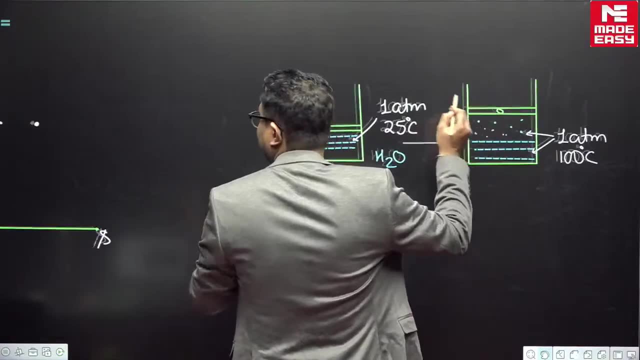 has 20 marks. that is the average. So if I say entropy is this much, if I say entropy is this much, then there is no substance having this entropy. this part, this part, is having this condition and this part is having this condition. it is just the average, it is average. 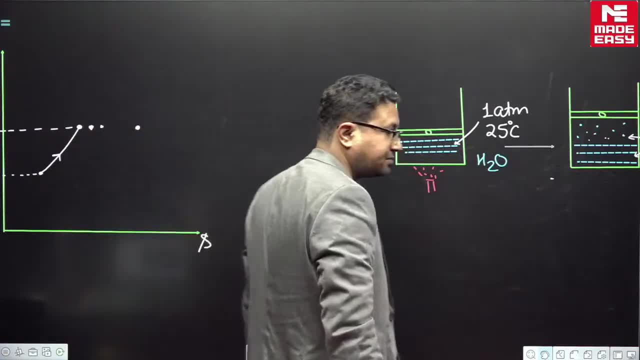 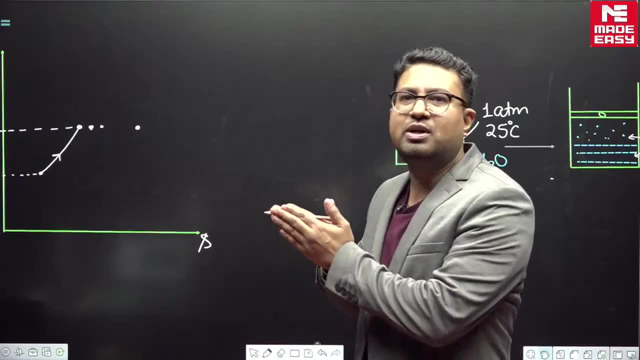 because we have more of this part and less of this part, as the heating is continued just like this. Just like this: the heating is continued. more of the liquid converts into vapour, so average shift towards the vapour. average shifts towards the vapour, so average shifts. 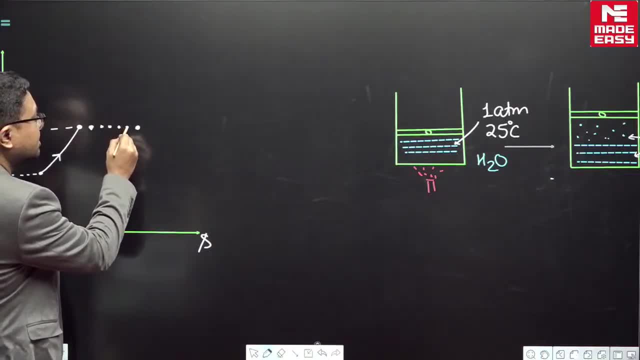 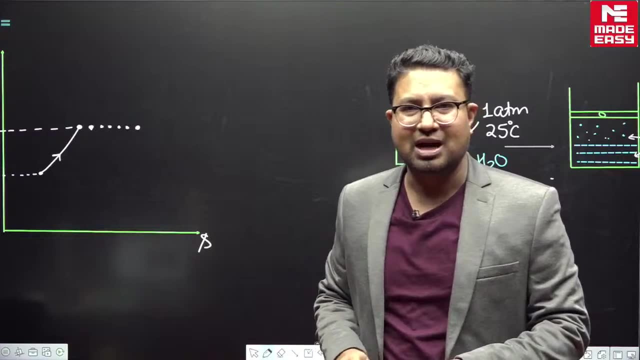 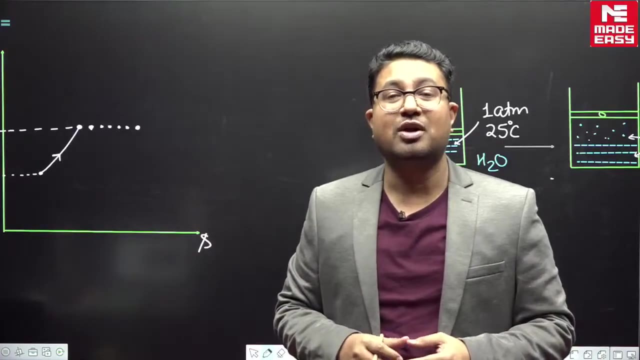 towards the vapour. average shifts towards the vapour. Now suppose, now suppose a class test was carried out. class test was carried out and everybody got 90, all of them got 90 marks, all of them got 90, so if you try to calculate, 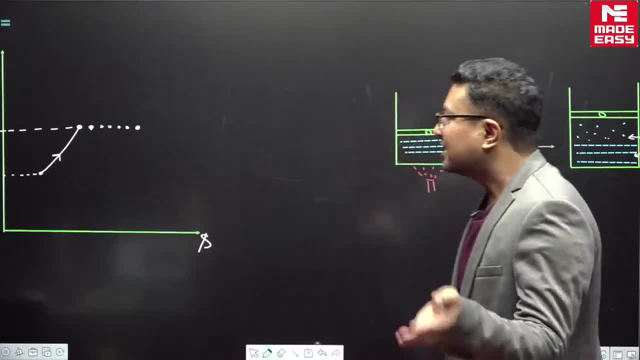 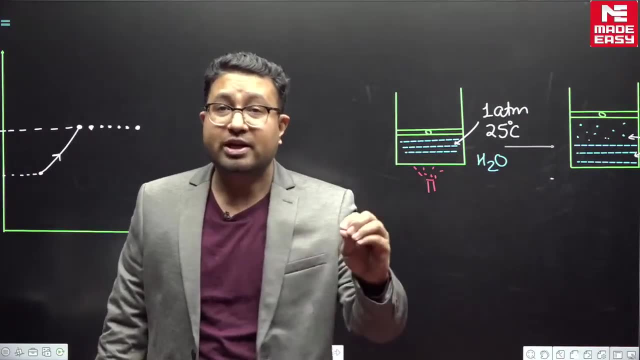 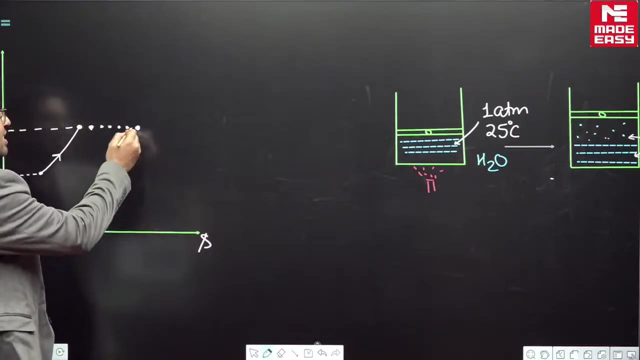 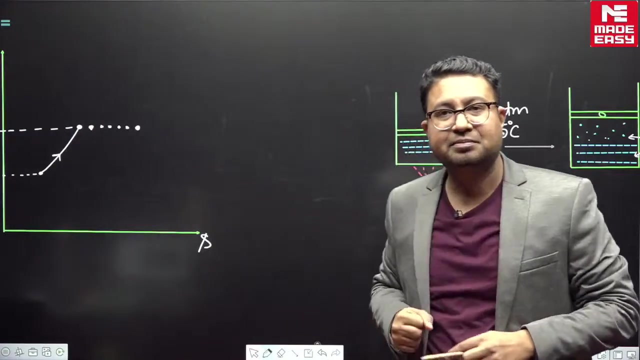 the average, it will come out to be 90,. 90 will come. Anyway, if all the liquid gets inside the vapour, the answer is 80, and finally it runs out to make 30. it will come out to be 35.. Ok, So there will be a condition. a condition will be there when all the liquid would have changed into vapour, All the liquid would have changed into vapour. When the liquid is changed in water, all the liquid would have changed into vapour, all the. 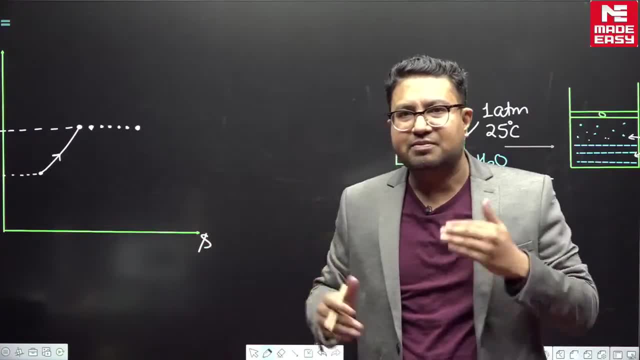 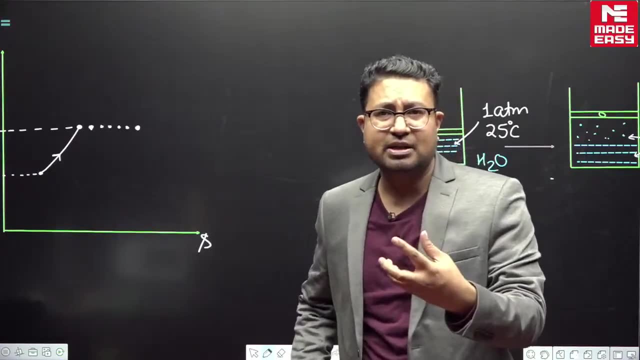 liquid is changed into vapour. when all the liquid is changed into vapour, then the average gets completed. So when the phase change is taking place, energy does not go in increasing temperature. So energy you supply that is not utilized to increase the temperature. 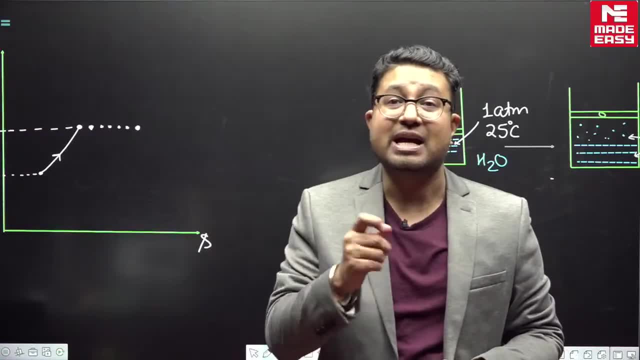 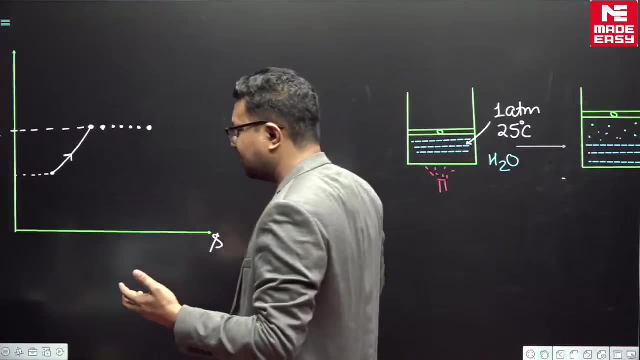 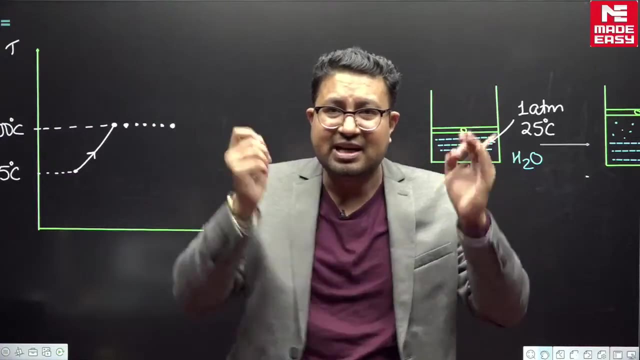 That is why it was called as latent heat. Latent means hidden. We do not know where the energy is going. Initially, people did not have much understanding, So they thought that we are giving energy. but the temperature is not rising, So the energy is hidden. It is. 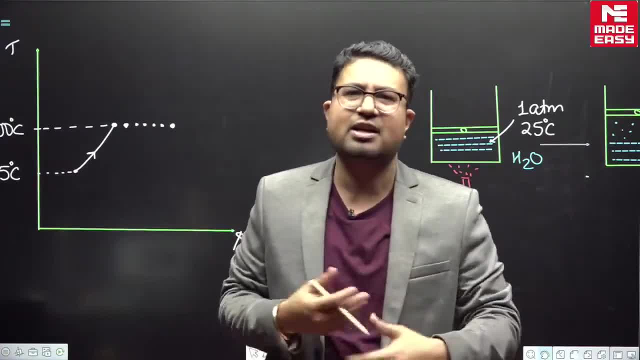 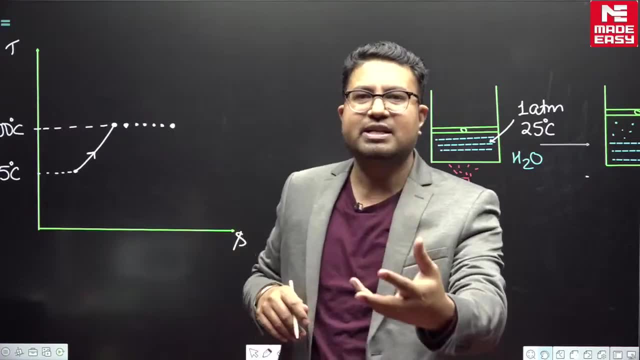 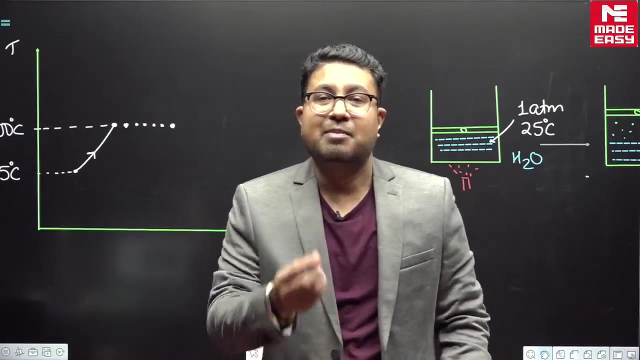 getting stored but it is hidden. So that is why the name came latent. Latent name came. So temperature is constant, Liquid is changing into vapor. When all the liquid has changed into vapor, Why it is taking time. Suppose you are boiling water, So time takes time. Because per 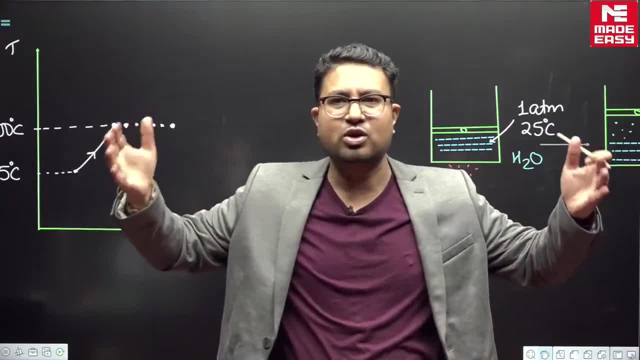 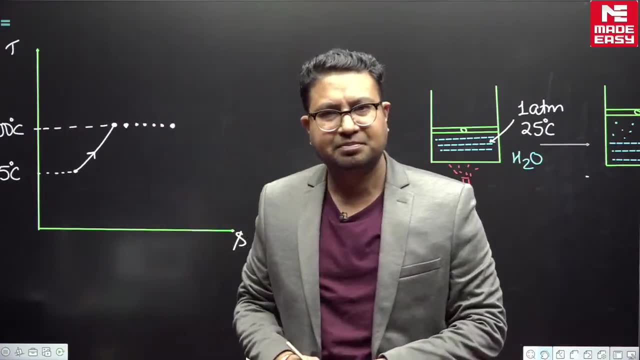 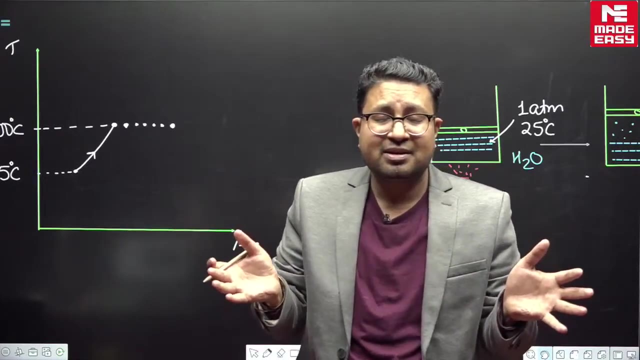 kg. the energy required is very huge. Energy required for phase change is huge. You are not able to supply the entire energy at once Because there is a lot of mass of vapor, There is a lot of mass of liquid lying there, So you are not able to supply all. 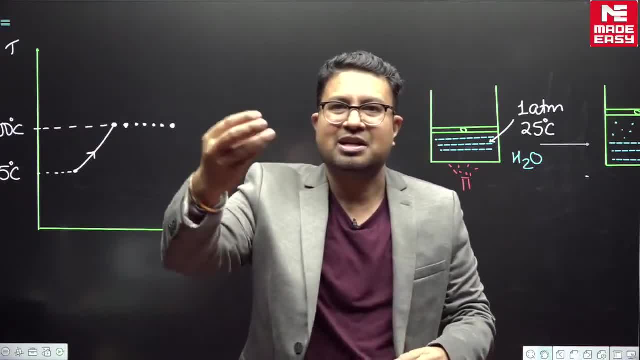 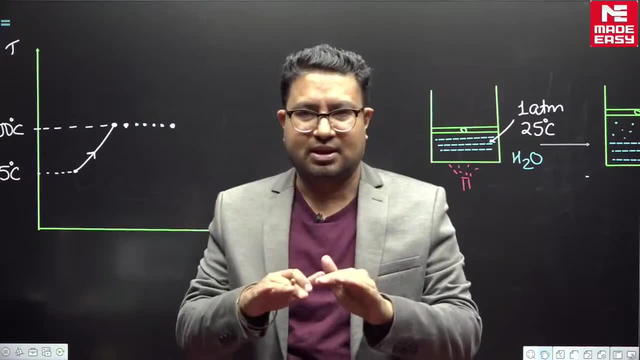 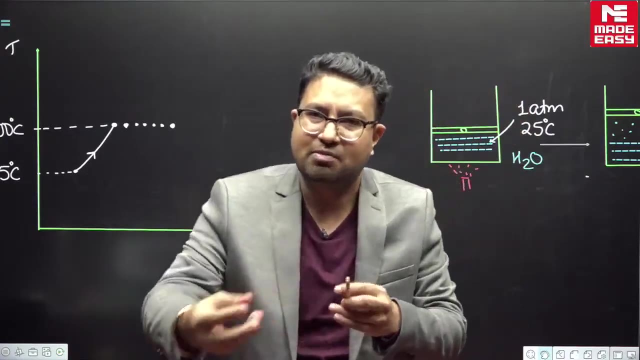 the energy at once. That is why it takes time As the energy comes, taking that energy. whatever mass of liquid can change into vapor. Then some more energy comes. Some mass of this liquid changes into vapor. Rest of the mass waits. Some more energy comes, That mass changes. 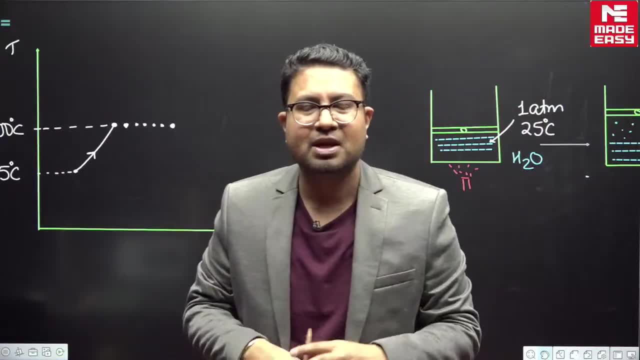 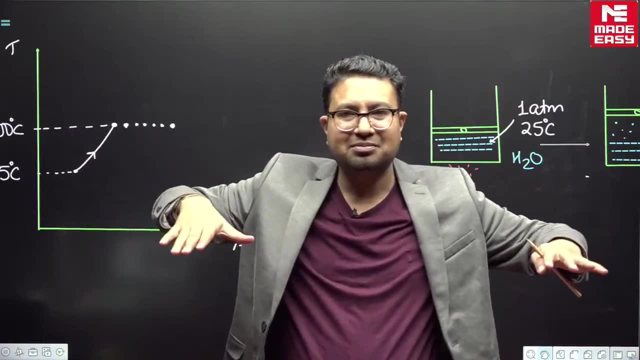 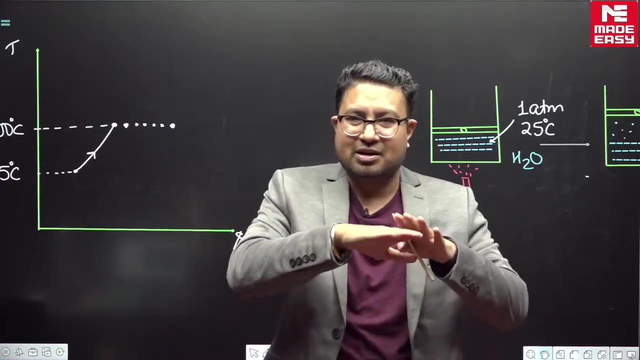 into vapor. Rest of the mass waits, Waiting time. You see, when somebody is preparing dosa, When someone makes dosa, So if the plate is very hot, When somebody is preparing dosa, If that is very hot, So if you drop one drop of water, Drop one drop of water. 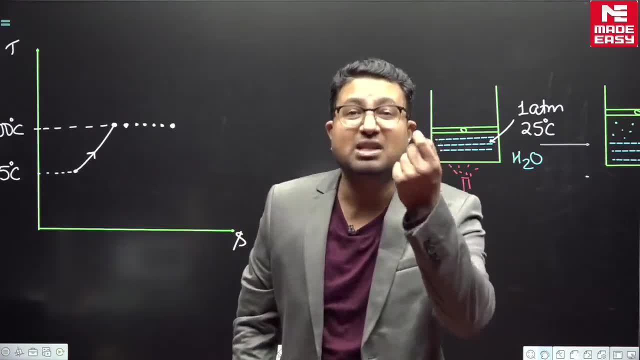 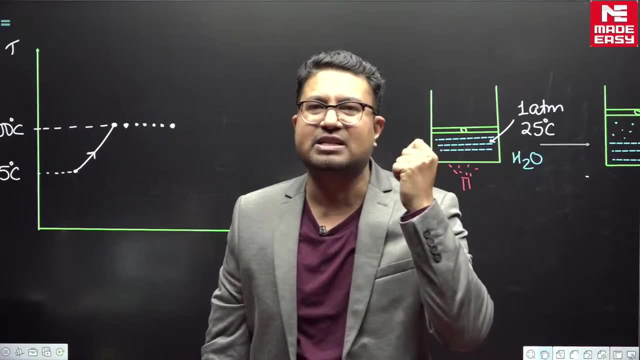 So it is not that latent heat is very less. Latent heat is significant, But the mass is very less. Mass is very less, So energy required for that mass to convert into vapor is received within seconds. Within seconds that energy is received, So there is no waiting time. 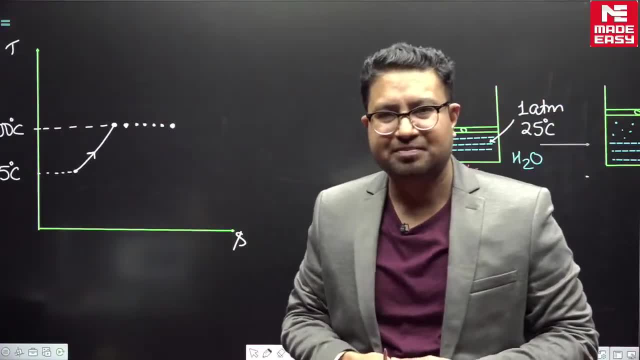 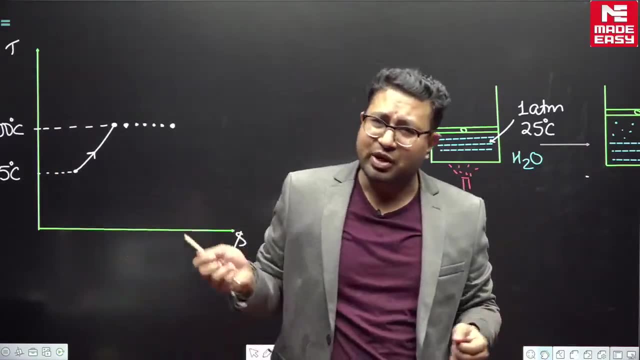 As soon as the drop falls, you feel that it has evaporated. But when there is a pan in which there is a lot of water, So when you heat it, there is time which is required for the entire water to convert. So when you heat it, there is a lot of water. So when 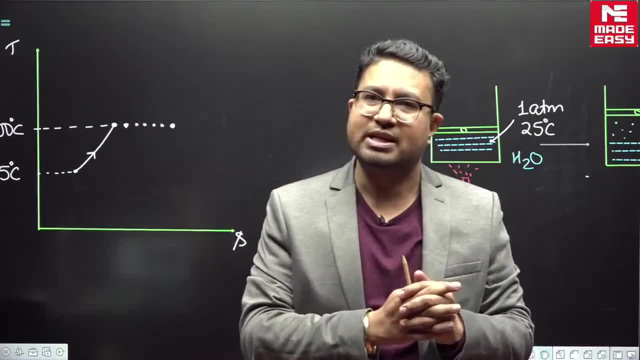 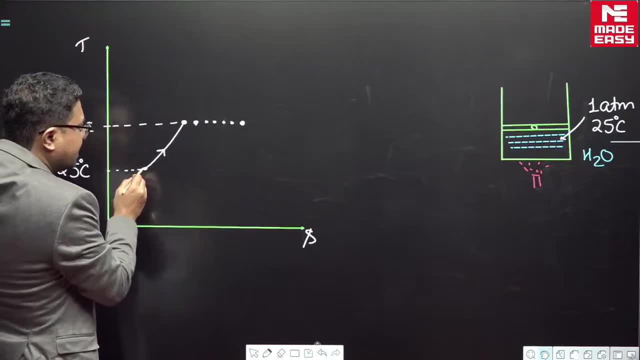 the pressure isquYUión, it can bemay change into vapor now, because alotte of energy we need to supply. We are going to have to supply a lot of energy. ok, So let us see here. we started heating. We started to heat, There was water at 25. 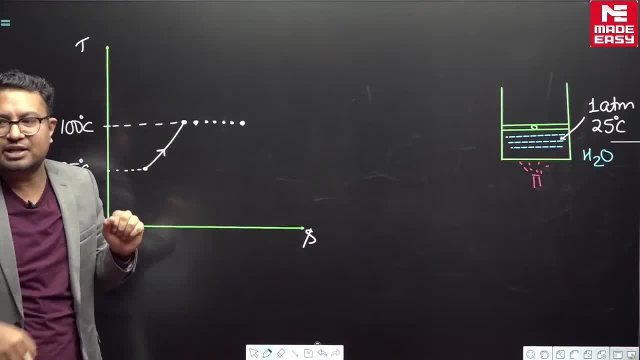 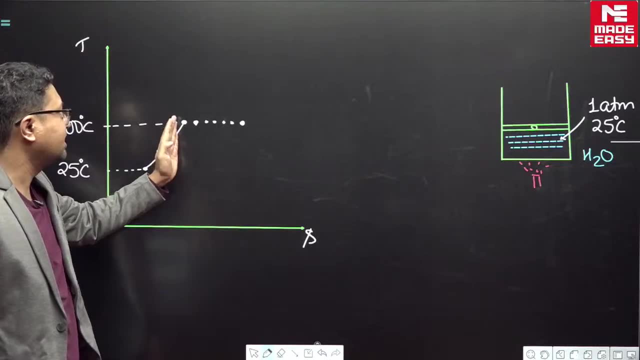 degrees Celsius. Temperature increased. Temperature started increasing When it reached 100 degree Celsius. A temperature reached 100 degree Celsius. A temperature reached 100 degree Celsius. Then then the liquid started converting into vapor. It started converting into liquid vapor. 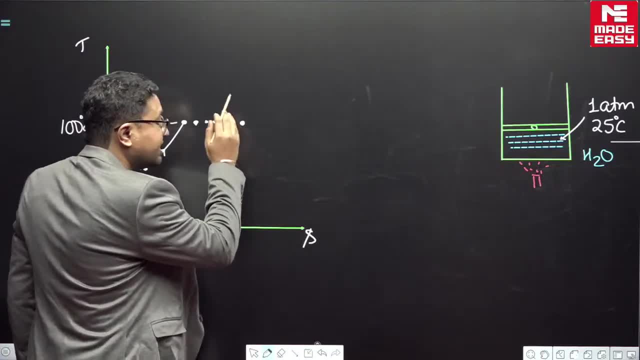 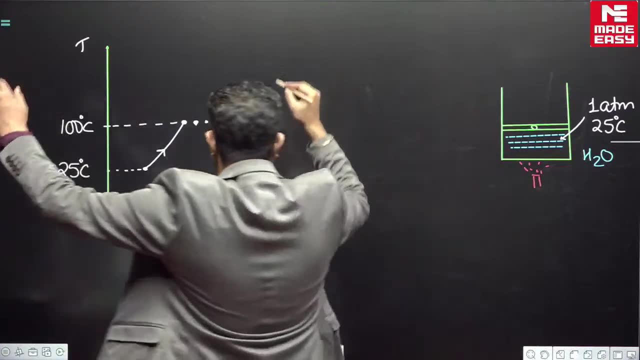 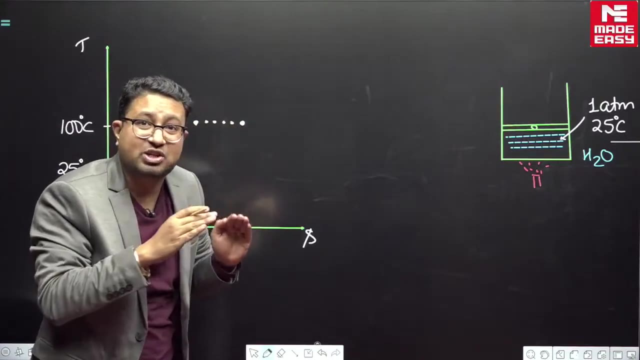 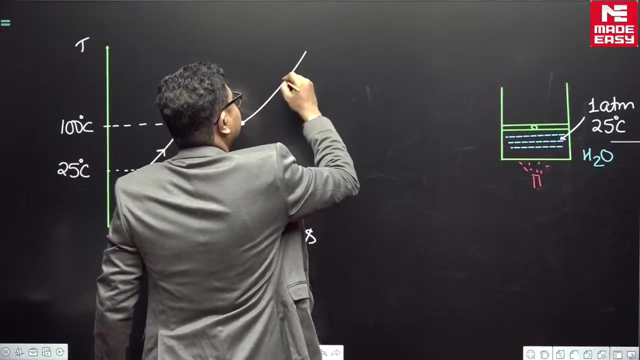 into vapor. the average is shifting every shift. when we are here, all the liquid has converted into vapor. all the liquid has converted into vapor. now, when all the liquid has converted into vapor, then if you again continue heating up, heating continue, pressure is constant, but now phase change, complete temperature will start rising, temperature rise and this is the curve, this is. 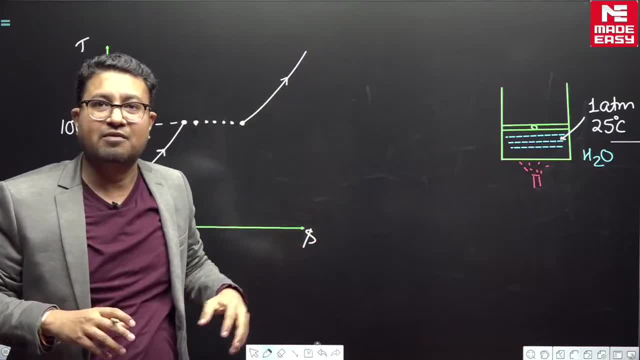 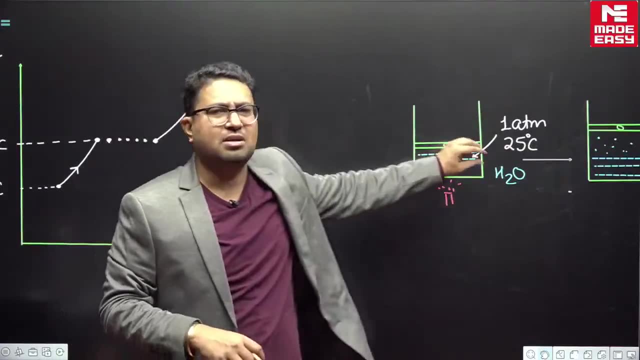 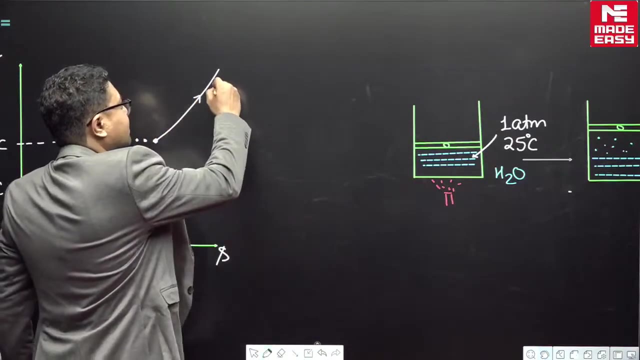 the curve. when this curve we got. under what conditions we got this curve? we maintained a pressure of 1 atmosphere. suppose there was a massless piston. massless piston, we were able to maintain 1 atmospheric pressure, 1 atmospheric pressure maintain. so this is the curve corresponding. 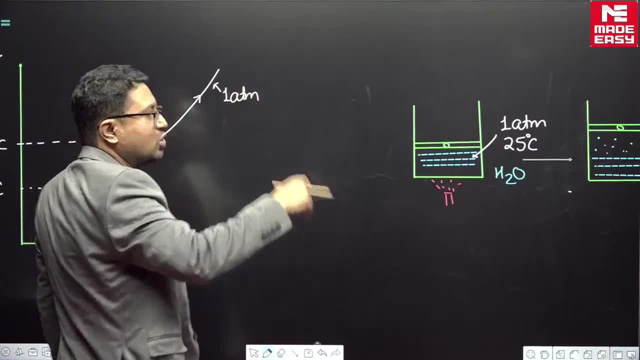 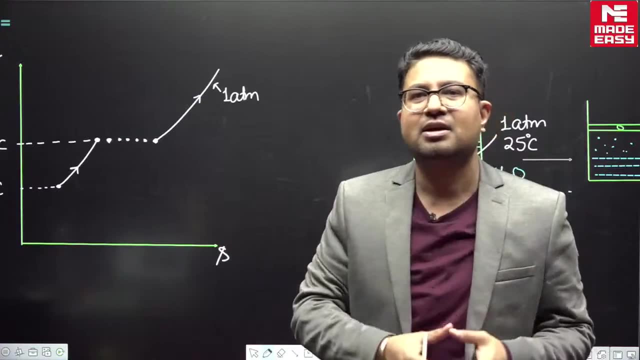 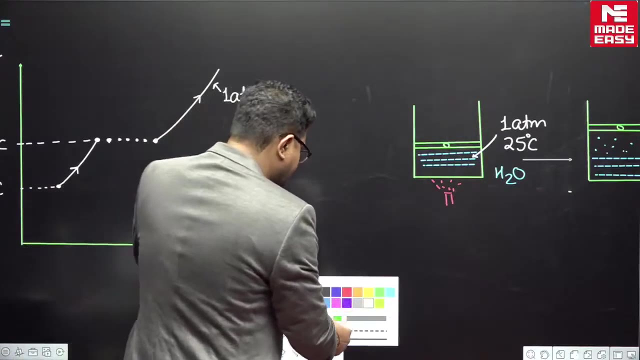 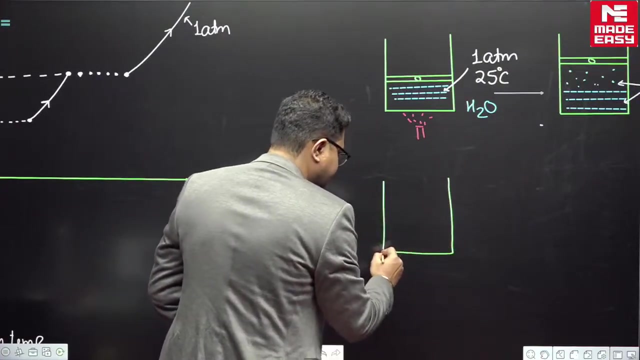 to 1 atmosphere now. now you can make a curve corresponding to 2 atmosphere also. you can make it corresponding to 2 atmosphere also. What you will do, You will put a small weight. you can put a small weight here and for the same, let us say, piston cylinder inbent, let us say, for the same, piston cylinder inbent. 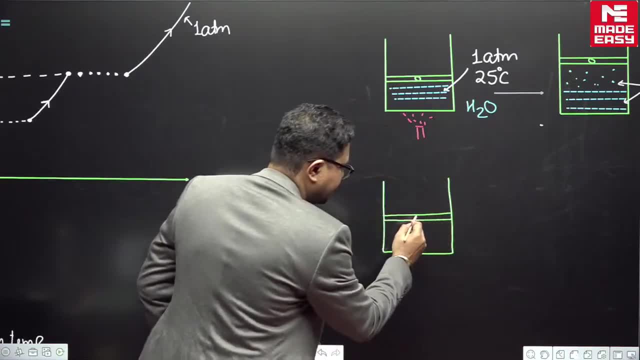 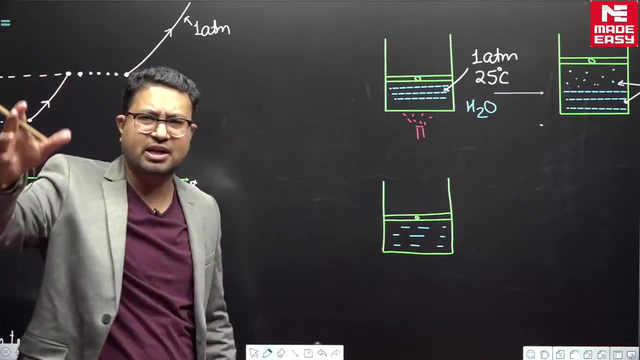 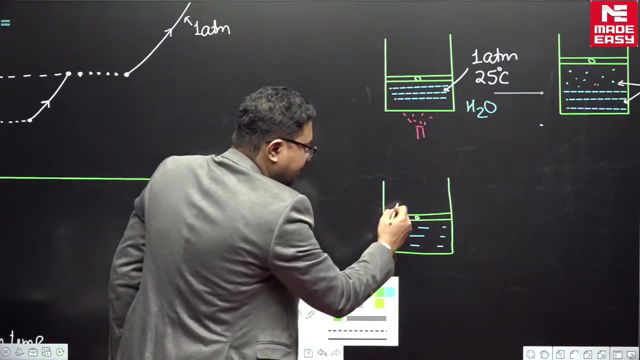 if I put a small weight, such that, such that. just let me show you here: this is the water. initially, We will take water at 25 degree Celsius, but at this time, this time, what we will do, What will we do? We will place a small weight, we will place a small weight. 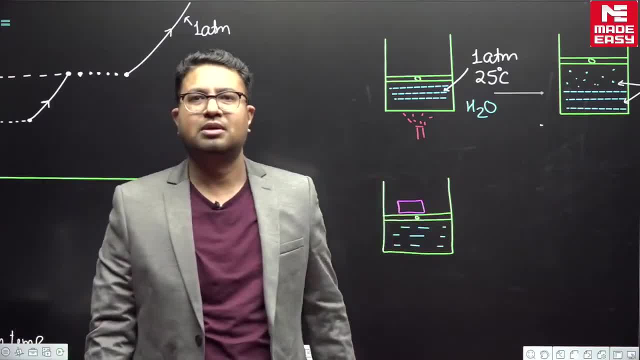 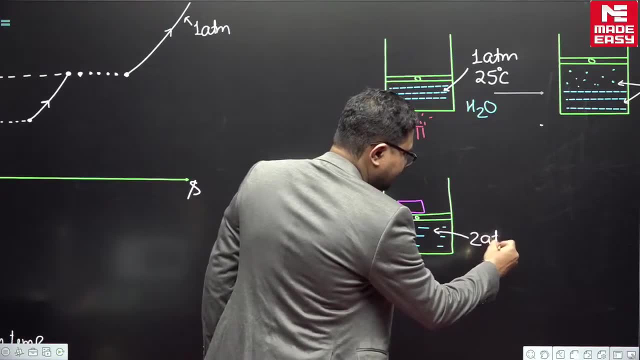 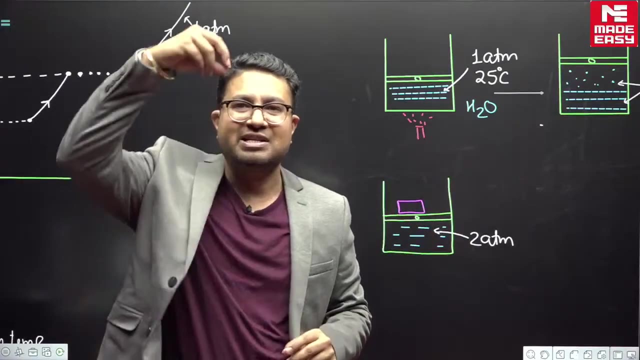 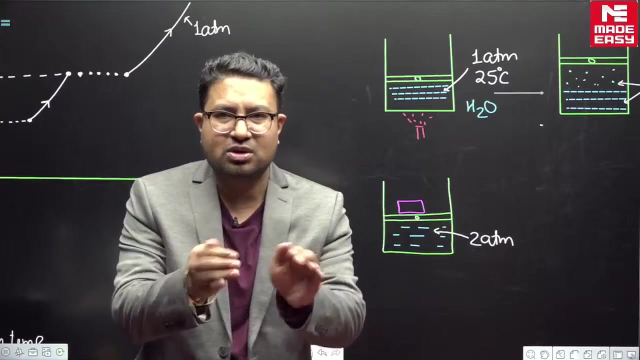 sufficient enough, sufficient enough that the pressure inside is 2 atmosphere, 2 atmosphere pressure cooker, may, pressure cooker, may. the whistle generally, generally, I am telling you an idea, I am just giving you an idea generally, the whistle weight is such that whistle weight is such that because rest, everything is closed, rest, everything is closed. The weight of the whistle is such that it will not open till the pressure. inside is 2 atmosphere generally bad dece. the pressure cooker is inside, can increase the pressure up to 2 atmosphere. that is 1 atmosphere more than the outside, and then the whistle will. 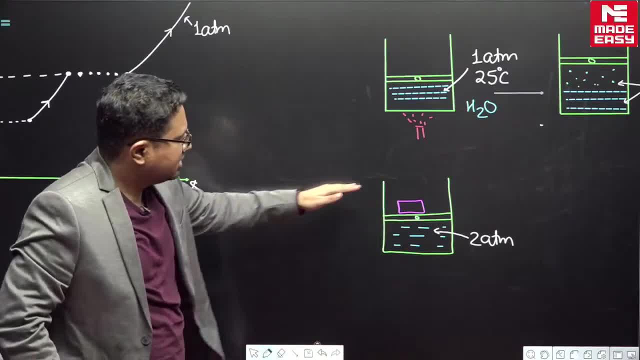 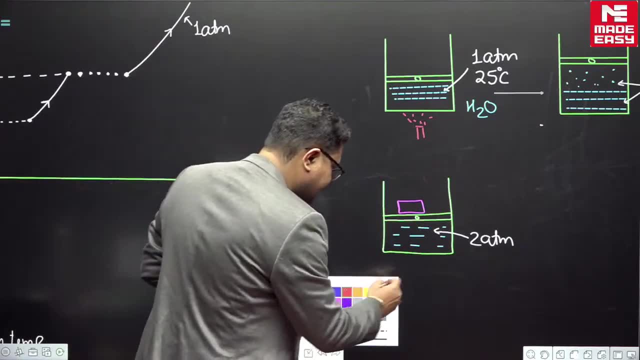 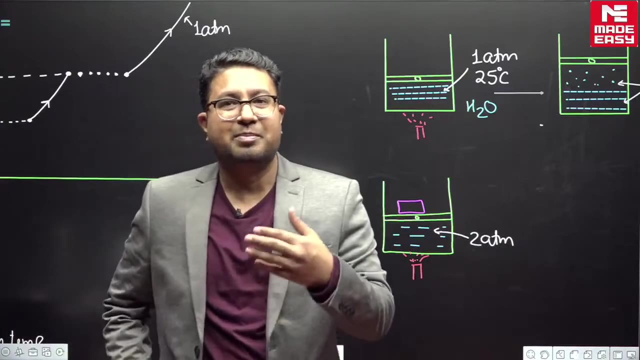 be lifted. this is the general data which I am sharing. so suppose this is the weight which is maintaining the pressure inside 2 atmosphere. Now if you start heating above, isko heet karna starrt karo isi liye. toh kya hota hai ki when you cook food in pressure cooker, pressure cooker me. 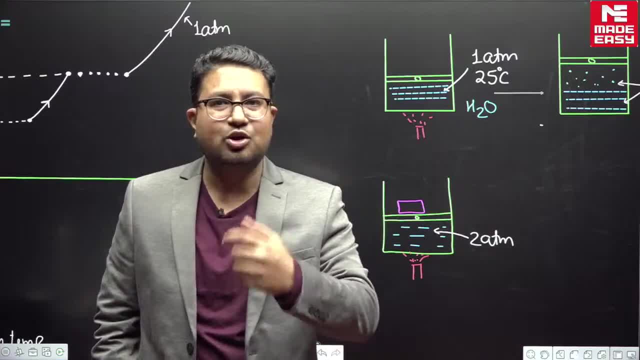 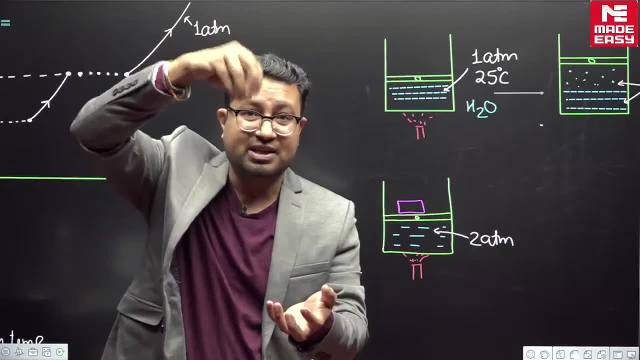 jab khana manate ho. toh why it cooks early jaldi kyo ban jata hai. one of the major reason, ek jo major reason hai, wo ye hai that you have put weight whistle laga di upar rest. everything is close. so till the pressure reaches 2 atmosphere, jab tak pressure, 2 atmosphere. 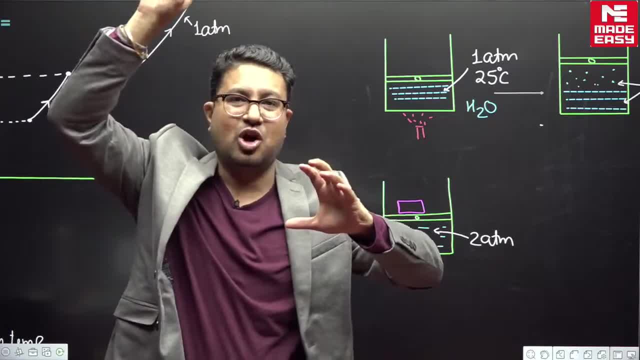 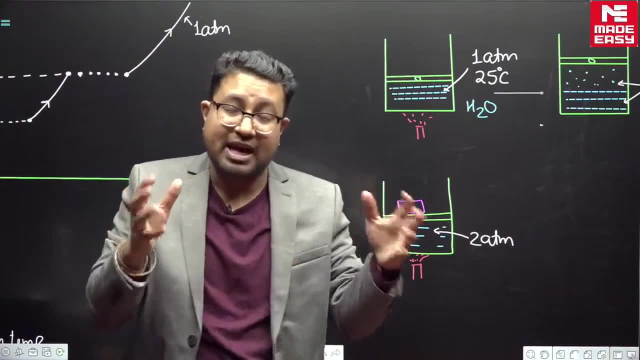 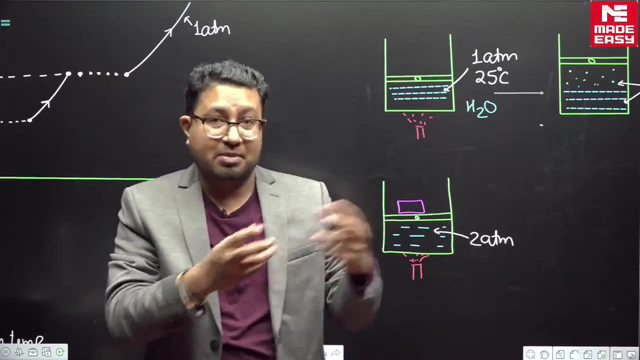 nahi paunchta, the leakage of steam will not start. so 2 atmosphere pe boiling hoti. the boiling starts at. i mean happens is happening at 2 atmosphere. so 2 atmosphere ke according, whatever the temperature of the water can be, paani ka jo bhi temperature ho sakta abhi. 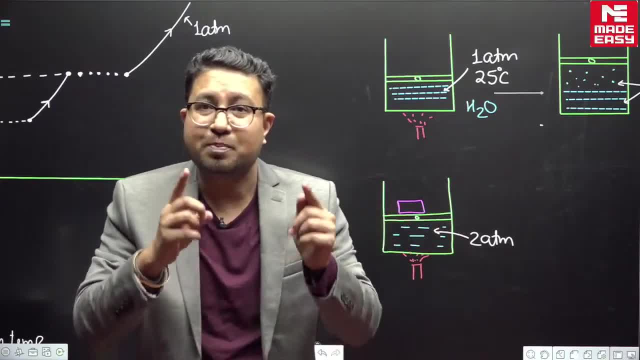 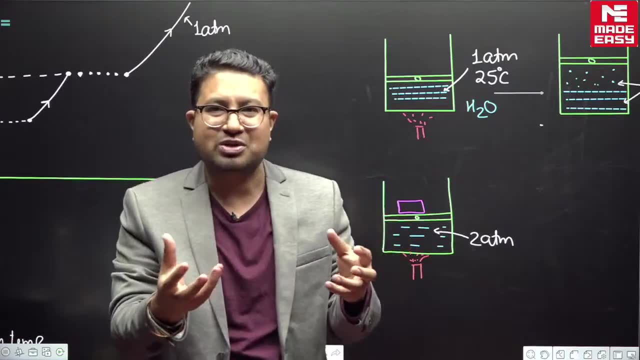 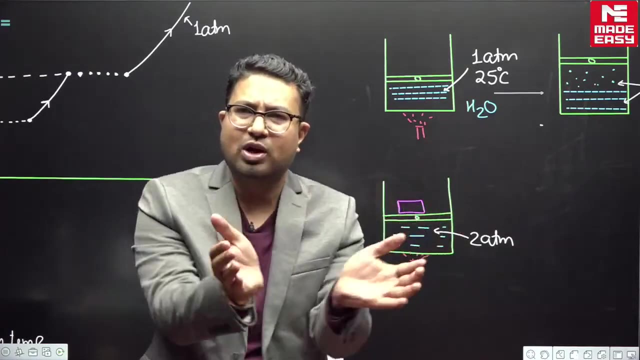 me dikhaunga aapko, it is 120.3 degree celsius, 120 degree celsius, 120.3. so if if you are cooking or boiling potatoes, aloo boil kar rahe ho, if you are boiling potatoes in pressure cooker. so versus compared with what open pan khule hue, bartan me boil karoge toh there. 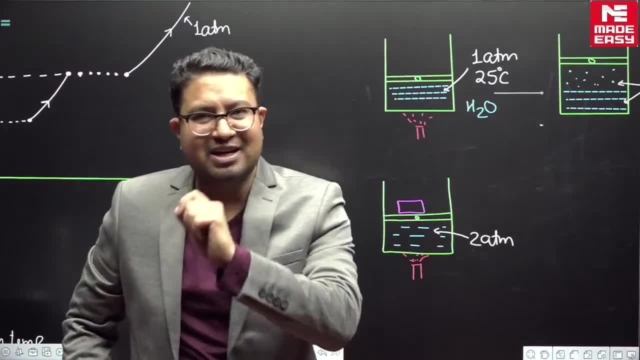 is one atmosphere, that is happening at 2 atmosphere. so if you are cooking or boiling at 2 atmosphere pressure, one atmosphere pressure, toh water will boil at 100 degree celsius. but if you are boiling it in in a pressure cooker, it will boil at 120.3 degree celsius. 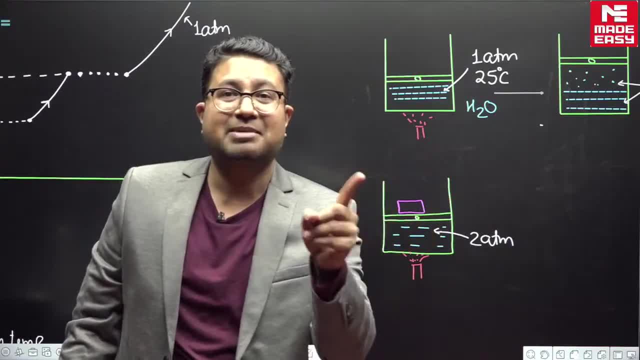 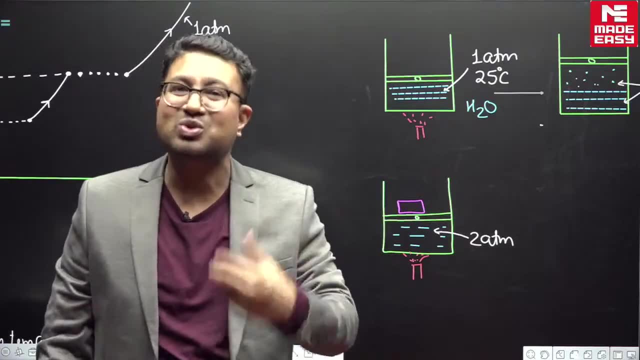 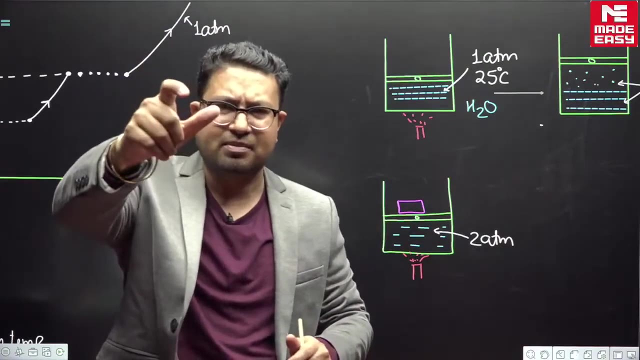 so aloo kis temperature pe rakha hoga. it will be kept at 120.3 degree celsius, so the chemical processes will be faster. chemical processes, jo hongi, wo kya hongi, fast hongi, even though it will take some time. 120.3 tak paunchne me thoda time lagega. it will take some time. 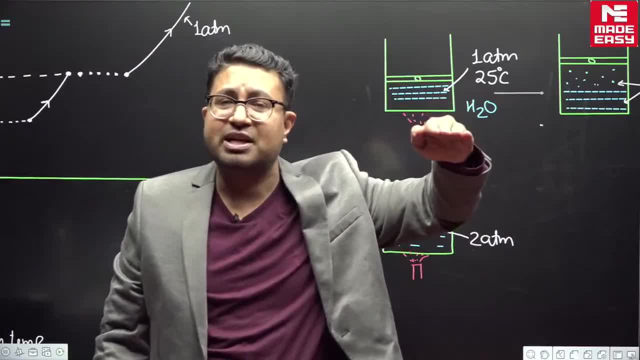 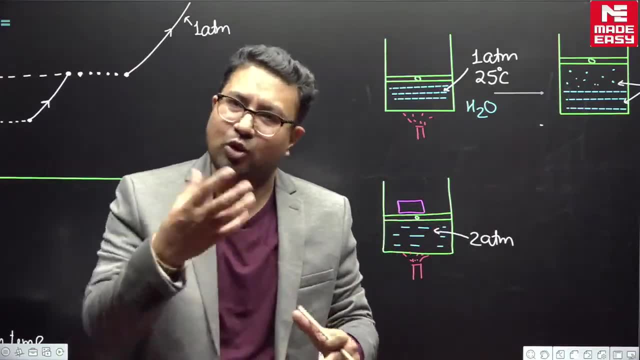 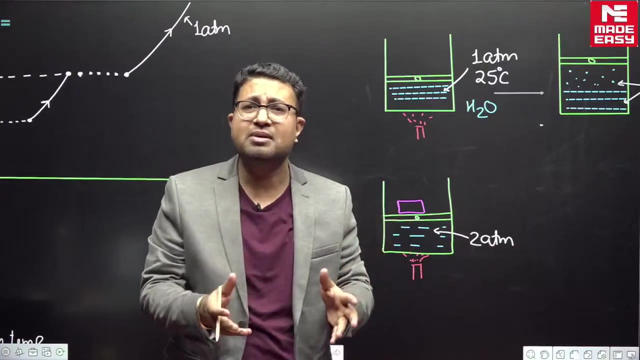 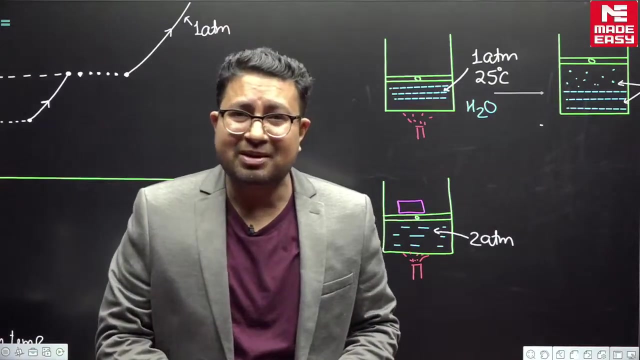 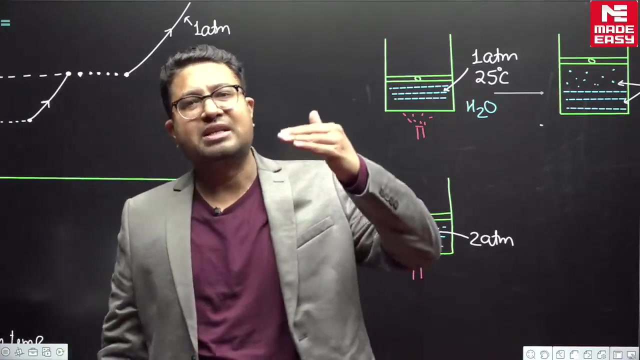 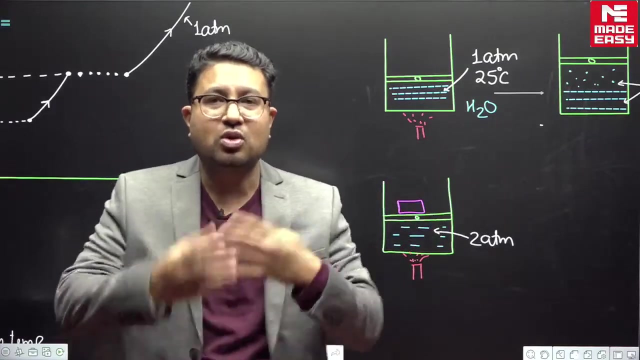 it will take some time, but once it reaches 120.3 degree celsius, it will be kept at 120.3 degree celsius. the processes will be faster. so that is why the so when you add salt so slightly, the boiling temperature increases, so the food will cook. 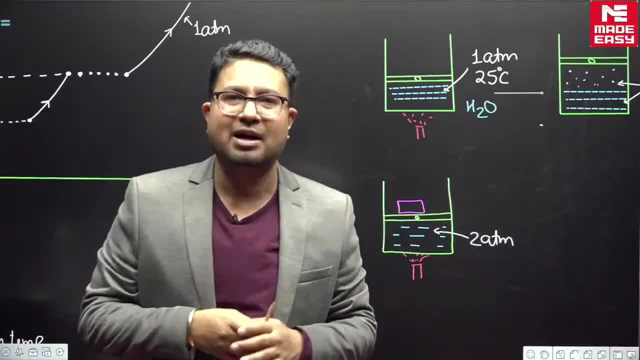 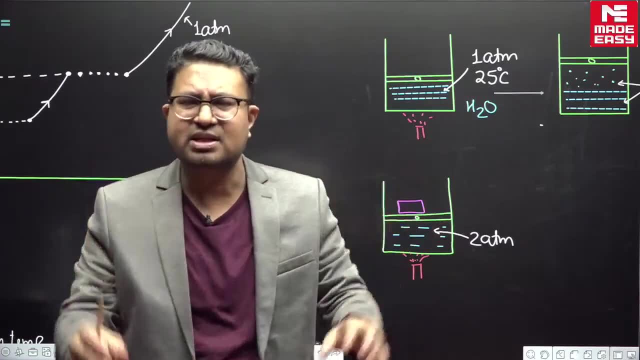 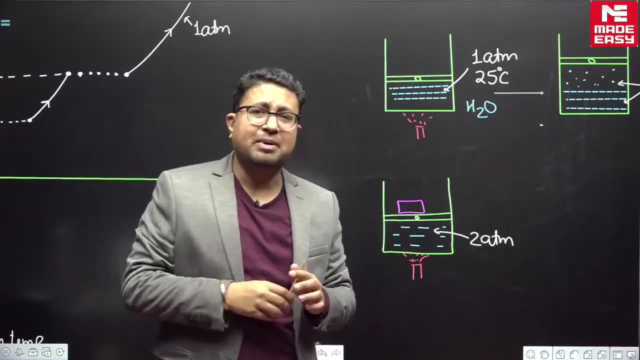 a bit faster because the food will be kept slightly above 100 degree celsius. 100 degree celsius is one of the reason is this. there are other chemical reasons, but one of the reason is this, and also, if i am discussing this, so let me also tell you that people who cook food, in the mountain regions. mountain regions- it is sometimes said that it takes longer to cook food compared to planes. the reason is there. the pressure is less. so suppose you are boiling potatoes in an open container, planes maybe. i mean, it is obviously land there also, but uh, in planes 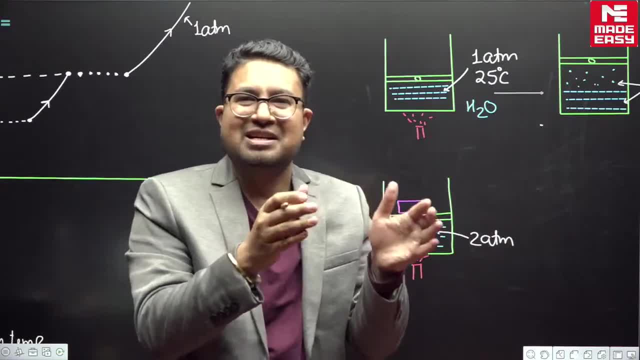 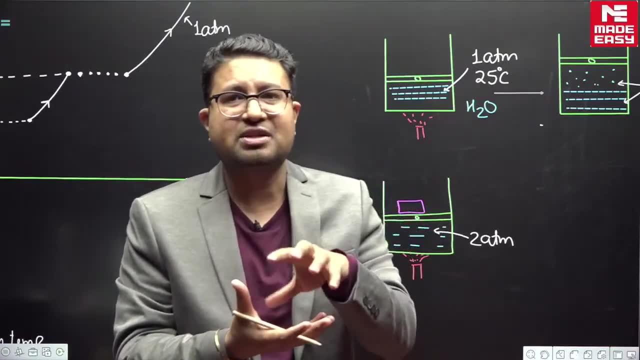 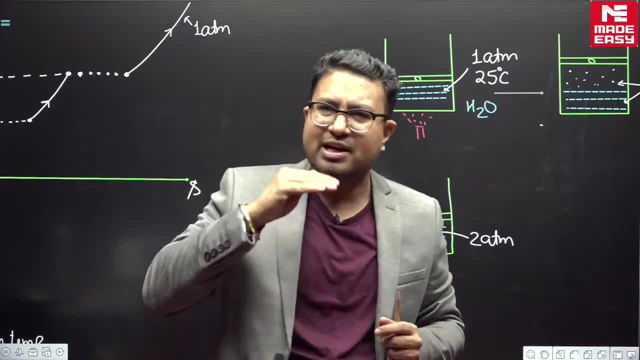 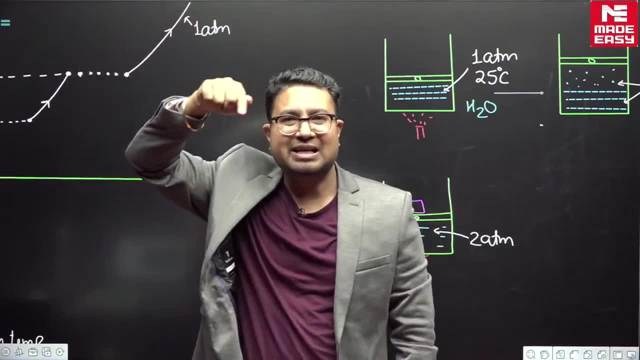 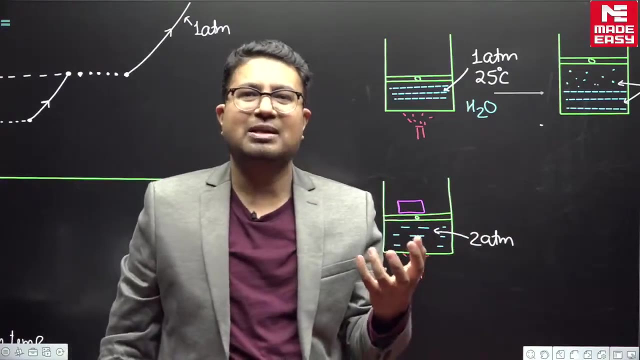 0.O. 0.0, 0.3. this we have, so you will have an open vessel. let us say, in that you are boiling the potatoes, in that you are boiling the potatoes in the mountain regions And the pressure is less than 1 atmosphere. 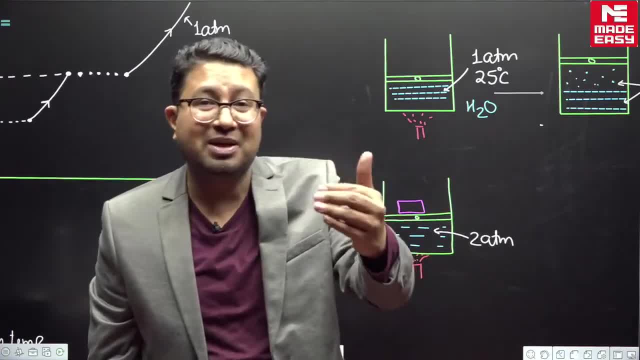 1 atmosphere is a little less, So boiling temperature will not be corresponding to that. It will not be that much, it will be a little less than that. Now I will show you on the graph also. I will show it on the graph. 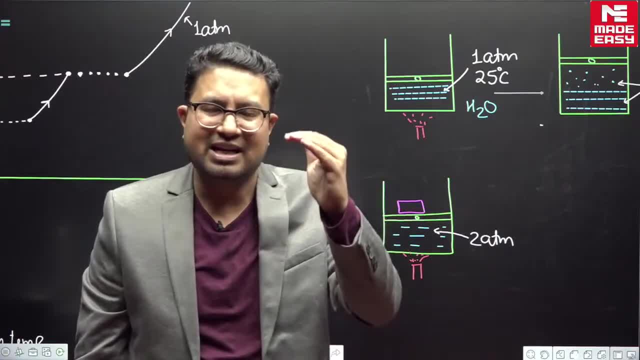 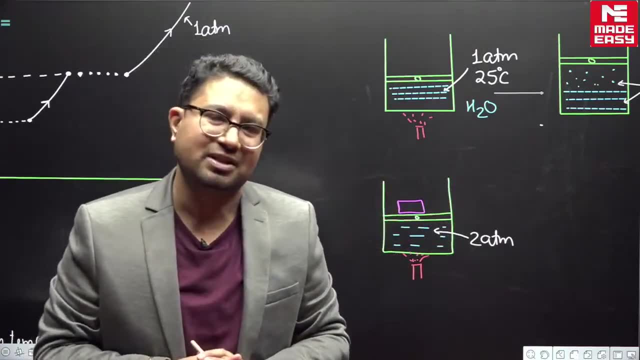 So the boiling temperature is, let us say, 98,, 97,, 99 degree Celsius, So corresponding to 99 degree Celsius. the potatoes will be kept. According to that, the rate of chemical reaction will be there. Yes, boiling temperature will increase quickly. 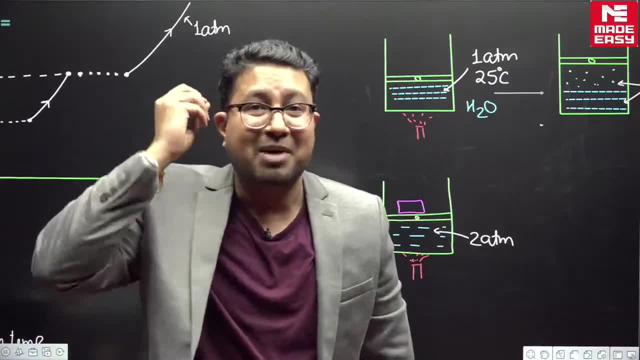 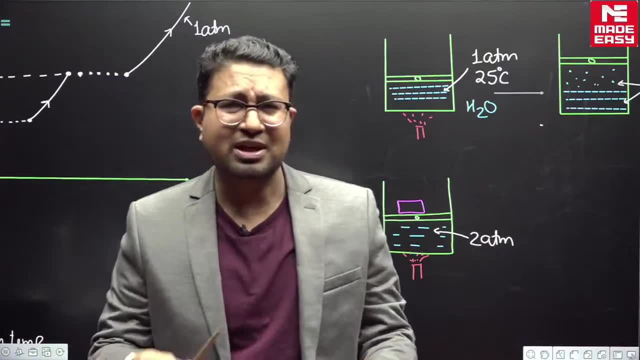 It will take less time to reach the boiling temperature, But potatoes will be kept at that temperature only, So it will take more time for the chemical reaction to take place. So that is why it is said when you cook food, But that time is very less. 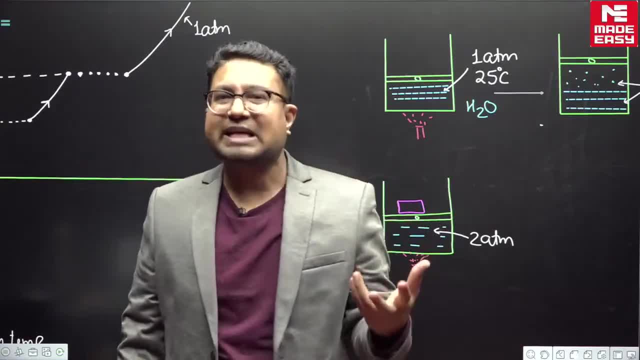 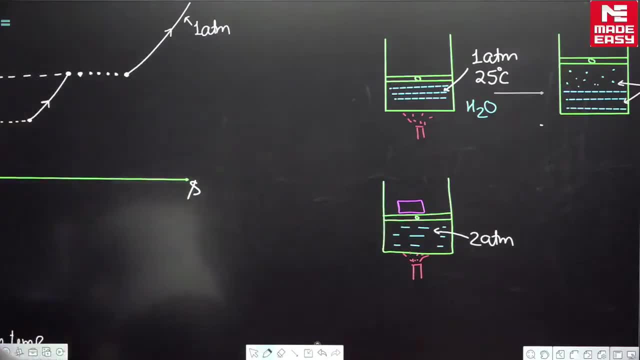 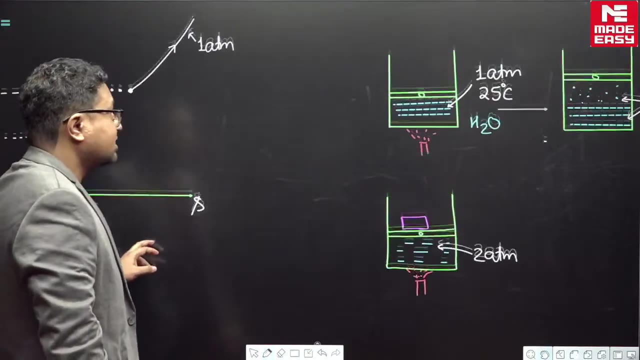 The time change is less, But if we speak technically, then, yes, it takes slightly more time when we cook food in the mountain region. Mountain region, Fine, So now. So just let me tell you once again. There are some people who are asking up to when it will be live. 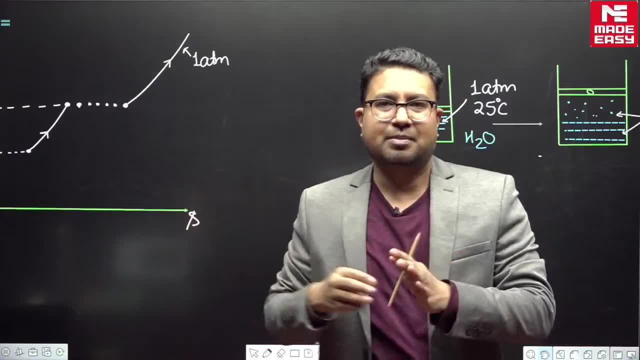 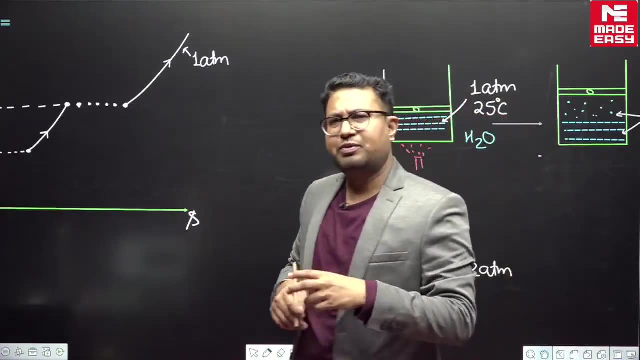 So what I have planned is 5 to 9. I have planned 5 to 9.. But 15 minutes here and there will take, Because in the discussion that much time extra we can take. So 15 minutes here and there. 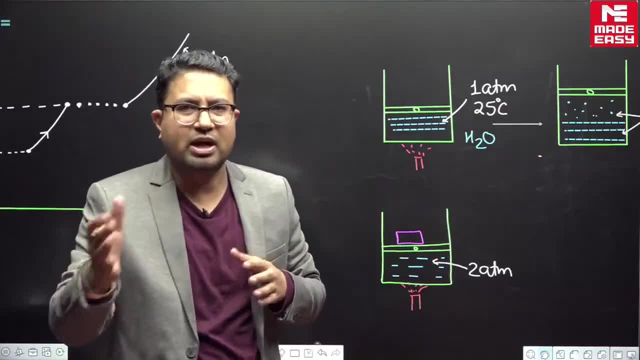 Otherwise up to 9 o'clock. I have planned We can go up to 9.15 also, depending on the discussion. So that is what I have thought of. Fine, Now suppose I have kept some weight. Again, I have kept some weight. 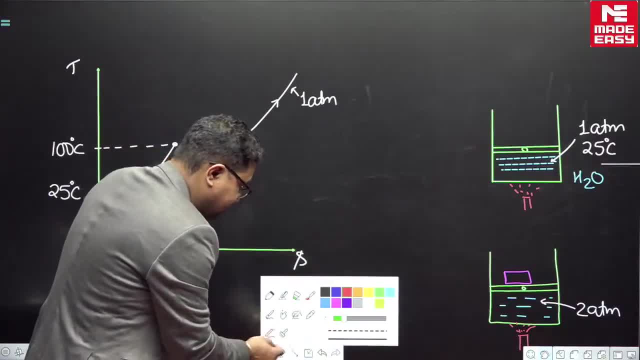 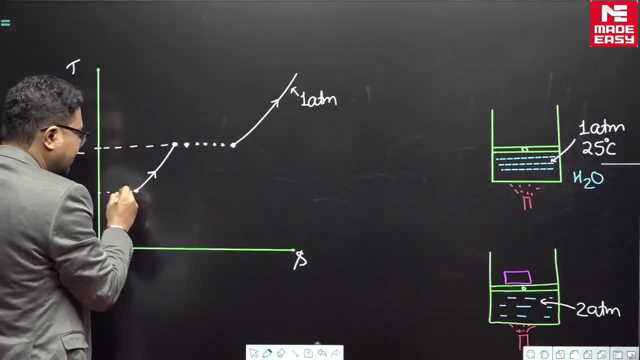 The pressure inside is 2 atmosphere, Pressure is 2 atmosphere. Now, Now suppose pressure inside is 2 atmosphere. Now suppose when the heating starts. Now suppose, when the heating starts, Suppose pressure is 2 atmosphere, Pressure is 2 atmosphere. 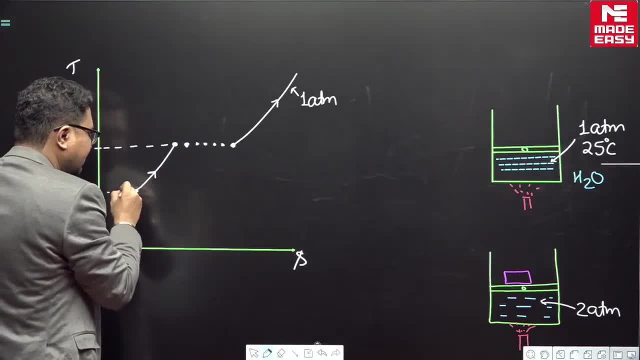 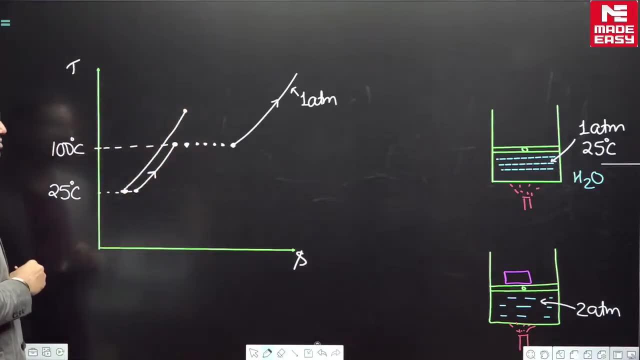 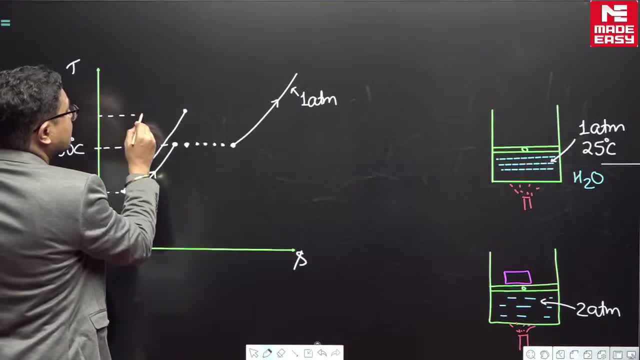 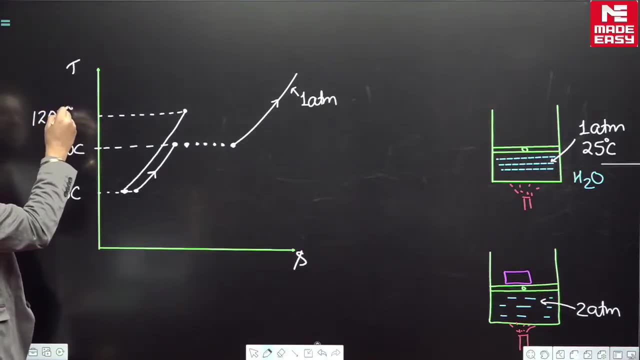 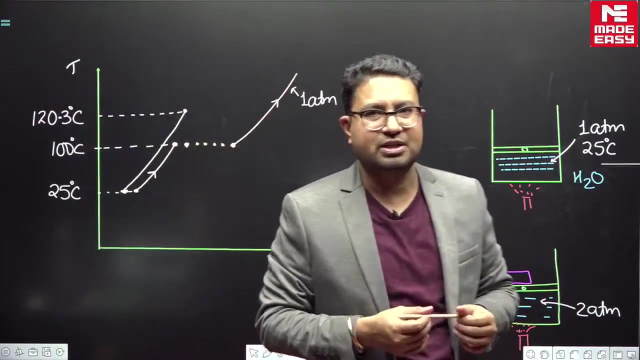 That, That, The, That, The. The boiling started at 120.3,. this is around this temperature, around 120.3 degree Celsius. The boiling started at 120.3 degree Celsius. this temperature boiling started and once. 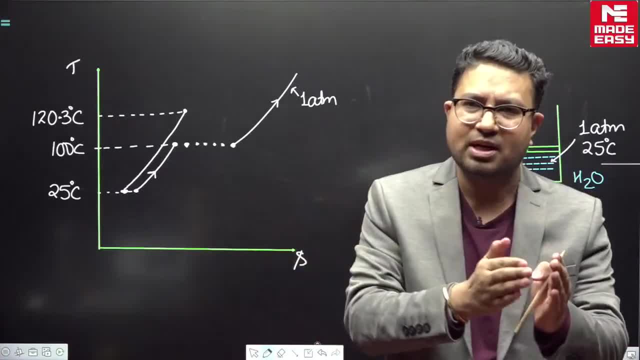 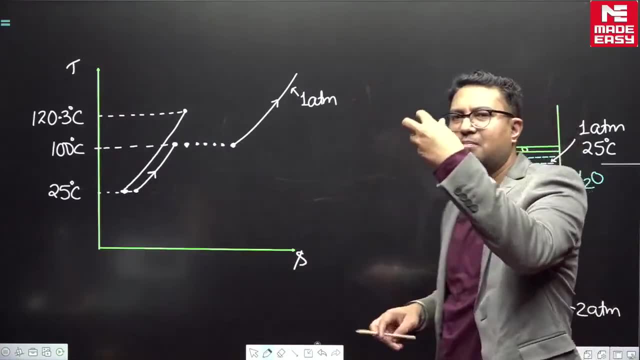 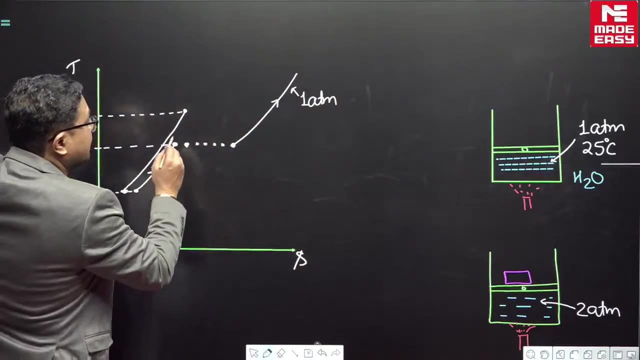 the boiling started. once the boiling started again, the same phenomena continued. you supplied heat, you supplied heat and temperature increment stopped. temperature increment stopped. temperature increment stopped. Liquid started converting into vapor, but the liquid which converted into vapor is in this condition. 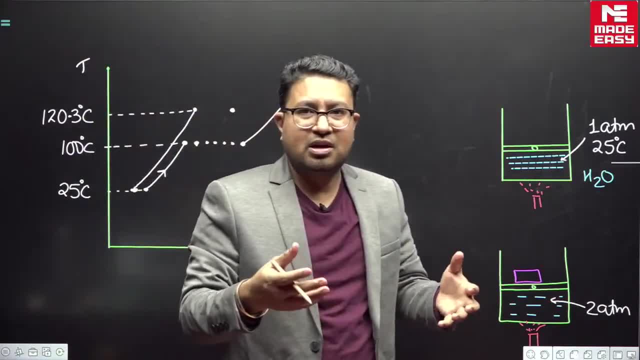 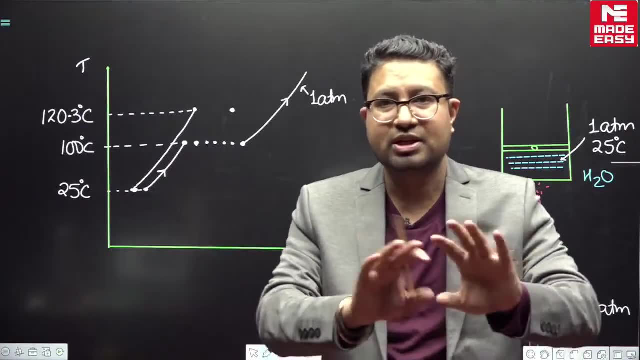 We are studying what is the properties of the substance. we are not making the property of the substance. We are not making it, We are not logically developing it. We are just looking at what is there. we are understanding that it is. this is the property. 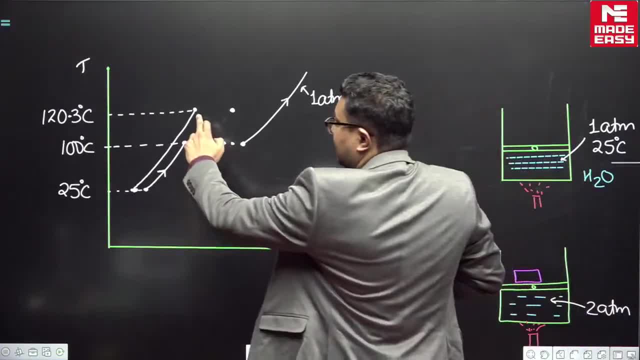 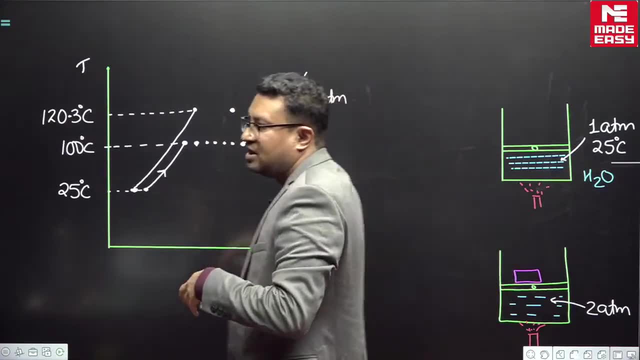 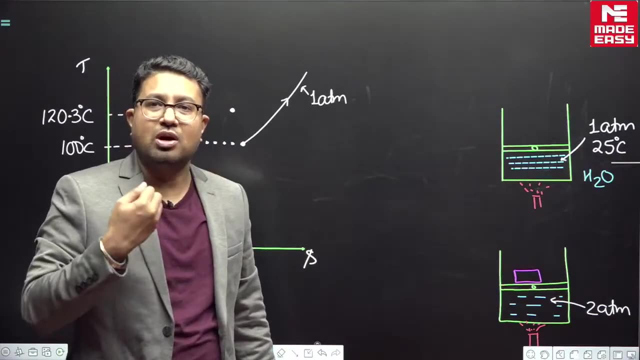 of the substance. So the liquid is having this. This is the condition. the vapor which formed is having this condition. this is the condition. Latent heat drops a little. One of the reason that is given is there is already a lot of energy which the liquid has. 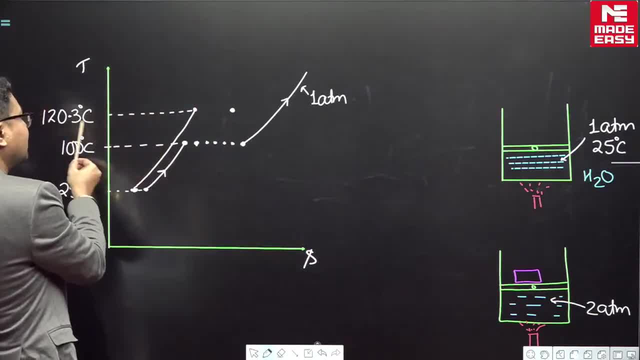 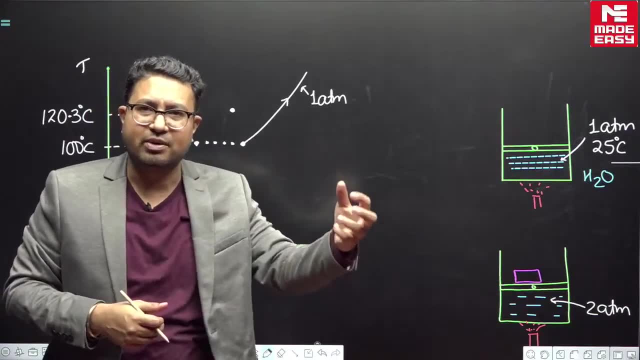 absorbed boiling. if you are doing the boiling at higher pressure, then before the boiling starts, there is a lot of energy which the liquid has already absorbed. a lot of energy liquid has already absorbed. Therefore, now I want you to listen carefully剛剛. 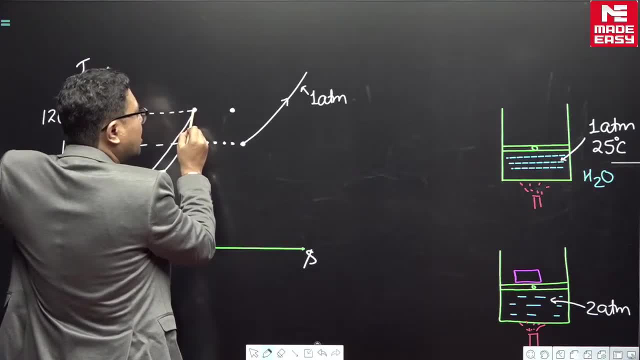 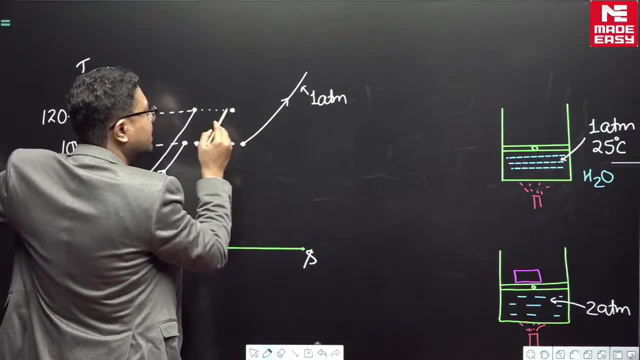 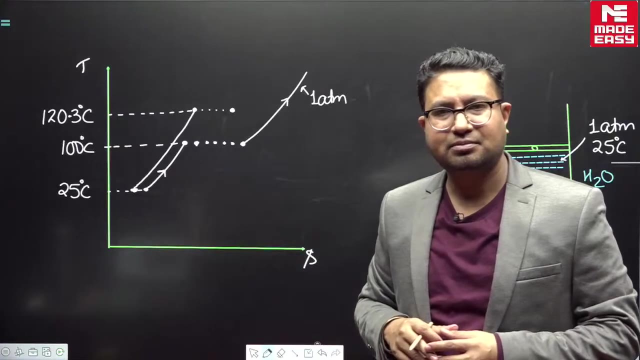 This is where, within the process, the food is all, water needed, sample product is being available from the supplier, from the supplier at the customerik boss, and the supplier can consume in the shop. After that, all we need One. you need to think. lastly, 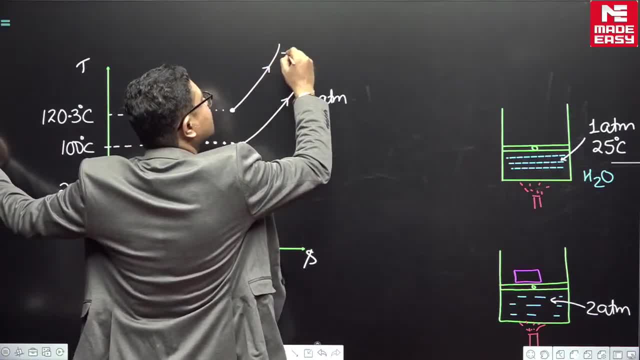 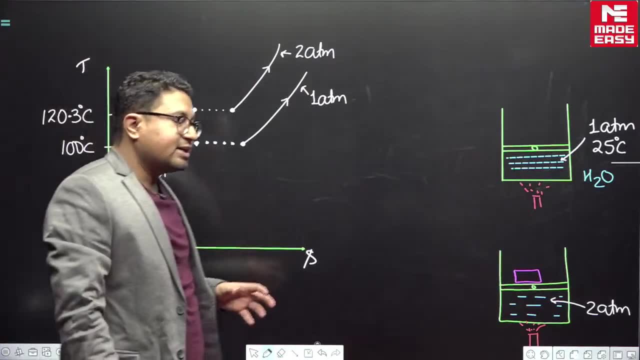 what will I do was w, because the main thing is, when you are doing the whole process in the kitchen, when you are doing the whole process in the kitchen, you are, of course, becoming a customer, Sponsoring customer- of the closed shop to 2 atmosphere. This is corresponding to 2 atmosphere. We conducted this experiment. 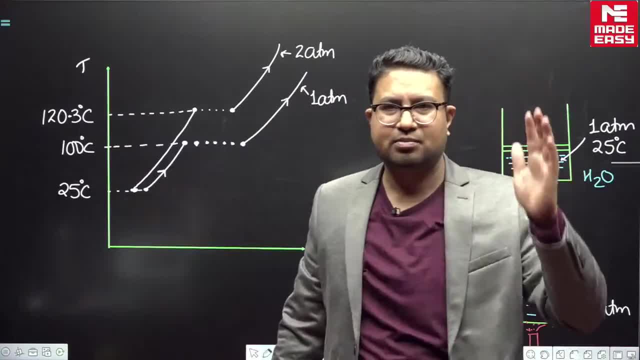 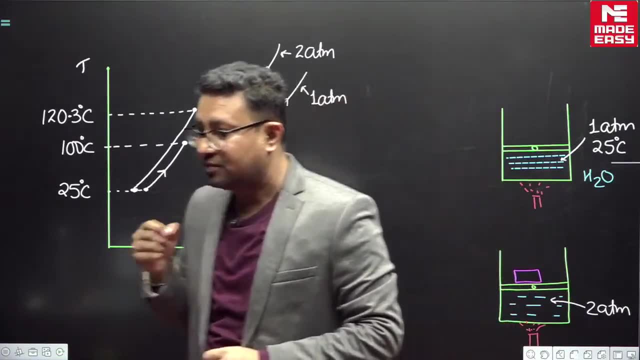 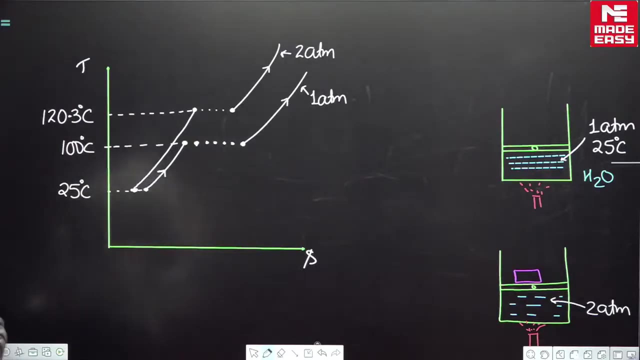 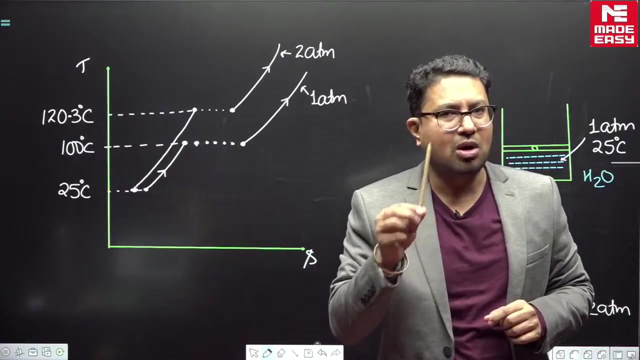 for 1 atmosphere, 2 atmosphere, 3 atmosphere, 4 atmosphere, and so on. We conducted many experiments, We conducted these experiments, We conducted many experiments. After that, what we did, What we did. So what we did, We joined all the conditions, all the conditions. 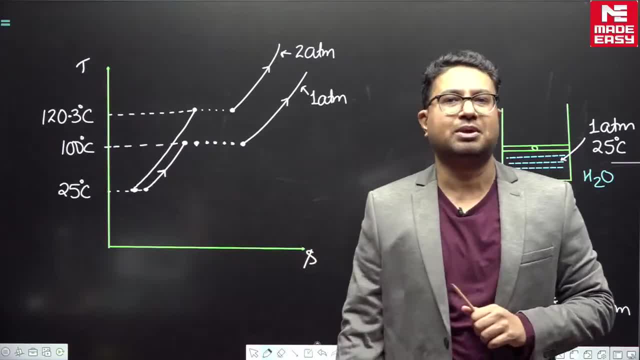 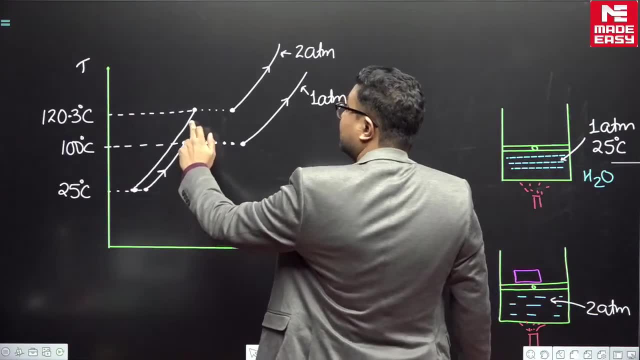 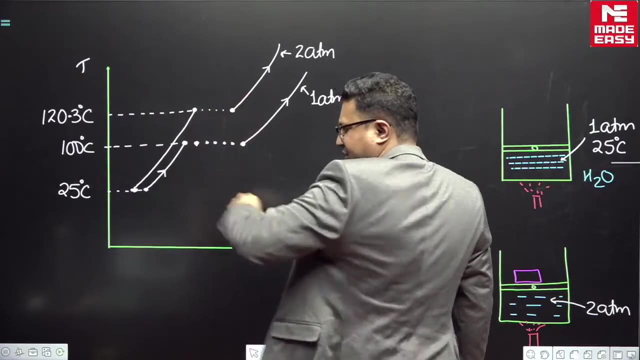 where the liquid was just ready to convert into vapor. Where is the condition for 1 atmosphere? This condition is here for 1 atmosphere. This condition is here for 2 atmosphere. This condition is here When the liquid is just going to convert into vapor, when the liquid is just going to convert. 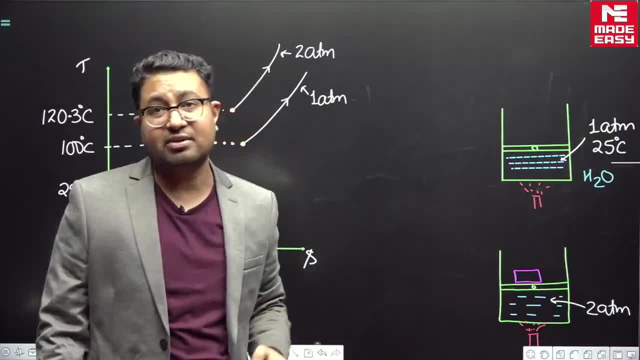 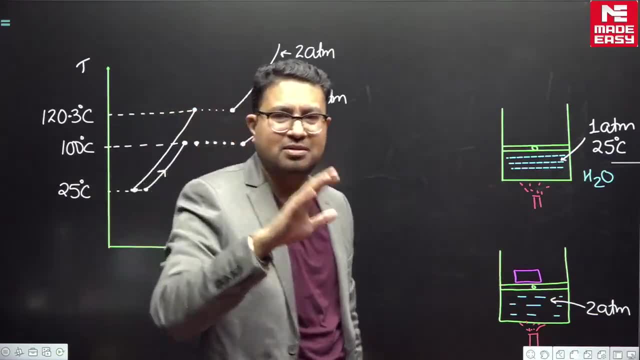 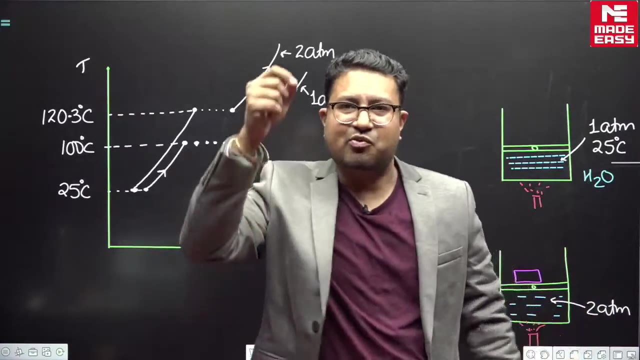 into vapor. we call it saturated liquid. Saturated liquid means, when we use it in the normal terms, I am saturated of this. It means I am completely saturated. It means I am fulfilled, Being liquid. whatever energy you can absorb, you have already absorbed. You have already. 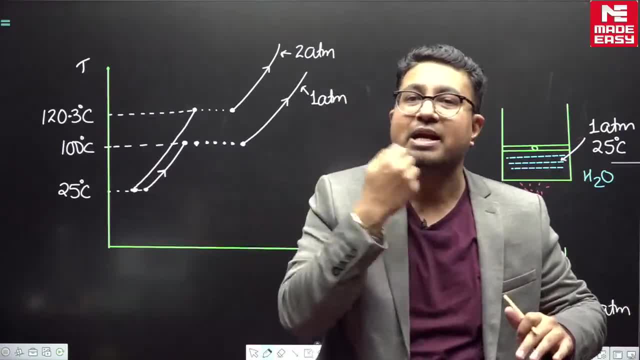 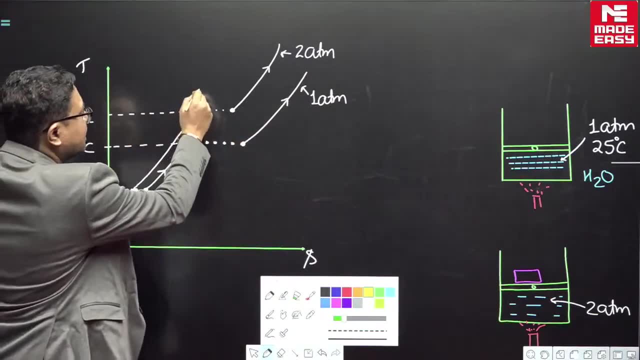 absorbed, Saturated as a liquid. Now, if more energy is supplied, you cannot remain liquid. You have to convert into vapor. So all these points, all these points which we call as saturated liquid points, we join it with a curve. We join it with a curve. That is why 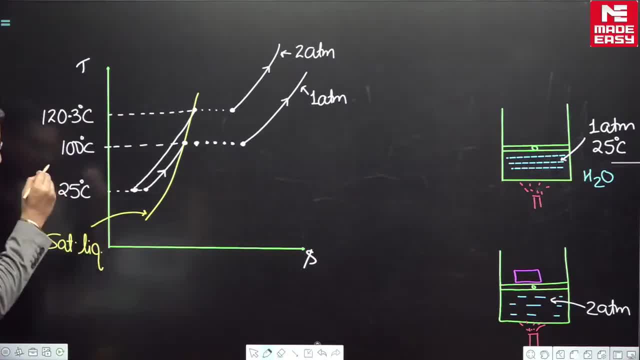 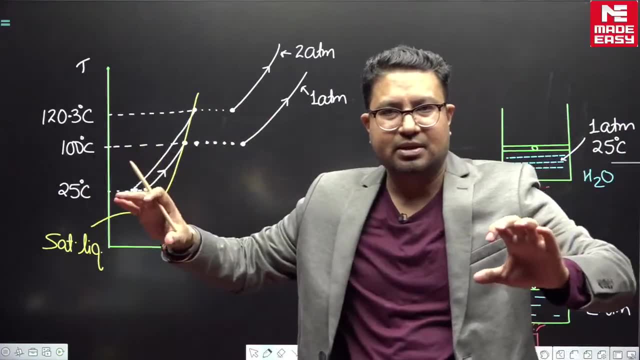 we call it saturated liquid curve. We call it as saturated liquid curve. We call it as saturated liquid curve. I have also written here everything. I have written here, many things which are very important to us. I have already written here. This is also an important 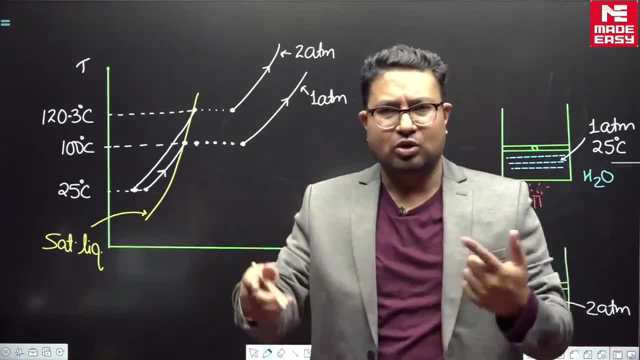 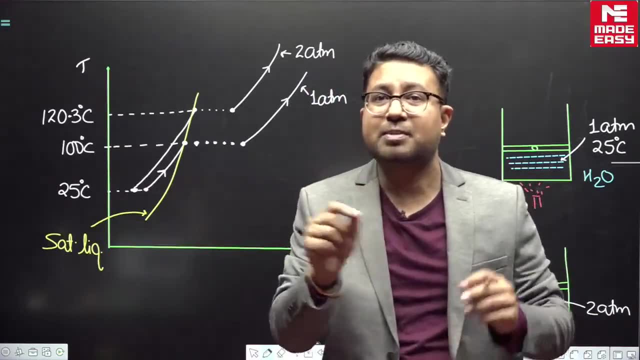 thing for us, The things which are the most important to us, which is very important to have already written here So that we do not waste our time in writing. you can just I will show you whatever I will speak and what it is relevant to you. examination purpose point. 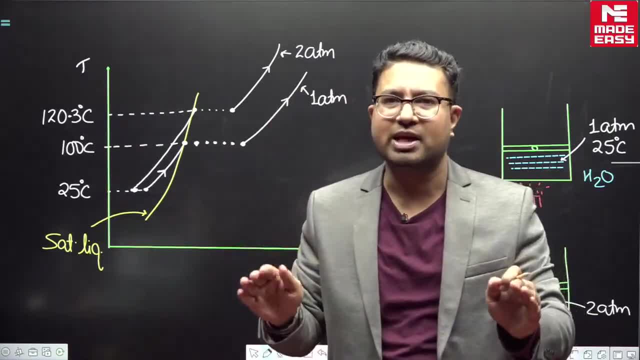 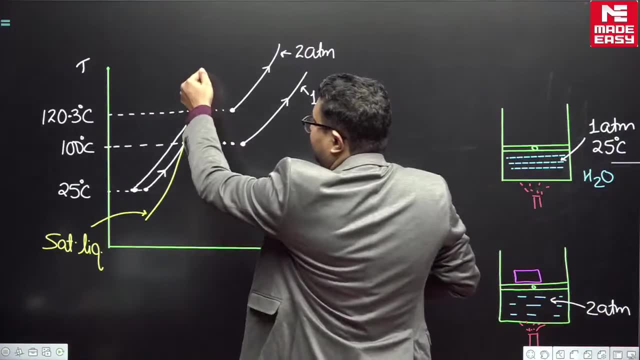 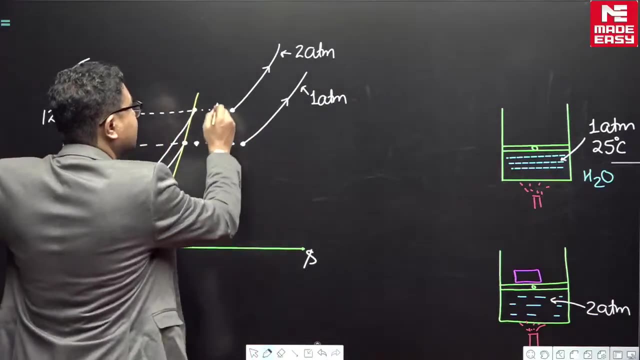 relevant notes that I have already written, So you need not worry about that once I will show you. if you want to take up a screenshot or something, you can do that Now. now these: these are the saturated liquid conditions. similarly what I did, I joined those conditions. 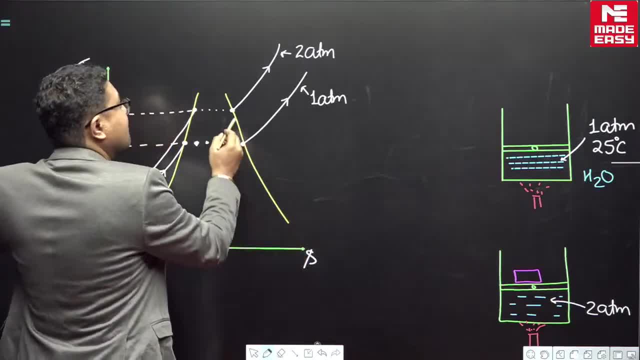 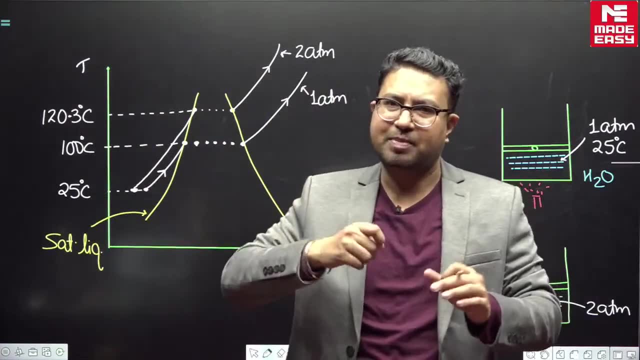 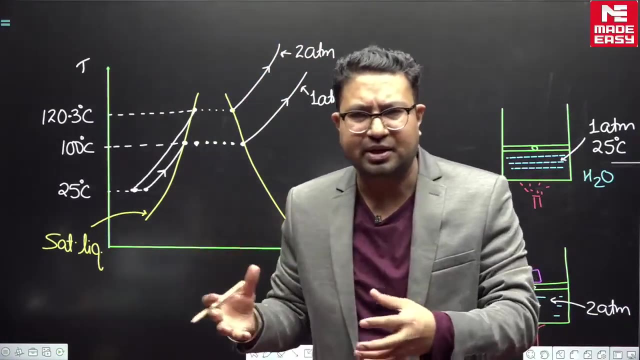 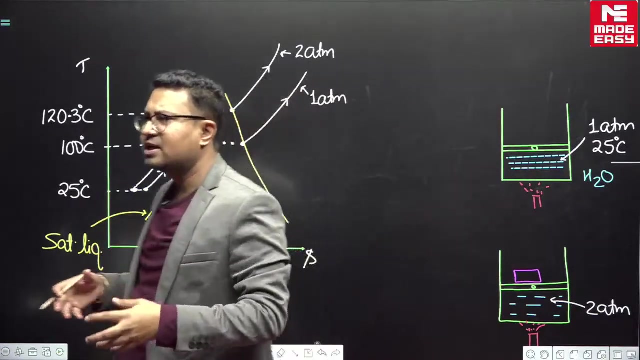 I joined those conditions where the, where the vapour was formed, and the vapour formed after that further heat will go into super heating. we call it super heating. So this, all the saturated vapour points, we joined. all the saturated liquid points, we joined. many experiments were conducted. we joined the saturated liquid points with a smooth. 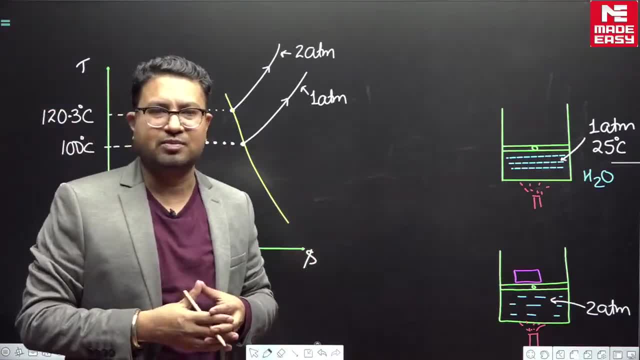 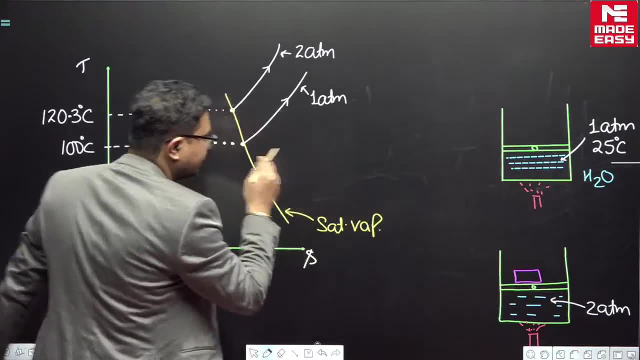 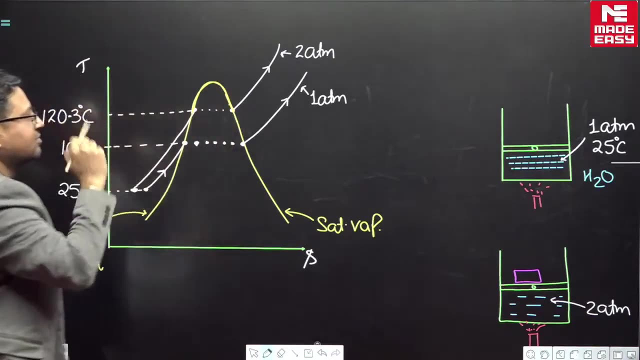 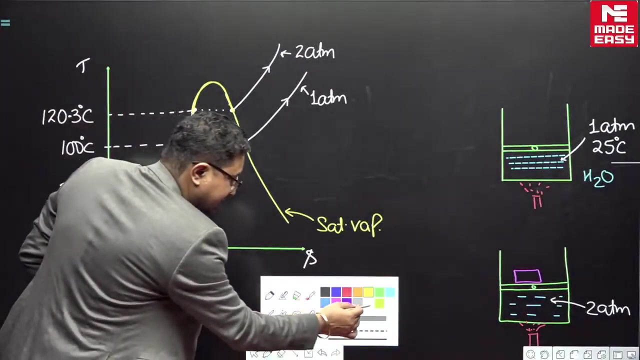 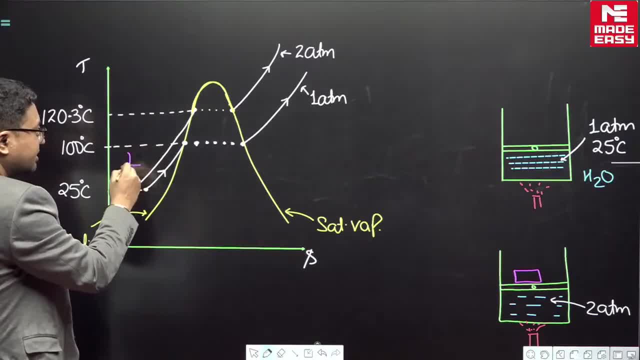 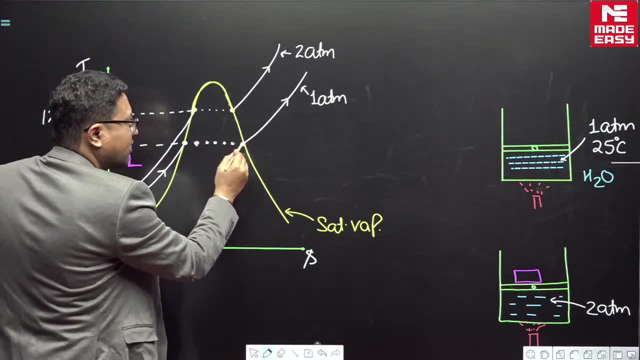 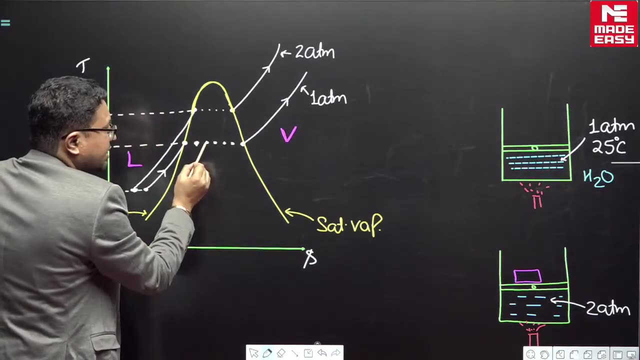 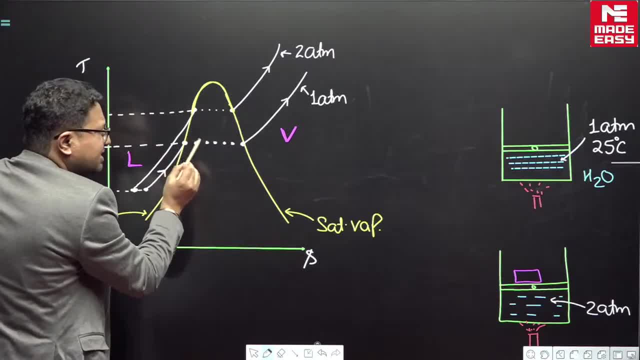 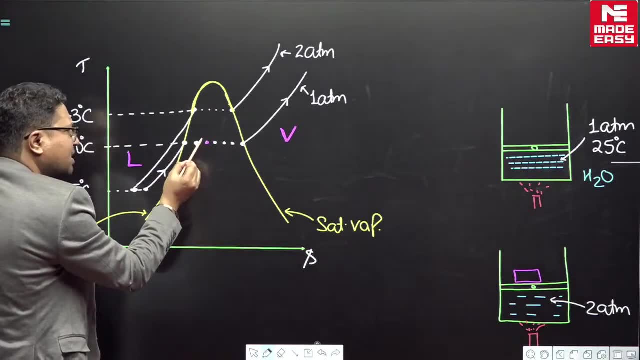 point on this side. when a point is marked this side, then the person is trying to say: suppose I marked a point here. I said this is the condition of the system, this is the temperature and this is the entropy. suppose I mark the point here. I will say, I will say: 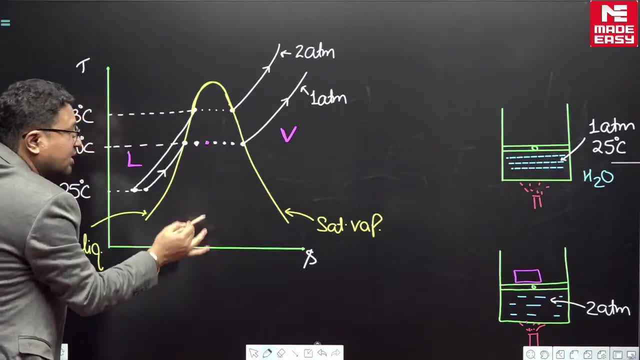 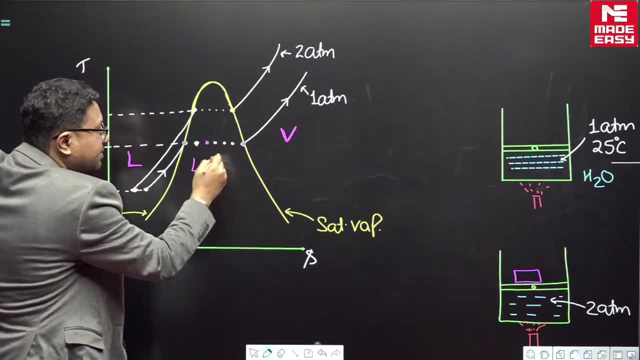 this, that if I am marking the point here, if I am marking the point here, then we have some of the mass as liquid and some of the mass as vapour. So that is why we call it as liquid plus vapour. there is no substance of this condition. 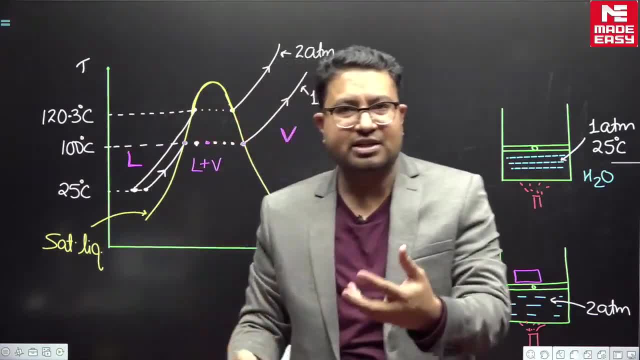 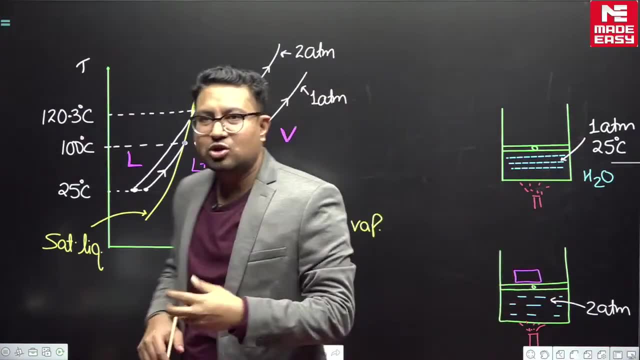 this condition ko substance nahi hai. it is just the average. it is just the average. there is a substance of this condition and there is a substance of this condition. this is just the average. And we also call this region hum is region ko bollte hai wet region. why? 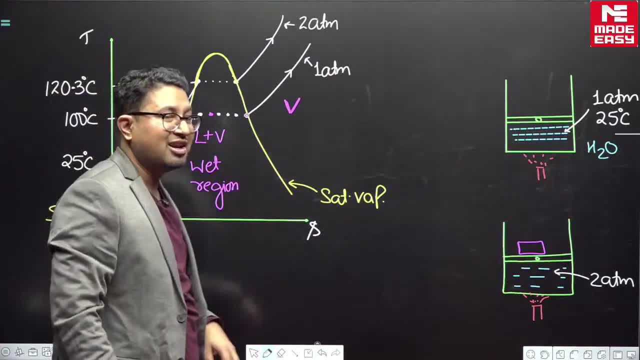 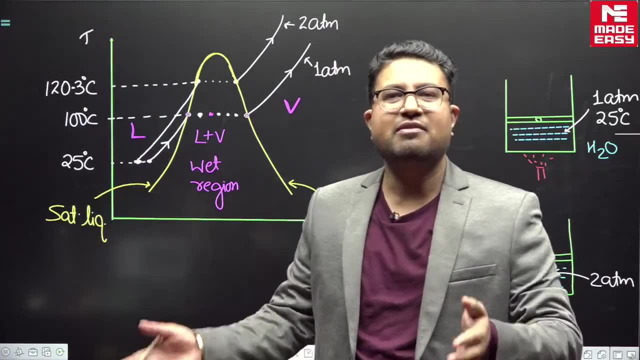 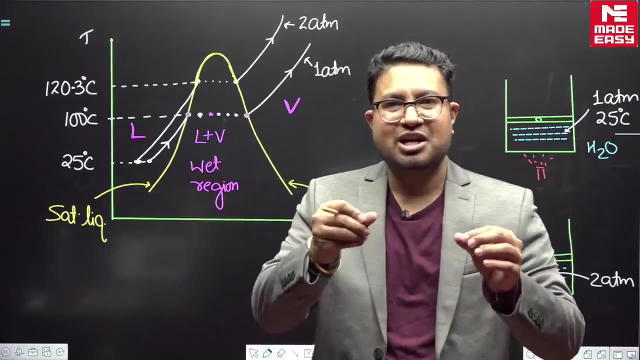 wet liquid has a wetting action. liquid ka wet karne ka action. wada gila karne ka. wet means gila karna. liquid has a wetting action. so because the liquid is present with the vapor, liquid present hai vapor ke saath, toh abhi bhi now also there is wetting action, if you will put this substance. 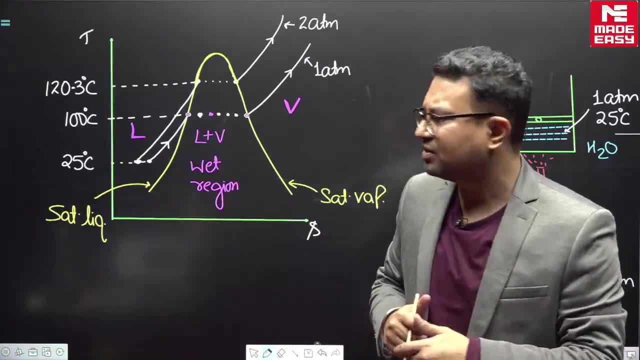 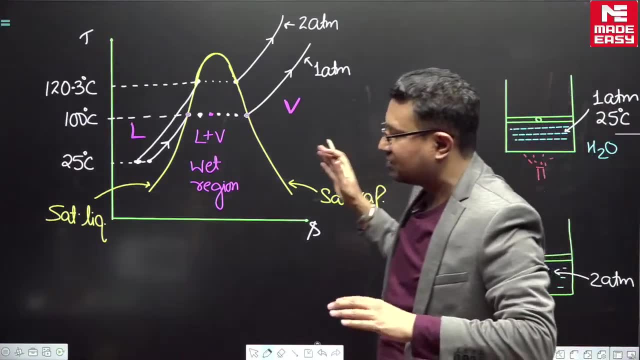 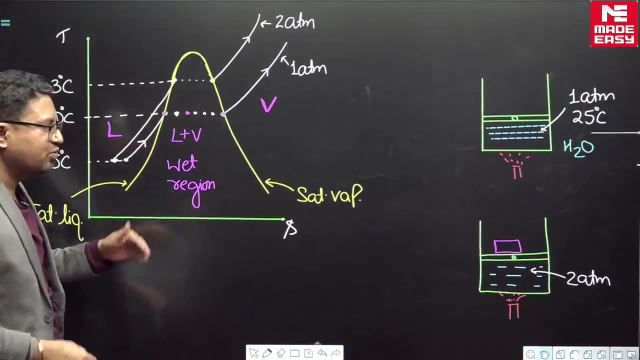 somewhere it will wet the surface. hu gila karega, wet karega. toh we call it as wet region. wet region, bolte hum isko tike. this is how we get the saturation curve. saturation curve, hume aise milta, experiment se milta hai now. now let us move forward. thoda sa aage baat karte hai. 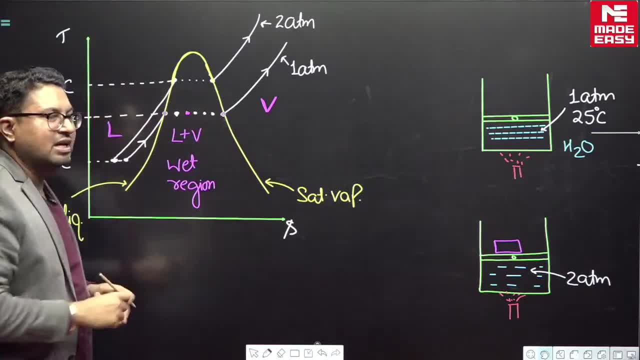 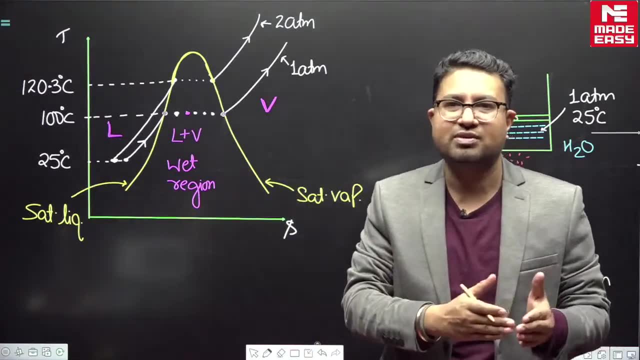 about these region in regions ke baare me thoda sa baat karte hai. let us talk about this, these regions. so i just discussed maine just abhi ye discussion kia ki how the saturation curves are formed. saturation curve kaise bante hai. i will just minimize it, jo discussion. 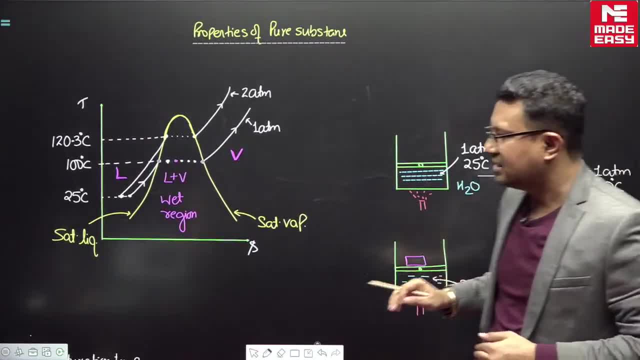 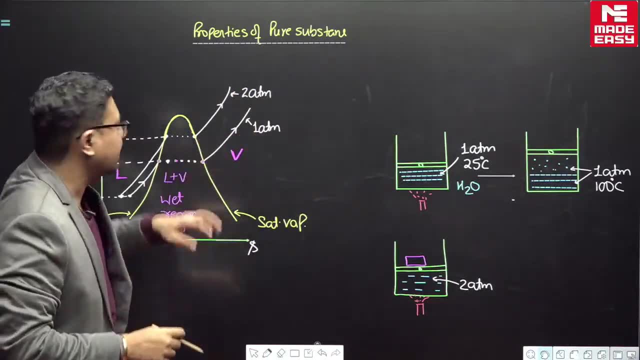 maine abhi kia hai, just thoda sa minimize karke aapko dikha raha ho, and then we will move on to the different region. We will talk about this region. we will talk about this region. we will talk about this region. hum baat karege will talk about this region, and we will talk about this point ye. 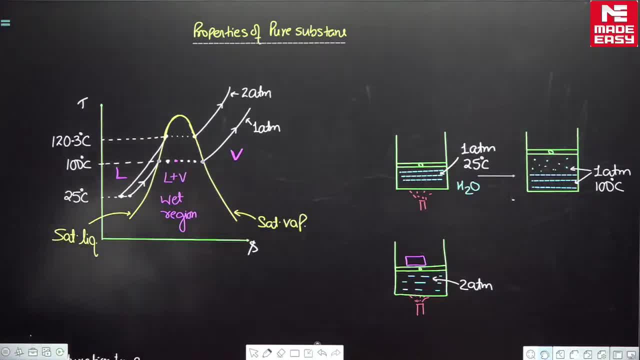 sari baat hum karenge. just i am giving you a moment, i will show you here. and lehkharaj wet region, you are saying, is moisture. see, when we say moisture, that is the vapor form of the h 2 o. waa h 2 o ka vapor form hai. waa h 2 o ka vapor form hai. 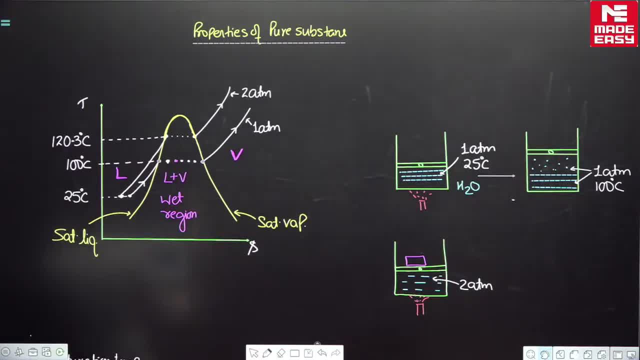 Now, If we see the here wet region, we have some liquid and its own vapour mixture. liquid and its own vapour mixture, not air mixture. air is not present with it. there is no air present in between. Now, here see Vishal Singh by: V f is decreasing. no, no, V f is not decreasing, I will talk about. 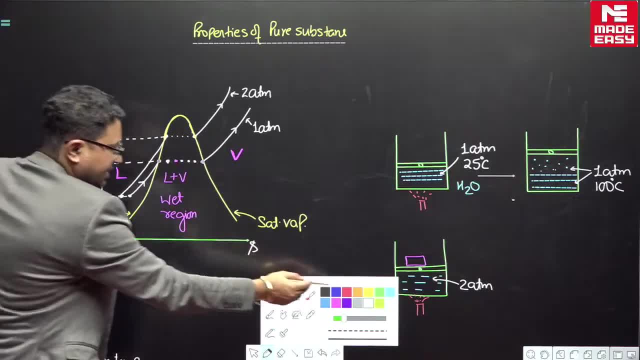 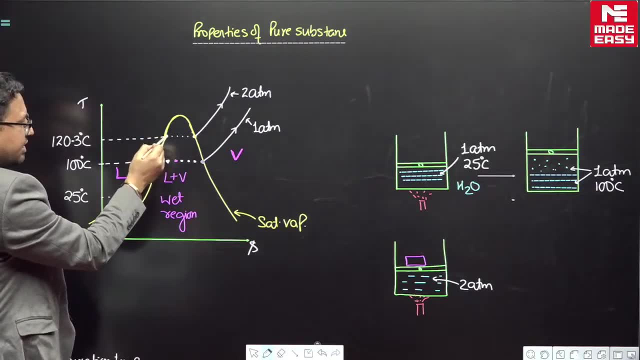 what is V? f? but if you see the volume, then it is increasing. Vishal volume is increasing. If you see the saturated liquid volume here, then saturated volume liquid will be here more than this. here volume will be more compared to this. we will talk about this, we will. 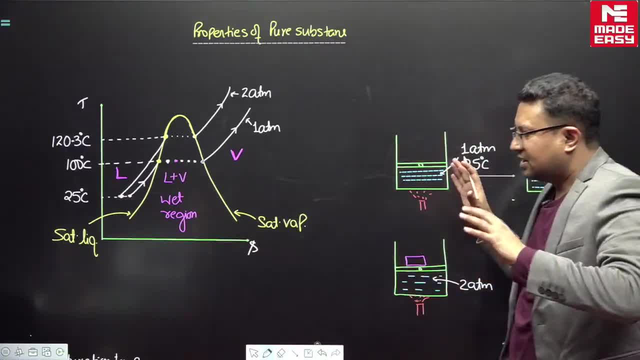 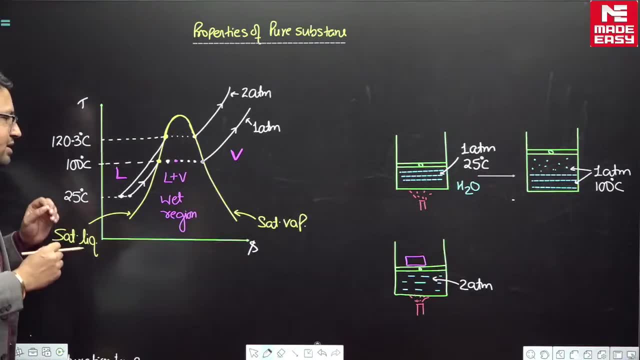 talk about this, But I just Just discussed. I just said that here we have the T S diagram. we have the T S diagram and this is how the saturation curve is made. fine, now let us move forward. let us talk. 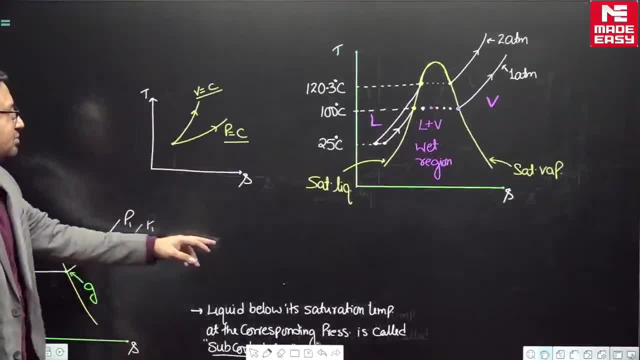 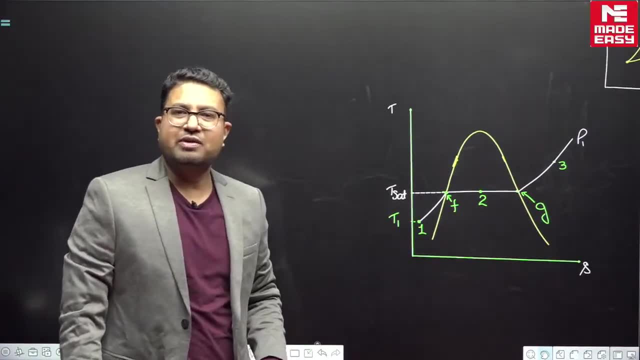 further. Now see here. let me show you a diagram. I have shown you a diagram here. this is a diagram. I have shown a diagram. So we will try to understand few things. we will try to understand some things. we. 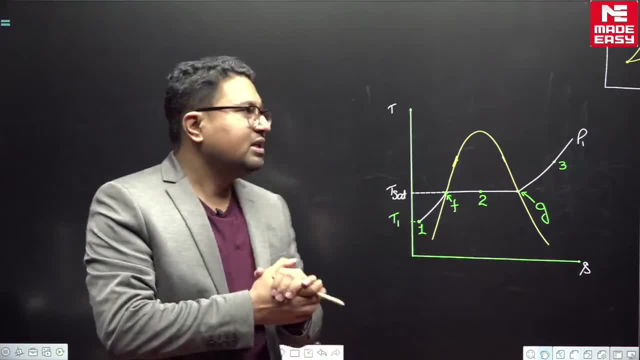 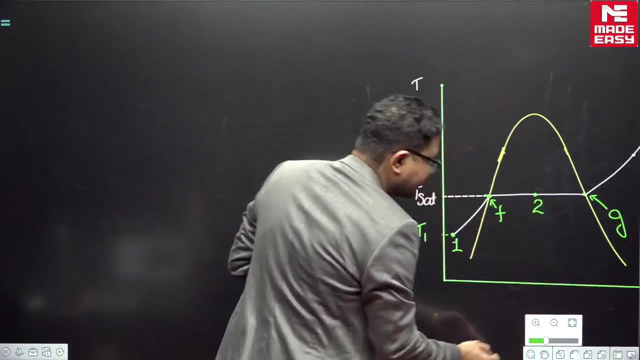 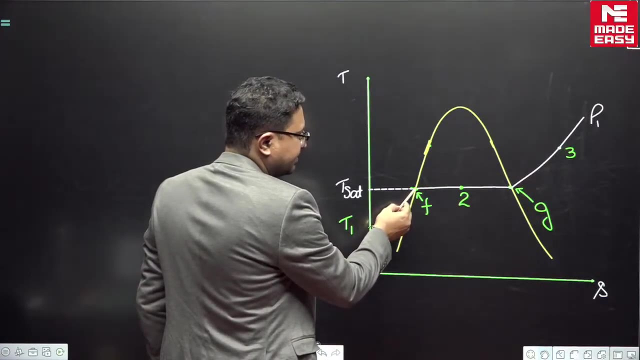 are trying to understand the regions. So this is a T S diagram, a T S diagram and this is the pressure curve. this is the pressure curve. this is the pressure curve which I have shown. Suppose you start heating from 1, so 1 say we will reach somewhere here, then heating. 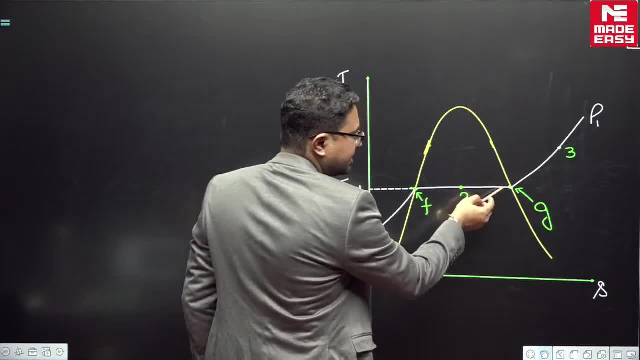 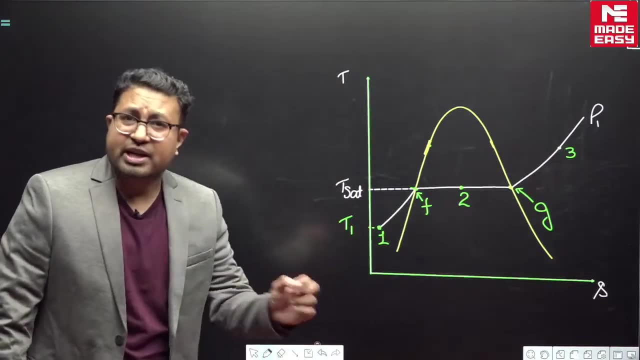 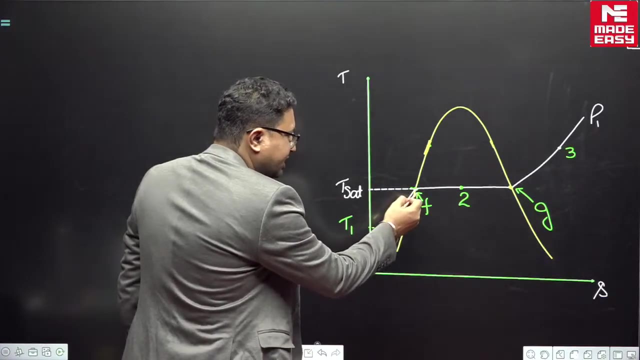 continue. temperature constant when the phase change is taking place, we will reach here, then the heating will continue and this will be curve. curve will be like this saturated liquid. So we will see: well, liquid is this also, and liquid is this also, so saturated liquid. 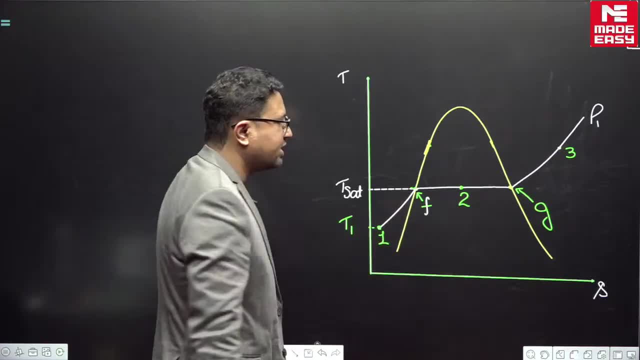 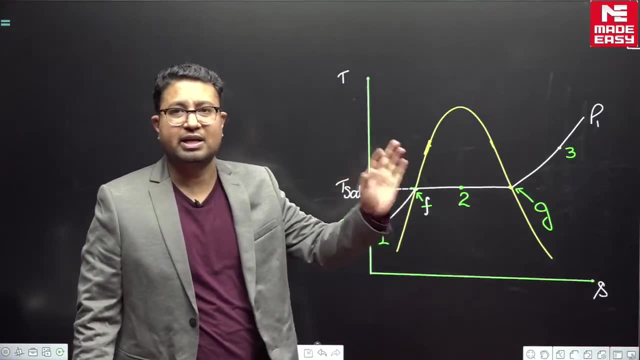 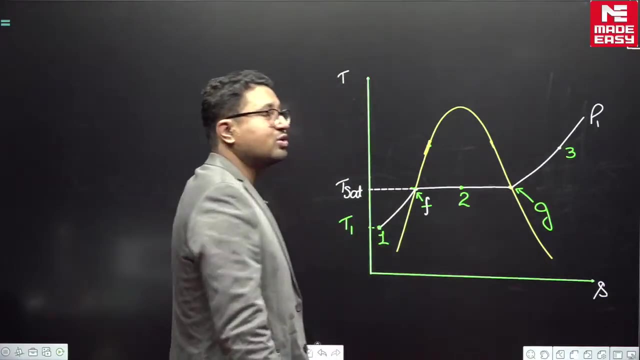 is denoted with F. F, say, denoted with saturated liquid, saturated liquid is denoted with F. So whatever are the saturated liquid points, point, you can take a subscript F, otherwise liquid is this? also, this is saturated vapour. now what is the saturated vapour? just formation. 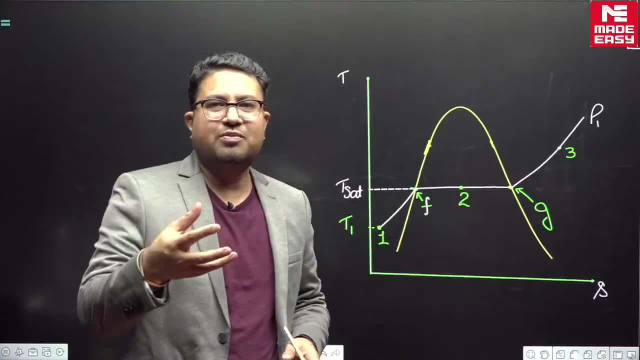 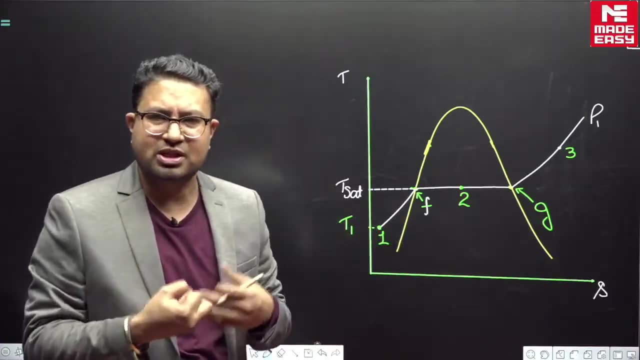 of vapour, Just formation of vapour. So if you remove some heat It will condense back. it will condense Just the energy which it has got is to change its phase. it just got the energy for phase change. 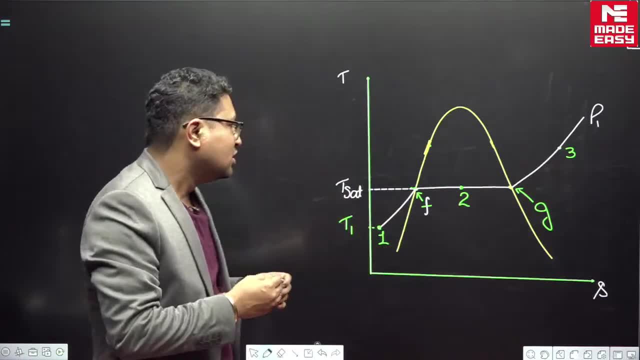 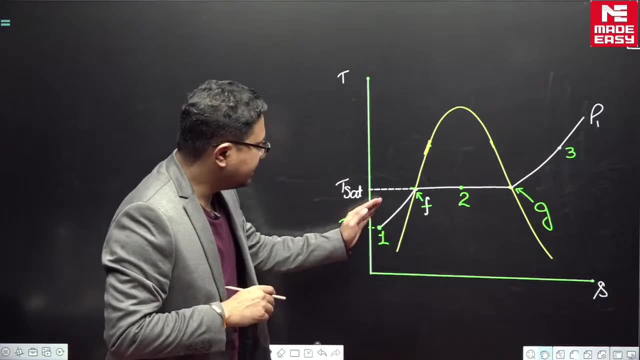 If you remove that energy, it will condense back. it will condense back. So this is the saturated vapour. this is the saturated vapour Now if you heat this, so this will go like this, and this is the entire curve. this is. 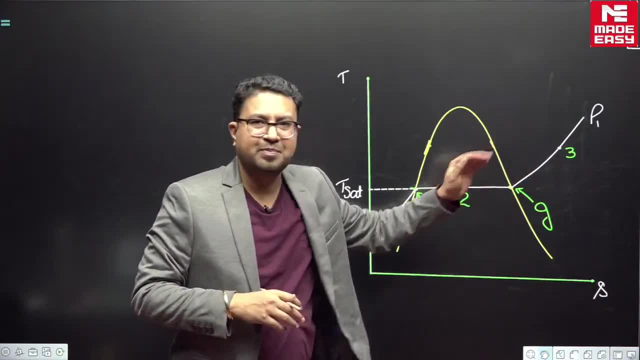 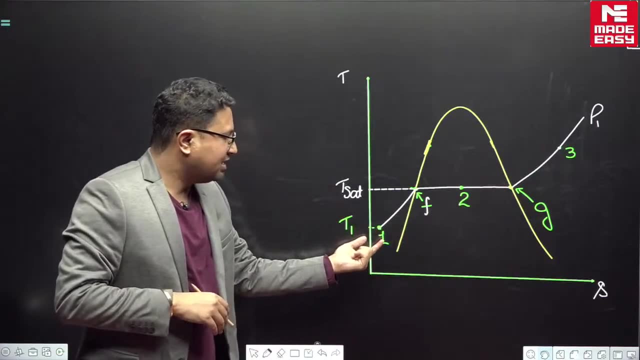 the entire curve starting from here and here. Now I have marked points: Point 1,, point 2,, point 3, point 1, point 1 is called as sub cooled region. Point 1 is called as sub cooled region. 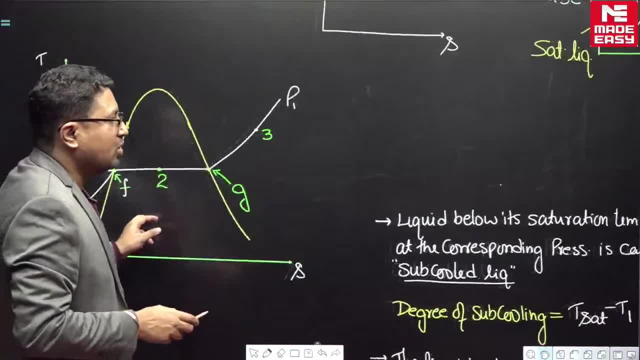 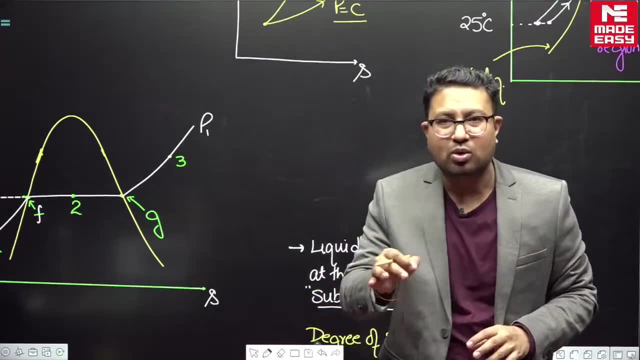 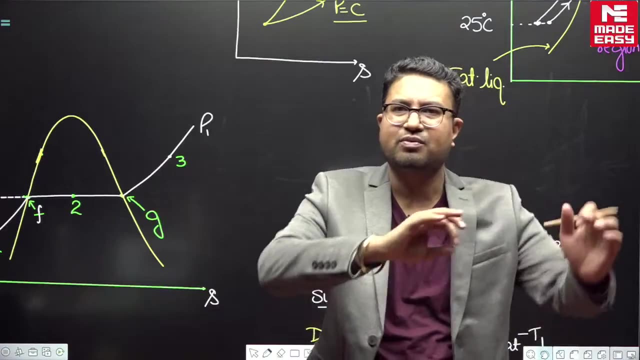 See. liquid below its saturation temperature at the corresponding pressure is called sub cooled liquid, Liquid below its. I have written it. I have written it because I do not want to take tension to write Whatever is relevant for the examination point of view, whatever should be in your notes. 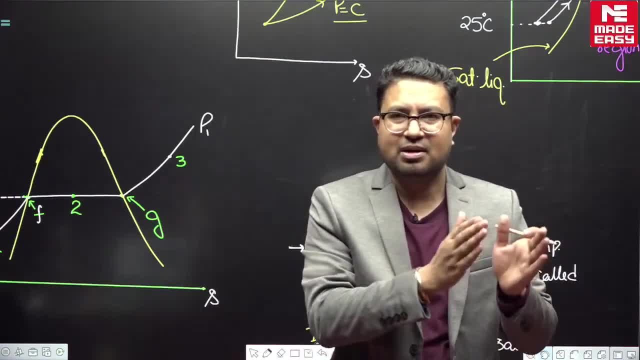 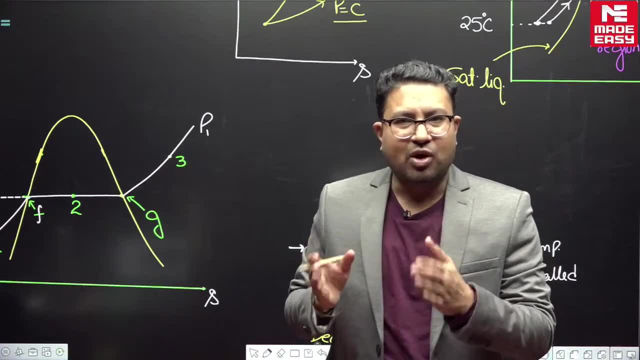 sometimes it should be in your notes. Sometimes it should be in your notes. So for this topic, that I will. I mean I have already written and I will show it to you. I will show it to you on the board. So now, what is the sub cooled liquid? 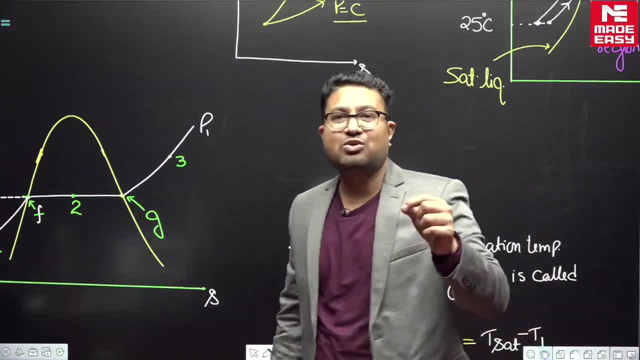 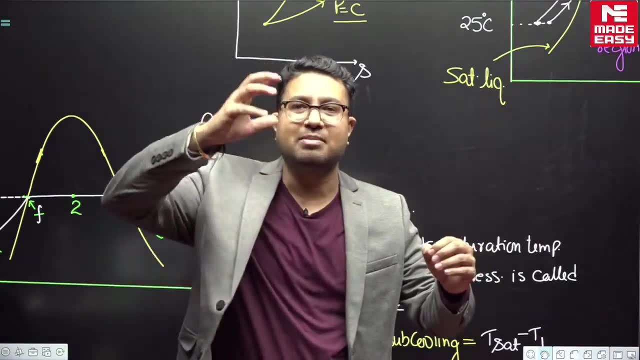 What is sub cooled? See what is the meaning of sub cooled. Suppose I have water at 25 degree Celsius. is there water at 25 degree Celsius? One atmosphere, When there is boiling at one atmosphere means when the water becomes becomes saturated. when the water becomes saturated At 100 degree Celsius. Depending to one atmosphere, water becomes saturated at 100, now it is at 25.. So what is the definition of sub cooled Liquid below its saturation temperature? below its saturation temperature at the corresponding 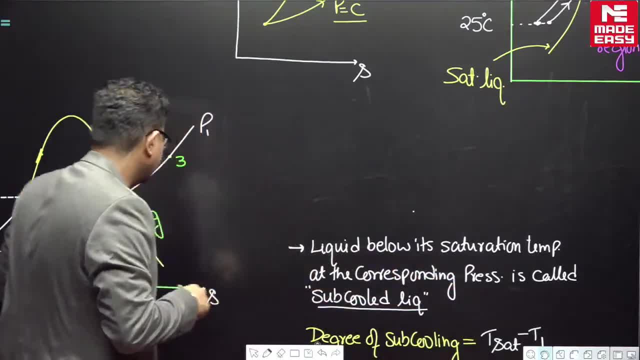 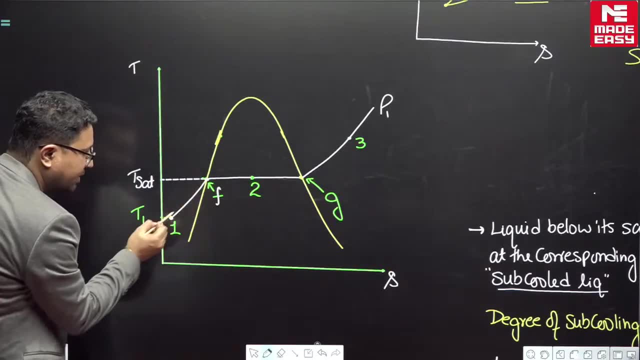 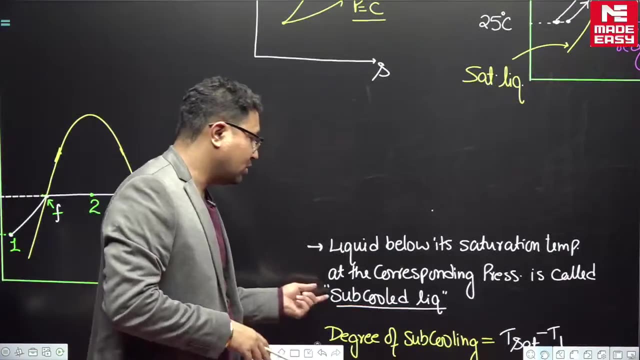 pressure. at this pressure you become saturated here, but you are at a temperature below that, so you will be called as sub cooled liquid. What will you be called Sub cooled liquid? You will be called as sub cooled liquid, So we call it as sub cooled liquid. 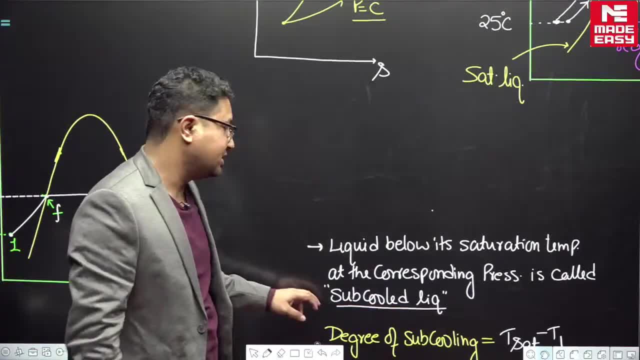 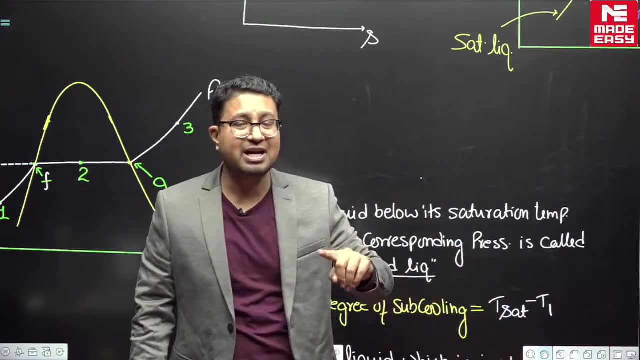 What do we call this Sub cooled liquid? What is the degree of sub cooling? What is the degree of sub cooling? Degree of sub cooling is equal to T saturation minus T 1.. What is the degree of sub cooling? T saturation, that is, saturation temperature. what is it? 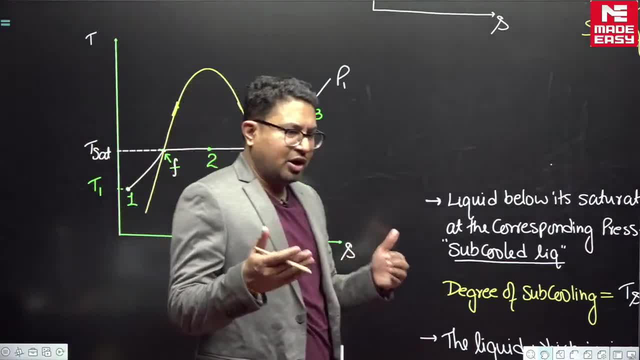 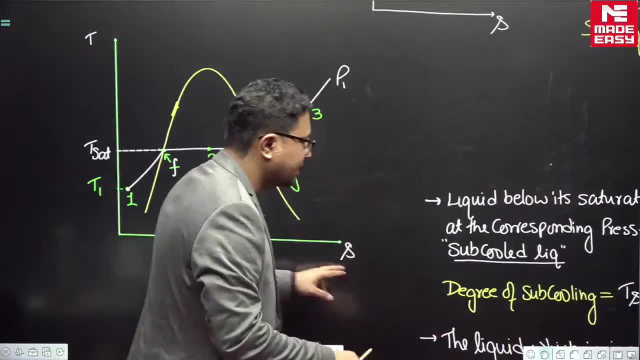 Minus. what is your temperature now, For example, if we talk about water at 25 degree Celsius, one atmosphere, one atmosphere where water boils at 100.. So what is saturation temperature? Saturation temperature will be 100, now it is at 25, now it is at 25,. so degree of sub. 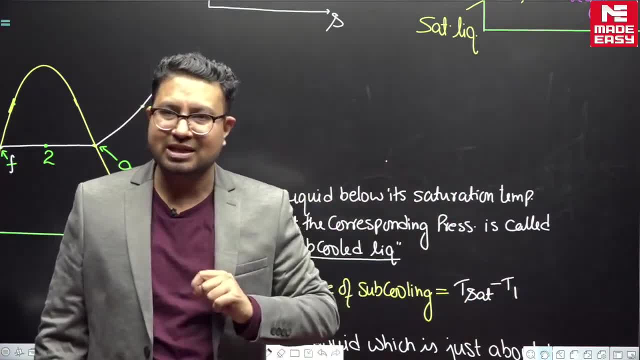 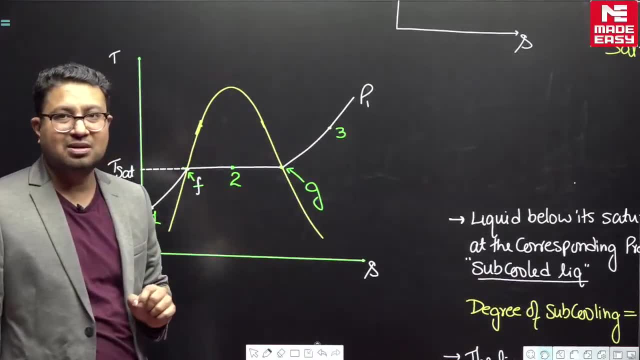 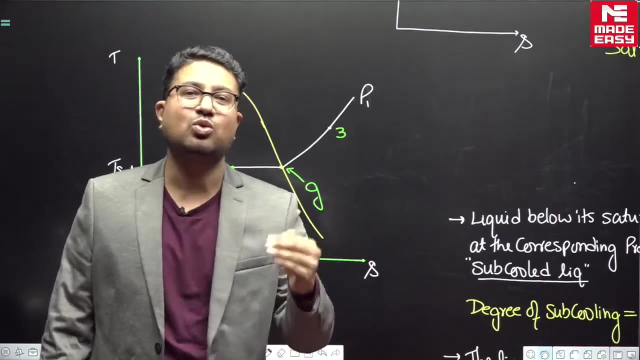 cooling is 100 minus 25, that is equal to 75,. sub cooled liquid is also called as under cooled liquid. sub cooled liquid has one more name. there is one more name that is called as under cooled liquid. it is called under cooled liquid. under cooled liquid is called: 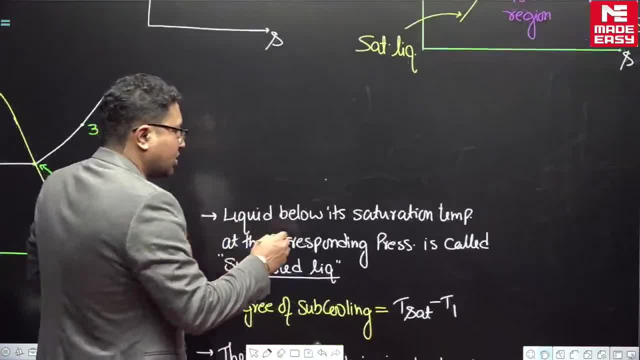 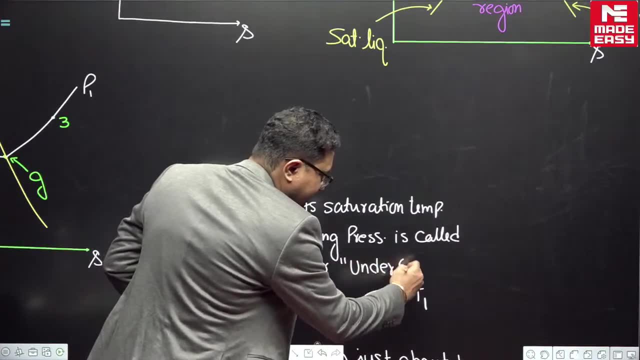 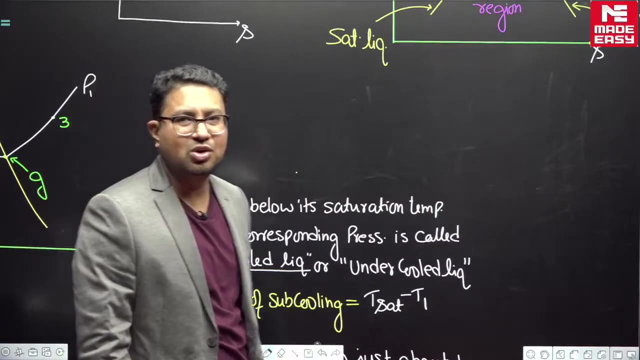 as under cooled liquid, sub cooled liquid, or, or, or. it is called as under cooled liquid. we call it as under cooled liquid, under cooled liquid, under cooled liquid. there is one more name. generally it is not written, but it may be. I mean, you may face it sometimes. 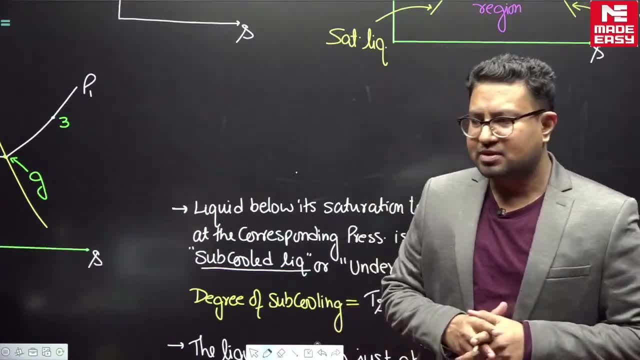 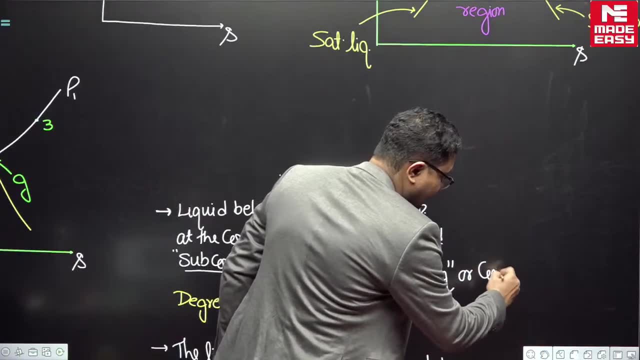 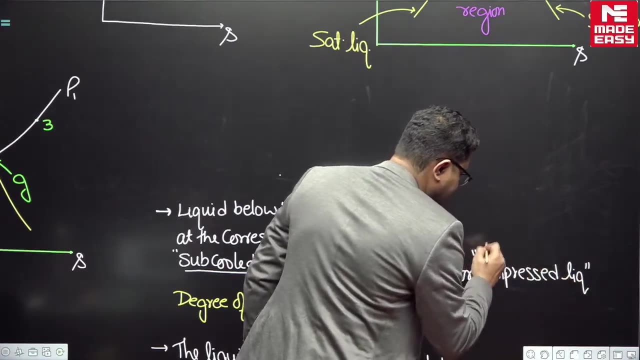 it may come in front of you. So there is one more name. there is one more name that is called as compressed liquid. what is it called? liquid? or? or? it is also called as compressed. it is also called as compressed liquid, hum. 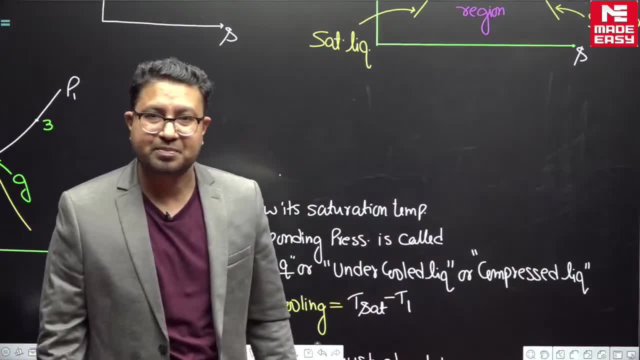 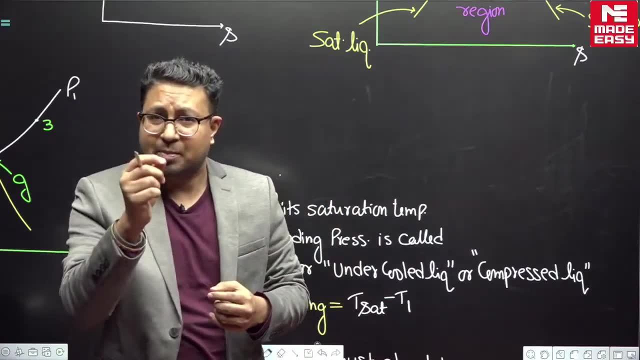 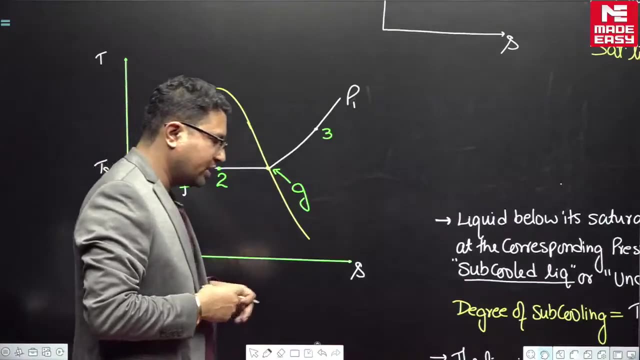 compressed liquid bhi bolte. it is also called as compressed liquid. So sub cooled liquid or under cooled liquid or compressed liquid. deko compressed liquid, kyo bolte. uska reason hai? try to understand this. try to understand this when I called it as sub cooled liquid. 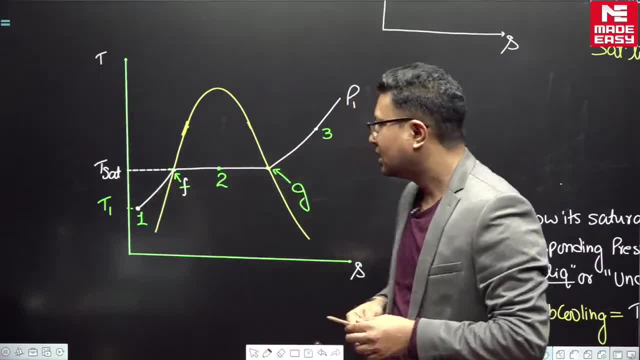 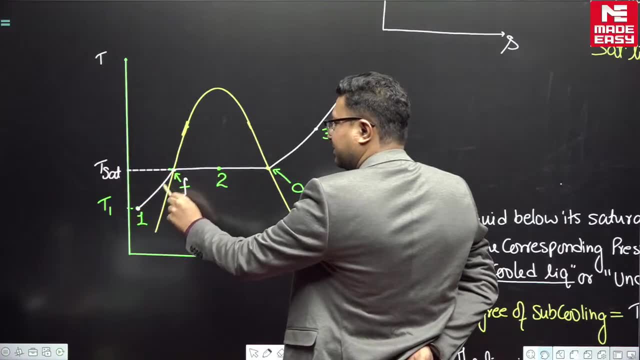 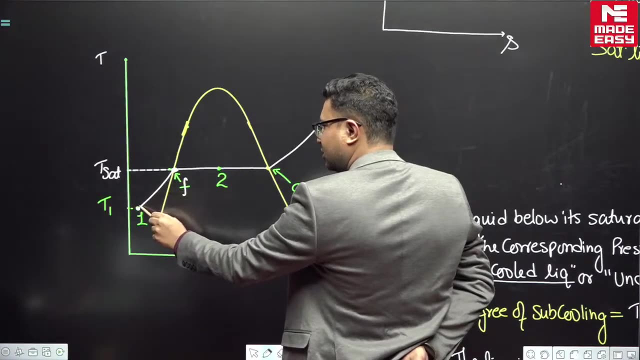 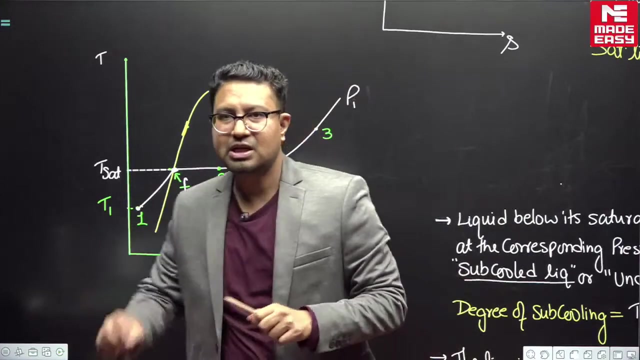 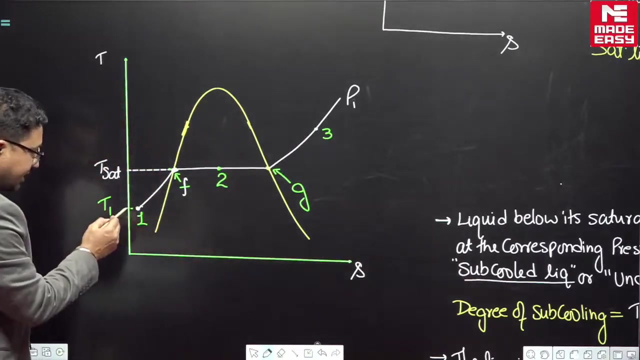 When I said sub cooled liquid, then what I said, I said at the same pressure, at the same pressure, saturation temperature: is this saturation temperature? is this? you are here. You are here. so below your saturation, sub cooled. okay, now you will see. we will compare at the same pressure. now, if I compare at the same temperature, same temperature, same temperature, if you would have been saturated, if you would have been saturated, then where you would have been? you would have been here, yes or no. 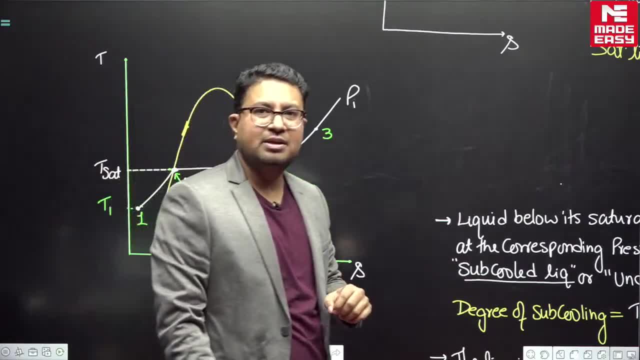 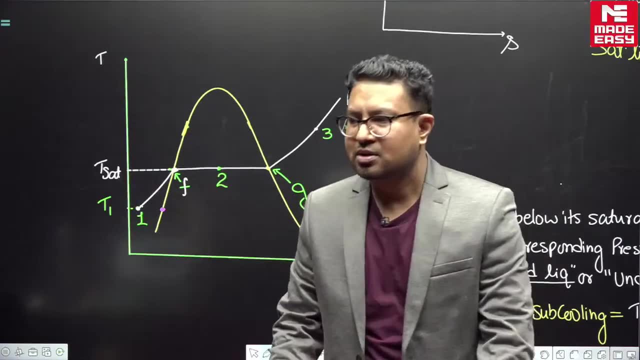 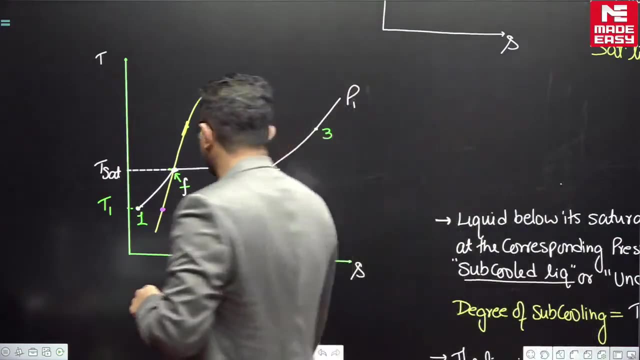 at the same temperature, isi temperature pe, if you would have been saturated. agar aap saturated hote abhi nahi hai, but if you would have been saturated, you would have been here. you would have been here. yes, now what the pressure would be here. yaha jo pressure hoga, agar aap dekho. 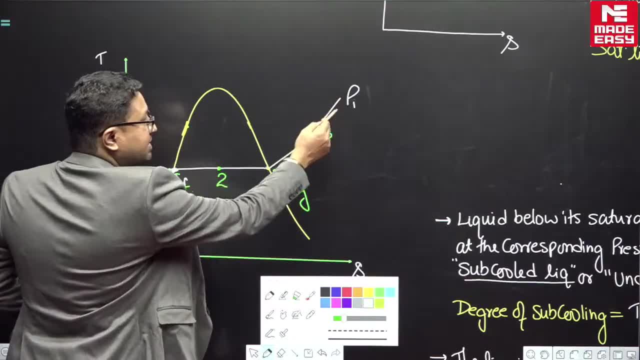 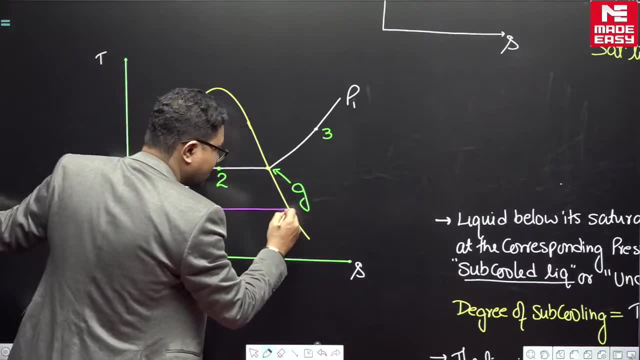 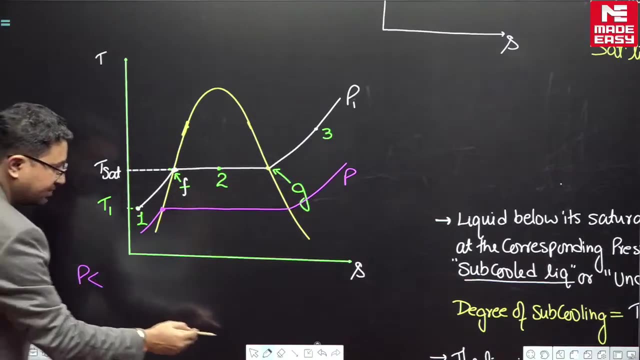 suppose here the pressure is p, p1, here is the pressure p1, maalo yaha pressure p1 hai. so here here, whatever pressure will be, yaha, jo bhi pressure hoga here, whatever pressure will be here, whatever pressure will be, p is less than p1, p kum hai p1 se. so if we compare, 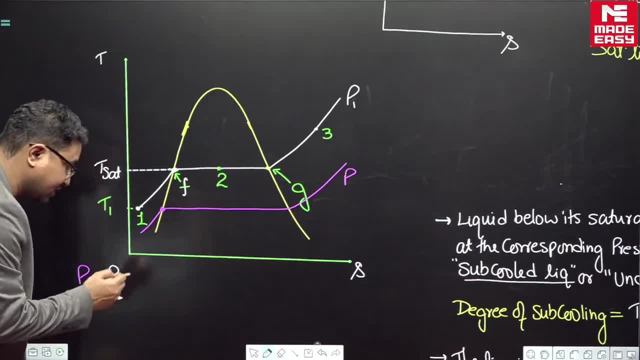 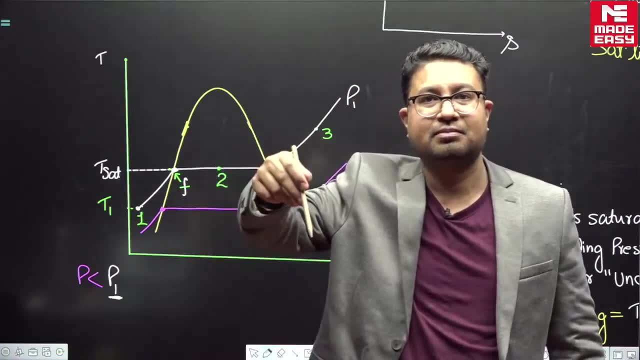 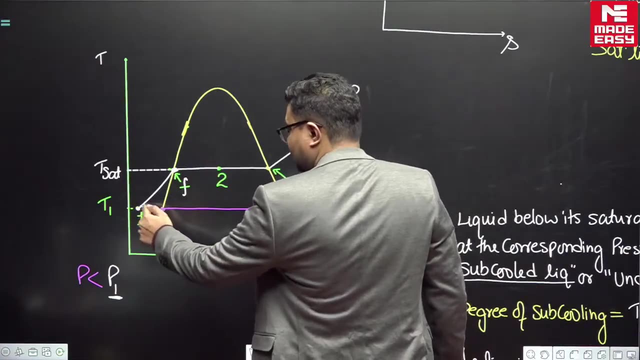 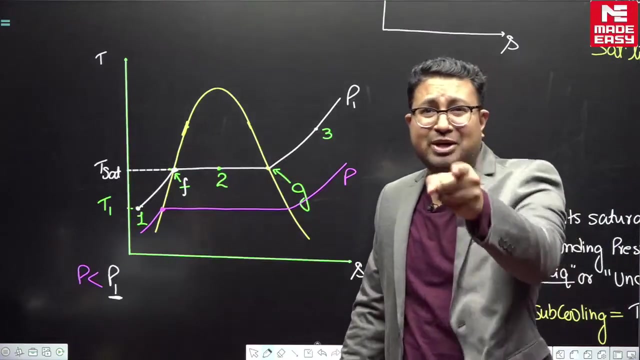 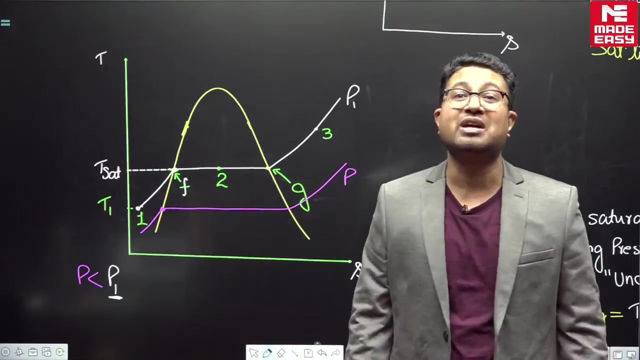 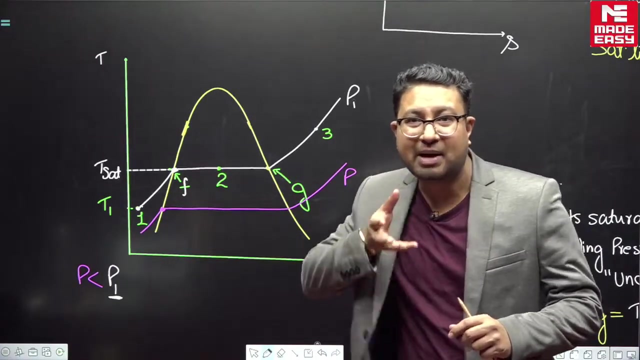 you are compressed means you are at a higher pressure. aap higher pressure pe ho issi temperature pe. if you have to be saturated, issi temperature pe agar saturated huna hai at the same temperature. If you have to be saturated, if you want to be saturated, then you should be here. you should be here, but you are here at a higher pressure. So if your pressure is dropped, if your pressure is also dropped, then you will reach the phase change condition. or you will reach the phase change condition. understand: boiling does not happen only by heating. 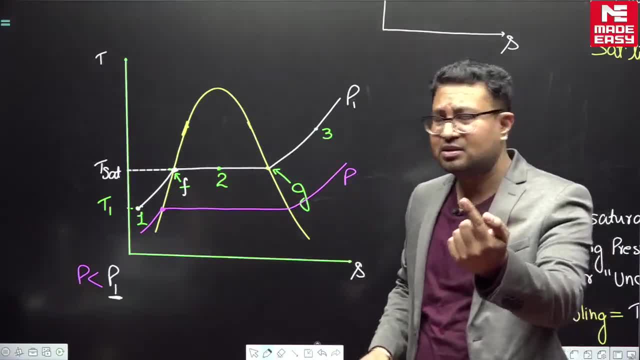 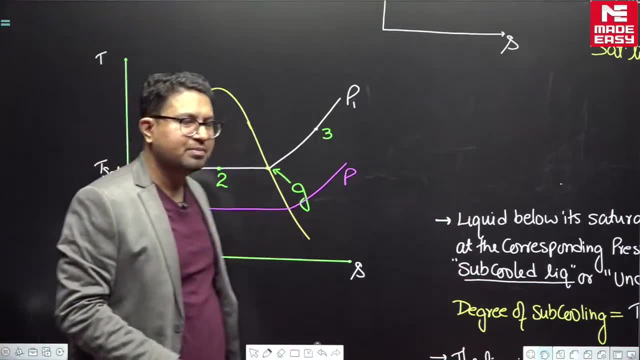 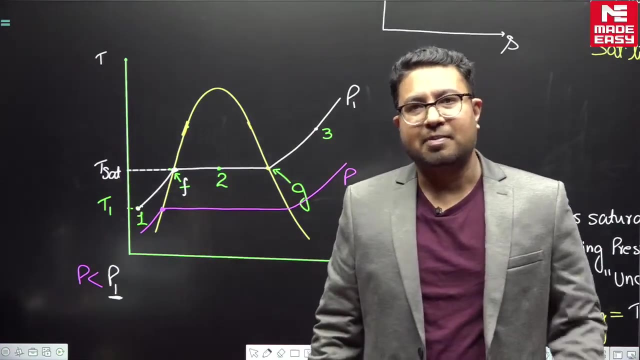 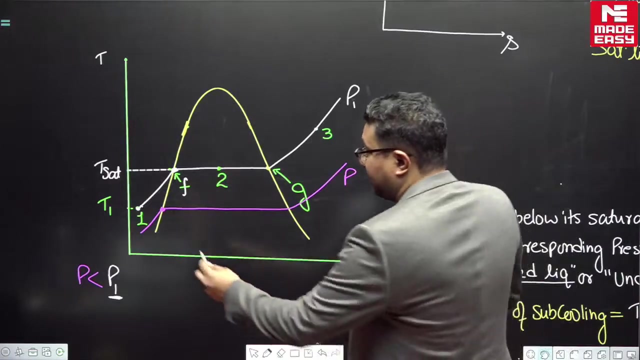 There is one method: If you are here, if you are here at constant pressure heat, you will reach the phase change condition. or you will reach the phase change condition. but it may be a case that if your pressure is dropped, if your pressure is dropped, you may reach the phase change condition. So if you want the water to boil at 25 degree Celsius, if you want the water to boil at 25 degree, then there will be a pressure for that also. You place a vacuum pump, drop the pressure, the water will reach its boiling condition. it will reach the phase change condition. 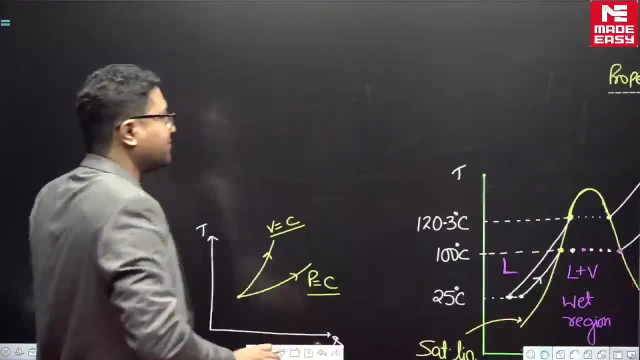 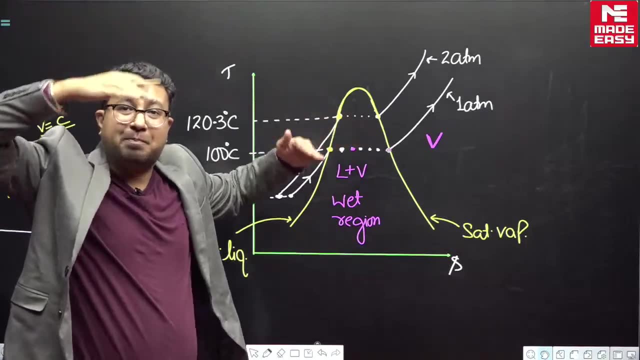 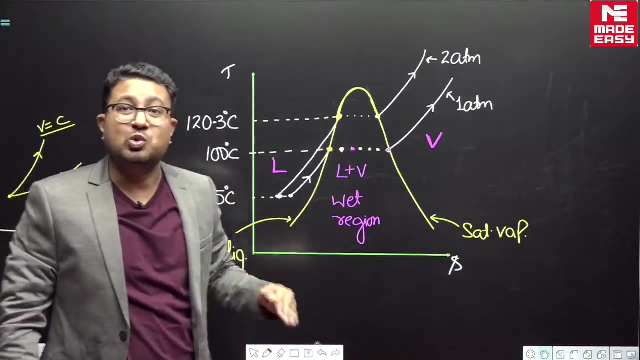 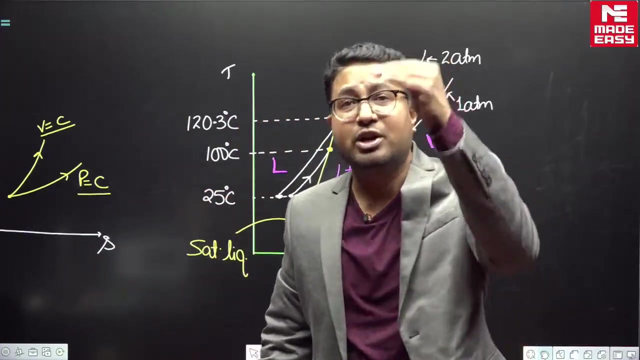 Understand if 1 atmosphere 100 degree Celsius, 2 atmosphere 120.3 degree Celsius, Pressure increase kar raha hai to boiling temperature is increasing. So if you drop the pressure, agar aap pressure drop karoge to, you can reduce the boiling temperature. the temperature at which the water will start boiling. jais temperature pe water boil karna start kardega wo reduce hota jayega. 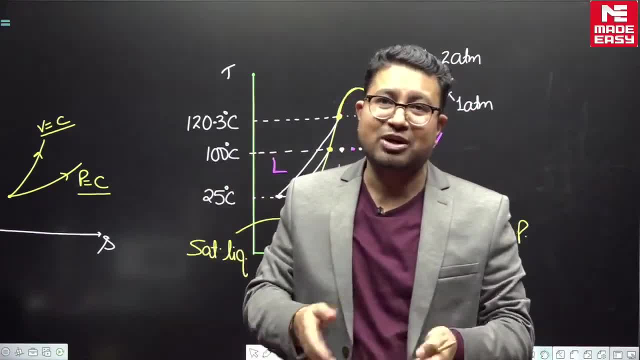 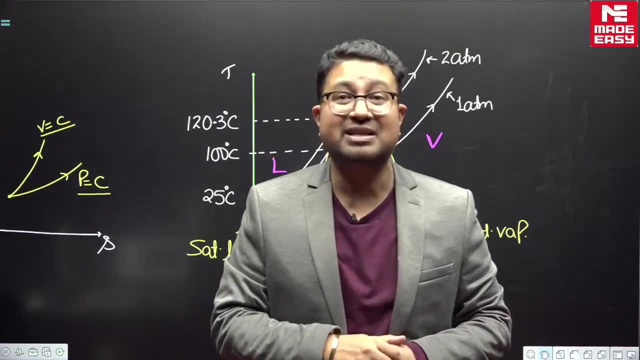 So there will be a temperature that you are at 25 degree Celsius, aap 25 degree Celsius. pe ho, you are at 25 degree Celsius and we have dropped the pressure. humne pressure, drop kar diya itna that you cannot exist. 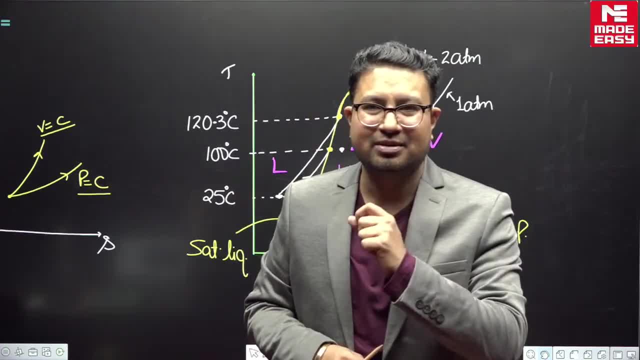 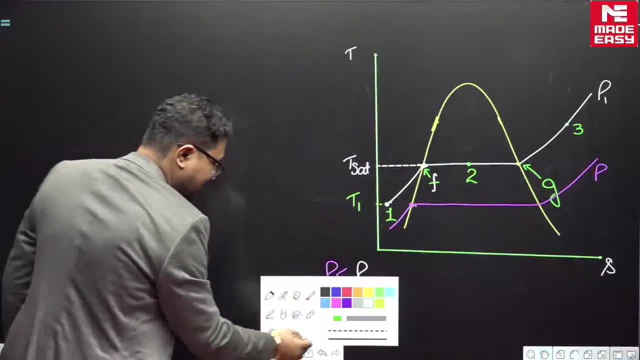 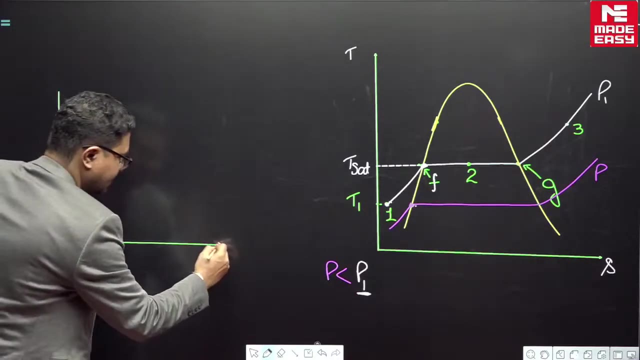 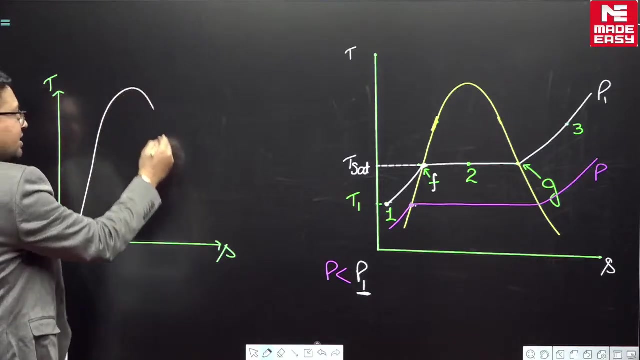 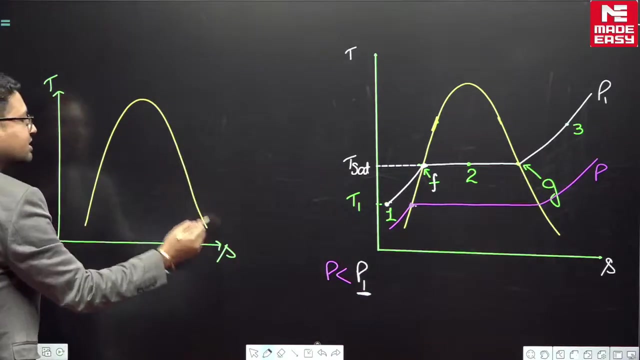 as liquid. Let me explain this to you. Suppose, suppose, suppose, if you see here, see here, see here, suppose this is the T-S diagram, this is the T-S diagram, and and we have, I will use the yellow color. Suppose this is the T-S diagram. this is the T-S diagram. fine, 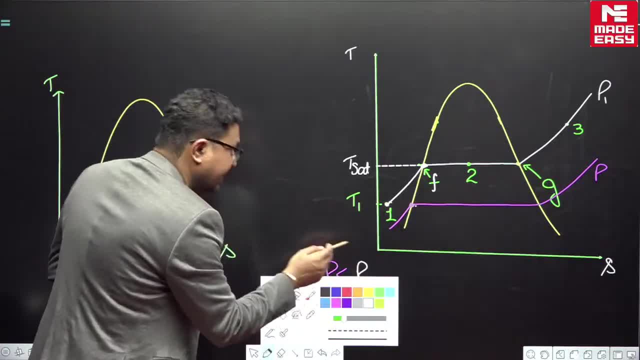 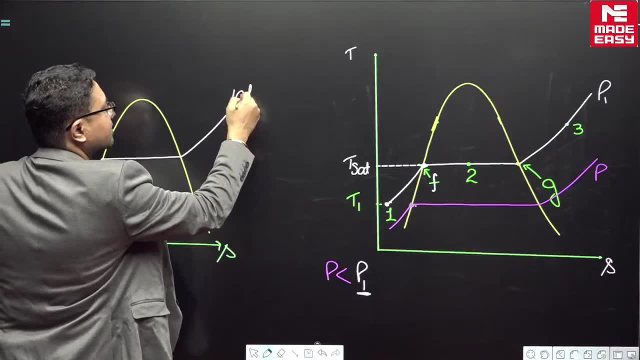 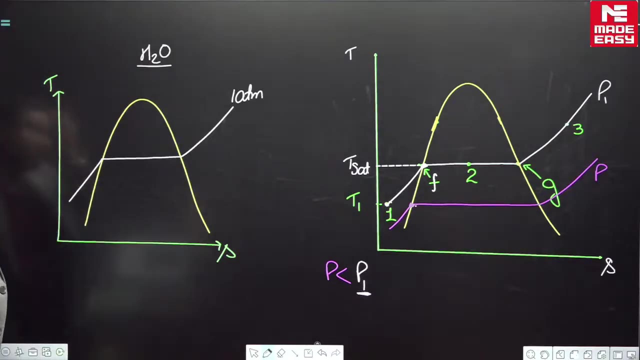 Now we have assume, assume, we have let us say this is: this is corresponding to 1 atmosphere, 1 atmosphere, What we are talking about. We are talking about H 2, we are talking about H 2, we are talking about H 2.. So we are talking about H 2, this is 1 atmosphere. 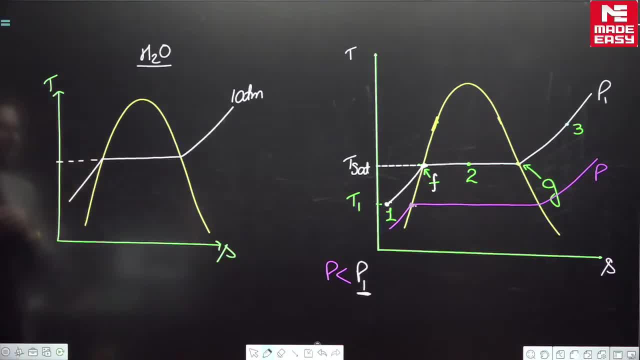 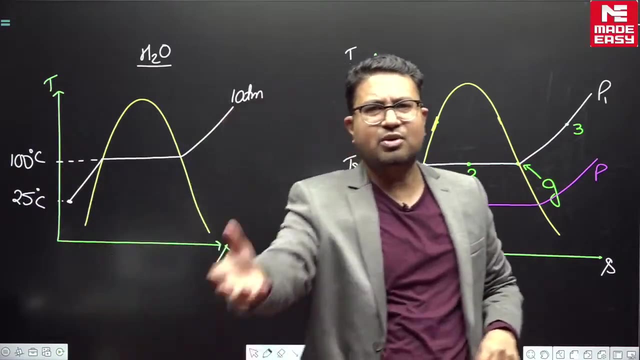 let us say, then we can say, we can say that here here, corresponding to 1 atmosphere, boiling chain takes place at 100 degree Celsius. you are at 25 degree Celsius, you are at 25 degrees Celsius. pressure is 1 atmosphere, So there is 1 way you start heating the. 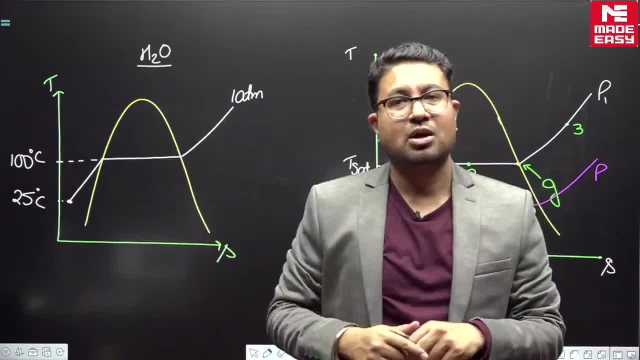 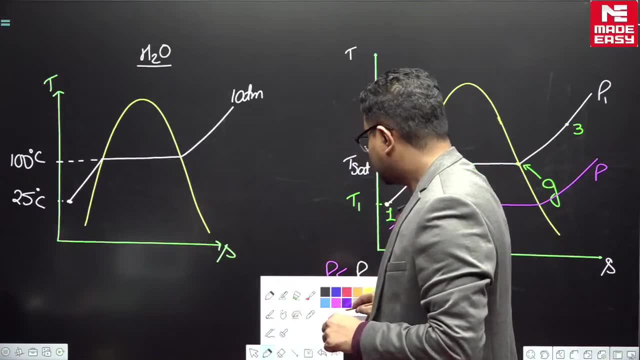 water, it will reach 100, pressure will remain same, Or what you do, you start dropping the pressure, start to drop the pressure. You dropped the pressure. Suppose you started reducing the pressure. you started reducing the pressure, So you brought it here you. 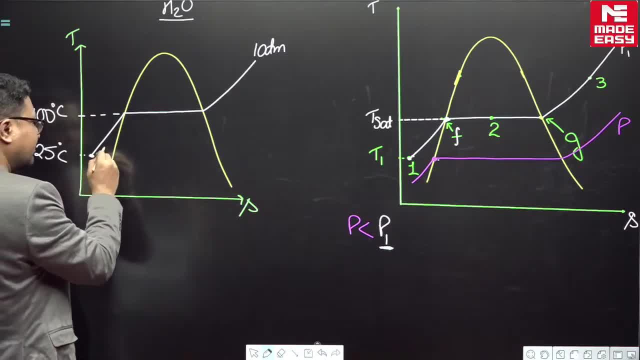 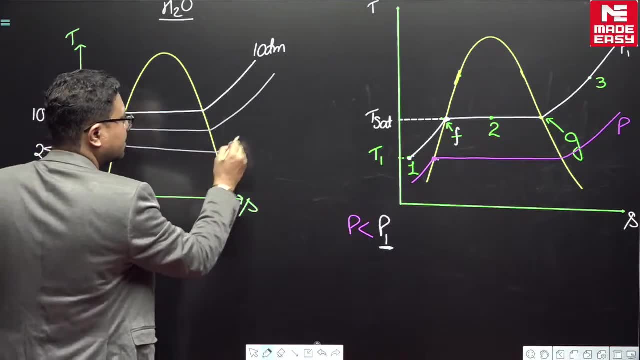 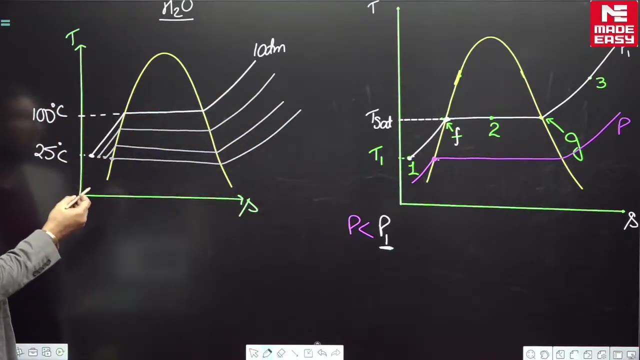 brought it here means it is 25 degrees Celsius, but you have dropped the pressure. you have dropped the pressure, then further pressure drop over. you have dropped the pressure, further pressure drop over. it came here at this condition here. after that, let us say: let us assume this pressure exactly one atmosphere is. let us 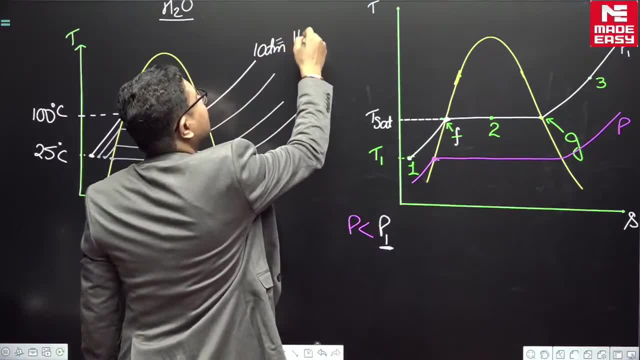 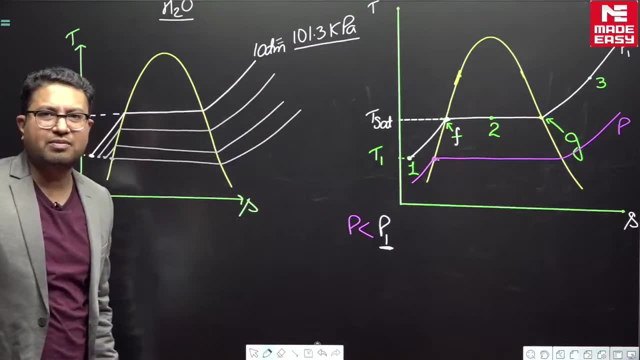 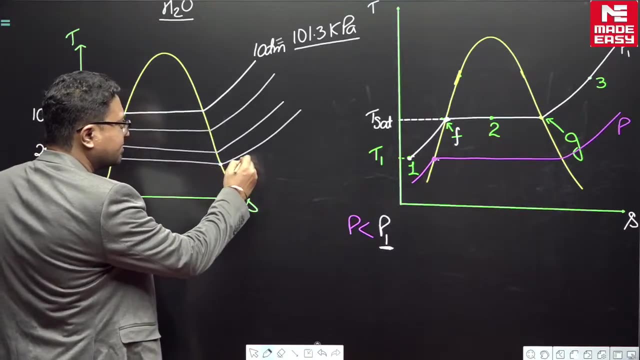 say the value comes out to be 101 kilo Pascal, 101 point something, 101.3 kilo Pascal. this is the conversion of atmosphere to kilo Pascal, so 25 degree Celsius. so here, suppose there is some pressure. I do not know the exact value. I do not know the exact value, but I am just 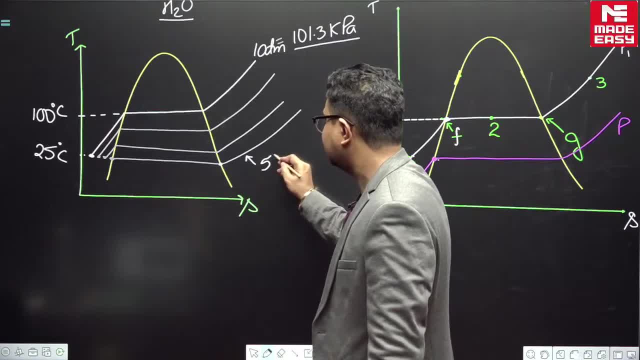 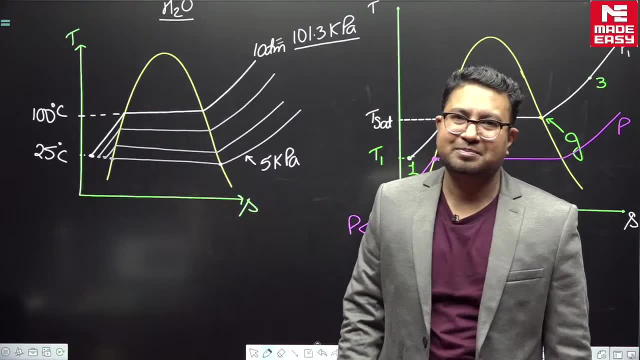 taking it for an example. suppose, for example, I take 5 kilo Pascal. 5 kilo Pascal, Let us say you have dropped the pressure to 5 kilo Pascal. you have dropped to 5 kilo Pascal. when you go down from 5 kilo Pascal, suppose I drop the pressure further 4 kilo Pascal, it is still. 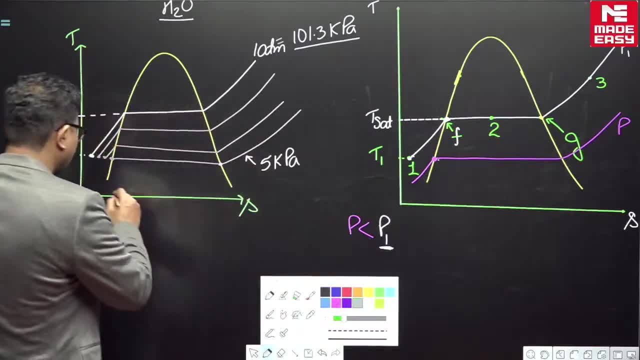 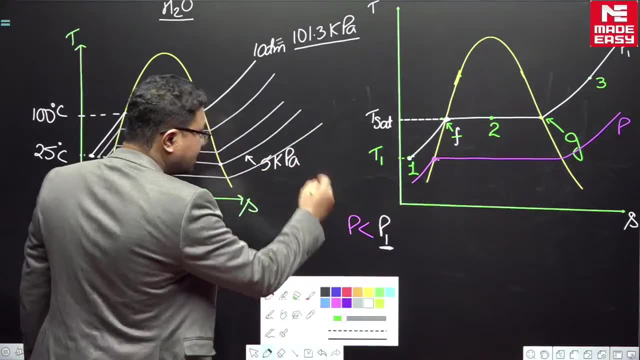 25 degree Celsius. pascal pe drop kar diya, suppose i drop the pressure. 4 kilo pascal toh. 4 kilo pascal pe samajhna, samajhna. this is, let us say, 4 kilo pascal. this is, let us say, 4 kilo pascal. 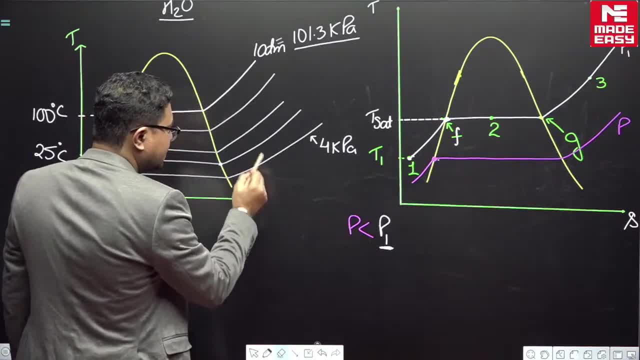 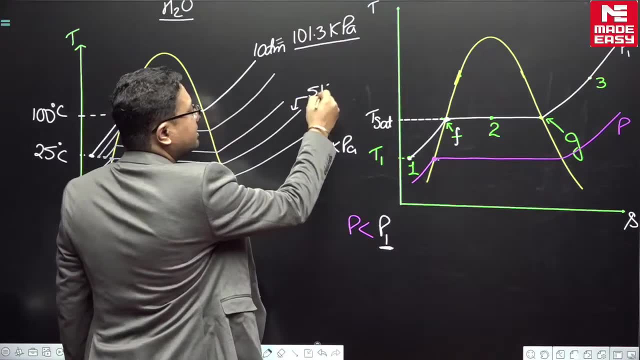 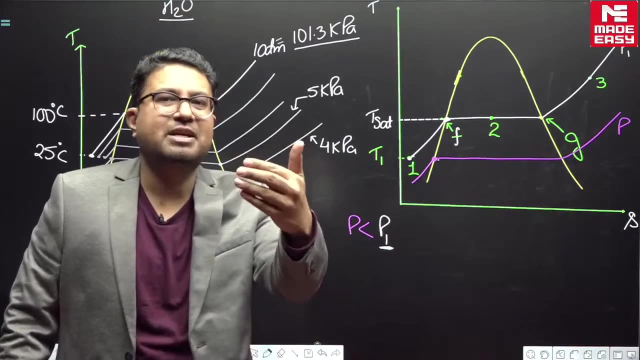 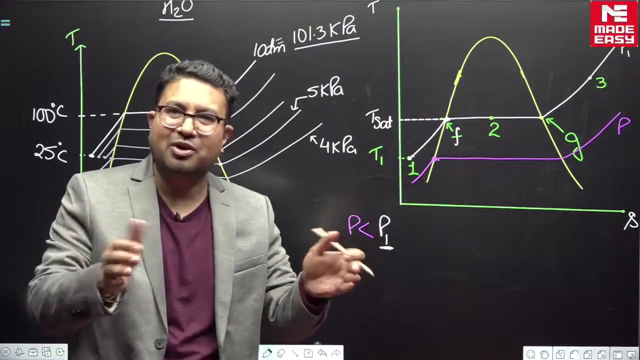 just try to understand the concept here, isko samjho. because generally people dont feel, because they have not seen. why people are not able to feel this? because whenever we see whatever matches our experience, we are able to understand it easier. jaldi samajh jate na whatever matches our experience. now our experience is the boiling of water in. 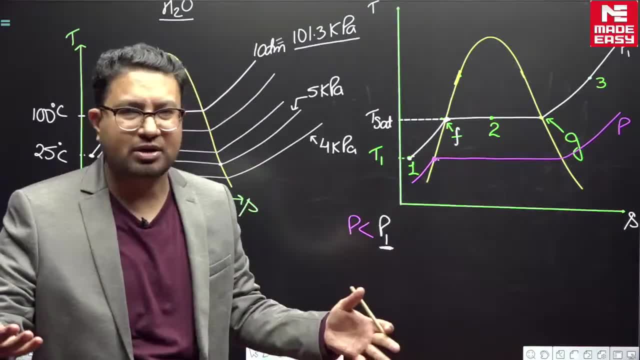 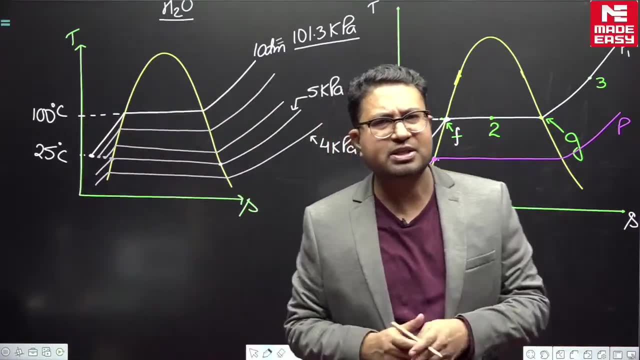 an open beaker. hamara experience open pan me water ki boiling ka hai. our experience is the boiling of the water in an open container. ek open container me water ki boiling ka experience hai hamara. so whenever we see, so the water boiling ham jab water boiling ko dekhte hai, water boiling dekhte hai toh we. 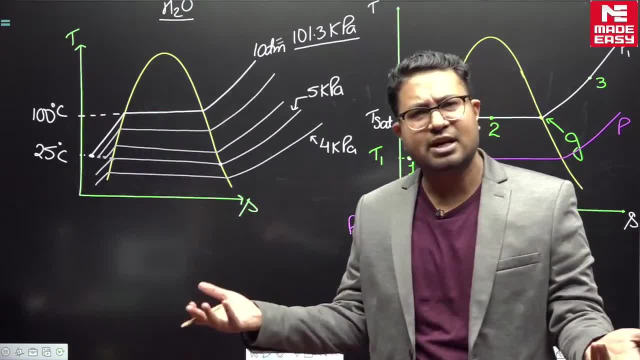 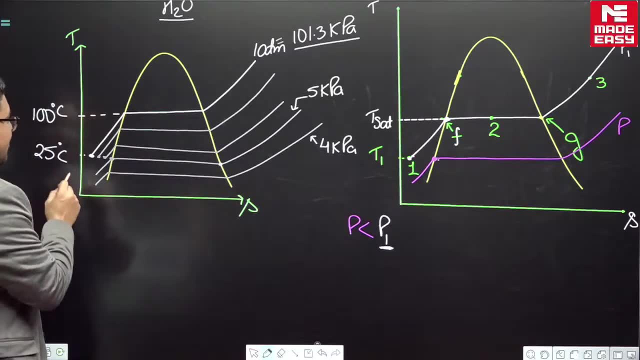 see that it boils at 100 degree celsius because we live at one atmosphere. hum, one atmosphere pe rehte hai. but suppose if i drop the pressure now? suppose if i drop the pressure to 4 kilo pascal water, water in the container, water in the container container, me jo paani tha. 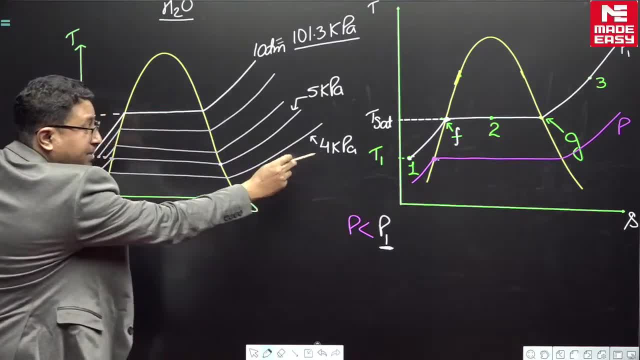 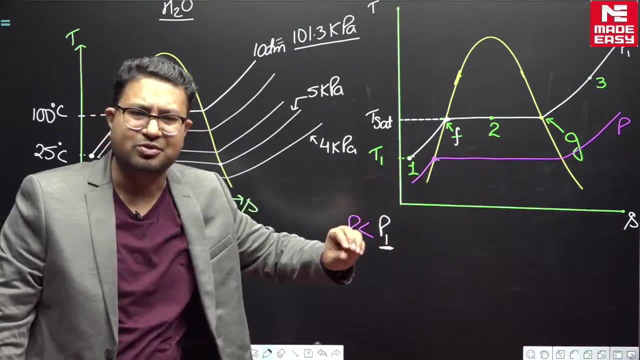 25 degree celsius pe tha corresponding to 4 kilo pascal. 4 kilo pascal ki condition pe corresponding to 4 kilo pascal. let us say me assume kar raha hu ye values direct aise rati hui nahi ye values pe. 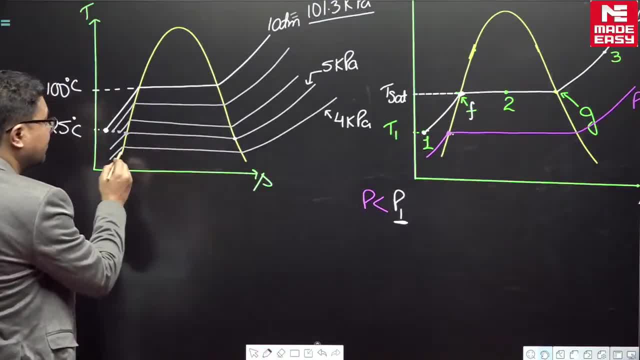 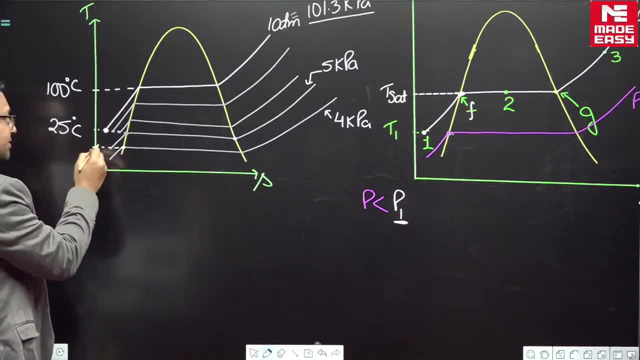 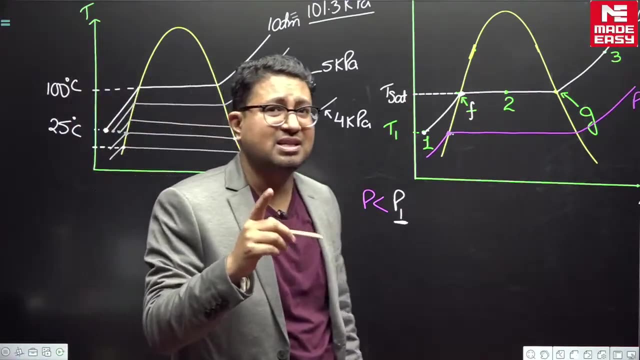 these are the properties, let us say, corresponding to the 4 kilo pascal. the highest temperature which you can exist. jo highest temperature hai jispe h2o can exist as liquid. highest temperature: jispe h2o can exist as liquid, the highest temperature at which the h2o can exist as. 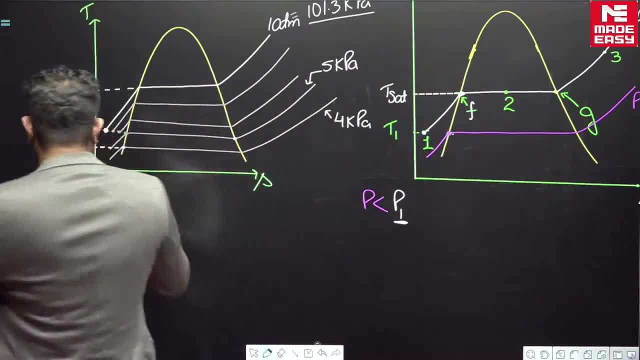 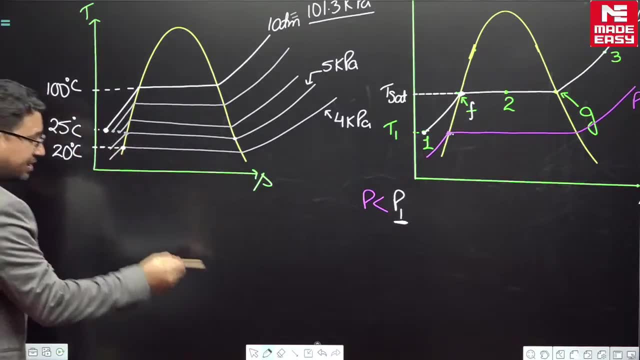 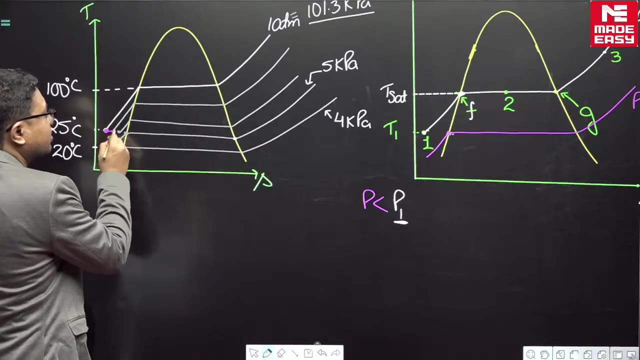 liquid is is. let us say, let us say 20 degree celsius maalo, 20 degree celsius, 20 degree celsius degrees Celsius Highest. or aap kahan the, you were here, aap yahape the. we were continuously dropping the pressure Pressure, drop kar ray the To. at this pressure, can you exist as? 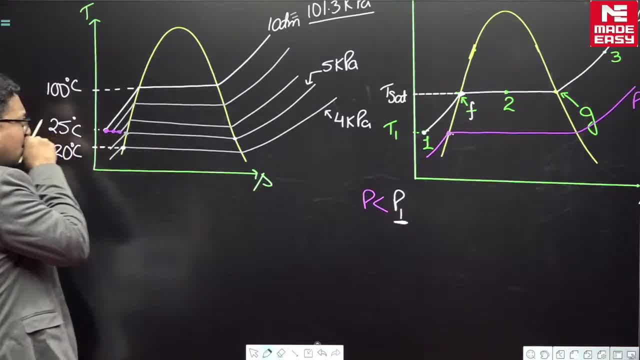 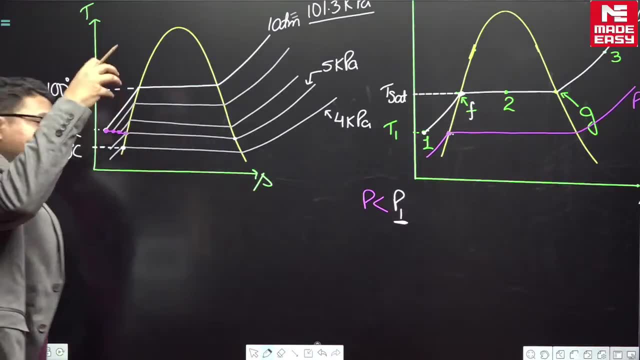 liquid? Yes, I can exist as liquid At this pressure. can you exist as liquid? Yes, I can exist as liquid At this pressure. can you exist as liquid? Yes, I can exist as liquid at this temperature. This temperature may be liquid. 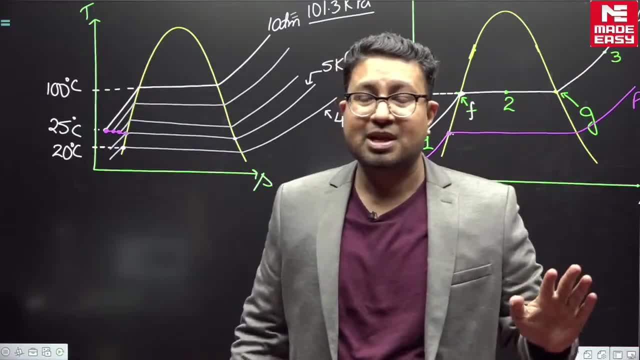 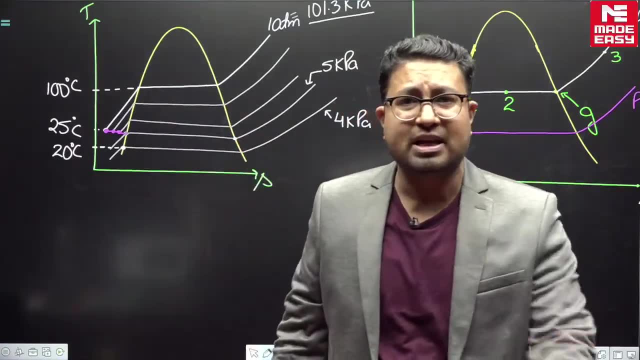 But this is the saturation condition. This saturation has come Now. if you drop the pressure Now, if you drop the pressure, then it cannot exist as liquid. at 4 kilopascal It cannot exist as liquid. It is the property of the substance. 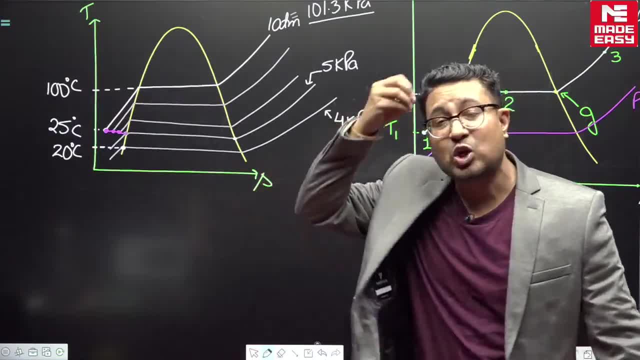 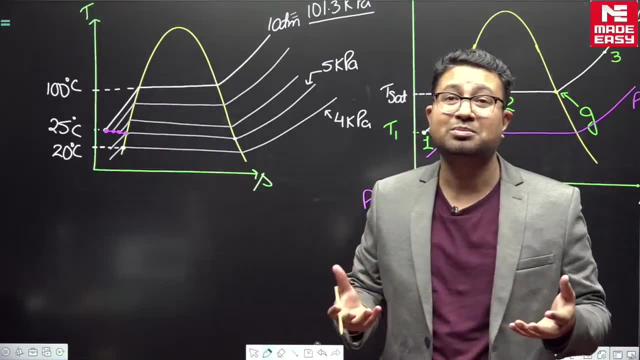 Corresponding to 4 kilopascal. Corresponding to 4 kilopascal. it cannot exist as liquid. It cannot exist as liquid. It cannot exist as liquid. So what to do? What to do then? You don't have to do anything, You. 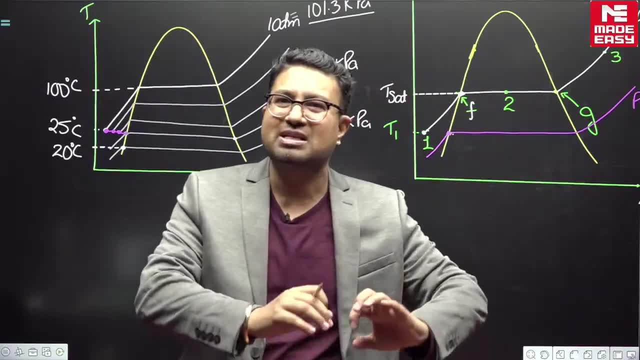 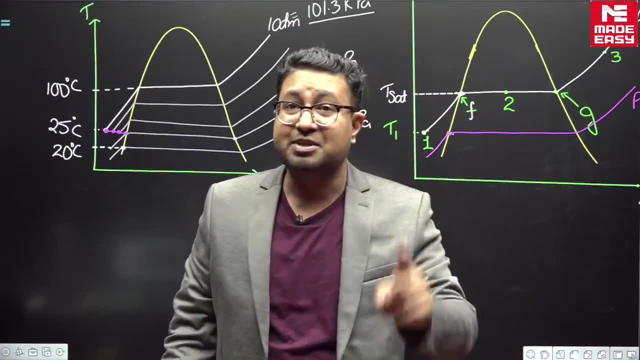 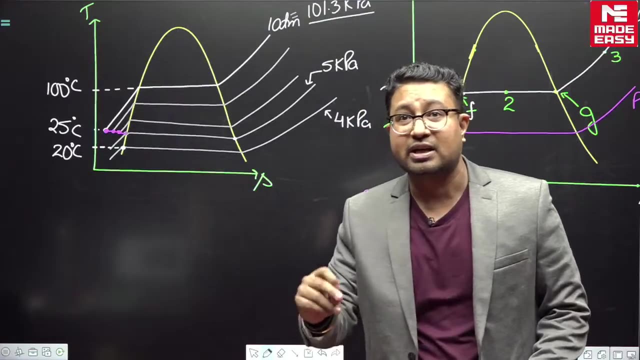 give the conditions. You give the conditions, substance will adjust itself accordingly. Whatever is its property, It adjusts according to its property, Substance adjusts itself accordingly. So as soon as you drop the pressure from 5 kilopascal to 4 kilopascal, What happens? 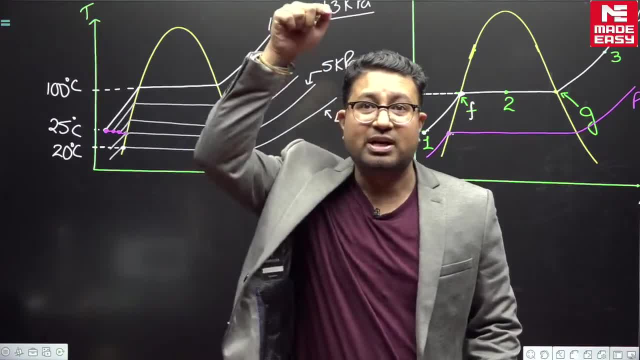 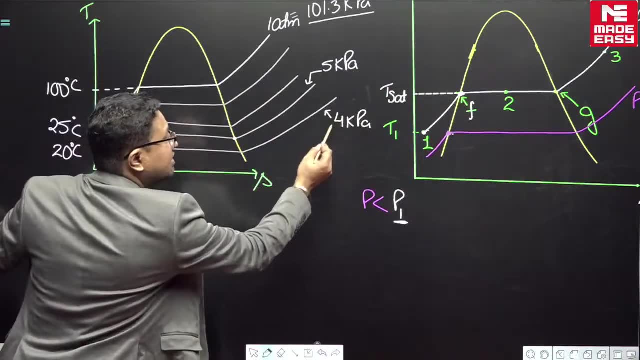 Liquid cannot exist at 25 degree Celsius. Liquid can exist. It can exist at 20 degree Celsius. It can exist at 20 degree Celsius. This is the maximum temperature While being at 4 kilopascal. While being at 4 kilopascal. 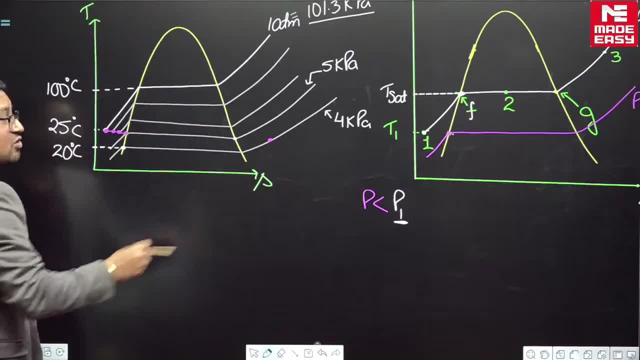 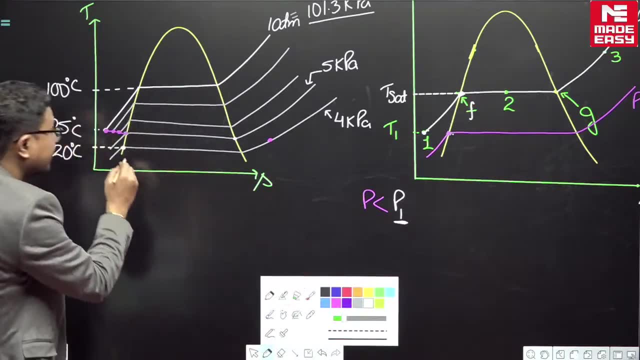 You should be. vapor at 25 degree Celsius, You should be here: 4 kilopascal 25 can be here 4 kilopascal liquid. maximum temperature at which the liquid can exist is 20 degree Celsius. Maximum temperature at 20 degree Celsius. 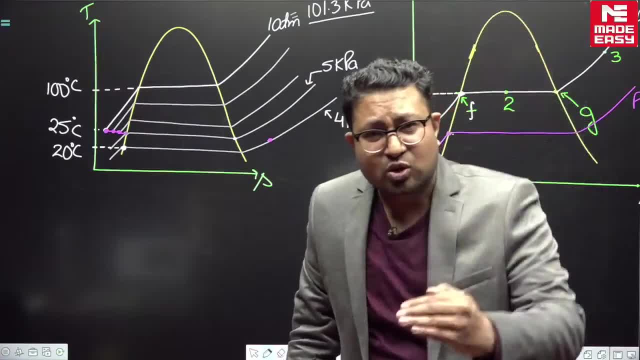 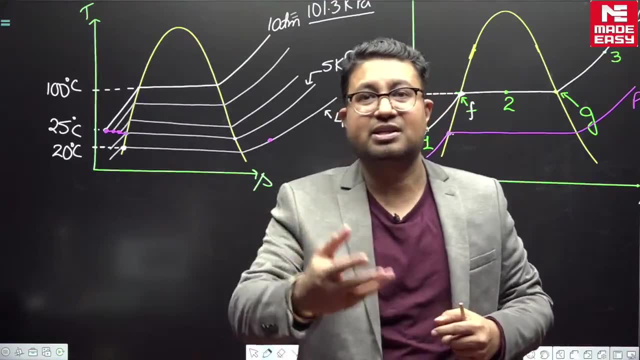 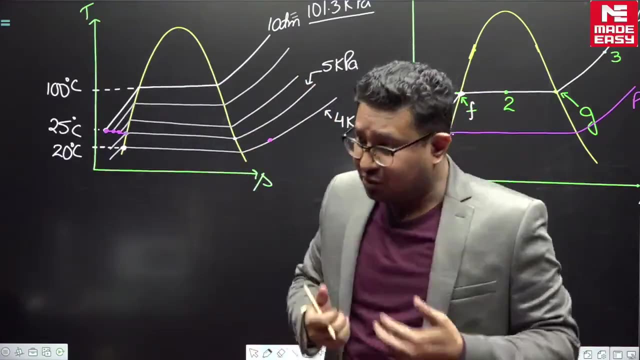 at which the liquid can exist. So as soon as you drop the pressure, The pressure comes on the liquid. now I cannot exist. so what happens? it started. it starts changing into vapor. vapor may change, gonna start. I cannot exist as liquid, so I have to change into vapor. 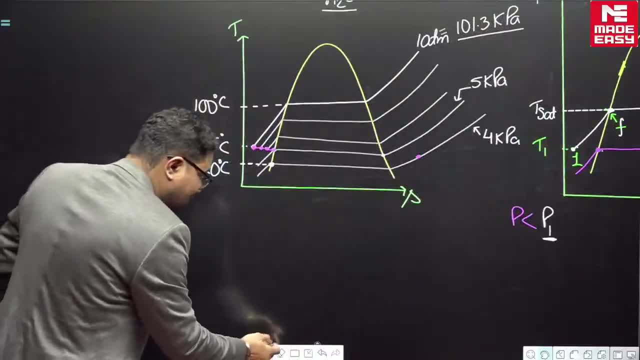 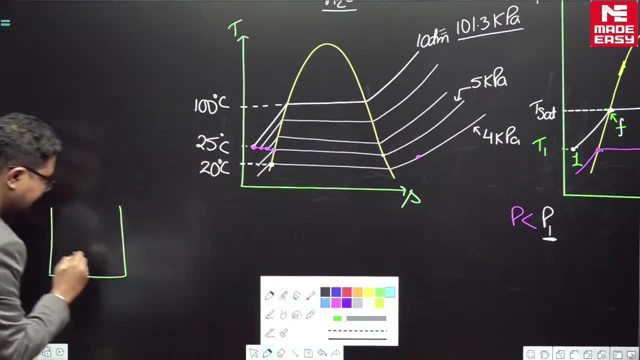 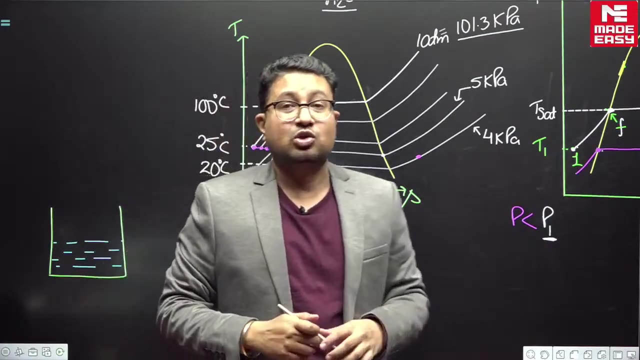 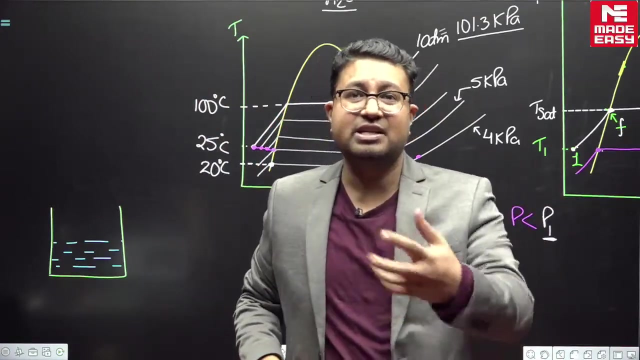 so if it has to change into vapor, if it has to change into vapor, just see what happens here- if the liquid has to change into vapor, as soon as the liquid changes into vapor, it needs energy. it needs the energy for the phase change it will absorb from its surrounding. 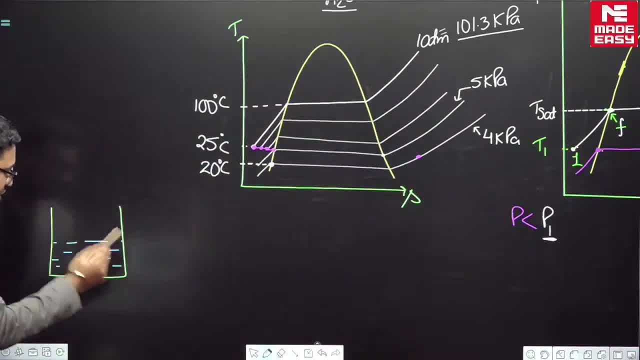 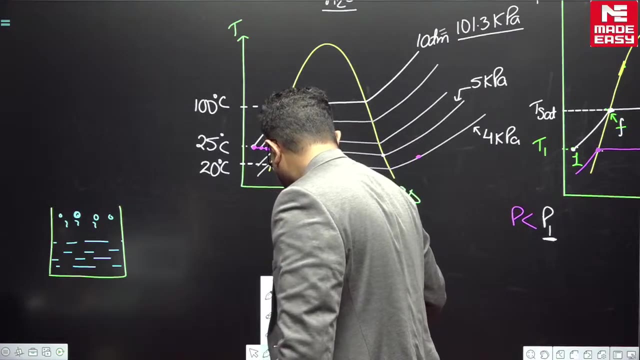 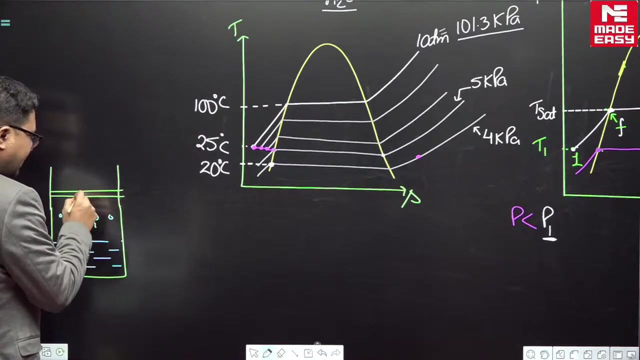 it will absorb from the remaining liquid and it will convert into vapor. it will convert into vapor and this is a. this is a piston cylinder arrangement and you are pulling the piston, you are dropping the pressure, you are trying to expand the liquid, you are pulling the piston. 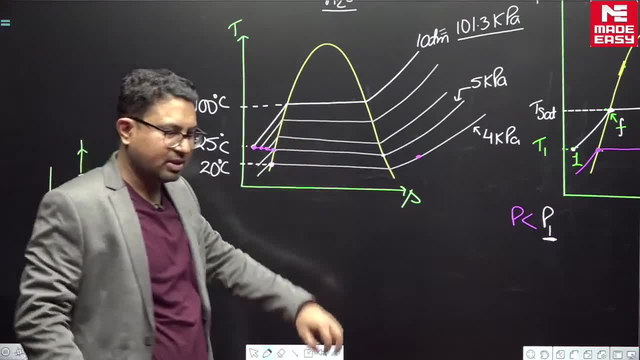 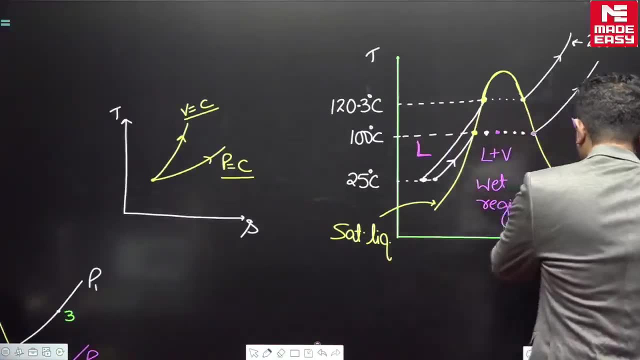 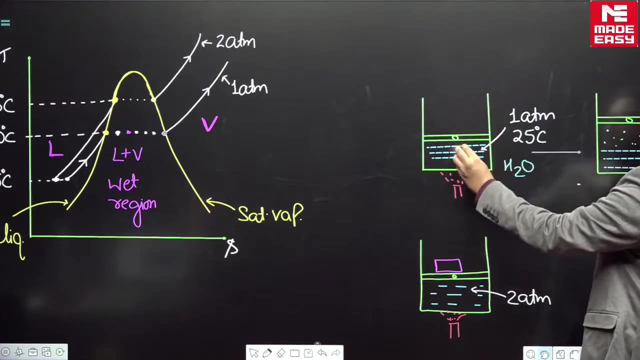 pressure drop will happen. you are trying to expand the liquid. you are not heating like in this case we were heating. in this case, we were heating. in this case, we were heating. piston was moving up because of the pressure, temperature increase and liquid was converting into vapor. Here you are not heating, you are 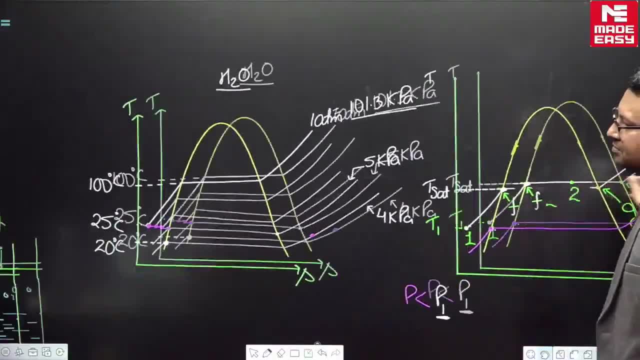 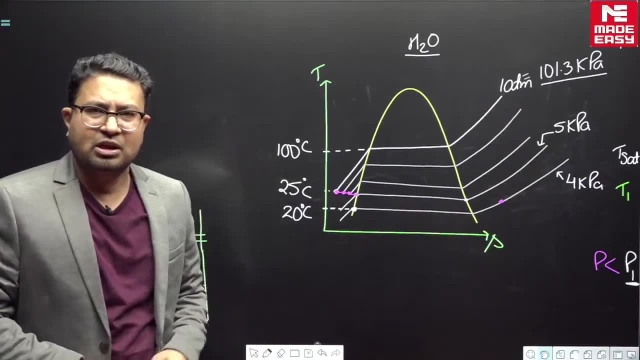 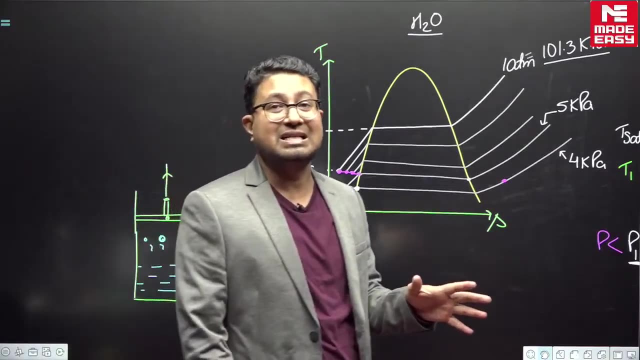 pulling the piston up to drop the pressure inside. You are pulling the piston, You are trying to create a low pressure. When the pressure becomes 4 kilo Pascal liquid says I cannot exist at 25 degree Celsius as liquid. What will I have to do? I will have to convert into vapor. 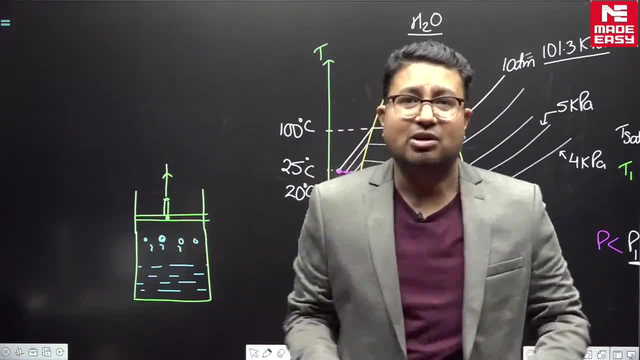 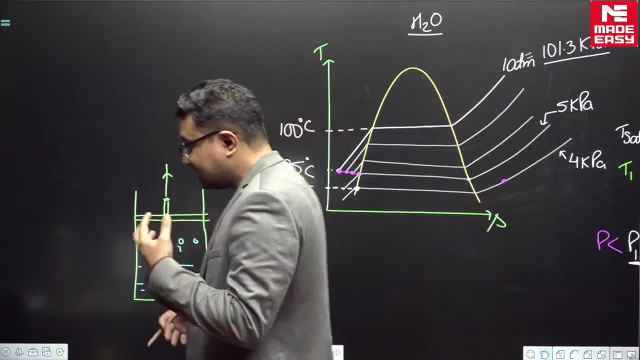 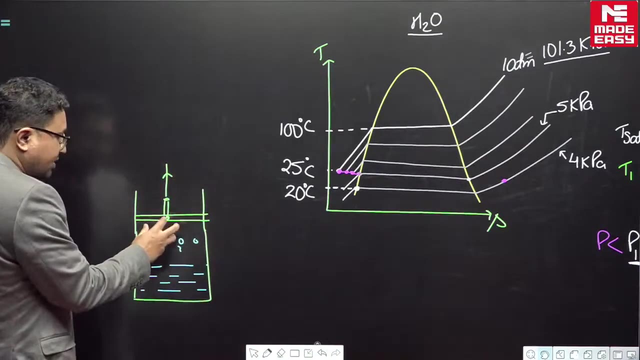 So, as the liquid converts into vapor, latent energy is required. What is latent energy? The energy required to change the phase. There is the requirement of the latent energy, The energy required to change the phase. That is the requirement. So liquid converts into vapor. 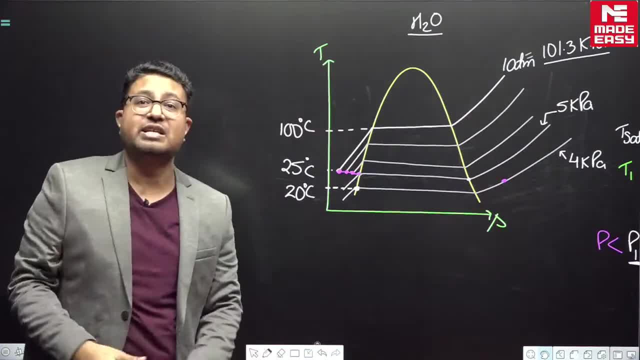 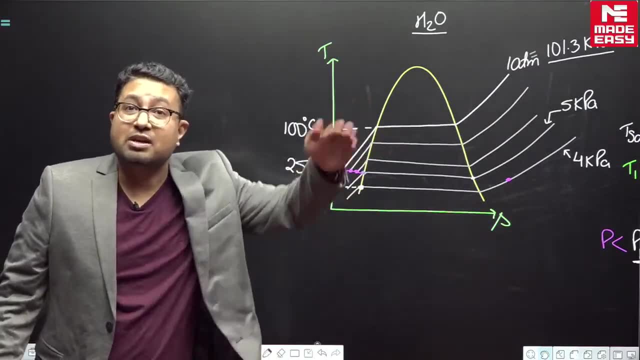 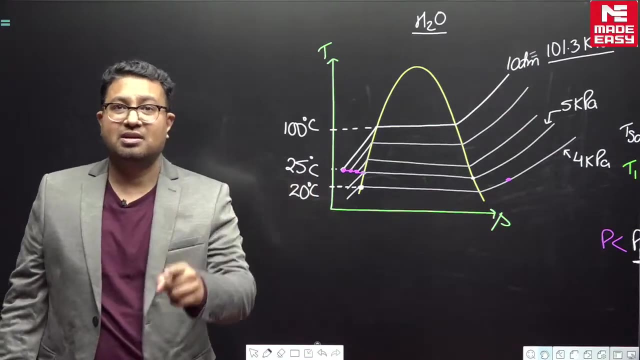 Liquid converts into vapor, So it absorbs the energy required from the surrounding as well as from the remaining liquid. So temperature of the remaining liquid drops. What happens to the temperature of the remaining liquid? It drops Till when this will happen. 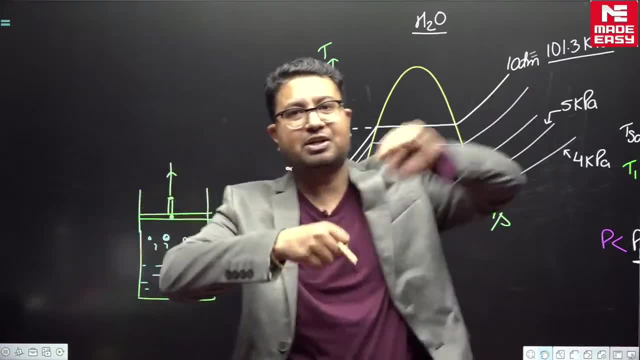 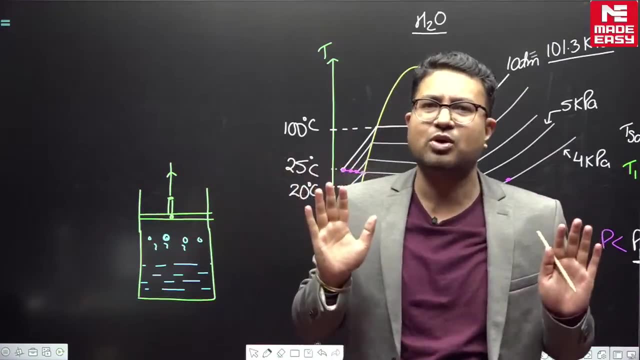 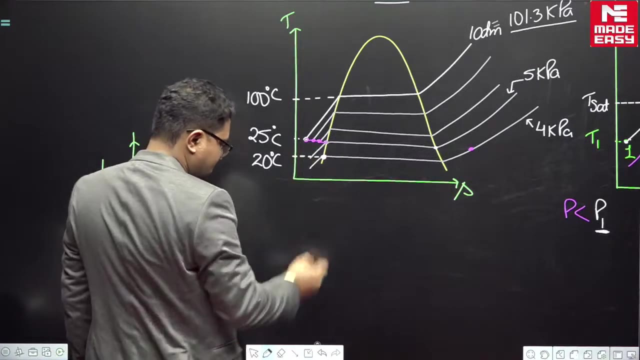 Suppose you brought the pressure to 4 kilo Pascal and you stopped. You brought the pressure to 4 kilo Pascal and you stopped. System is at 4 kilo Pascal. What adjustment will take place? See, the condition was here. You started dropping the pressure. So what is the condition? 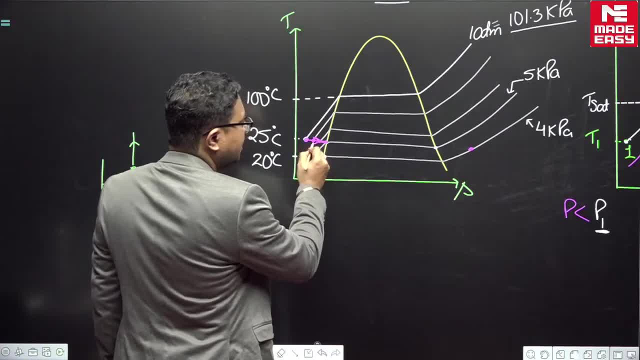 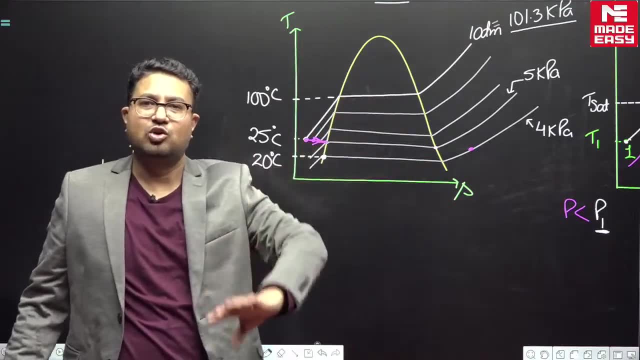 It is liquid. It is liquid, but till 5 kilo Pascal it was liquid. When you suddenly drop the pressure to 4 kilo Pascal, some of the liquid will convert into vapor. Remaining liquid's temperature will drop, So it will achieve an. 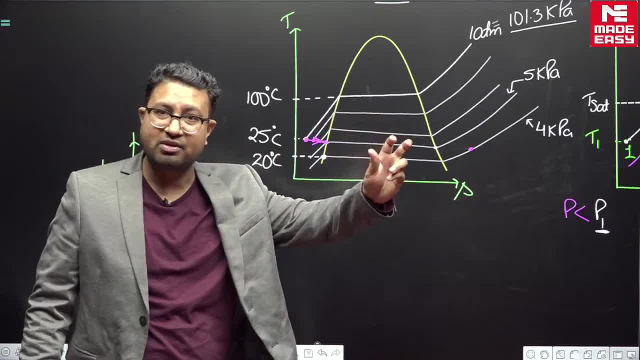 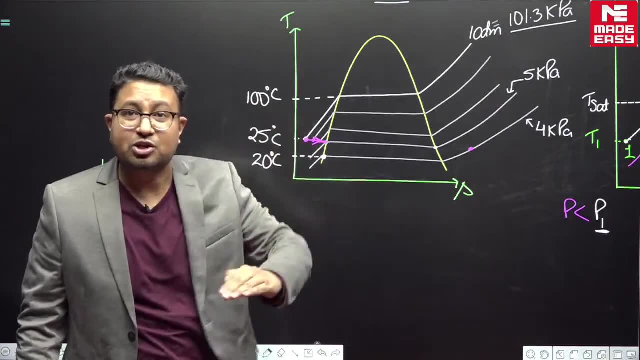 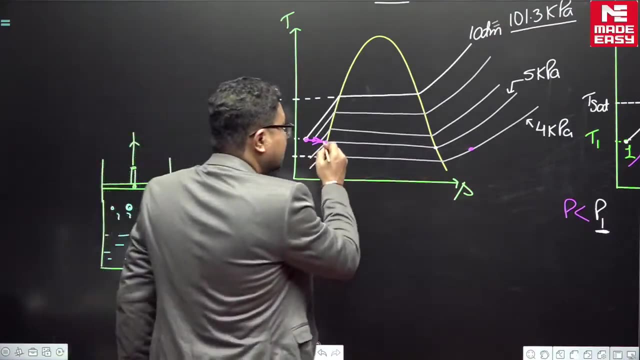 equilibrium condition. So what will happen? Some liquid has changed into vapor, Some of the liquid is still existing, Some are still liquid, So temperature dropped. Why? Because the liquid converted into vapor. Because liquid converted into vapor, so temperature dropped. So some of the 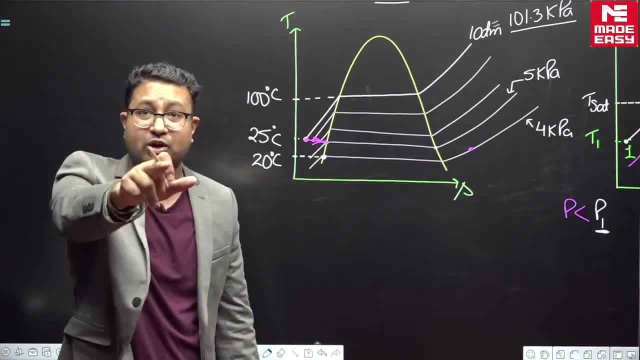 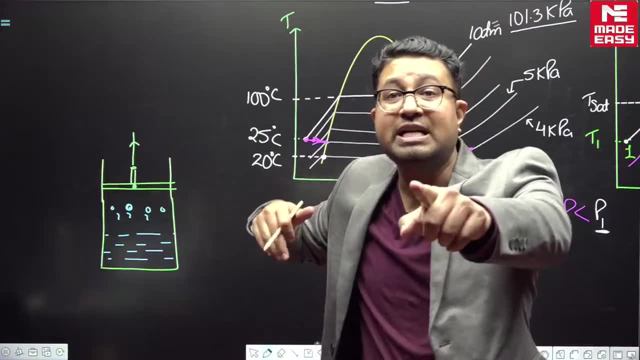 liquid can still exist at 20°C. It can't exceed that At 4 kilo Pascal. So how much liquid will be converted into vapor So that the remaining liquid, The remaining liquid temperature will be dropped to 20°C? So the remaining liquid temperature drops to 20°C And the vapour 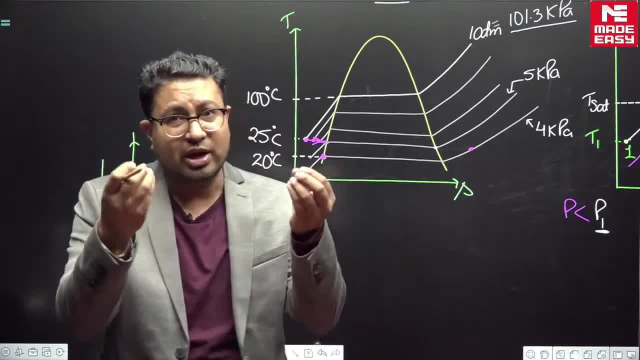 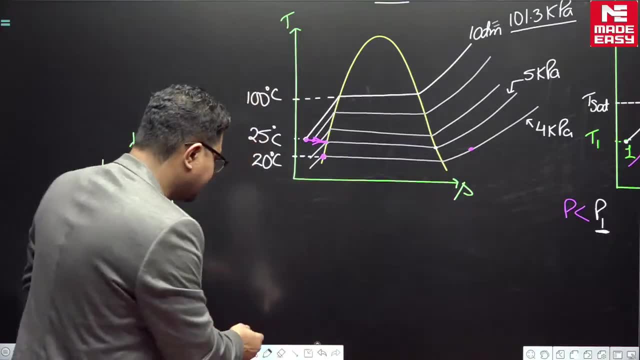 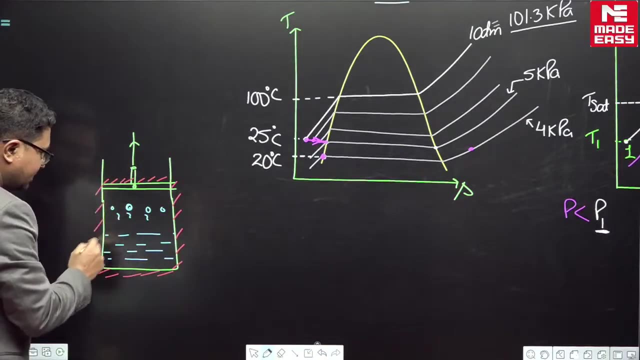 is there because there is no contact of the liquid, So it is in contact. So for equilibrium it also has to be at 20°C If you have insulated it. if you have insulated it, there is no transfer. heat from outside: there is no transfer of heat from outside. there is no transfer of. 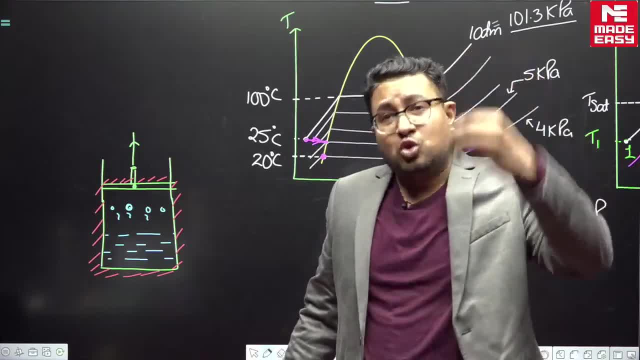 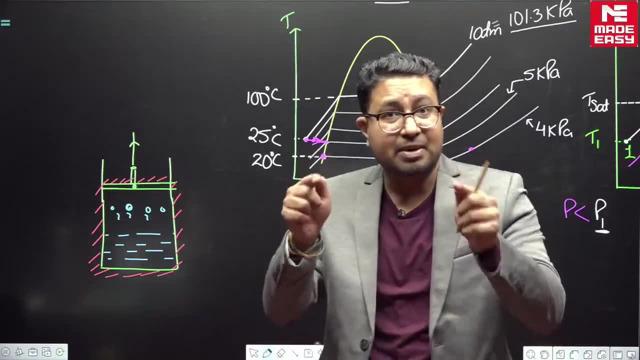 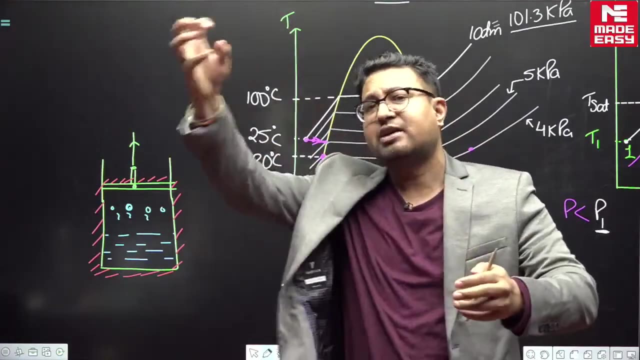 heat from outside. so you will be in the, you will convert into the vapour phase. you will convert into the vapour phase and equilibrium will reach like this: liquid can exist up to 20,. it can exist up to 20,, not beyond that. so some of the liquid will convert into vapour. 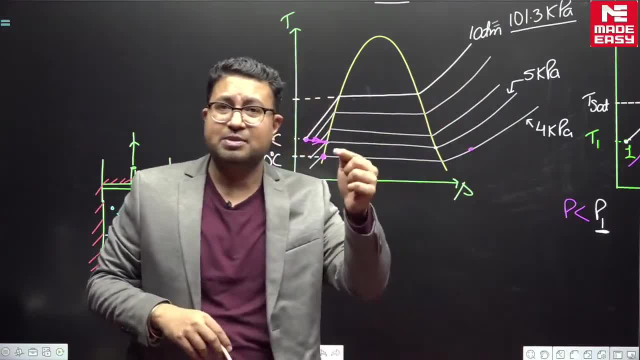 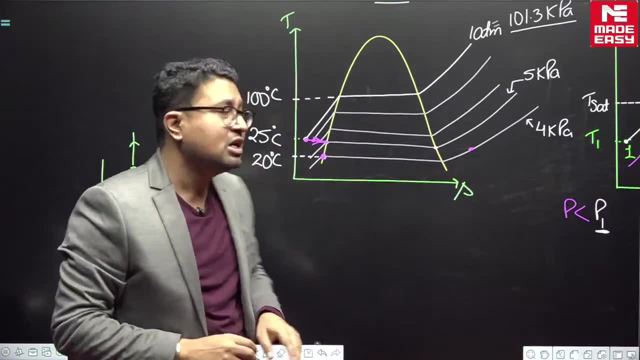 some liquid will convert into vapour and some of the substance will remain liquid. how much? much so that the temperature of the entire mixture drops to 20 degree Celsius. so finally, you will see, suddenly, sudden conversion will happen. sudden conversion will happen. 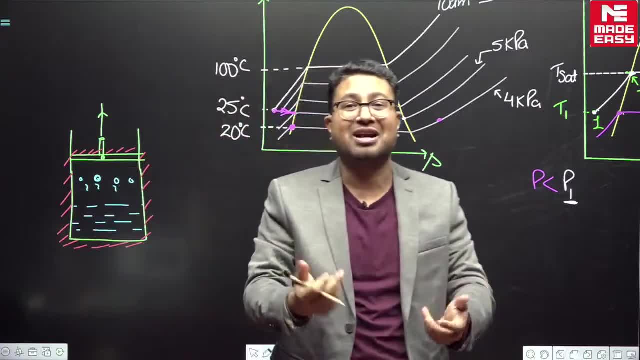 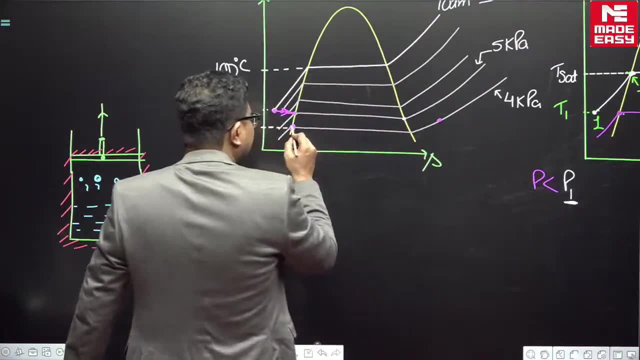 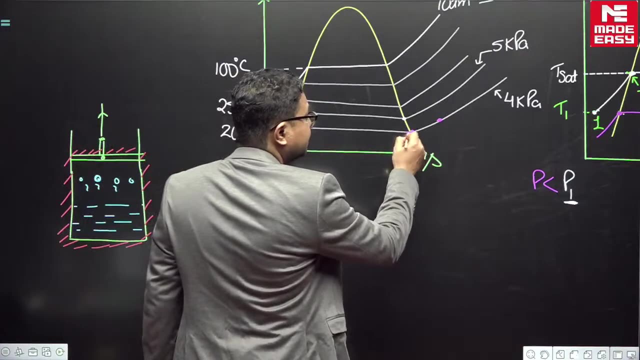 some of the mixture. we cannot make a graph of this sudden conversion. we will not be able to draw the graph, so there will be a sudden conversion of liquid into vapour. so this is here. some part liquid will be here, some part vapour will be here, some part liquid. 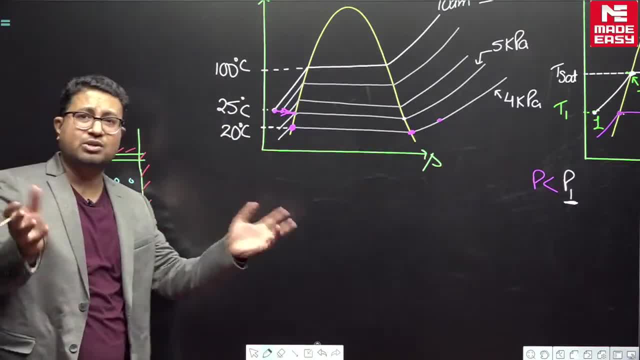 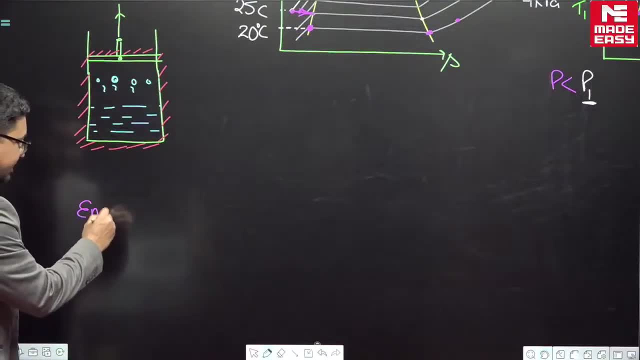 will be here some part, vapour will be here, And if it is insulated from outside, there is no energy coming from outside. so you say: okay, sir, how did the temperature drop? where did the energy go? what is energy? what is? 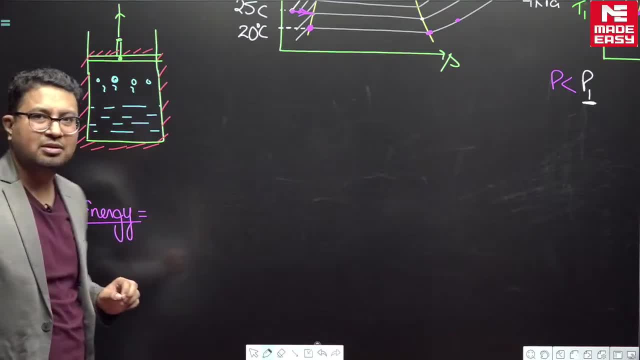 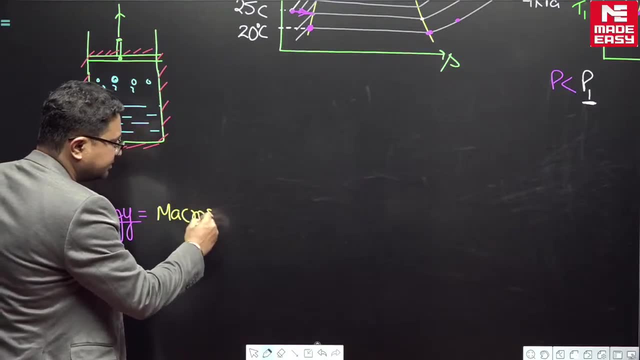 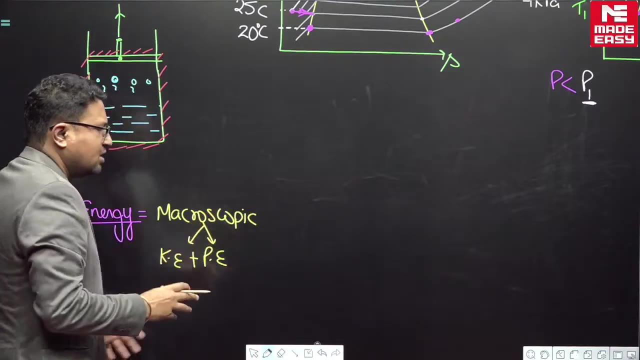 the energy. energy is what is the energy. energy can be what can be: macroscopic, scopic, which includes kinetic energy plus potential energy. nothing is changing in this kinetic energy. you are not moving the piston cylinder arrangement anywhere. you are not moving the 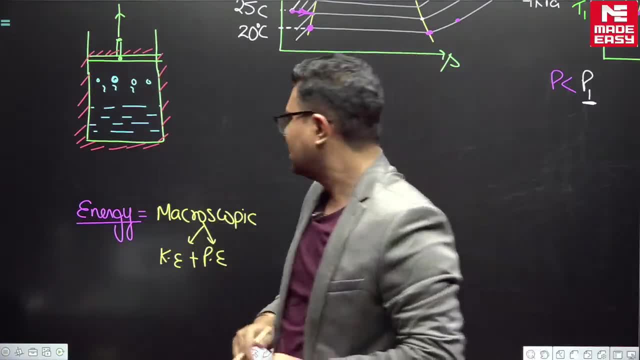 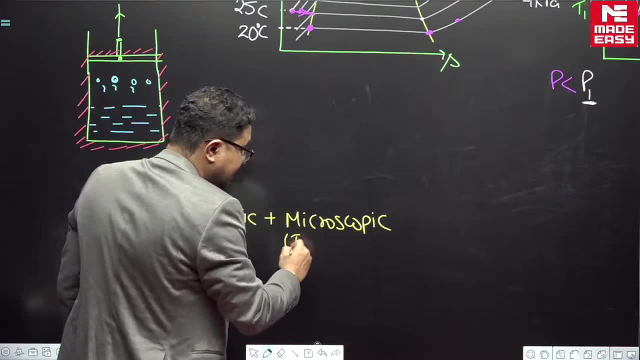 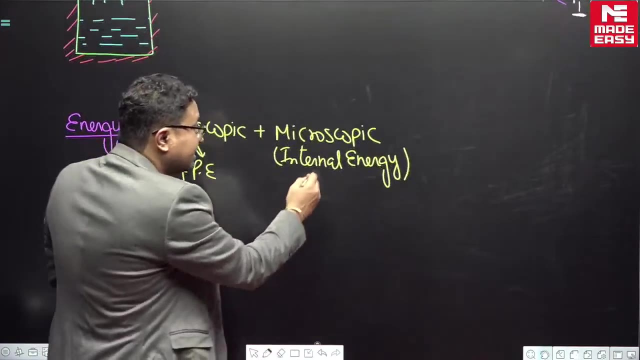 piston cylinder arrangement. anywhere it is stationary, it is stationary. then there is microscopic energy. what is the energy microscopic? this is what. what is this internal energy? this is internal energy. this is internal energy. now, in internal energy, there is sensible. 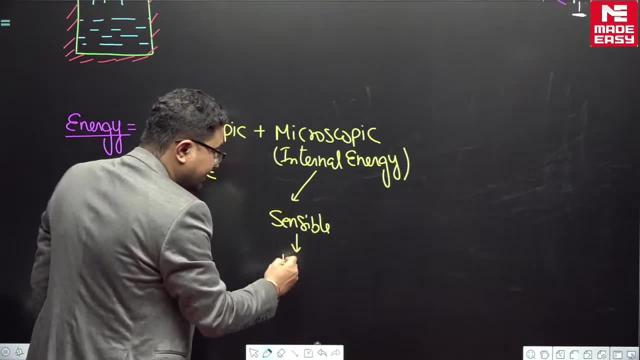 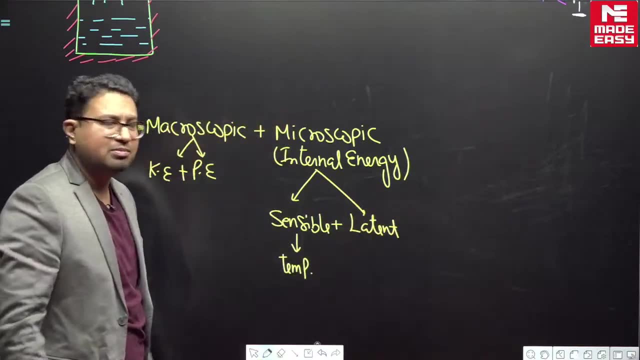 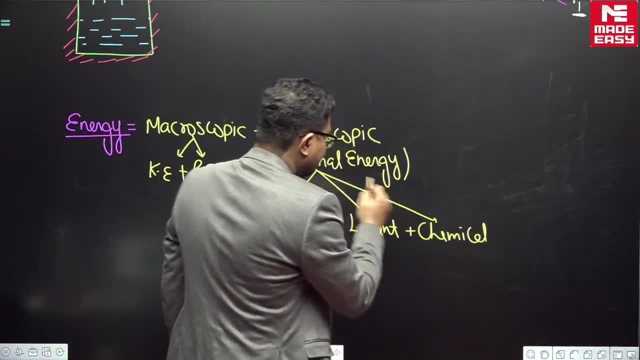 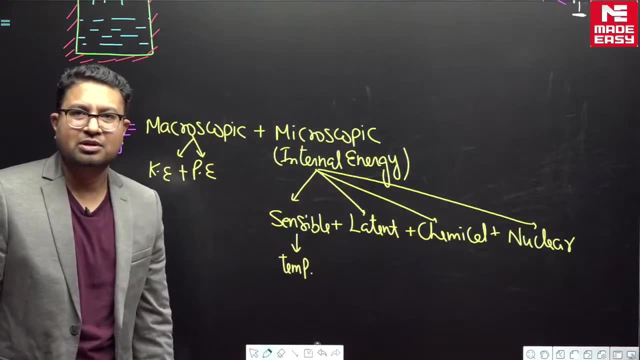 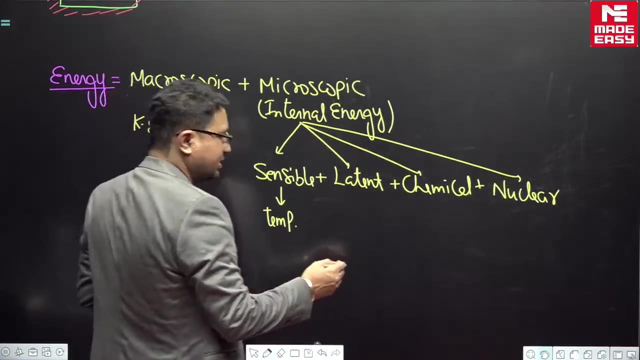 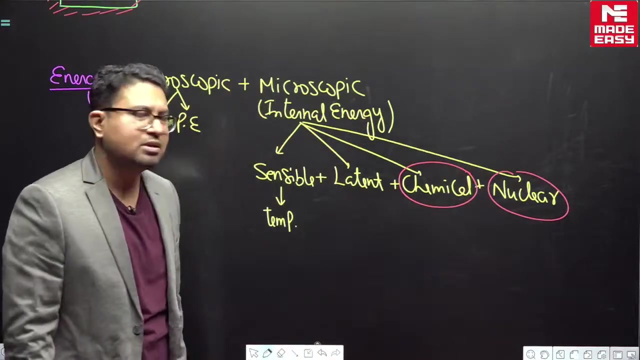 energy, also chemical energy, and there is nuclear energy, also nuclear energy also. So if you see, if you see here, if you see here, if you see here chemical energy transaction, transaction. we are not doing any chemical change, we are not doing any nuclear change, we are not doing any nuclear change, we are not doing any nuclear change. 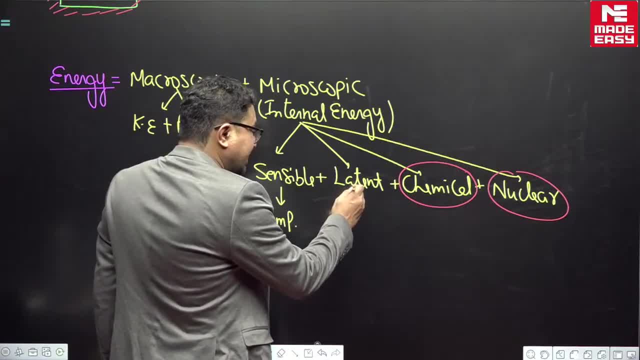 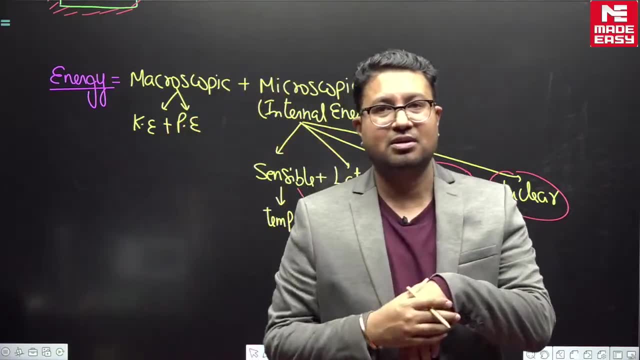 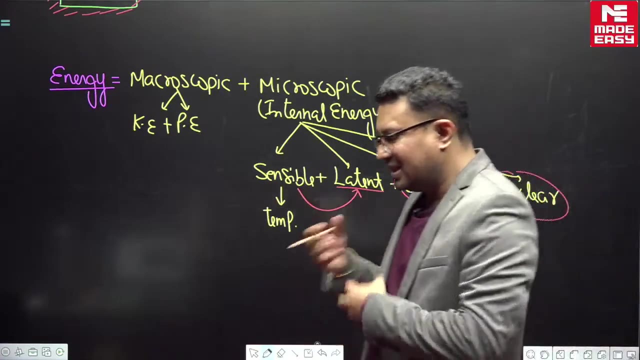 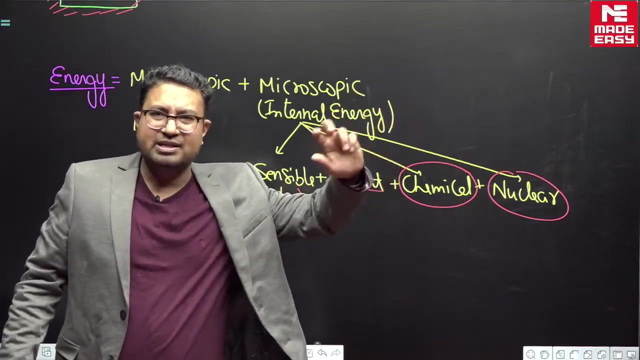 latent energy. latent energy, may conversion or a sensible energy is converted into latent energy. when the sweat dries, you feel colder. why? because liquid converting into vapor takes the energy from the remaining water or from your body, takes energy from your body. so latent energy comes. energy is hidden. 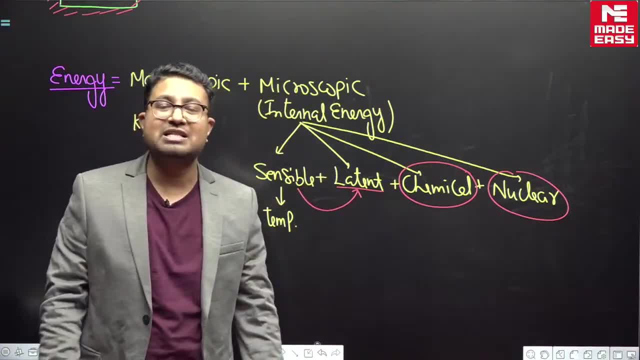 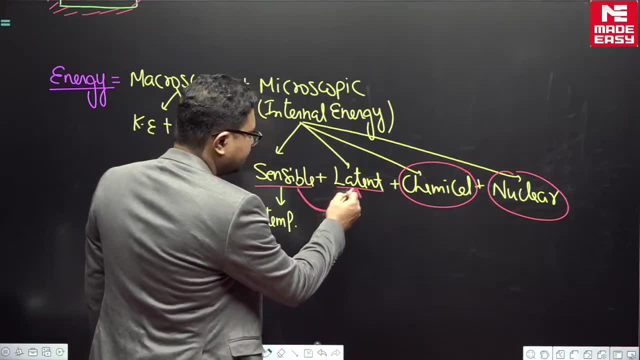 sensible energy, which I was sensing, will be less. the energy which can be sensed by the thermometer will be less, so this energy converts into this energy. this energy will be converted into this. this energy will convert into this. there will be an effect of expansion too, which you have pulled. 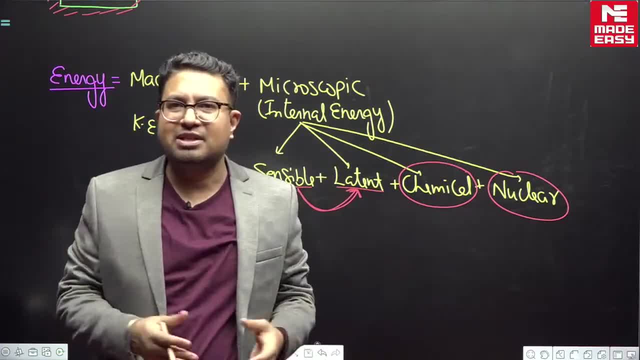 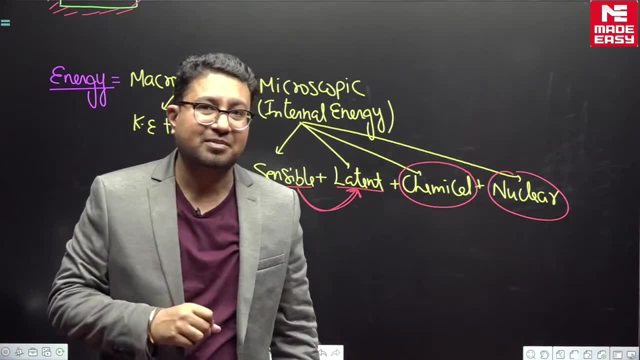 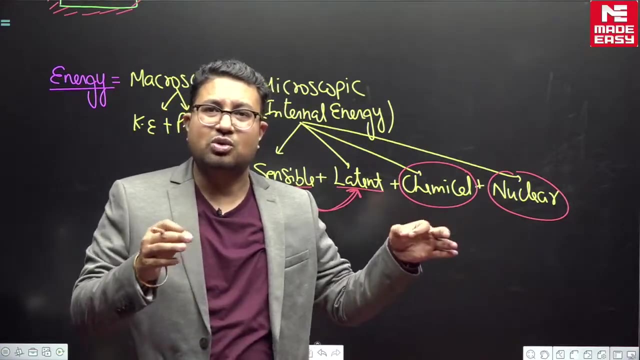 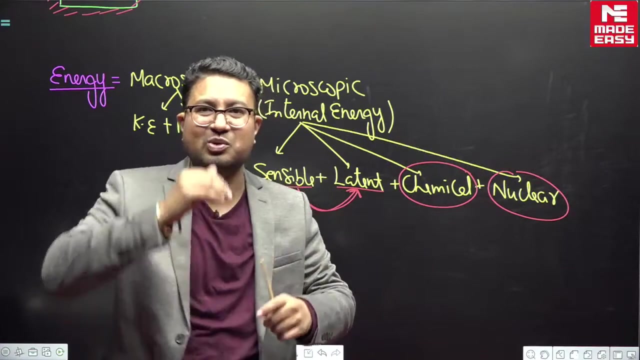 but some of the sensible energy converts into latent, which drops temperature, which just refrigers the body, which just refrigers the body In refrigeration, air conditioning. there is a separate video on YouTube, VCRS. you can see it. I have recorded it in English. So the refrigeration which is taking place, the refrigeration by dropping the pressure, first you compress, you increase the temperature, then you drop the pressure. you will understand it in a very beautiful manner. 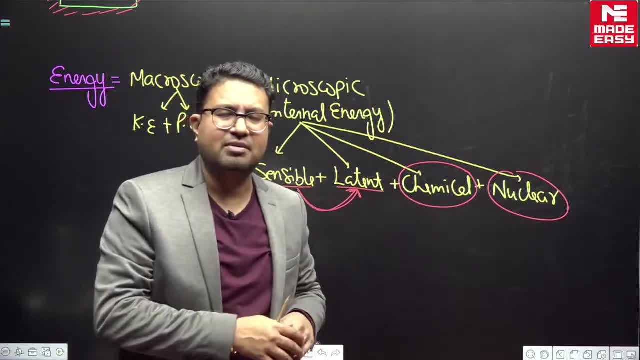 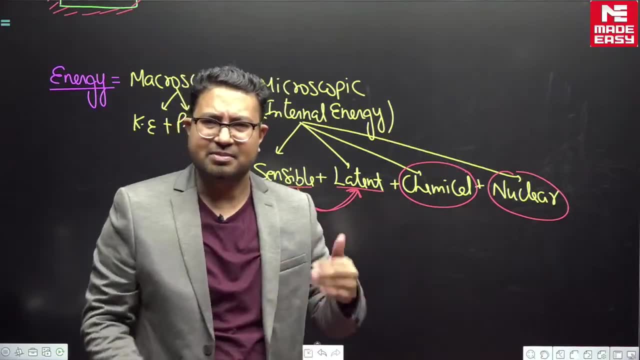 You will understand it very well. there is on YouTube earlier. I have recorded it. that is in English. it is in full English, but you will understand it in a very beautiful manner. I am not going into that discussion here. I am not going into that discussion here, but because I mentioned something. I explained you that how? dropping of the pressure? 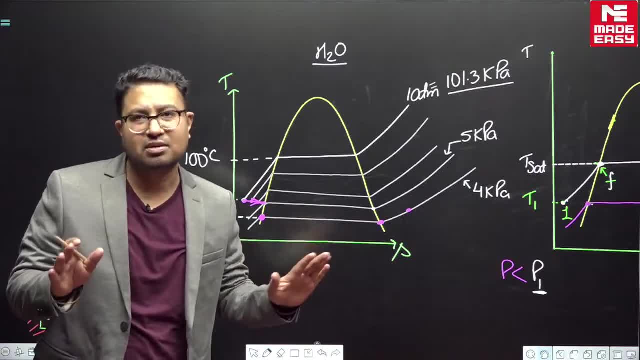 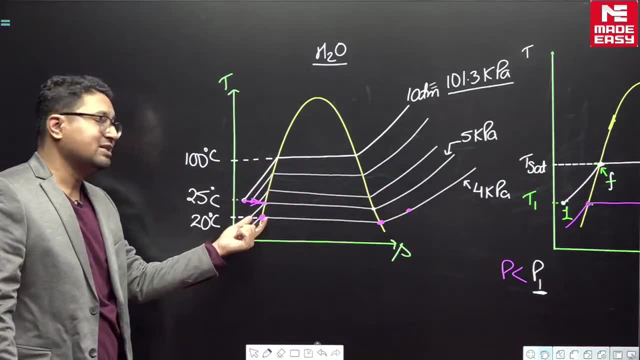 So now it will be stable at 20 degree till you don't disturb it further. it is stable, till you don't disturb it further, because corresponding to 4 kilo Pascal liquid can be there. liquid can be there at 20 degree Celsius, but above 20 cannot be there. 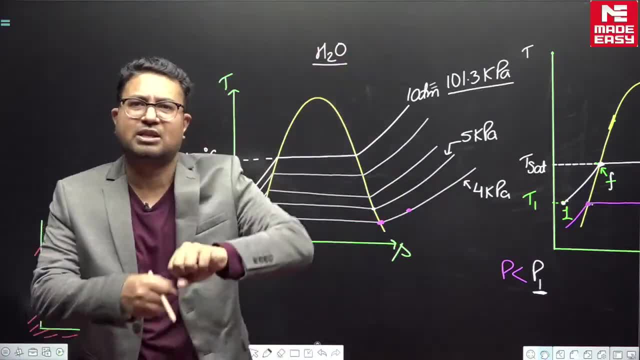 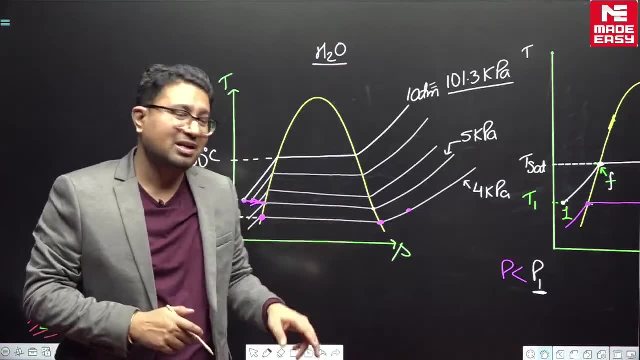 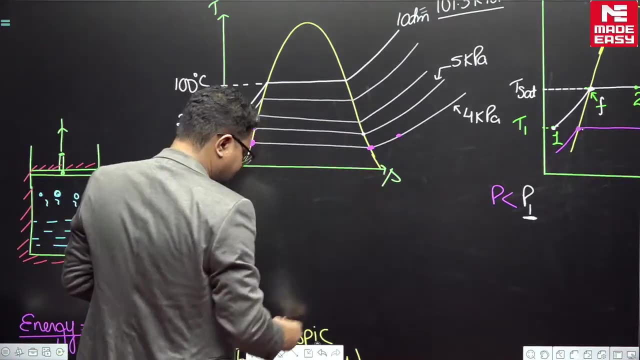 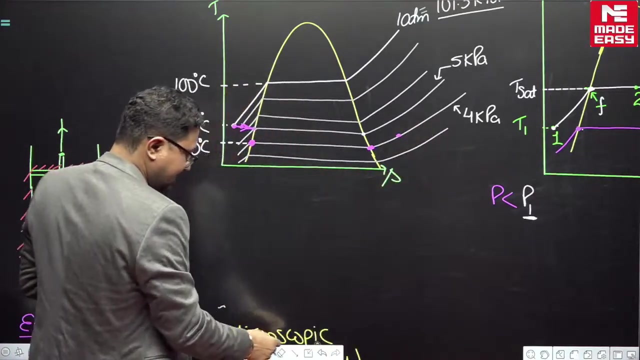 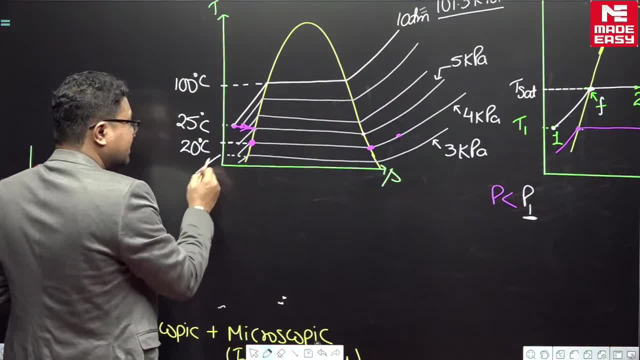 and 3 kilopascal. let us assume that 3 kilopascal the saturation can take place up to, let us say, 17 degree Celsius. I am taking random values. I am taking these values randomly because there is so much data. 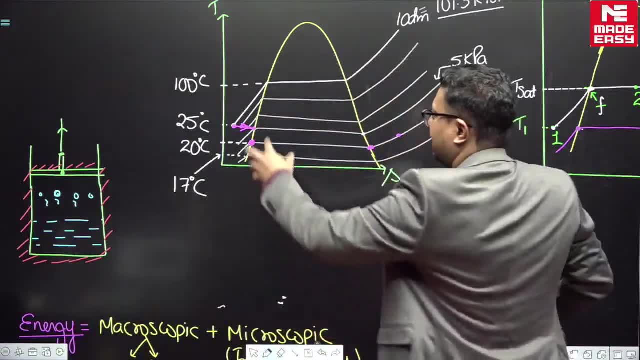 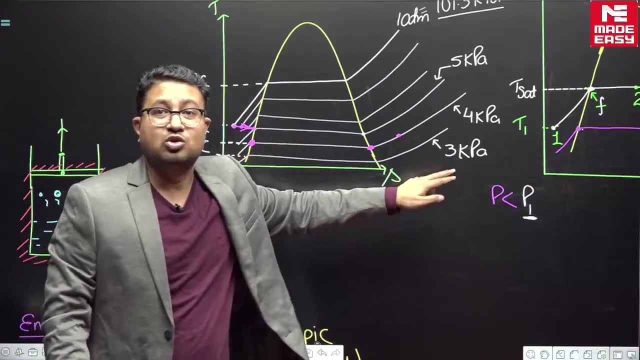 it is not possible to remember each and every data. so let us assume, if you drop the pressure further, so 20 degree Celsius, it cannot exist. so if you have brought the pressure to 3 kilopascal, then liquid can remain till 17,. 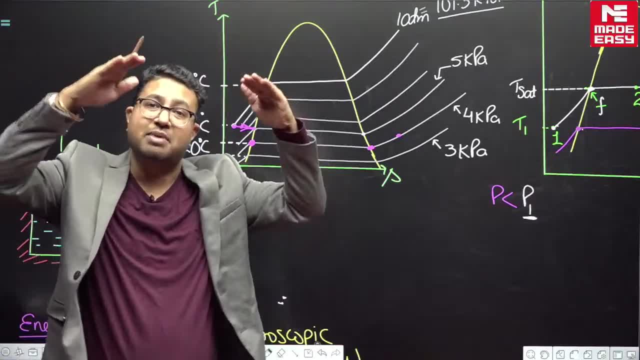 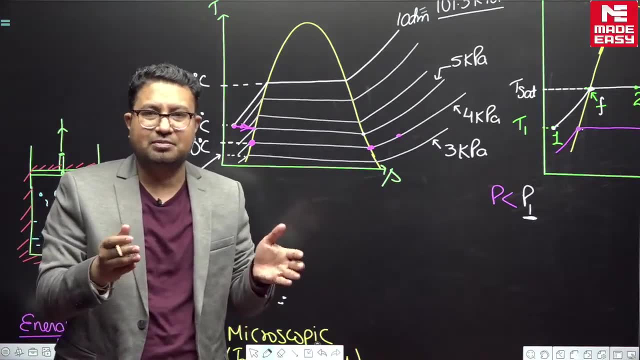 so that much liquid will convert into vapour, so that the mixture can be at 17,. that means liquid can be at 17,. it will reach there, so you can drop the temperature also, if you allow, if it is adiabatic. 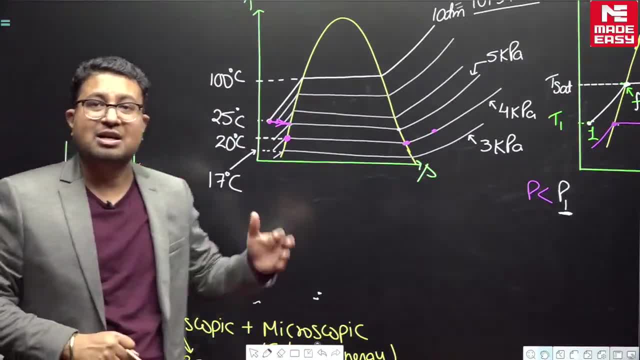 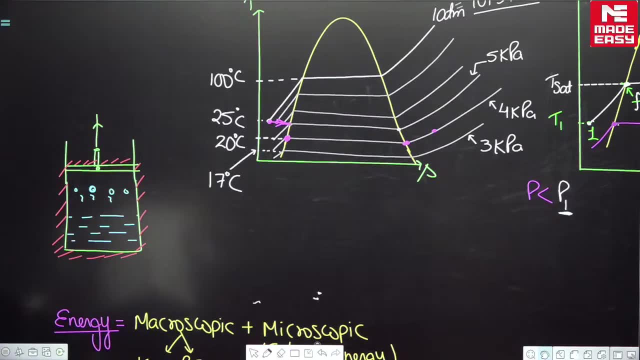 then heat will not transfer from outside, so it will become very cold. it will become very cold because of the liquid changing into vapour, so this is one of the thing we discussed. we discussed this thing, Ankit. the team of gate course will reply. 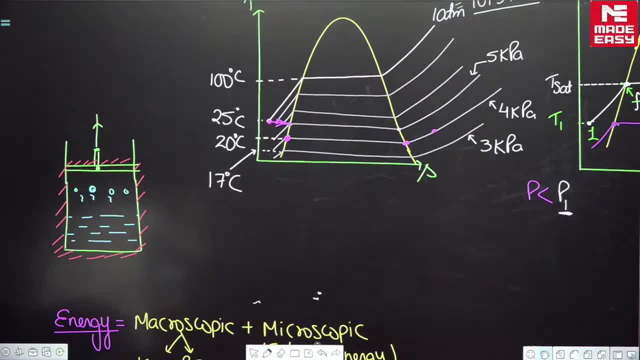 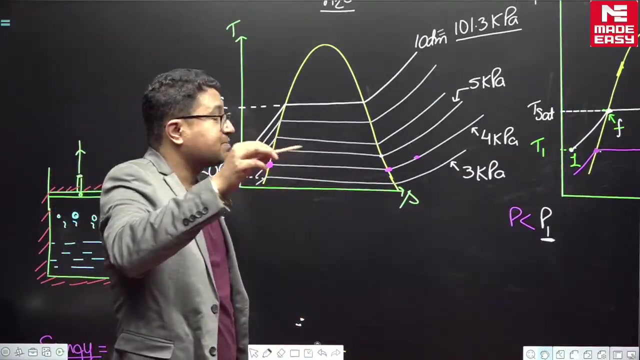 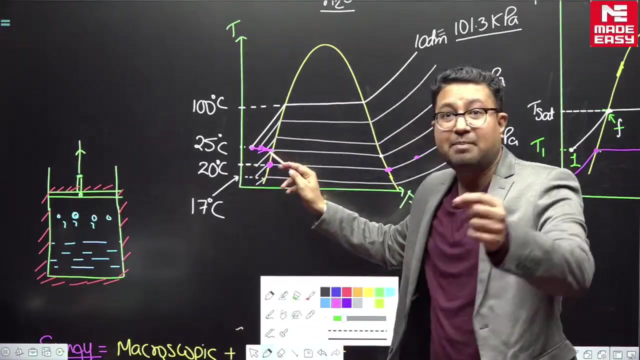 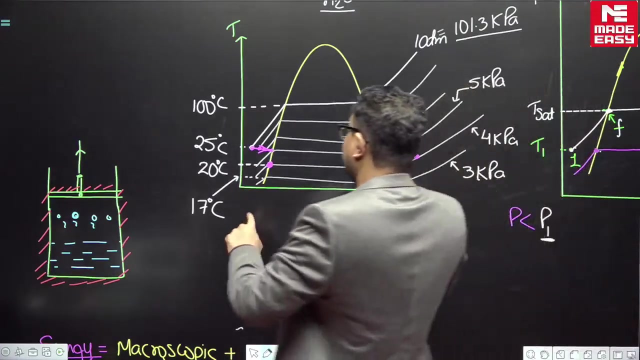 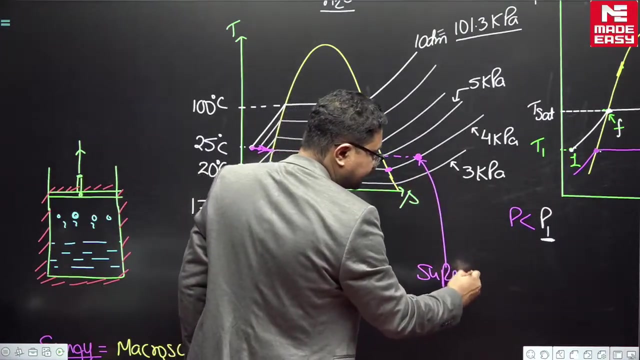 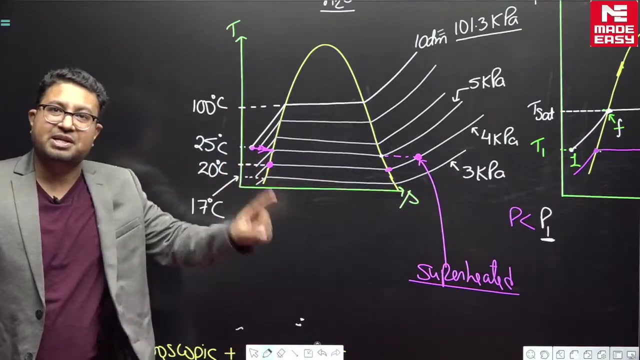 I am not talking about the course, I am talking about this. you are absolutely right. if it is specifically mentioned in the question, the temperature will remain 25, but you have dropped the pressure to. you have dropped the pressure to 4 kilopascal, so you will be here, 25 degree Celsius. where will you be? at 4 kilopascal, you will be here, so this will be the superheated state. what state will this be? superheated state? I will discuss this also. I will discuss it. so, if you have supplied sufficient heat that you are able to maintain the temperature through the external heat supply, 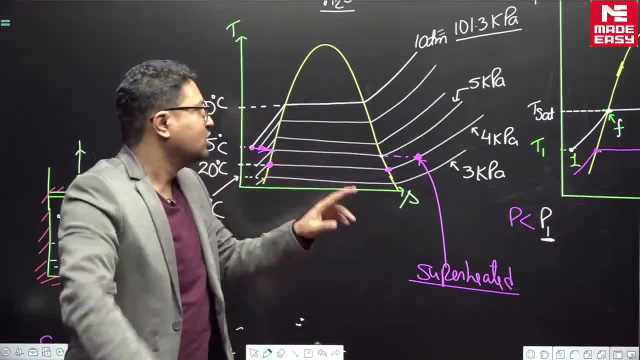 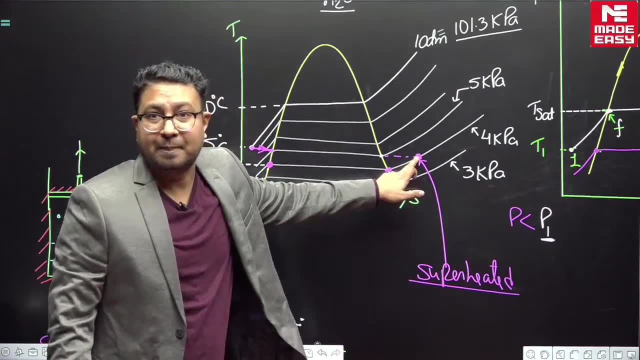 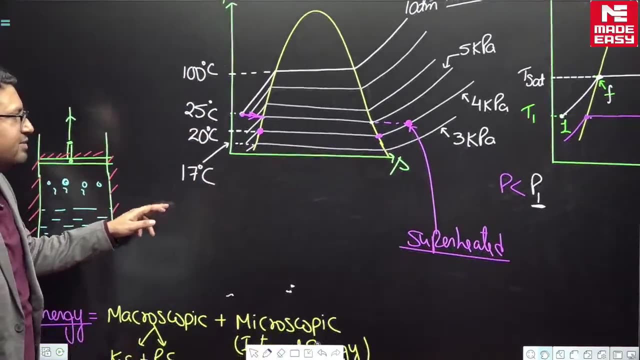 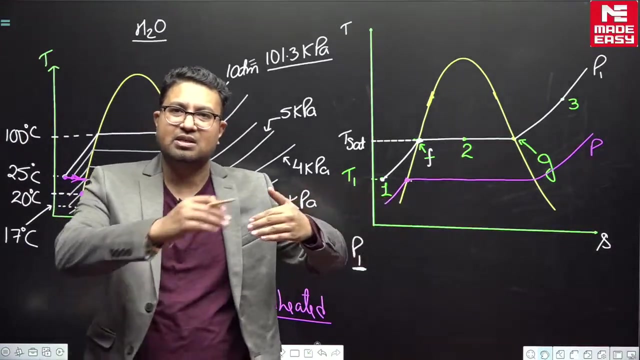 you do not need to convert the liquid into vapor. you are supplying heat from outside. so if you drop the pressure at 25 degree Celsius and bring 4 kilopascal, so you will exist in this condition, you will exist in this condition, you will exist as a superheated state. very good, you have understood, and so on. you have understood what I have explained. you have understood correctly. so we just understood. we understood that sub cooled liquid or under cooled liquid, or we call it as compressed liquid, we call it as compressed liquid, we call it as compressed liquid. 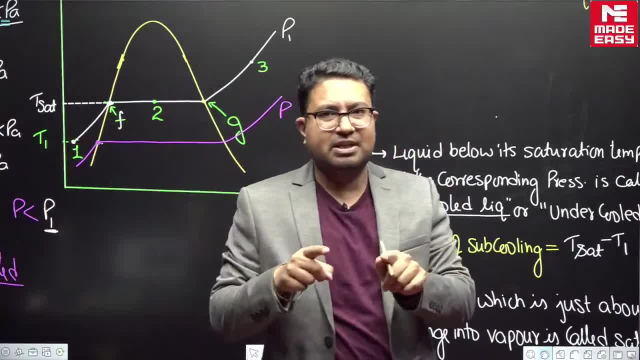 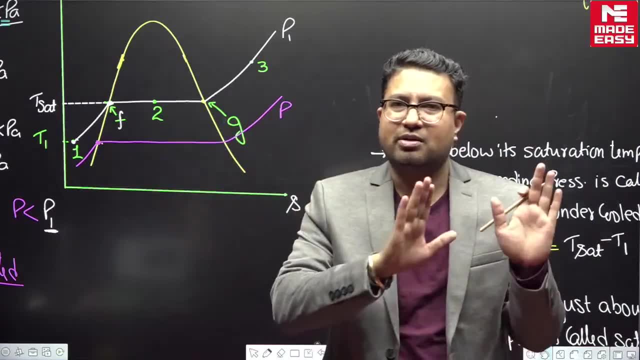 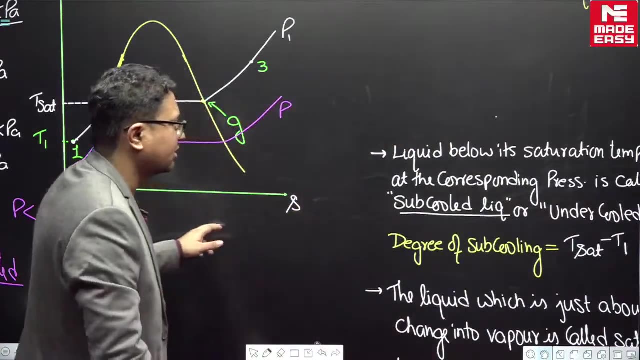 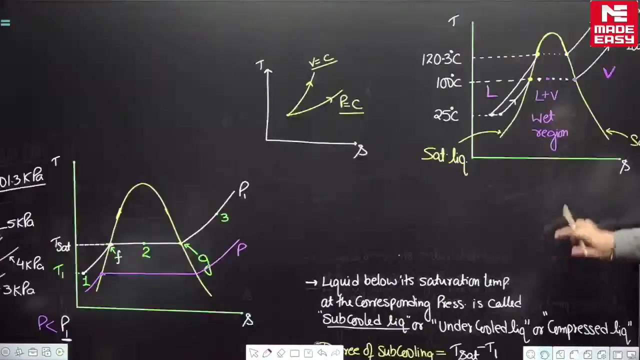 I will show you whatever see in parts, whatever I am discussing, I will just show you and I will move aside. I will not give time to write after that. you can take a screenshot, you can write down whatever it is. but, yes, I will have, I will discuss it in parts and I will move aside so that you can write down whatever you want. you can write, okay. so we have discussed something. let me just move aside. let me just move aside this discussion. we have already done. 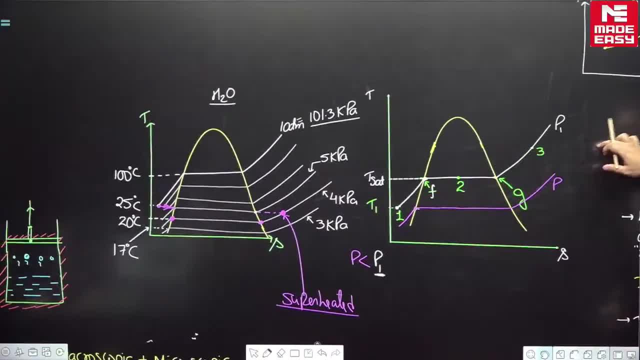 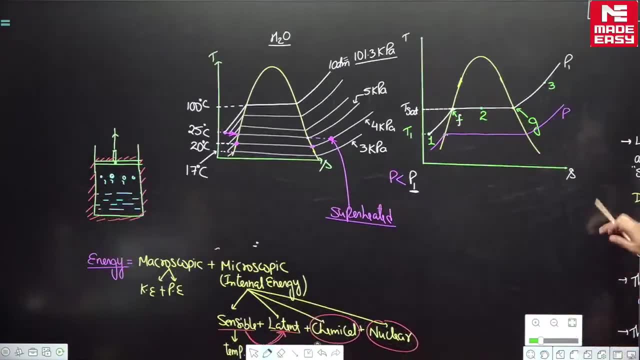 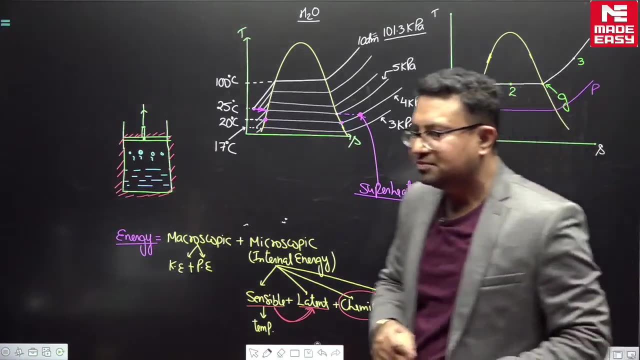 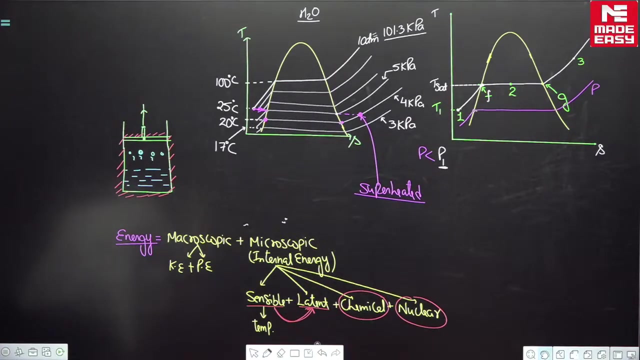 we are doing this discussion right now. whatever I have written, whatever I have written, I will show you in a different way, in a continuous discussion. I am just showing you this which I have discussed here. whatever points are written that I will show you, I will show you right now. this is the discussion. okay, now we will. Krishna Prakash, love you, sir, love you too, Krishna. 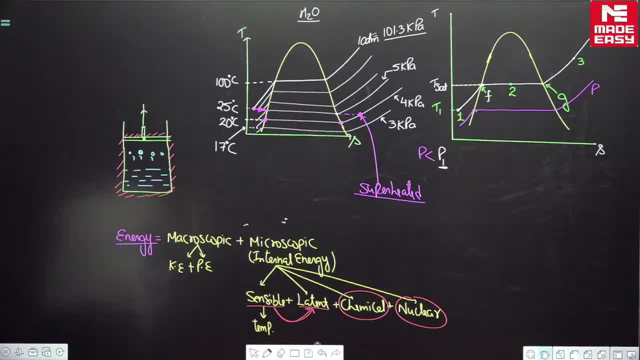 Sachin Patel. thank you, thank you to you too, knowledge hub. it is also the reason for drawing clothes at atmospheric pressure. exactly, exactly. this is the reason because see, when you, when you see the h2o, when you see, let me tell you this, but because we are discussing the depth of this, 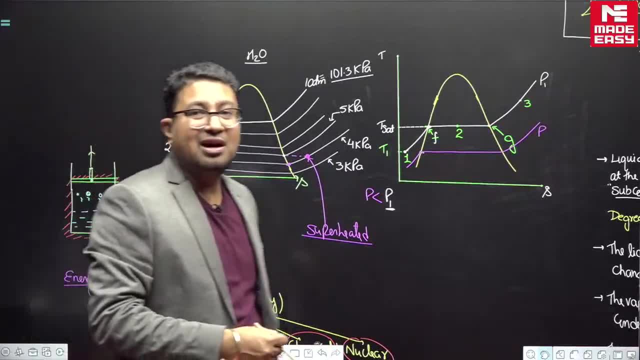 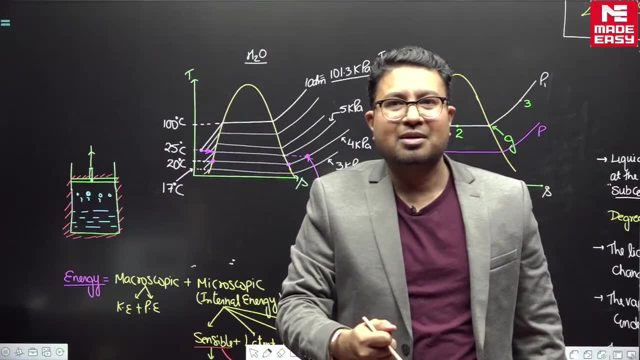 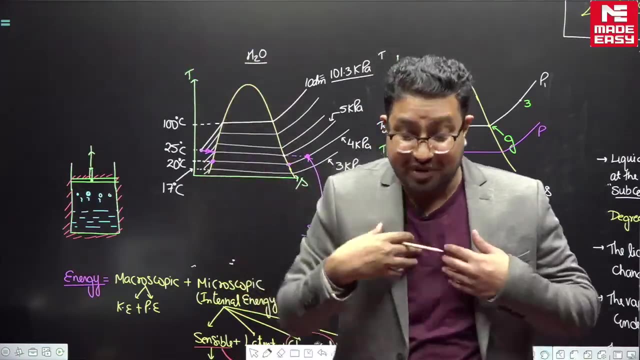 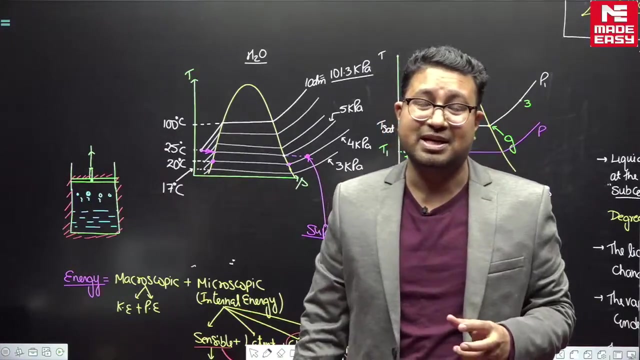 how the how the liquid exists as vapor state in the air, h2o, why it is in the vapor state in the air. we see water boiling at 100 degree celsius and even if the temperature is, if the temperature is 25 degrees celsius, then also how the h2o can exist as vapor. how can it stay in vapor state. understand. 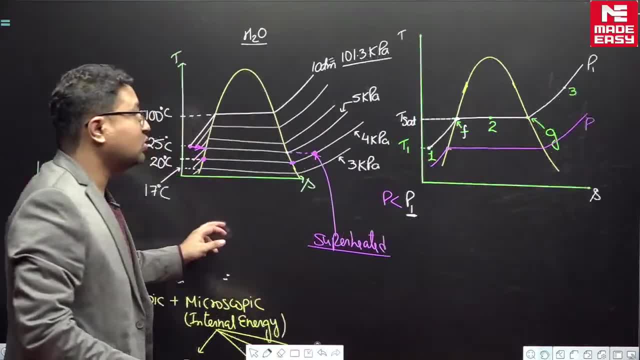 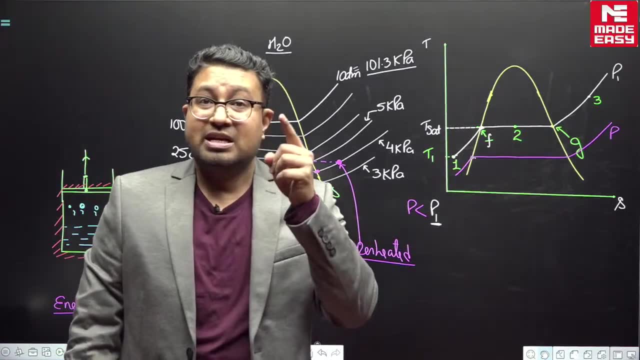 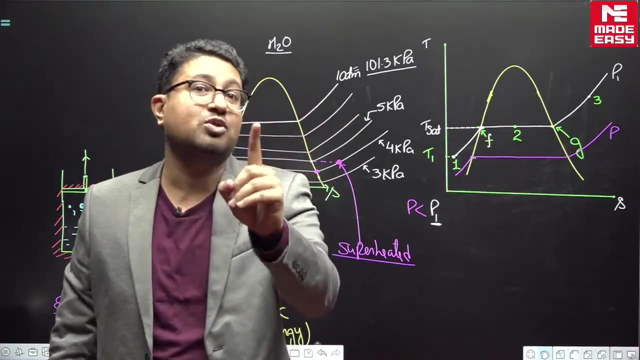 this thing, h2o. h2o will exist as liquid or vapor, depending on its own pressure. how much is its own pressure? air's total pressure is 1 atmosphere in the air. total pressure is 1 atmosphere in air. total pressure is 1 atmosphere. total pressure: 1 atmosphere is of air. but but what is the? 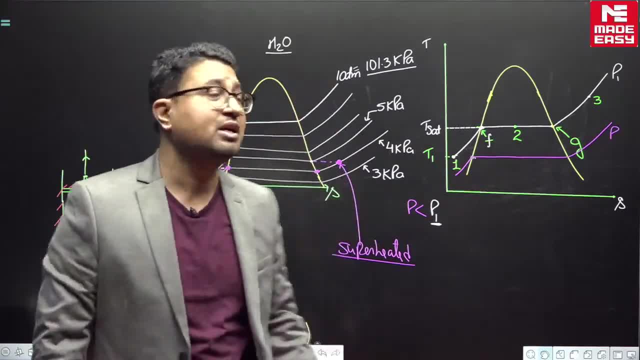 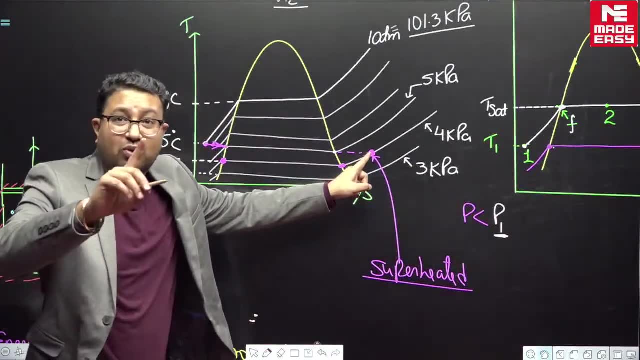 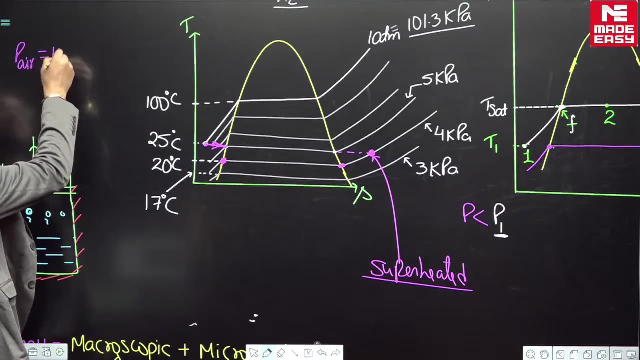 contribution of h2o In that. Now, if you see, if you look at this, if you look at this, that if H2O is 4 kilopascal, is the partial pressure the total pressure of air. if it is 101.325 kilopascal, if the total pressure of air is this, the total pressure of air is this, then in that, if we look at the pressure of water vapor plus pressure of dry air, it is about RAC, refrigeration, air conditioning. 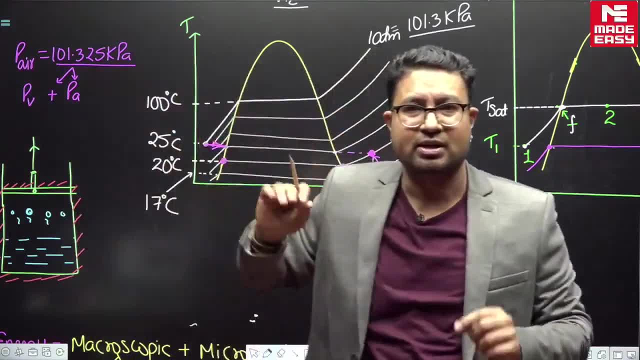 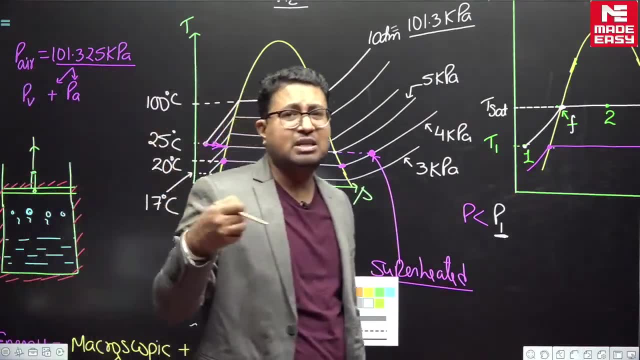 Dry air means the remaining air at O2,, N2, etc. Water vapor pressure is 4 kilopascal. You understand this thing, Understand, You will understand. And this is something in which the people have a lot of confusion. Books keep reading, but this cannot be understood just like that. 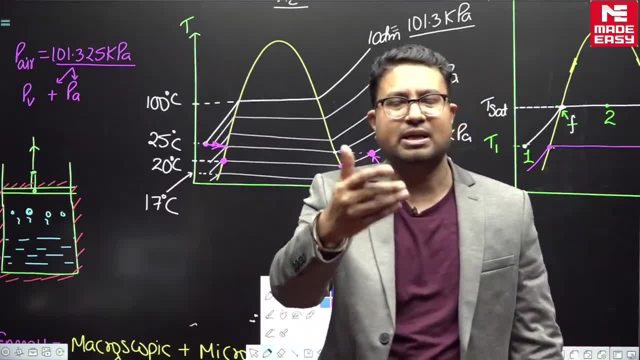 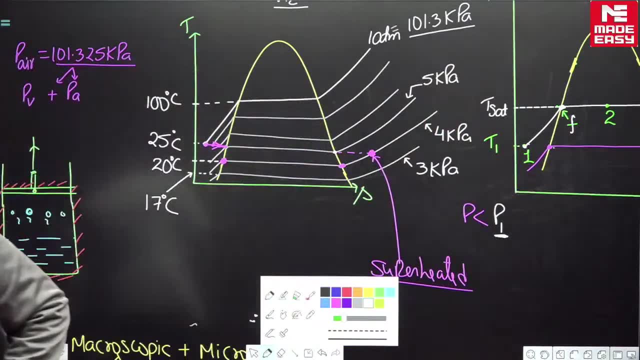 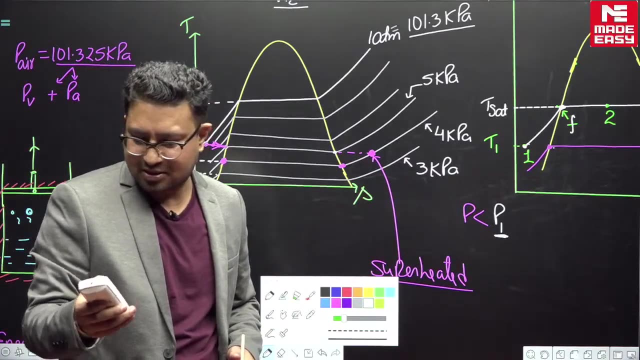 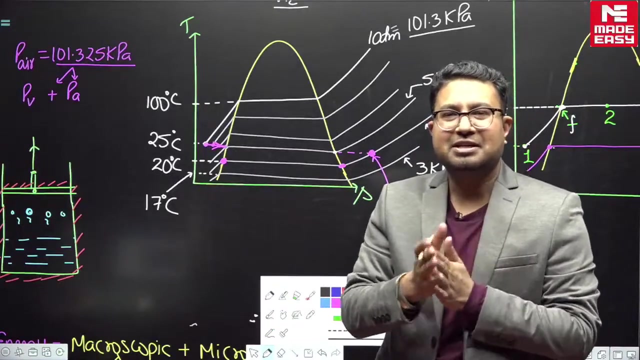 If we go step by step, we discuss, then it is understood and we can exactly understand not only thermodynamics, not only thermodynamics. we will be just. I think We are. let me switch on the air conditioner because there is a lot of heat that has been generated. The heated discussions are taking place. So see what you asked. what you asked, I am answering that. 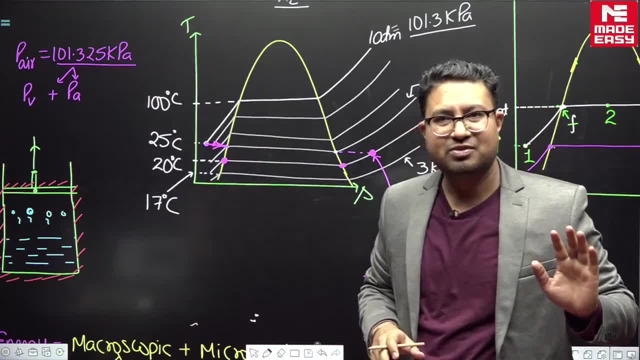 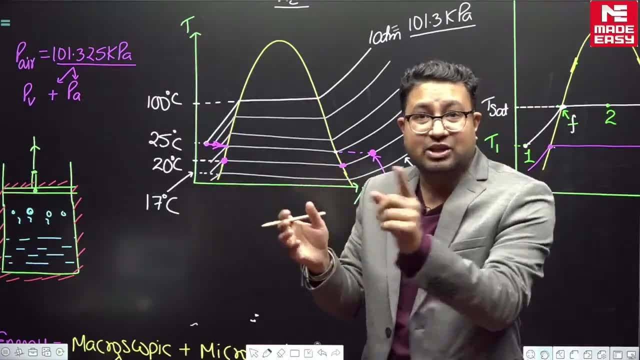 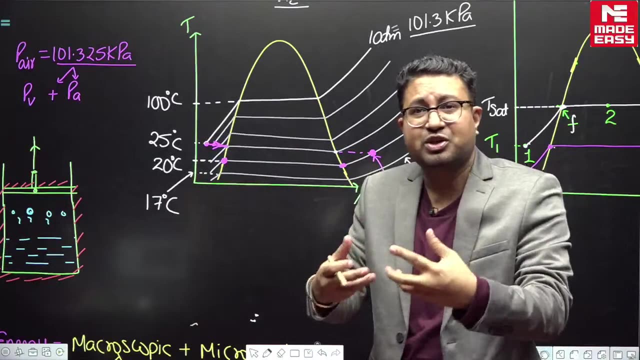 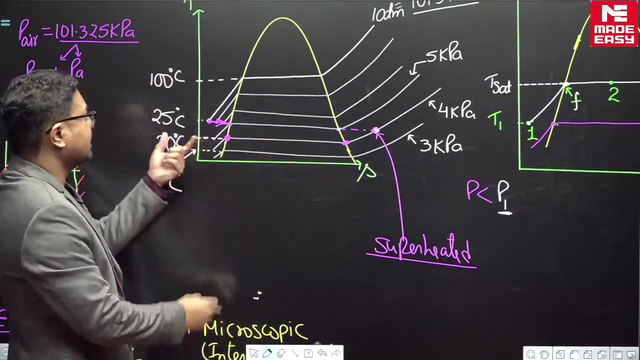 That in air total pressure is 1 atmosphere. but the vapor which exists, the vapor which exists, that can exist in the vapor form. H2O can exist in the vapor form Even though the temperature is 25 degree Celsius. let us say because partial pressure, the individual pressure of H2O, individual pressure of H2O, if it is 4 kilopascal, you see the individual pressure, how much is the pressure and what is the temperature. 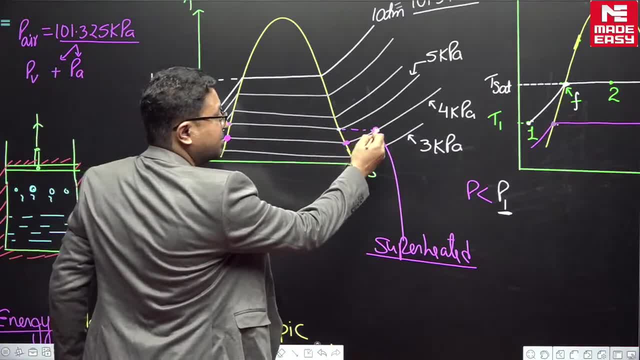 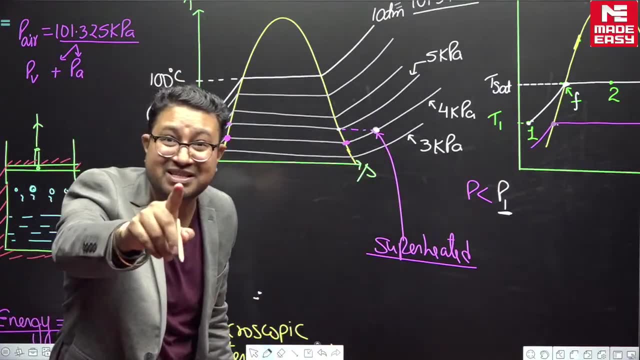 So at 25 degree Celsius, if the partial pressure of H2O is 4 kilopascal. so this is existing in the superheated state. it is existing in the superheated state. in the superheated state, and when will it condense? At 4 kilopascal? 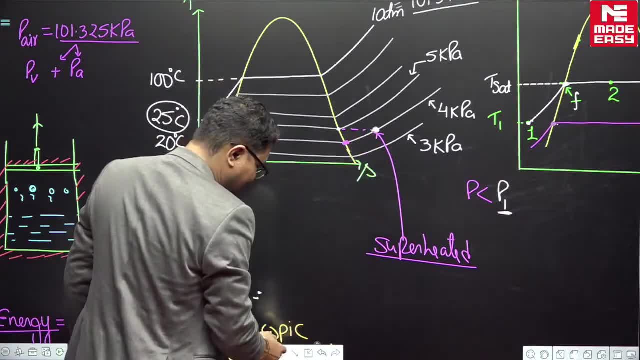 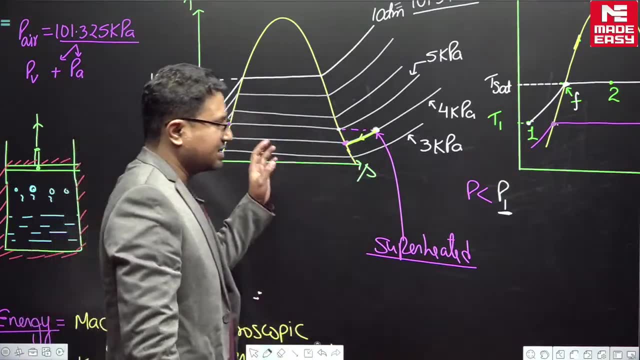 If you start cooling 4 kilopascal, if you start cooling, you will understand very well. If you start cooling at 4 kilopascal- this is something which I was not thinking of, but because this question is asked, you will understand. you will understand something. 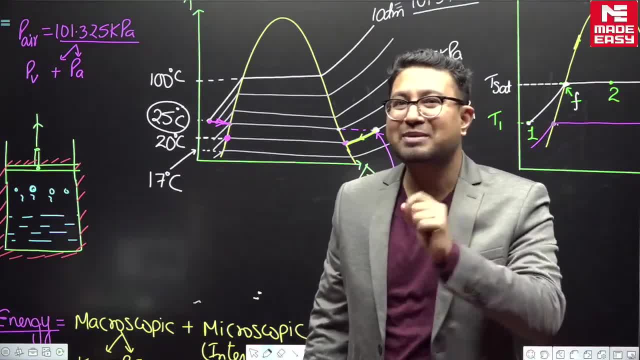 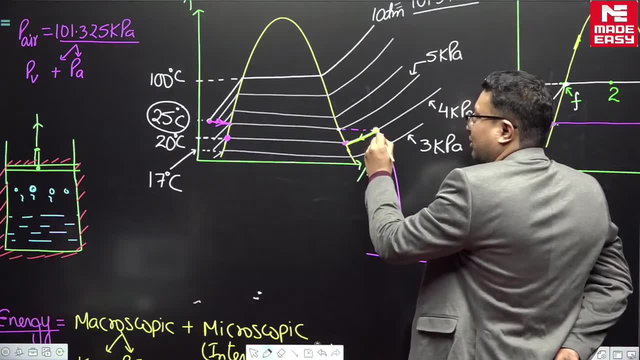 RAC makes term with a dew point, dew point temperature. So let us assume there is water vapor in the air, there is 1 atmosphere, 25 degree Celsius, 4 kilopascal. So there is 1 atmosphere, but pressure due to H2O is 4 kilopascal, So you will be lying here. 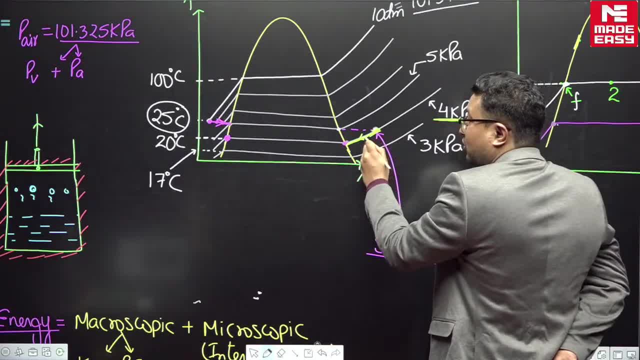 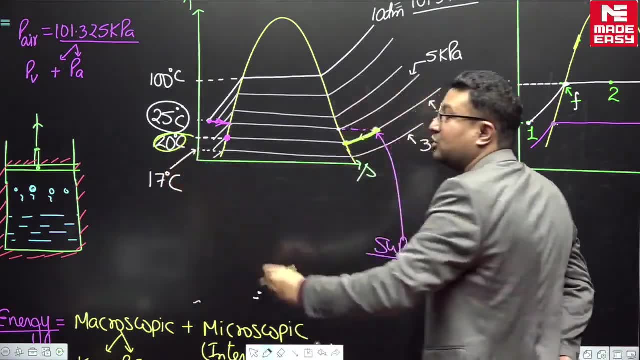 Now if I start cooling, now if I start cooling, so H2O at 4 kilopascal, at what temperature does it condense? It condenses at 20 degree Celsius. So 20 degree Celsius will become the dew point temperature of the air. 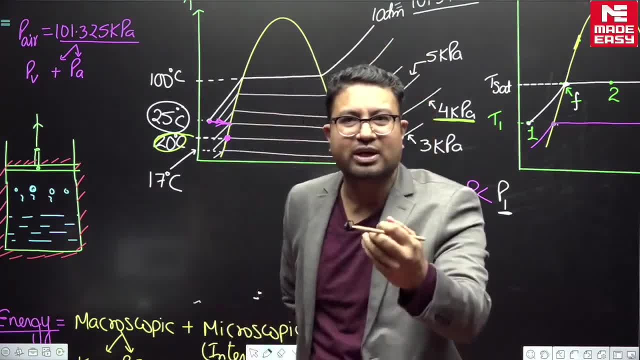 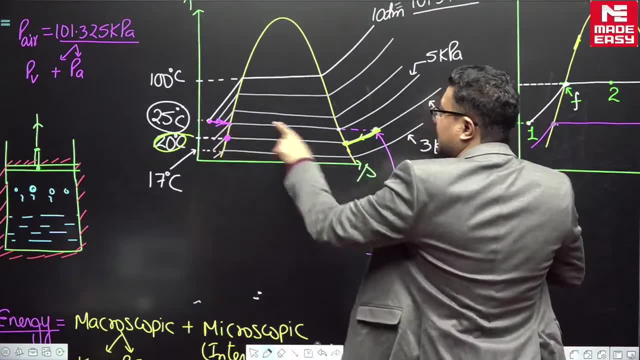 The dew point of the air. dew means it will start becoming os. if you cool the air, then H2O will also cool. H2O present in the air will cool. So H2O is at 4 kilopascal and 25 degree Celsius. 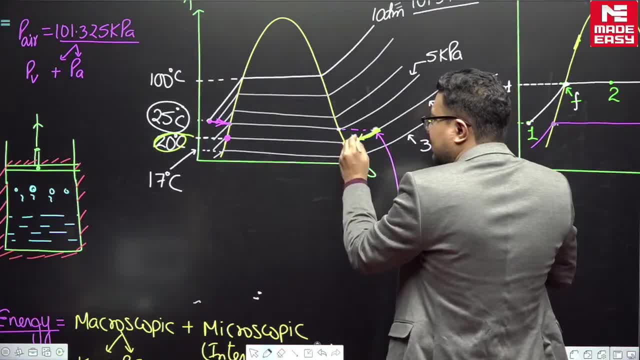 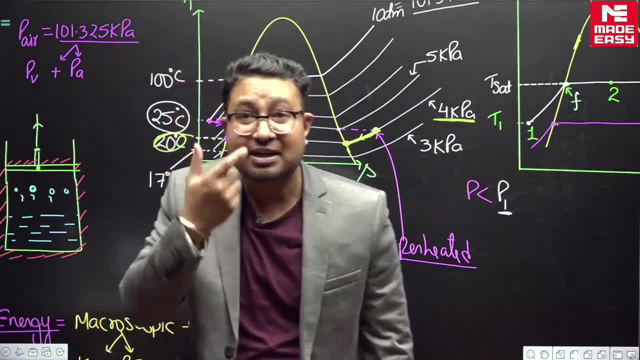 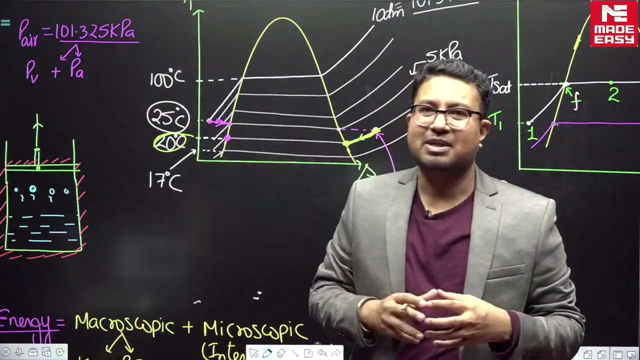 So when it will start cooling, When it will start cooling, then at 20 degree Celsius, it will start condensing. it will start condensing. so that is the dew point temperature. How do we define dew point temperature? Dew point temperature is the temperature. do you understand how? I will not write it, because this is something which is related to RAC. 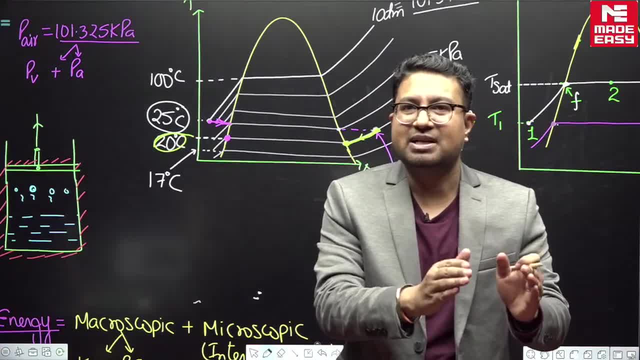 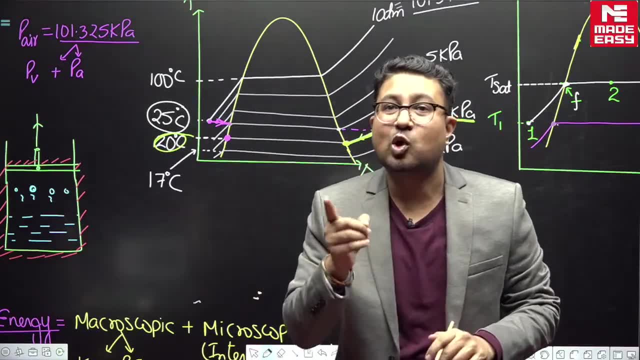 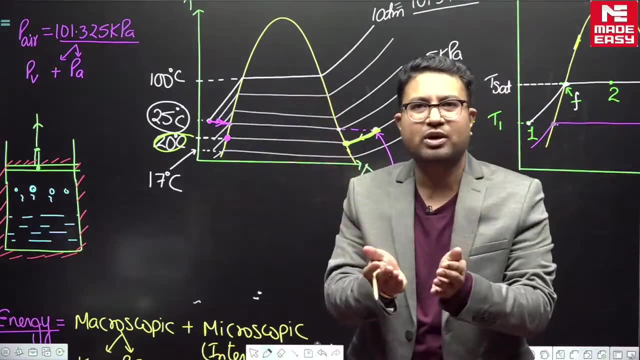 Dew point temperature is the temperature at which at which the water vapors in the air starts condensing. water vapor present in the air starts condensing when cooled at constant pressure. What does it mean? So if the pressure of air is constant in one atmosphere, then H2O also pass 4 kilopascal. 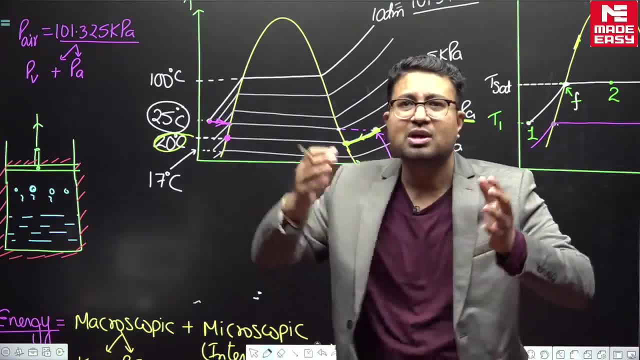 H2O also pass 4 kilopascal. do you know how to keep the pressure constant in the passing atmosphere, as you which have to cool But infinite air? it will reduce the volume, will keep the pressure constant. what problem? The volume decreases, is it not? you also cool. Volume will reduce. pressure will remain constant. There is no pressure for it. You are not cooling it in the rigid container how you are cooling in the rigid container, as the volume should remain constant. 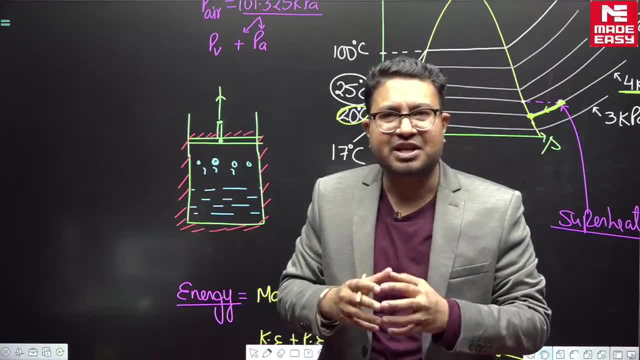 Normal cooling will be like this: Air will shrink, air shrink kar jayegi Kitchen mein khana banate ho. when you are cooking in the kitchen, air gets heated up to pressure. thodi padh jata hai 1 atmosphere to 2 atmosphere. 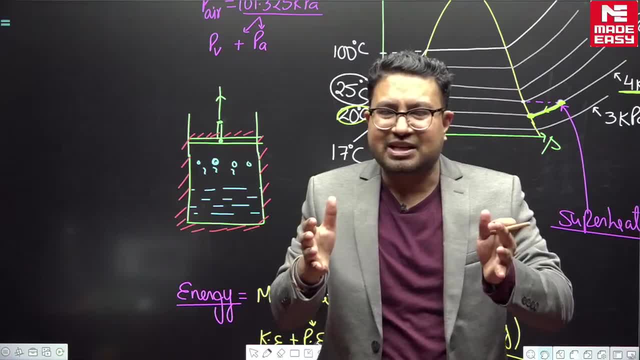 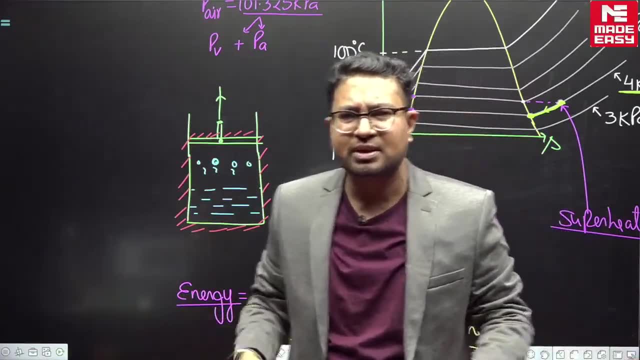 the mass of the air that was present in the kitchen. it expands, so it goes out. some of the air goes out. the mass of the air in the kitchen reduces. Kitchen mein jo air ka mass ho reduce, ho jayega hai. So this is the discussion which we have done, Fine. 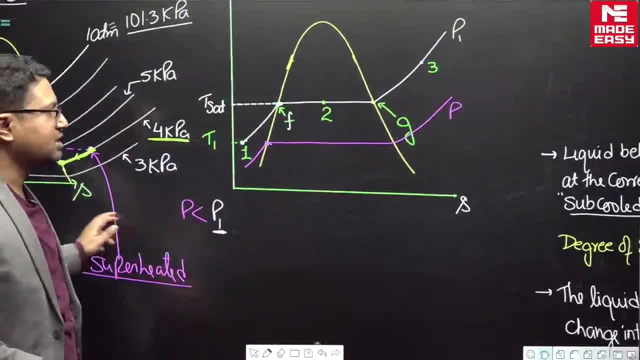 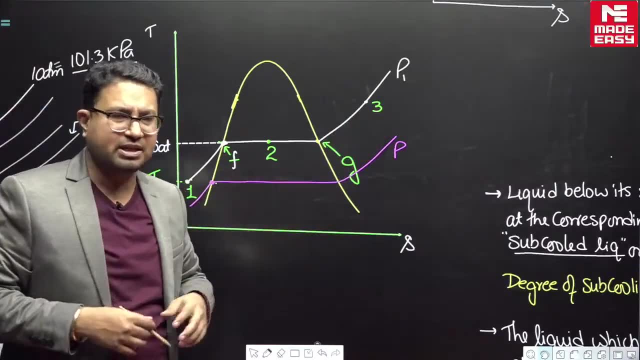 now see, let us see, let us move forward apne discussion. pe aage badte, So I have just shown this aapko agar screenshot lena tha now or afterwards. I think you can take it. so now, degree of sub cooling: tak, we have discussed fine. 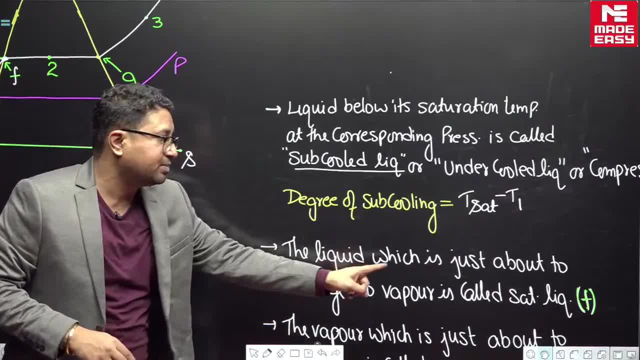 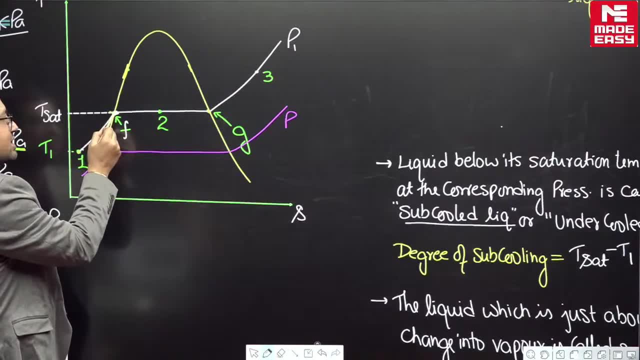 the liquid which is just about to change into vapor is called saturated liquid, So sub cooled gaya hai. below the saturation temperature is sub cooled liquid. now, this is the condition. the liquid which is just about to change into vapor, Jo liquid, just vapor. mei change hone wala hai. 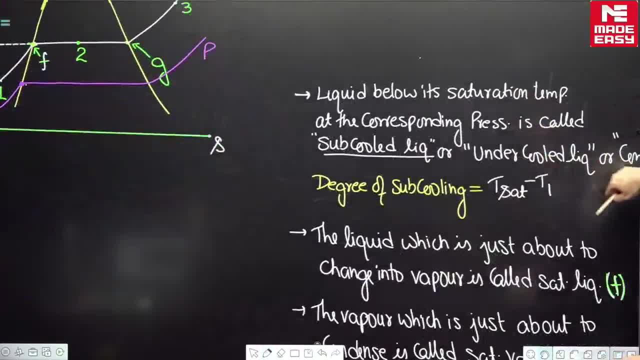 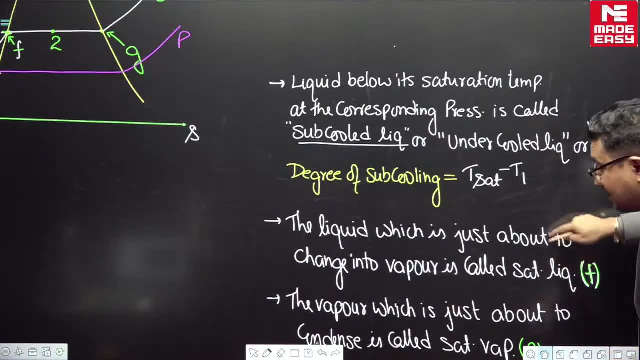 that is called as saturated liquid. So this is the liquid which is just about to change into vapor, is called saturated liquid. We denote it with f hum usse, f se denote karte hain. The vapor which is just about to condense is called. 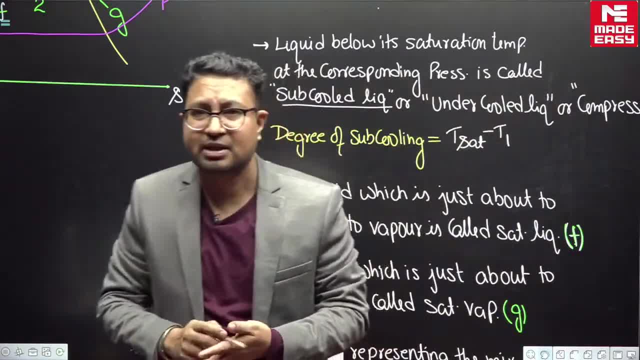 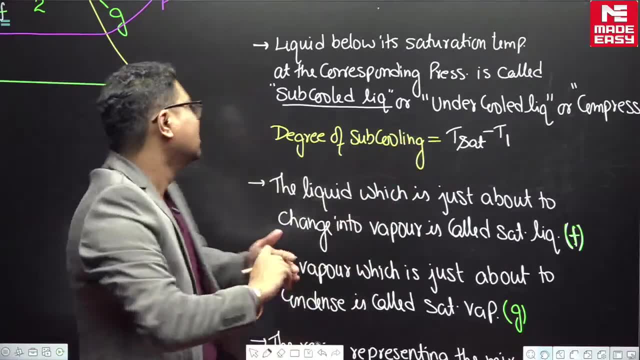 saturated vapor. Saturated vapor kab kehte hai, But jo just abhi abhi vapor bana hai, The vapor which has just been formed. Now, if you remove some heat it will condense. So if the vapor is in this condition, agar vapor. 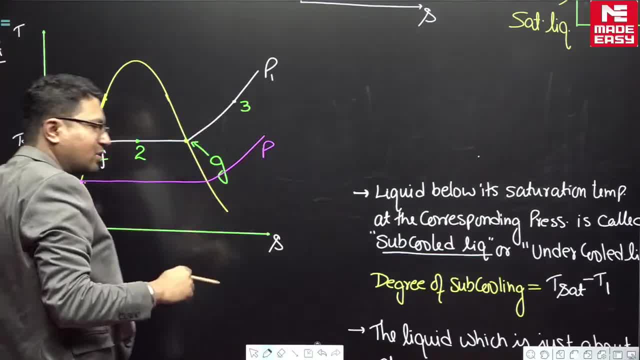 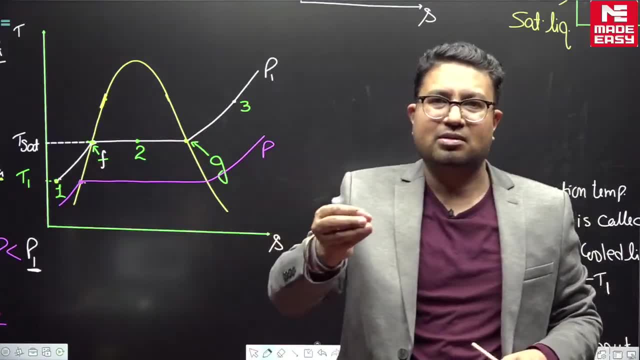 is condition mein hai. you start removing heat, so condense kar jayega na, Because after changing into vapor it has not got further energy usko. So if you heat, then its temperature will increase, But if you take out heat it will condense. 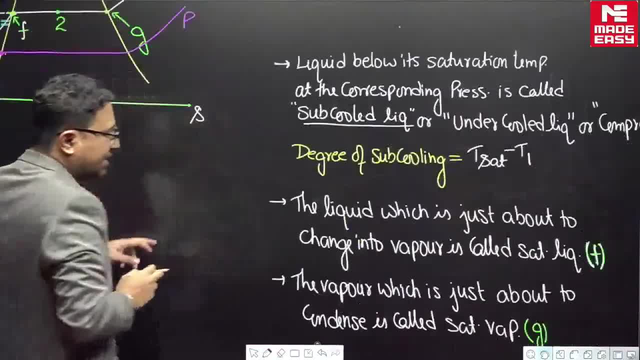 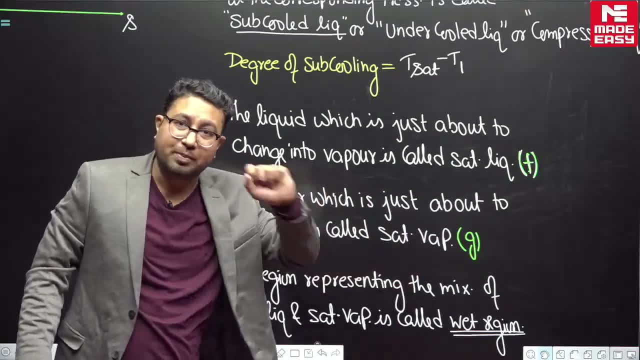 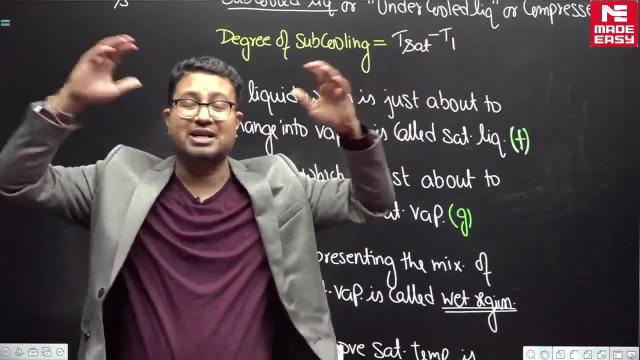 It will go back to its liquid condition. So we can say: the vapor which is just about to condense is called saturated vapor. Now see what is superheated vapor. Superheated means not that generally what happens in our mind is that superheated H2O. 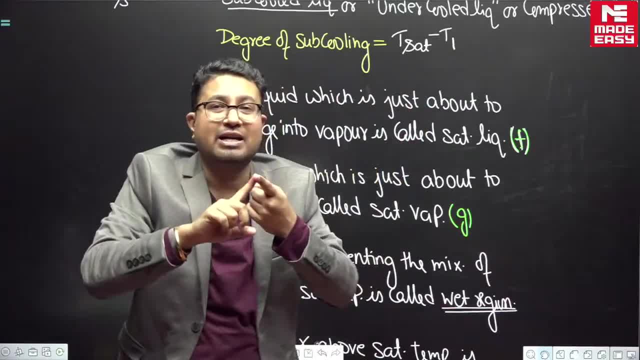 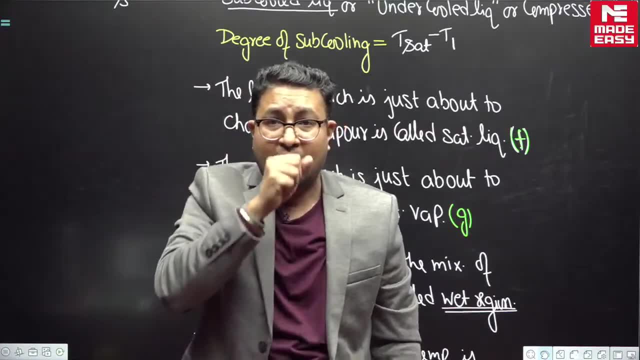 means at least it should be very hot. It should be very hot. It is decided by the combination of temperature and pressure. The present water vapor in the air is mostly in the superheated state, But because the partial pressure of water vapor is very less, 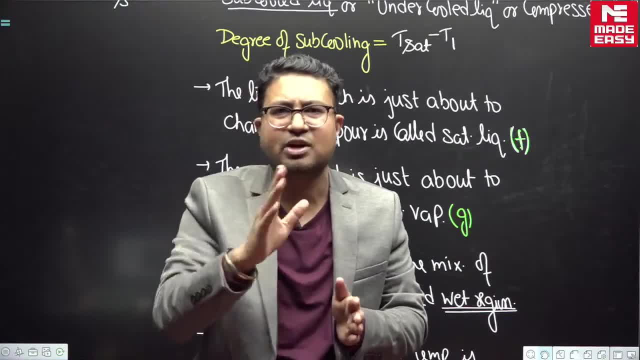 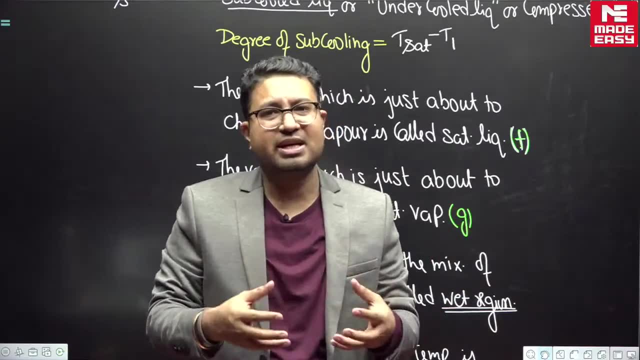 So even at very low temperature, it can exist in the superheated state. You must have understood If there would have been any confusion regarding this, Because people have confusion, But discussion is required to understand this And that, like sometimes people ask me doubt. 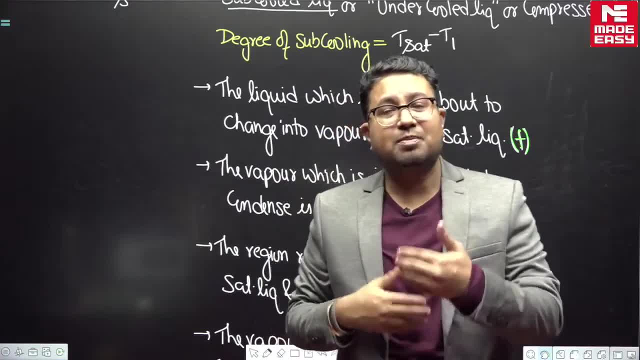 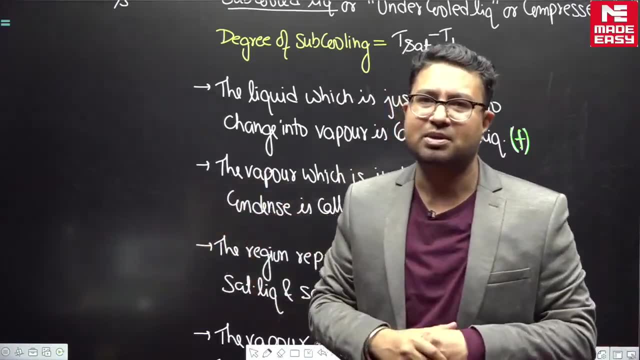 So, sir, tell me in two minutes how it happens. It is not see, I will tell you, but it is not possible for you to understand till we do a lengthy and complete discussion. It does not become possible to convey this. Convey karna possible nahi ho paata. 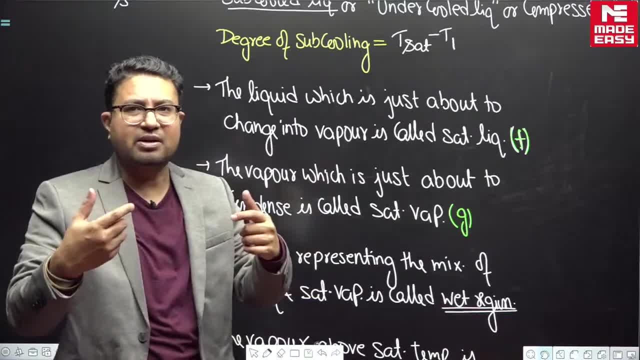 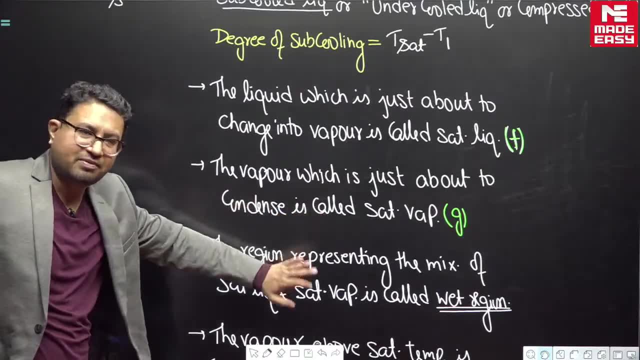 But step by step, agar am discuss karte. So there is nothing which we are not able to understand. Kuch bhi aisa nahi jo hum nahi samajh sakte. Now, the vapor which is just about to condense is called saturated vapor. 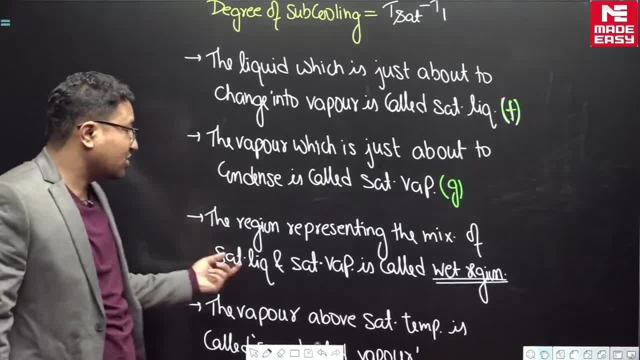 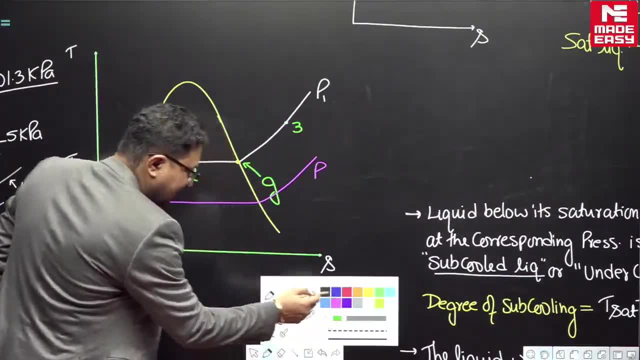 Fine Dekho. the region representing the mixture of saturated liquid and saturated vapor is called wet region. I told you Kya Isko wet region bolte. We call this as wet region. So if you are here, Agar ab yaha ho. 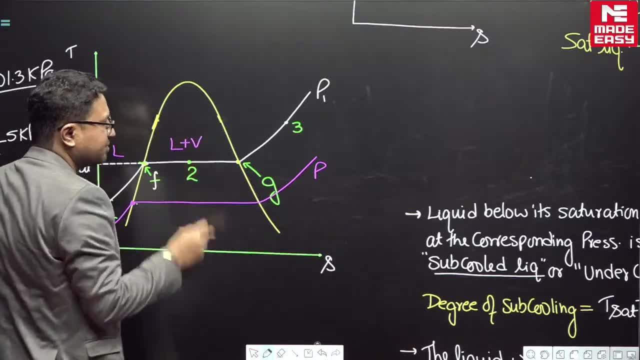 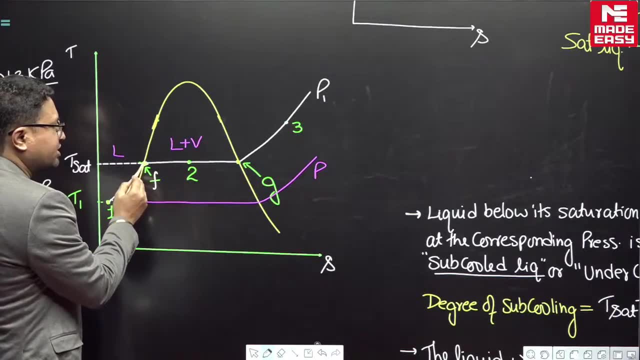 You are in the liquid state Here, liquid plus vapor. that is the wet region. Now sub cooled liquid, Saturated liquid, Wet region. Matlab kuch saturated liquid hai. Some is saturated liquid and some is saturated vapor. Fine Wet region, bolte. 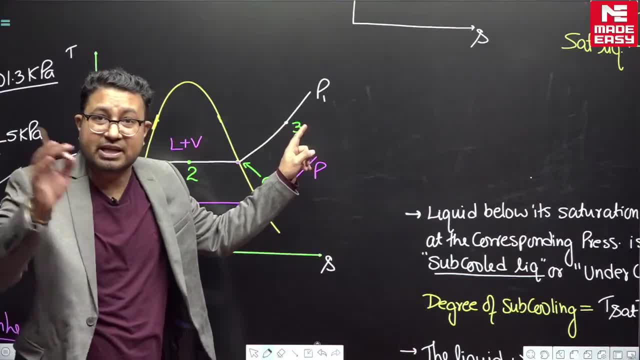 Now point three: Superheated vapor. Superheated vapor ka matlab, kya Dekhna, Ye hi se samajhna. I have already written the definition, Likhi hu hi hai, But samajhengi ye hi se. 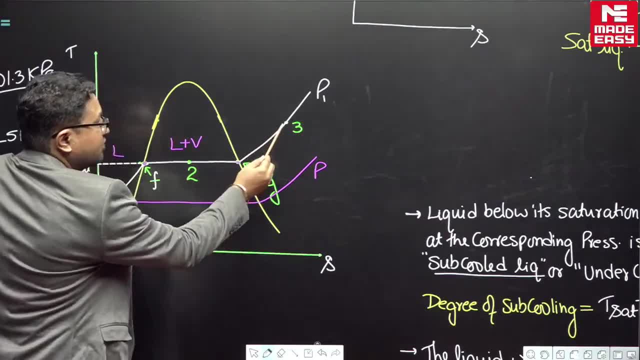 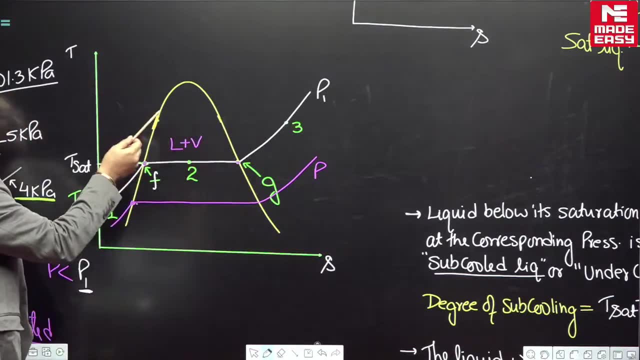 The vapor Vapor present above the saturation temperature. Ye jo vapor hai Saturation temperature: ye hai na. This is the saturation temperature. The vapor present above the saturation temperature at the corresponding pressure. Isi pressure pe. Isi pressure pe Saturation temperature se upar. 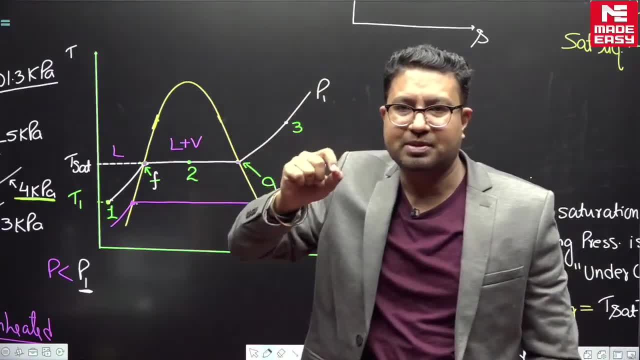 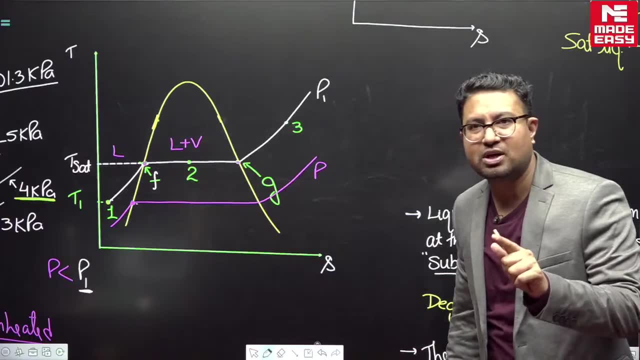 Above the saturation temperature, The vapor which is present, Jo vapor present hai, That is called as Is vapor ko kya bolte. Is vapor ko bolte. This vapor is called as superheated vapor. This vapor is called as superheated vapor. 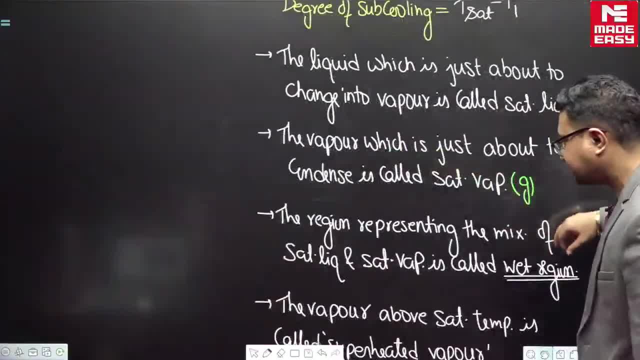 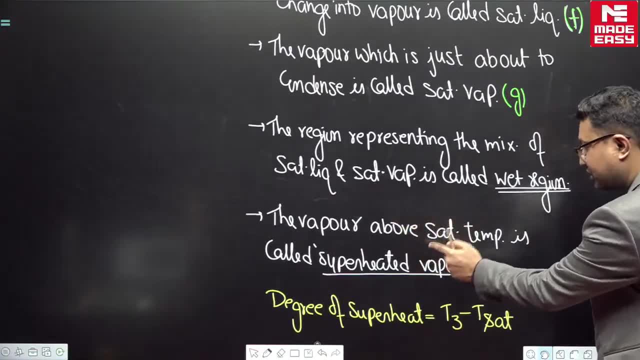 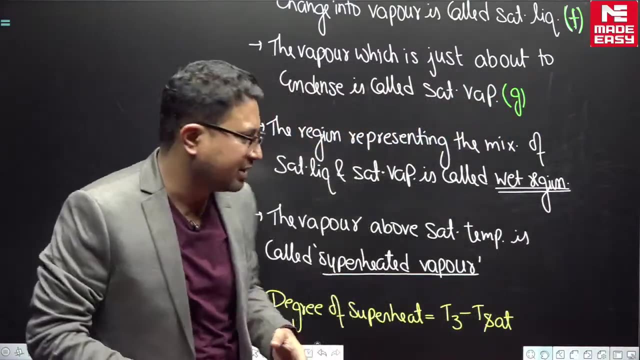 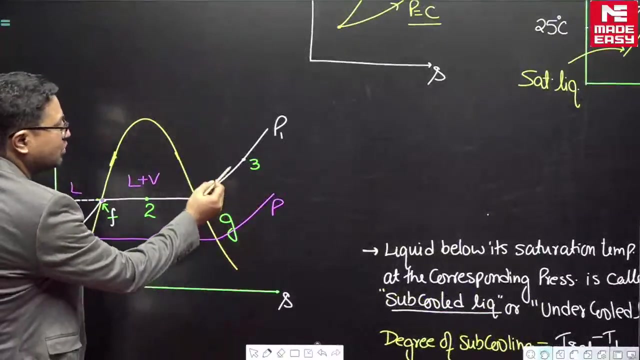 Okay, So we can see here. Hum yaha dekh sakte already written. the vapor above saturation temperature is called superheated vapor. so what is degree of superheat? degree of superheat is equal to t3 minus t saturation t3. what is t3 degree of superheat, t3 t3 temperature? 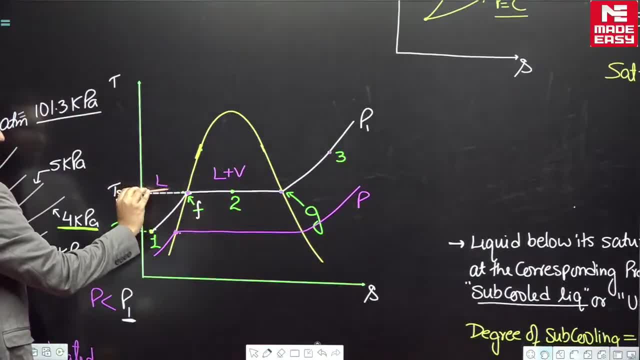 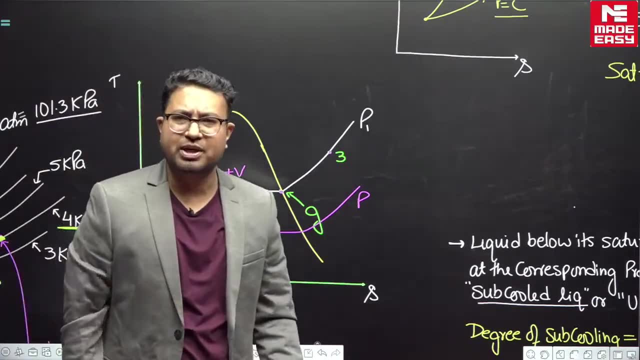 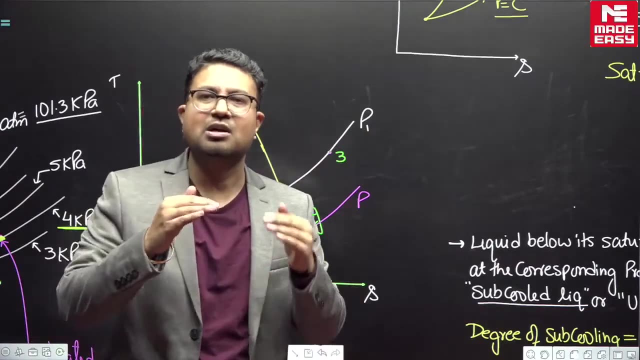 abhi kitna hai Minus. what is the saturation temperature? What is the temperature now minus? what is the saturation temperature? Saturation kya? That is the degree of superheat. This is suppose H2O hai. H2O 120 degree Celsius pe hai 1 atmosphere pe. Saturation temperature: 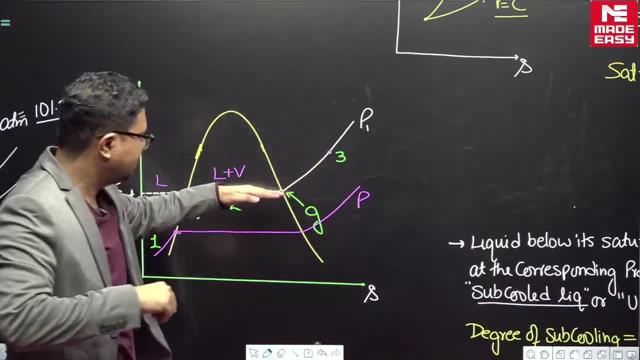 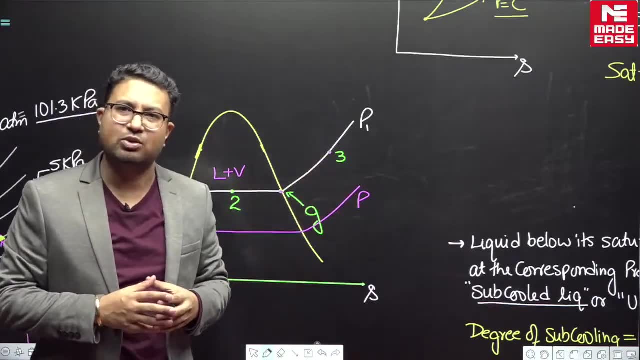 means phase change 100 pe hota hai. You are at 120, let us say Phase change takes place at 100.. So 120 minus 100, that is 20 degree superheated, is your condition? Ye, apki condition hai, 20 degree superheated. So all these statements I will show you. Then there is: 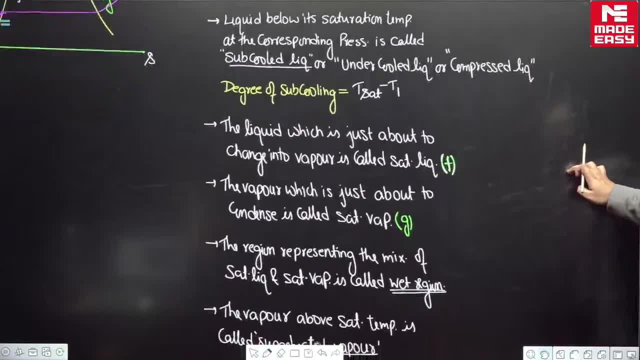 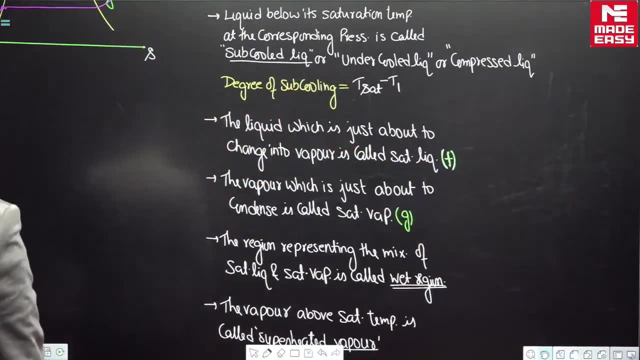 a discussion which I have to do further. Ma apko ek baat dikha deta hu. If somebody wants to note down or take a screen shot, Note karne ka pura to time nahi I will be able to give, But step by step, whatever discussion we are doing, I will just show you. 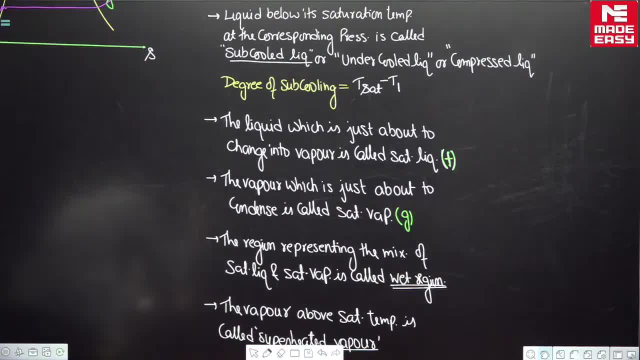 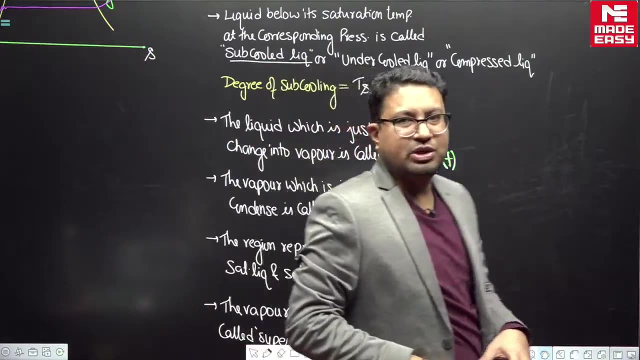 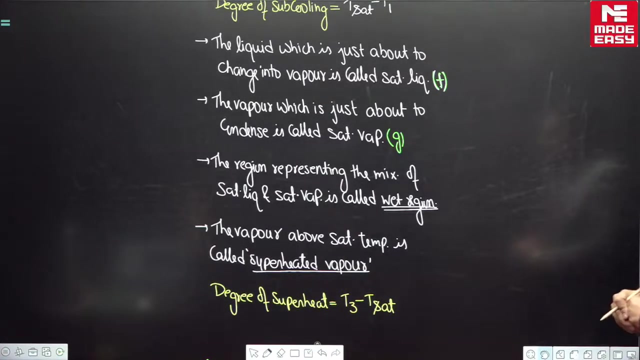 Fine, So now, now see, now see here, here, now see. this is something which I have further written. you can just see this. So we have discussed the details of how the saturation curve is being made. I am leaving it like this: only, How can we make a saturation curve? 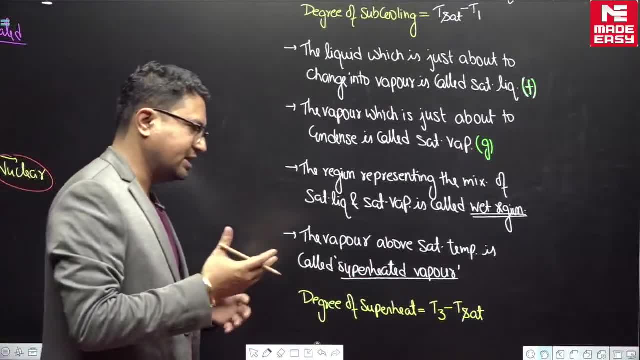 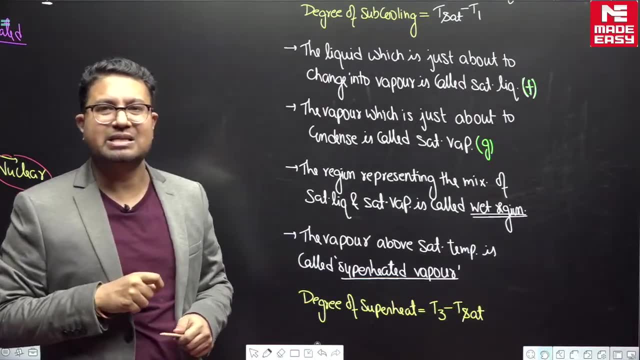 This is the main point I have told about in my lecture, So that is why this is called. have discussed the details, how the saturation curve is made, and minute details regarding the existence in the various phases, like existence in liquid phase or liquid plus vapor phase. 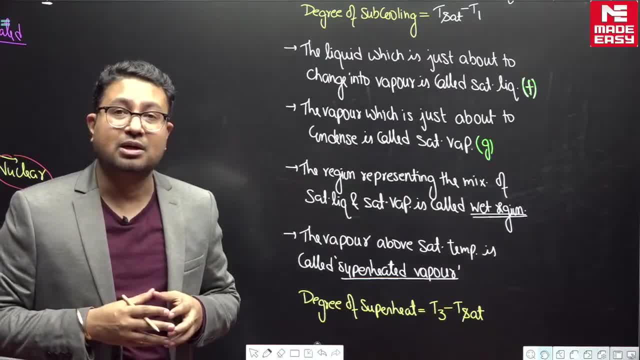 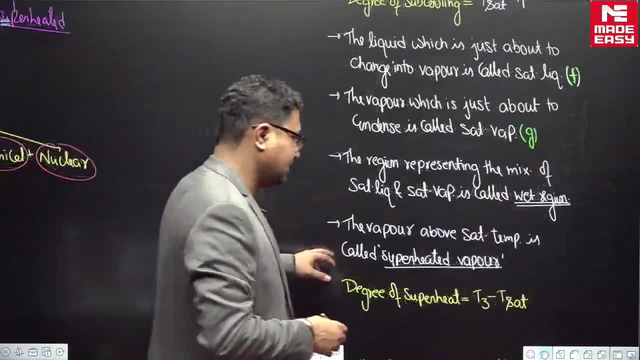 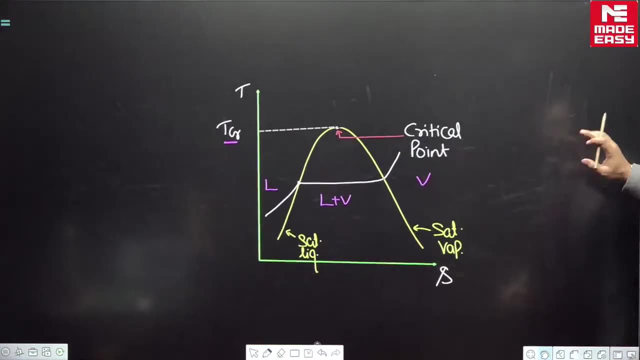 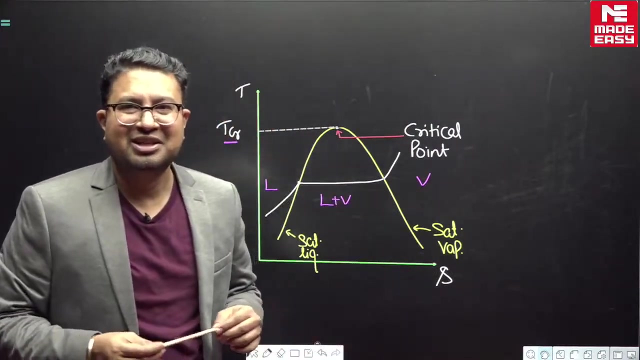 or vapor phase. So minute details about that I have discussed. Now let us talk further about this. So here now I have one more diagram, just a fresh diagram, because explaining things on a single diagram becomes complicated. So we have a fresh diagram. 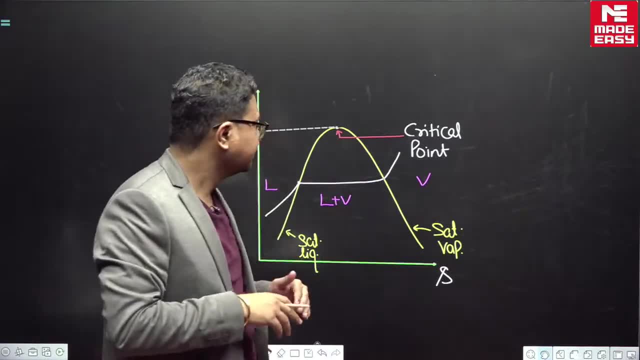 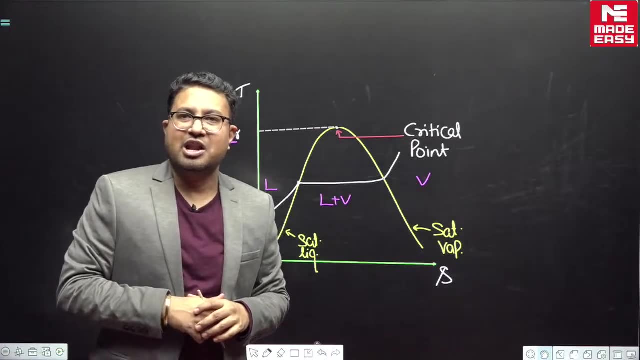 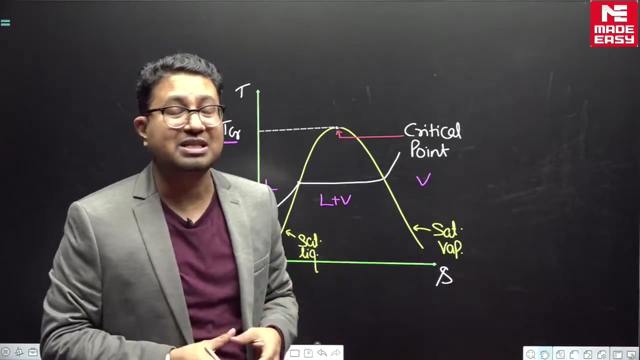 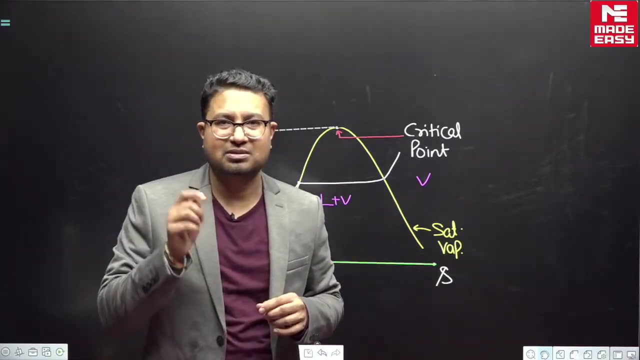 So here, if we see- I have shown this saturation curve- this is liquid, this is liquid plus vapor, this is vapor vapor condition. Now, this is critical point. What is a critical point? Critical point is a point where both saturated liquid and saturated vapor curve meet. 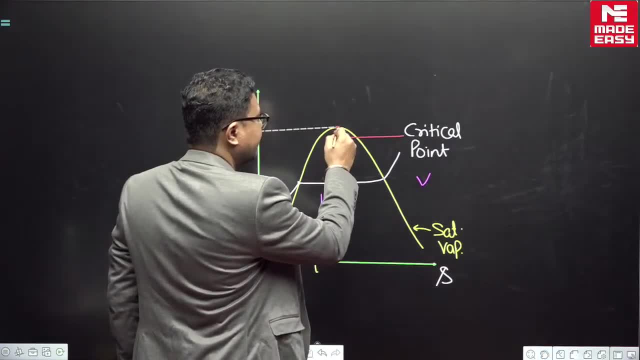 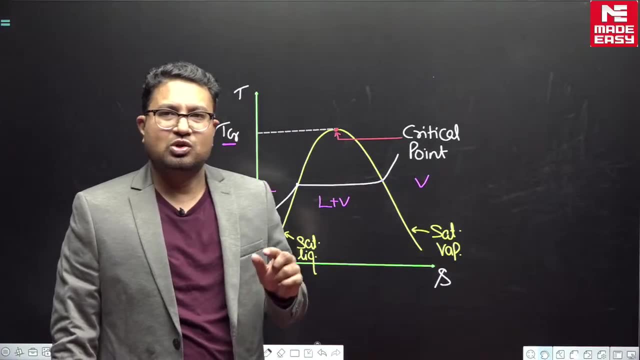 Critical point is a point. Critical point is a point where saturated liquid and saturated vapor curve meet. Now we will talk more about this. This is a critical point. Critical point is a point, and I have also written, so there is no need to worry. 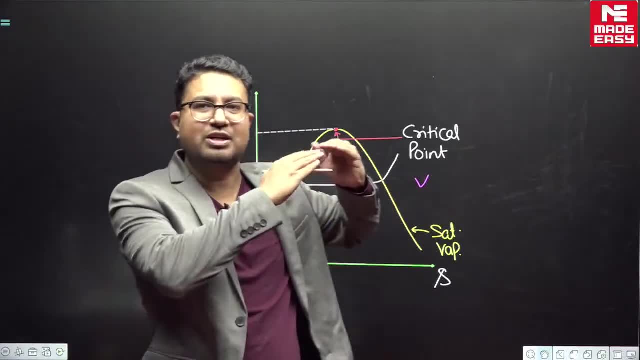 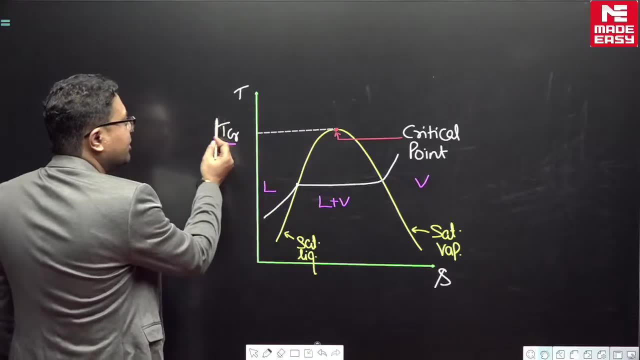 So critical point is a point where saturated liquid and saturated vapour curve meet. Saturated liquid and saturated vapour curve meet here. that is the critical point. Now, this is the temperature corresponding to critical point. The temperature corresponding to critical point, this is T critical. 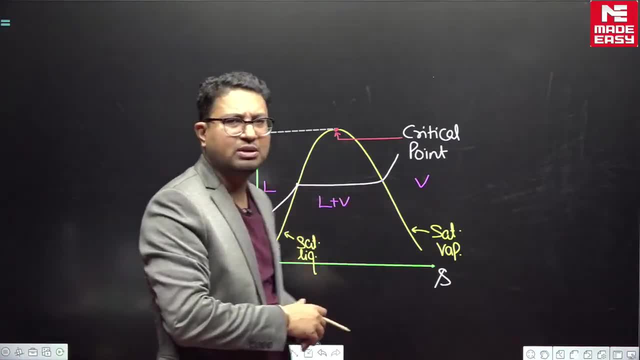 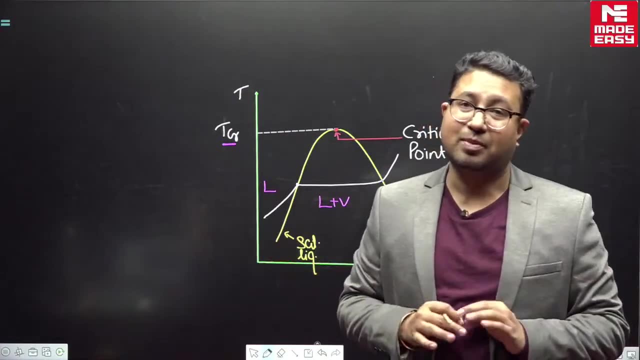 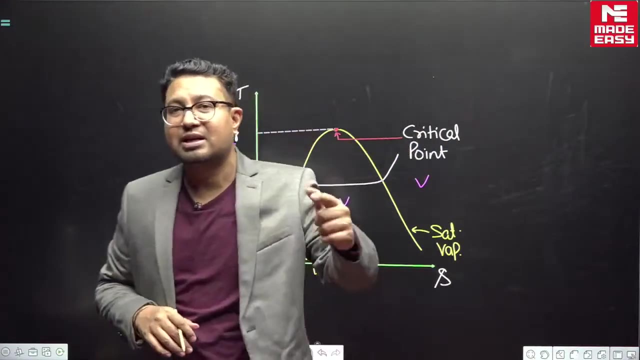 For water, this temperature is 374.15 degree. I have written Now: property of every substance. there is a property of each and every substance. There is a property of each and every substance that if you keep it above critical temperature, 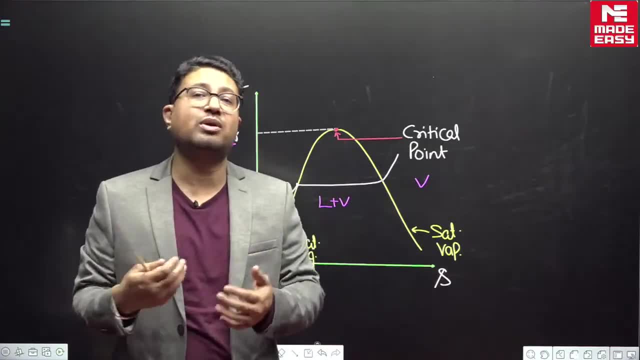 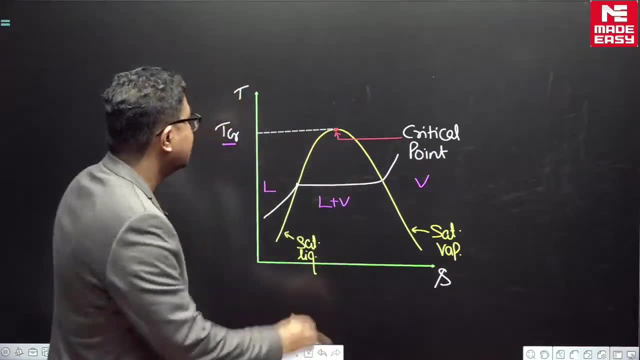 if you keep it above critical temperature, no matter at what pressure you keep, it cannot exist in the liquid state. That means critical temperature. irrespective of the pressure, irrespective of the liquid state, irrespective of the pressure, you are vapour. 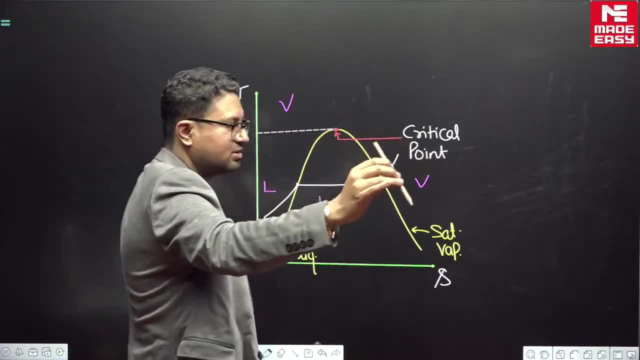 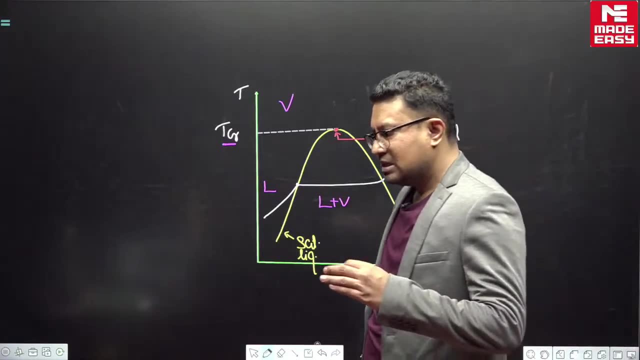 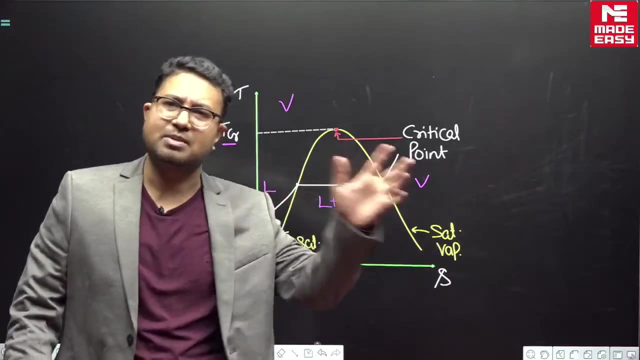 Above critical temperature, above critical temperature, liquid cannot exist. I am repeating this again, I am repeating it again: There is a property of the substance. there is a property of the substance that, above any substance, it is not only about water. 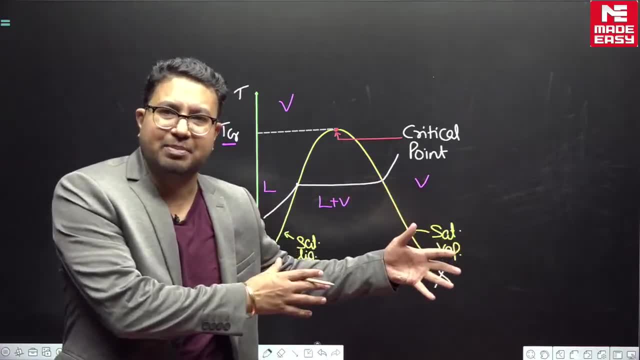 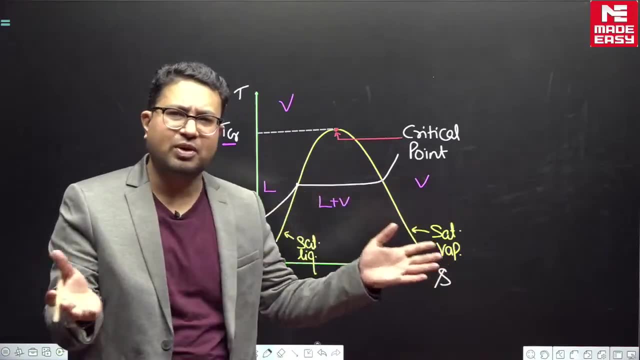 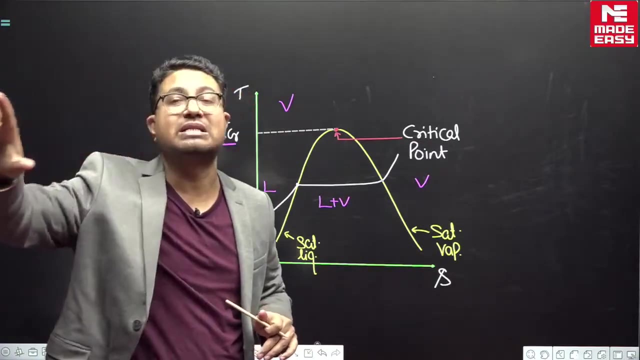 it is for every substance. We are just taking water as an example. We are taking water as an example. Things are common for whatever we are talking about in general. they are common for every substance. Above critical temperature, above critical temperature, liquid state cannot exist. 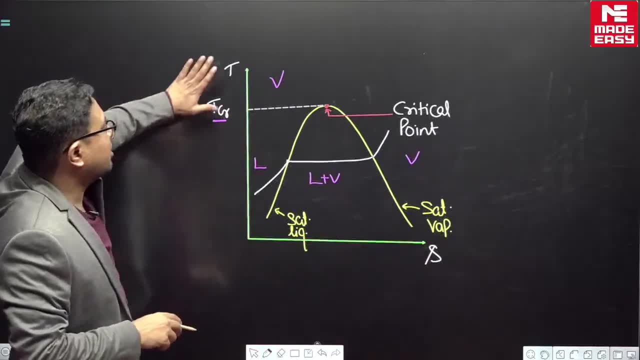 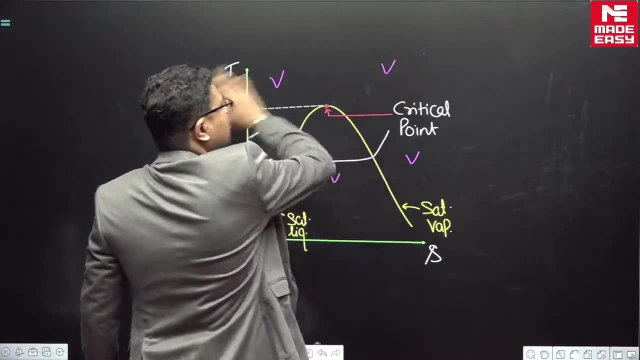 Liquid state cannot exist. So liquid state cannot exist. You are only vapour. What are you? You are vapour. Here liquid liquid plus vapour, here vapour and here vapour. Everywhere, everywhere, you are only vapour. 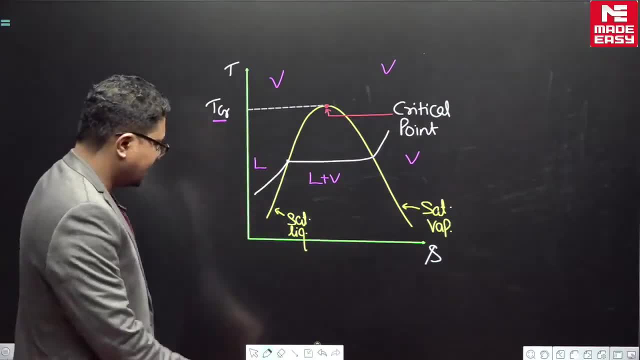 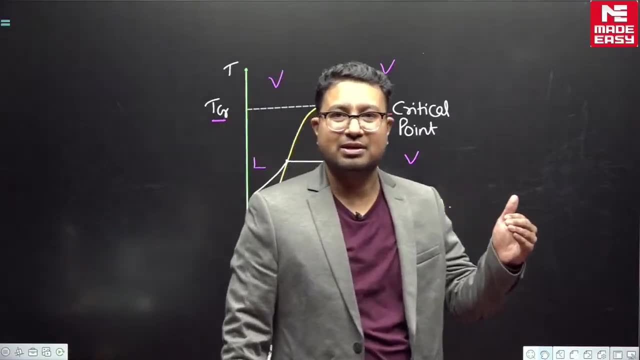 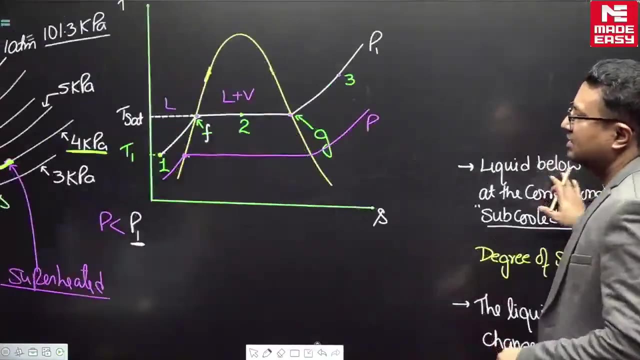 You are only vapour. Okay, Now you see, as the pressure increases, as the pressure increases, we see above everything I told you. I have already written which is relevant to us. I have written all that and have stood up and done it step by step. 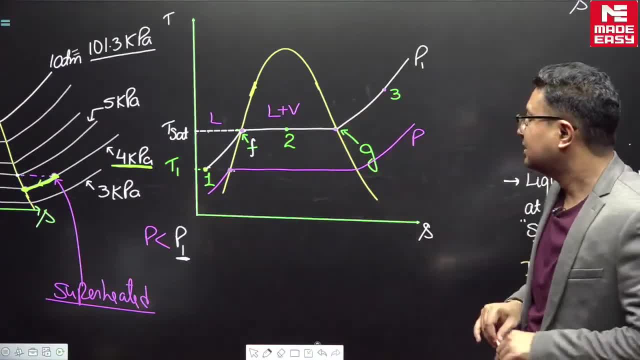 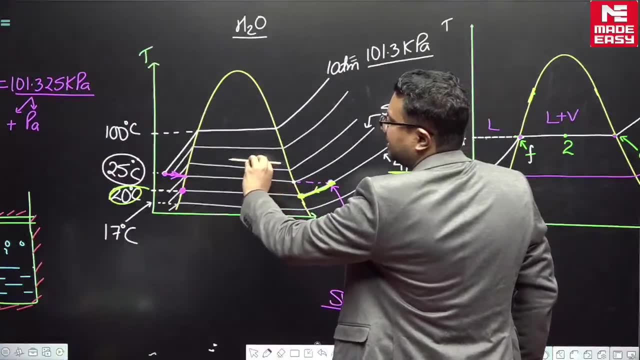 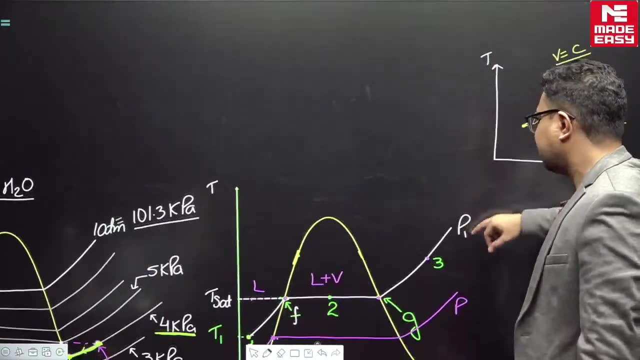 so that we are able to make the diagram understand things and write it. As the pressure increases. as the pressure increases, the boiling temperature increases. as pressure increases, boiling temperature increases The temperature at which the boiling is taking place. at whichever temperature the boiling is happening. 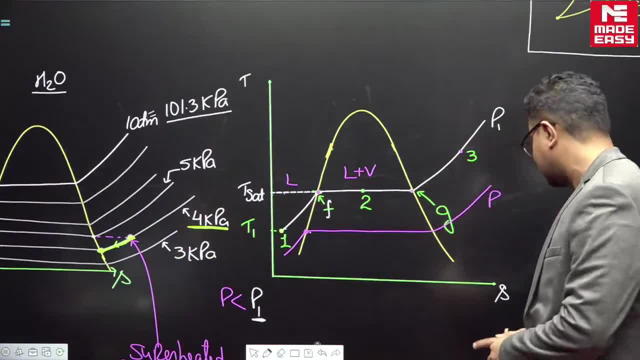 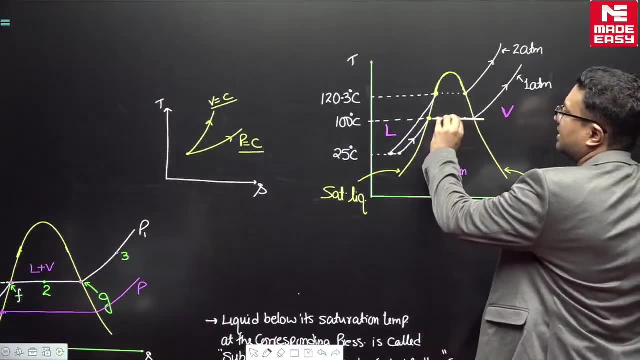 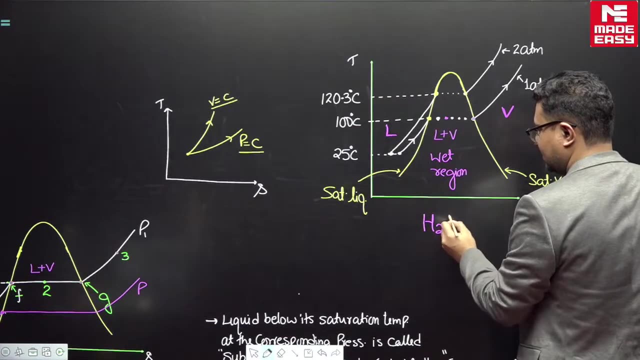 As the pressure increases, the boiling temperature increases. the boiling temperature increases, Just say, one atmosphere corresponding 100 degree Celsius for water. obviously we are talking about water here. I am writing with my left hand, just for a change. So we are. 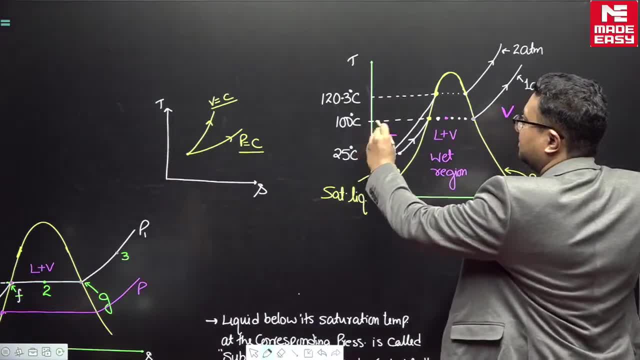 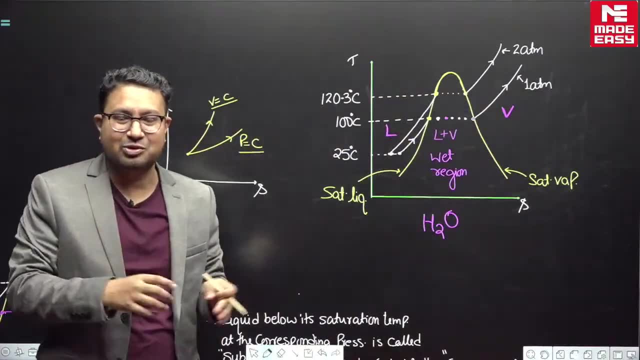 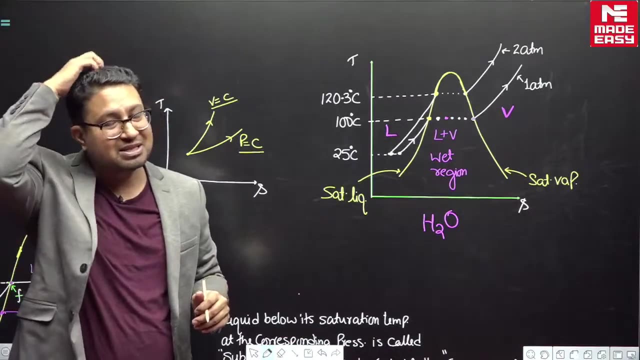 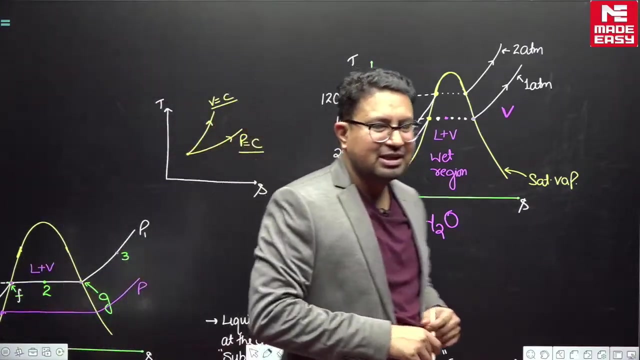 talking about water, 100 degree Celsius. it is When I was a kid- I was- I tried to use both my hands, they told So. I tried to write many days, I mean for many months. I tried and I started writing also, But I was very slow in writing. I am right hand person mostly. 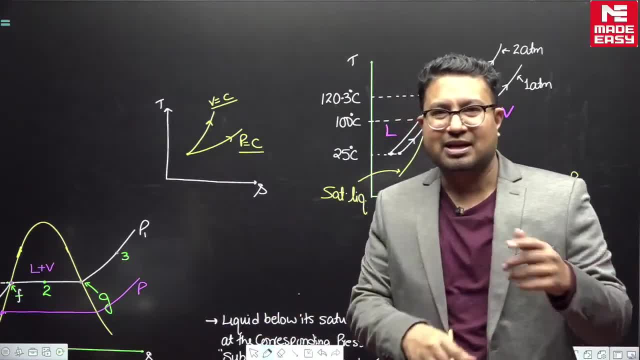 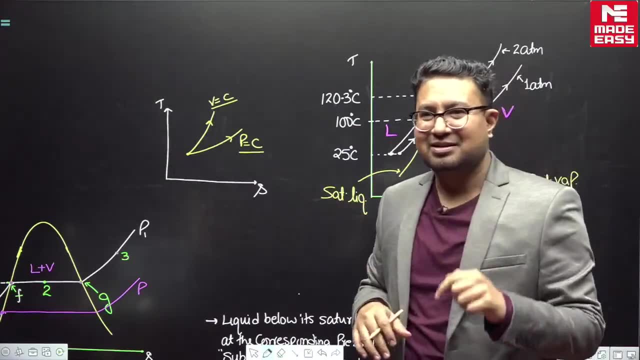 I started writing, but then eventually, and I started doing certain tasks, like I started brushing with left hand. So now everything else stopped, but now also I brush with left hand only. So, anyways, So I am writing this, So I am writing this. 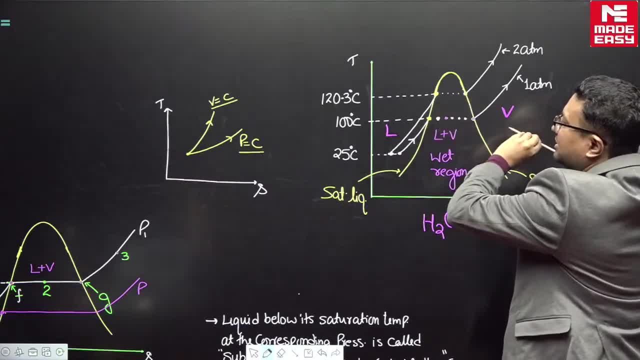 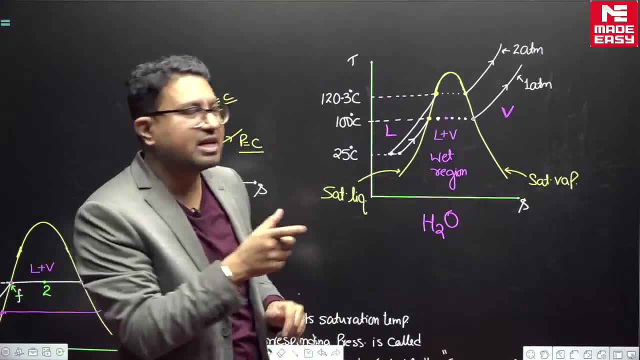 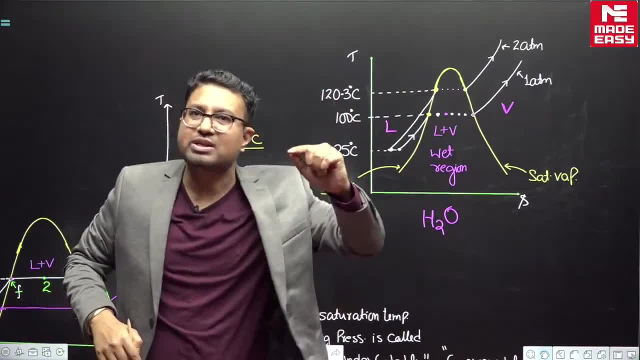 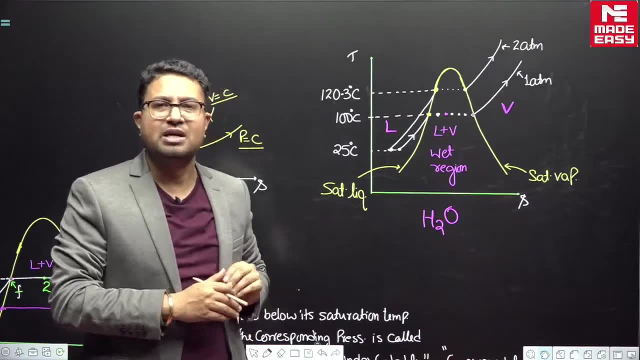 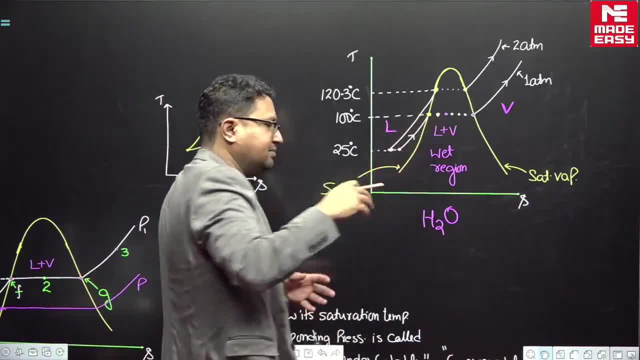 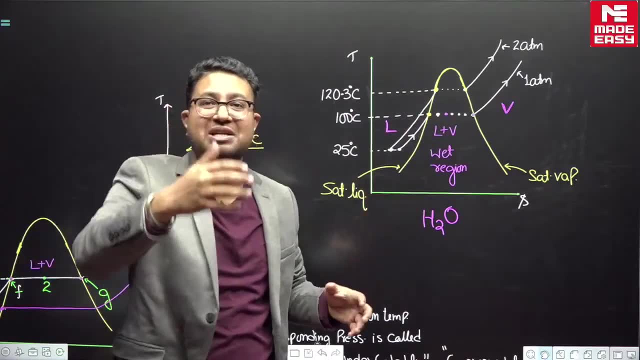 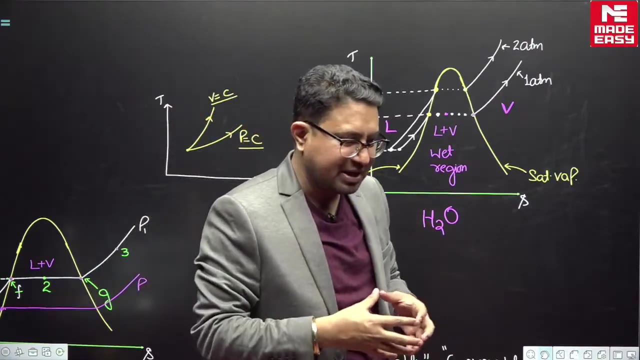 ka ek reason maine aapko pata hai. ae bhi diya gaya hai ki when the pressure is high, jab pressure high hota hai, toh it requires more energy initially, so that the molecule can move away from each other. India mein aisa hota na ki when the people are married. 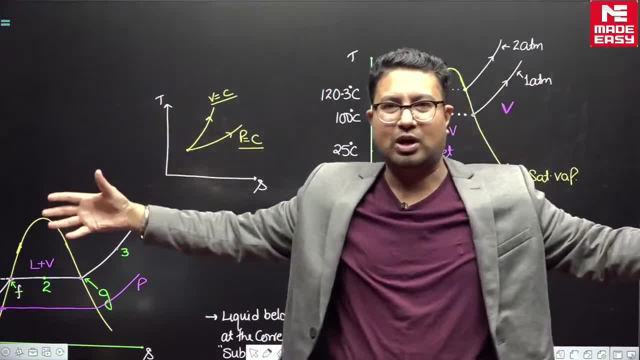 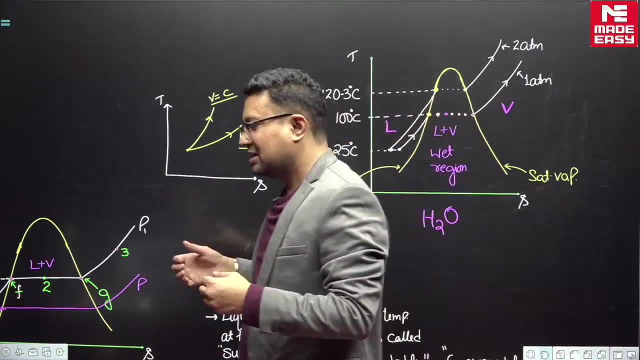 jab logon ki shadi karte. toh lot of people are called baho sare logon ko bulaya jata. why so that? and that is the reason: in India the separation is not that much because lot of people get involved, so there is a huge family pressure. so even if they are colliding, 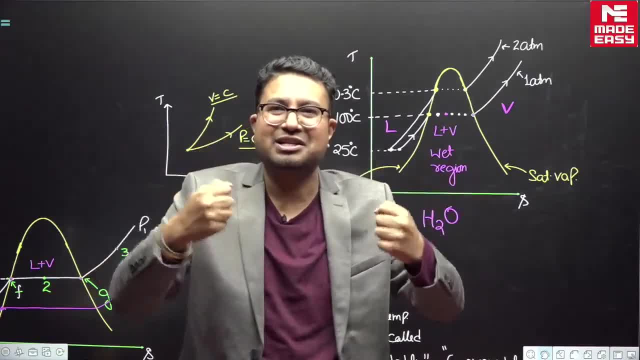 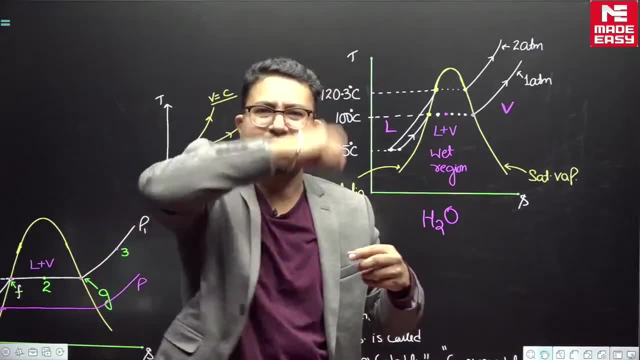 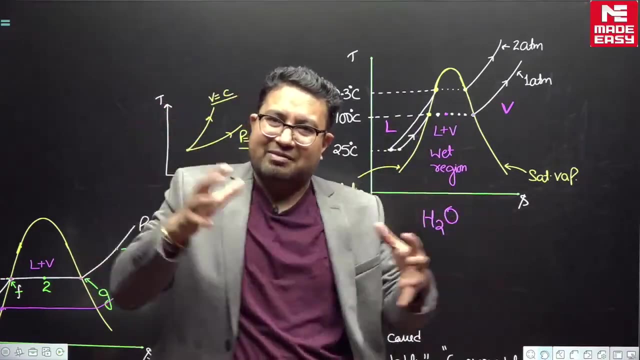 colliding temperature. temperature agar badh gaya. even the relationship gets very colliding. there is high temperature, more collisions are happening because when you increase the temperature the movement of the molecule increases. jo molecule ka bhagna hai na the movement. it increases. so when the pressure is high, when the pressure 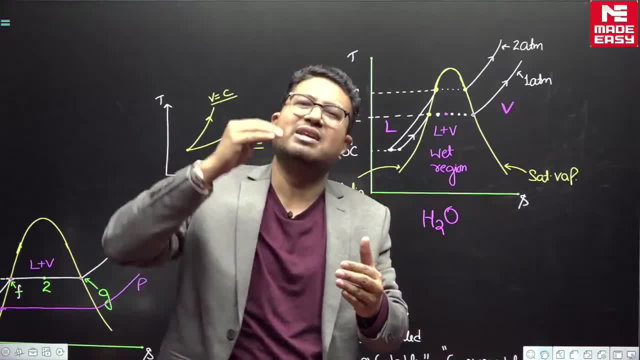 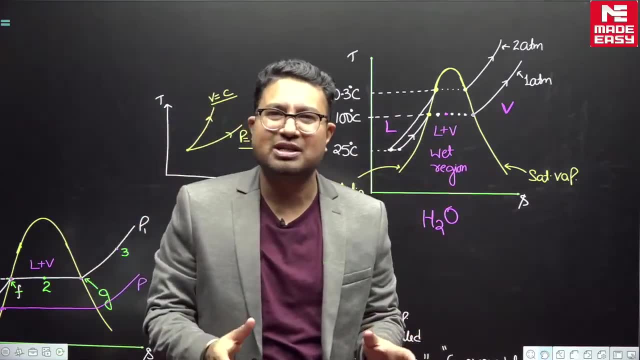 is high. so when the pressure is high, society ka pressure, family ka pressure high hai, toh you require a very high collision to separate separation ke liye collisions jyada chahi hongi. otherwise if the society pressure is not there, society ka pressure nahi hai. bhai, we call thousand people five. 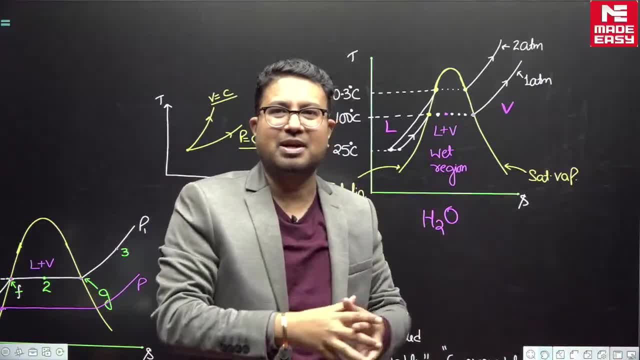 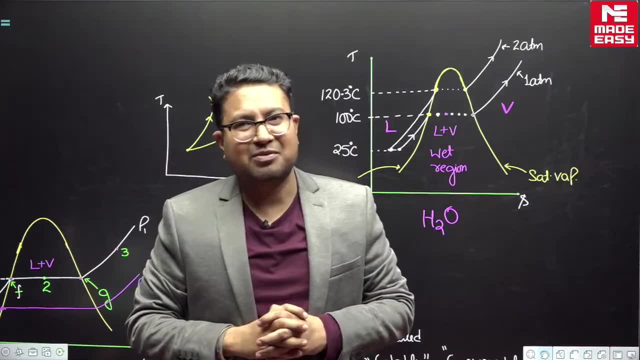 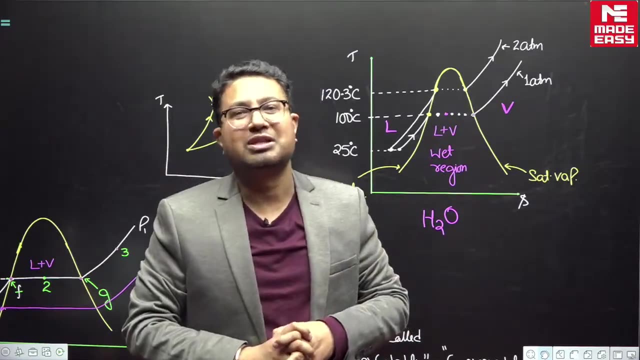 hundred people and we show them that see, these people are getting married. so back of the mind somewhere. it is ki if they get back from their decision, if they step back from their decision, then you are here. aap log yahan ho or aap in ko yad di lana ye baat. there is lot of pressure that gets created right. so the higher temperature. 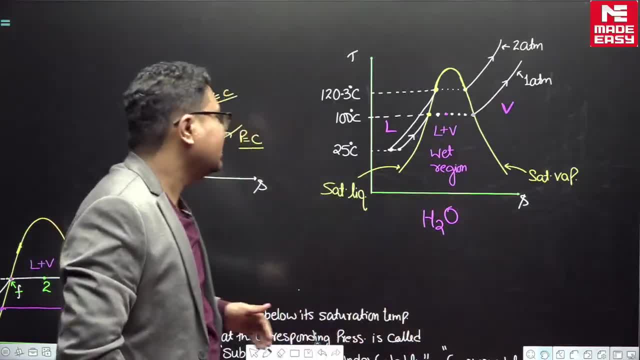 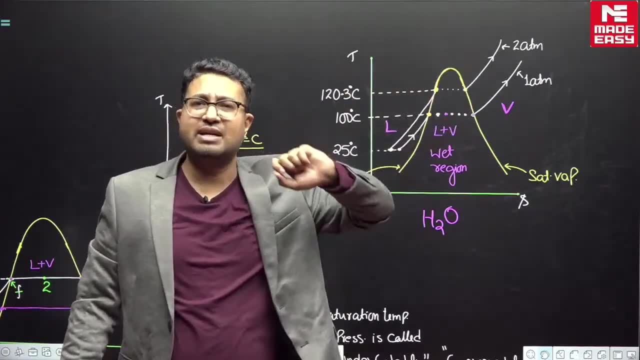 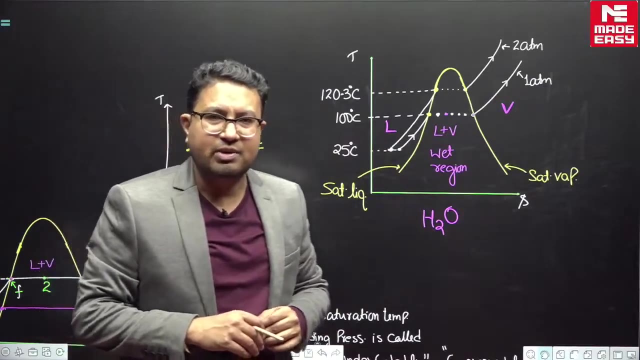 is the required for the separation and for the latent heat reducing. one reason is given that because at higher pressure phase change starts at very, very high temperature, phase change ka hi high temperature bhi start hota to. already there is a lot of energy that has gone into the liquid already bohut saari energy hai toh the energy required for that phase. 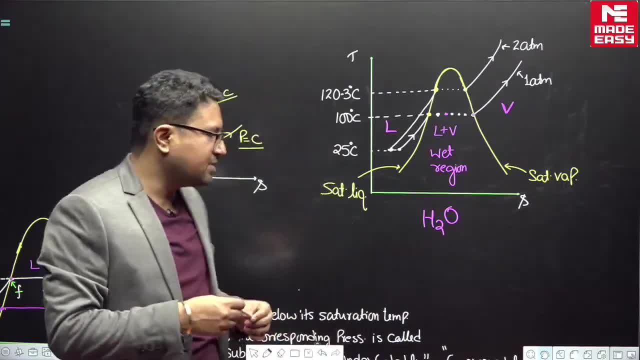 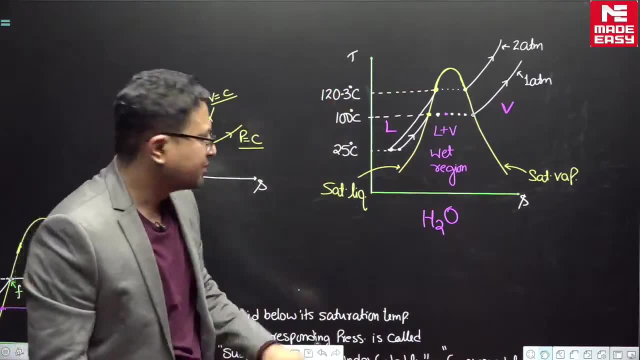 change reduces phase change, ki energy reduce ke jaati. so this is the behavior which we observe, that as the pressure increases, saturation, temperature increases but the latent heat reduces, latent heat reduces. So we can see here. we can see here, here I have written. 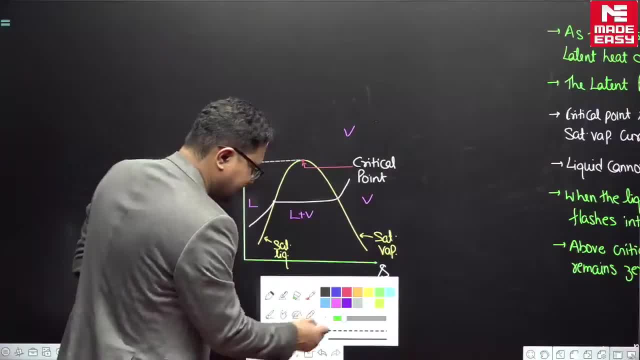 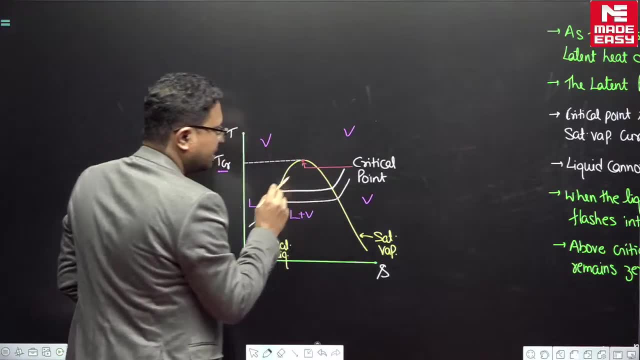 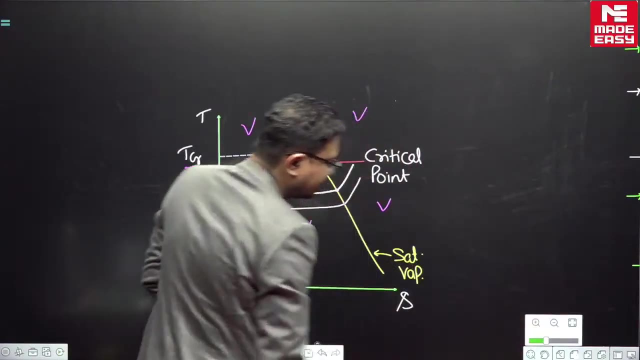 I have written this and I have also drawn here. So we can see that as the pressure increases, as the pressure increases, the saturation temperature increases but the latent heat reduces. latent heat reduces. I have written here: as the pressure increases. 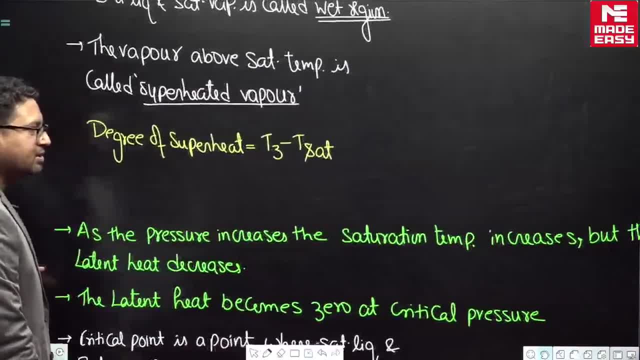 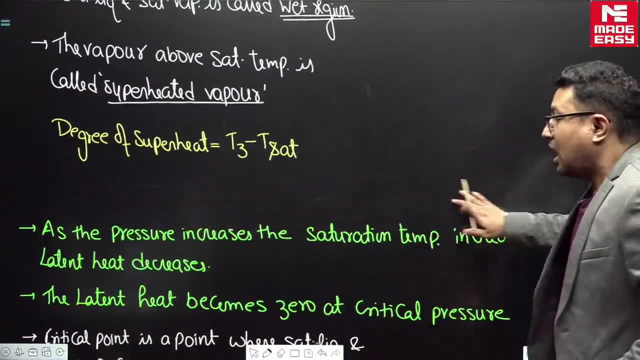 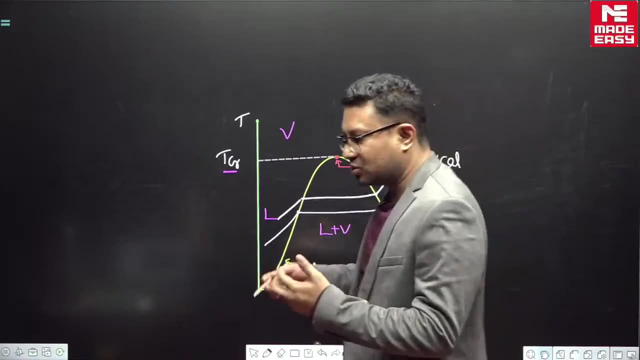 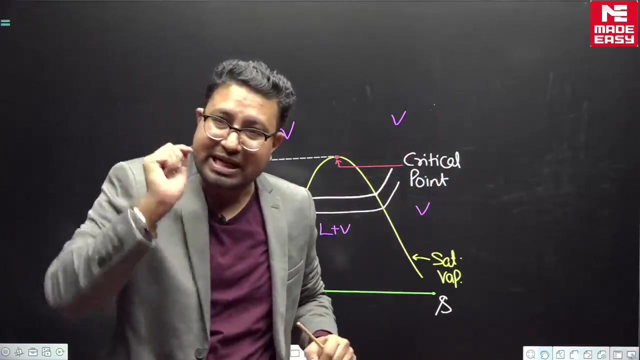 the saturation temperature increases, but the latent heat decreases, but the latent heat reduces. now latent heat becomes 0, there will be a pressure at which you are heating. there will be some pressure at which, when you are heating, the latent heat is 0,. 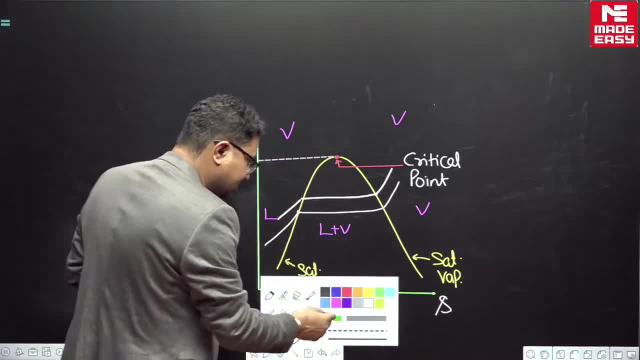 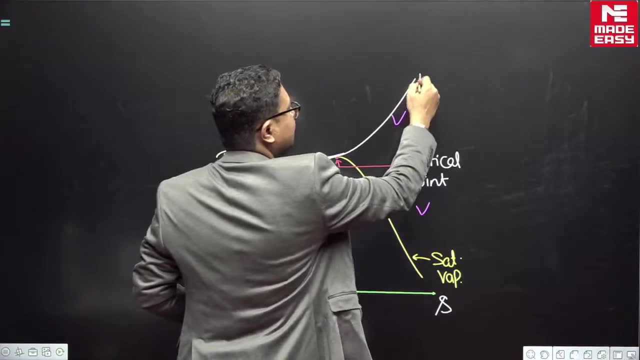 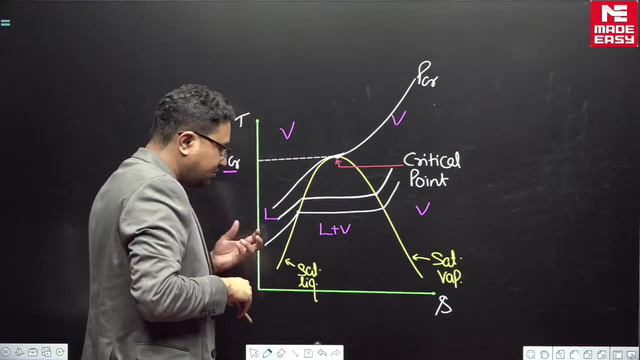 latent heat is 0,. so when the substance reaches its critical pressure, when the substance is at its critical pressure condition, critical pressure means the pressure at critical point, pressure which is at critical point when the substance pressure is so high when the 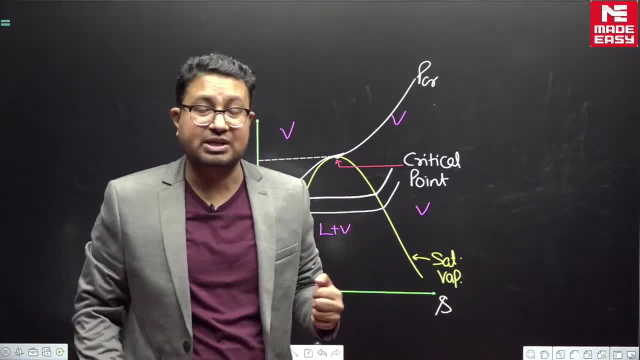 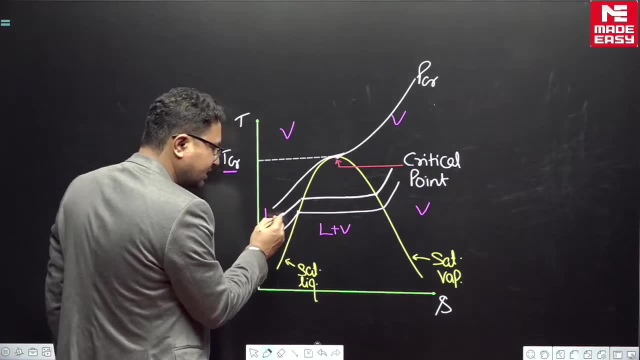 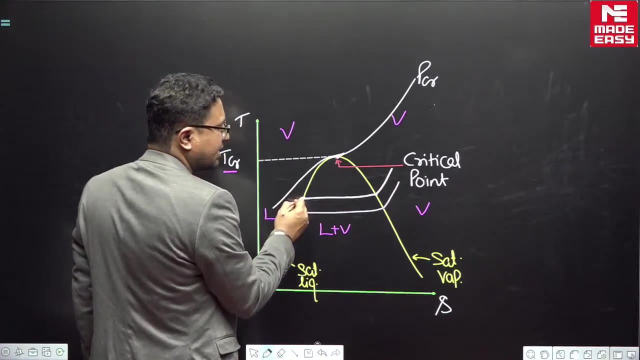 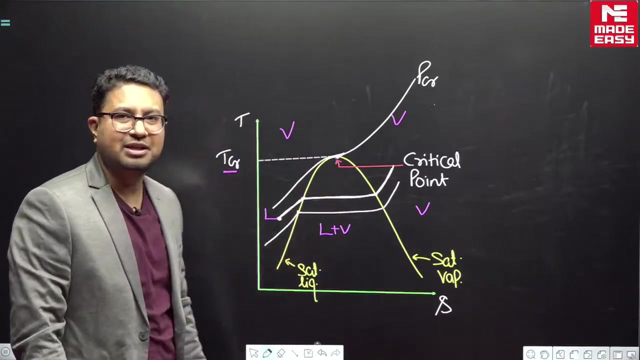 substance is corresponding to its critical pressure condition. so, before this, whenever, whatever pressure you were before this, whatever pressure you were when we were heating, when we were heating, and then the phase change starts. phase change starts, then phase change happens, and then the temperature again increases, then temperature increases, then temperature. 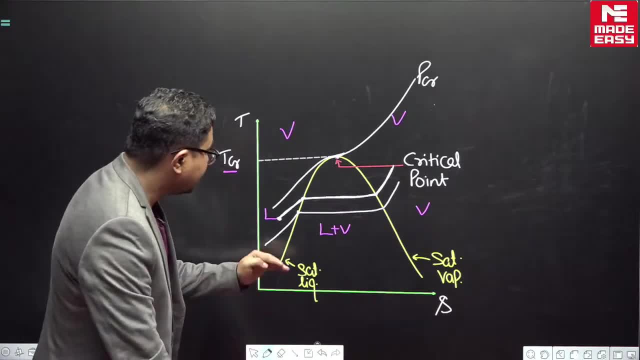 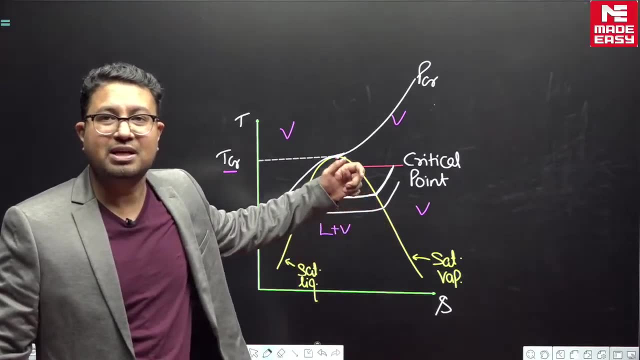 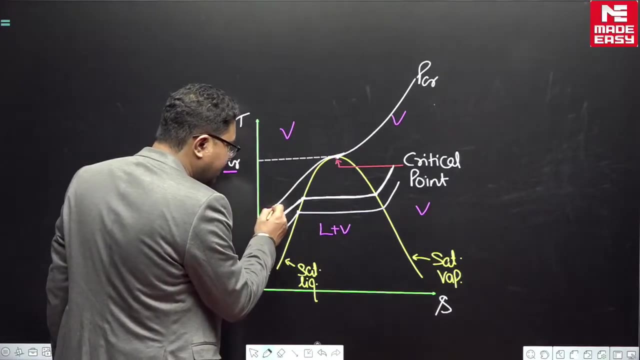 again increases Now if the pressure is 0.. increases if you increase the pressure, like you have reached critical pressure. So now suppose, if we have increased our pressure and we are at the critical pressure condition, if we are at the condition of critical pressure, then now, if we heat, if we heat, heat, heat. 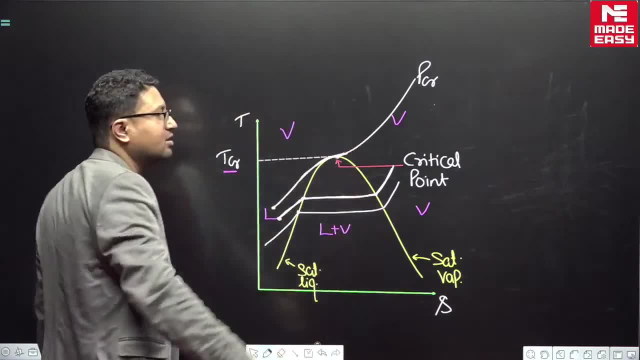 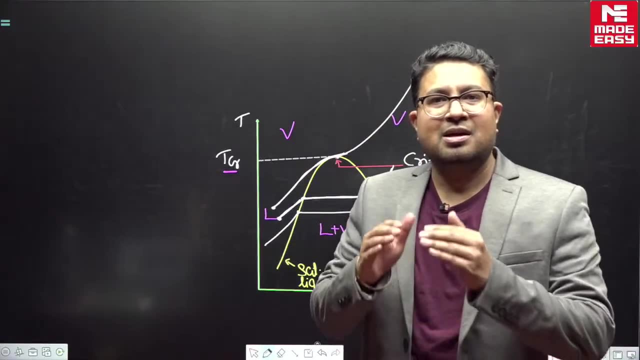 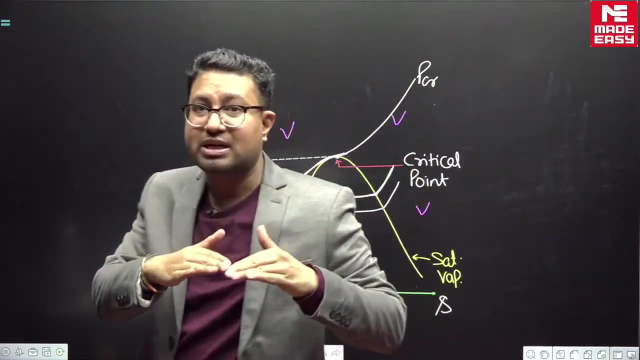 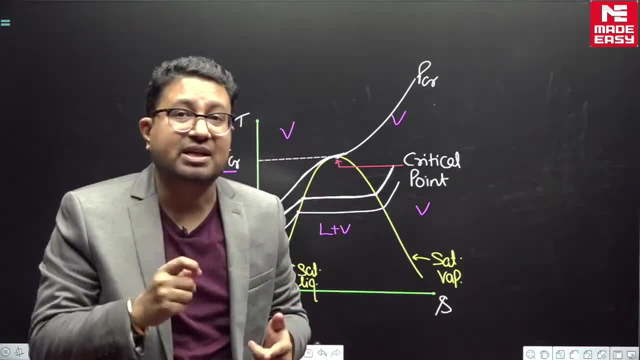 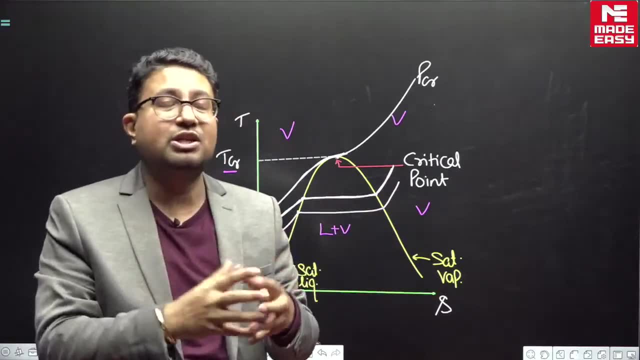 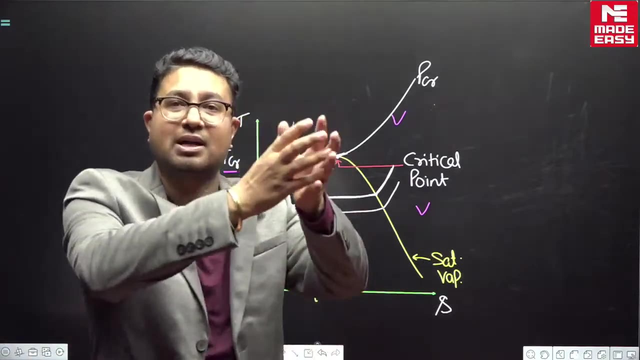 heat reduces. Latent heat becomes zero at critical pressure. I mean critical pressure is such a pressure when you heat it, then the liquid has to change into vapor. Zero energy is required. Like the liquid was giving energy, the temperature was continuously increasing. That continuity is maintained. This discontinuity does not. 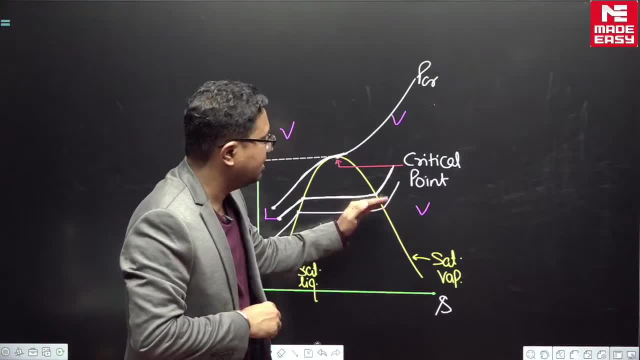 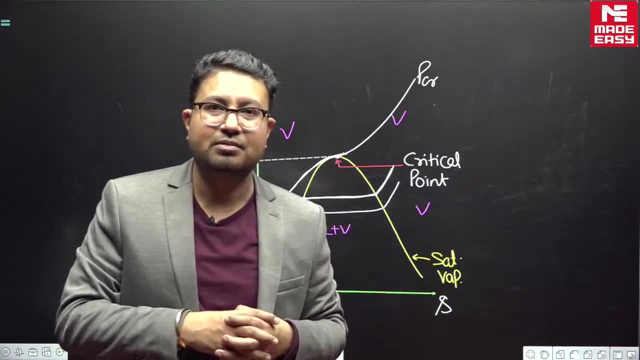 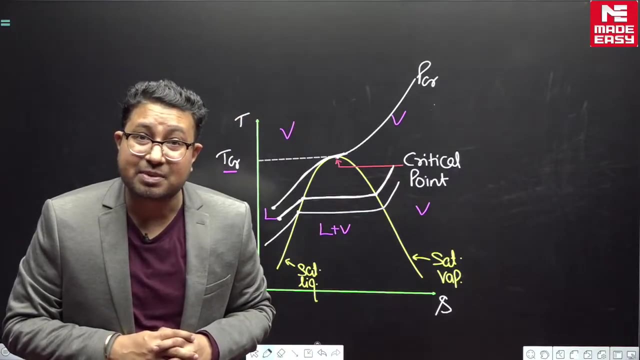 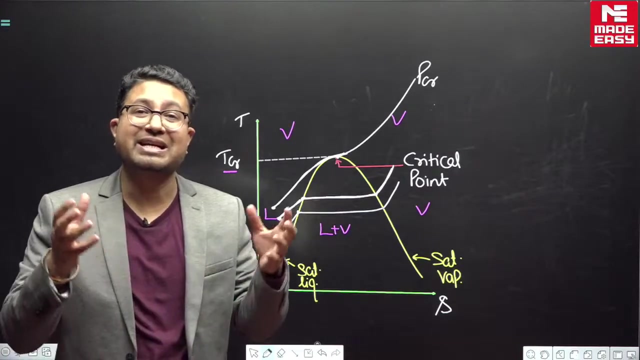 come that the temperature increases, then it is stable, then it increases. This discontinuity does not increases, does not encounter, you do not get, because the latent heat has become zero, Latent heat has become zero. Now see why it takes time for. 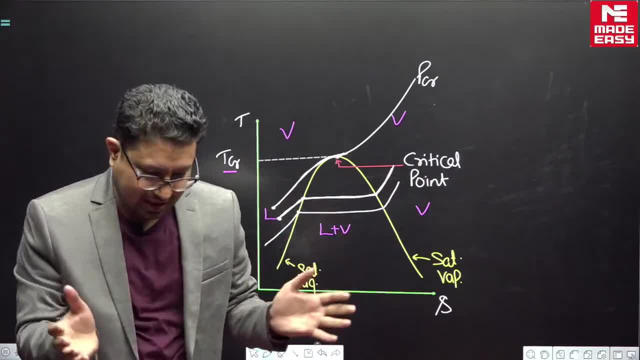 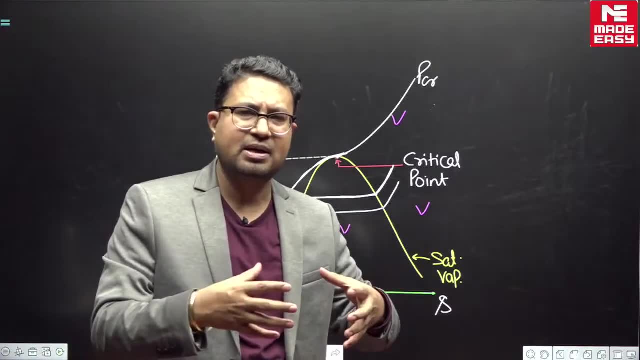 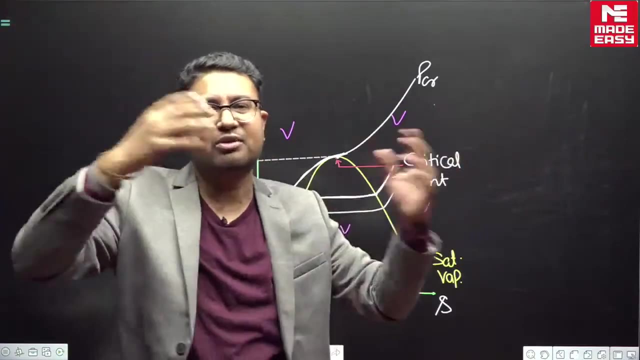 the water to boil. I have explained in the beginning. If you take water in a pan, if you take water in a vessel and if you start heating, you start heating. So it will take a lot of time for the entire liquid to change into vapor. It will take a 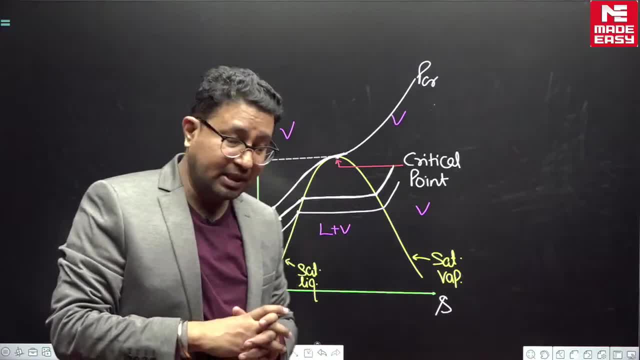 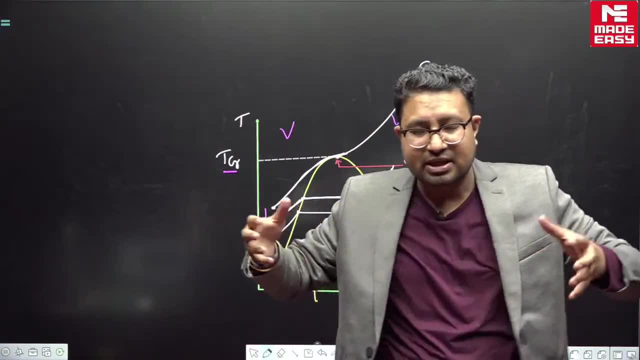 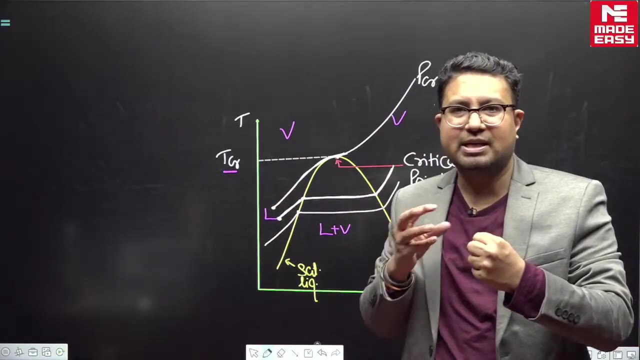 lot of time. it will take a lot of time, But but as you continue supplying heat, as you keep on supplying heat, there is significant value of latent heat. Latent heat has a lot of value. So whatever energy enters, whatever energy enters, absorbing that energy does not cause. 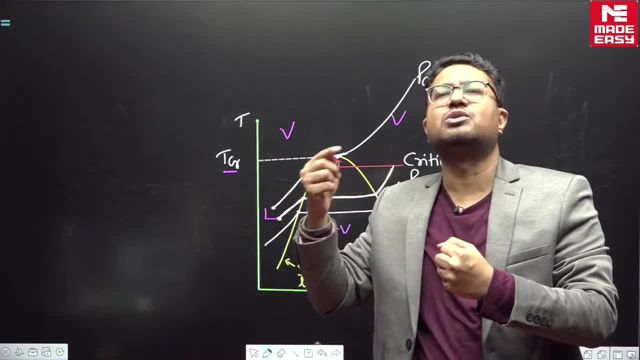 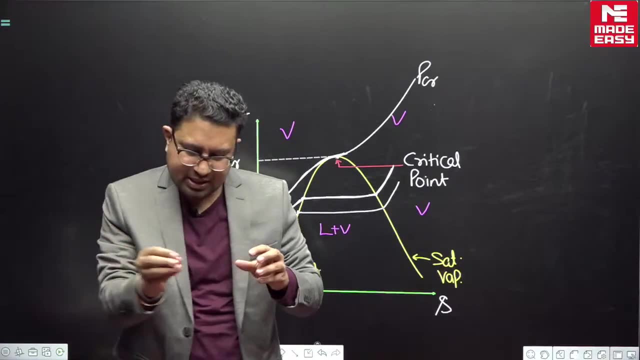 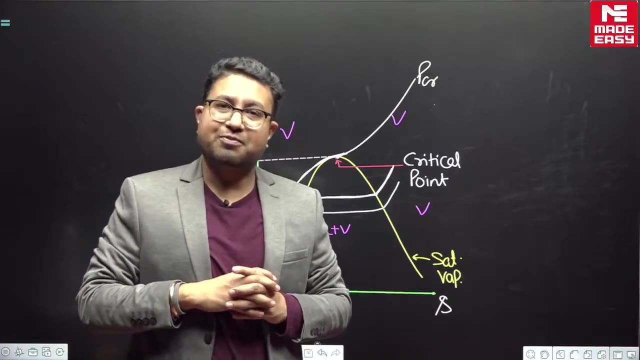 that energy, absorbing that energy, Some of the liquid changes into vapor, some liquid changes into vapor, remaining waits. then some more energy enters, some more liquid changes into vapor, remaining waits, remaining liquid waits. So if this happens, if it continues continuously, if this happens, 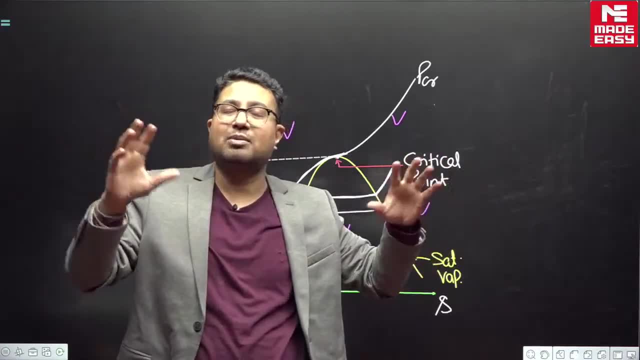 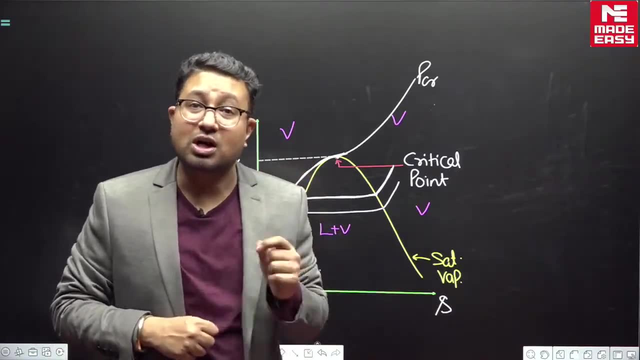 So after some time you will see the entire liquid has changed into vapor. entire liquid changed into vapor. but time kyo laga. why the time was taken? time kyo laga because because, why the time was required? because latent heat has the significant value. bahut saari value thi latent heat ki. 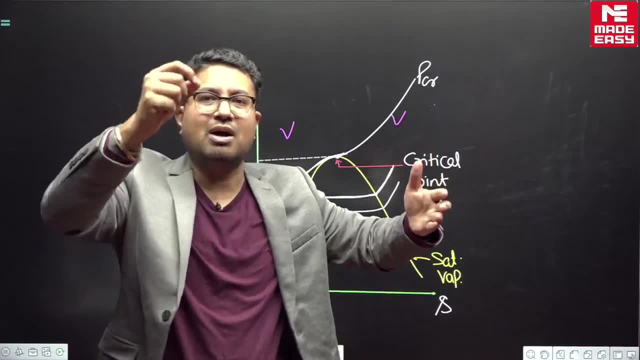 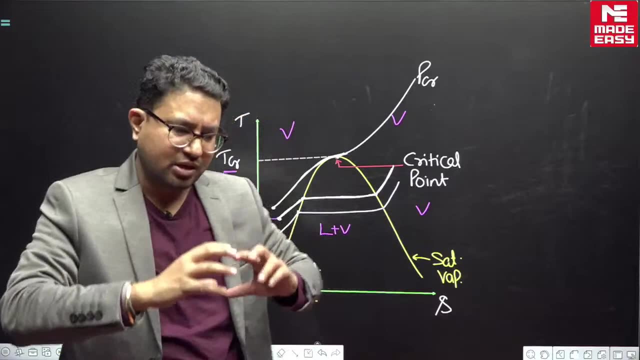 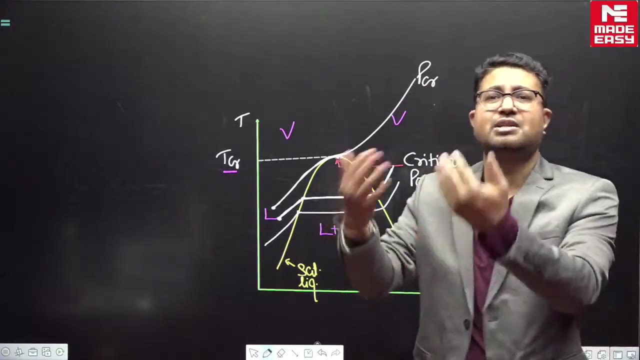 to each gram required energy to change phase from liquid to vapor. har gram ko energy ki zeerat padhi to jis rate se energy aari thi corresponding to that. whatever mass can change from liquid to vapor, jo bhi mass liquid se vapor change ho sakta, tha that changed remaining. 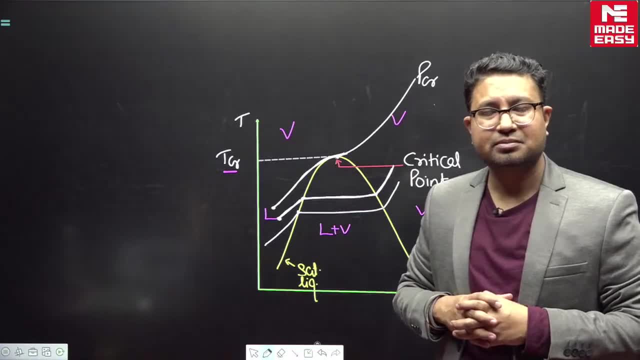 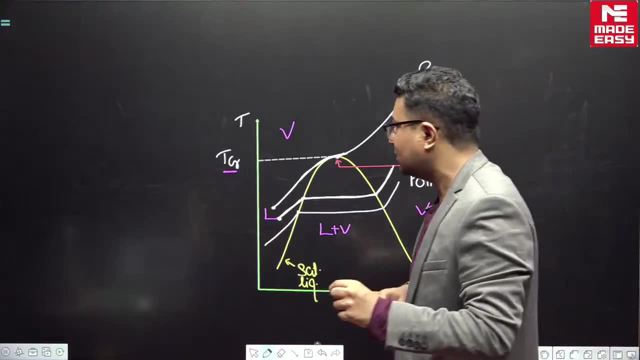 ne wait kiya. remaining waited when you are heating the liquid at critical pressure. jab aap critical pressure pe heat karte ho, latent heat zero hai to waiting time hi nahi hai. there is no waiting time. you are liquid, you are liquid. you are liquid. suddenly you get. 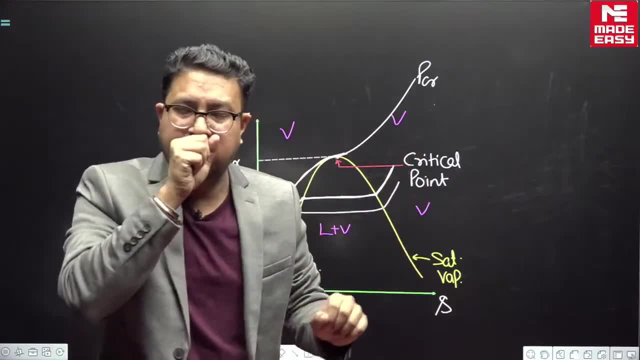 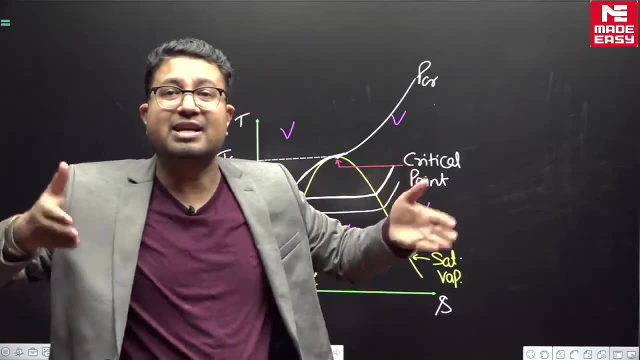 converted into vapor. suddenly aap vapor me convert hoga hai koi time nahi laga whether you are 1 kg or 10 kg or 20 kg 1 kg liquid hai 20 kg liquid hai 30 kg liquid. hai time to tab lagayega na when there is latent heat. so per kg, this is the time kyo laga kya, kya. 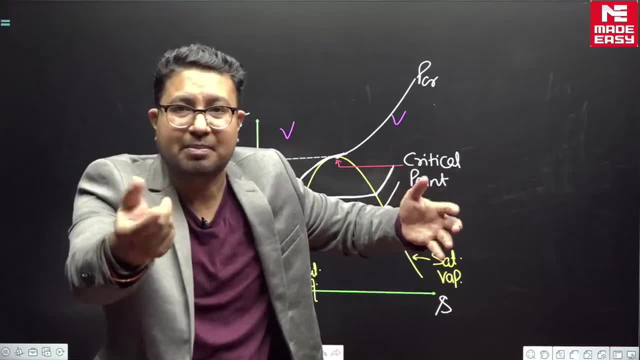 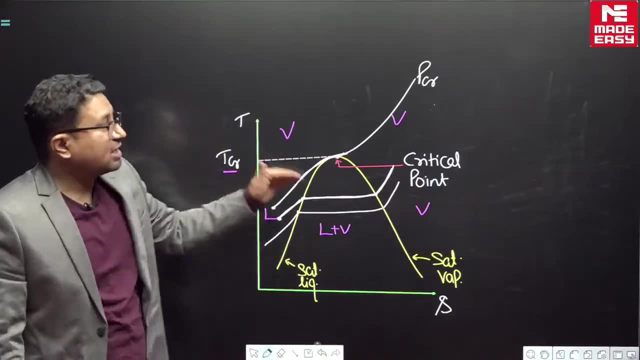 kya sabla hai aapko latent heat kar sakta hai. this is the requirement, and you are supplying this energy per second. abhi itni energy per second supply kar rahe ho, so remaining will have to wait. koi waiting time nahi hai. at critical pressure the latent heat become. 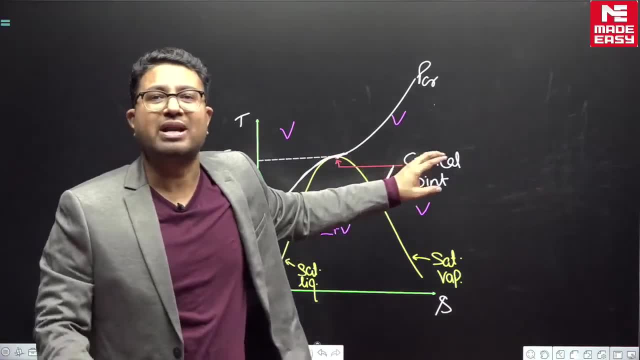 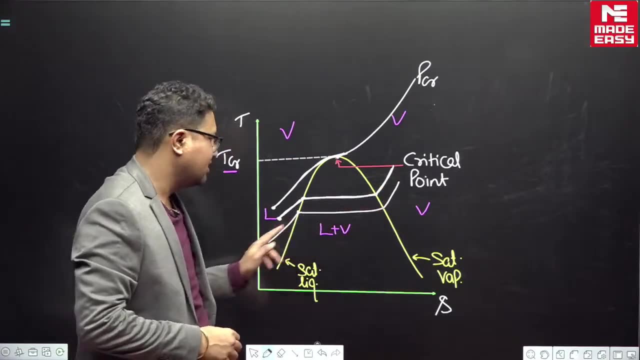 zero. latent heat, zero. ho jati koi luk kyahta hai critical point pe zero? kya hai critical point to beech me pada? when you are heating at this pressure, you encountered latent heat. when you started heating at this pressure, you encountered latent heat, aapko latent heat. 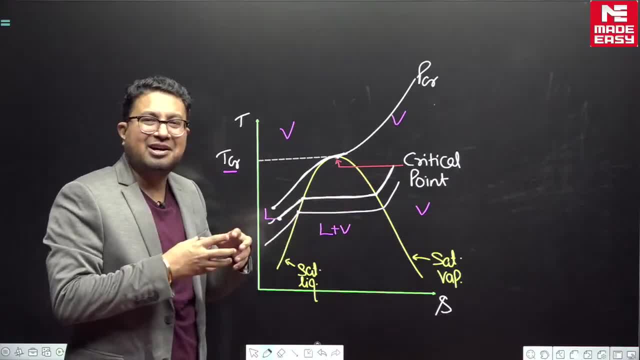 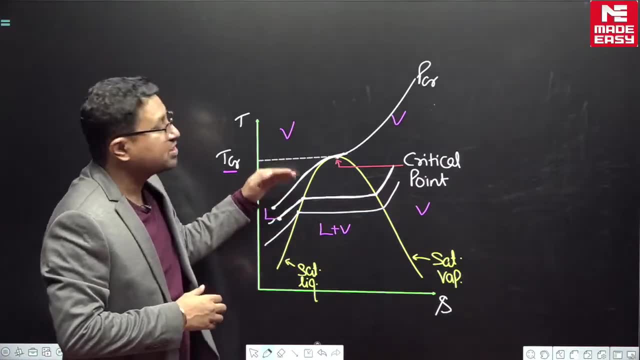 ka saamna karna mein lau. latent heat: are you are done with latent heat after you are Robert R participate now encounter. you witnessed the latent heat. there was some energy required for the phase chain but just as a higher pressure, we heat when you reach the critical pressure. 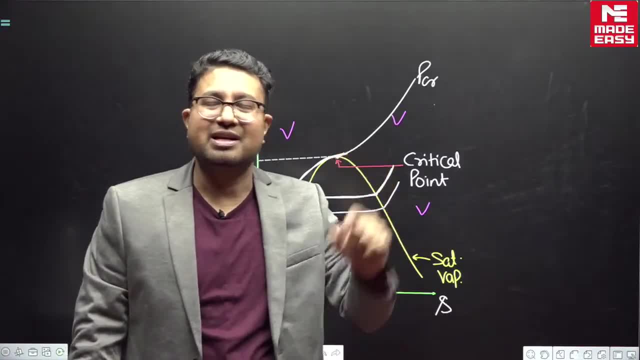 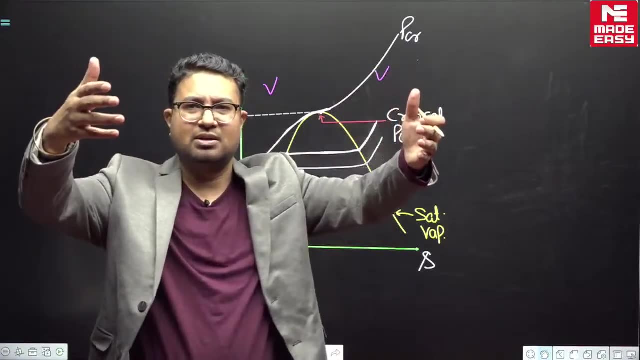 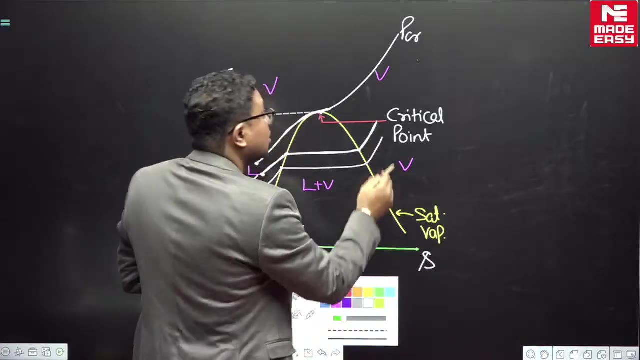 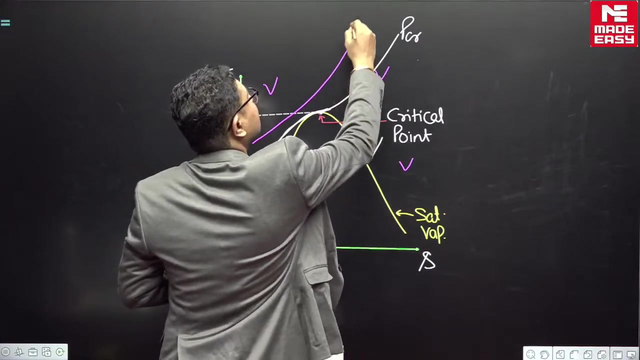 when you reach the critical pressure, the latent heat will be zero- let me take zero- and the liquid flashes directly into vapor. flashes into vapor suddenly, no time is required. that is flashing above critical pressures. also critical pressure. above critical pressures also the p greater than p critical. above critical pressures, also critical pressure. 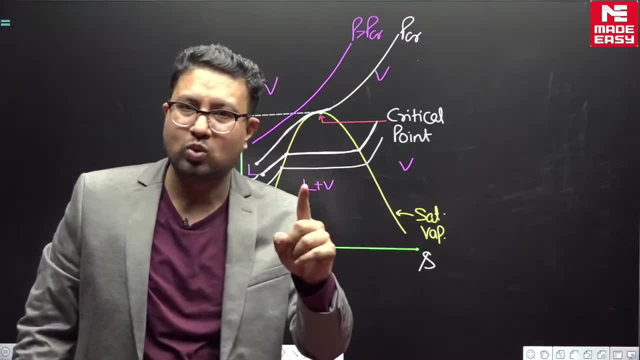 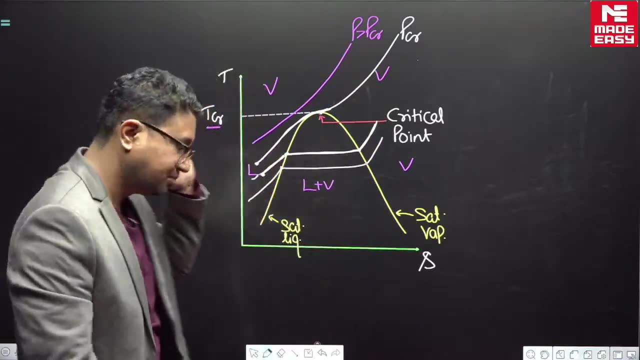 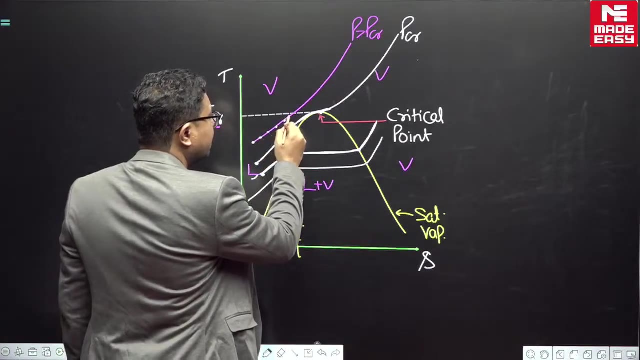 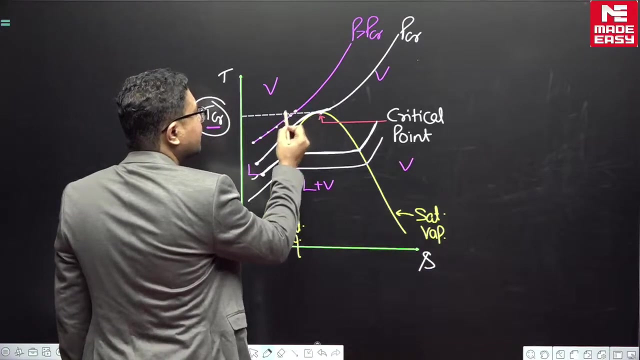 latent heat remains zero. flashing continues, flashing continues. see, suppose you are heating at this condition. you are liquid. liquid here, here, here, above critical pressure. As soon as you cross the critical temperature, as you cross the critical temperature, you will become vapor. As you cross the critical temperature, you will become vapor. 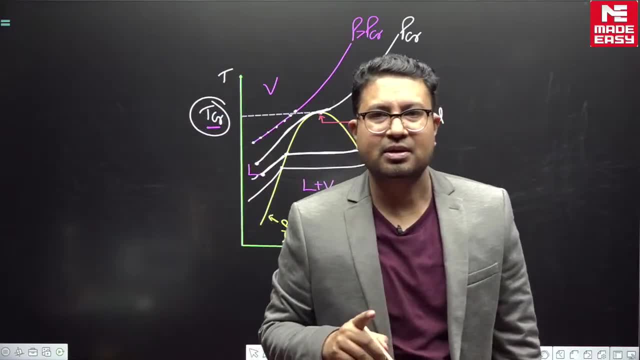 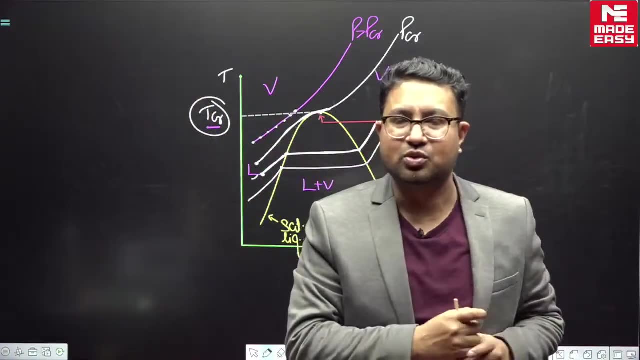 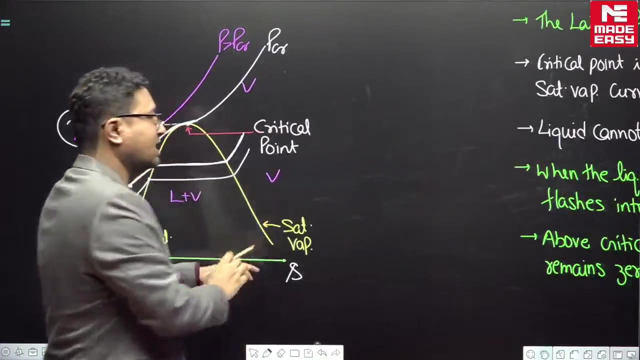 So, above critical pressure also, latent heat remains 0. So, once it is 0, it remains 0. And the flashing phenomena continues. The flash phenomena, the sudden conversion phenomena, it continues. So this I have written. 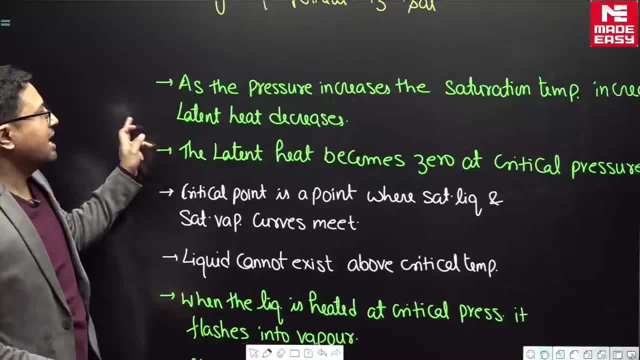 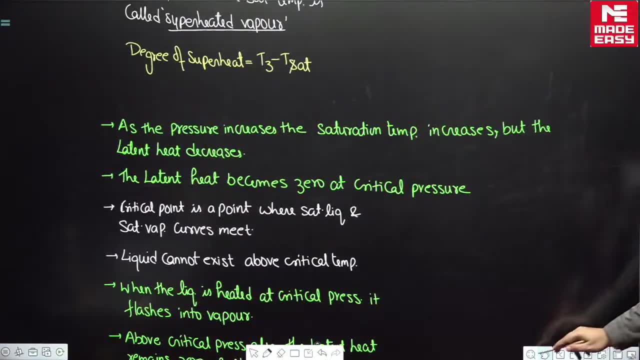 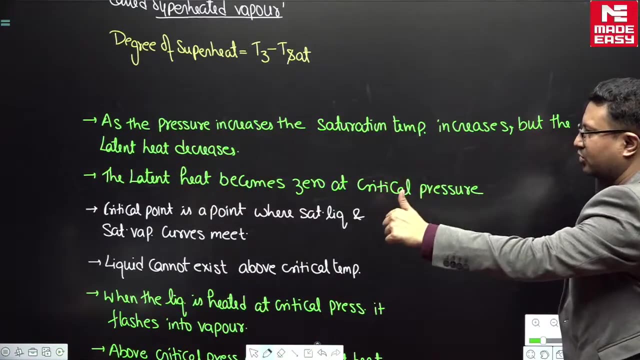 I have written this also. See, As the pressure increases, the saturation temperature increases. I will just slightly minimize it. As the pressure increases, the saturation temperature increases, But the latent heat decreases. Good, The latent heat becomes 0 at critical pressure. 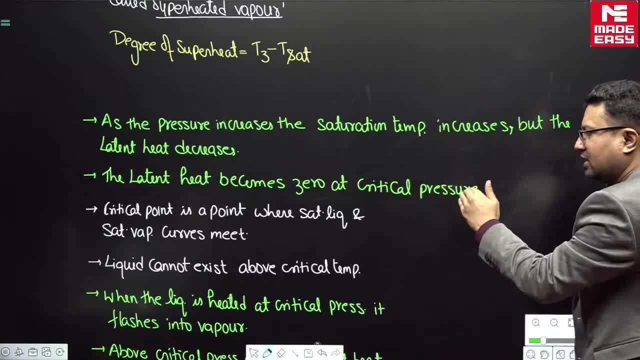 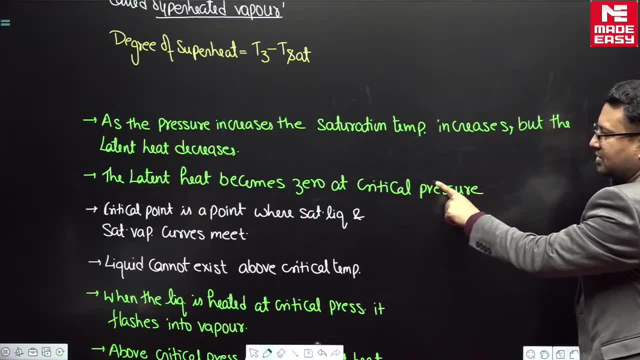 Where did the latent heat become 0 at critical pressure? If you heat it, then the critical point also increases. There is critical point which you pass through, But latent heat will be 0 when you are heating at this pressure. Critical point is a point. 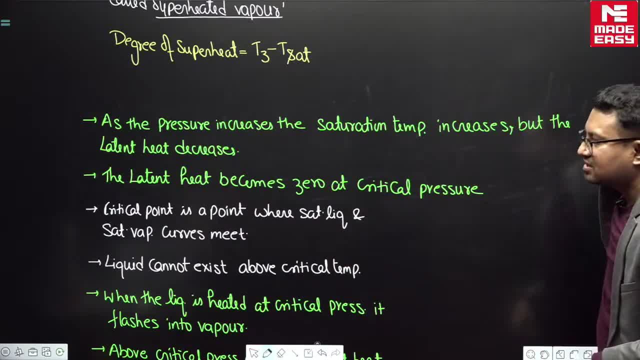 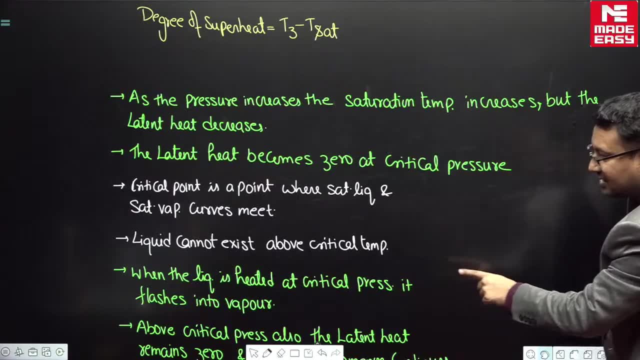 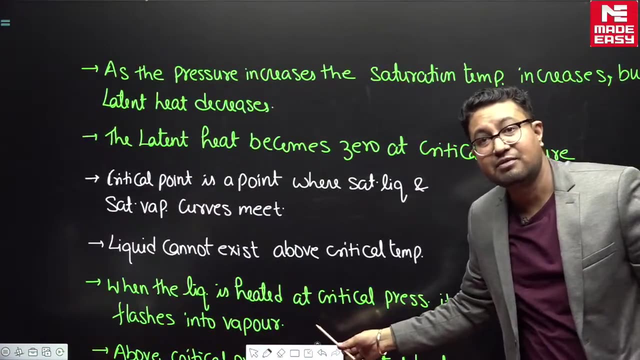 Where saturated liquid and saturated vapor curves meet. I have already discussed Liquid cannot exist above critical temperature, Already discussed, Very good, When the liquid is heated at critical pressure. When the liquid is heated at critical pressure, it flashes into vapor. It flashes into vapor. 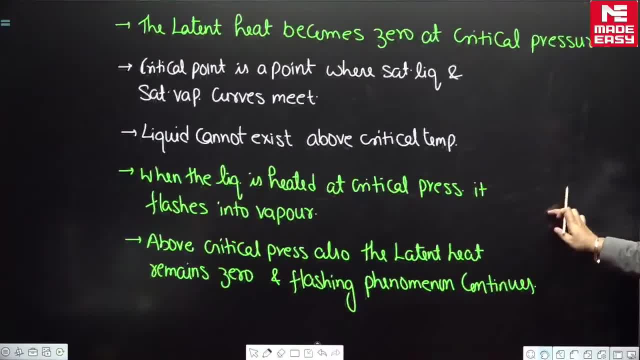 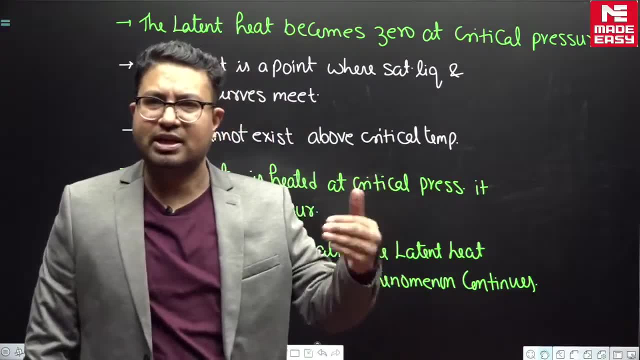 Above critical pressure also. the latent heat remains 0 and the flashing phenomena continues. Above critical pressure also, latent heat remains 0 and the flashing phenomena continues. It continues. So we have discussed one more thing. We will talk about the dryness fraction. 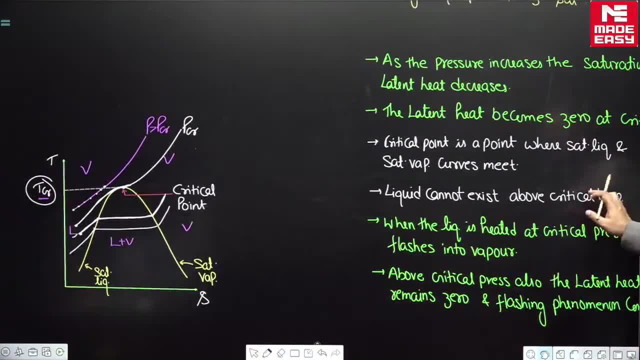 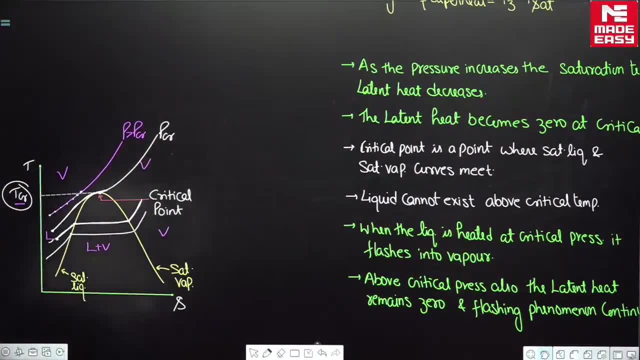 But before that, let me just show you this diagram And I will show you this, These statements also, I will show you this statement also, And we will continue the discussion. Umesh Educator, Guruji, Namaskar, Namaskar. 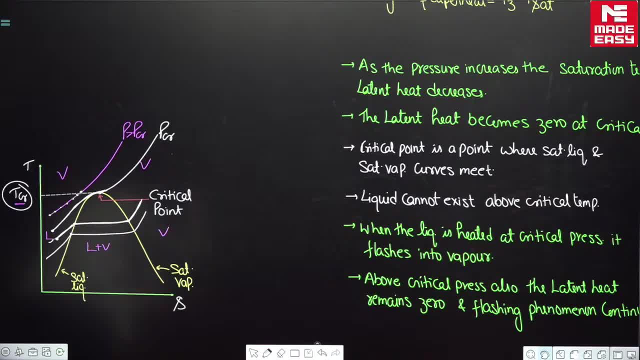 Beg Prajapati. It is always a blessing to see you, sir. That is my pleasure to listen Such words. Wonderful comments, Vapor start. Okay, This is a previous message, Kanisha's. Oh, what an application, sir. 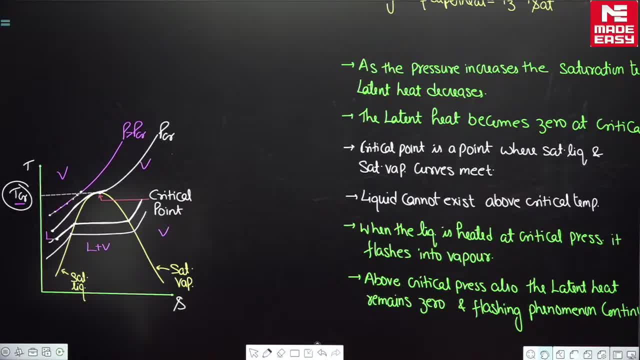 Beauty. Thank you, Nice So. Thank you Wonderful Rajinder. Oh, there are So beautiful messages. Anil Rajendra, Nishanth. Anil Rajendra, Love you, sir. Love you too, Nishanth. 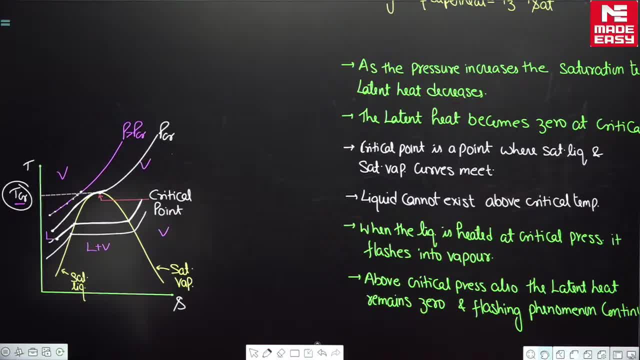 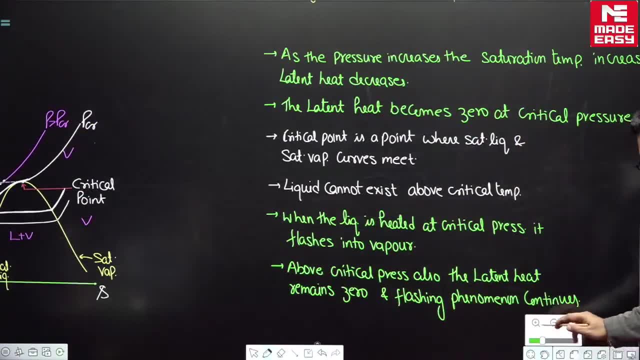 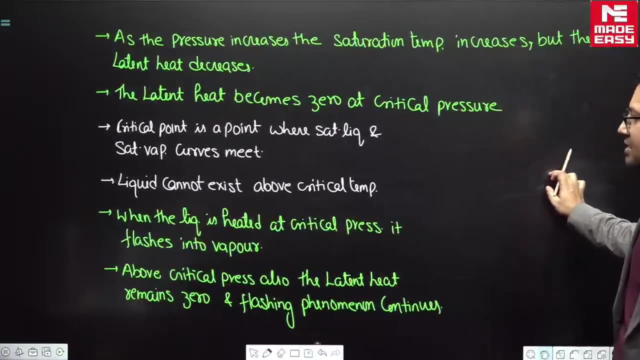 Yes, Yes, So wonderful. See Now, now. now You can just just take this and we will move forward. We will move forward in the discussion. So now see what we discussed. What we discussed, What we discussed. 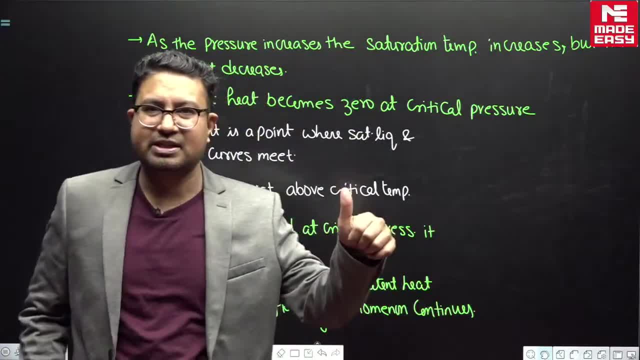 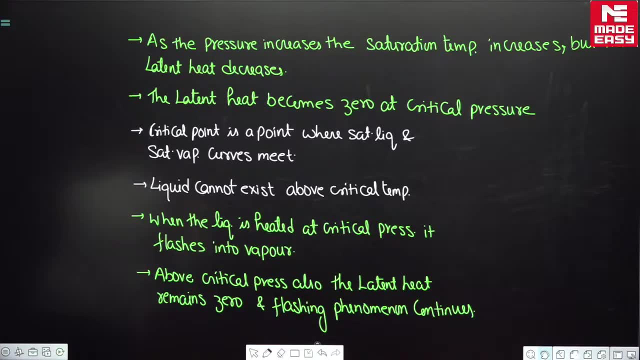 So we discussed, We discussed That first First thing. we discussed about the- I will just move aside, It will be a little sad- So we discussed, we discussed, we discussed about the first thing, that is, how the saturation. 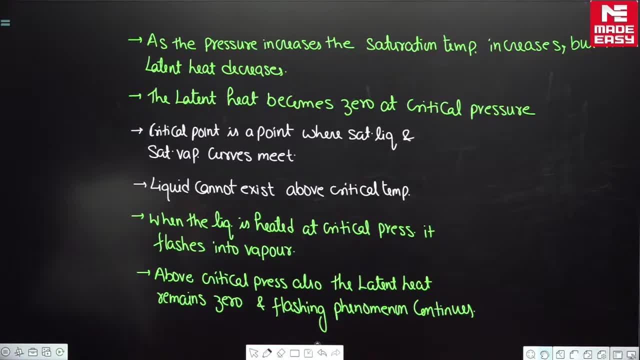 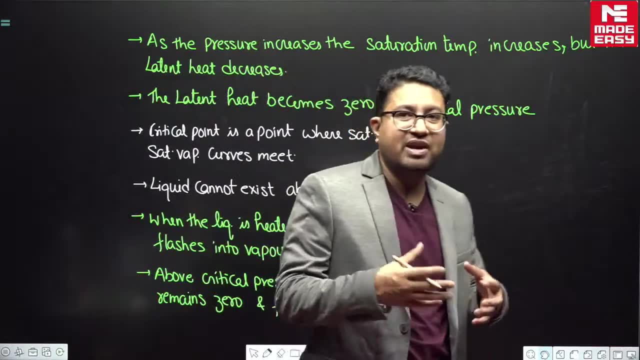 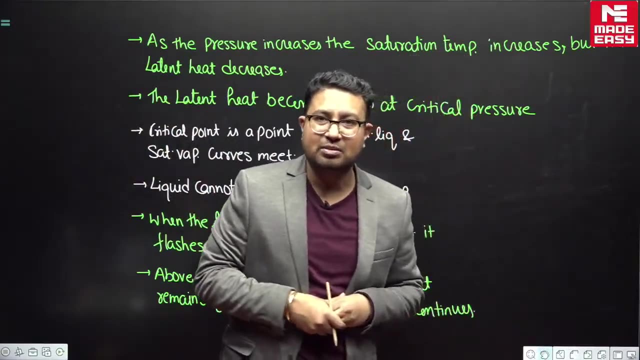 curve is drawn. How do we draw the saturation curve? Second thing: the second thing that we discussed, that we discussed, that we discussed is that how the various regions are various regions: saturated liquid, saturated vapor, and so on. Then we are talking about the critical point. 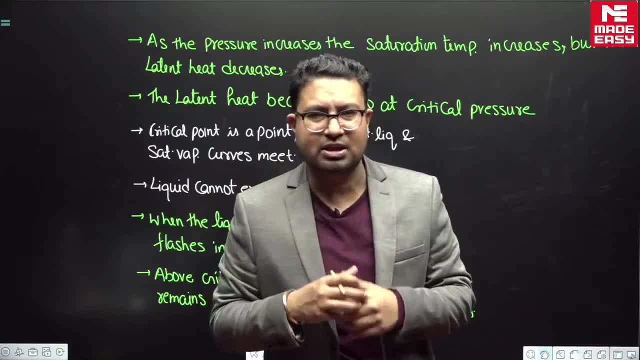 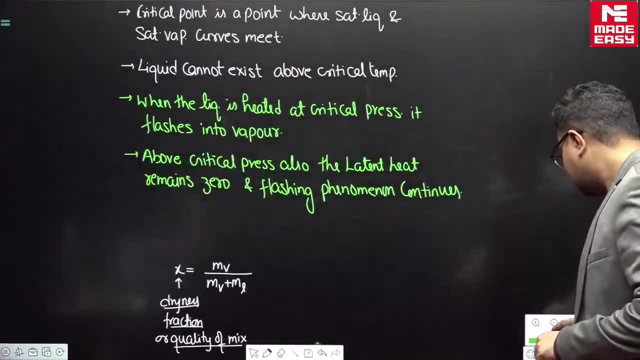 We talked about the critical point. We talked about the critical point. We will talk about more. we will talk more about it, And we understood few things. We understood few things. Now, you see, there is a term called as dryness fraction. 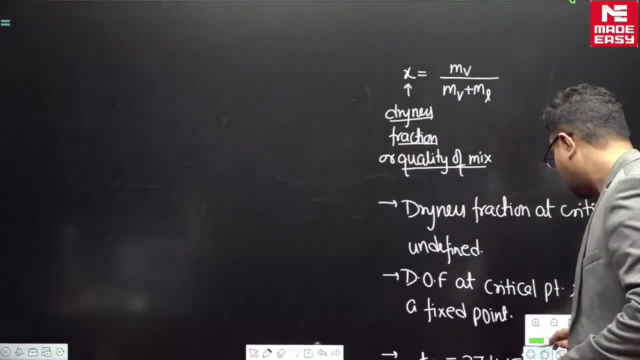 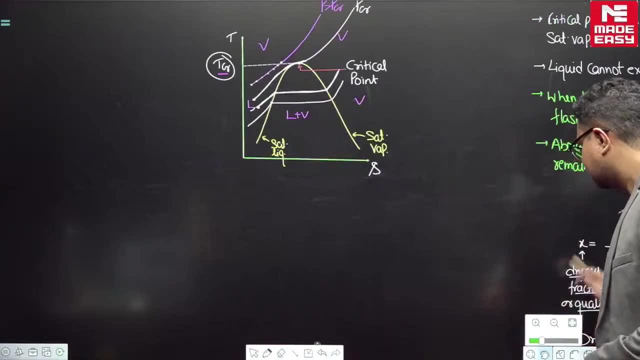 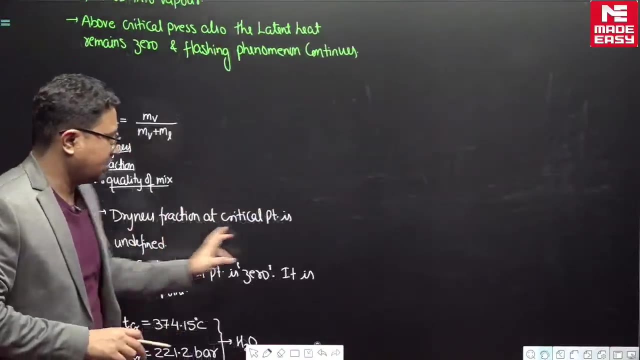 There is a term called as dryness fraction, or we call it as quality of the mixture, We call it as quality of the mixture. So just a second See Now. let us see here. Let us see here We, I will draw a diagram. 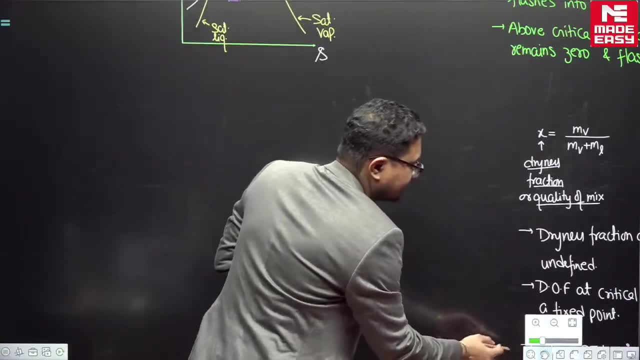 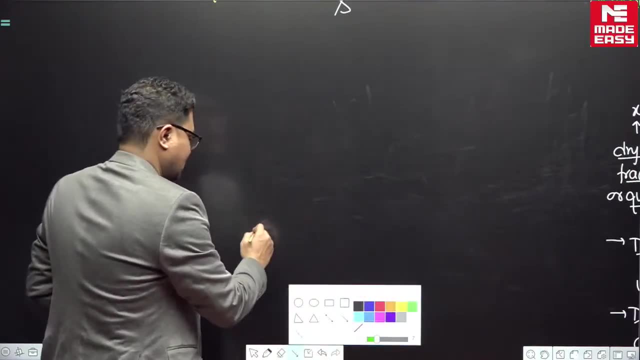 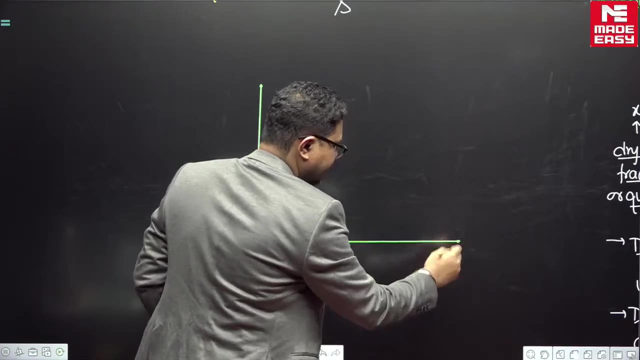 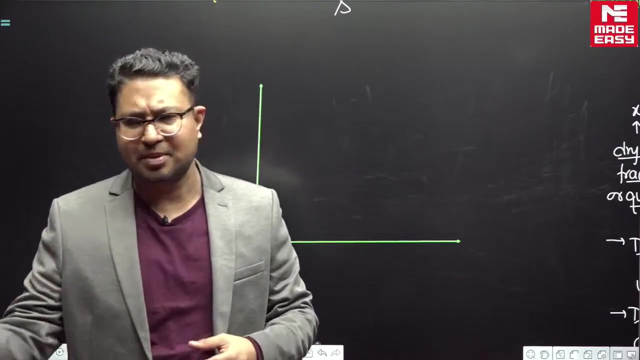 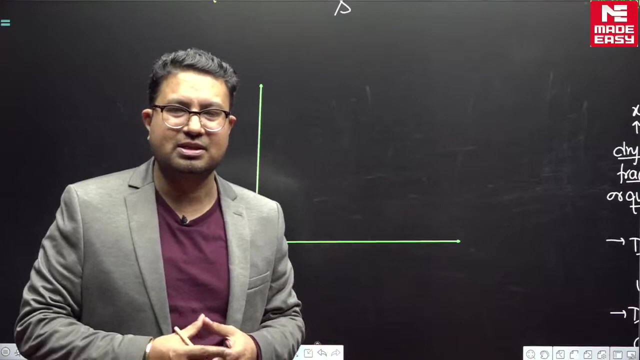 So Here I will draw a diagram. Let us see here. See, So now I hope this discussion is clearing many of your doubts. This discussion will clear many of your doubts And whatever preparation you are doing, there will be many people, obviously from college also, So whatever exams you are studying for this. properties of pure substance. 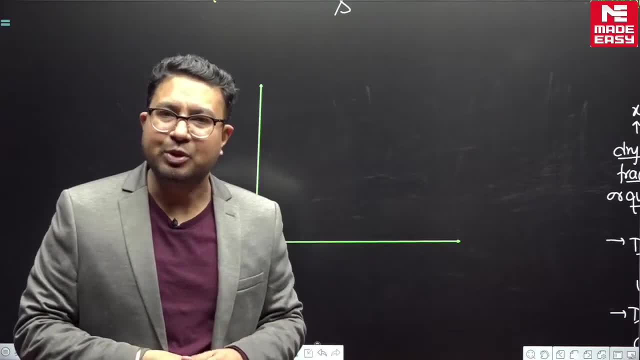 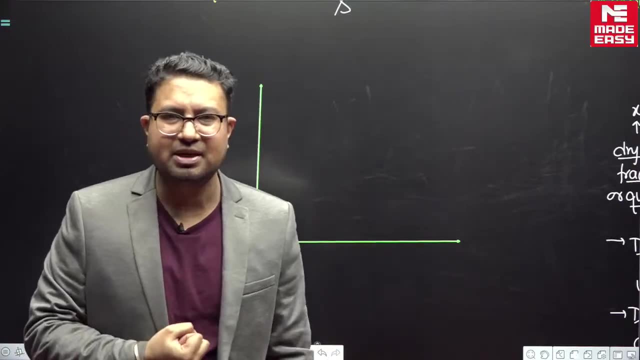 So this discussion will help you to understand the depth. See, we know the formulas, We solve questions, But when we have the depth in our understanding, So this discussion will help you to understand the depth. See, we know the formulas, We solve questions, But when we have the depth in our understanding? 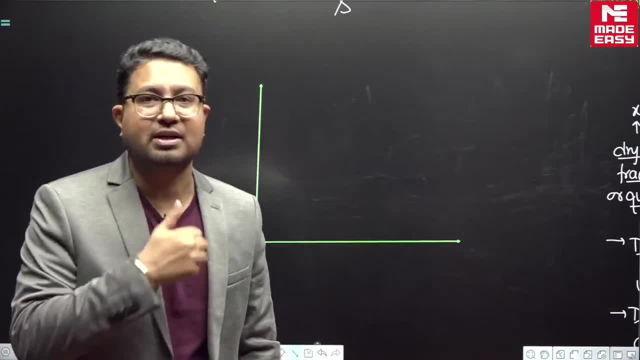 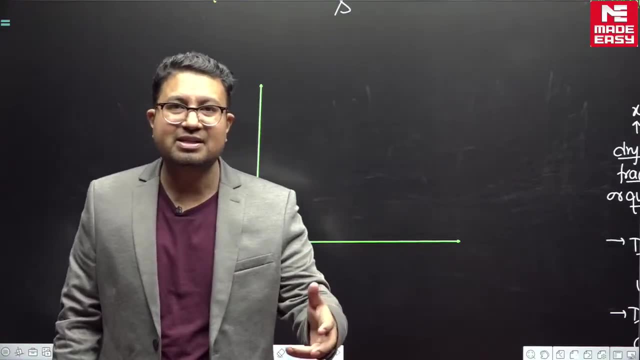 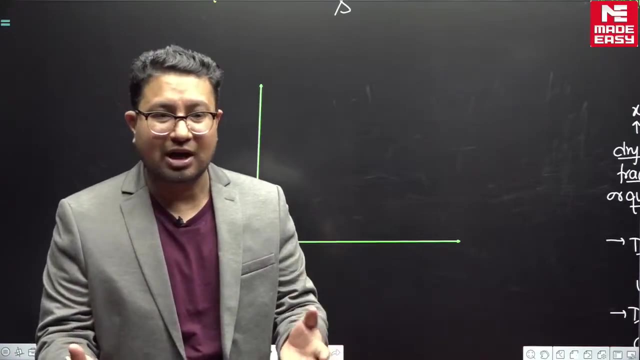 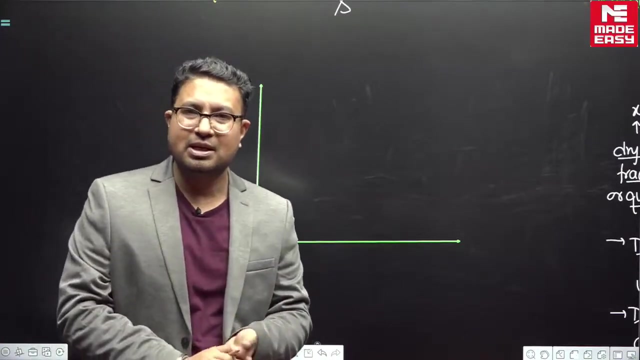 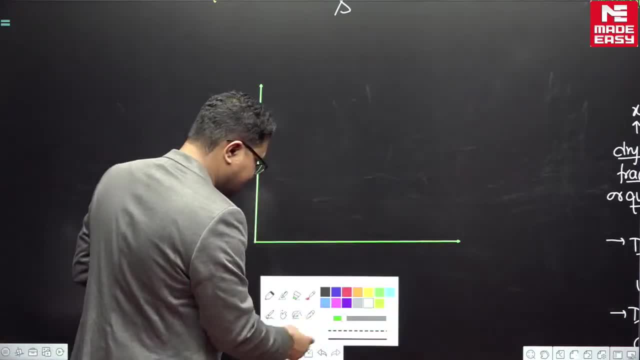 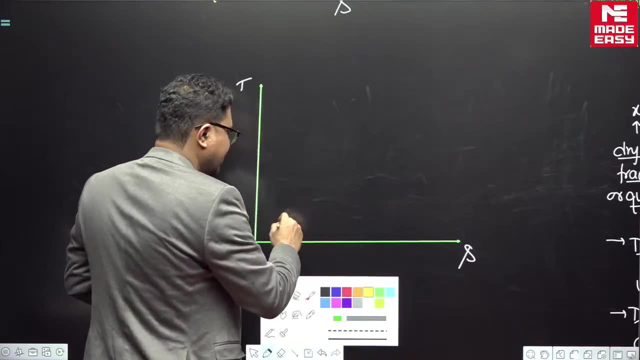 So this discussion will help you to understand the depth. See, we know the formulas, We solve questions, But when we have the depth in our understanding. So now, if we see this T-S diagram here- T-S diagram I am drawing again- So now we have. 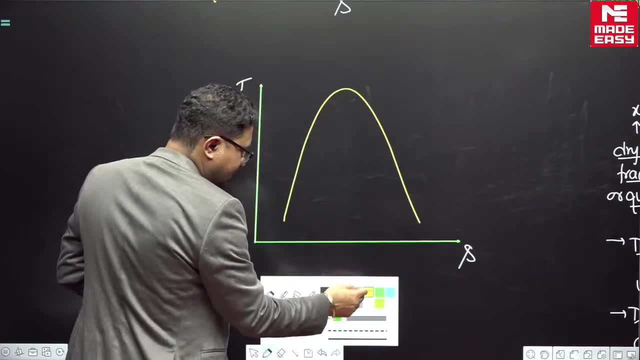 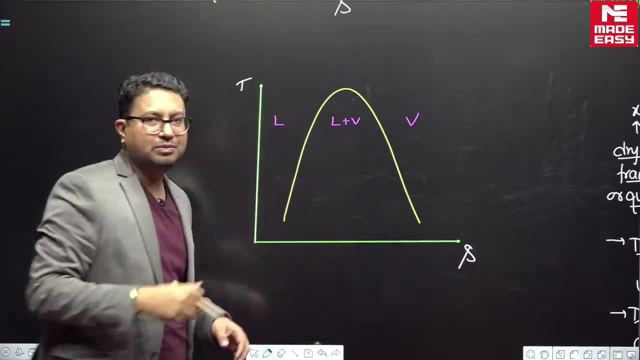 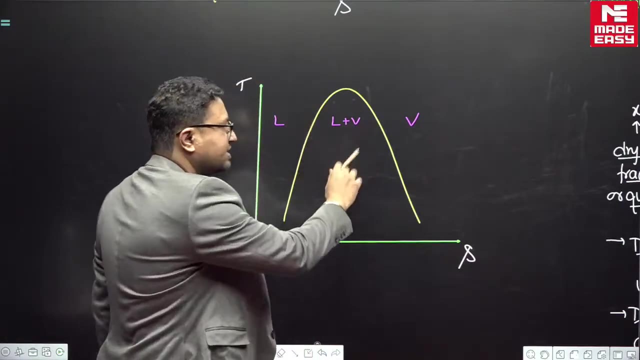 this saturation curve. let us say this is saturation curve and this is here liquid. then this is liquid plus vapour and then this is vapour. Now you see, there is a term called as dryness fraction, specifically for wet region. liquid plus vapour region. specifically, term is defined. 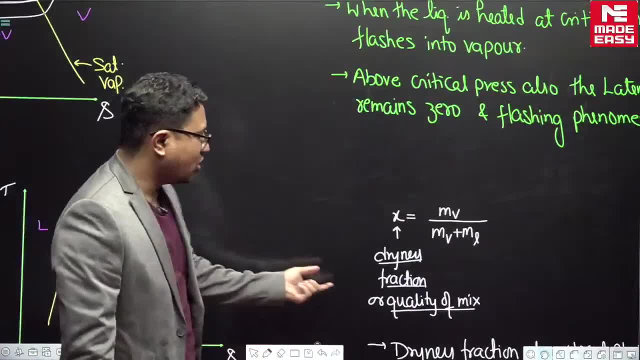 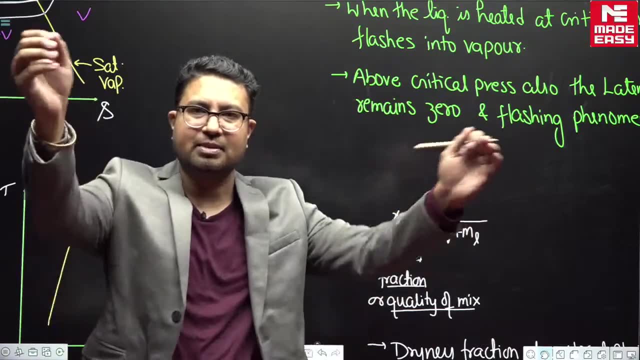 as dryness fraction. Now what is this? Dryness fraction? or quality of mixture? this is called the quality of mixture. So suppose we have a mixture, suppose we have a mixture. so we say that what is the mass of vapour? how much is the mass of vapour in the mixture compared? 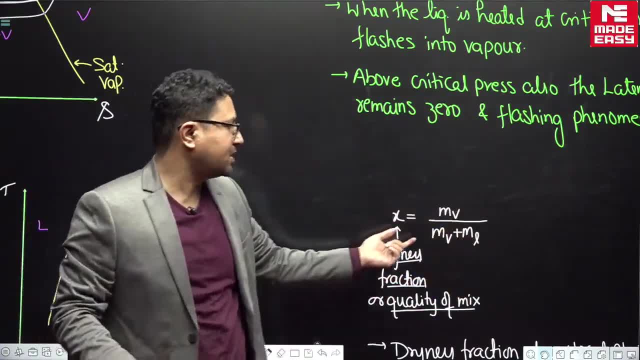 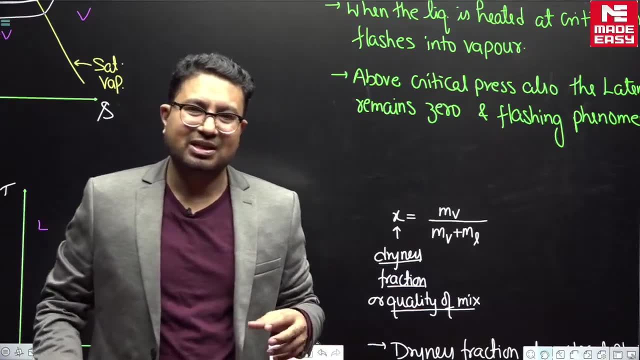 to the total mass. the total mass, the mass of vapour plus mass of liquid. in comparison to this, what is the mass of vapour which we have? Why we call it dryness fraction? Because see vapour does not have a wet region. 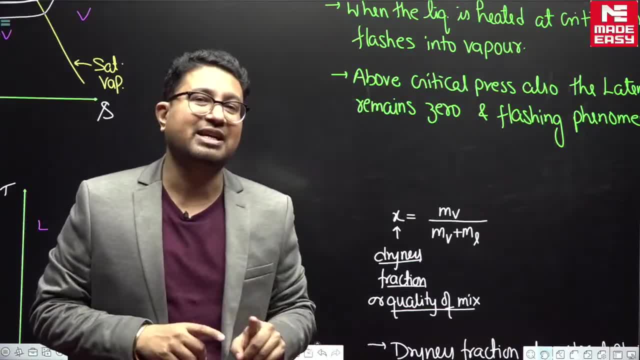 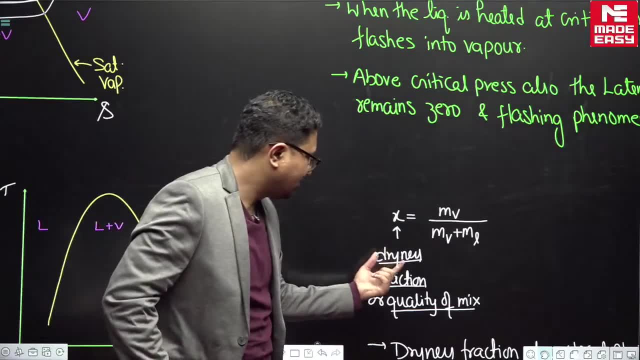 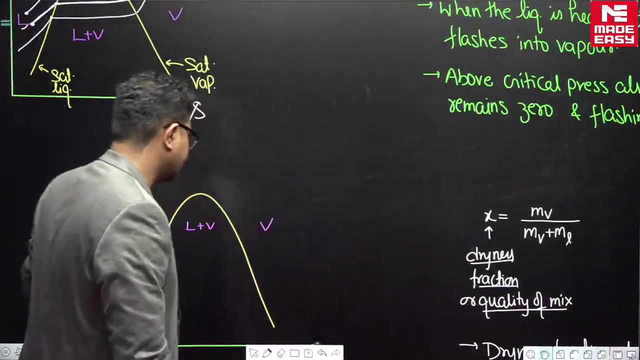 It does not have a wetting action. So how much is the dry part? That is, what is the dryness fraction. That is the dryness fraction. So, out of the total, what is the part that does not wet? that is the dryness fraction and this is the quality of mixture. Now, here let us. 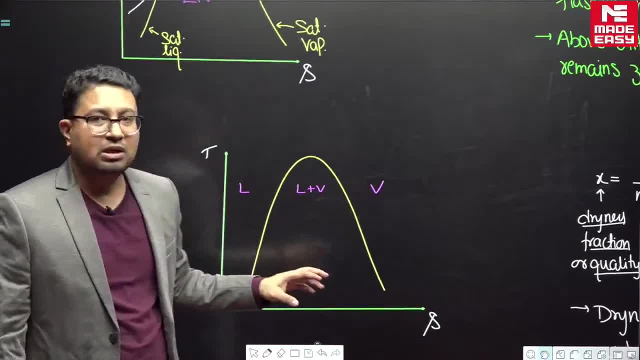 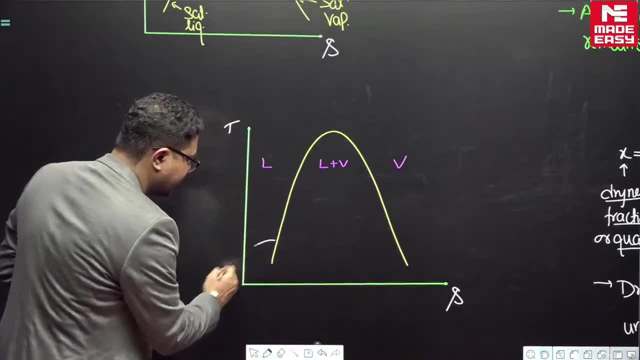 see, let us see here. see, if suppose you have only liquid, suppose saturated liquid. So if we have saturated liquid, if there is a saturated liquid, then we will say that we have any vapour. so the dryness fraction is 0.. 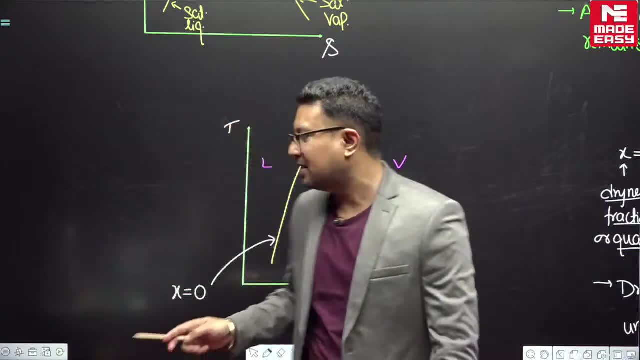 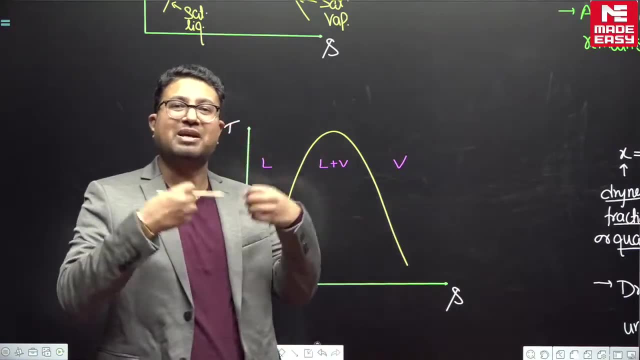 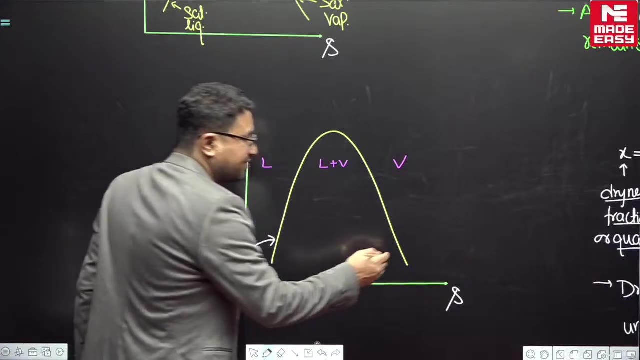 If we have only saturated liquid, wherever you are on this curve, there is only saturated liquid. If there is saturated liquid, there is no vapour. so we are only liquid. dryness fraction is 0,. if we are here some only liquid, then dryness fraction is 1, chso we are only 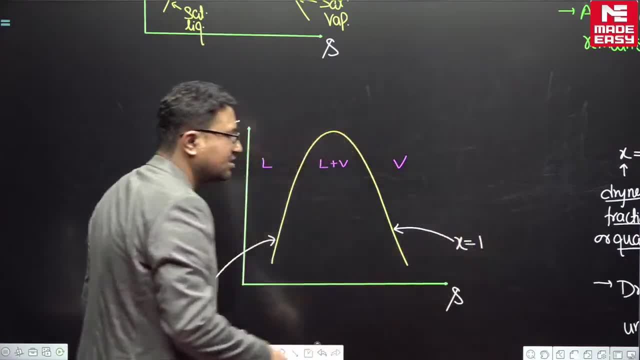 vapour. What are we only? We are only vapour. If we are talking about moisture distribution here, then let us say that we are only vapour. How much is the dryness fraction? We are only vapour. Wíem e hoti pubert centre. 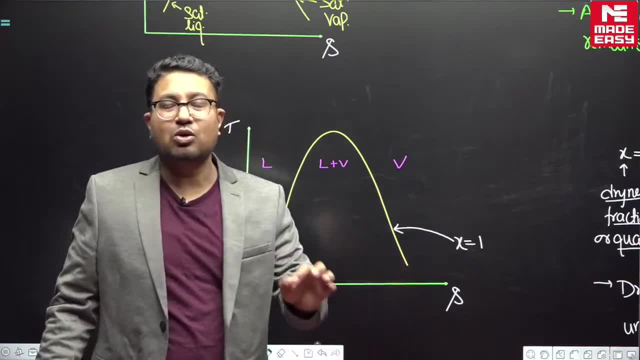 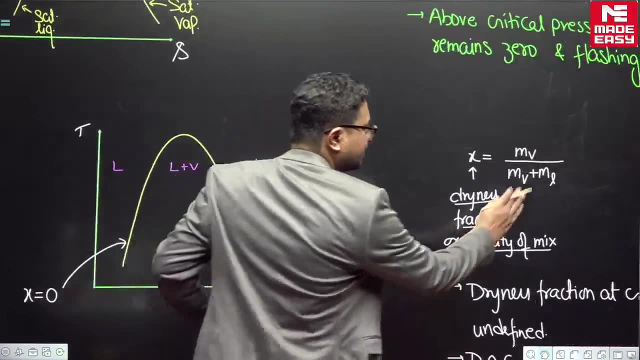 we are anywhere on this curve. if we are anywhere on this curve, then we are only vapor. we are only vapor. So dryness fraction is 1, because there is no liquid. mass of liquid is 0, mass of liquid is 0,, only vapor. But if you are suppose here, if you are in this, 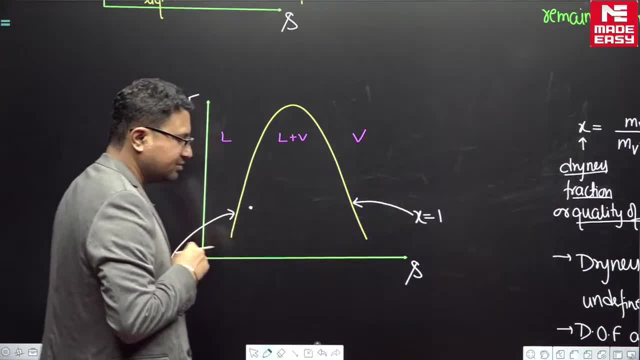 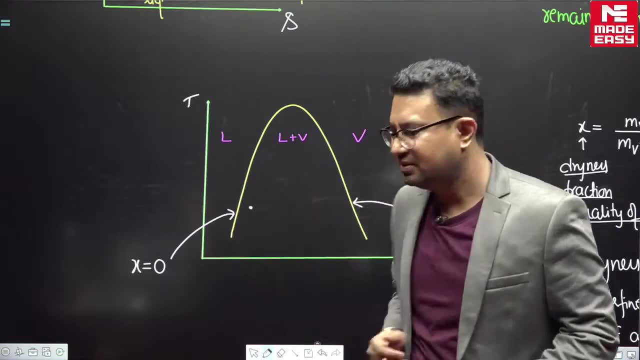 condition. if you are suppose here, so you are in a condition. you are in a condition where some part of you is liquid and some part of you is vapor, fine. So if you are in this condition, if you are in this condition, then some part of you is liquid. let us say: 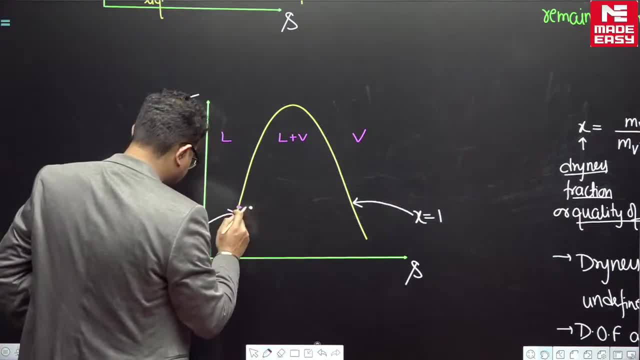 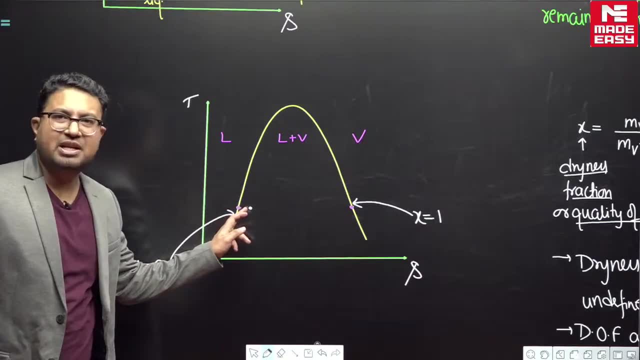 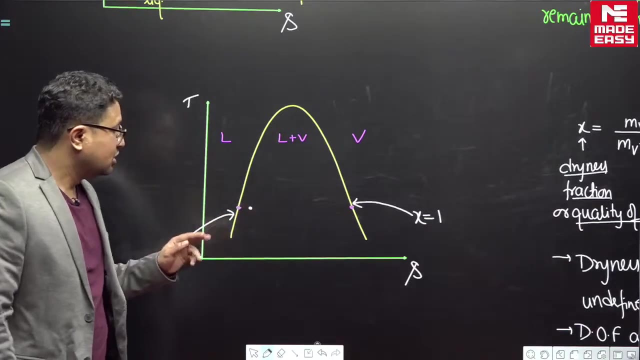 the liquid part is this: some part is your liquid and the some part. the some part is vapor, some part is vapor. fine, So obviously liquid will be more. the average is closer to liquid, average closer is of liquid, so liquid part will be more. So let us say there: 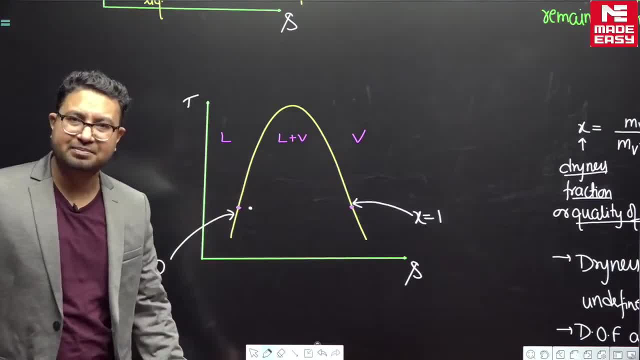 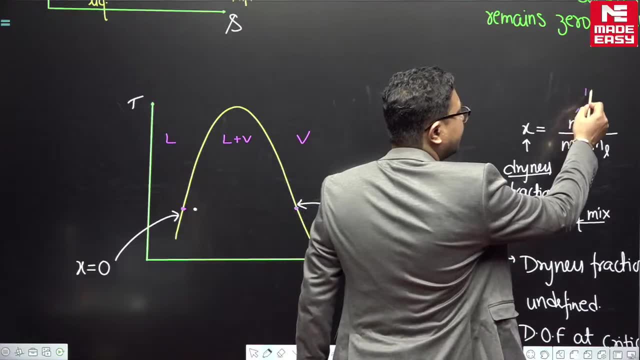 is 10 percent vapor. suppose 10 percent vapor is there, 90 percent liquid is there. So if there is 10 percent vapor, So vapor is 10, liquid is 90, 10. let us say 10 gram, say 10 gram, this is 10 and this. 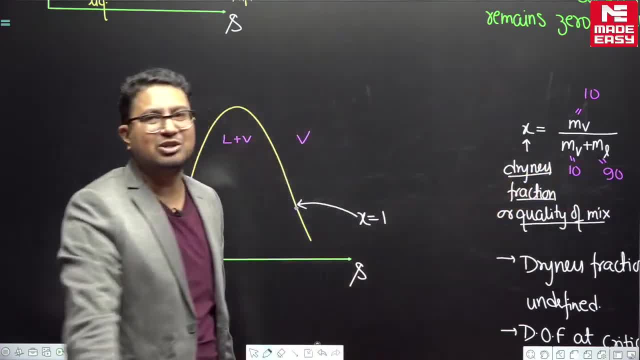 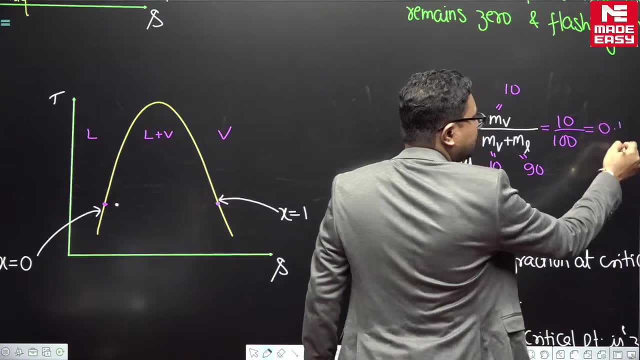 is 90.. So 10 upon 100, that is 0.1, 10 upon 100, 10 upon 100, that is 0.1.. So dryness fraction is 0.1, or quality of mixture is 0.1.. So 0.1 dryness fraction. there will be many points. 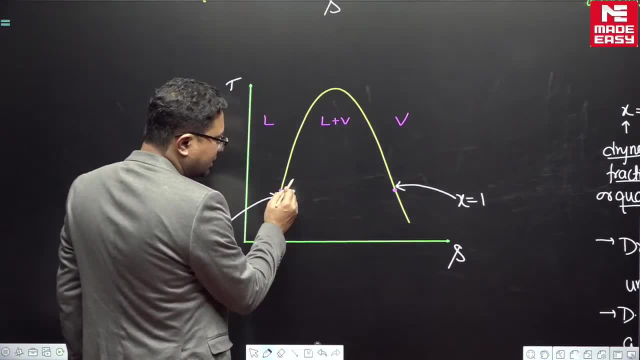 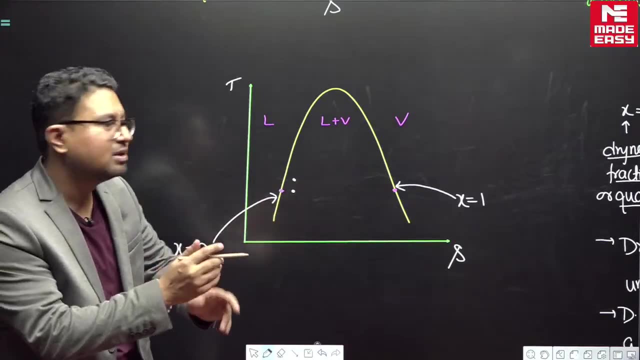 like this. there will be many points like this which are closer to liquid curve. So all these points which have this composition: 10 percent vapor and 90 percent liquid. So, if we join all these points, if we join all these points, if we join all these points, 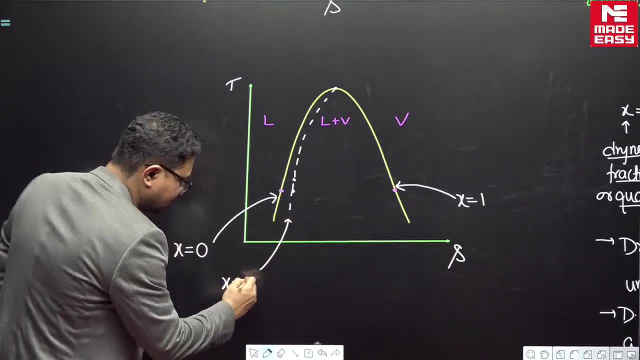 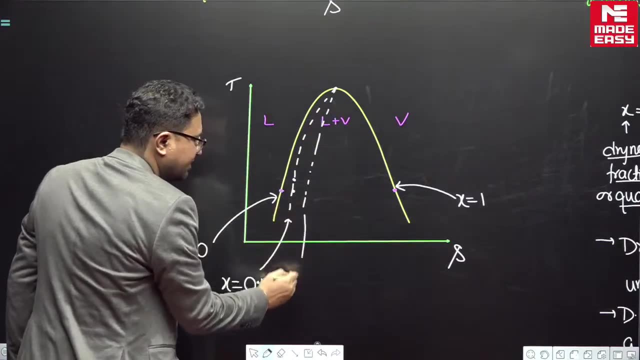 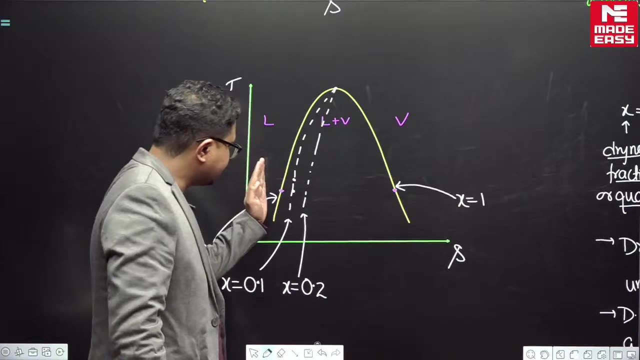 so we get constant dryness fraction curves. So X, 0.1, this curve has come. Then there will be other points which are having the dryness fraction 0.2.. As we are moving away from the saturated liquid, as the saturation liquid is going towards to the other side. 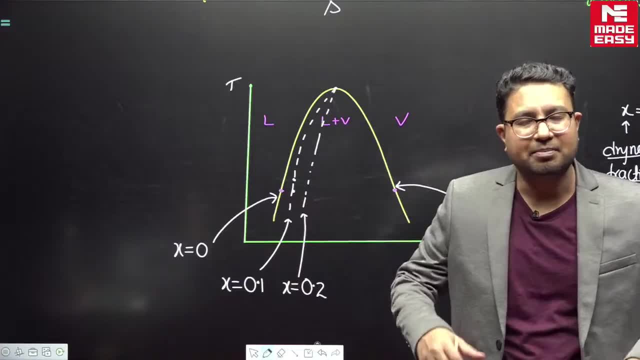 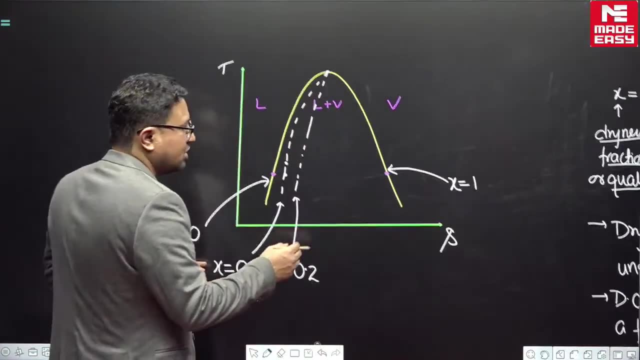 As we are moving away from the saturated liquid, the vapor percentage will increase. Vapor percentage will increase. So the dryness fraction will increase. Dryness fraction will increase. So here, if you are closer to here, there will be points who will have 90 percent vapor. 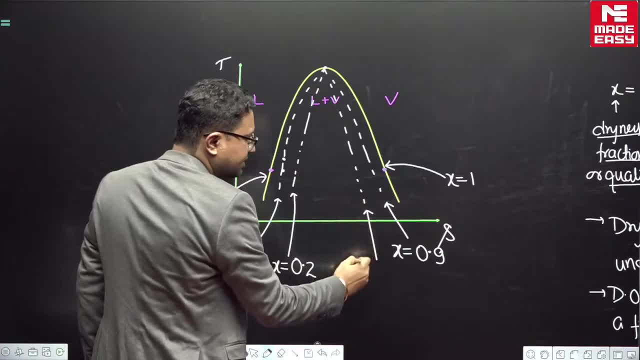 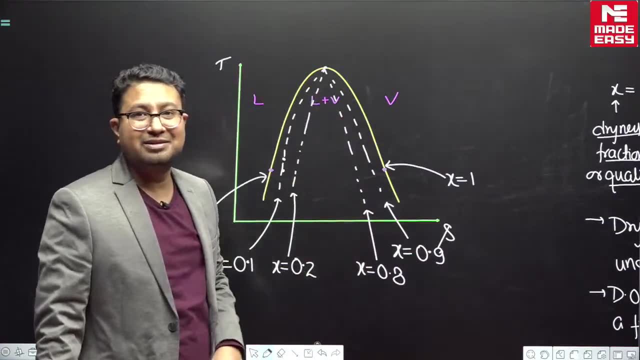 Then there will be points who will have 80 percent vapor. So dryness fraction will be 0.8.. There will be dryness fraction 0.8.. Critical point: What is the critical point? At the critical point there is liquid or vapor. 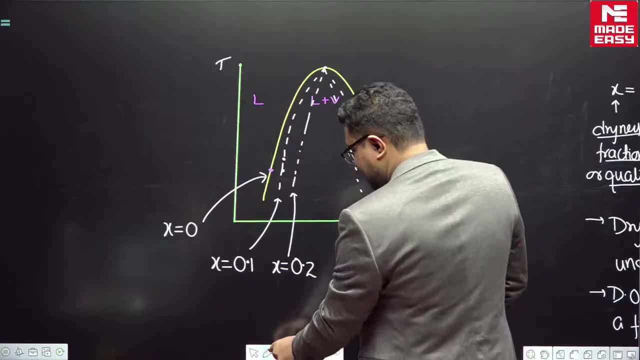 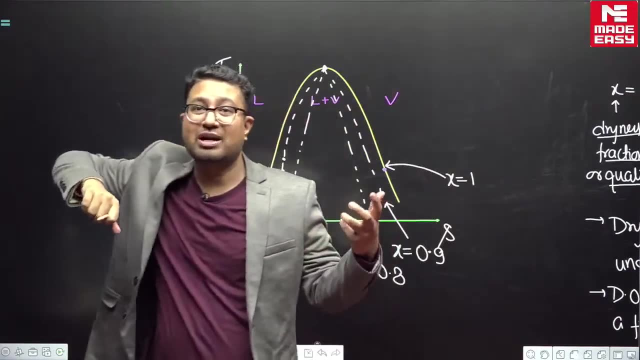 Look: saturated liquid and saturated vapor curve meet. Saturated liquid and saturated vapor curve meet So exactly at the critical point. what are you? You are liquid or you are vapor. We are not able to define, We cannot tell exactly. 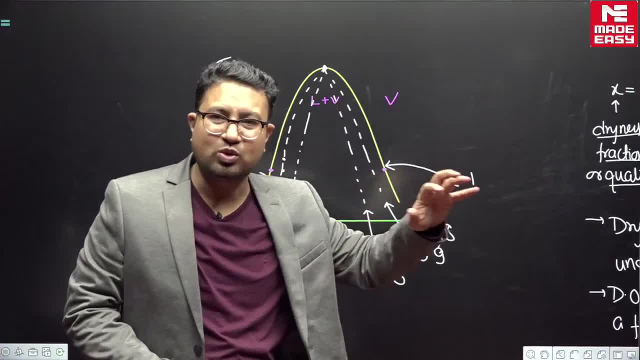 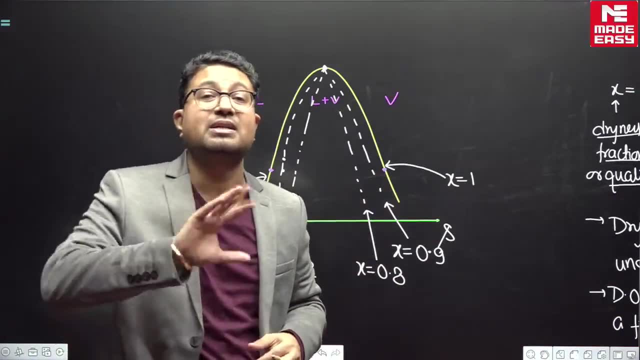 There are the properties which will be closer to liquid. There are some properties which will be closer to vapor. Some properties are closer to liquid. Some properties are closer to vapor. So you cannot tell, You cannot name it. Some people will say better to consider it as liquid. 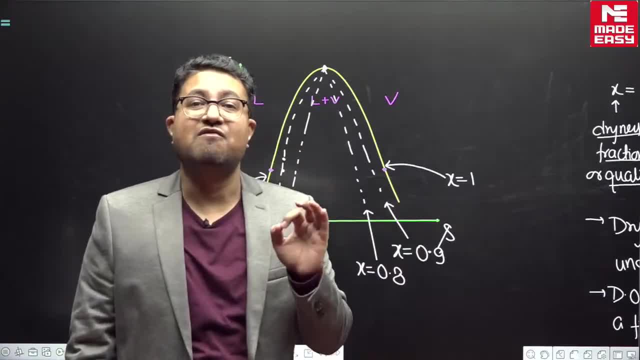 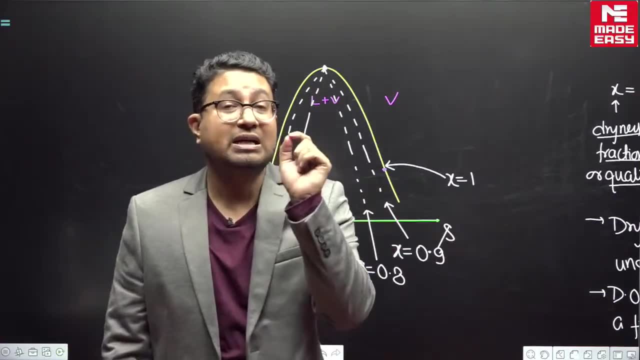 Some people will say better to consider it as vapor, But we are not able to clearly say that we should treat this. It is not like there is a mixture. Understand, At the critical point there is not mixture of liquid and vapor. There is no mixture of vapor and liquid. 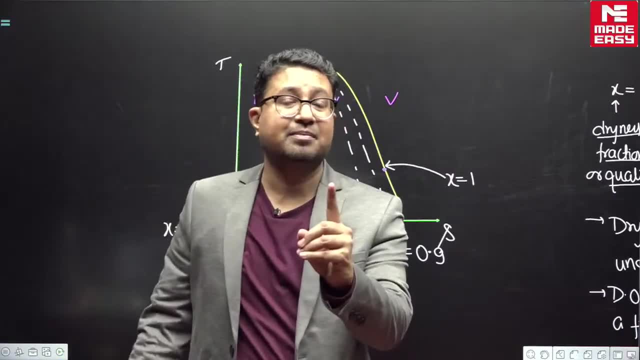 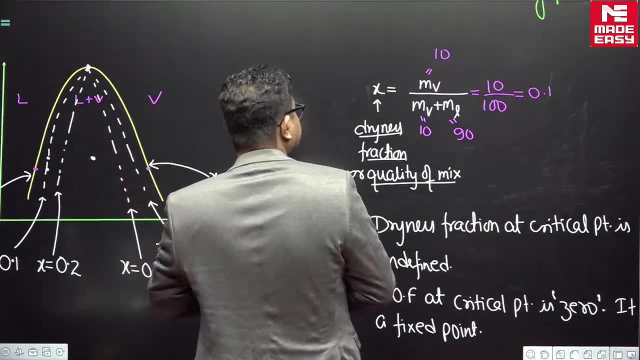 It is a single condition. There is one state, There is one state and one condition Here, Brother, Here, If you are here, Suppose if you are here, So you are. mixture of liquid and vapor. Some part is liquid. 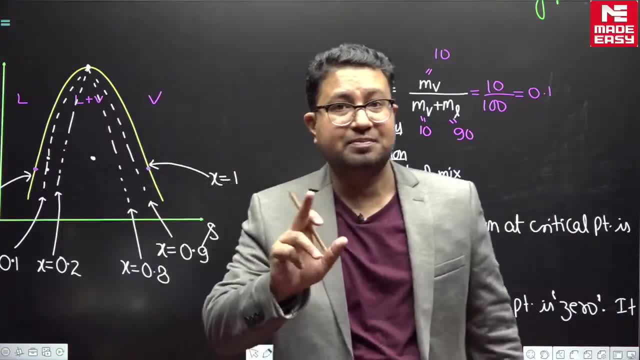 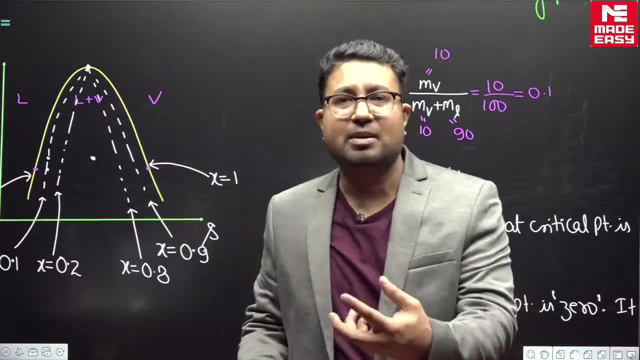 Some part is vapor At the critical point. you are not a mixture. It is not like there is a mixture. You are at one condition: We are not able to judge. We are not able to judge whether we should call you as liquid or whether we should call you as vapor. 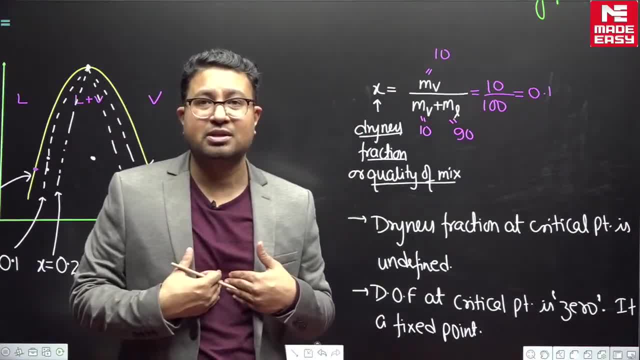 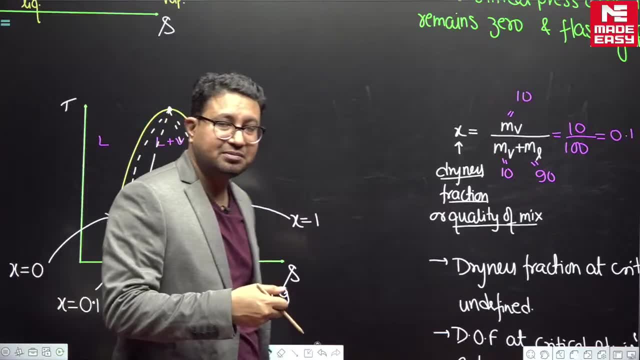 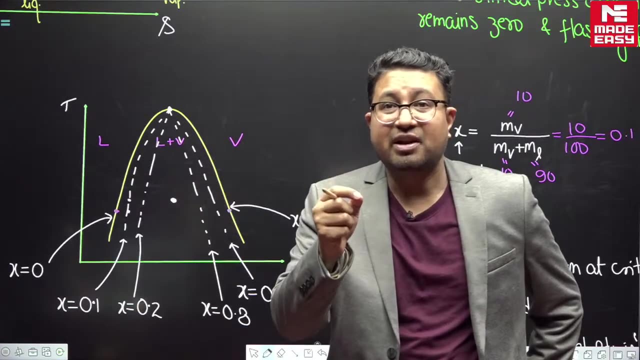 We call you liquid or vapor, We are not able to judge. So if we are not able to judge, If we are not able to judge, So we say, We say we say that we will not be able to define your dryness fraction. If we are not able, 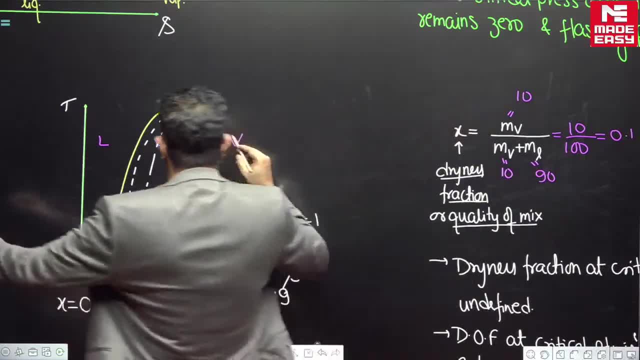 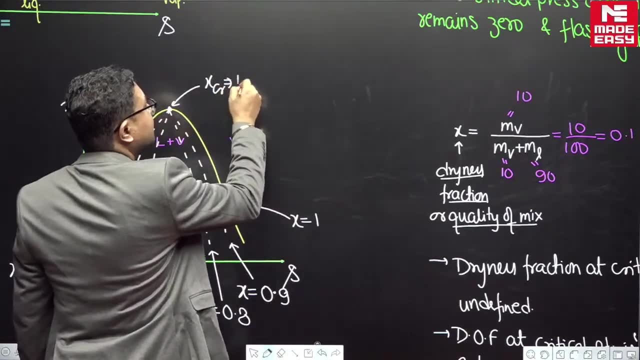 to judge, we will not be able to define. So. dryness fraction is undefined. So critical point, So critical point with dryness fraction is not 0,, it is not 0,, it is not 0,, it is. 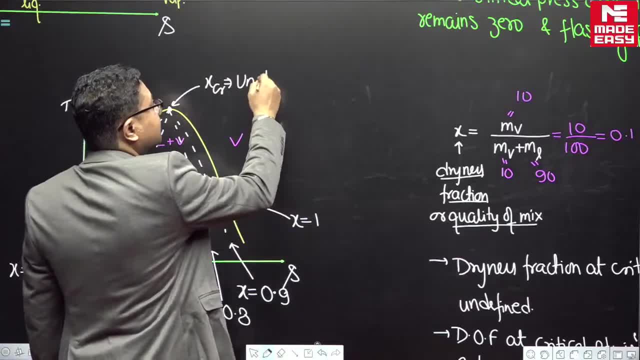 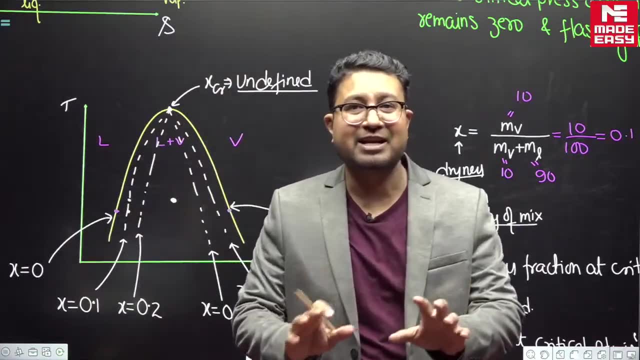 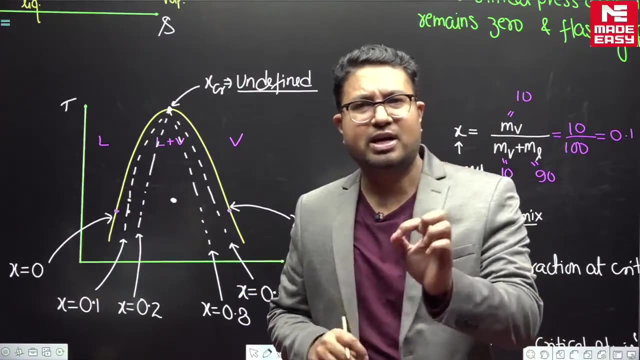 not 0.5,, it is not 1,, it is undefined. We are not able to define undefined undefined. That is why we are not able to apply the Gibbs space rule directly. Gibbs space rule directly apply Degree of freedom for critical point is 0.. It is a fixed point. It will be a single. 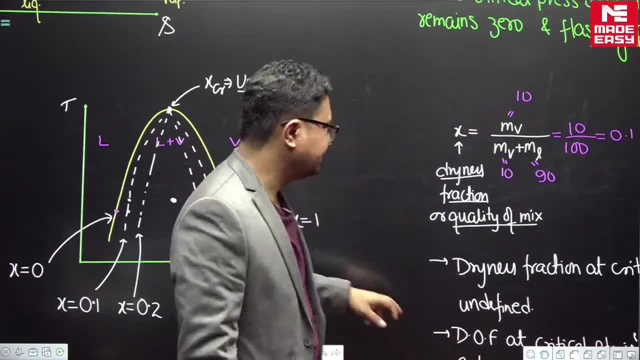 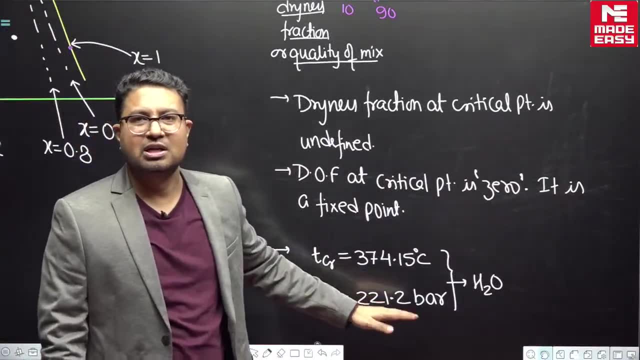 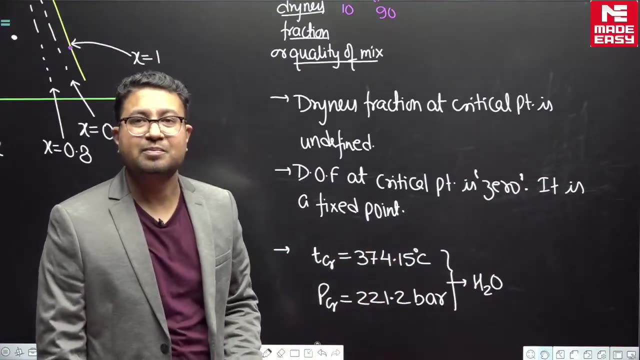 point for each substance. For water, the critical point- temperature is this and pressure is this. You have to remember this value because in some of the exams they randomly ask these values for water. So critical temperature is 374.15 degree Celsius If the H2 is above. 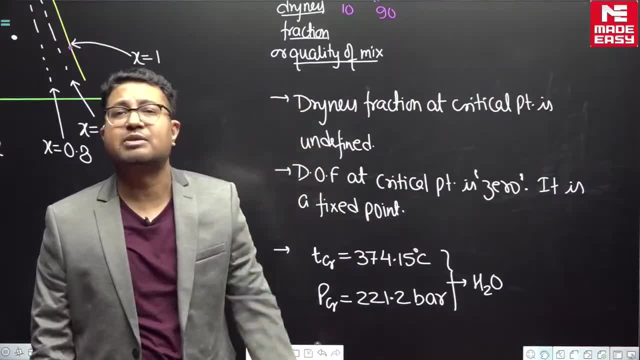 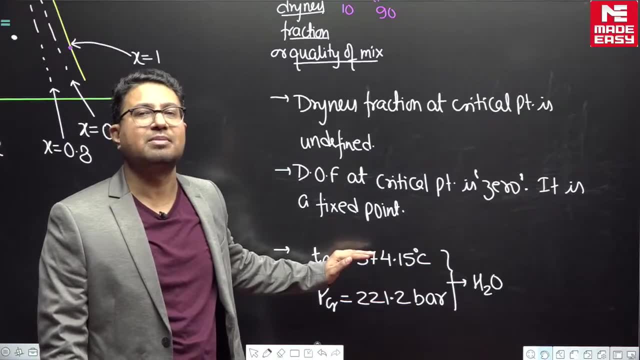 this: no matter how high the pressure is, it will not be in the liquid state. Above critical temperature, substance cannot exist in the liquid state. This is the pressure: 221.2 bar. So these are the properties of critical condition and degree of freedom. 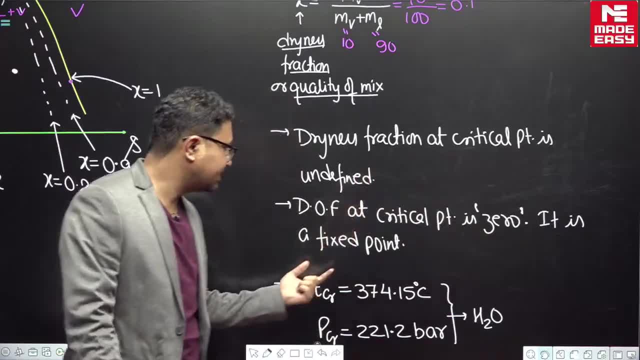 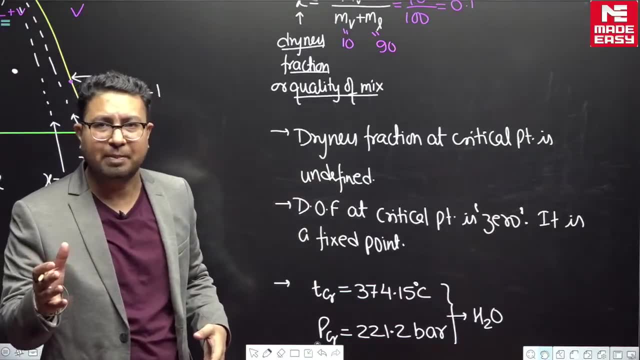 Degree of freedom at critical point is 0.. I have already told you: It is a fixed point. It is a fixed point. You cannot apply the Gibbs space rule because you are not able to decide the phase You will not be able to apply. It is an exception. So here you. 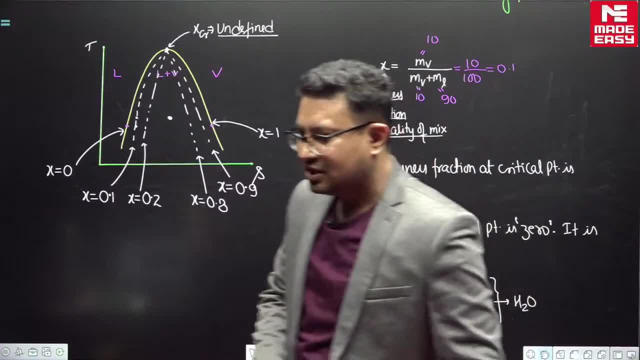 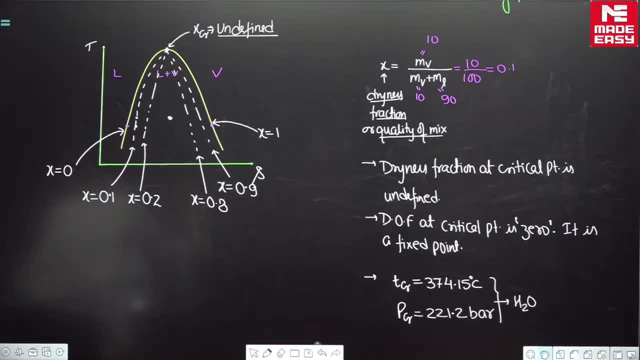 can just take this. So we have discussed this, So let me see how the discussion is going. Fine, So very nice. Yes, I will solve some questions. I will also solve some questions, Deepak, on this topic. So I am discussing the theory part and then I will move on to the questions. also, We will 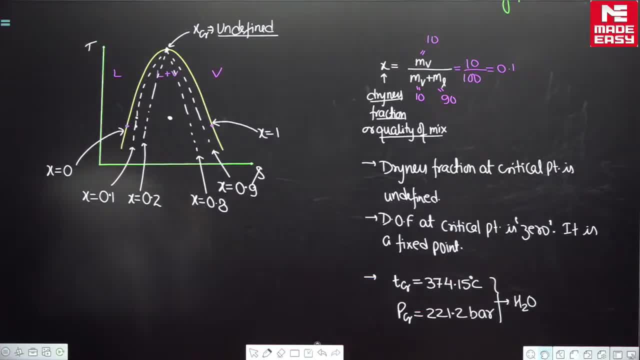 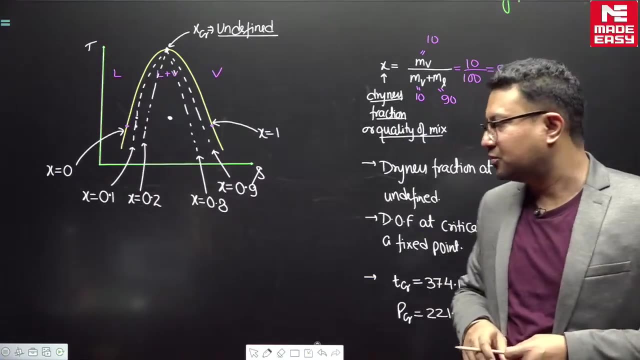 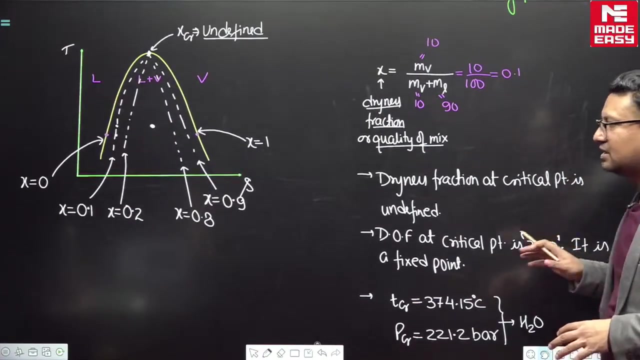 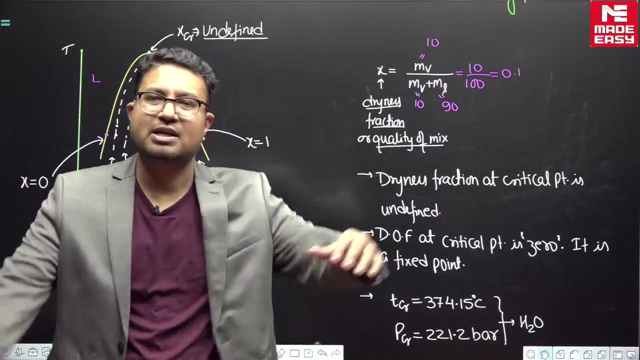 move on to the questions also for this topic. So fine now see Degree of freedom at critical point. This is a D degree here. This is a D degree here. So if we move further, if we move further, so we can say that, we can say that here we discussed about the dryness fraction. So, step by step, we are developing the concept. We are developing the concept step by step and we are trying to understand things. We will solve questions also. 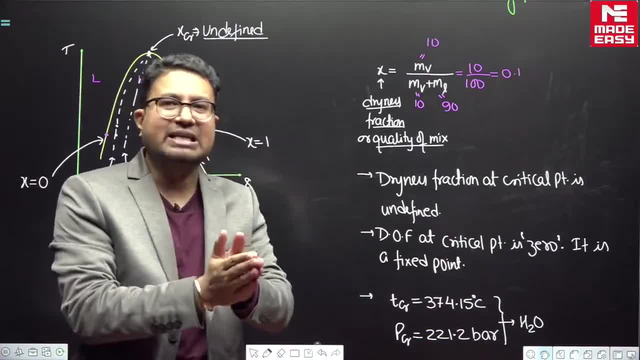 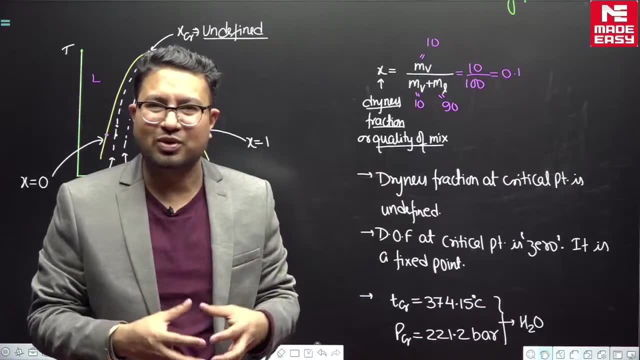 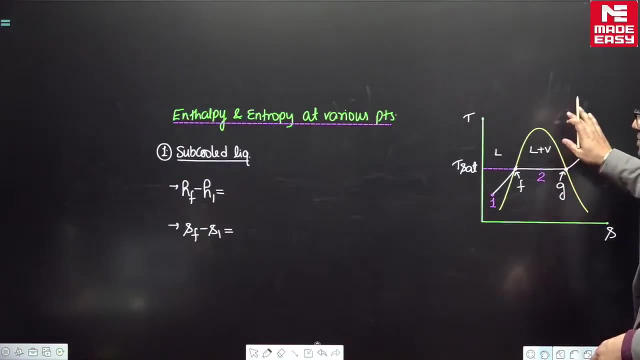 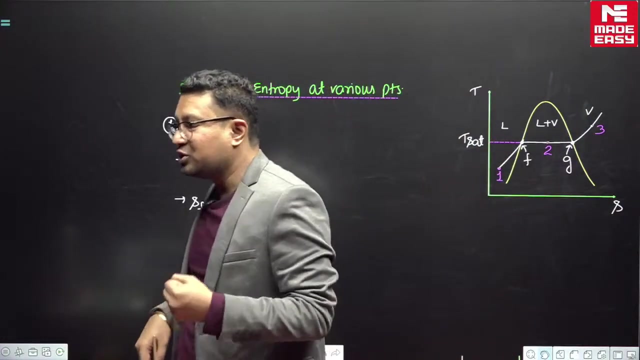 Because, look, if we have not applied anything, then that is not very useful in understanding Our discussion, will not be very useful if we have not applied it. So, next, if we talk about, next, if we talk about, look, so when we have to solve questions, when we have to solve questions, then we should know the formulas. we should have the formulas. 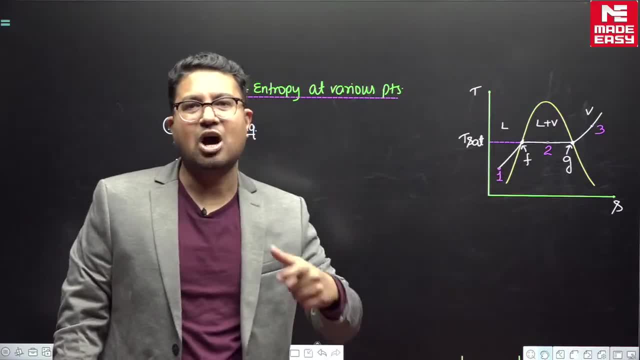 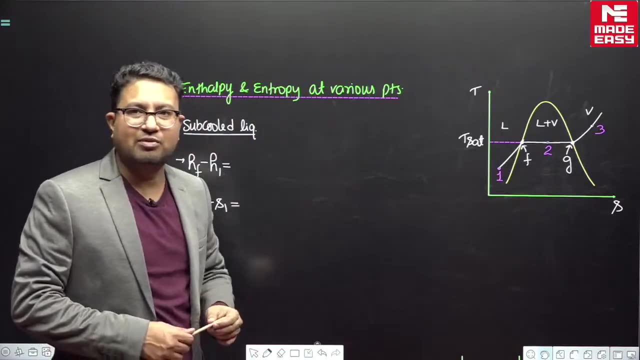 We should have some formulas right. So let us Understand how we develop the formula. How we develop the formula, So: enthalpy and entropy at various points, we want to write. We want to write: enthalpy and entropy at various points. 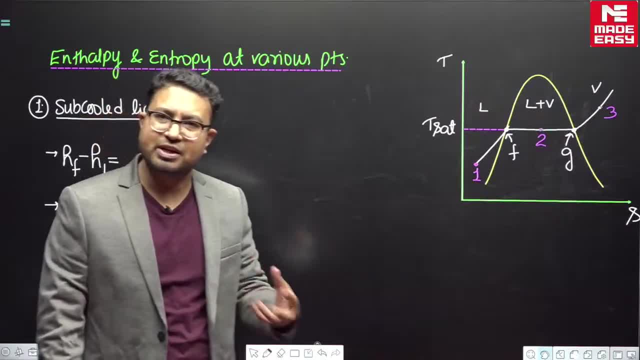 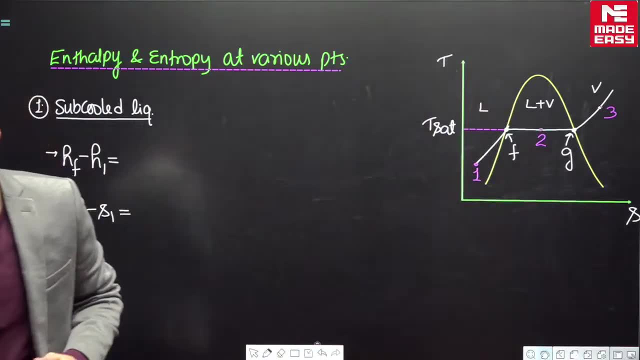 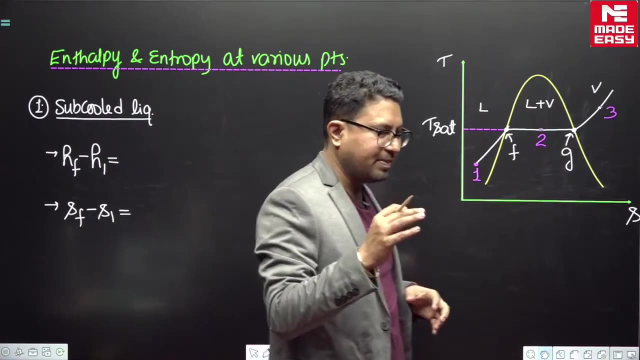 This is what we will need in our analysis. We will need it for question solving. So, step by step, let us see how we can write the enthalpy and entropy at various points. So let me just Sub cooled liquid First of all. 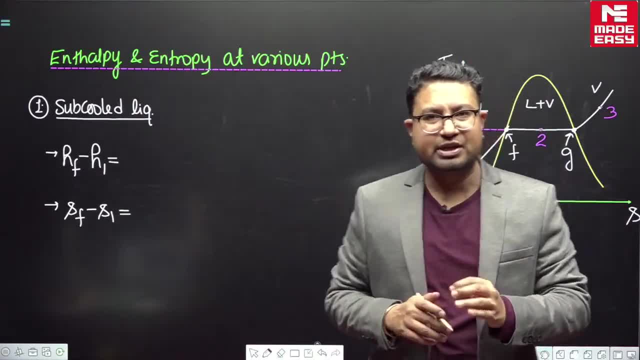 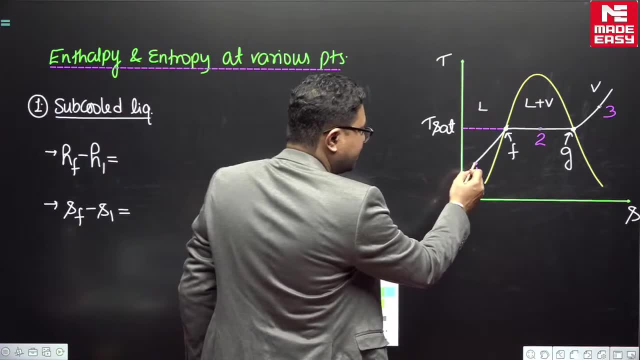 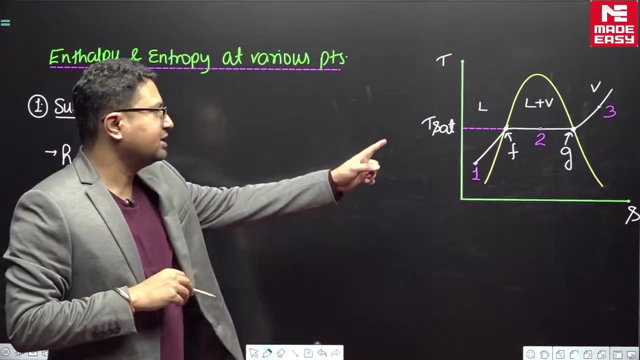 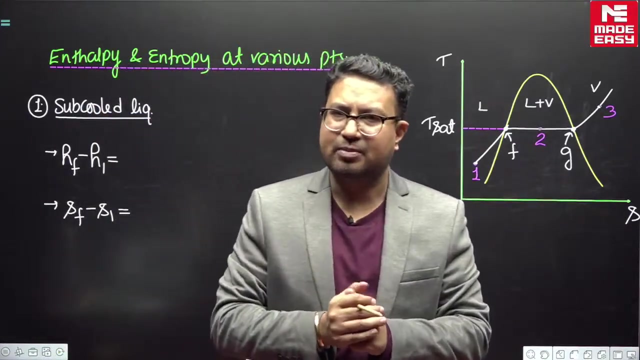 What is the condition of sub cooled liquid? So look at the condition of sub cooled liquid. We are here- suppose I am here. If we are here and we have to write here, this is the saturated liquid, we have to write enthalpy change because if we write enthalpy change, if we know the enthalpy change, so if one of the enthalpy will be known, you will be able to find out the other enthalpy. you will be able to find out the other enthalpy. 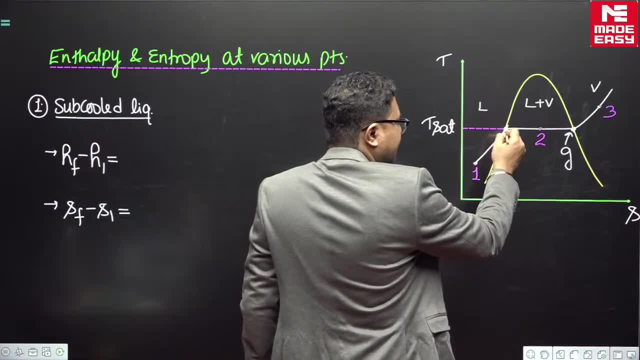 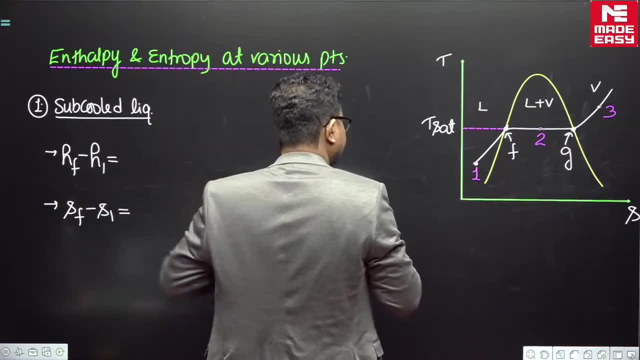 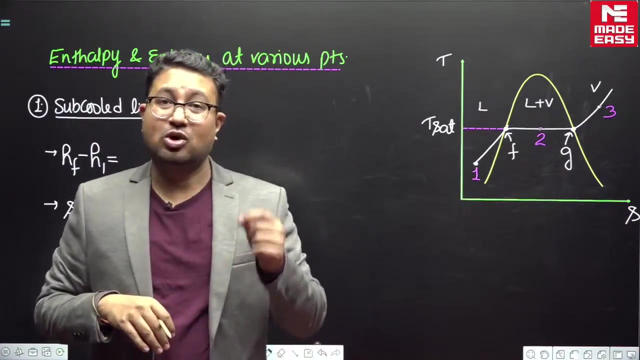 So this is hf. This is hf Enthalpy for saturated liquid. This is h1. Enthalpy sub cooled liquid. So hf minus h1.. hf minus h1.. Pressure constant. So Enthalpy change, Constant pressure. 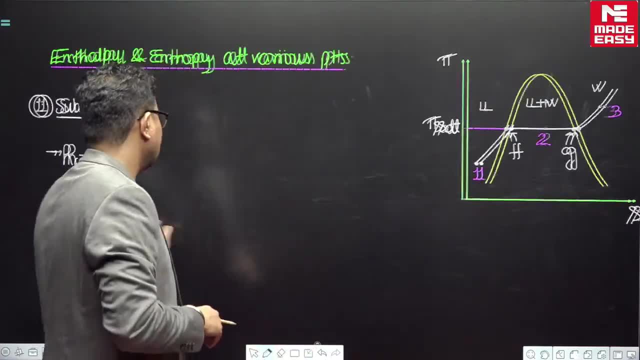 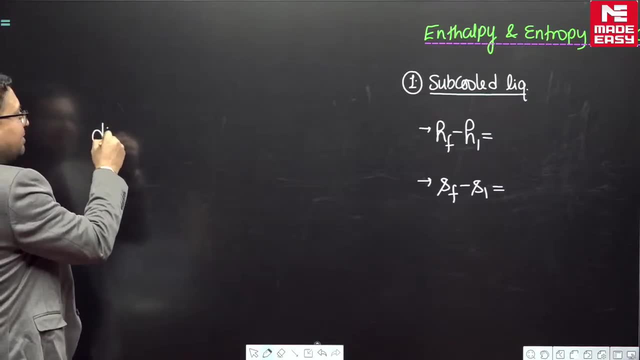 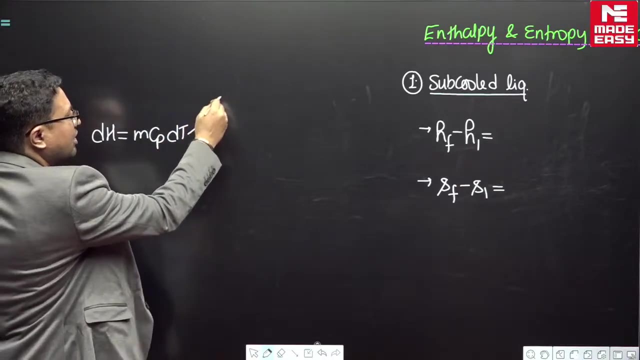 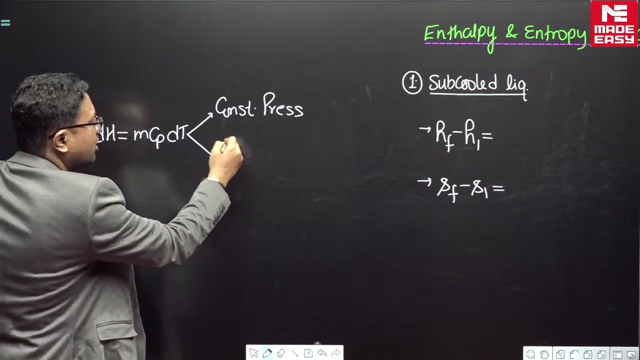 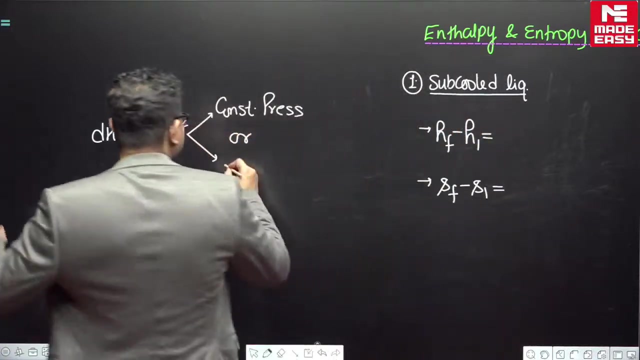 Enthalpy change, constant pressure, M, C, p, d, t. No matter what the substance is, I will write it once and show you. You can remember this. also. Enthalpy change is equals to M C, p, d, t. We can write d h equal to M C, p, d, t for constant pressure. we can write this for constant pressure. we can write this for constant pressure, or. or I can write this for constant pressure, or, or. the substance should be an ideal gas. 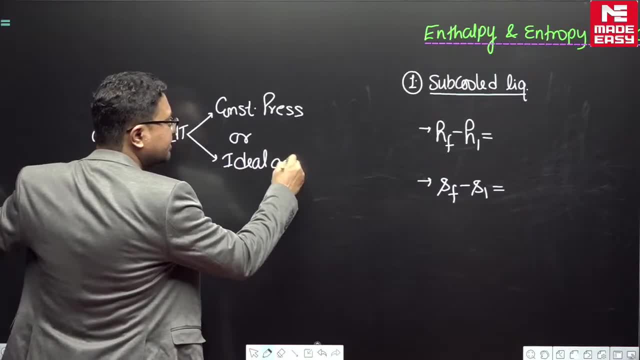 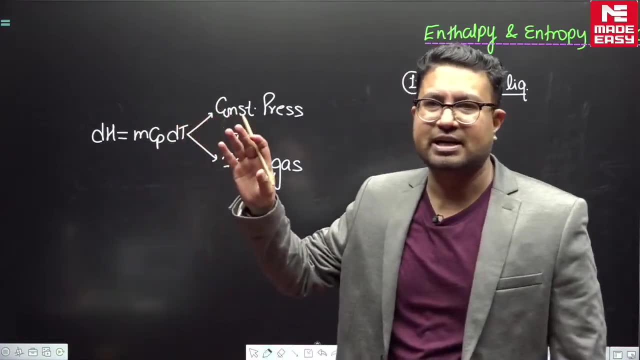 What should be the substance. Substance should be an ideal gas. If it is an ideal gas, then without bothering about the process- There is no need to worry about the process- You can use this Whenever you want, Whenever it is an ideal gas. 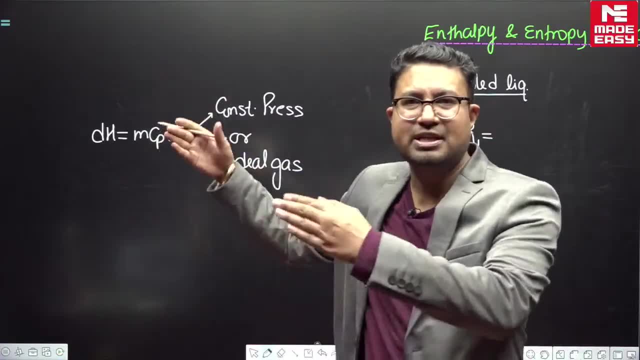 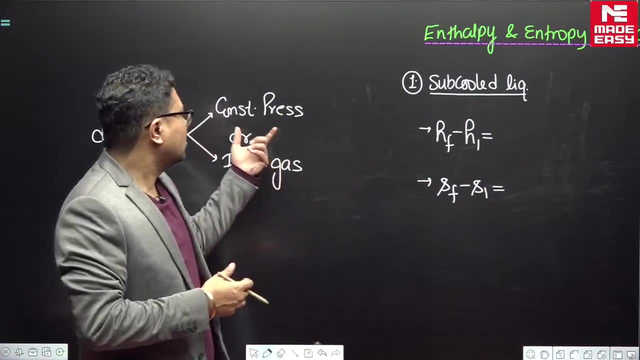 We will not go into this detailed discussion. We will not go into this discussion, Otherwise we will lose our track of the present discussion. We will go out of the discussion. So for writing this, we can remember, We can remember this constant pressure. 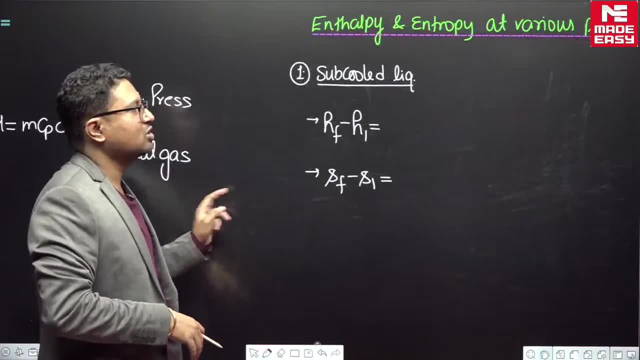 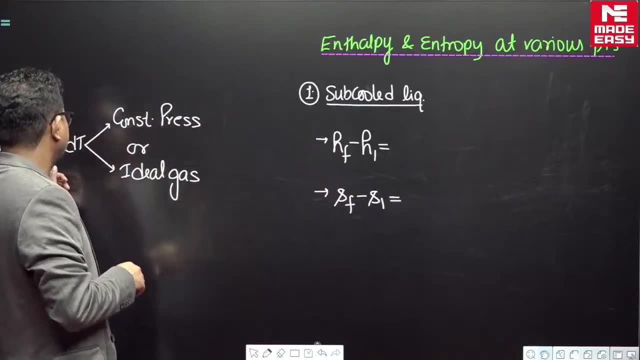 This is ideal gas. So because it is a constant pressure, Because it is a constant pressure, we can use this. And unit mass is M 1. M C p d t, M C p d t. So M 1 is C p d t. 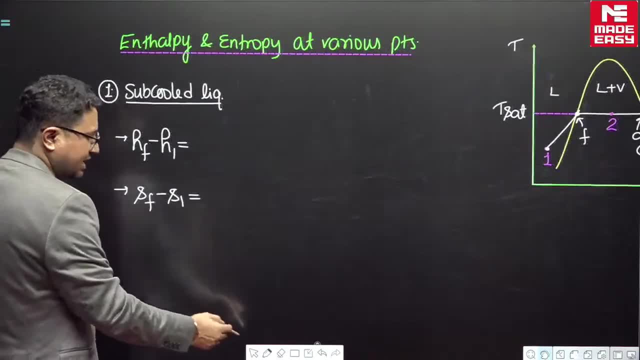 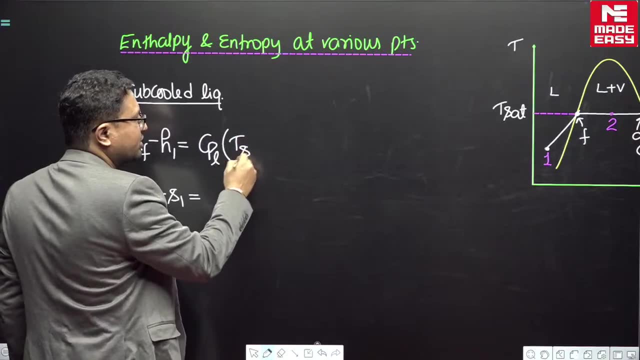 So we can write here. We can write it. We can write here: This is equal to C p. C p for what Liquid? C p for liquid Into d t. D t is T saturation, H F temperature is T saturation. 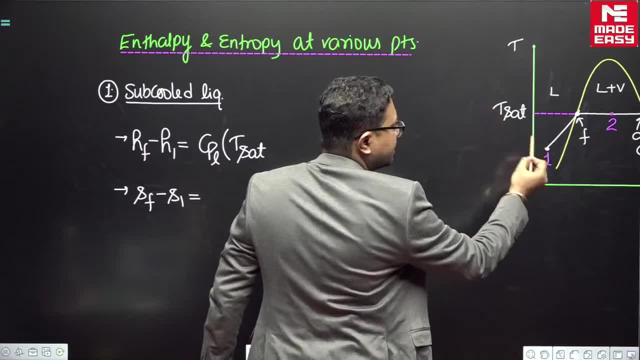 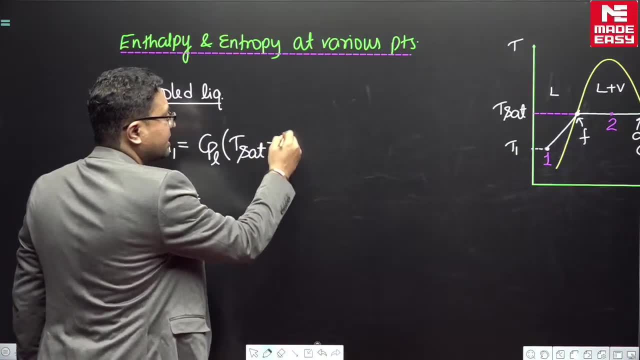 Now the temperature is T 1.. How much is the temperature? now It is T 1.. Now the temperature is T 1.. So T saturation minus T 1. T saturation minus T 1. So we are developing a formula. then we will solve questions so that we can solve the questions. 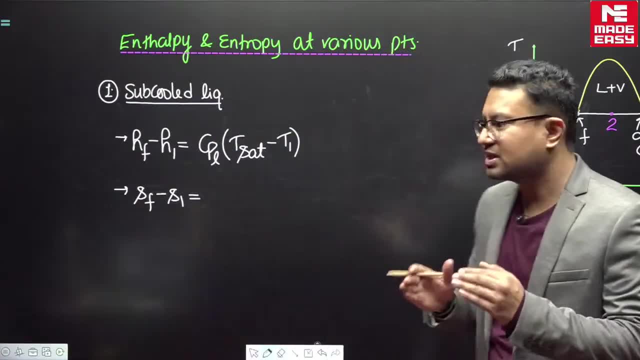 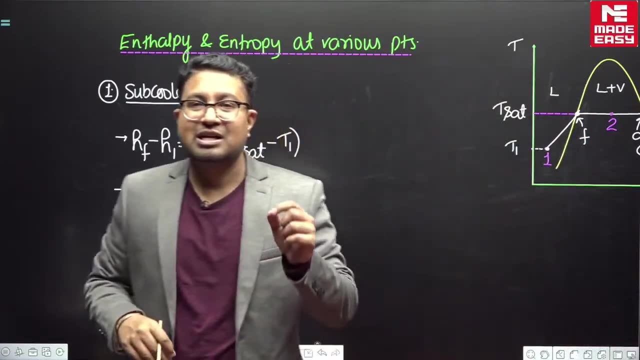 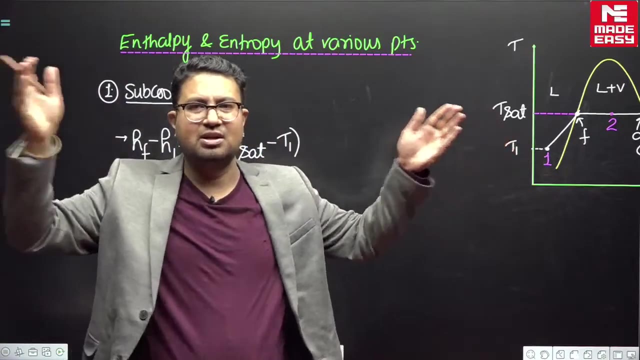 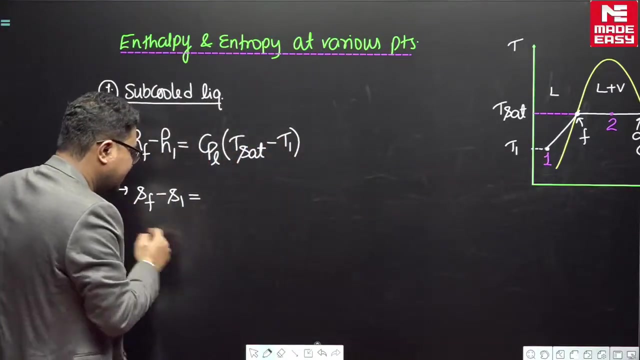 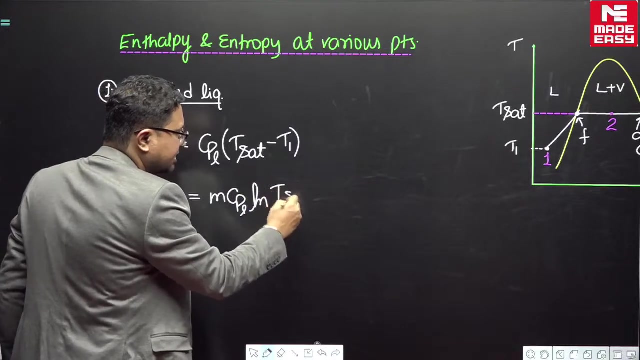 Okay, So just let us develop the expression. We are developing the formula: Now S F minus, Now S f minus S: 1. entropy change: liquid or solid, if there is a finite mass of solid. If there is a given mass of solid or liquid, then entropy change can be written as M Cp log of T final, that is, T saturation upon T 1.. 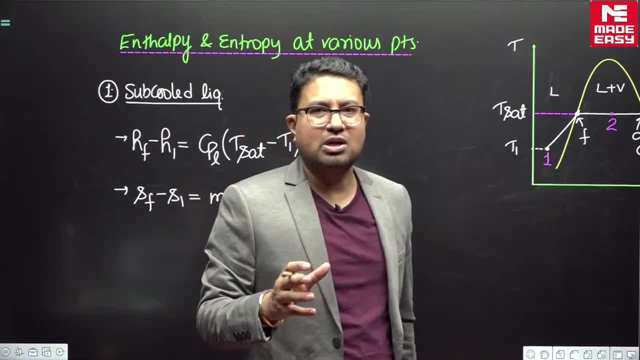 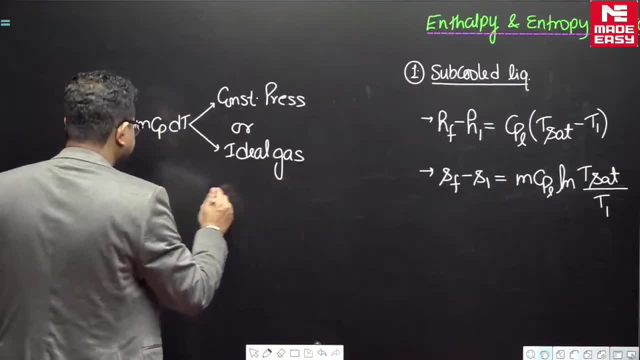 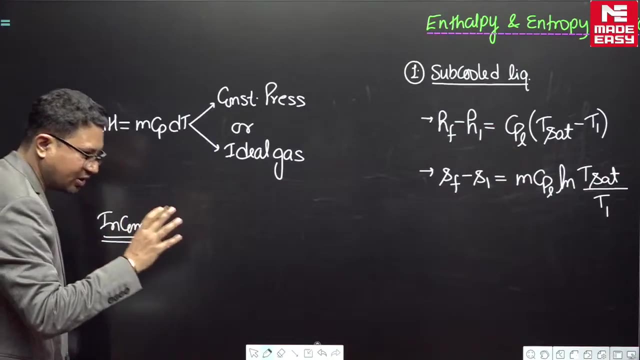 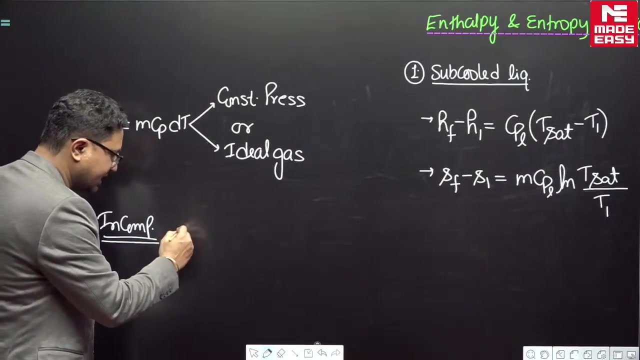 For solid or liquid, because the volume does not change. solid and liquid are incompressible substances. So for incompressible substance, what we can do: If it is an incompressible substance, we can say that Cp is equal to Cv is equal to C. 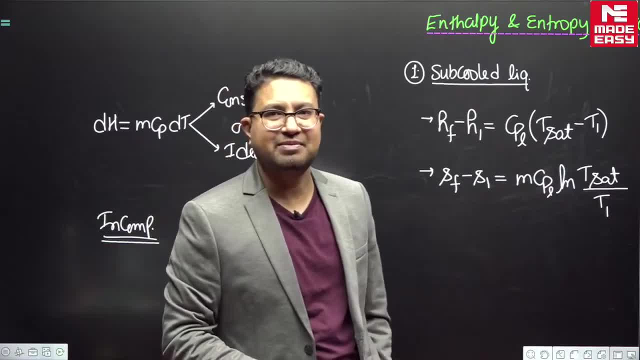 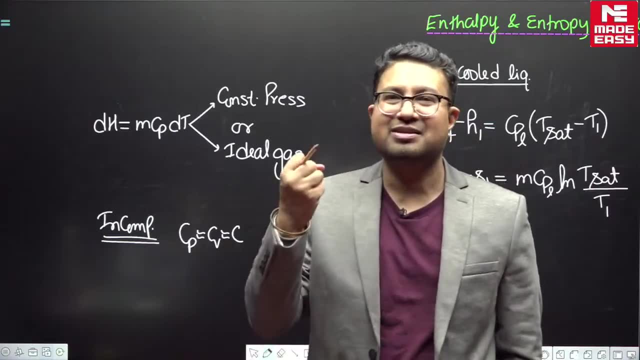 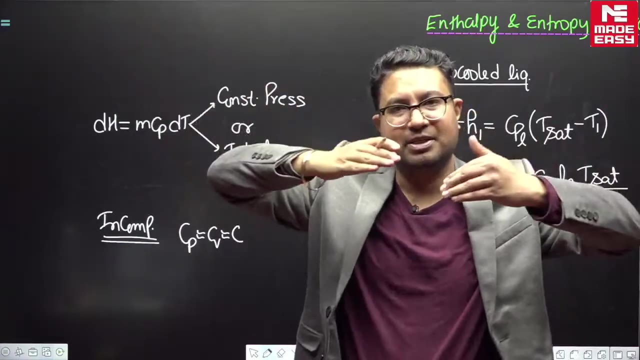 Specifically specific heat will be same. specific heat will not change. why there is no change in this specific heat. specific heat are different for different processes because boundary work can take place, Expansion, compression can take place. that is how the specific heats we have different specific heats. 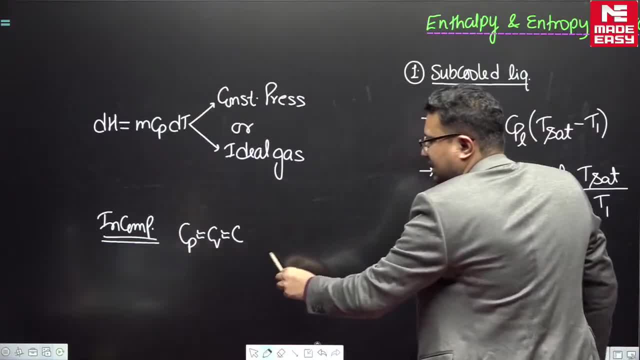 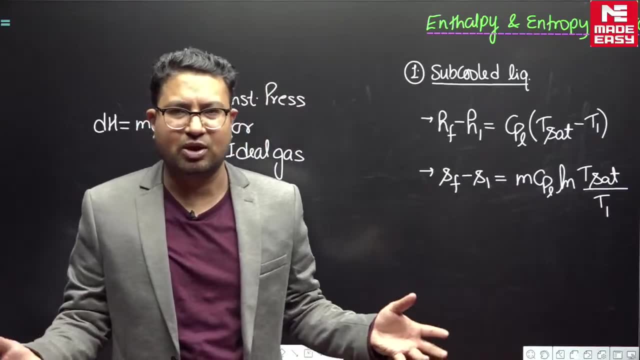 But if we have an incompressible substance, there is no volume change that can take place. That is why we use specific heat for water. That is why we use specific heat for water. What do we talk about? Specific heat for water? 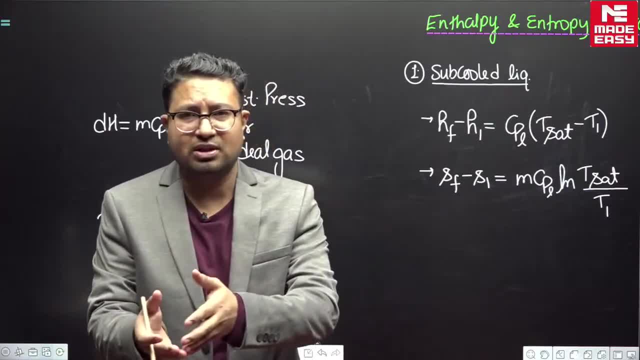 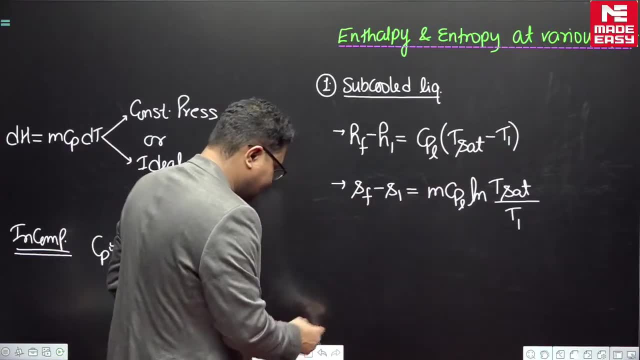 We say Cv for water or Cp for water. we do not say that fine, Now this here: M Cp dT. So for unit mass, if we are talking about the unit mass, this entropy change, we can write like this: M Cp dT. 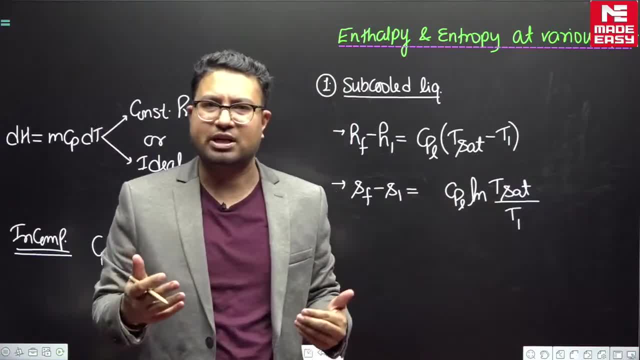 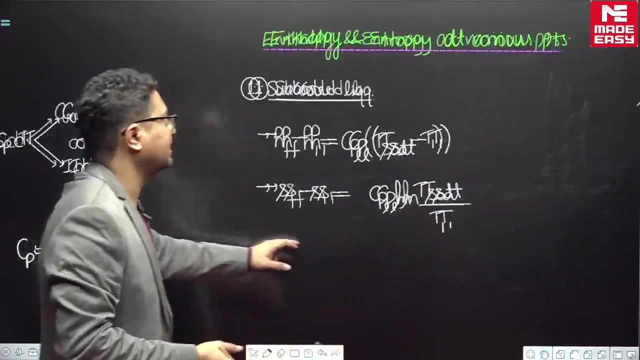 There is no term of volume, because volume change does not take place. So it will be like this for liquid: Whether we are writing Cp, Whether we are writing Cp or C, it does not matter. Anyways, we can write like this for liquid phase: fine. 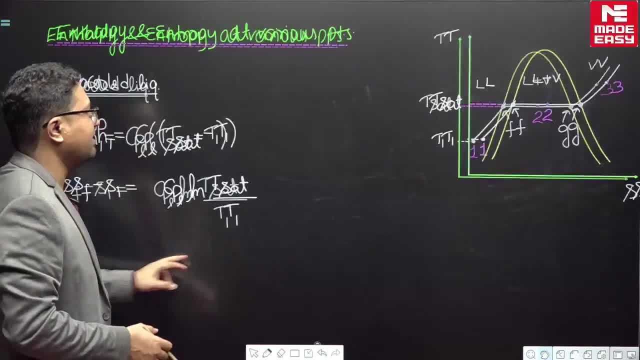 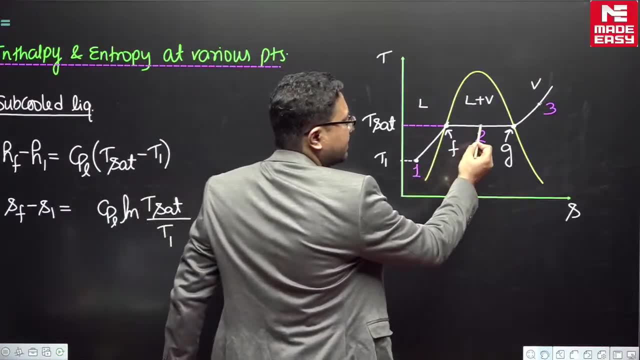 Then if we have to talk about, if we have to talk about the wet region, if we have to talk about the wet region, see How can we say for wet region, What is the meaning of wet region Here? suppose we are here. 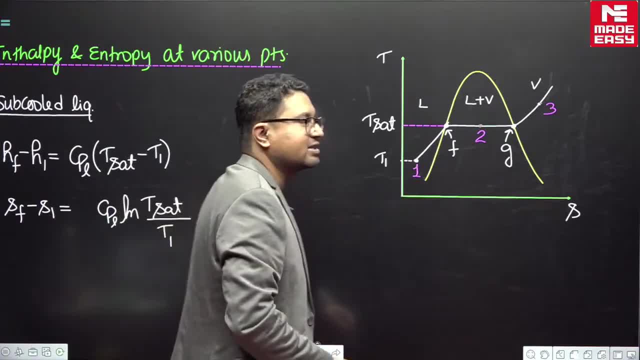 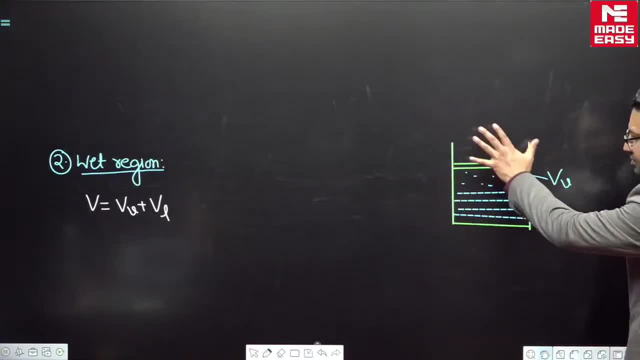 So how we can write it for the wet region. How can we write for wet region? We are trying to understand. see Now, suppose we have a piston cylinder element. Some portion is liquid, Some portion is vapour, Some portion is vapour and some portion is liquid. 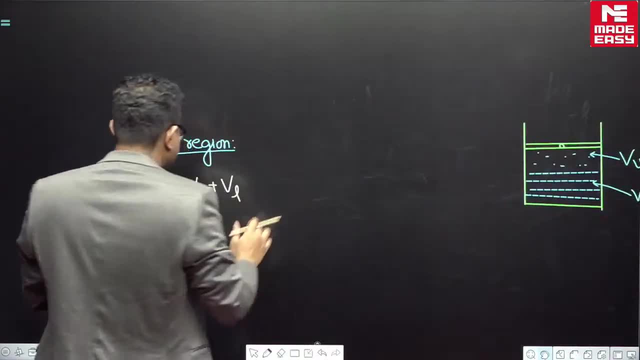 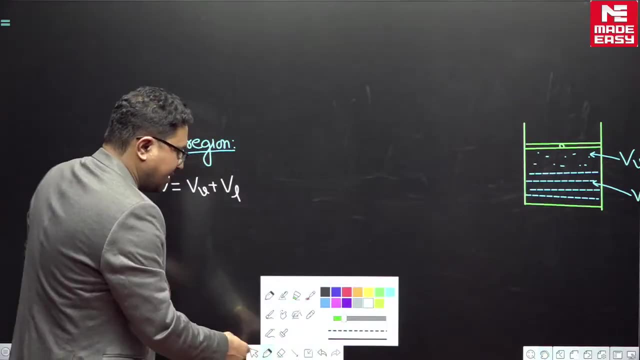 Now, total volume in the wet region can be written as volume: total volume, Volume of vapour plus volume of liquid. Can we write this? Yes, Now I can see. I am trying to develop. I am trying to show you here how the formulas come. 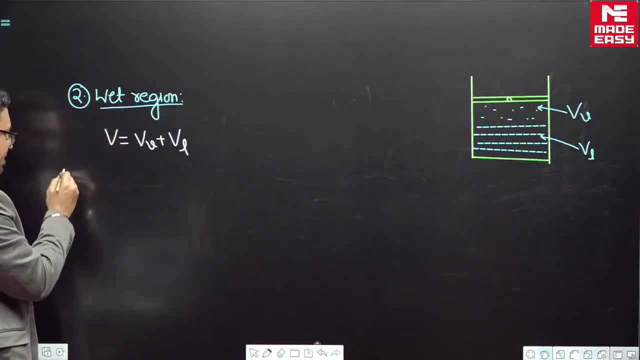 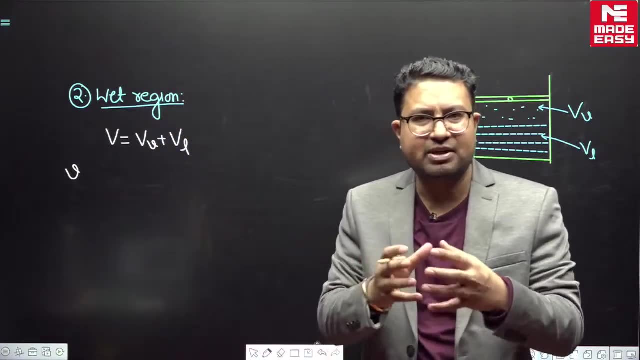 See, You can write the total volume like this also: Average is specific volume. Small v. What is small v. Average is specific volume of the mixture. There will be some average of the mixture. Specific volume: Specific volume Into total mass of the mixture. 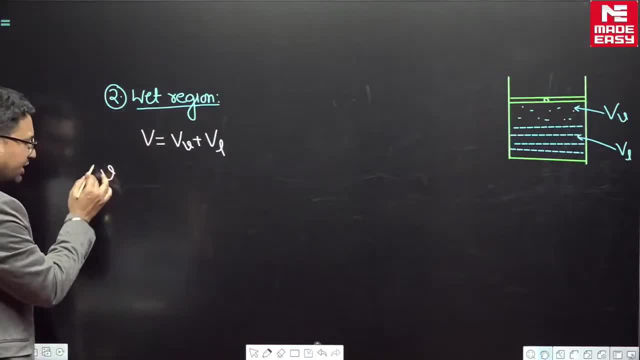 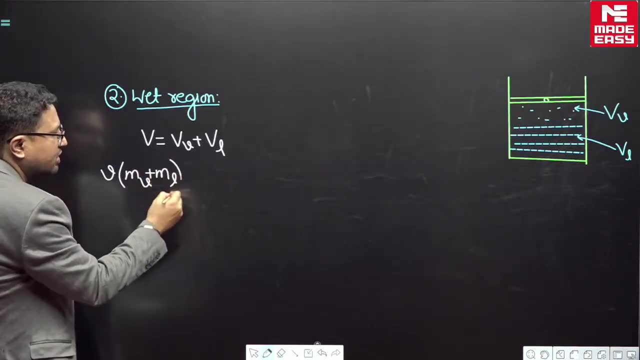 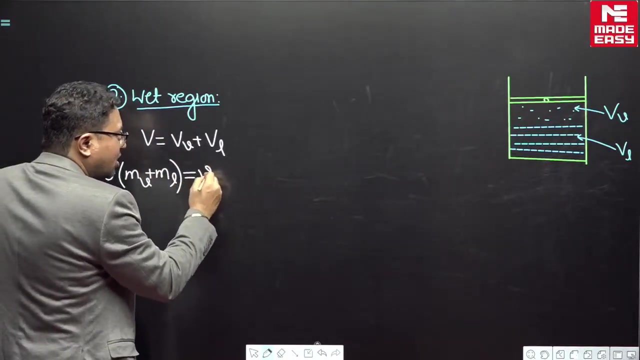 Into total mass of the mixture. What is the average volume per kilogram? Into how many kilograms of the mixture are present. Mixture is how many kilo mv plus ml This will be Is equals to volume for vapour. So what is the volume of unit vapour? 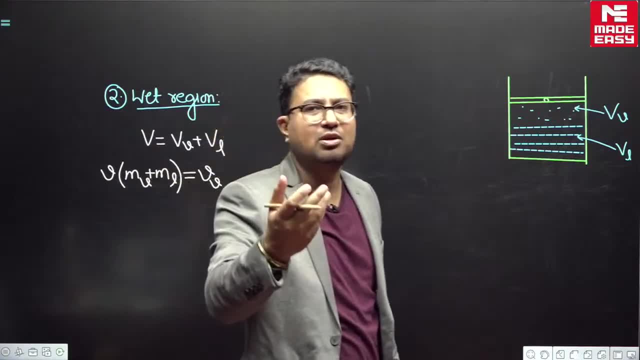 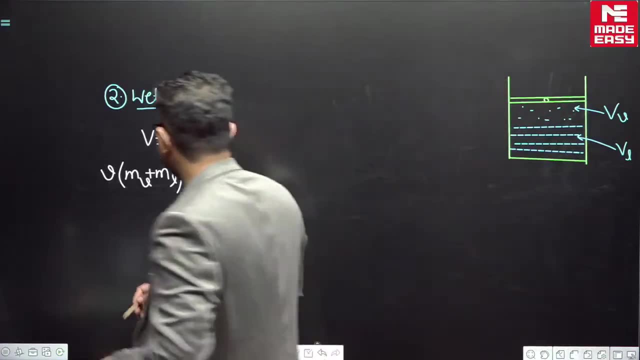 Unit mass of vapour. How much volume is there of 1 kg vapour? What is the volume of 1 kg vapour Into Into? What is the total mass of vapour Into Total? How much is the mass of vapour? 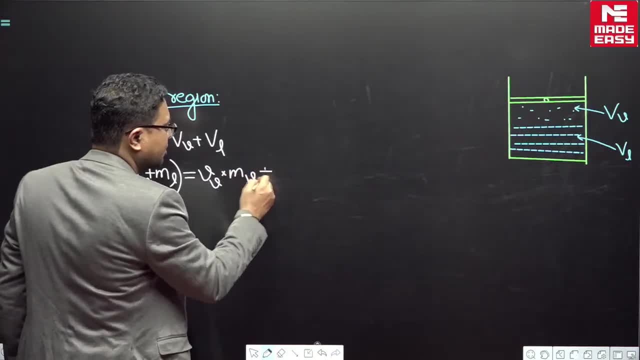 Into. What is the total mass of vapour? How much is the total mass of vapour? It will be this. This will be Plus, Plus Volume of liquid. What is the volume of liquid? So what is the volume of liquid? 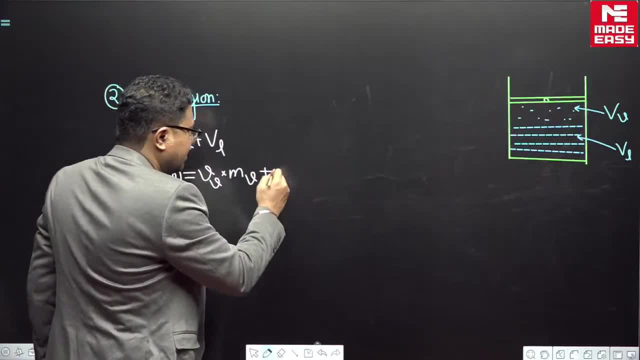 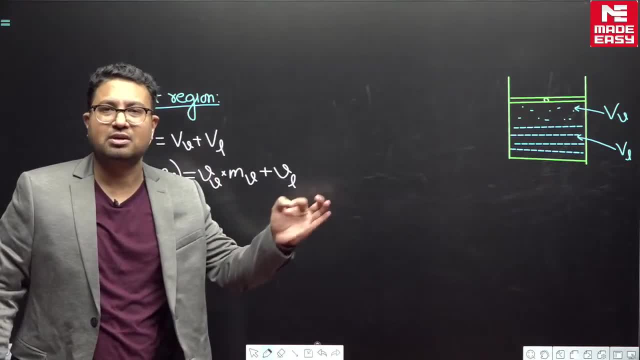 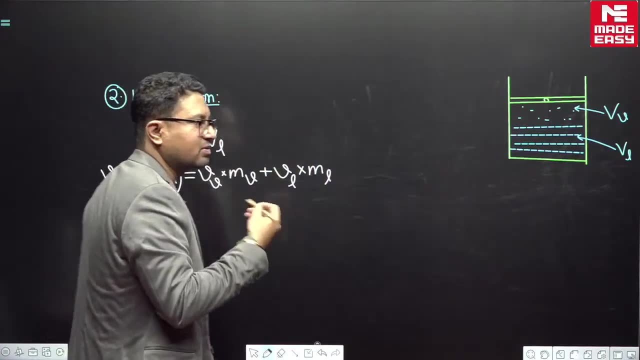 What is the volume of unit mass of liquid? What is the volume of unit mass of liquid? What is the volume of unit mass of liquid? unit mass of liquid, Unit mass of liquid volume will be into the mass of liquid, into mass of liquid. We can write like this: Now let me divide with this, So let me divide with. 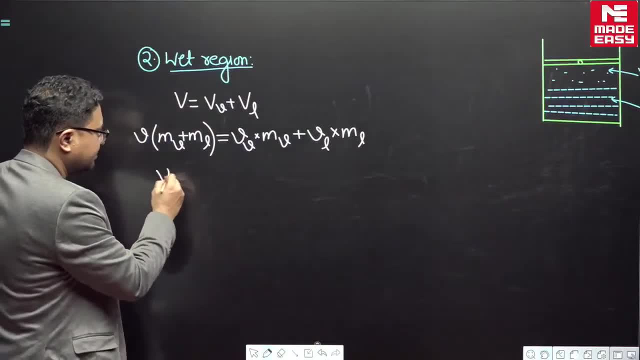 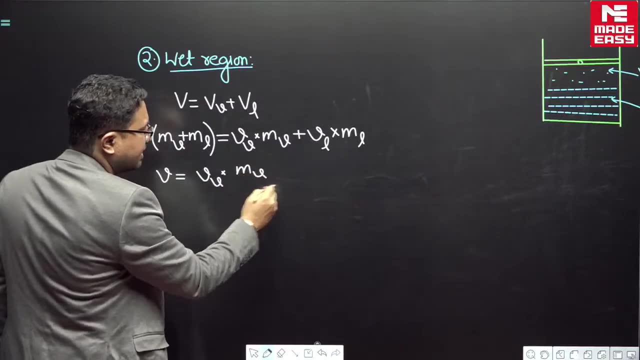 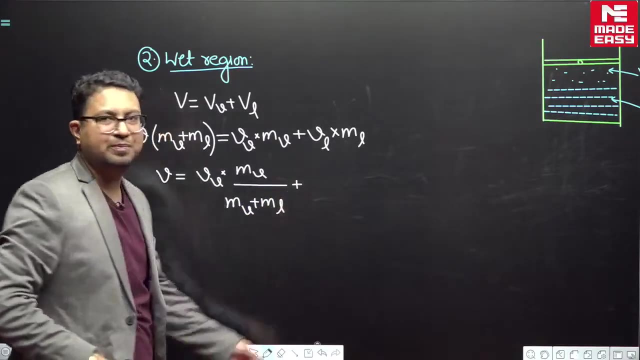 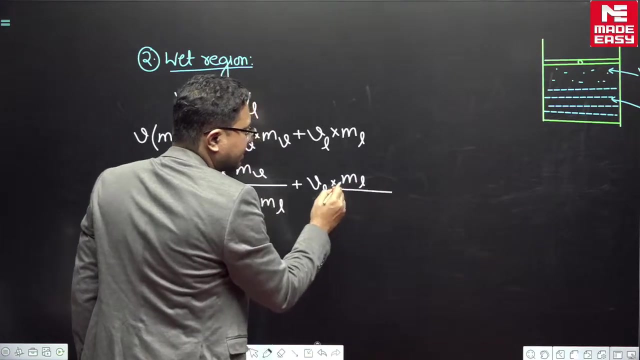 this, So average specific volume will be equal to. this will be equal to specific volume of vapor into M? v is the mass of vapor divided by divided by this: M v plus M L plus. This is the specific volume of liquid into mass of liquid divided by divided by M v plus M. 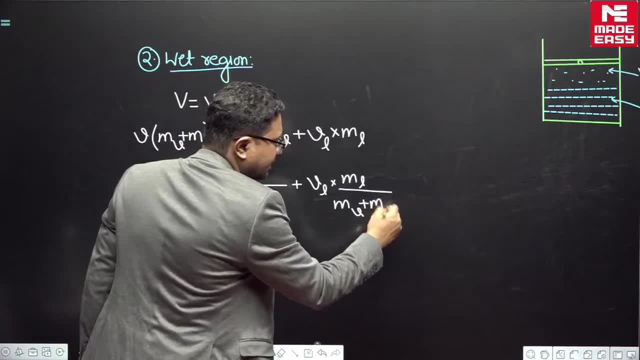 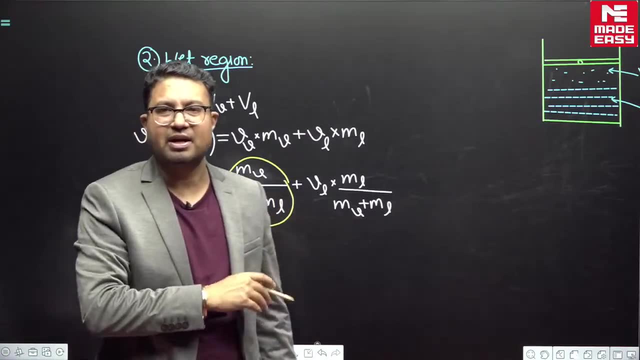 L, M v plus M L. If you see this, if you see this M v upon M v plus M L. just now, we defined. this is just in discussion. We have defined. it is what. What did we define? This is the dryness fraction. What is this? 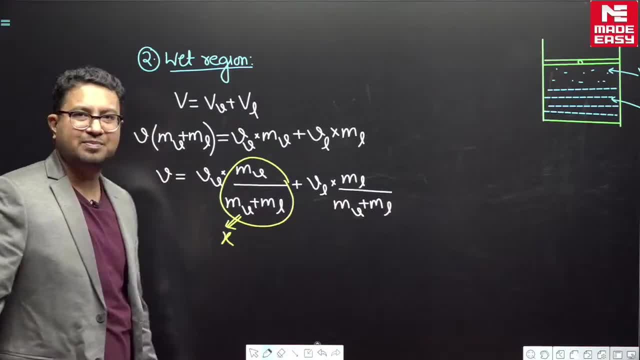 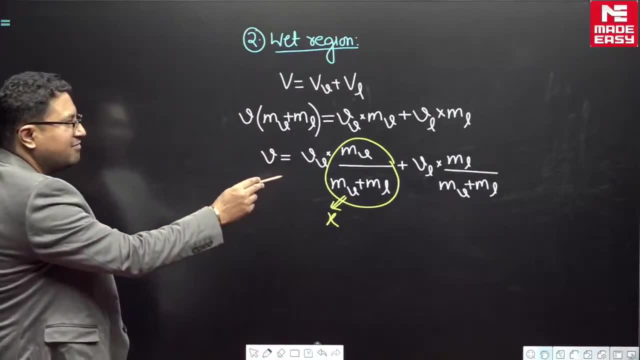 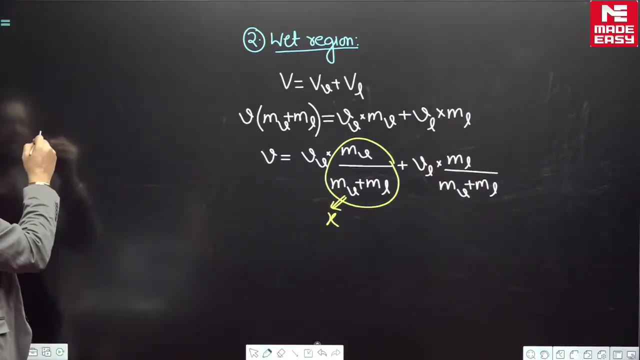 Dryness fraction. This is the dryness fraction x. Dryness fraction is x. If we see this, if you see this, then we can say this: M v plus M L. if we say this is x, if this is x, then what will be? 1 minus x. See So: 1 minus x is 1 minus M v upon M v plus M L plus M. 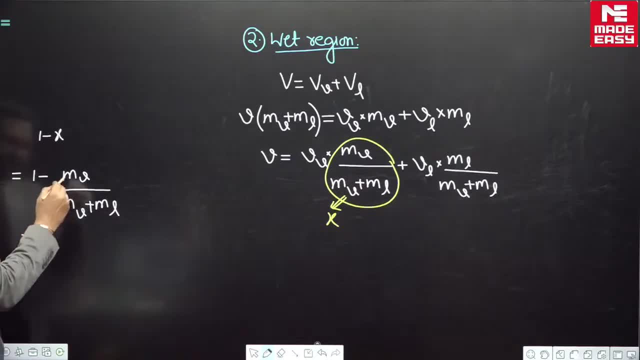 L, So M v plus M L will go here, minus M v. So we will have M L upon M v plus M L. We will have this. So this is actually 1 minus x. This is 1 minus x, So this is 1 minus. 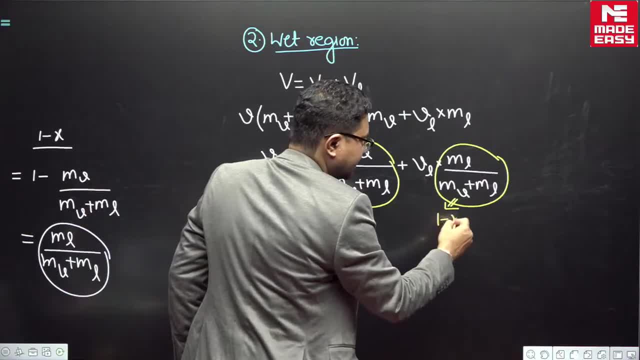 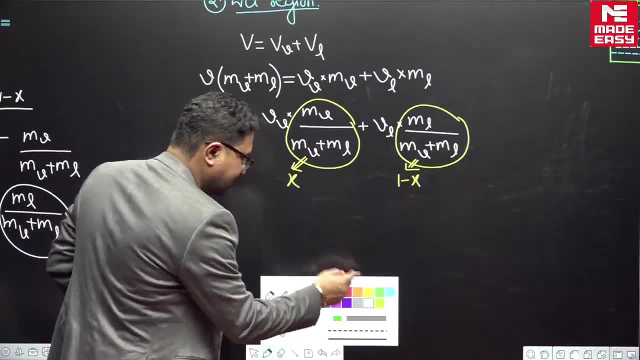 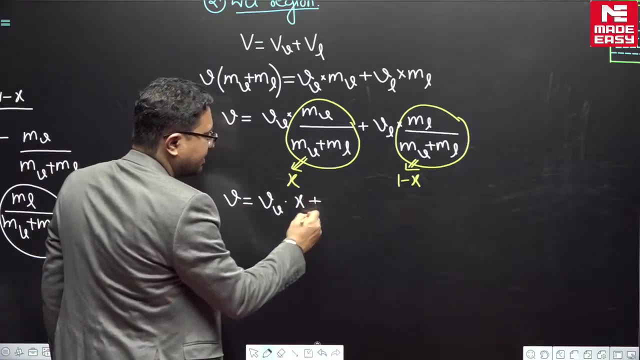 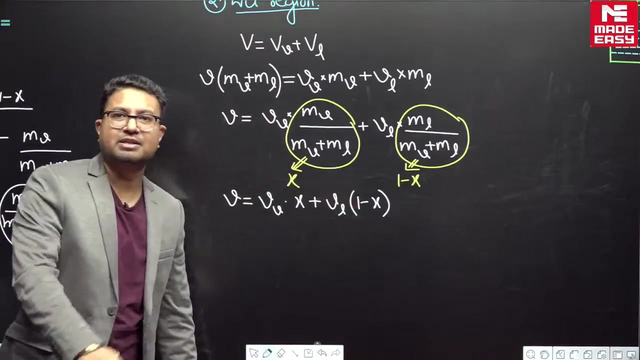 x. This is 1 minus x. Now, if we see this entire expression, if we see this, then we can simplify it. We can simplify it: Average specific volume will be equal to specific volume of vapor Into dryness fraction plus specific volume of liquid into 1 minus x. It will be this: 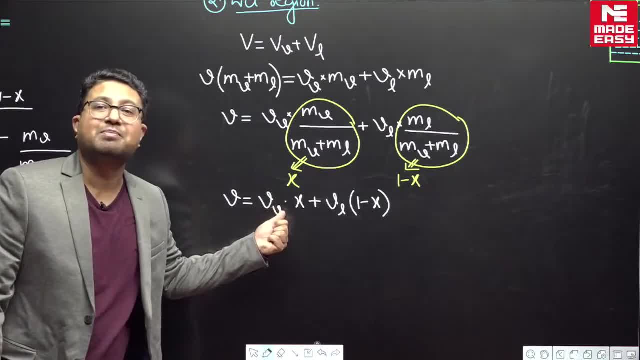 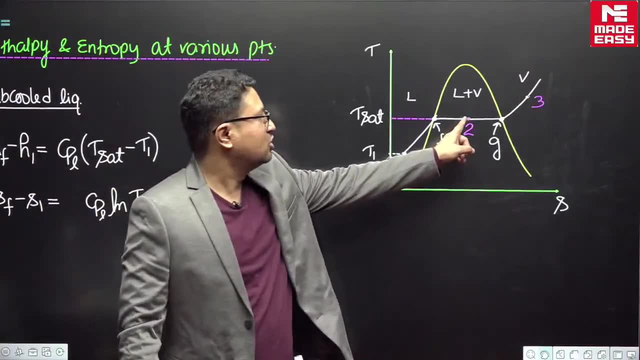 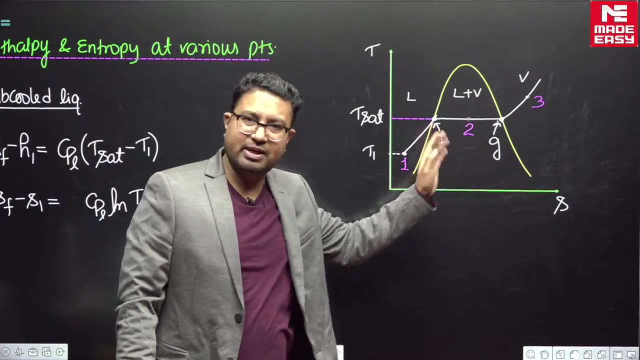 Now this specific volume of vapor. what type of vapor? it is Superheated, It is saturated vapor. We are talking about this condition, So the vapor is the saturated vapor and the liquid is the saturated liquid. Vapor is saturated vapor, Liquid is saturated liquid, So vapor. 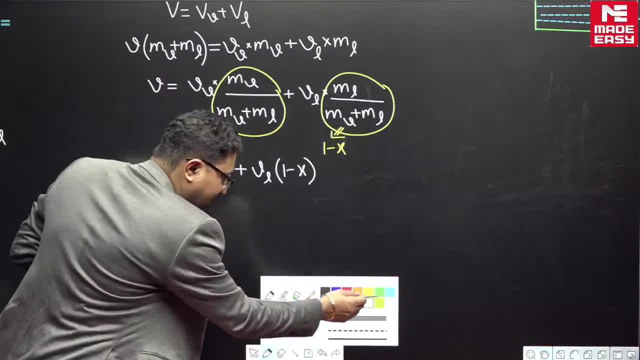 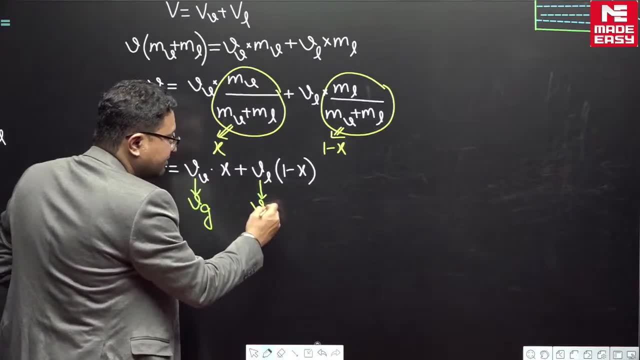 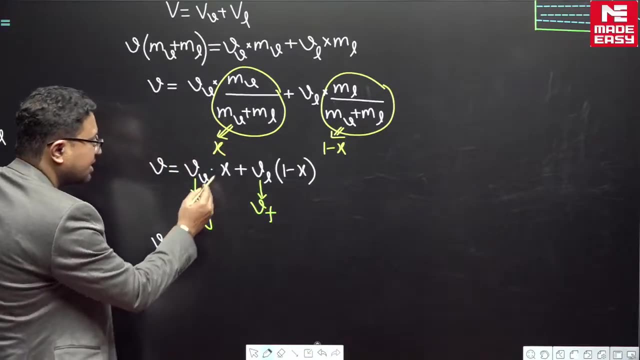 is the saturated vapor and liquid is the saturated liquid. So what we do, What we do, We write the specific volume of vapor as vg Liquid, specific volume. we write vf, We write vf, So we write, we write v is equals to x into vg, x into vg plus. 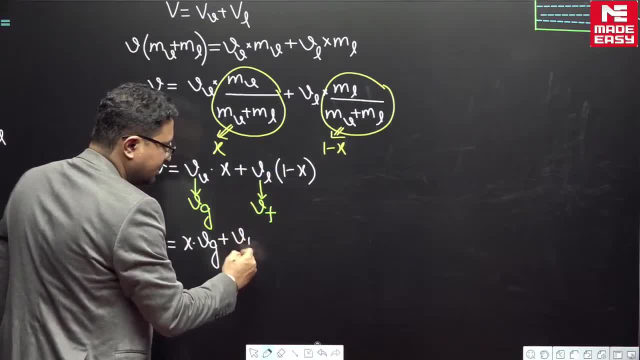 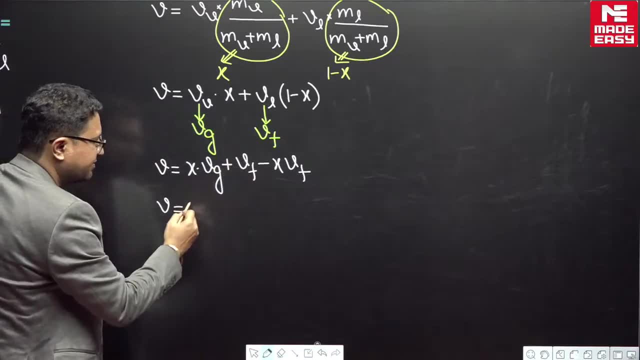 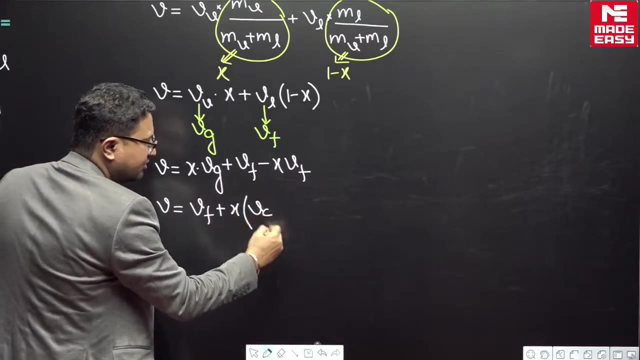 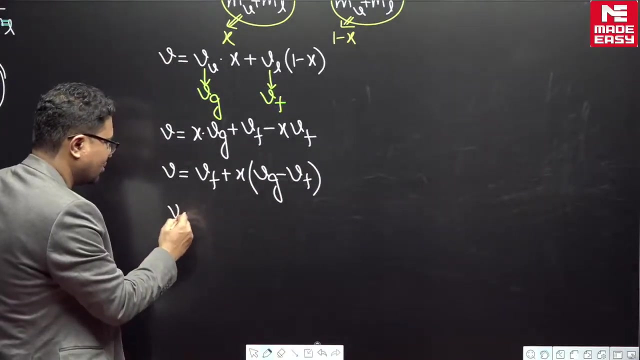 vf. So vf into 1 will be vf minus x into vf. This will come rearrange isko rearrange karo. V will be equal to V f plus x into V g minus V f. V g minus V f. So V g minus V f ko. we can also write generally: there is this notation we use So: 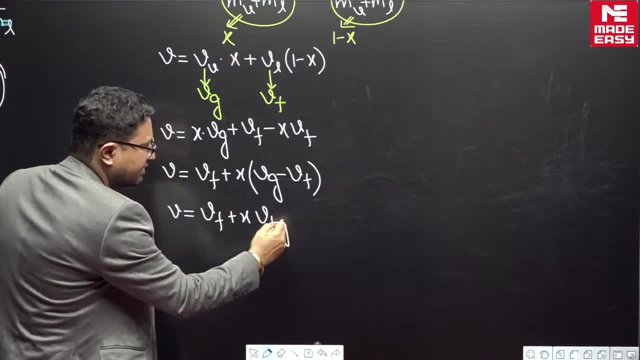 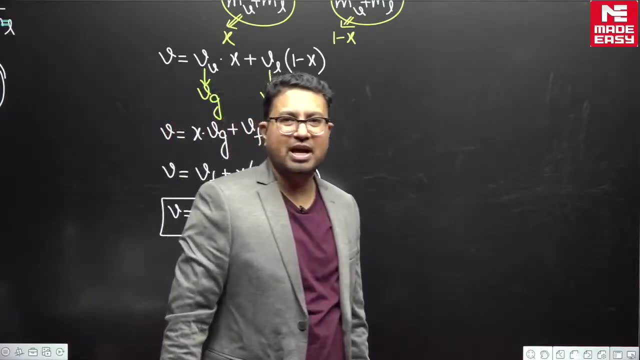 V f, plus we write it as x, V f g. V f g means difference of V g and V f. ye likh sakte. So this is how we develop formula. Aise, hum, formula develop karte You may have, many of you may. 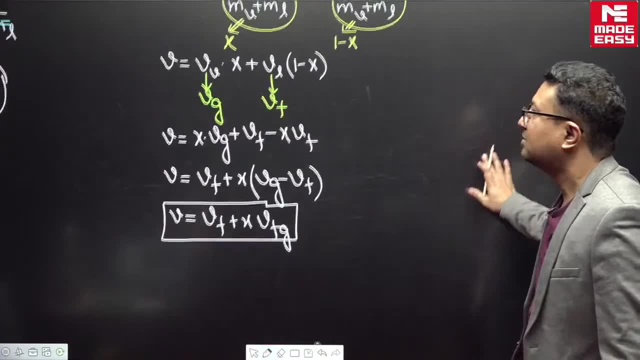 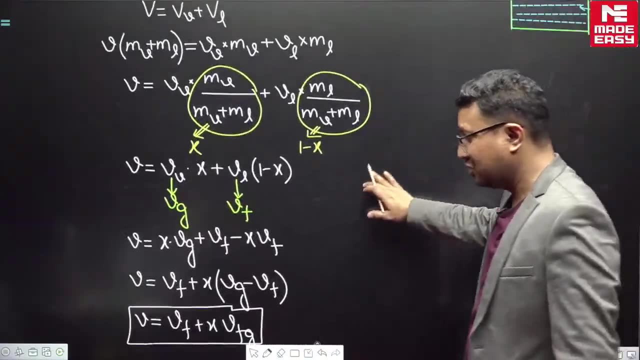 have directly seen this baho saare logo ne shah directly isko dekha ho, but we have derived it humne aaj derived kia isko. So you can understand how we derive different formulas. Now, in the same manner isi tarike, se we can say in the same manner: total volume is the. 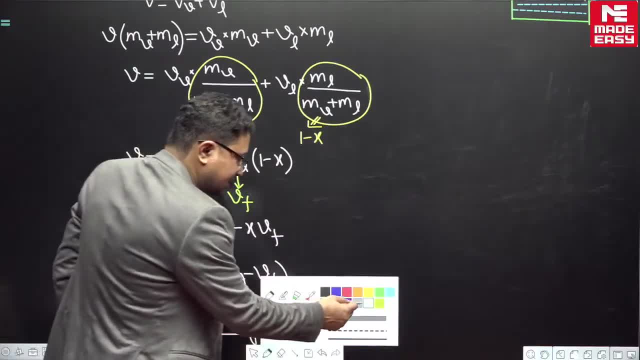 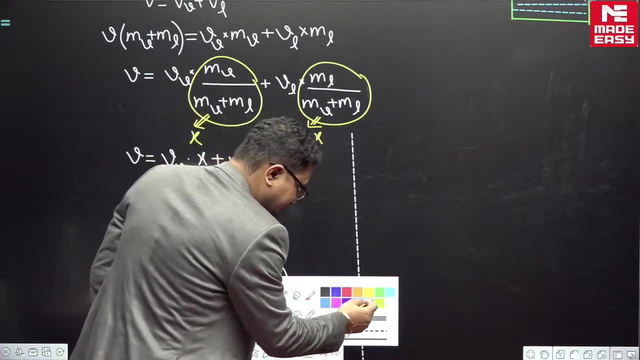 volume of liquid plus volume of vapor. In the same manner, we can say: same manner: me hum ye kai sakte hain dekho. in the same manner we can say: in the same manner, we can say that. that same manner, we can say that: 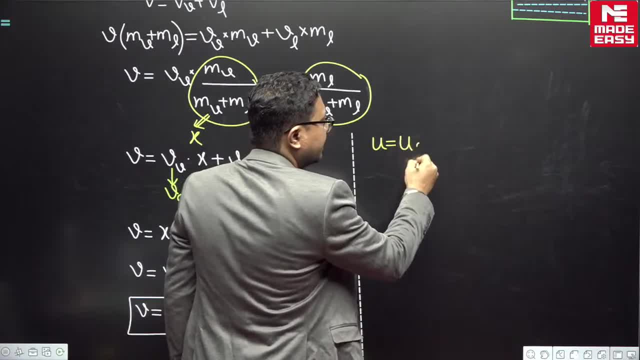 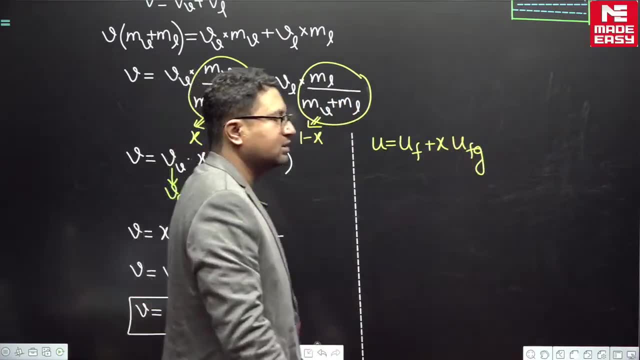 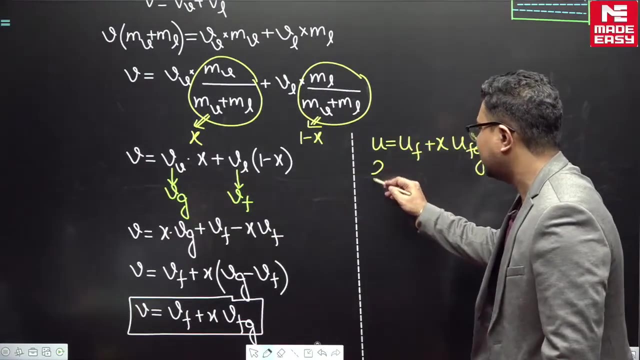 Average internal energy of the mixture will be equal to internal energy of the saturated liquid plus x into U f g plus x into U f g. Average internal energy is equals to internal energy of liquid plus x into U f g. Same manner me enthalpy: average enthalpy will be equal. 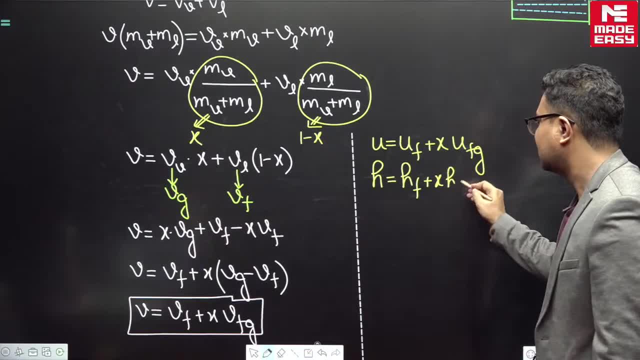 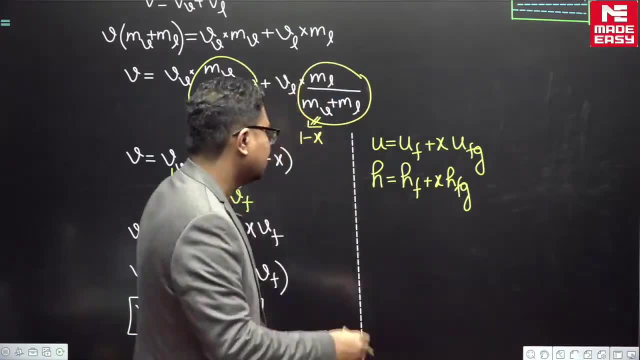 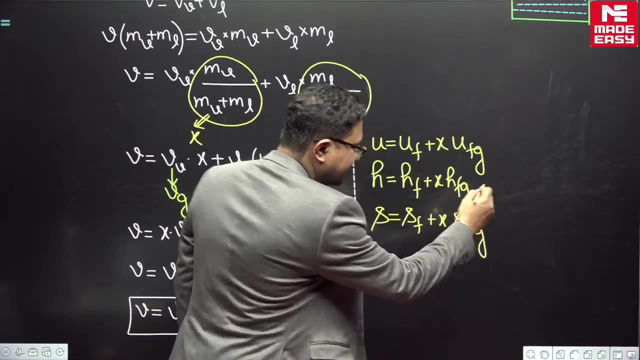 to h f plus x into h f g. Kyo total enthalpy: ko add kar sakte na Enthalpy. total enthalpy is enthalpy of liquid plus enthalpy of vapor. add kar sakte na entropy. S is equals to S f plus x, S f g. We can write like this, But we cannot write. 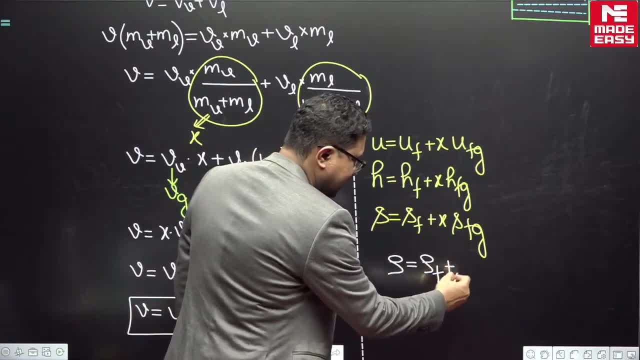 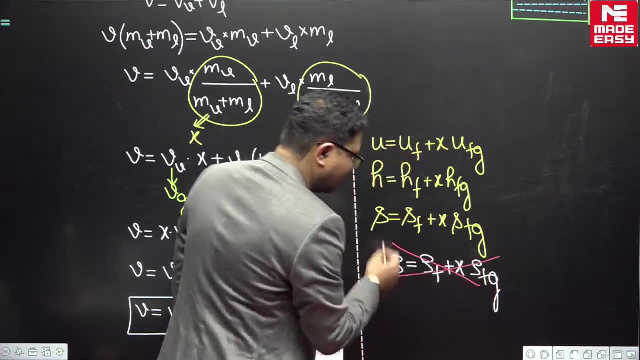 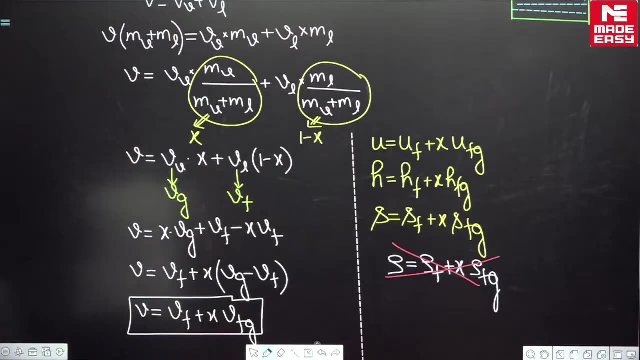 rho is equals to rho f plus x, rho f- g. We cannot write this. Just tell me why we cannot write this, why we cannot write this reply. I am just waiting for your replies: why we cannot write this, why we cannot write this, why we cannot write this vector. 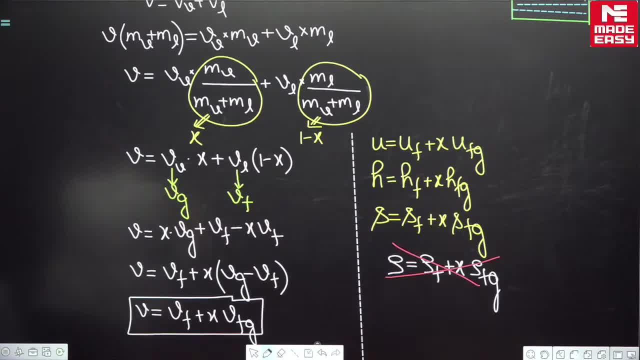 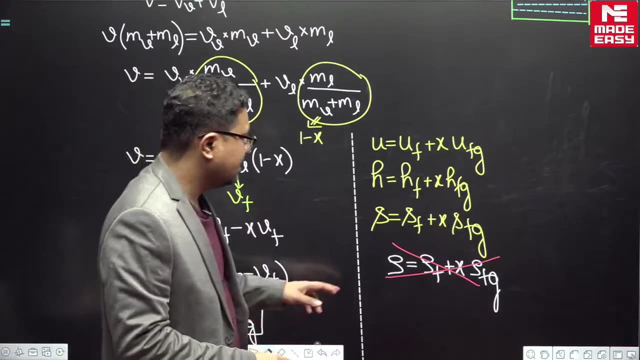 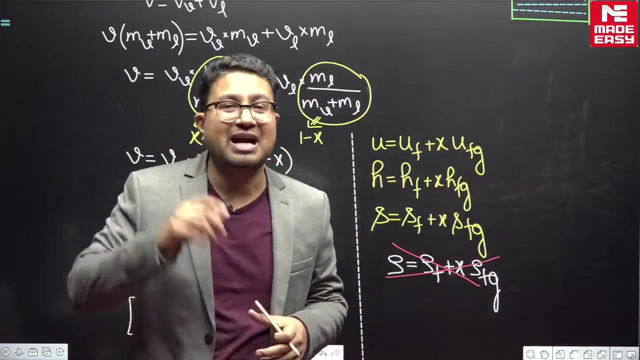 0 rho is inverse of specific volume. you are correct. you are correct. why we cannot write this? Just understand this. you cannot find the density of the mixture by adding the density of the liquid and the density of vapour by mixture: ki density. Liquid plus vapour, ki density. 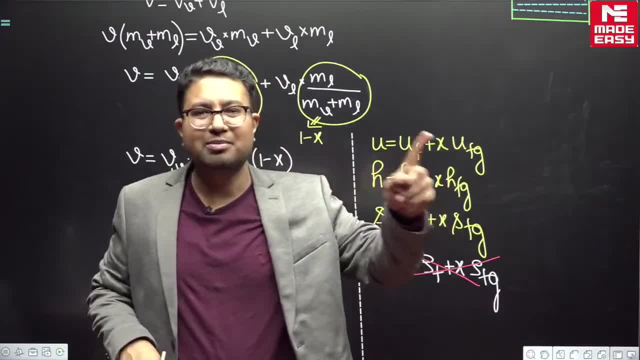 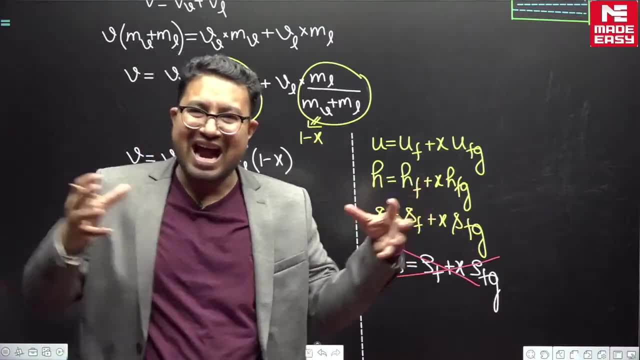 Add karke thodi milegi volume. totally you can get like this. total volume mil sakta hai. the total volume is the volume of the liquid plus the volume of the vapour. you can get like this. But you cannot add the density of the liquid plus the density of the vapour to get the 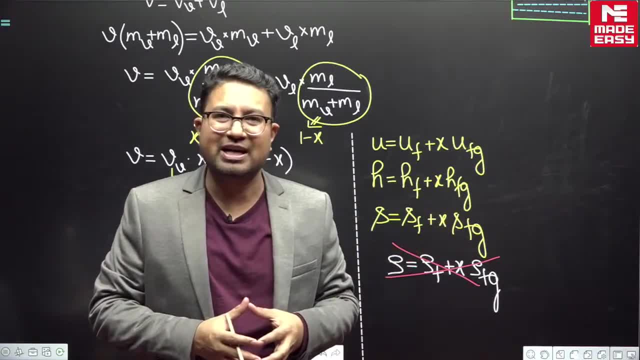 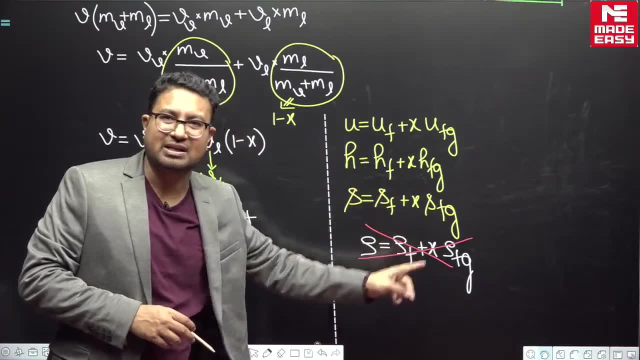 total density. total density as a ni milti aapko. you cannot get it like that. So the density is equals to density of liquid plus x. into this, ye galat hai, how we can, if we have to find out the density, how we can find out. 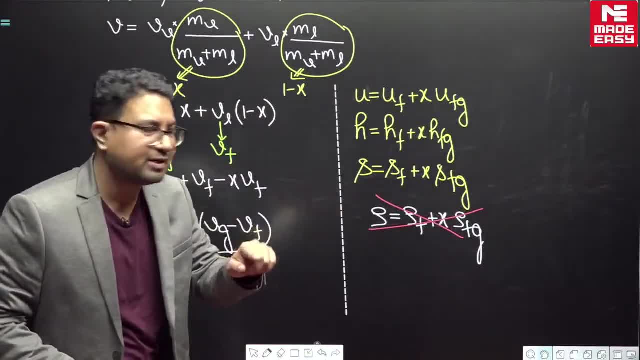 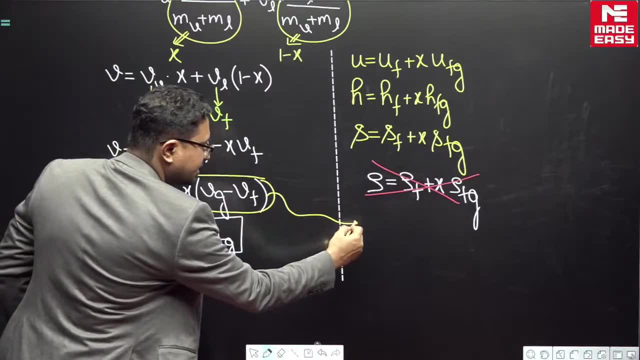 We can say: density is the inverse of specific volume. right, so density is specific volume ka inverse hai. Dekho, we have already written this, ye likha hai humne, So let me write this isko likhte. let me write this: average specific volume, average specific. 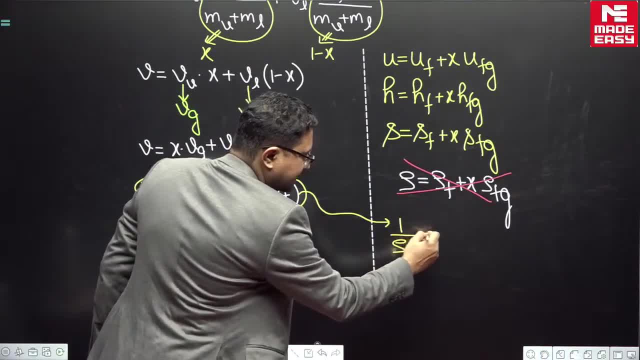 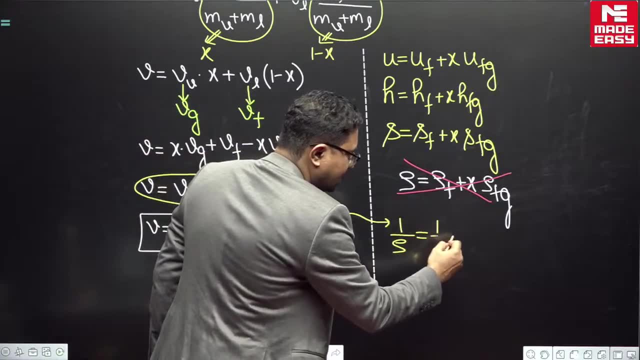 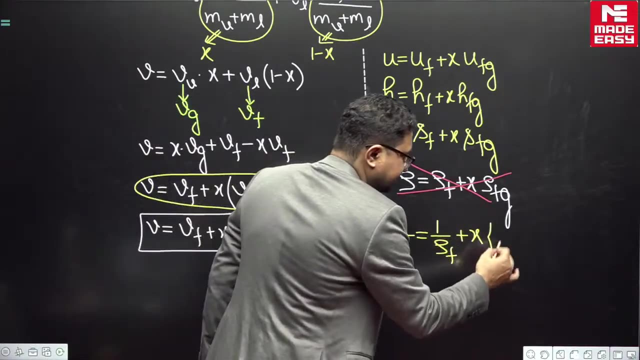 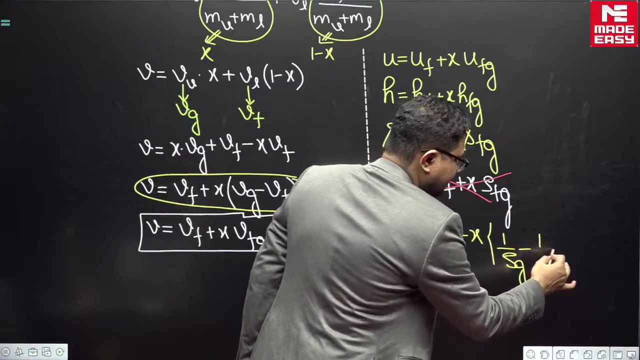 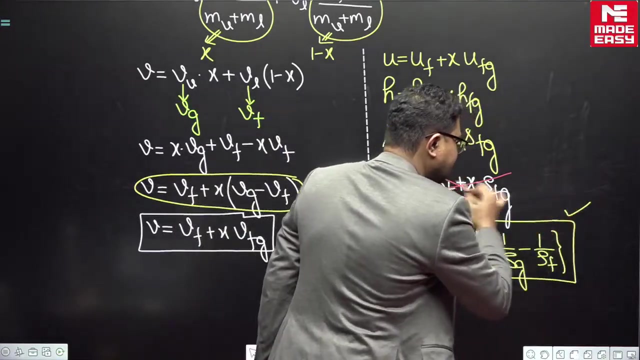 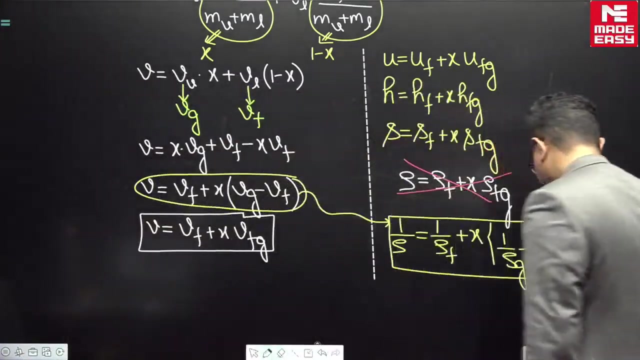 volume is equals to 1 upon density. average specific volume is equals to 1 upon density. From thereat we get as much as 0.3 k or 0.2 k. it is phase which is the. the umi is 3,2, so 3.1. about the sub cooled liquid and the 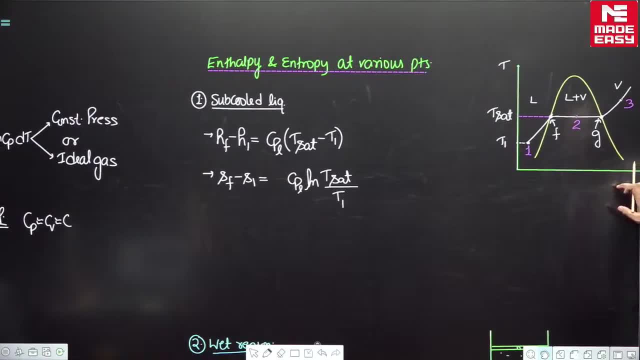 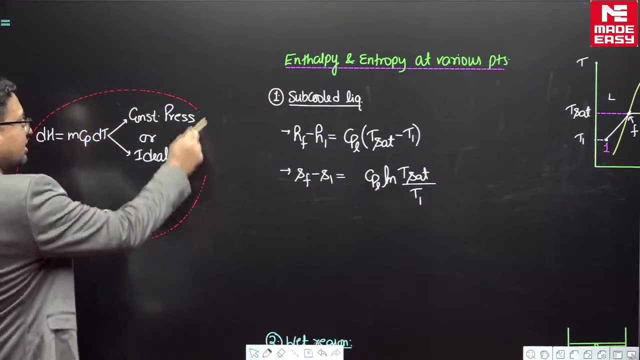 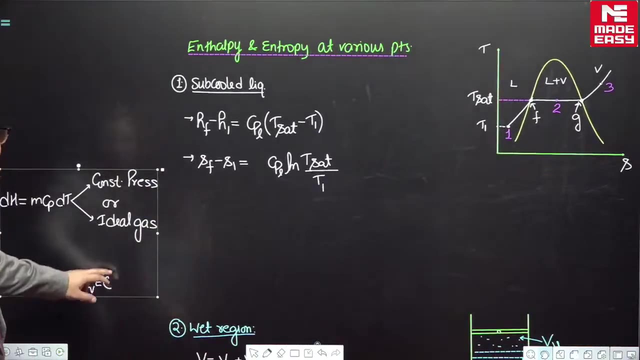 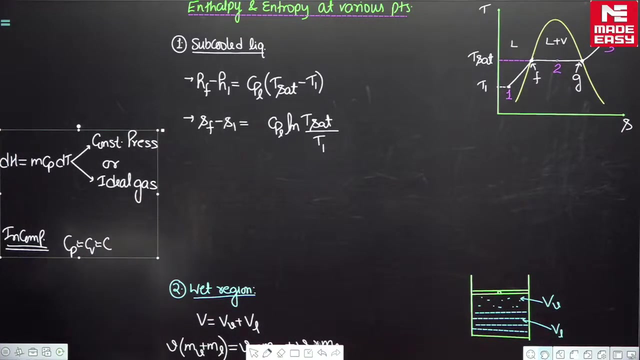 wet region. just if you want to take a screenshot or something you can do like, do it here, you can just take it. i will move on, but let us talk about the superheated region and then we will solve few questions. we will solve few questions, just take the screenshot. 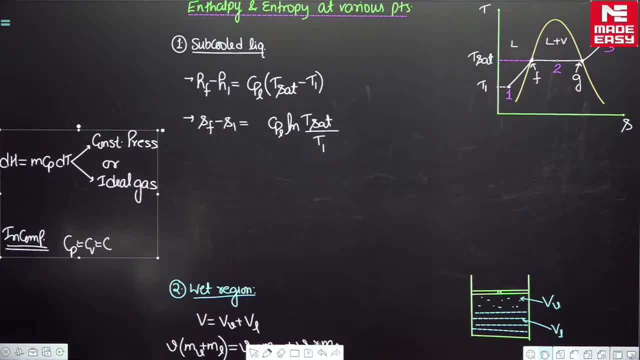 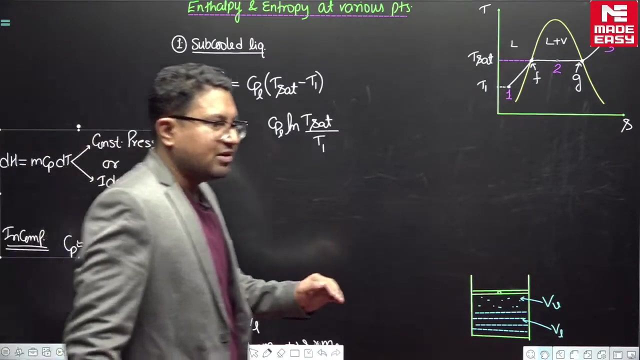 Ankit Raghuvanshi, you have. whatever you have said is also correct: that specific volume is reciprocal of density. yes, specific volume is reciprocal of density, correct? this is correct. this is correct. fine, now, now see. see here further. we discussed, we discussed, we talked about the wet region, wet region. 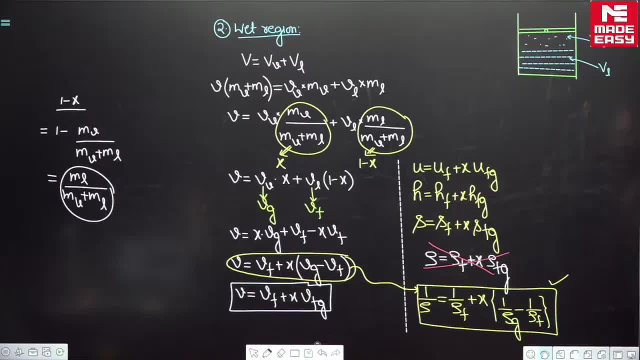 so so this is the discussion we have done up to now. we have discussed. so see, we are developing the expressions, we are developing the formula and, as we are developing the expressions, we are discussing basics. we are discussing all the things while developing so that when we are solving the questions, when we solve the questions, we are very comfortable, we are very 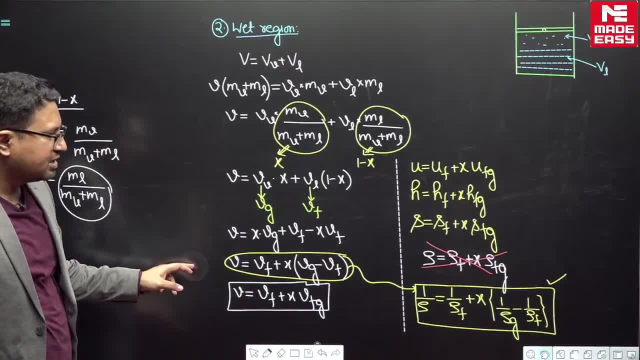 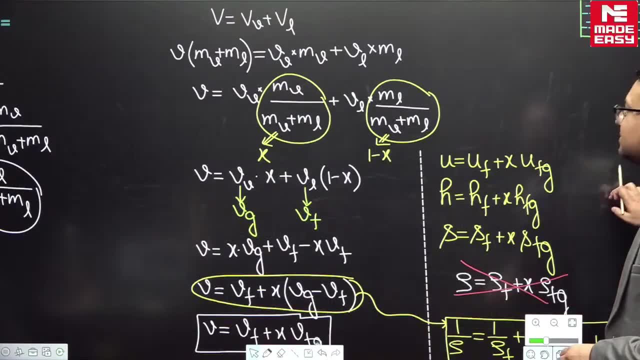 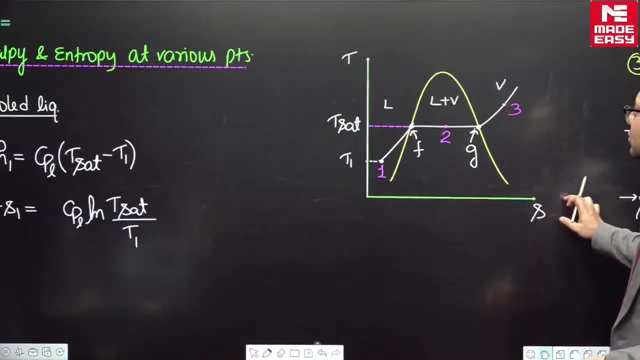 comfortable in question solving. ok, so here, now, now, let us see. now we will see. see now, let us see this: the wet region, wet region. there is something very important: formulae RAC may be used. there are important expressions RAC may be used. if you see, if you see from: 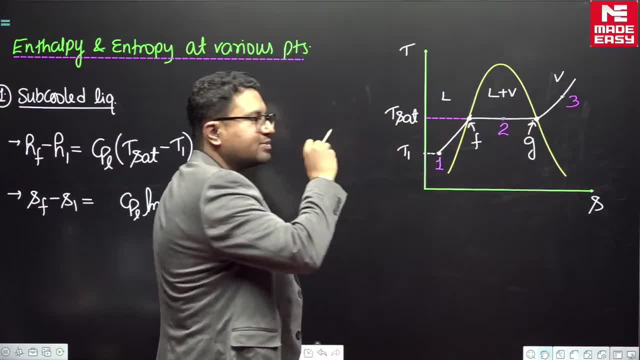 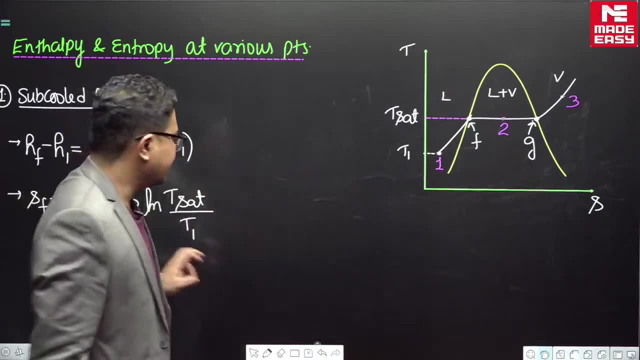 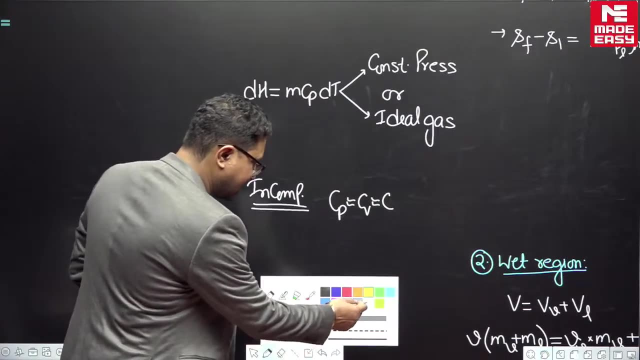 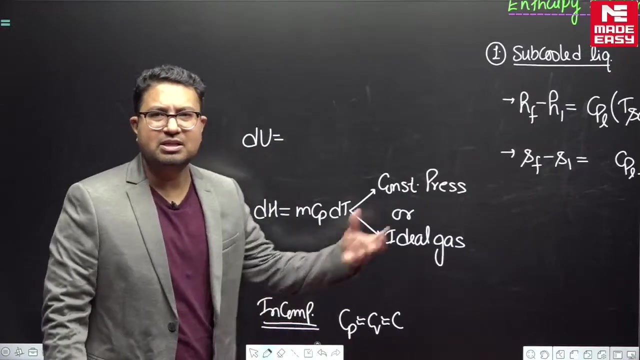 here to here. there are two important expressions which I will write, two important expressions. so heat supplied, like here on the side I am writing, which is different. there is some different discussion apart from the discussion which we are doing like DU. we have written DH, we can write DU also, even though we are not discussing it now, but just because we have written DH. 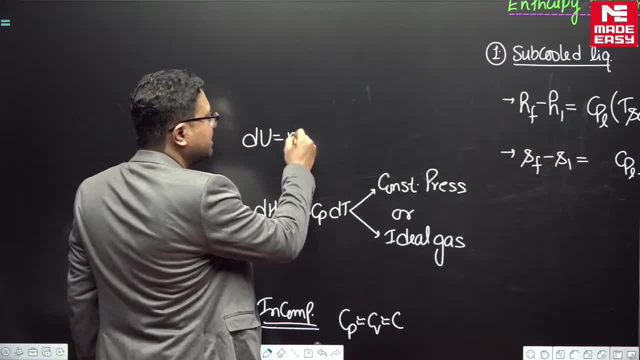 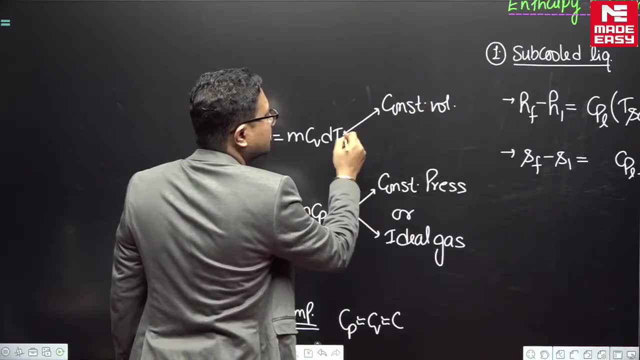 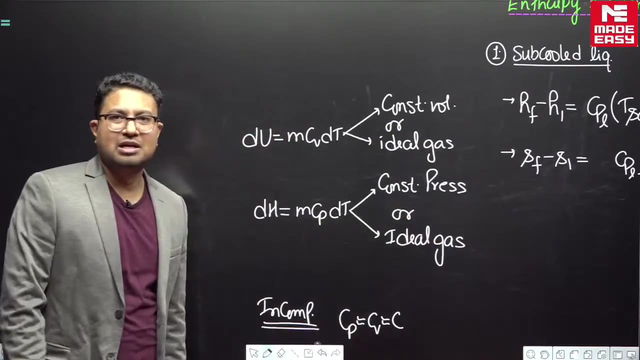 we have written DH, so I will write DU also. DU can be written as MCVDT. under what condition? under which condition it can be written? constant volume. we can write it under constant volume. or or what ideal gas or ideal gas constant volume ho ya, ideal gas ho. we can write this: 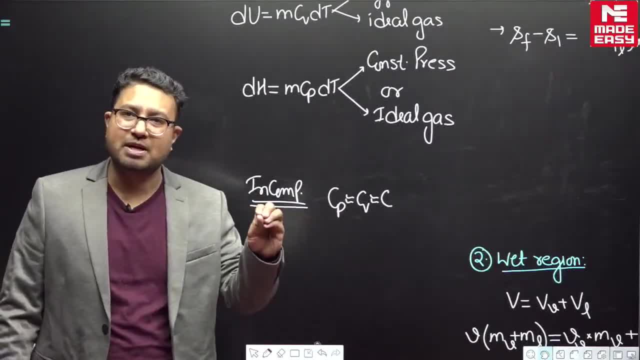 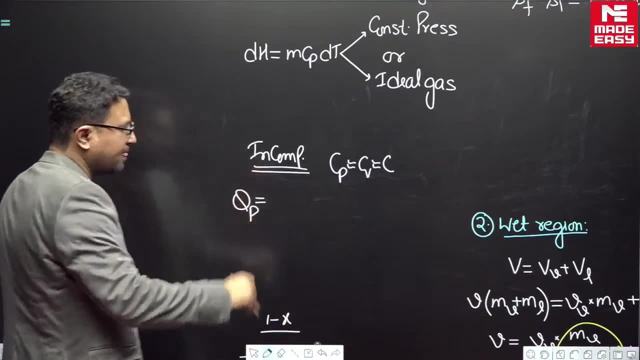 abab dekho. whenever heat is supplied at constant pressure is baat ka use aane wala hai. when we will solve the questions. whenever the heat is supplied to constant pressure, jabhi heat constant pressure pe supply hoti. whenever the heat is supplied at constant pressure. 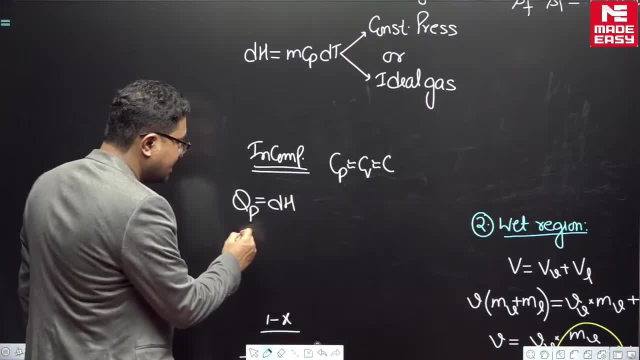 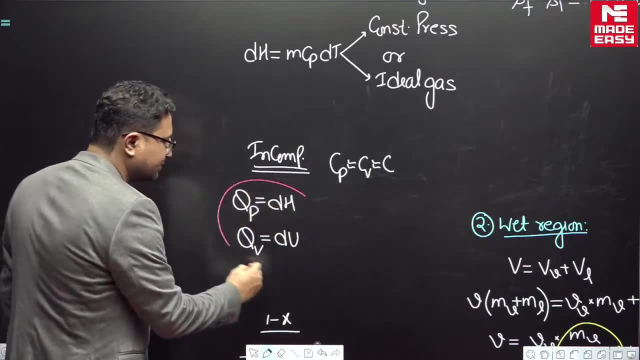 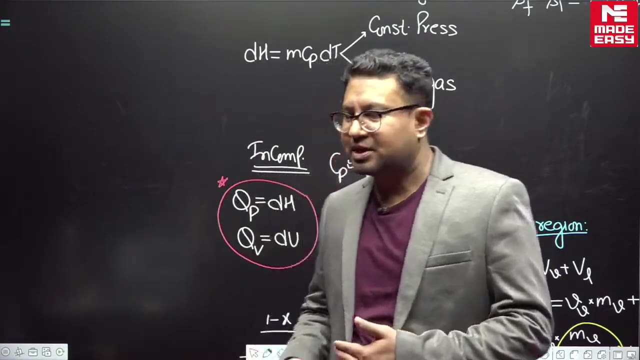 it can be written as enthalpy change. enthalpy change: likh sakte. whenever the heat is supplied at constant volume, We can write this it as internal energy change. This is an important thing. We should remember this. We should remember this When the liquid is changed into vapour, when the liquid is changing into 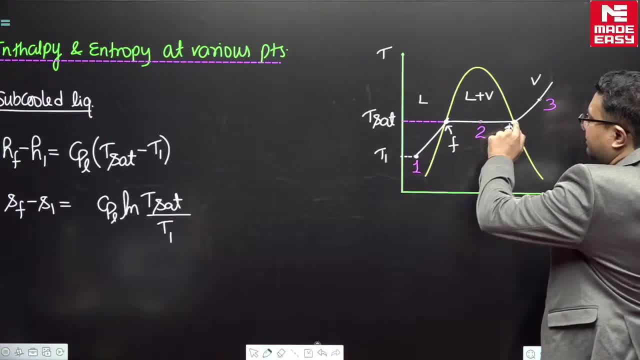 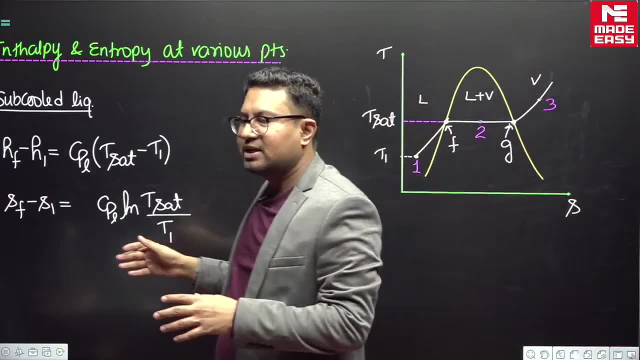 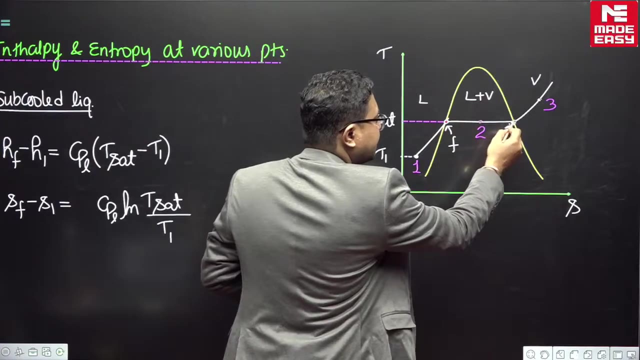 vapour. when the saturated liquid is changing into saturated vapour from here to here, pressure is constant. You see, saturated liquid is changing to saturated vapour. The pressure is constant, Pressure is constant. So saturated liquid is changing to saturated vapour. Pressure. 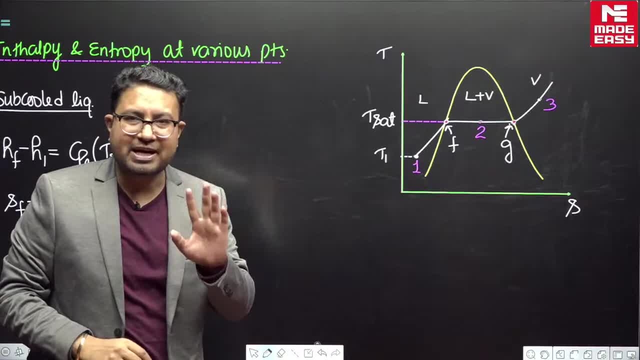 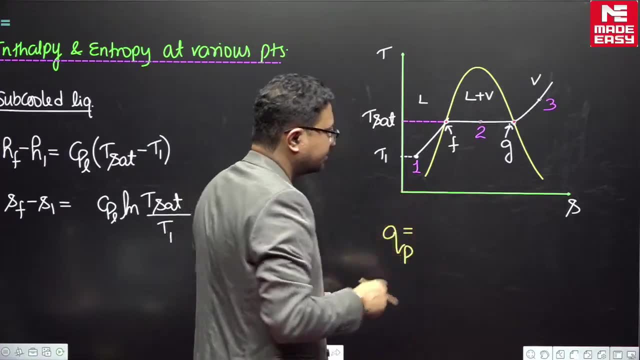 is constant, Pressure is constant, So heat is being supplied at constant pressure. Yes, Yes, So heat supplied at constant pressure is what Heat supplied at constant pressure can be written as enthalpy change. Just now I told you Heat supplied at constant pressure. 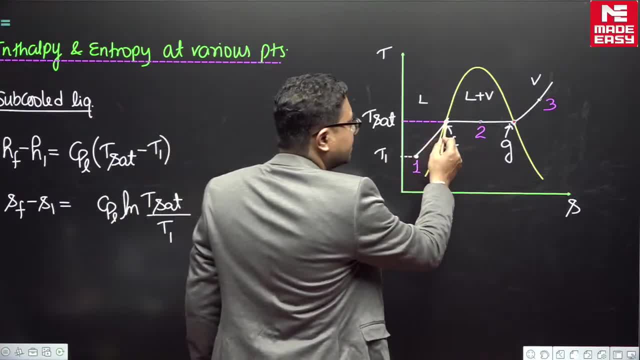 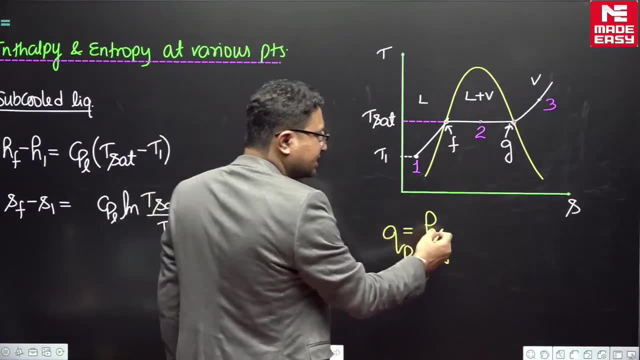 can be written as enthalpy change. So from here to here, here to here, the heat supply will be Hg. What will be the enthalpy change? Heat supplied constant pressure is enthalpy change: Hg minus hf. 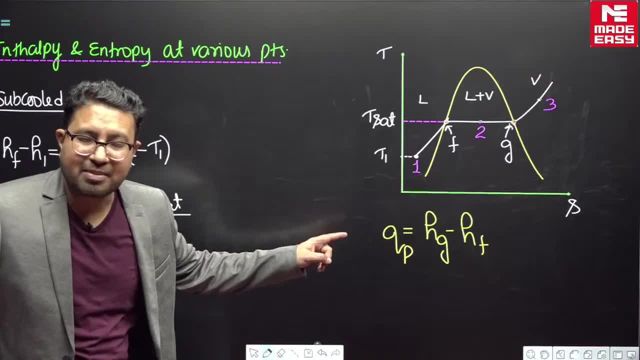 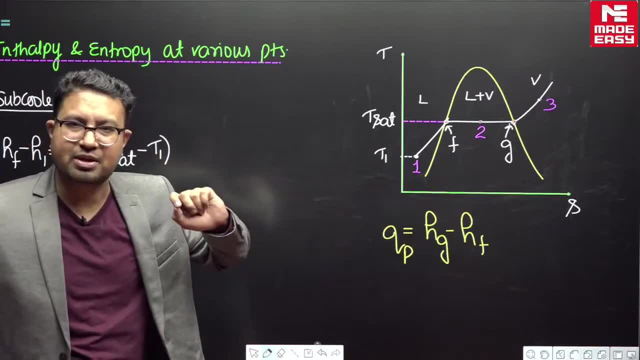 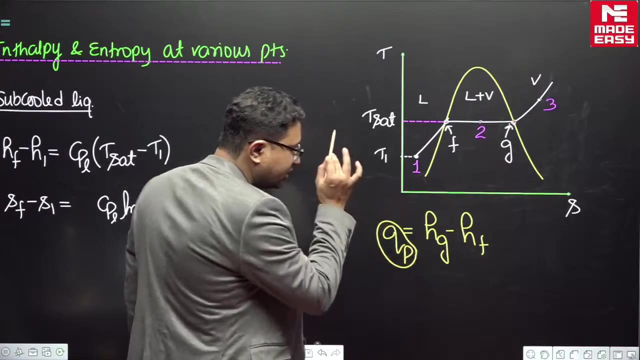 This is the enthalpy change. Why I am writing enthalpy change? Because heat is supplied at constant Pressure. constant From liquid to vapor conversion Pressure remain constant. Then we can say The heat which has been supplied Is used during the phase change. 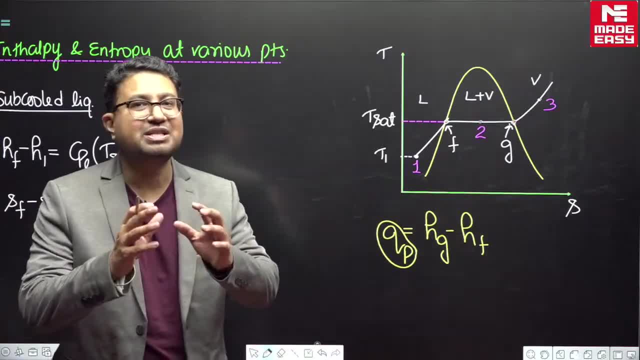 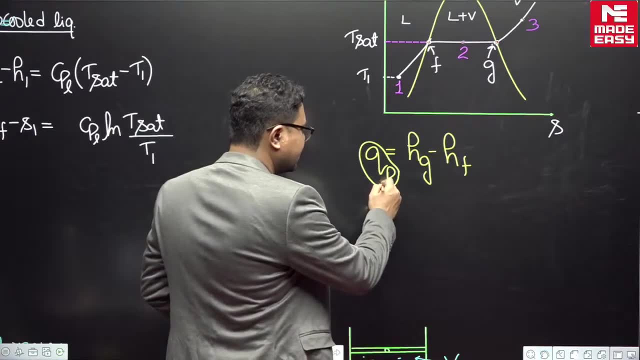 Is used for the phase change. Heat which is supplied Is used for the phase change, So that can be called as latent heat. What can we call it? Latent heat? We can call this as latent heat. We can call this as latent heat. 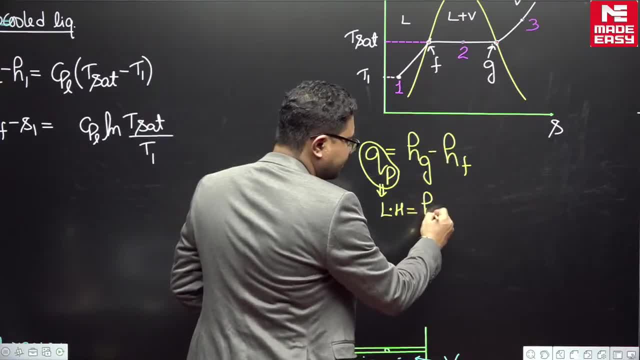 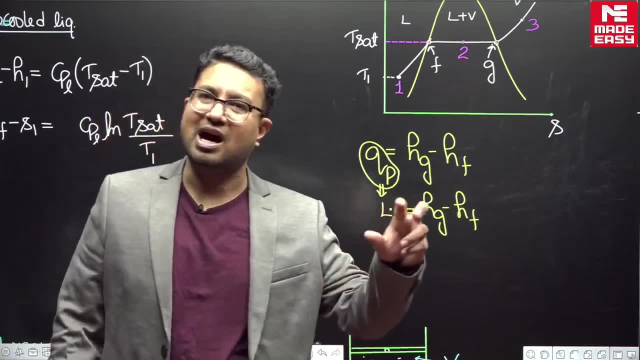 So latent heat can also be written as Hg minus hf, Or hfg we can also call it, So this is one expression which is used. This expression Is used in REC frequently, So this is one of the expression Which is frequently used in refrigeration. 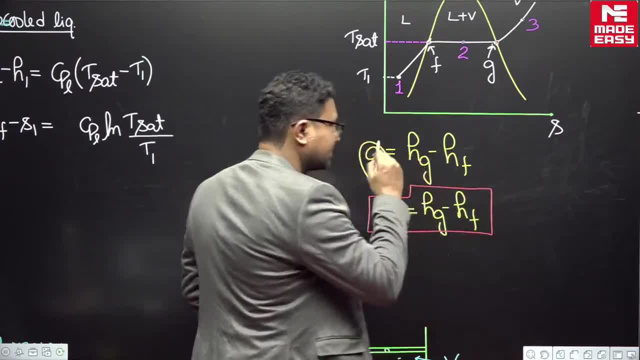 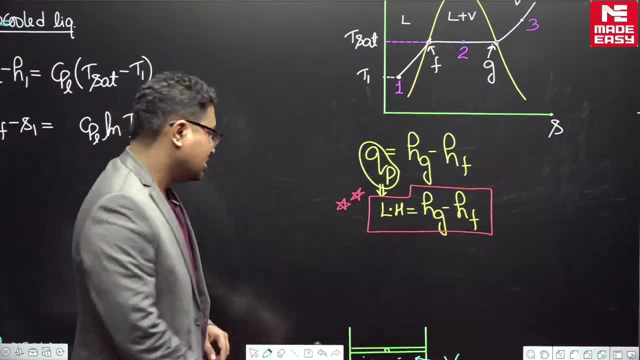 And air conditioning. REC is used in this expression. So this is important. This is how we get it. This is how we get it Then, If we want to write the entropy change, If we want to write the entropy change, So, if we want to write the entropy change, 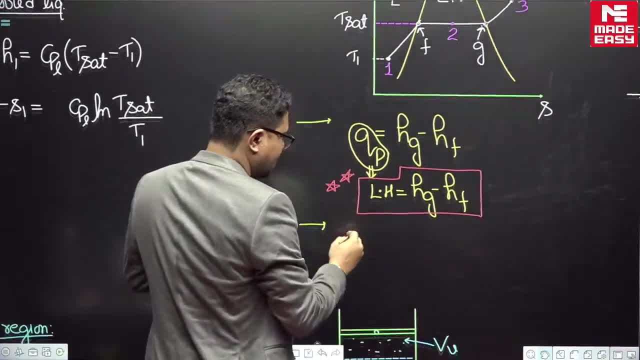 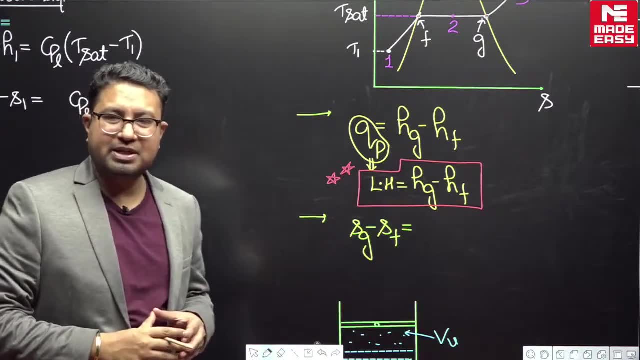 From here to here. If we want to write the entropy change, Sg minus sf, Sg minus sf- Entropy change. if we have to write So, entropy change is heat supplied upon temperature, But the temperature is constant, Temperature is constant. 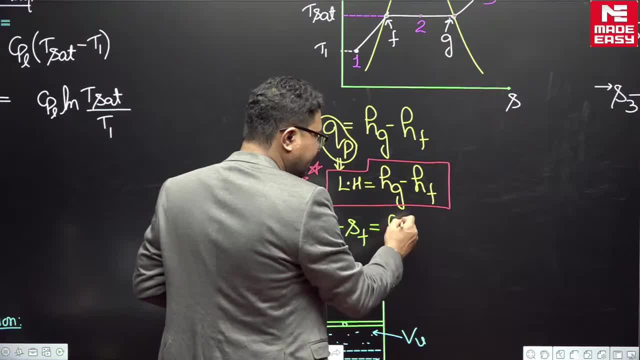 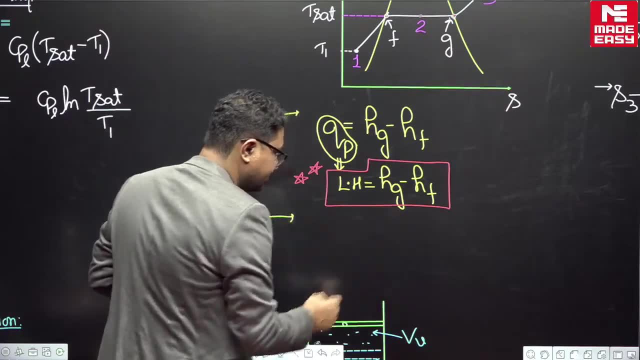 Entropy change is the heat supplied. Del Q by T. D S is equals to Del Q by T. This is D S. Let me write it like this: D S is equals to D S is equals to Del Q by T. Del Q by T. 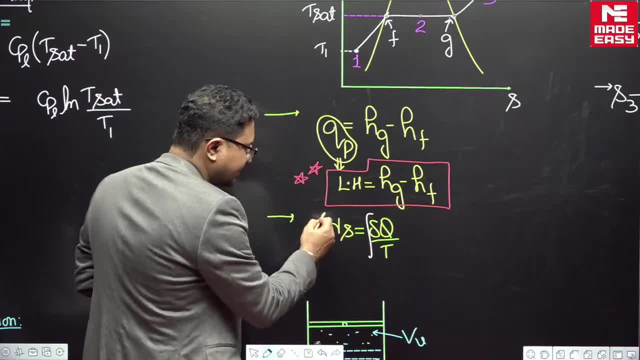 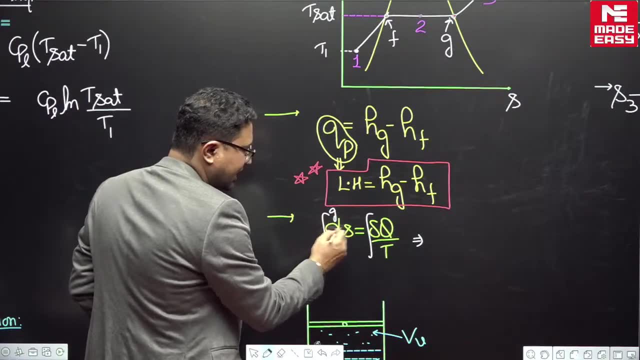 Let us integrate this for the phase change condition, For the phase change. If we integrate this, then what will we get? This is the phase change: Liquid: Saturated liquid versus saturated vapor. S G minus S F. We will get S G saturated vapor. 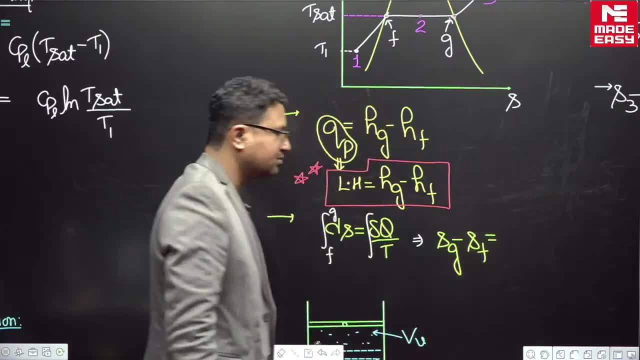 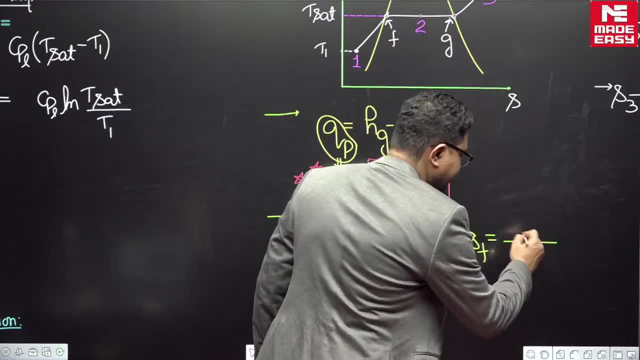 minus saturated liquid entropy. It is equal to. It is equal. Temperature is constant. It will come out of the integration sign. It will come out of the integration sign. What is this? Heat supplied at constant pressure. Heat supplied at constant pressure. 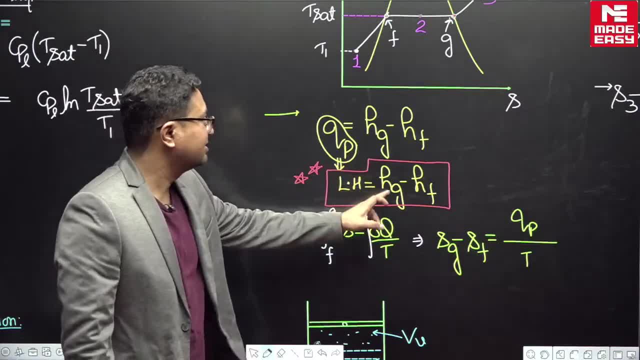 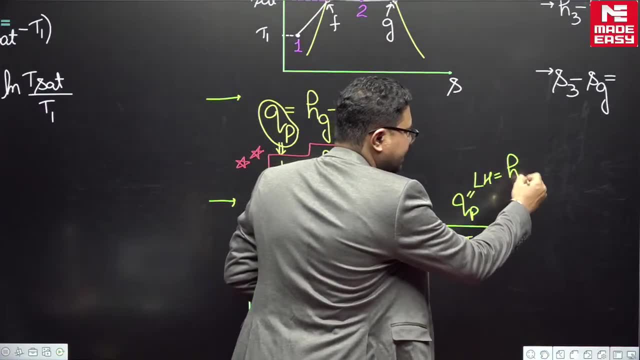 Now, heat supplied at constant pressure is what Enthalpy change or latent heat. We can write both, So this can be written as this can be written as latent heat, or this can also be written as H F- G, that is H G minus H F. 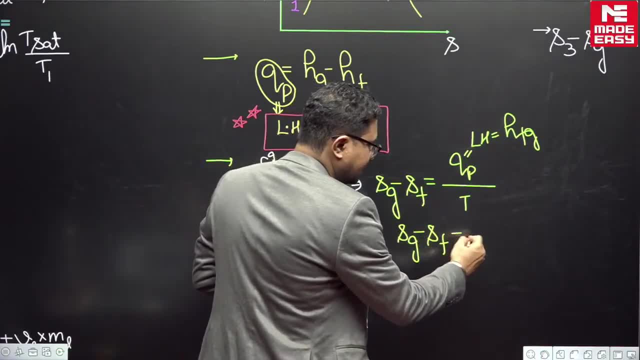 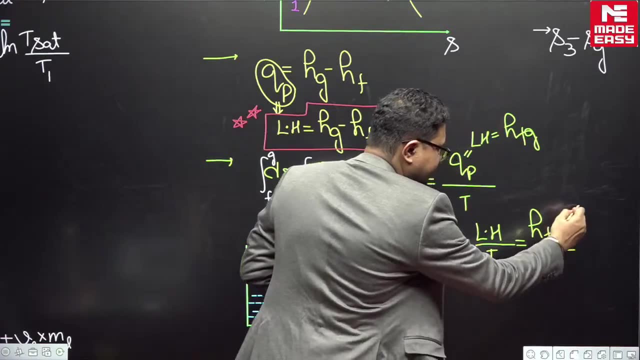 So we can write: S G minus S F is equals to latent heat upon temperature. or this can be written as H F G upon temperature, because latent heat is: this is the temperature of phase change. This is the temperature of phase change. This is the temperature of saturation. 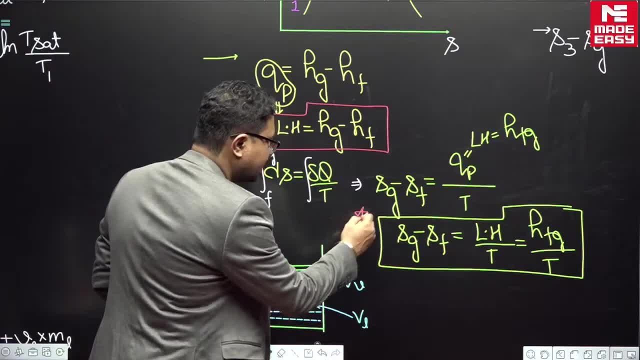 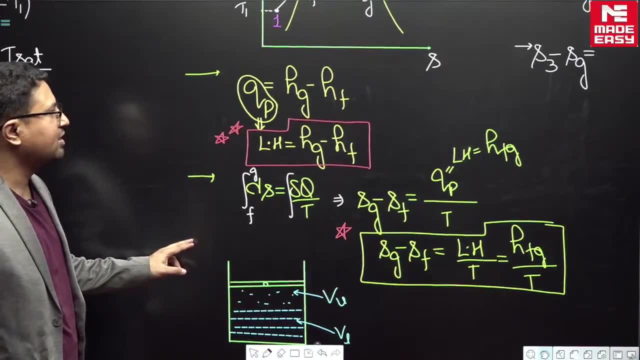 So this is also important, This is also important for us, This is also important, Important. So we will develop one more expression for the superheated region and then we will move on to the questions. Then we will see the questions. 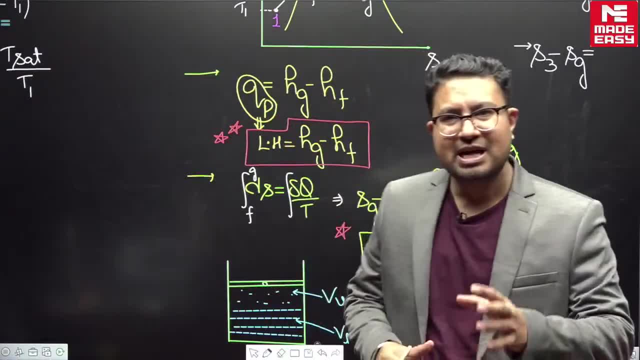 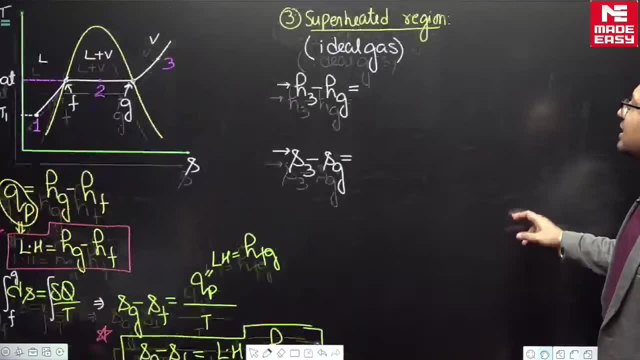 Look, Let us talk about the superheated region And then let us see the problems based on this. So we have discussed the details And now we can comfortably move to the questions In the superheated region. suppose you are here? 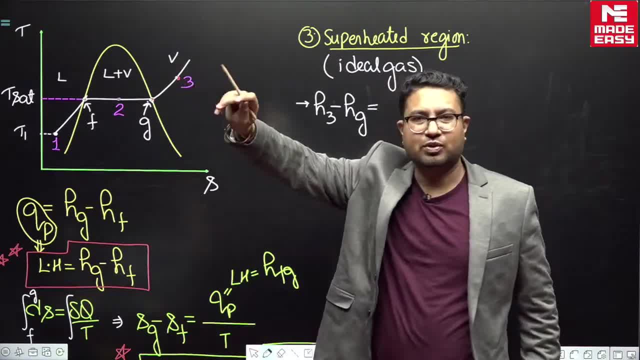 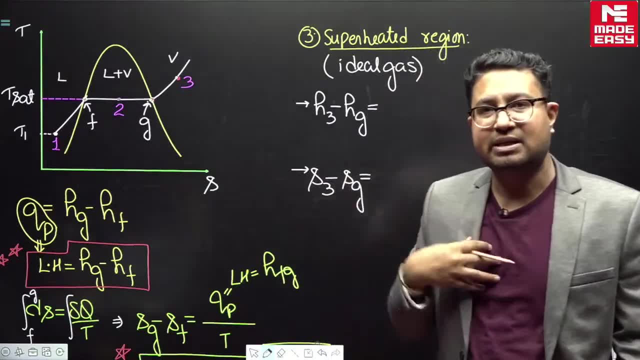 You are here In the superheated region. suppose, Suppose for the superheated region, you are in the vapour phase. So in the superheated region. whenever we need, whenever we need, we assume ideal gas behaviour. 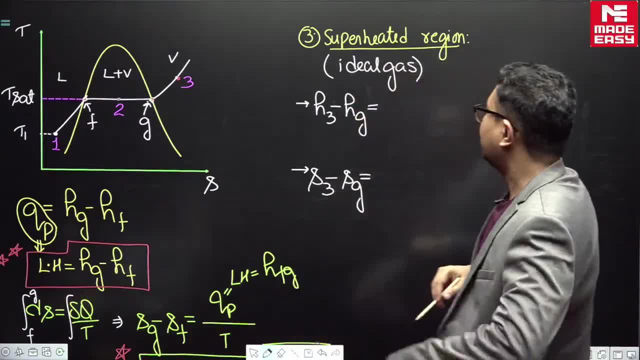 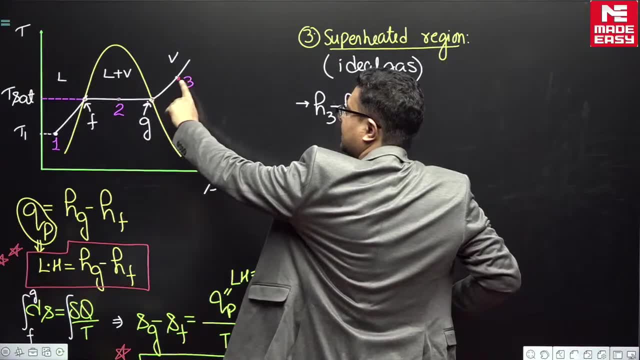 We assume ideal gas behaviour. We assume it. So we have discussed so we can say H3 minus Hg. H3 minus Hg Enthalpy change, H3 minus Hg Enthalpy change. This can be written as: 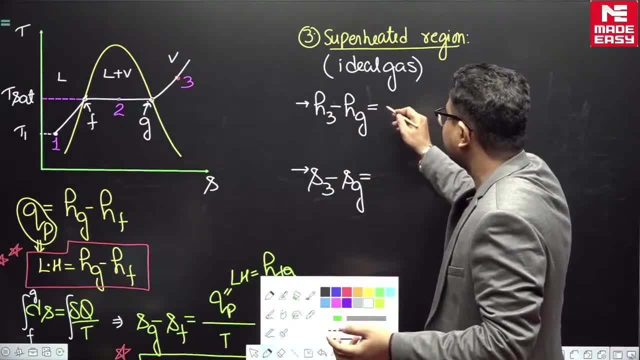 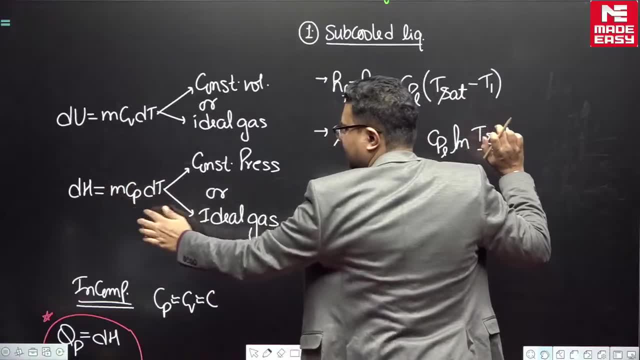 pressure constant, Pressure is constant, So constant pressure Enthalpy change can be written as Cp dT. Enthalpy change can be written as mCp dT: unit mass. cp dT, Constant pressure or ideal gas. In both cases, 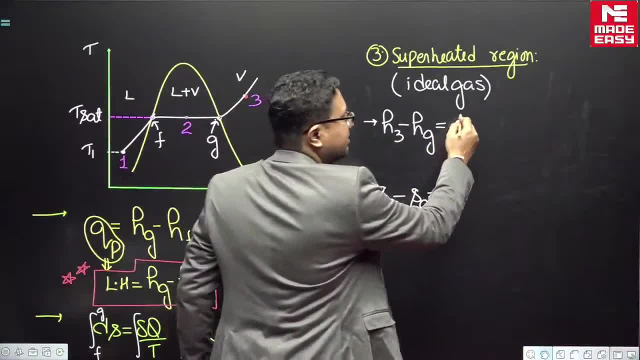 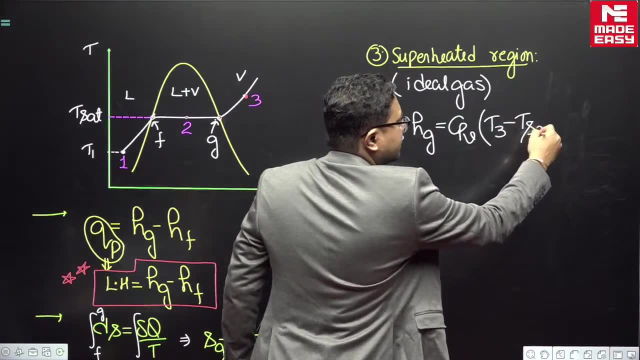 you can write, So we can write Cp, But here the Cp is for vapour, Because it is in the vapour phase, Cp into dT, So T3 minus T saturation, T3 minus T saturation. We can write like this: 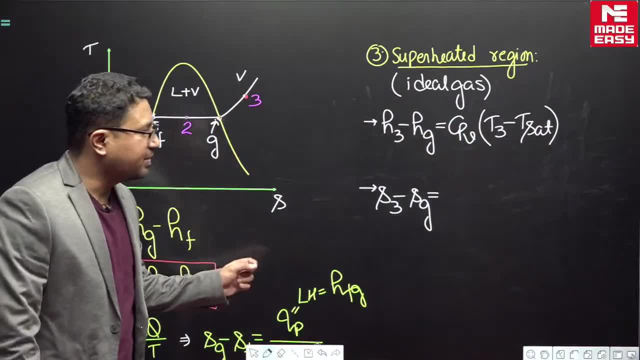 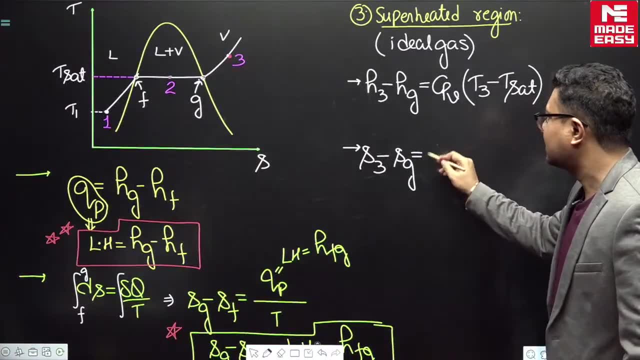 As I have written Now, the entropy change. Entropy change if we write, assuming the ideal gas, If we assume the ideal gas and write, so there are expression and the formula of ideal gas is Cp, ln, T2 by T1.. T2 is T3. 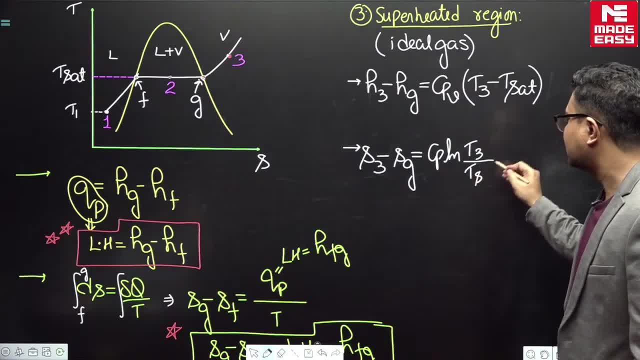 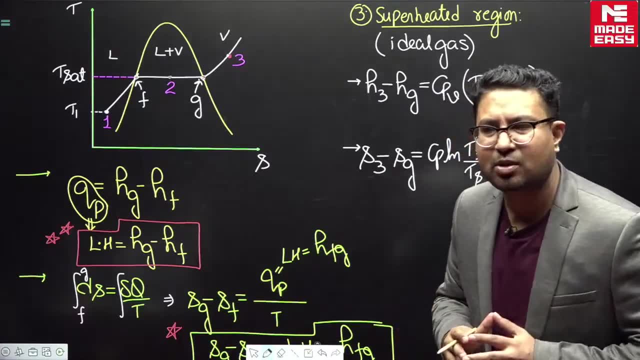 that is T3 upon T saturation, minus R, ln, P2 by T1.. I am using the formula for entropy of an ideal gas. I am using the formula for entropy of an ideal gas. Temperature pressure: P3 upon P saturation. Now you see. 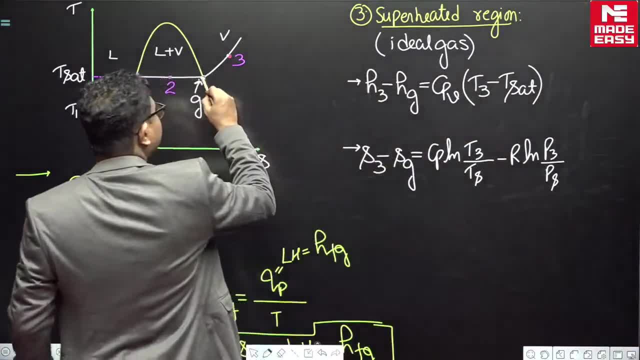 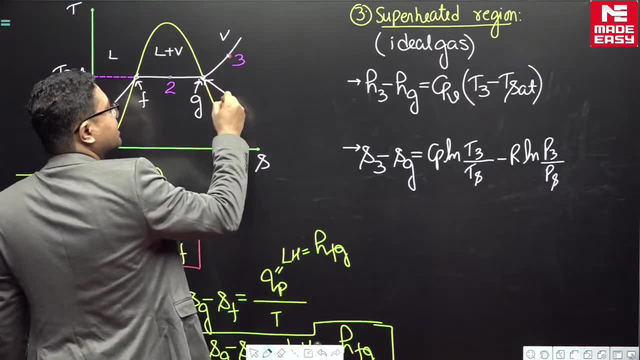 from here. this is this is what I am calling as saturation. From here to here. from here to here. this is basically saturation condition. This is saturation condition. So from here to here, pressure is constant. Pressure is constant, So this will become 0.. 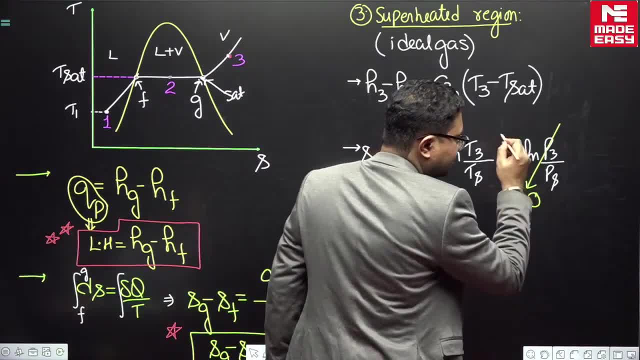 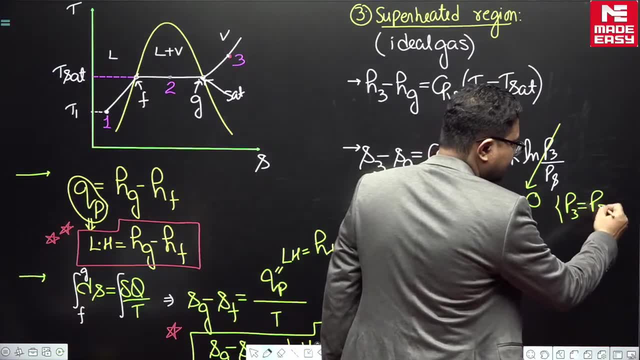 This is pressure constant, So this 1 will come and ln of 1 is 0.. P3 is equals to P s. Why it became 0?? Because P3 is equals to P s, So this became 0.. 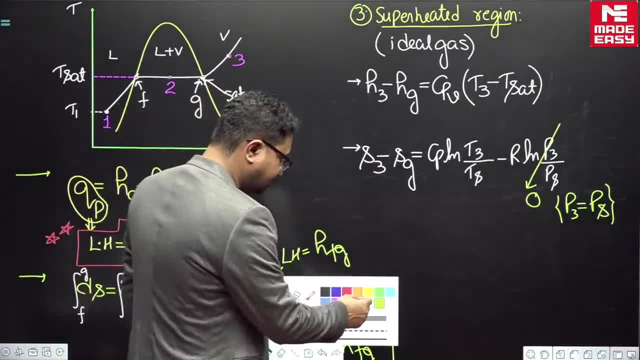 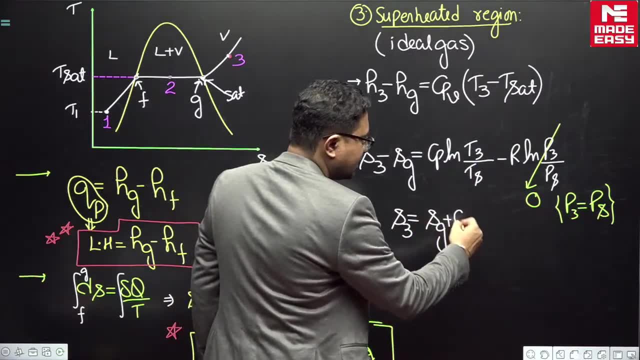 This became 0.. Okay, So S3. S3 is equals to- we will move it to. the other side is equals to Sg plus Cp: vapour, Cp it is for vapour. What are we talking about? We are talking about vapour. 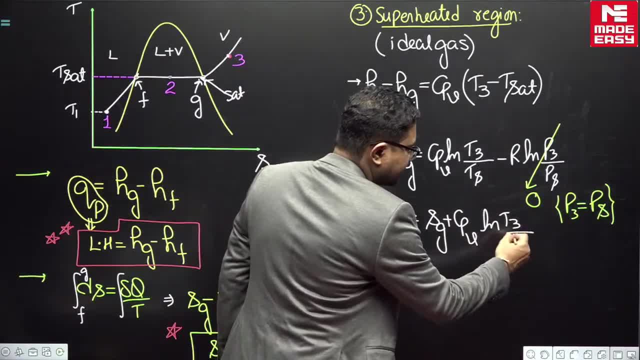 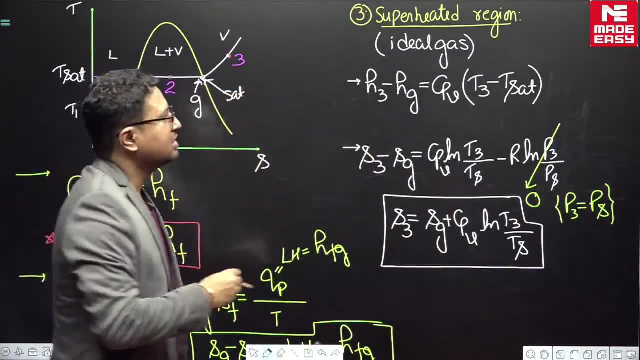 Cp vapour ln ln. T3 upon T s, ln T3 upon T s. So this is the expression. This is the expression. T s is saturation temperature. This is the expression for enthalpy change. Now we can move on to. 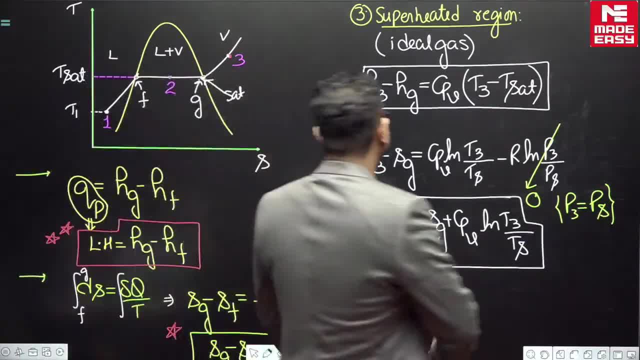 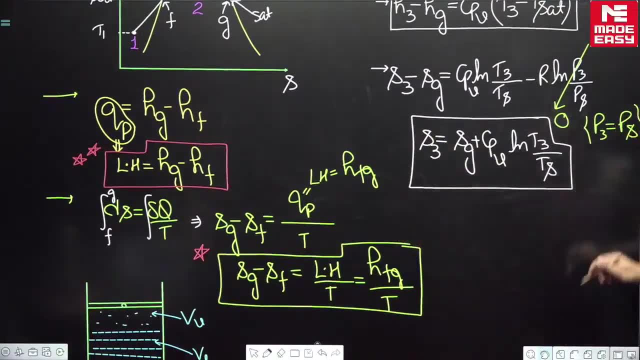 the questions. Some questions we will solve. Okay, Now you see, this is the during the phase change. This is the expression of phase change which we have developed, And this is for the superheated region. I will just show you for a moment. 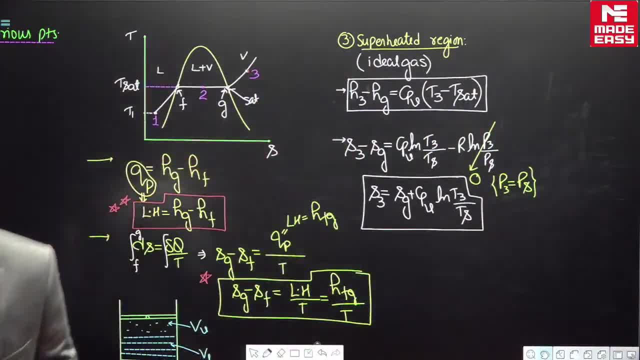 I will just show you for a moment And then we will move forward to the question solving From question solving way. Abhishek, you are asking only we can apply PV equal to MRT in superheated region. See in the PV equal to MRT. 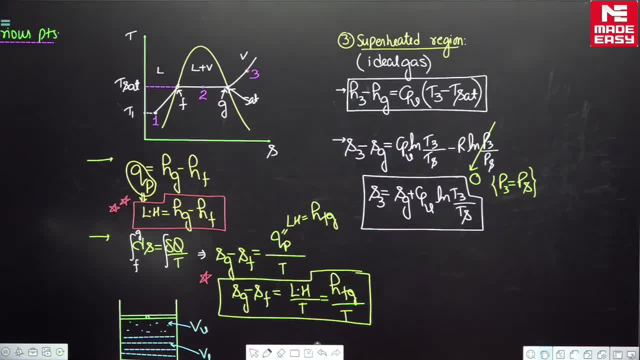 PV equal to MRT. superheated region: may, we can not definitely apply, but only in the superheated region. actually, you can consider the substance to be gas. You can consider the substance to be gas in the superheated region only, So you can consider it. 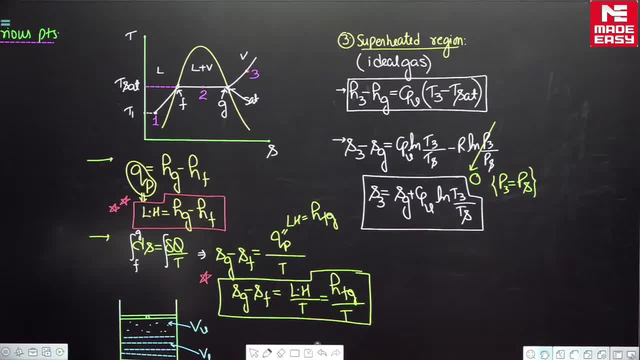 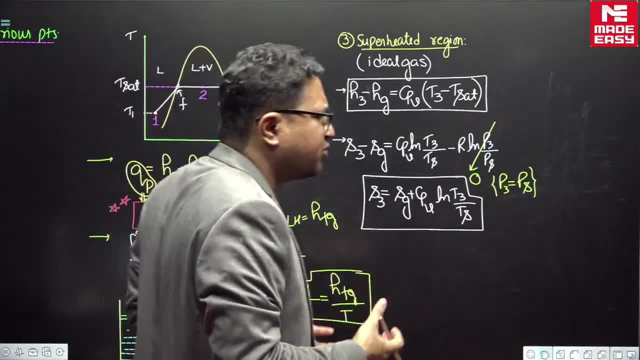 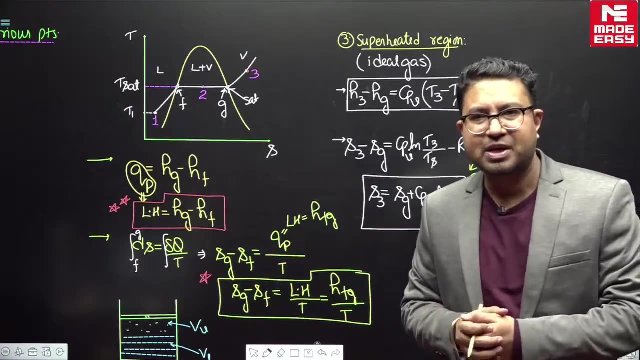 for the superheated region only. Okay, So now let us move forward and let us apply this understanding. Let us apply this full understanding. Let us solve some questions. Okay, Let us move forward to the question solving part. Now, here we have to solve the question. 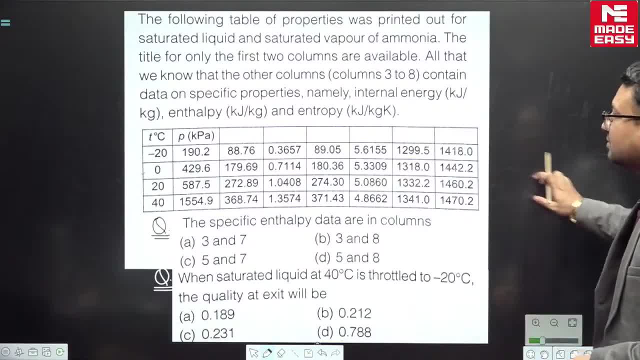 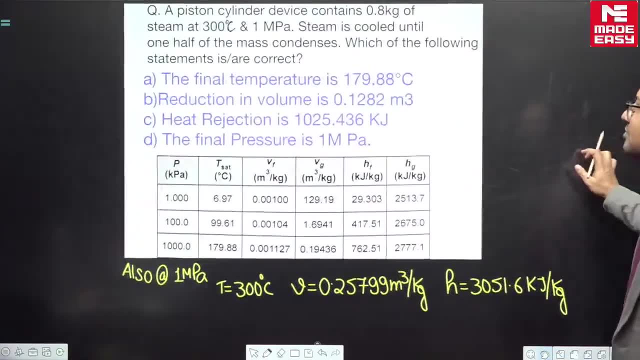 Now here we have to solve the question. Now here I have here, we will solve this question, but before this, let us solve this question. There is one question Now. see, this is the problem. Let me read this problem. 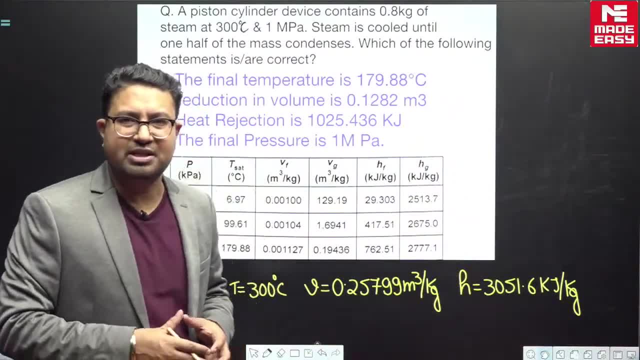 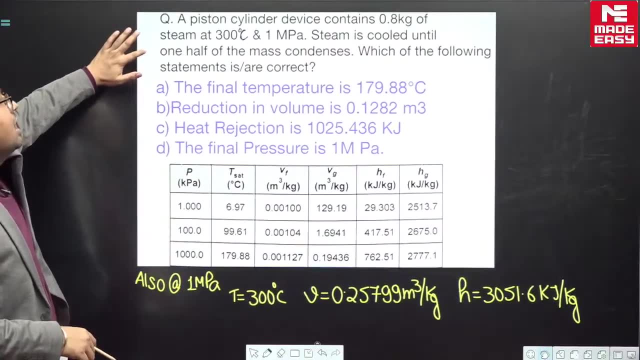 and let me explain how we will discuss this on the diagram. We will represent it on the diagram and then we will discuss it. So if you see here, a piston cylinder device contains 0.8 kilogram of steam at 300 degree Celsius. 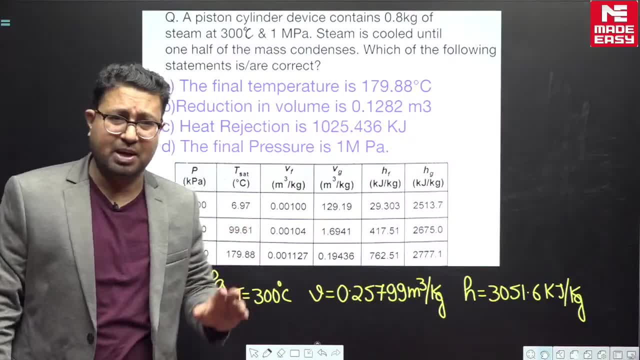 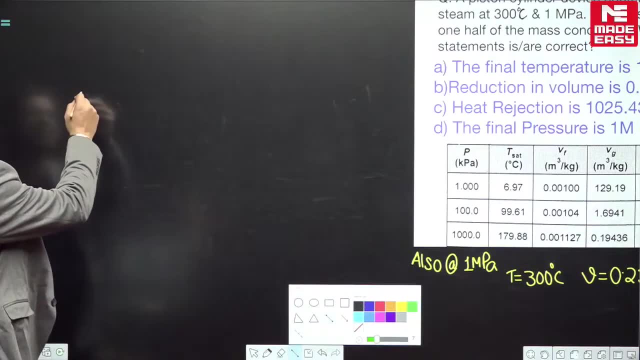 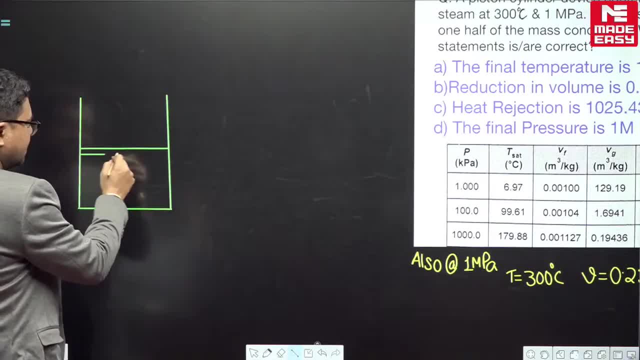 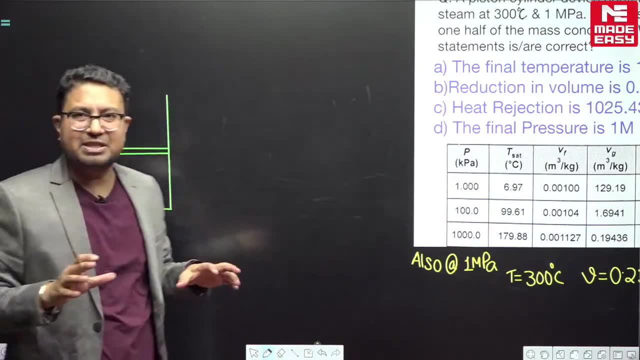 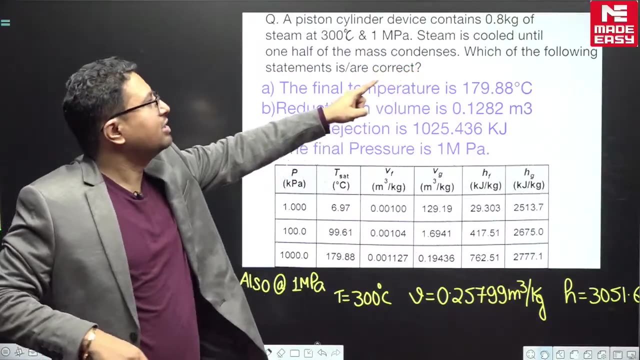 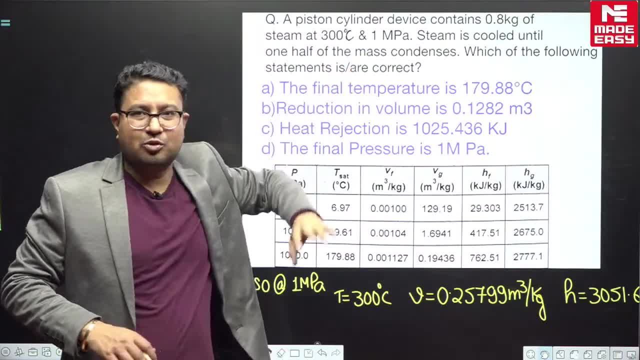 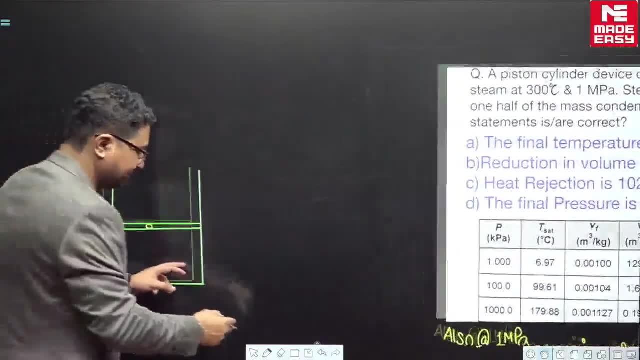 have given. This is the temperature and this is the pressure. So, parallely, let me also plot the T-S diagram. Parallely T-S diagram. we plot kartao na. We will be able to visualize and visualize kar payenge, condition ko. So let me, parallely, also plot the T-S diagram. 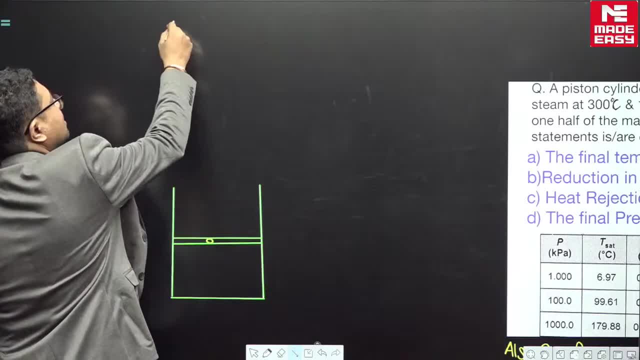 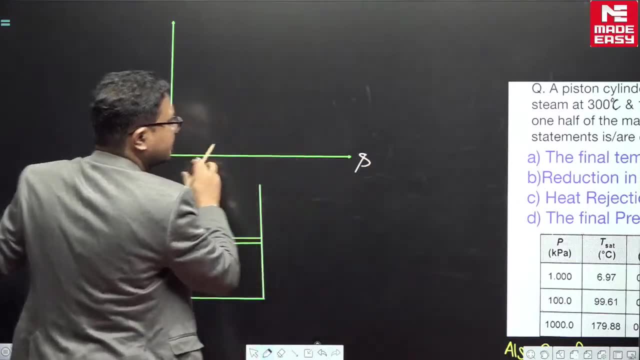 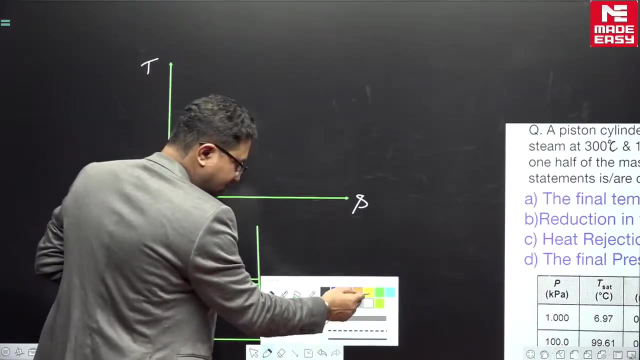 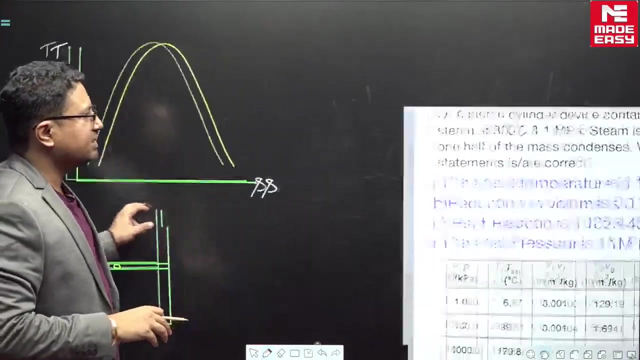 T-S diagram. ko plot kartao. So this is the temperature axis, this is the entropy axis, and we are trying to plot this here. We are plotting this here. T-S diagram. Now, if you see, suppose this is the saturation curve, If we see, the condition given is 1 megapascal. 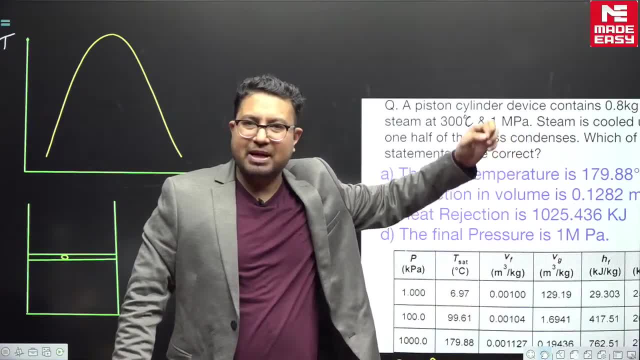 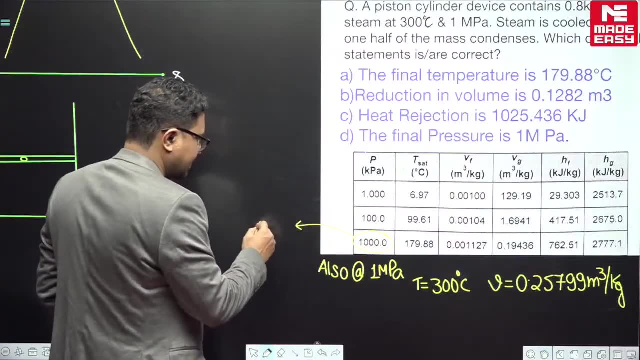 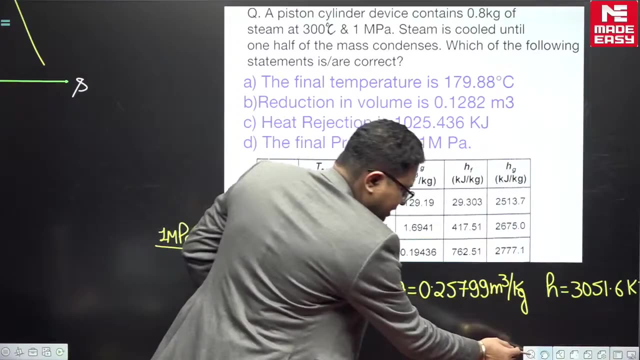 pressure. So 1 megapascal means 1000 kilopascal. this is the data. This is the data for 1 megapascal. I hope the data is visible to you. I will. in any case, I will slightly expand it here. So, 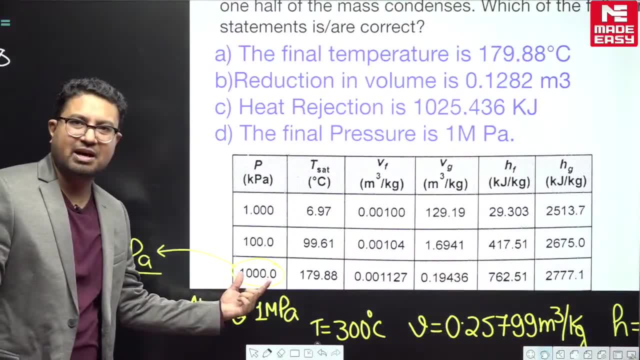 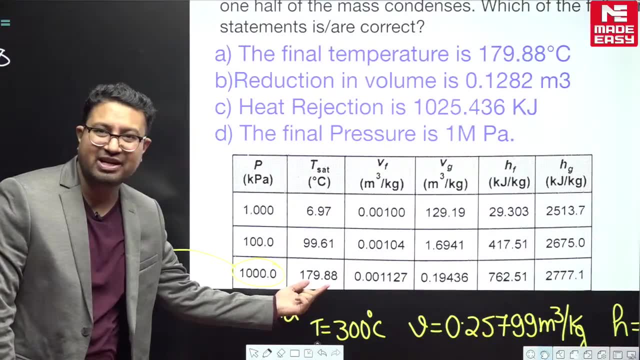 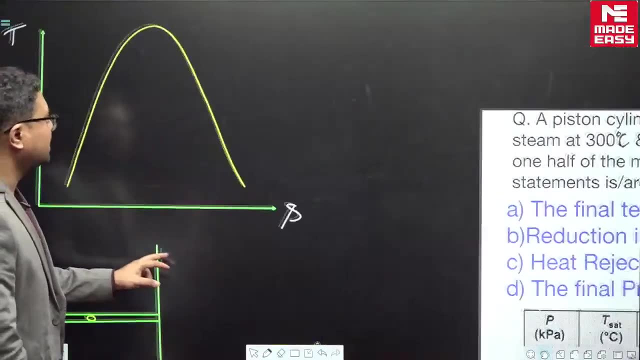 1 megapascal. ye 1 megapascal hai Now 1 megapascal k corresponding. corresponding to 1 megapascal, this is the saturation temperature. phase change ka temperature to ye hai 179.88.. This is the saturation temperature: 179.88.. So corresponding to 1 megapascal. let me just draw a constant. 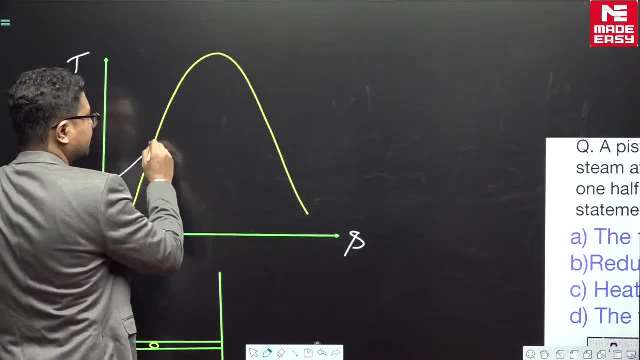 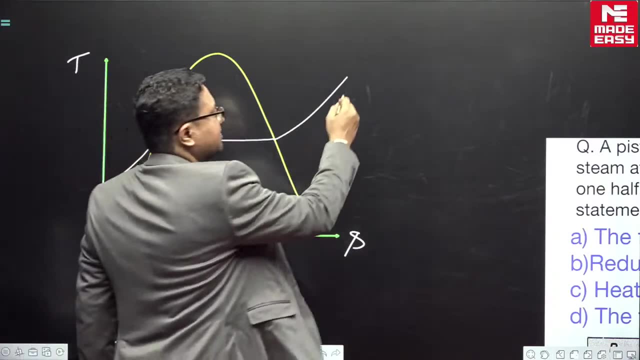 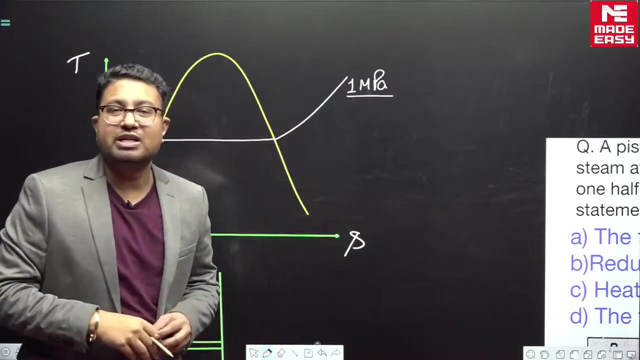 a constant pressure curve. here a constant pressure curve could draw. let me draw a constant pressure curve. constant pressure curve could draw. what is the pressure on this curve? the pressure is 1 mega Pascal. pressure is 1 mega Pascal Saturation: what is the saturation temperature? so, saturation temperature, if we see corresponding 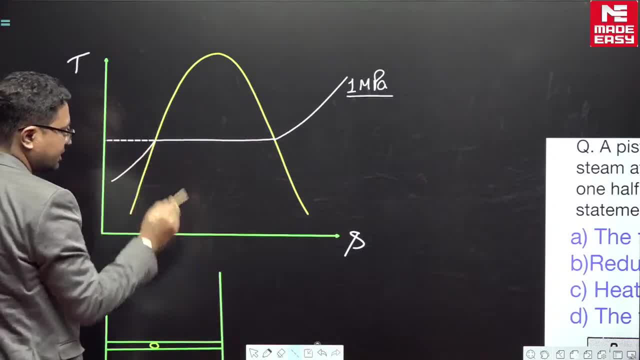 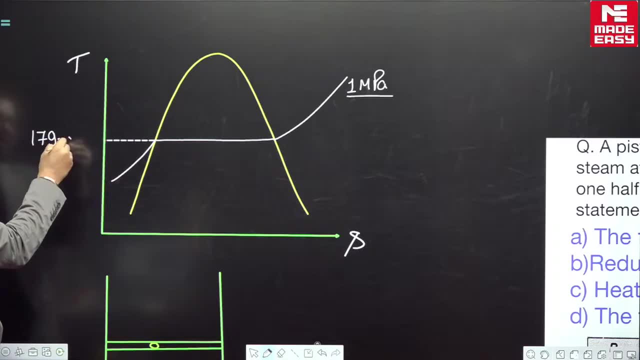 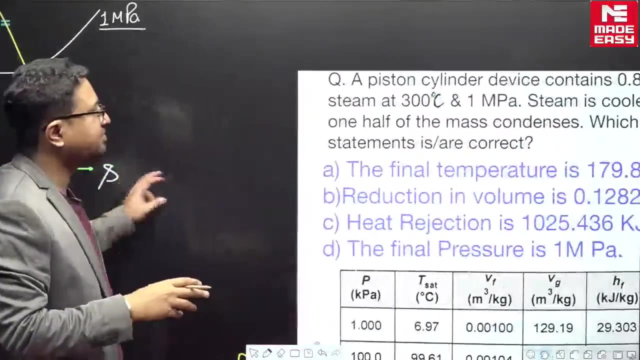 to this. corresponding to this, the saturation temperature is 179.. So the temperature is 179.88 degree Celsius, 88 degree Celsius here. and at what condition the steam is steam. this condition, when they go mass of the steam, 0.8 steam, is at 300 degree. 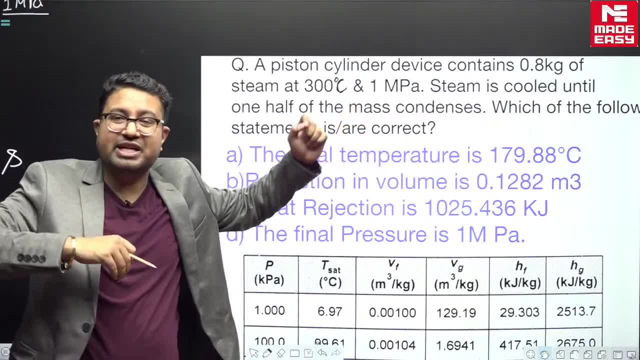 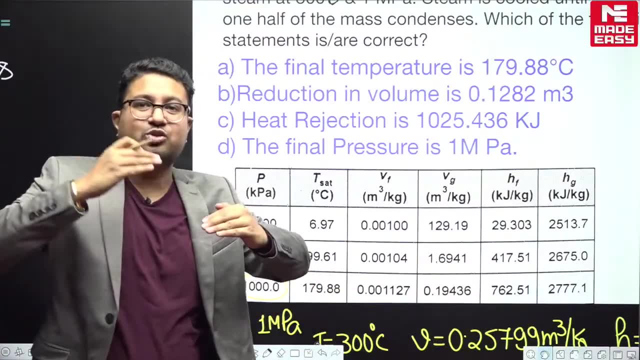 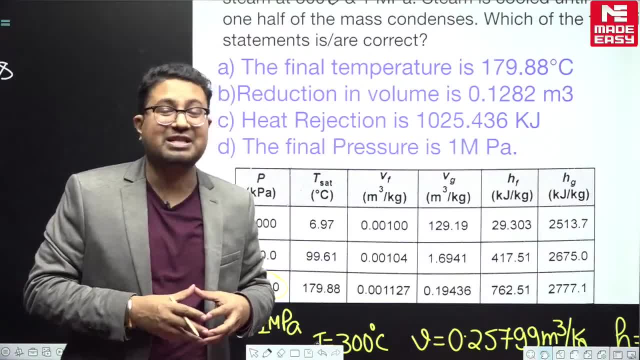 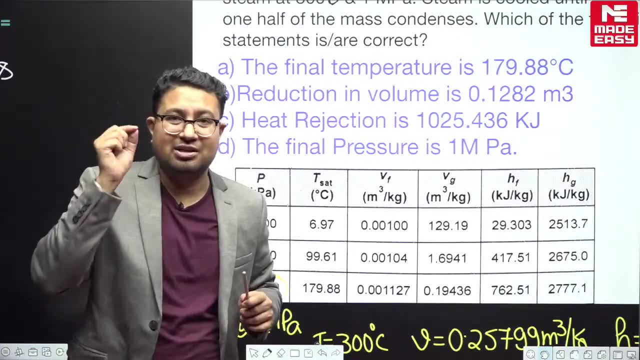 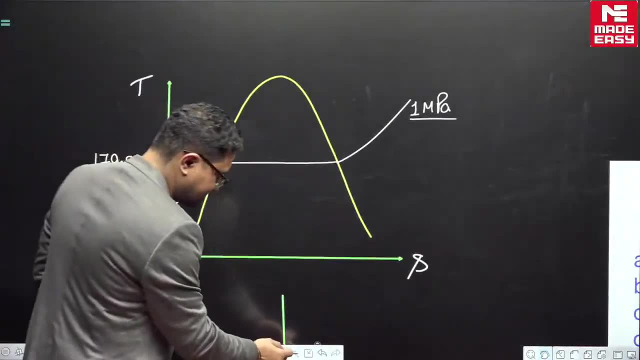 present above the saturation temperature, if it is present above the saturation temperature. so we call it what we will call it as we call it, as we call it, as the superheated vapor superheated state. So this is the superheated state. this superheated state will be 300 degree Celsius. let us mark. 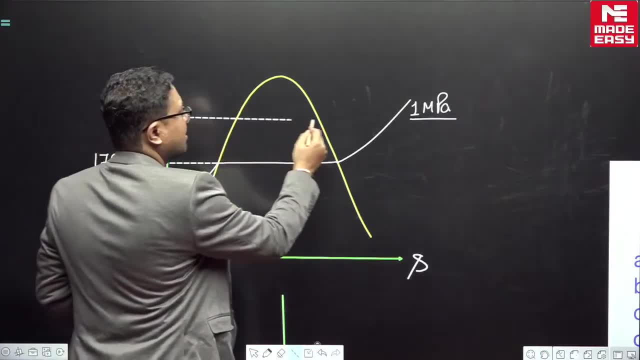 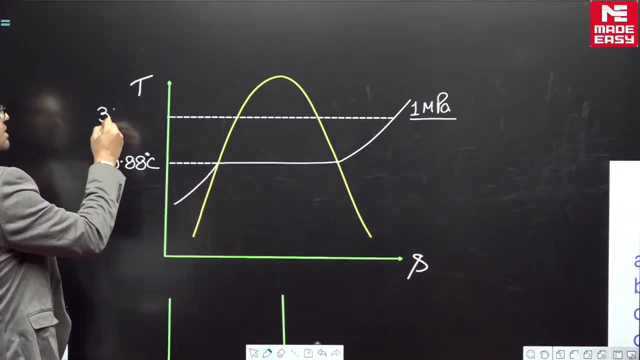 it here. let us mark it: 1 mega Pascal. 1 mega Pascal and 300 degree Celsius. so this is the 300 degree Celsius temperature. this is the temperature: 300 degree Celsius. this so we are here. our initial condition is here. 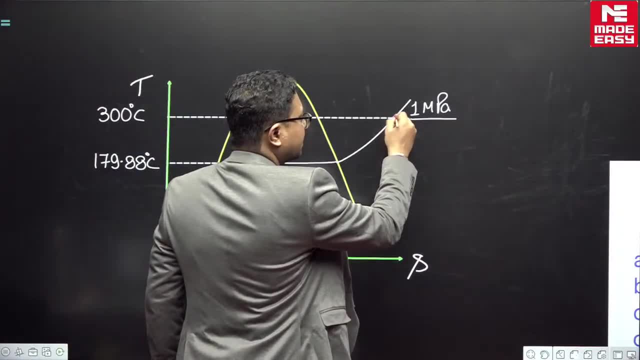 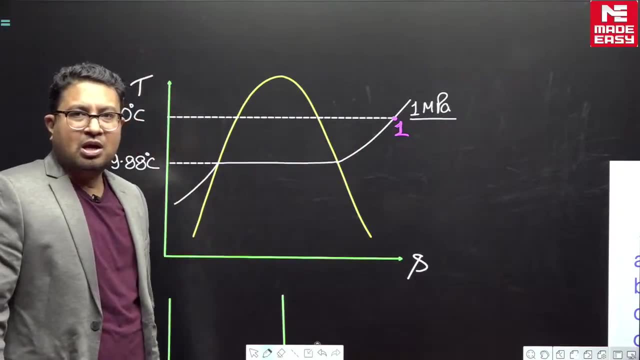 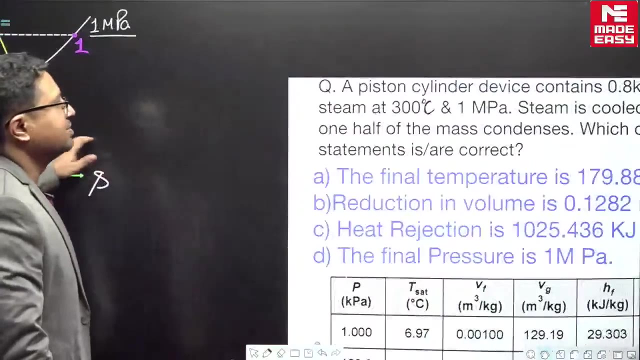 so let me just plot the initial condition. initial condition is marked. this is the initial condition at which we are present. we are present in this initial condition. now we will reject heat. we are rejecting heat. you see what is happening. piston cylinder device. 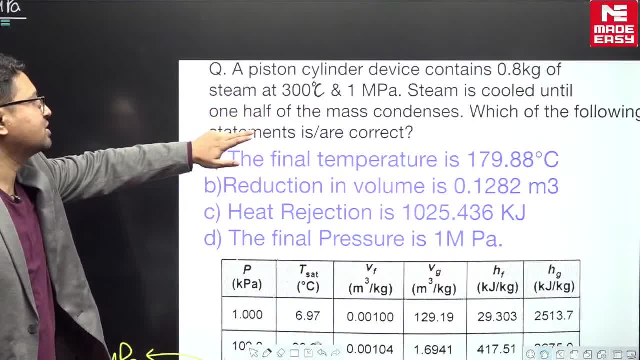 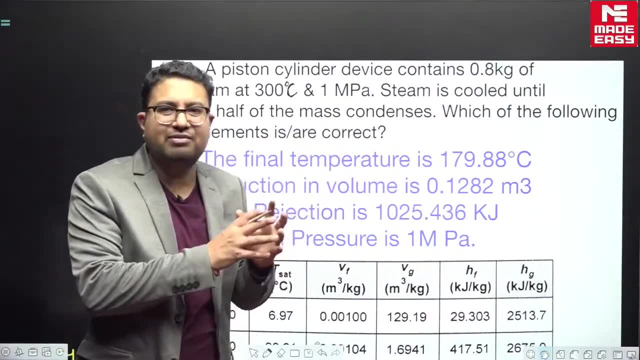 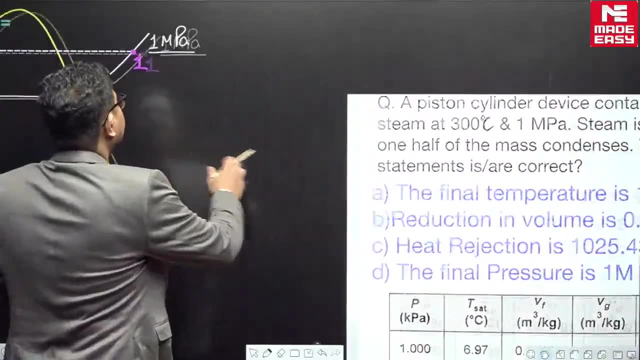 contains 0.8 kilogram of steam at this and this steam is cooled until one half of the half of the mass condenses. that is, half of the mass would have changed into the liquid, so remaining half will be in the vapor phase. see what will happen when you are cooling. 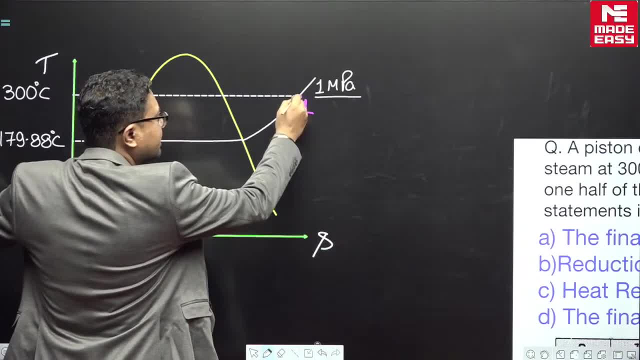 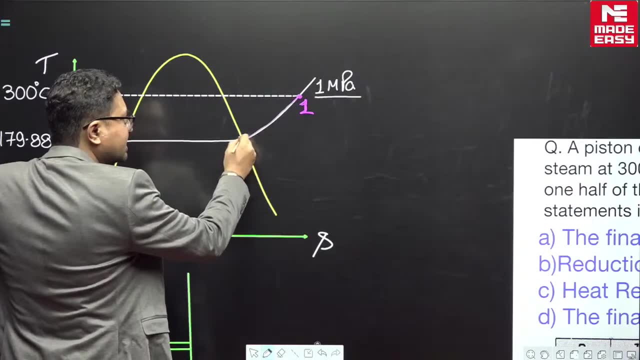 when you will cool initially, you will follow this curve. the pressure is constant in piston cylinder arrangement. there will not be condensation. you will cool from here to here to here. pressure constant is there at this condition, At this condition, At this condition, when you reach, then all the mass, whatever the total mass, is the 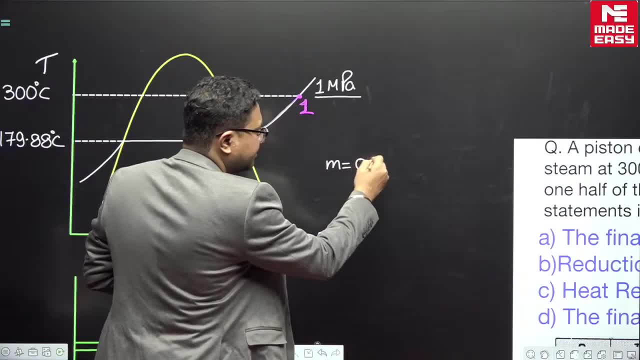 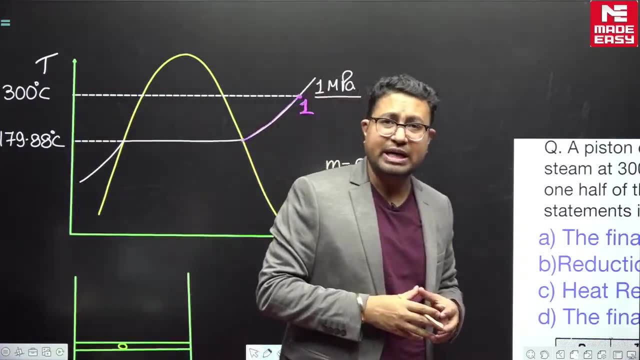 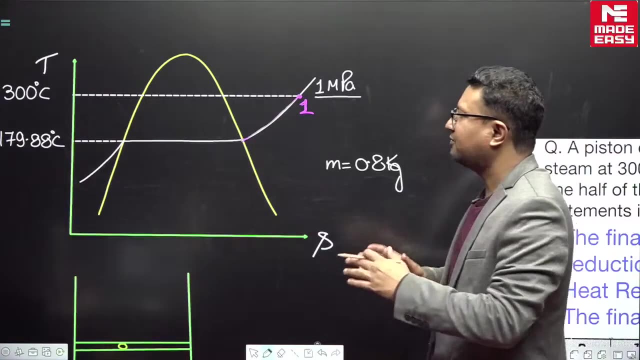 mass is: the total mass is 0.8 kilogram. total mass is 0.8 kilogram. so when you will reach this condition, that is, 1 mega Pascal and 179.88 degree Celsius, when you reach this condition, then you will reach this condition, so you will have half of the mass I am representing. 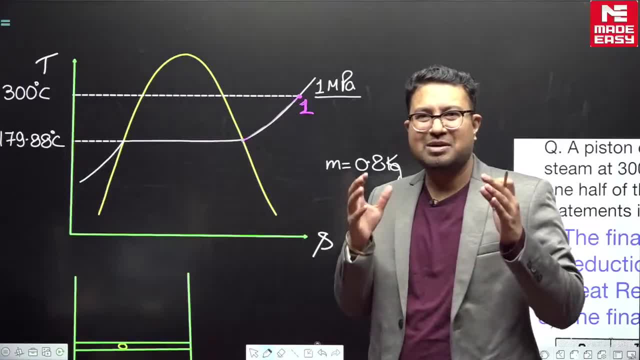 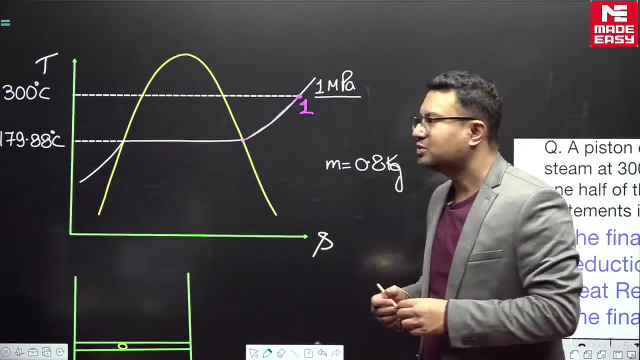 you have to solve, I will discuss it. I will discuss it, but I will represent it and you will have to solve it. you will have to give the answer. You have to answer. I am representing it and showing you the condition. 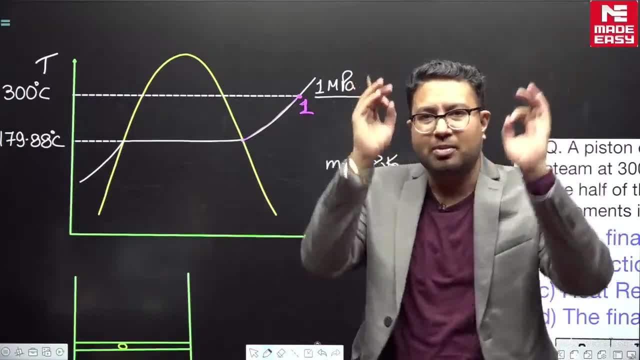 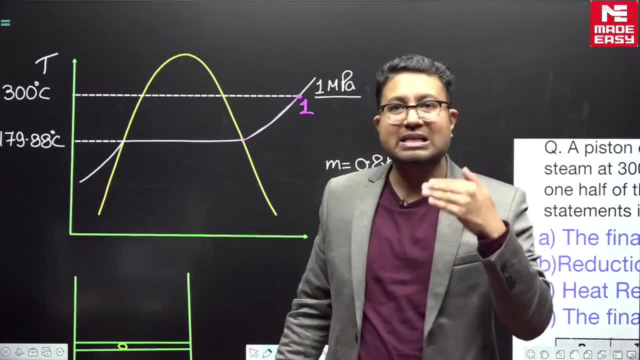 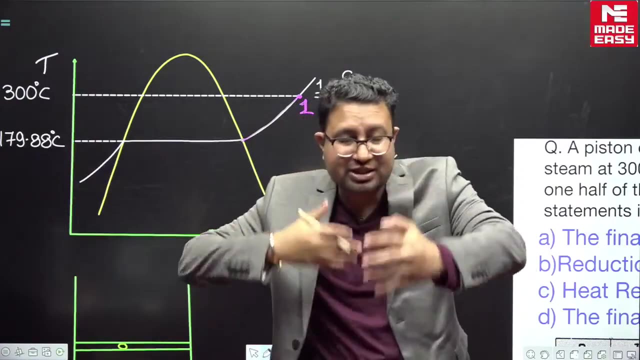 So understanding the diagram helps us in visualizing. so whenever you do the question, solve. so whatever diagram can be made, just draw the diagram. Two things are there. first, you will understand what steps to right when you have to solve the question. you will be visualized what is the situation so you will know what steps. 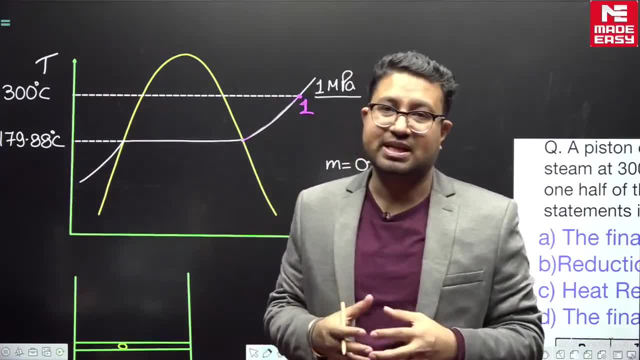 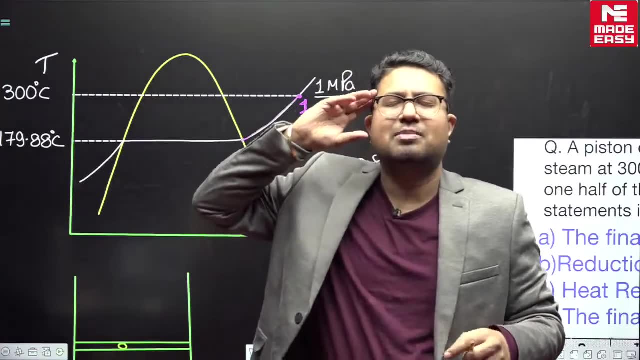 to right. Secondly, you will make less mistakes. You will reduce your mistakes. Otherwise what happens? The mistake will be reduced. You will not get anything. Otherwise what will happen? You will not get anything take place when you try to solve, when you try to solve a lot of things in your mind. 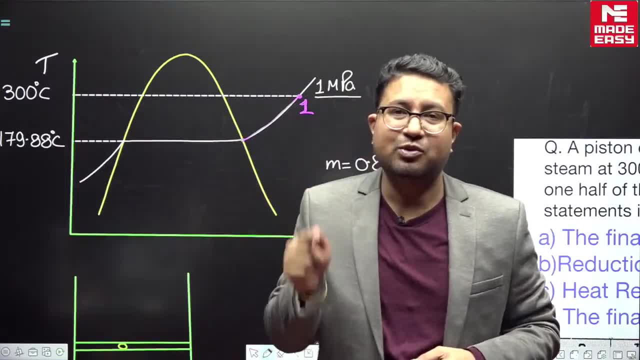 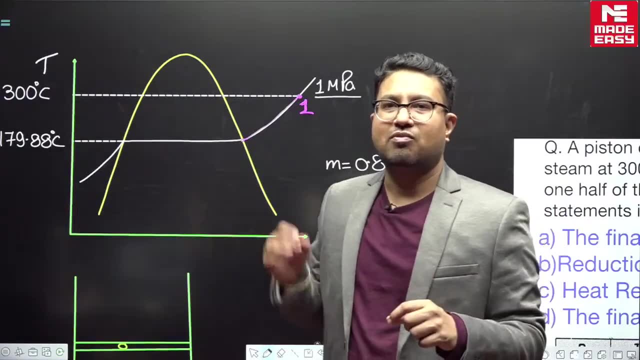 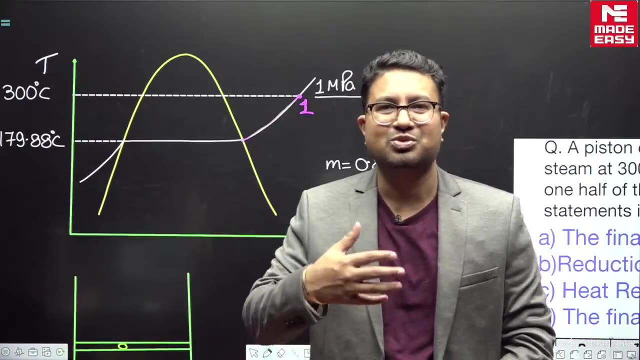 then mistakes happen. but if you write down, draw diagrams, mistakes are reduced. so whatever mistake you make, just make sure whatever is in your mind don't do too much in your mind. in life also it happens. if we don't live the situation and keep thinking so we create a lot of problems in life. 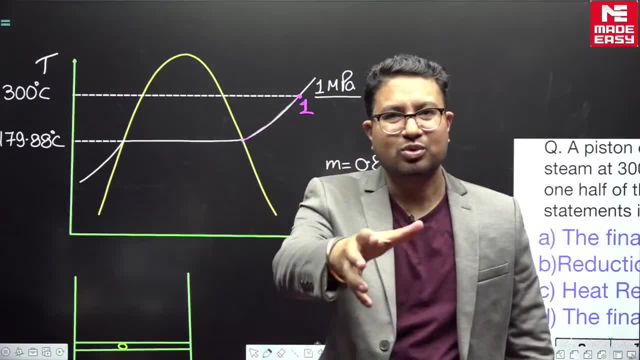 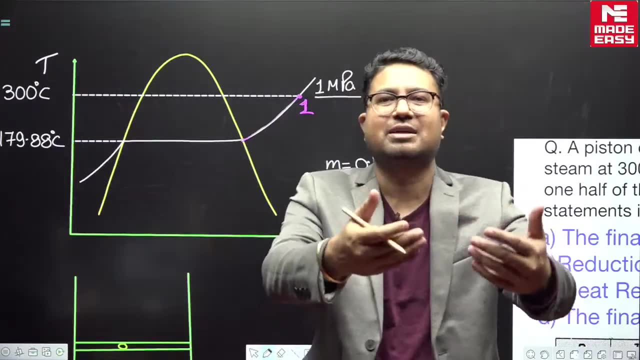 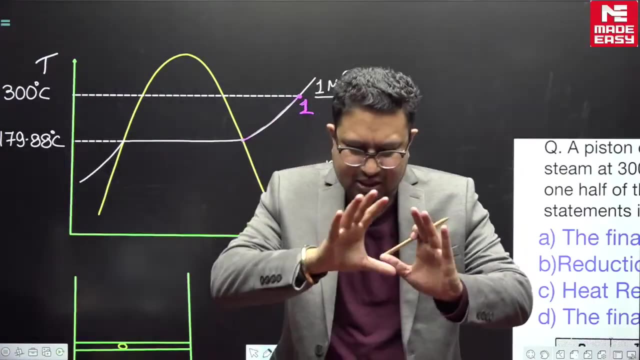 so we have to go through the reality, we have to go through the experience and that is how the things, automatically. then you can see the next step. so it is same in the life also, and with the problems also. so you take one step, you write down things. 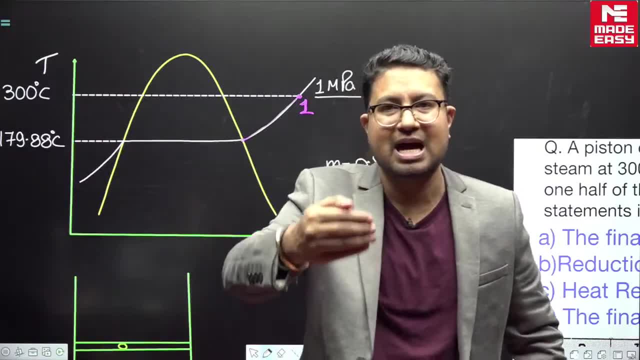 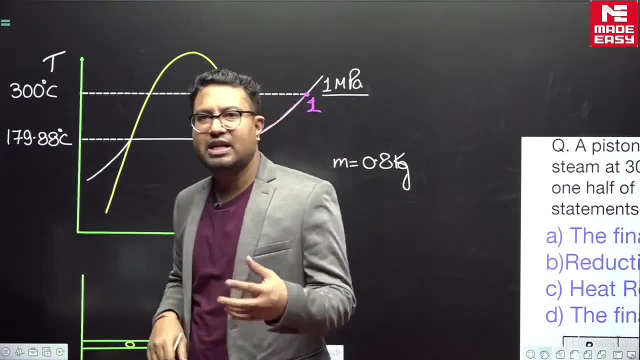 you see what is the situation, then you will know the next step, and then the next step, and so on. so now here we are cooling. so when we reach here, 179.88 degree Celsius. so up to here, all the masses- still now all the masses is vapour. 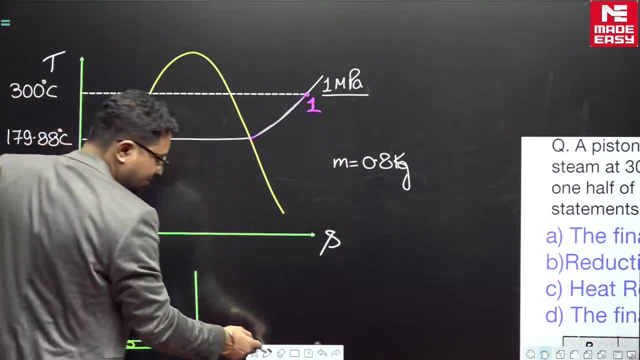 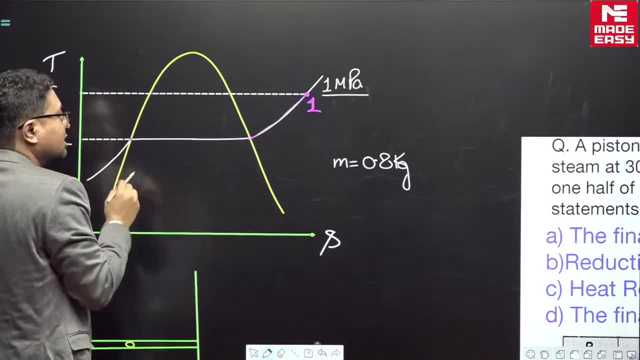 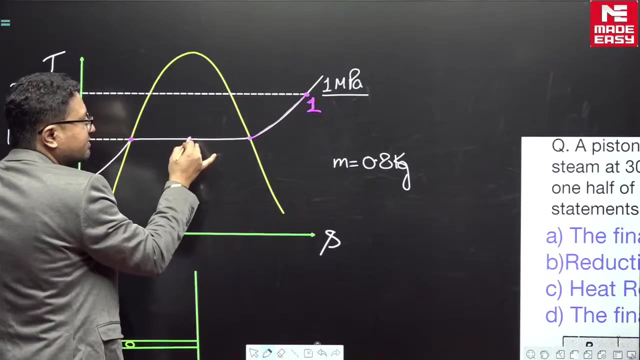 now we will cool it further, then some mass will change into some mass will change from vapor to liquid, then some more mass will change, and so on. finally, half of the mass is this, other half this and other half that. so average condition will be seen here. Yang color. 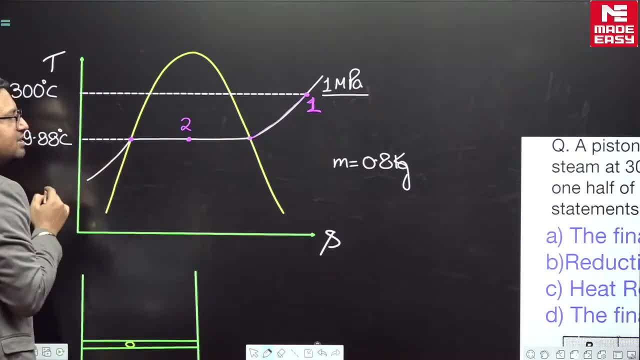 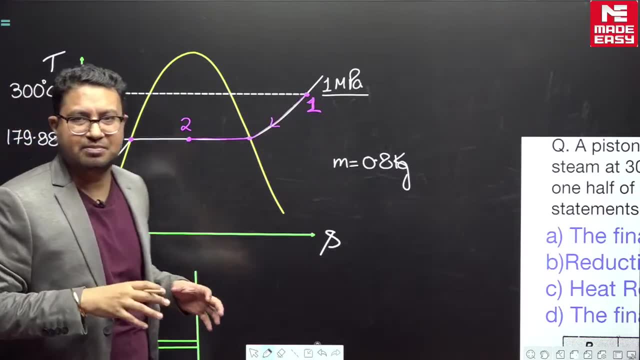 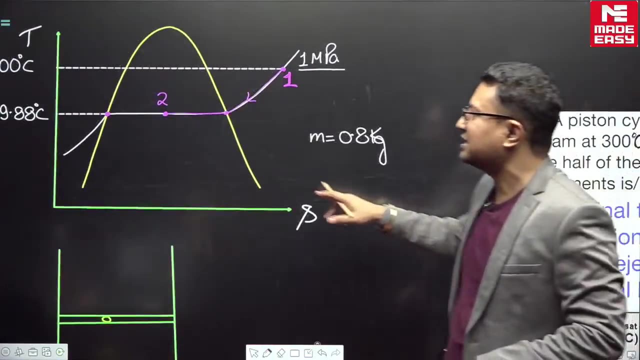 finally, half of the mass is in this condition, other half in this condition. final condition is like this: so this is process, this means the process represents. I mean you had created like this for this system: 1 to 2,, 2 is the final condition. and now we can say: and what is the dryness? 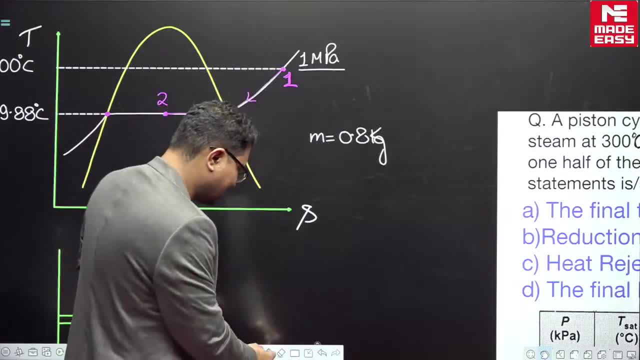 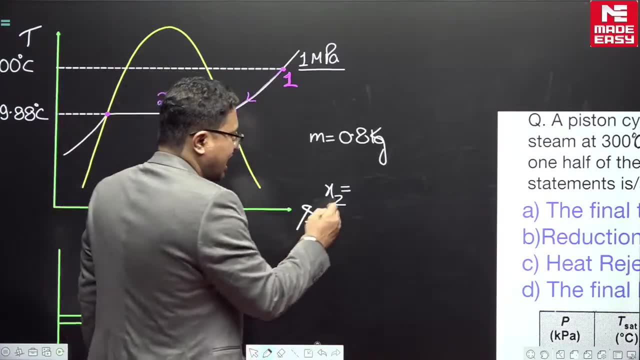 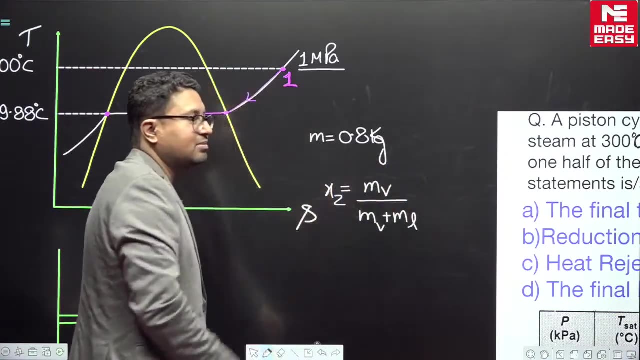 fraction at 2, you will say 2 at condition 2,. this is not given directly. question is not given directly, but we can calculate. x2 is equals to mass of vapor and this is mass of vapor plus mass of liquid. so half of the mass has become liquid. half of the mass. 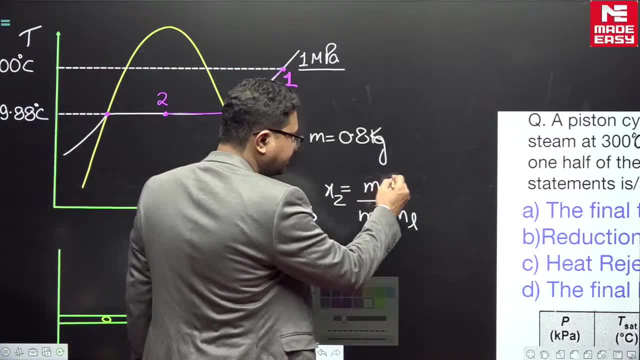 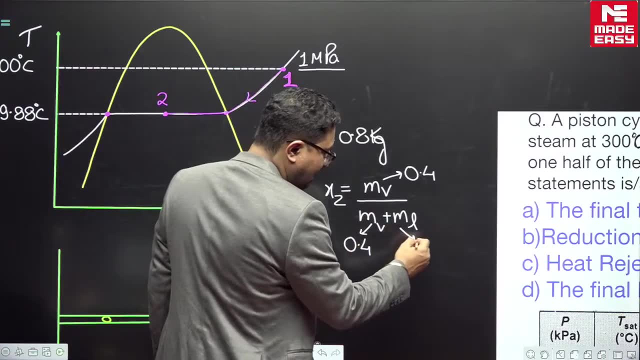 has condensed. so, out of 0.8, this is 0.4, remaining, how much is 0.4,? this is 0.4, how much vapor, how much liquid? 0.4,. so this x2 will be equal to half. this will be half. 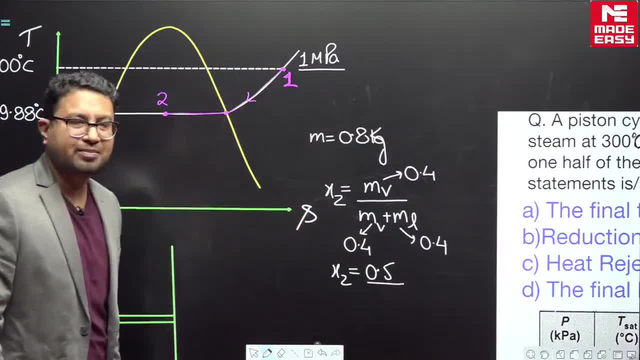 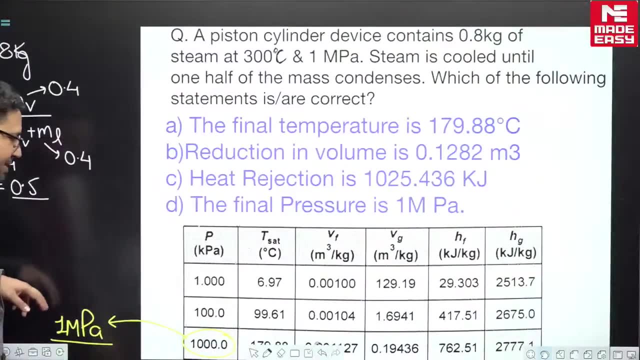 that is 0.5,. dryness fraction has come now. see, this is the situation. I have represented the situation. now, what they are saying, final temperature is this: so this is an MSQ, a multiple select question, more than one option. 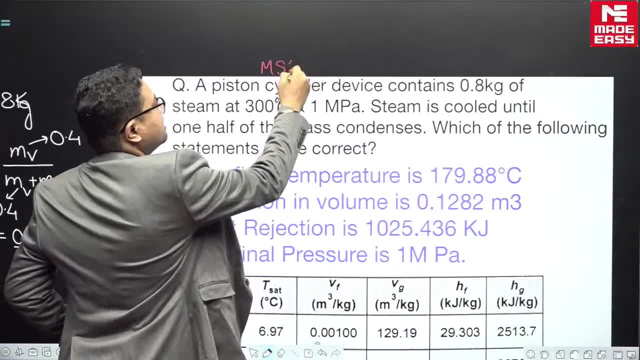 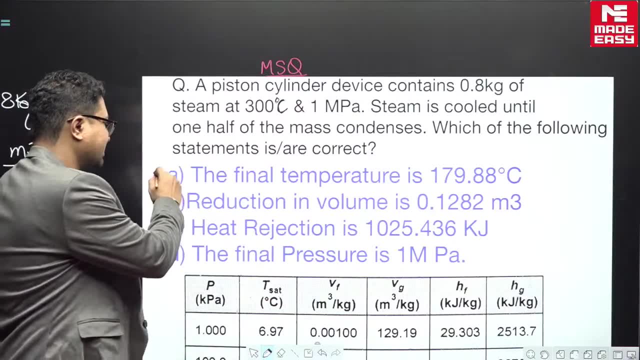 Can be correct. MSQ multiple select question: more than one option can be correct. final temperature is this: this is correct. we have already known, so this is correct. this is correct. final temperature is this: final pressure is 1 mega Pascal. this is also correct. 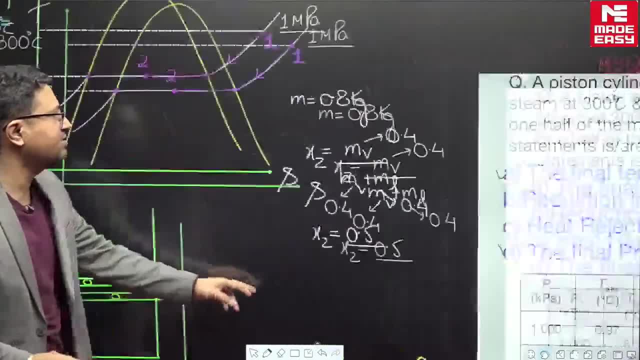 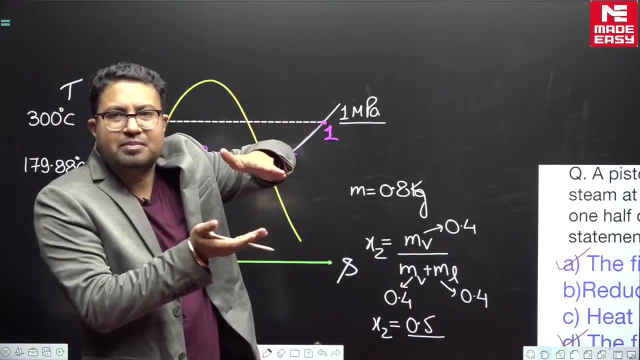 this is also correct. final pressure is 1 mega Pascal. if you are cooling in the piston cylinder element here, so piston will go down, volume will come as the vapor will condense. volume will come, so it will go down. but whatever is the pressure of the 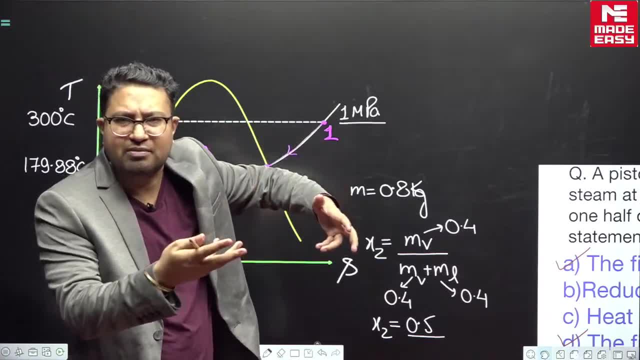 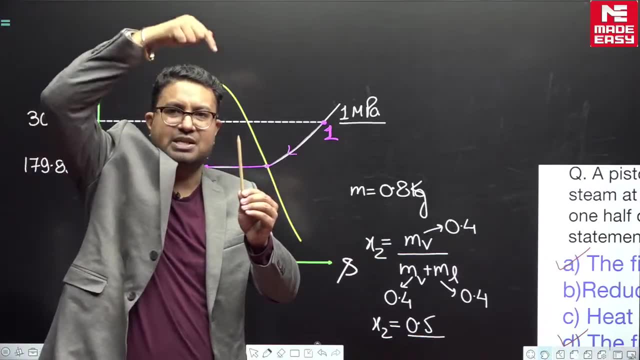 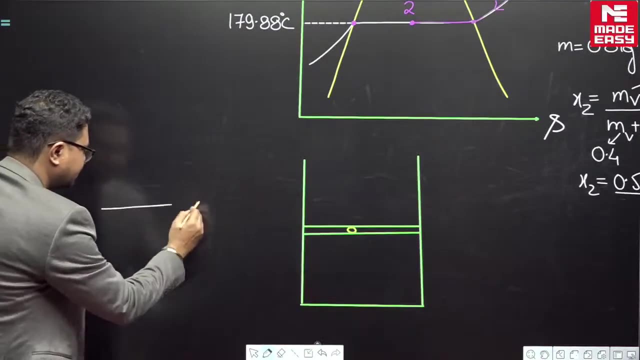 steam. There is no external force you have applied, no weight is kept. so whatever was the pressure which was balancing the weight, MG and P naught into A means, whatever pressure was balancing the piston earlier, whatever pressure, there was some pressure: 1 mega Pascal. so this: 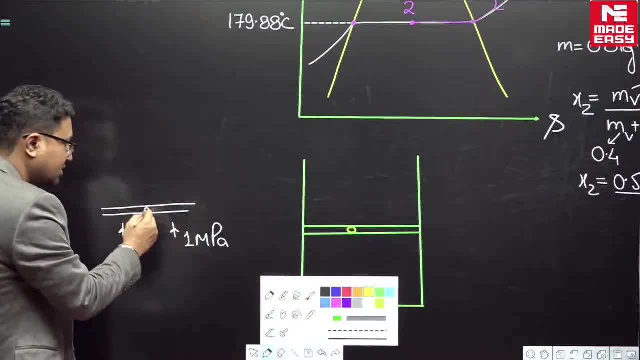 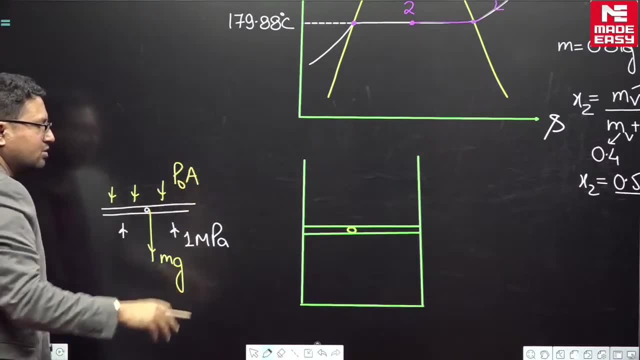 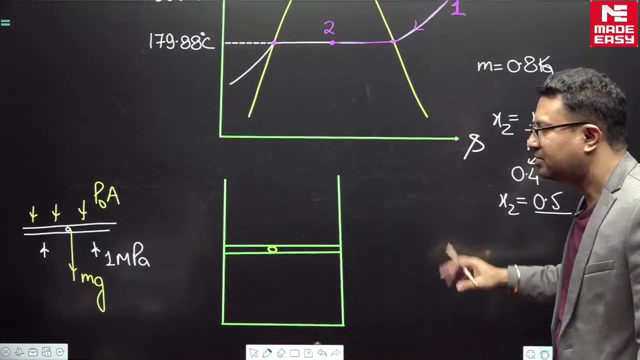 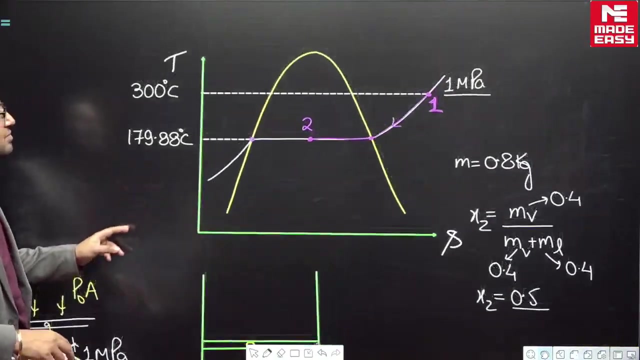 much pressure is required to balance what, to balance MG and P naught into A, So almost same pressure will be required. almost that same pressure will be required to balance this, to balance this, so almost same pressure will be required. So see, we will have this condition. we will get this condition that if we see 1 to 2, 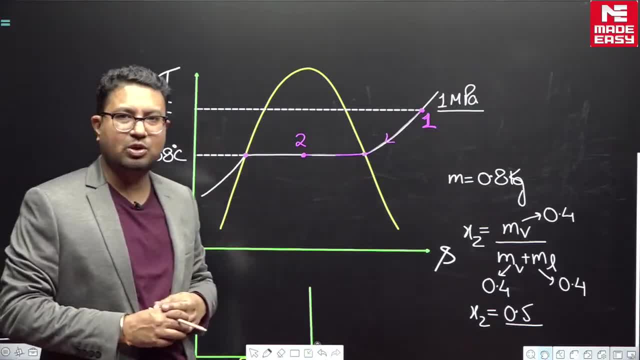 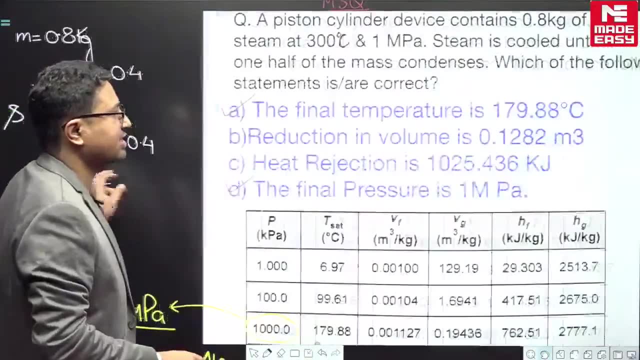 finally, we will reach here now. now see, two statements are correct, because pressure is 1 mega Pascal. so A and D are correct. these are correct. reduction in volume: is this So how we can find out the reduction in volume? 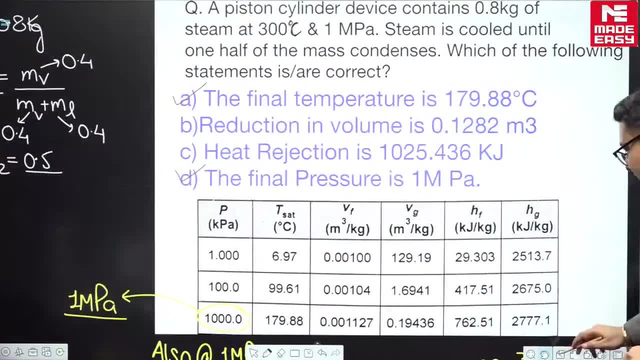 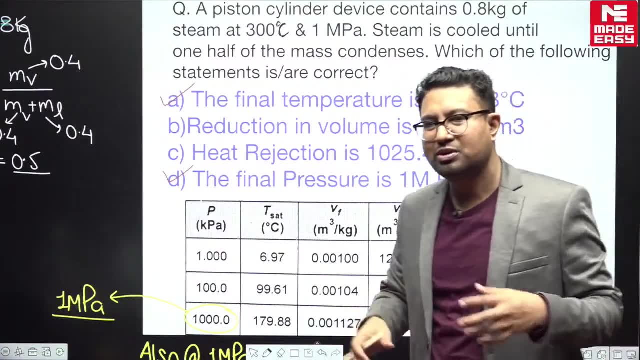 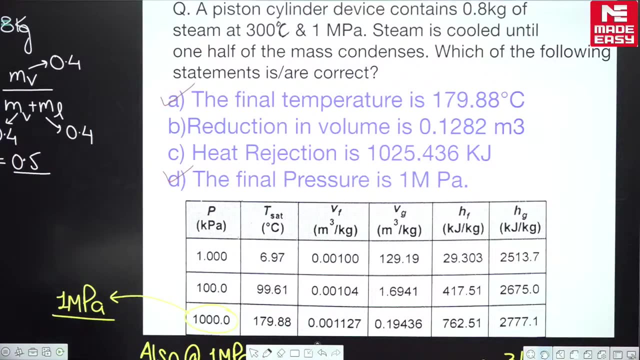 I need answers from you whether this is correct or not. just calculate this, calculate this, calculate the reduction in volume. I have shown you how we can represent reduction in volume, calculate and tell who will calculate and tell Who will calculate the reduction in volume. 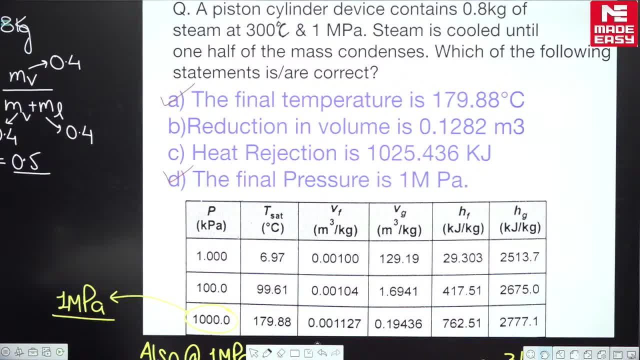 Who will calculate the reduction in volume? Prabhat, Prabhat, Prabhat. Yes, you already calculated the dryness fraction x is 0.5, correct, this is correct, So reduction in volume, reduction in volume. who will calculate the reduction in volume? 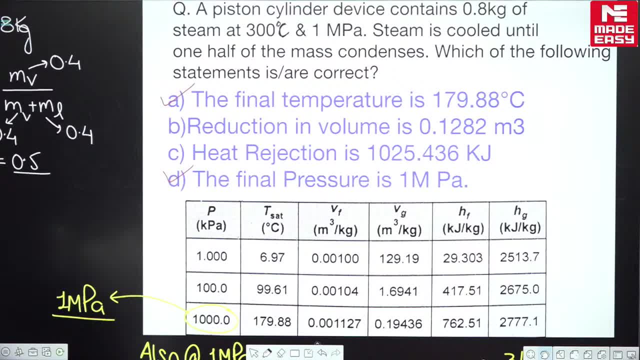 Shreesh Bhardwaj, please. his diagram is a cavitation. cavitation it will take, I mean our discussion will go in a different direction, If somebody can, Since he can understand the cavitation from the discussion, which I have done because 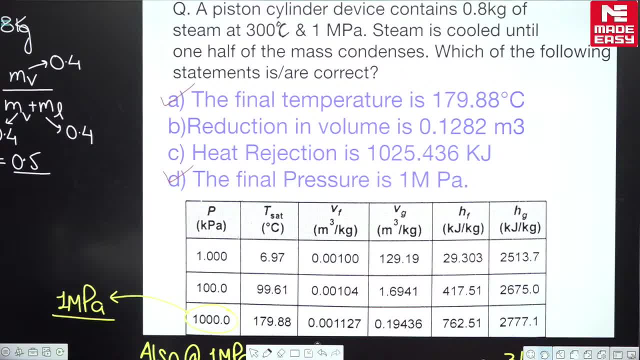 I have done the discussion. cavitation can be understood from it. if you put a little mind, we can understand the cavitation. we can understand the cavitation, just calculate- I need answers from you. I need answers from you- calculate the final volume or the reduction. 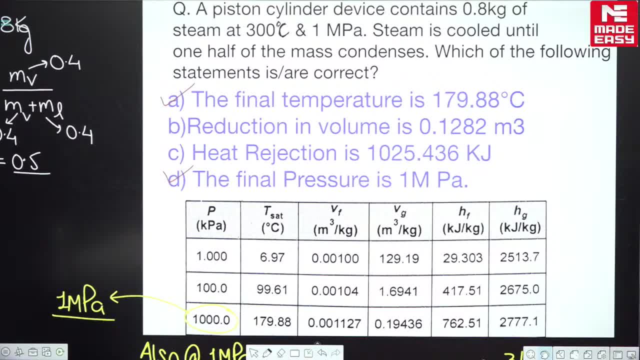 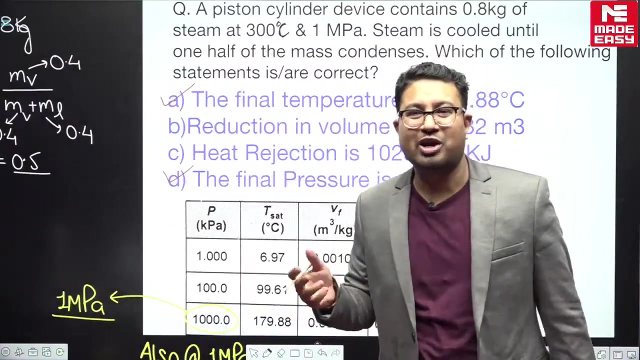 in volume. Tell me the reduction in volume. tell me the reduction in volume. So, reduction in volume, you are saying it is 0.160245, 0.160245, see reduction in volume. reduction in volume means you should not calculate per kg. see I will calculate. 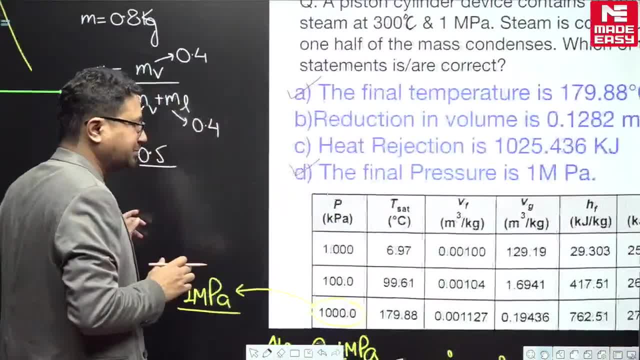 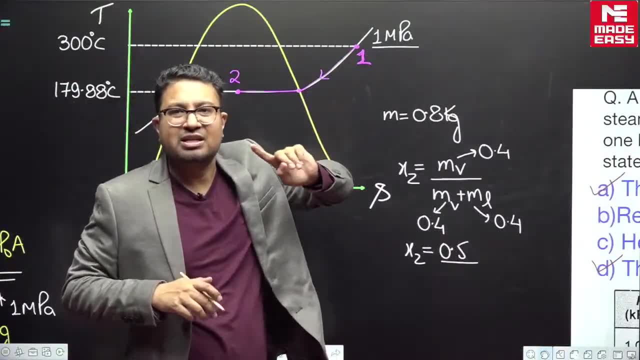 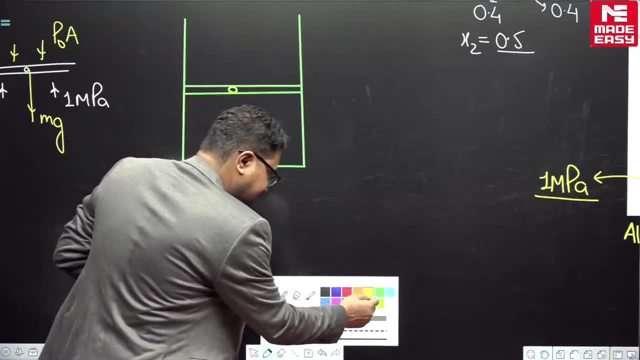 I will calculate. see how I will calculate how I am calculating. see Now: what is the volume at this condition? how much is the volume at this condition? V1, let us see the specific volume. let us see the specific volume. so, second part, if 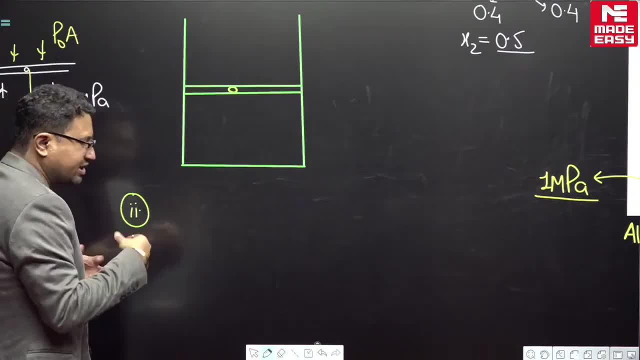 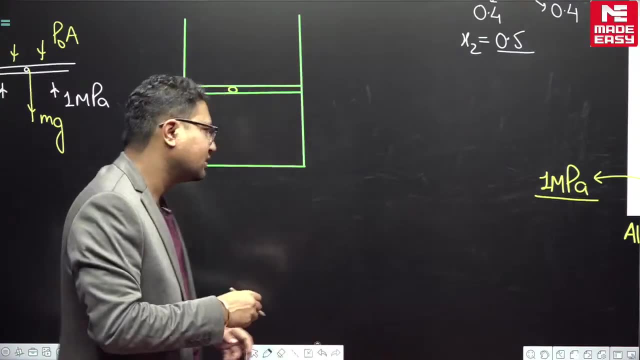 we have to solve. if we have to solve the second part, then reduction in volume. obviously we know the volume is reducing, so let me write the value. let me write the value. so V2 minus V1, I am writing minus- sign will come that means it is reduction. 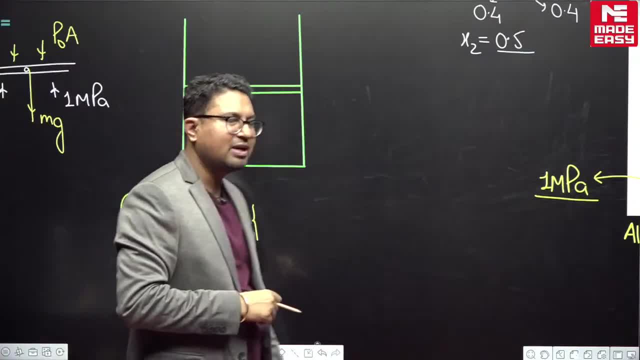 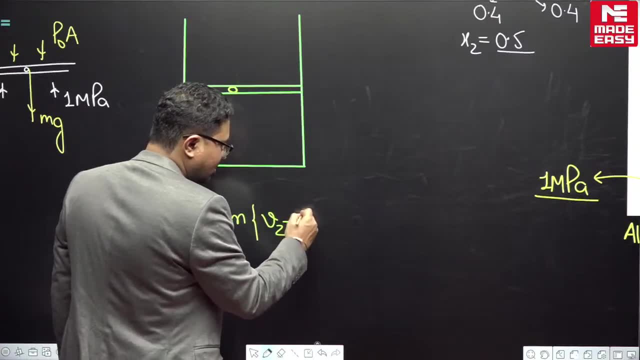 So I can write this: M mass mass. I will multiply and let me write the volume of a unit mass. So small V2 minus small V1, this will come. small V2 minus small V1, this will come so. 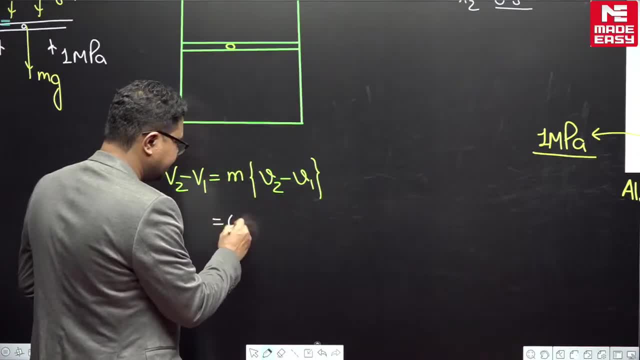 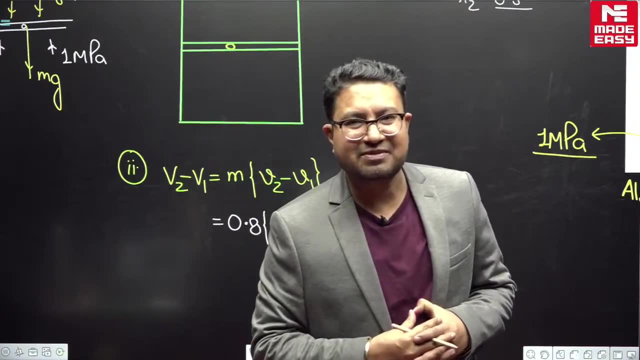 mass is. the mass is 0.8,. mass is how much? it is 0.8,. the mass is 0.8,. mass is 0.8,. the mass is 0.8.. Now, what is the specific volume for the final condition? 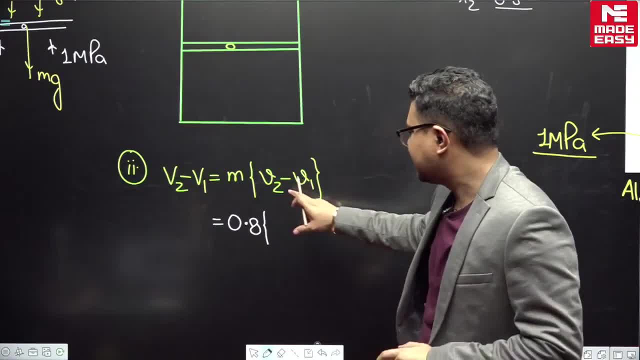 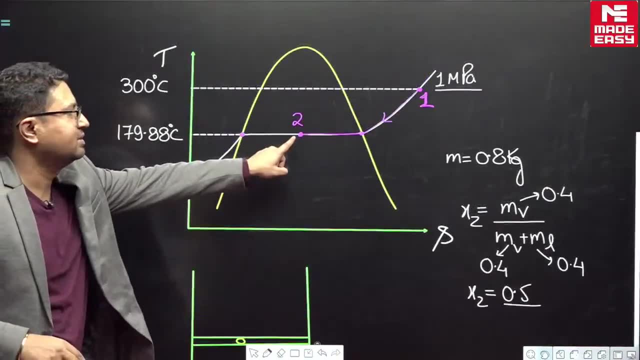 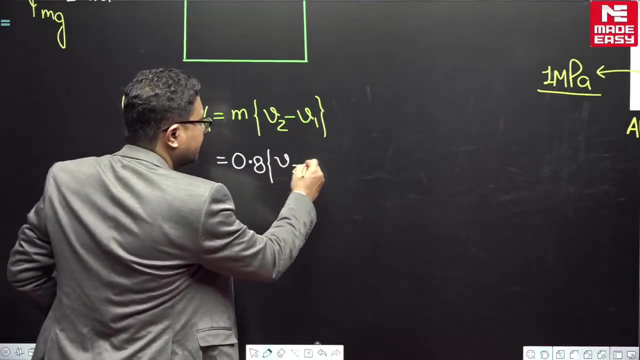 Final condition For this, the specific volume is V2,. specific volume for the final condition: V2,. this will be equal to see how we will get out V2 specific volume for this condition. the specific volume for final condition, So V2 will be equal to this- is V2 minus V1, let us calculate this, so V2 will be. 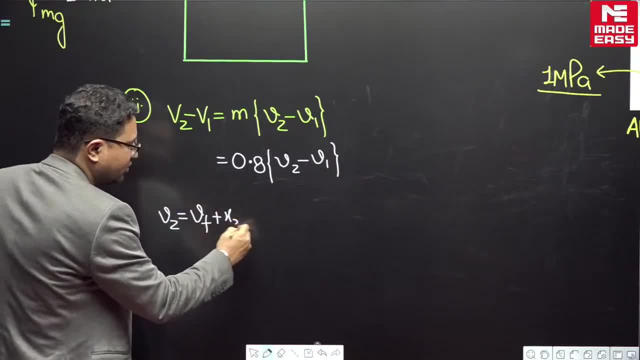 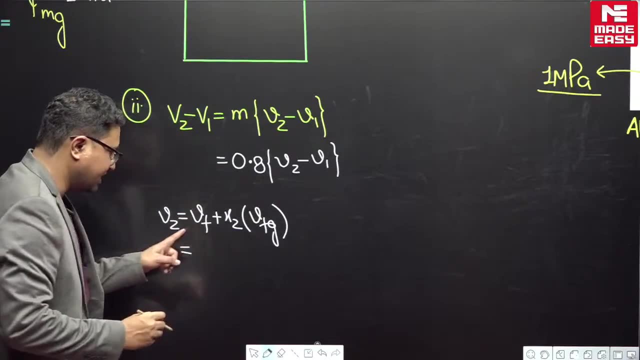 equal to Vf plus X2, into Vfg, X2 into Vfg, that is, Vg minus Vf. this will come okay. So Vf, Vf corresponding to 1 mega Pascal. we will see the data from here. we will see. 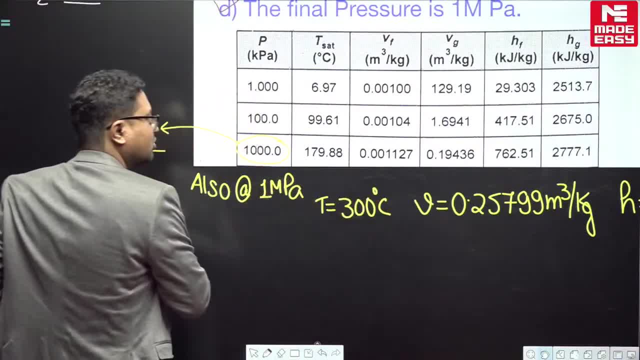 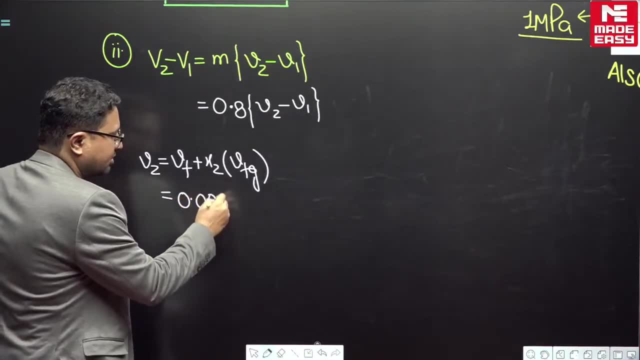 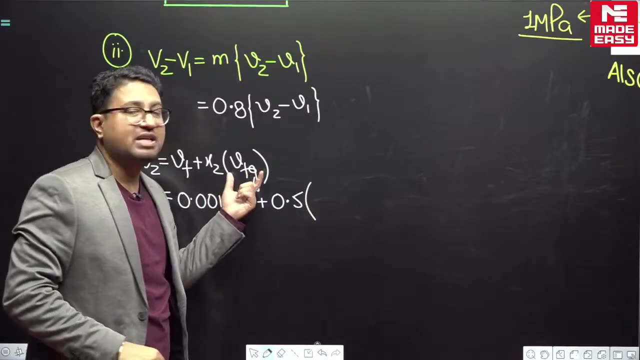 from here: 0.001127, 0.001127, so 0.00, 0.001127 plus X2. dryness fraction is 0.5, this dryness fraction is 0.5 into Vg minus Vf. what is Vfg? 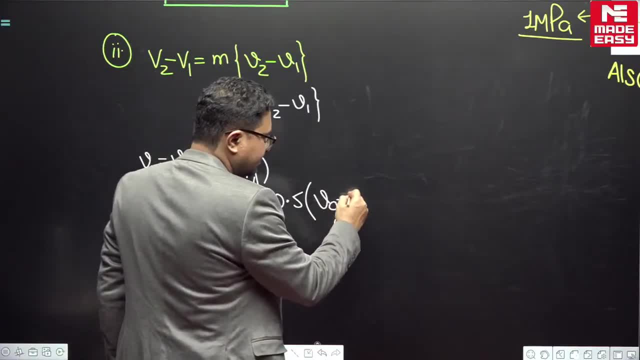 Vg minus Vf. So this is Vg minus Vf. So this is Vg minus Vf. So this is Vg minus Vf. Now what will be Vg minus Vf? So Vg minus Vf is? let me write the values here. I will write the value. 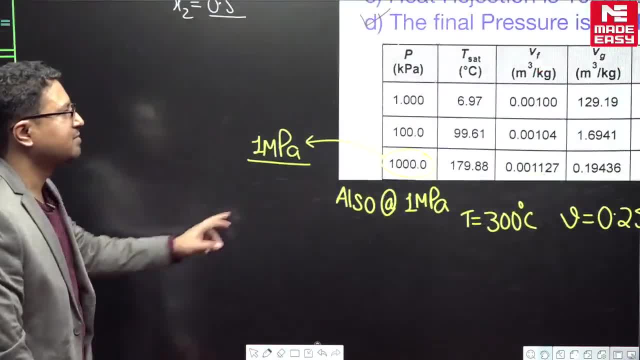 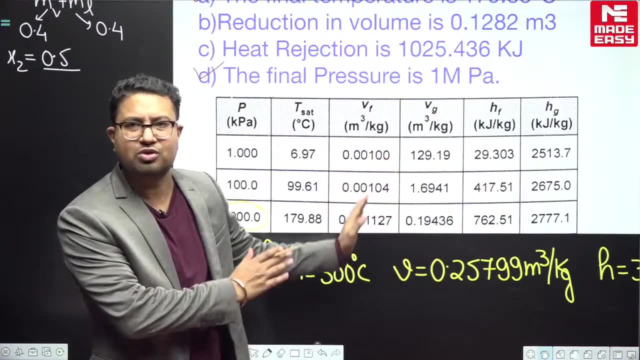 So what is Vg? What is the value of Vg? See, I have also given Vg value. I have given the value of Vg. this is the value of Vg. I will show you the question once I solve. I will show you the whole question and solution. 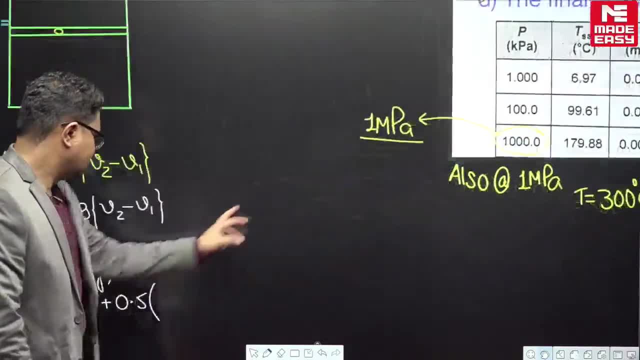 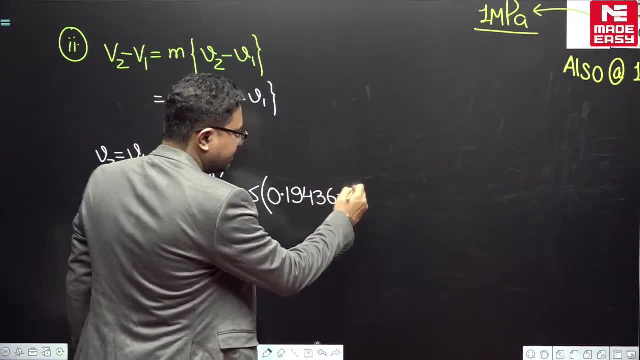 0.19436, 0.19436,. this is the value of Vg 0.19436, so 0.19436, this is the value of Vg, So 0.19436.. So this is the value of Vg. this is the value of Vg minus Vf. if we see the value of Vf, 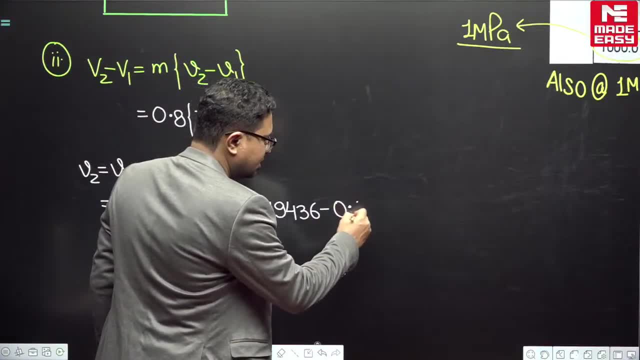 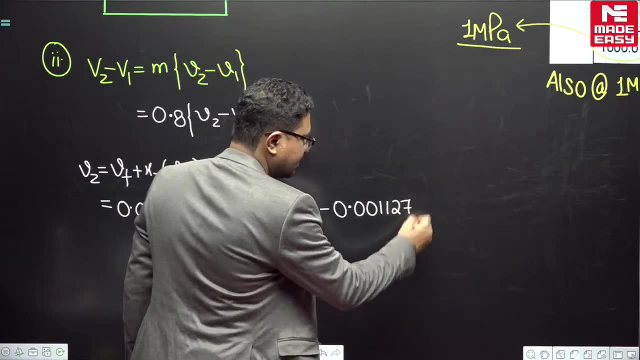 the value of Vf is already known. this is 0.00 minus 0.000001127, 0.001127,. fine, So we can write like this, we can write this, so we can write the specific volume: V2, we. 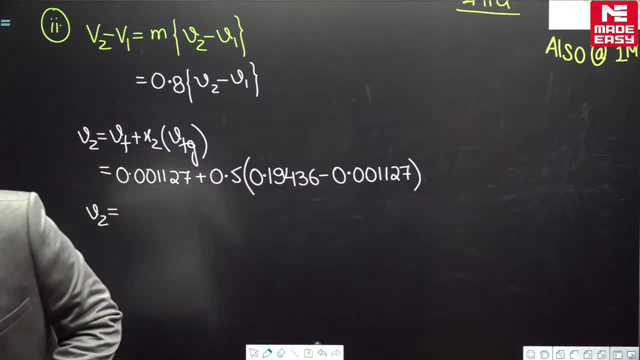 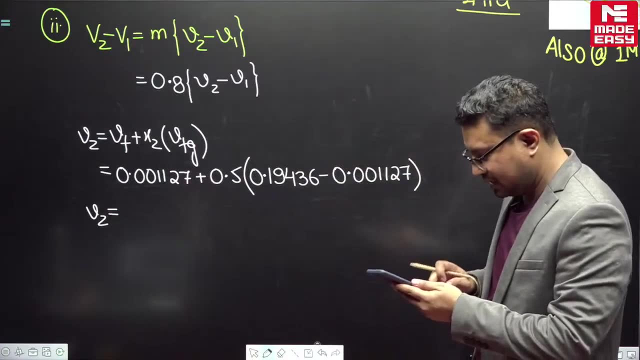 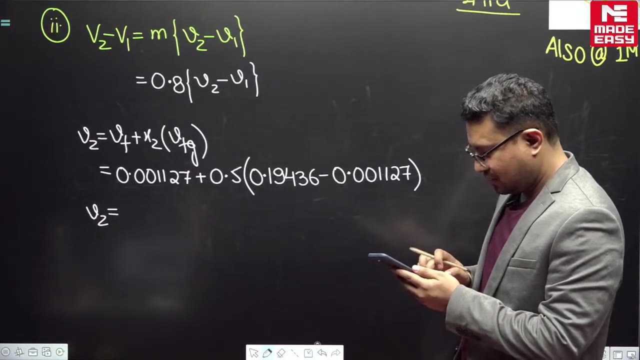 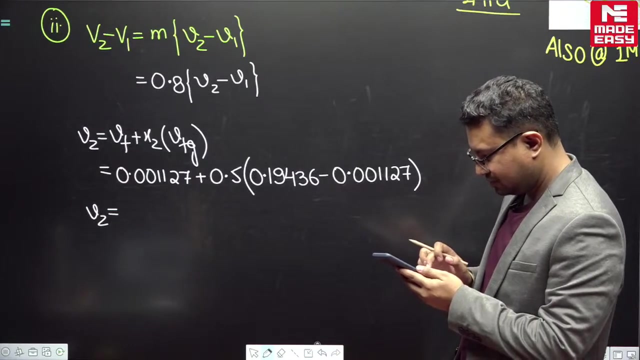 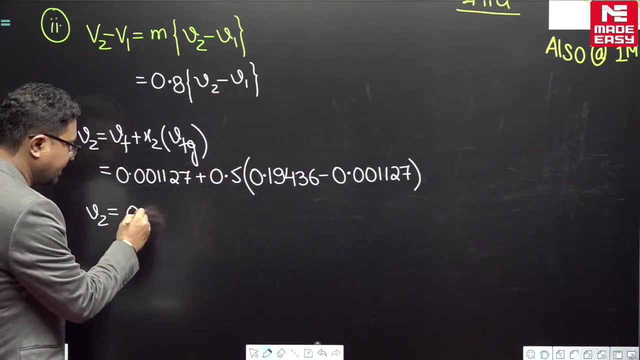 can write V2, calculate it, tell V2, calculate it. I am calculating this. calculate it and tell it quickly So we can write V2.. So we can write V2.. So V2, 0.001127 plus 0.5 into 0.19436 minus 0.001127, so 0.09777, this will be 0.09774,. 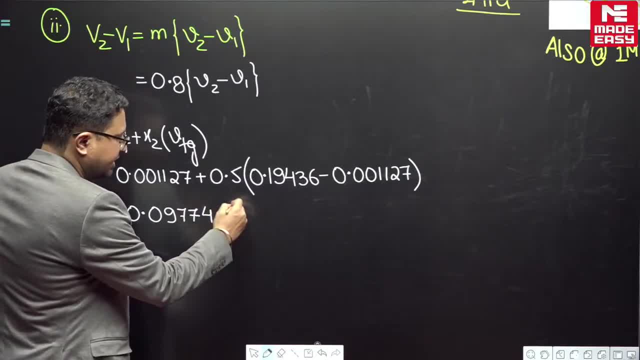 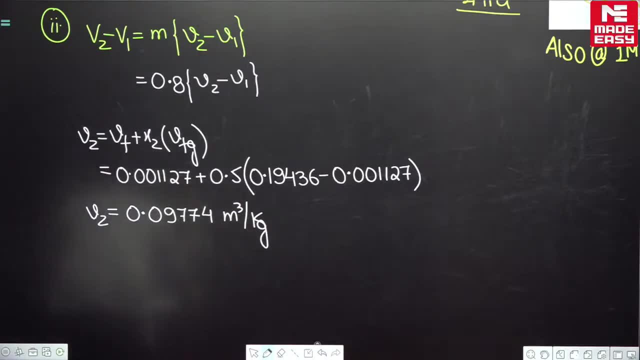 this is 0.09777.. So 0.09777.. So 0.09777.. So 0.09777,. this much meter cube per kg. this much meter cube per kg. So many people are giving the correct answers: Baha seri log, Yogesh Rai, Raju Kumar Maditya. 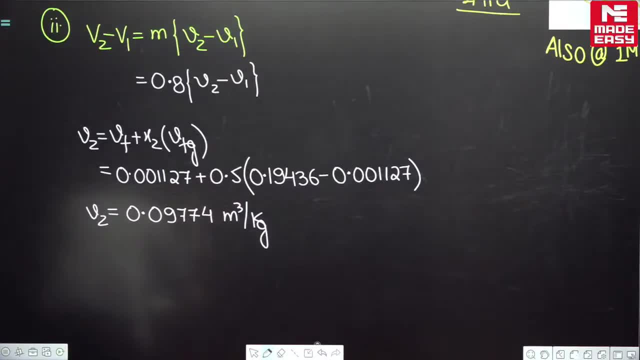 is fine. ok, you got it correct. knowledge hub: 0.00977, Raju Kumar Yogesh Rawal. very good, see, so fine Here. so V2 answer. many people are giving the answer for V2.. 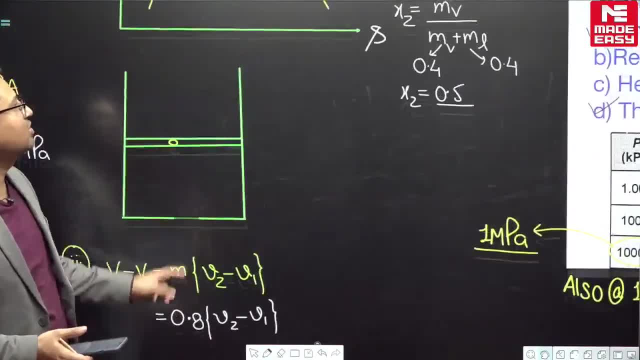 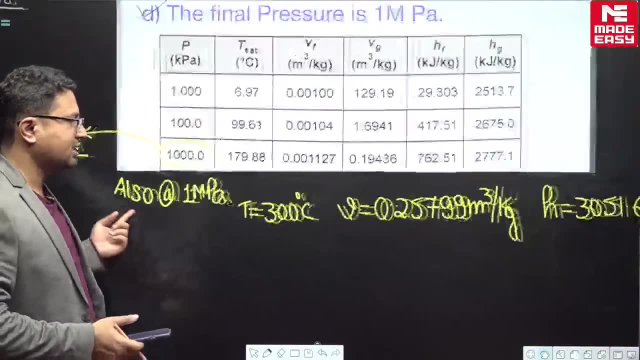 V1,. we can also see V1.. can also see V 1,. we can also see V 1, V 1 though direct, the initial condition given to us. this has been given at also at 1 mega Pascal. they have given this, this data. they. 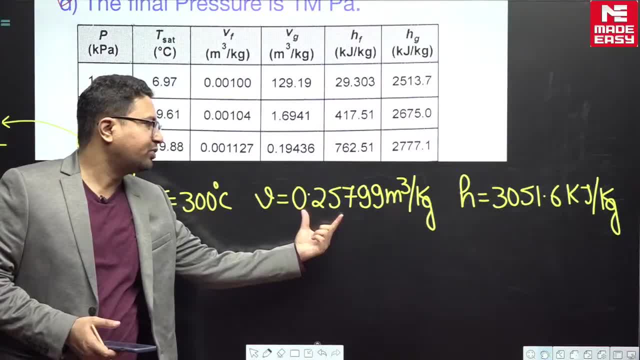 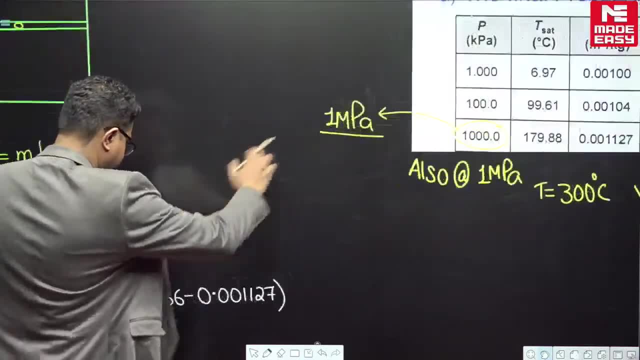 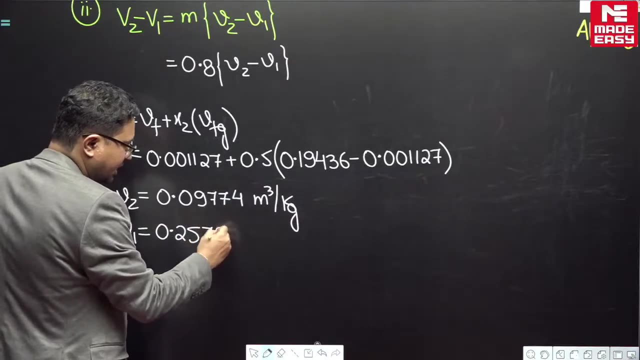 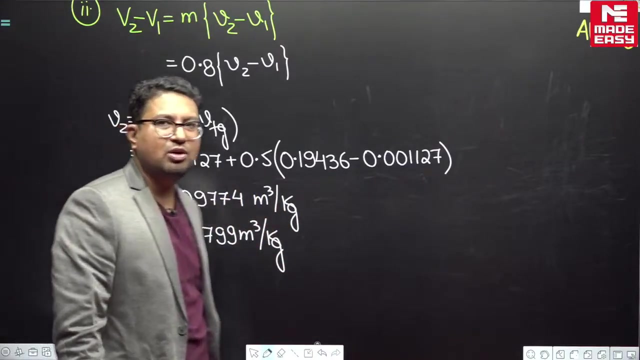 have given Specific volume is this: 0.25799 meter cube per kg, So 0.25799.. So V 1 will be equal to 0.25799 meter cube per kg. meter cube per kg. this will come, So specific volume. 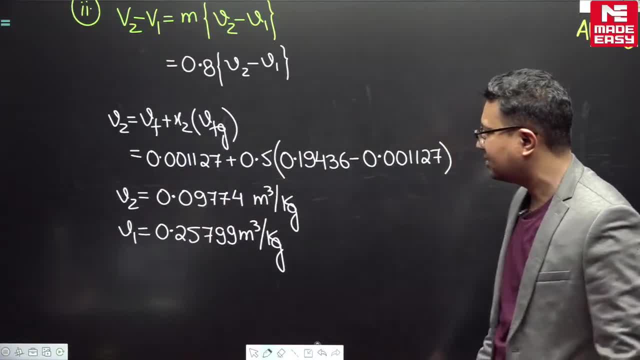 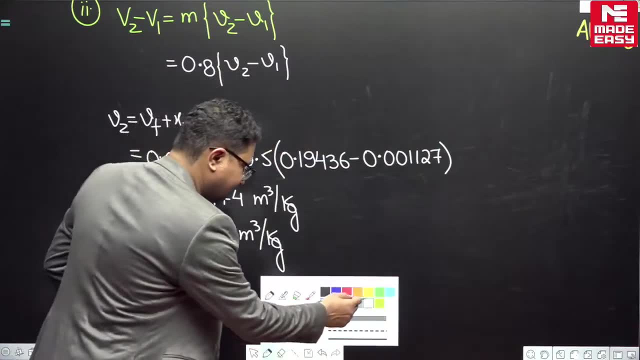 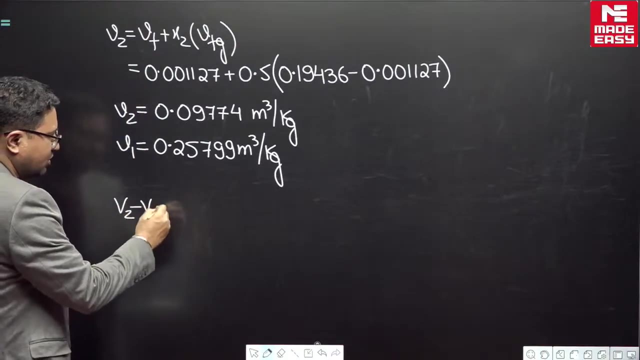 at condition 2. we know this condition for specific volume at 2, we know the condition for specific volume at 1.. Then we can say we can find out. we can find out the change in volume V 2 minus V 1.. So V 2 minus V 1 will be equal to 0.25799 meter cube per kg. 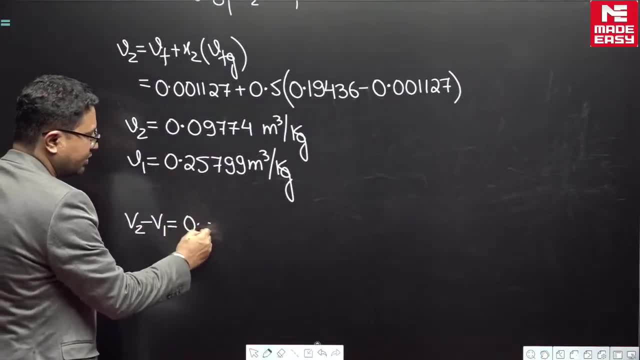 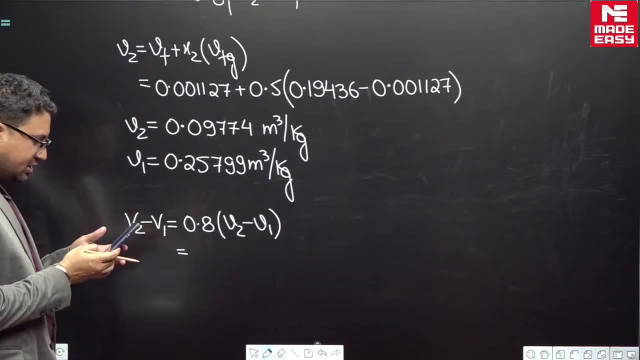 the mass: this 0.8, 0.8 into V 2 minus V 1.. So let us calculate this, this, calculate this: So this is minus 0.25799 into into 0.8, into 0.8.. luggage: so this is coming out to. 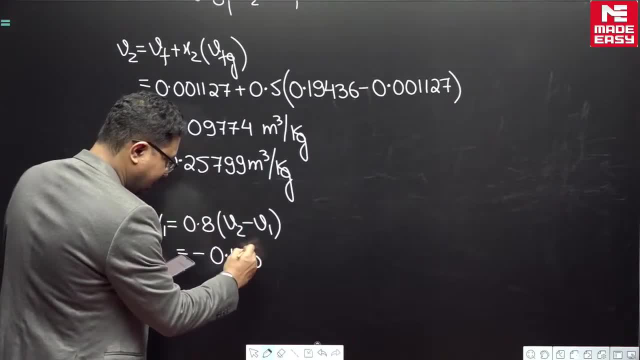 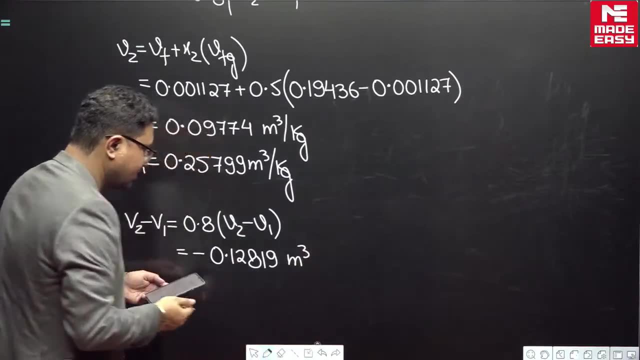 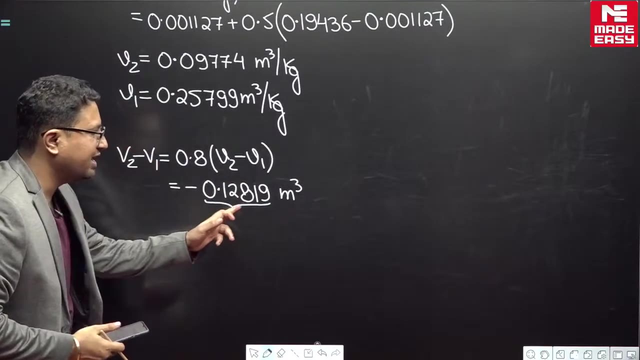 be 0.12819 meter cube per sorry meter cube because we have already multiplied the mass. So negative sign means reduction. So reduction is this much: 0.12819, 0.12819.. Now see in the option. 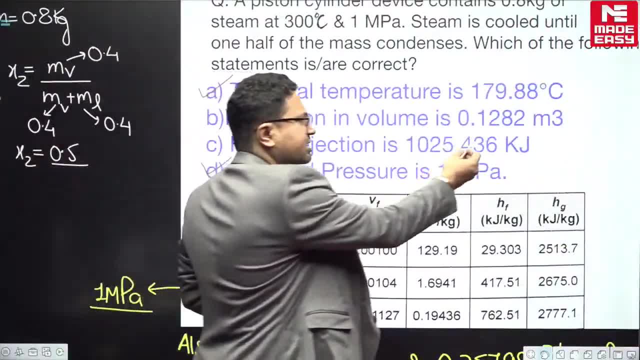 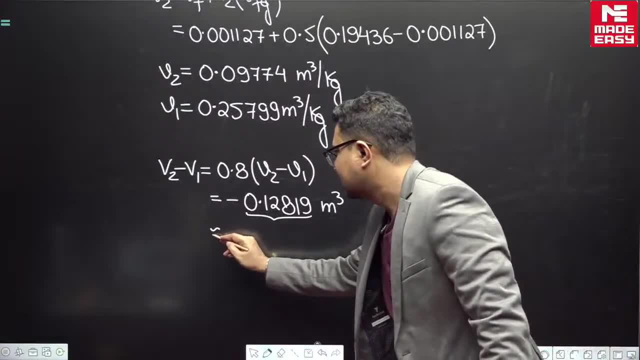 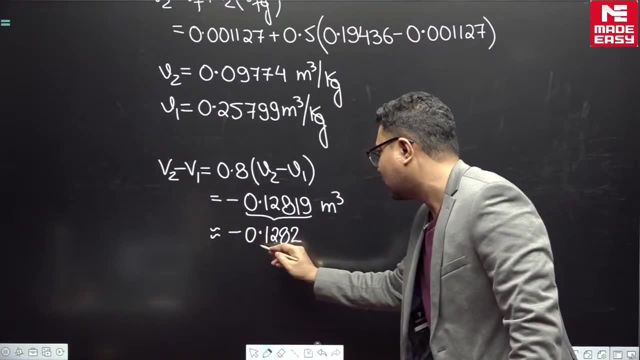 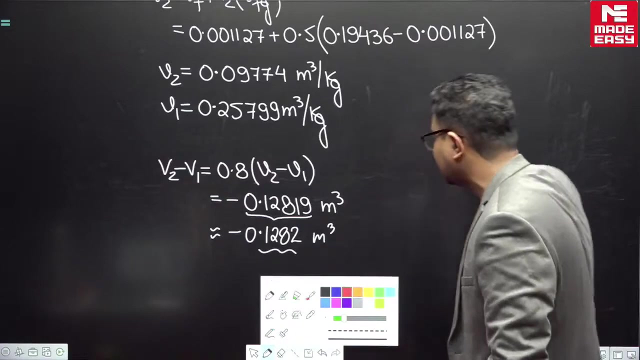 what is given: 0.12819. this is correct. round off: 0.12.. So we can almost write this, as we can almost write this, as we can almost write this as minus 0.1282. we can almost write it like this: this much meter cube. So the option B is also correct. option B is also. 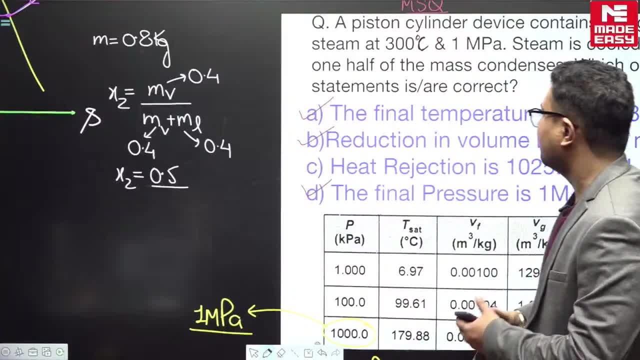 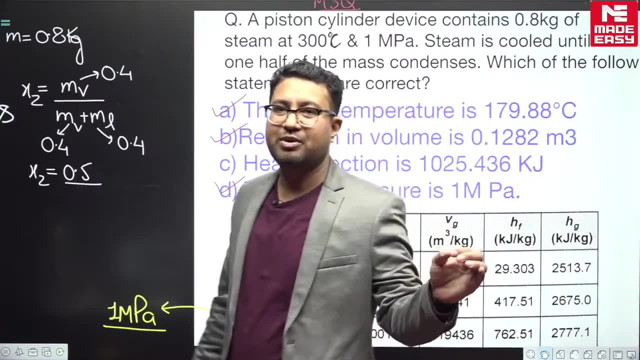 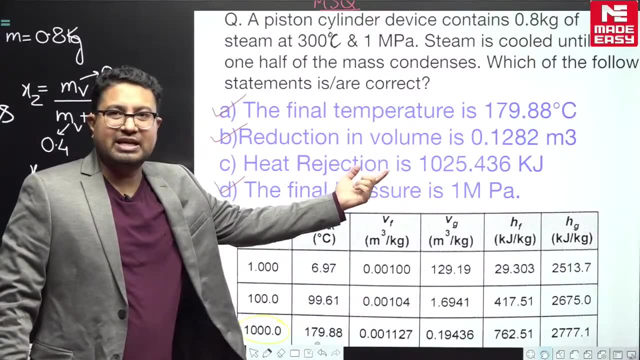 correct. option B is also correct. this is also correct. Then what we have to find out: heat rejection is 1025.436, heat rejection: 1025.436.. This is what we have to find out. So we will understand this. Pressure is constant, So 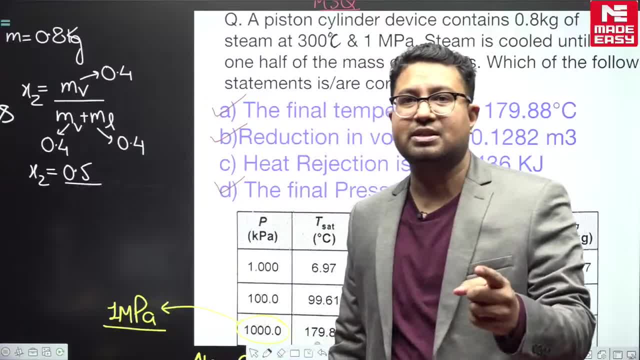 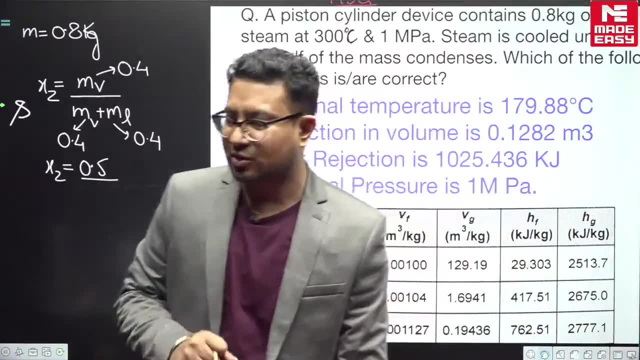 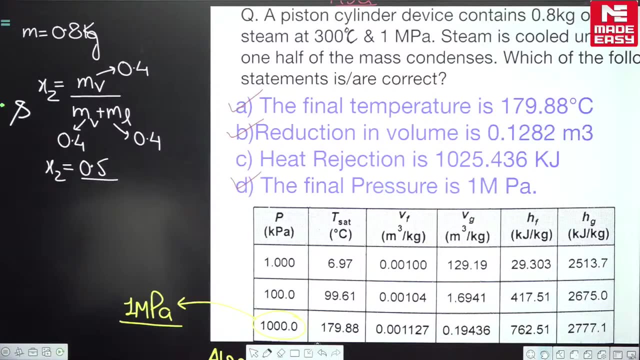 heat rejection at constant pressure or heat interaction at constant pressure is change in enthalpy change. So we will have to find out the enthalpy change. Find out, Yogesh Rai, Mukesh Kumar Raj gaming. fine, You are giving the correct answers. 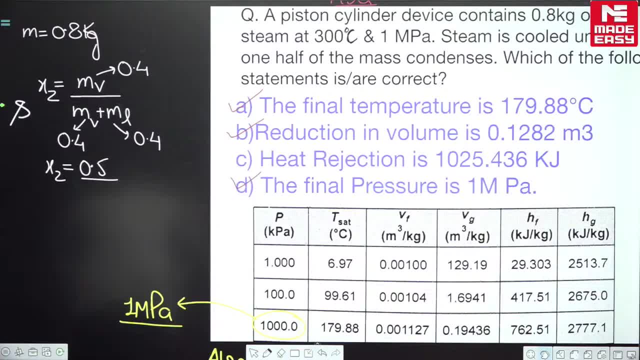 I think answer very good, You are giving the correct answers. good, Now next, let us see. next. dekhte hain The enthalpy change, enthalpy change. dekhte hain. Let us find out: the sorry enthalpy change, enthalpy change. dekhte hain. 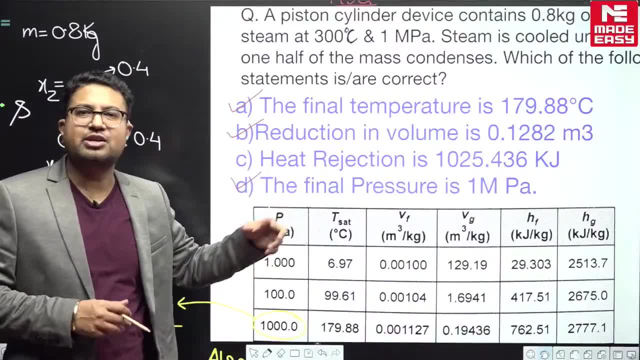 So now we have to find out the heat rejection, So heat rejection at constant pressure hain. that is why I am saying, I am saying this is the enthalpy change. enthalpy change ke bharabar ho jayega. 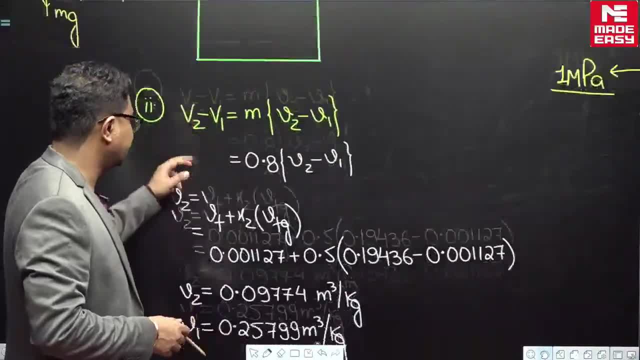 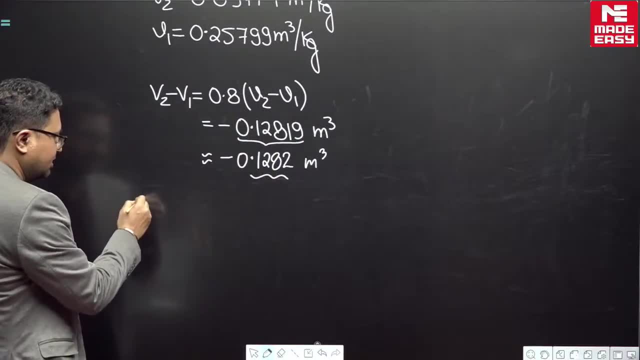 So see, this is enthalpy change. enthalpy change ke bharabar ho jayega. So see, this will be So: constant pressure pay. heat rejection at constant pressure. this is second. this is the third. third part. third part. third part is heat rejection at constant pressure. 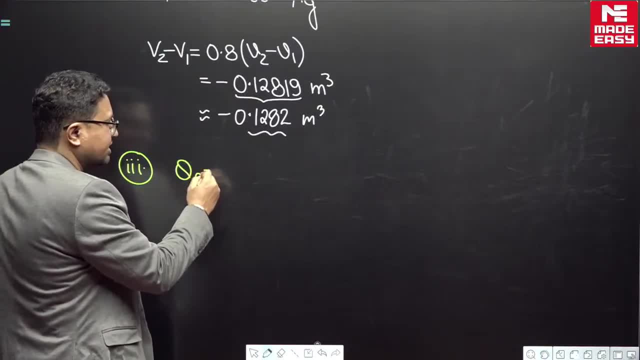 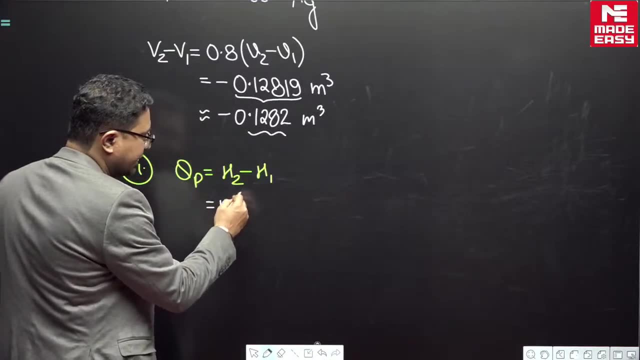 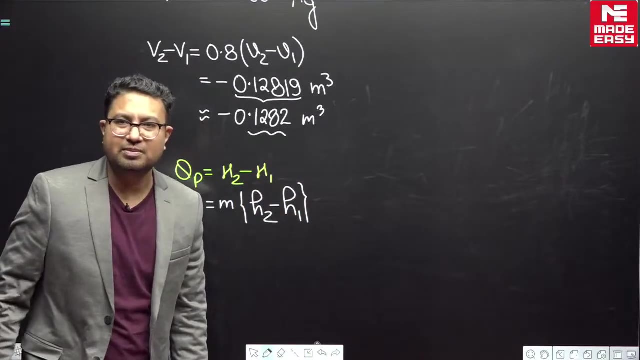 So constant pressure heat interaction. constant pressure heat interaction is equals to H 2 minus H 1, enthalpy change. this can be written as M mass into enthalpy per unit mass: H small 2 minus H small 1.. 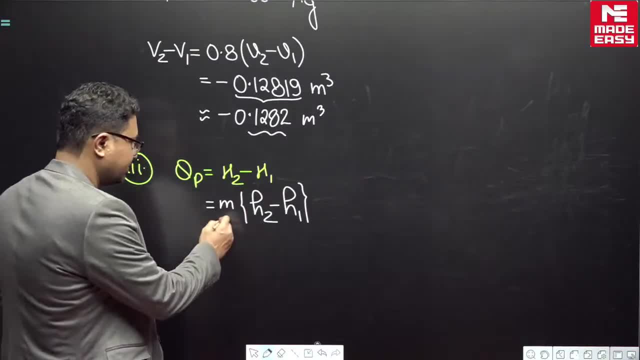 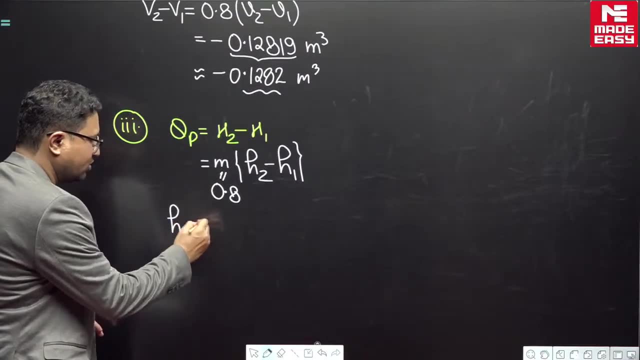 So let us we know the mass is 0.8, let us calculate H 2 and let us write H 1 also, this is 0.8.. So H 1, H 1, see what will happen. H 1 is already known. value is directly given value. 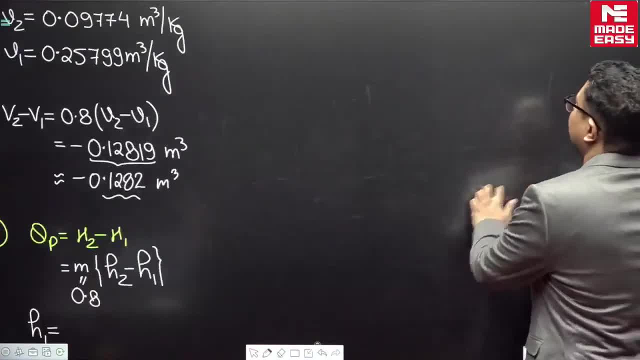 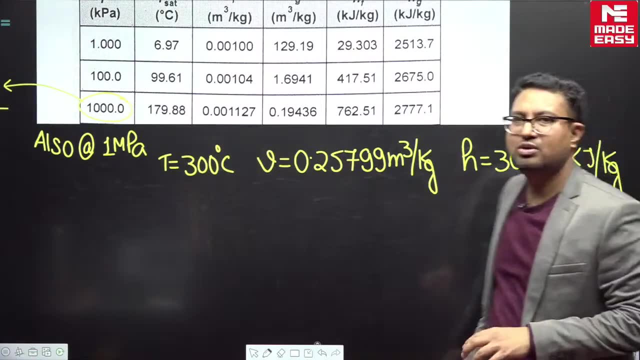 is directly given for initial condition. So let us write this value from here. let us write this value from here directly, given 3051.6, 3051.6,. this is the value given directly, direct value given 3051.6.. 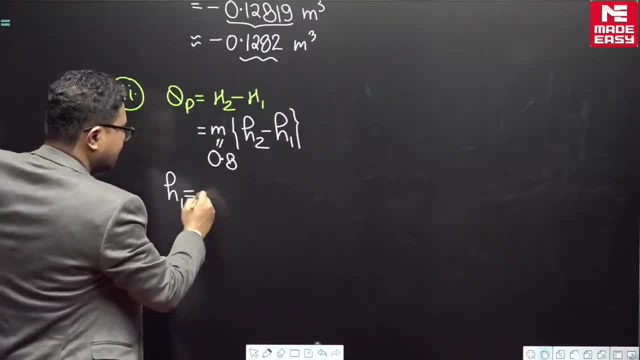 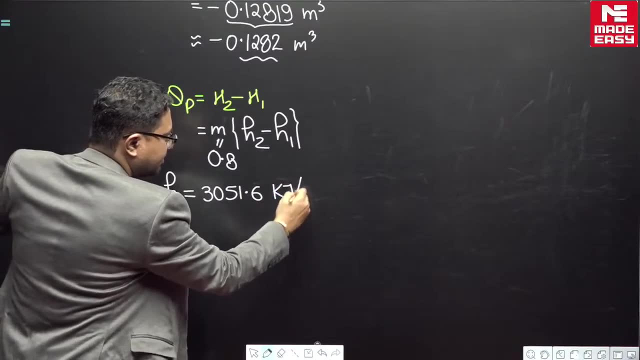 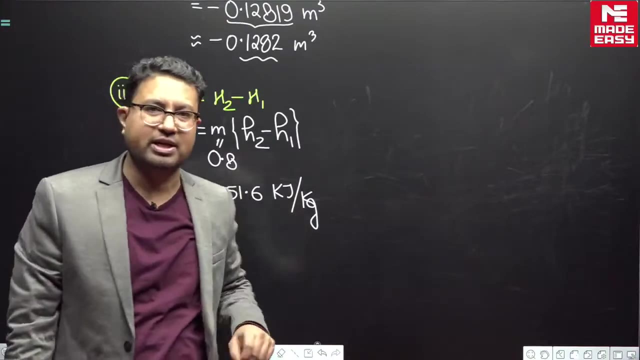 So we can write this. We can write this: 3051.6 kilo joule per kilogram. kilo joule per kilogram, this is given. then if we write H 2, if we write H 2, so we will write: H 2 is in the wet region. 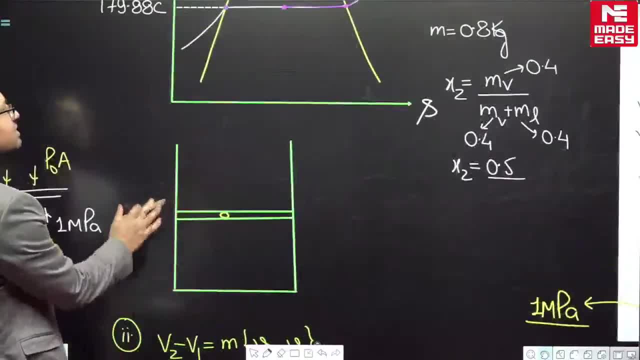 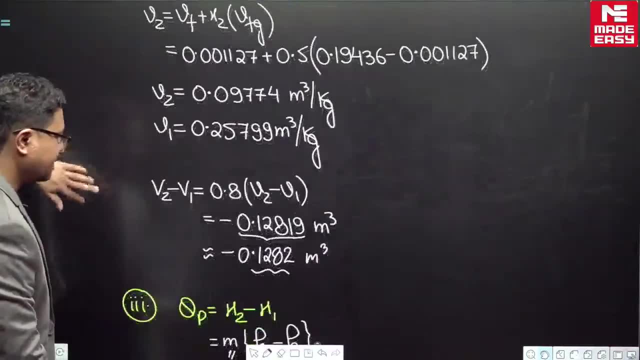 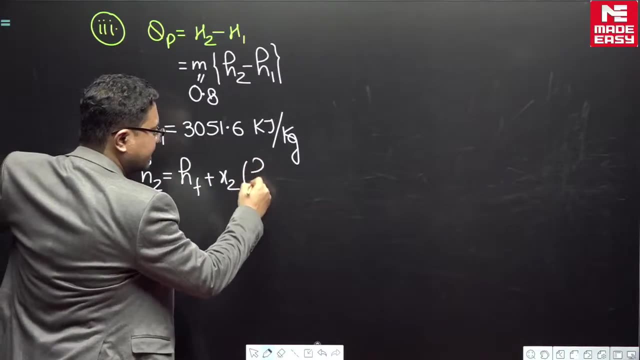 wet region. see here: 0.2 is in the wet region. this is in the wet region here. so H F plus X 2 into H F G, H F plus X 2 into H F G. We will write this: so H F plus X 2 into H F G, that is H G minus H F, H G minus H F. 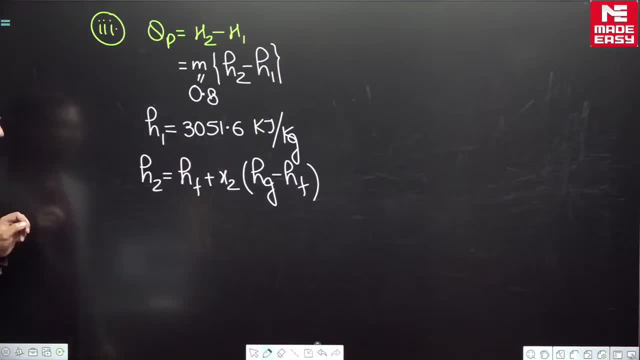 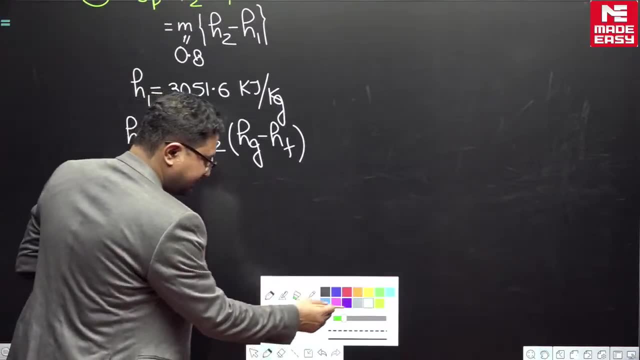 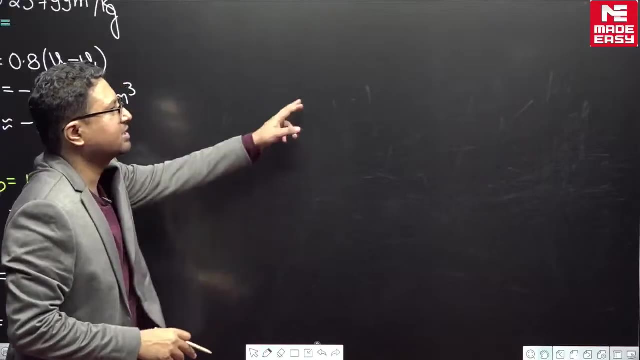 we can write like this. we can write this: okay, So H F plus X 2 into H F G. now see, X 2 is known H F. let us see, let us write H F, the value of H F. let us write, we can write it from here: we can write H F value. so this: 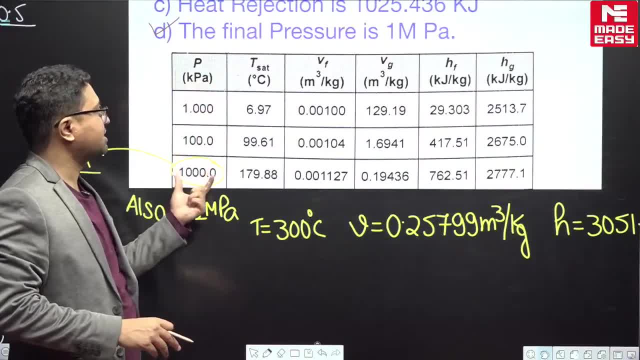 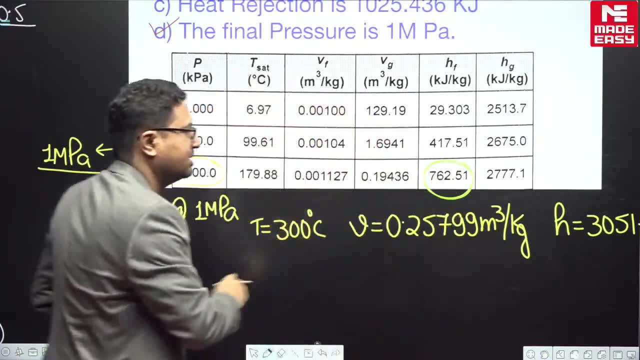 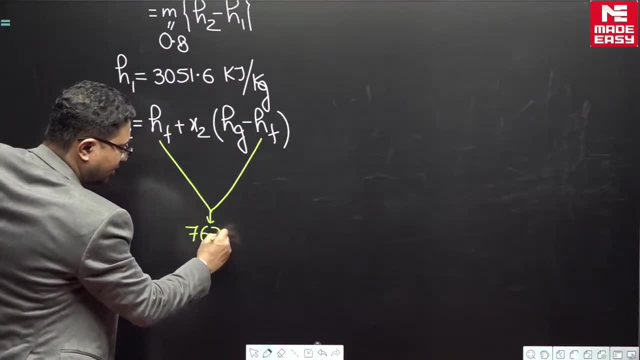 is the hf value. 1 mega pascal per hf 762.51- 762.51- this is 762.51, fine. so 762.51 is hf 762.51 kilo joule per kg- this is hf, fine. dryness fraction x is 0.5. we already know. 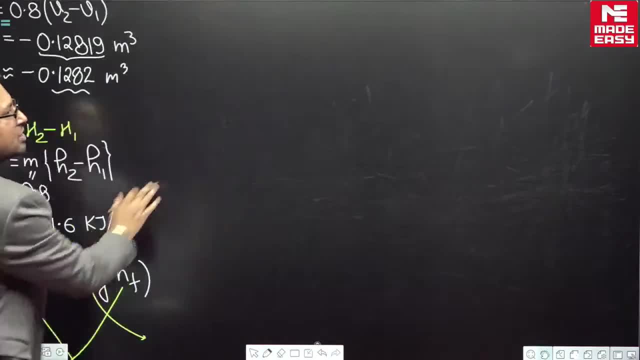 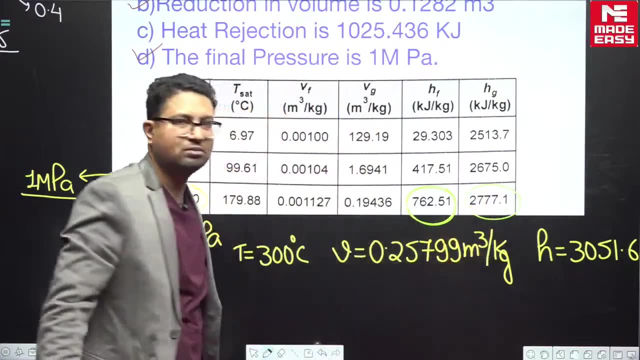 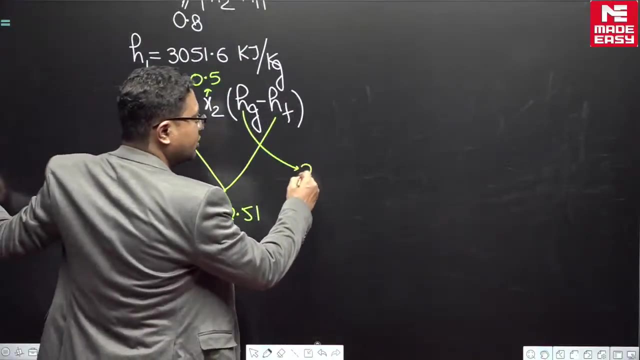 this, we know: hg, hg. see what will happen. hg, so we can write hg also. hg can write: hg is 2777.1, 2777.1, 2777.1, so hg will be 2777.1, hg will be 2777.1. this will be hg, so we can. 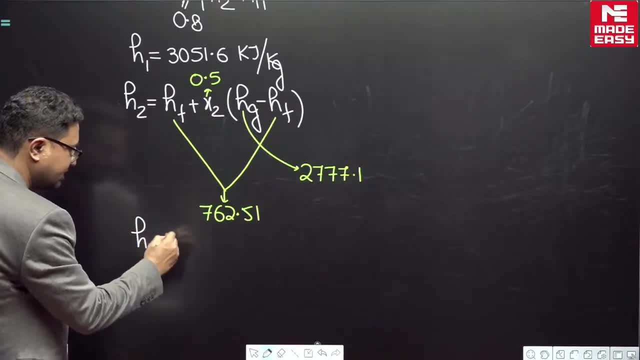 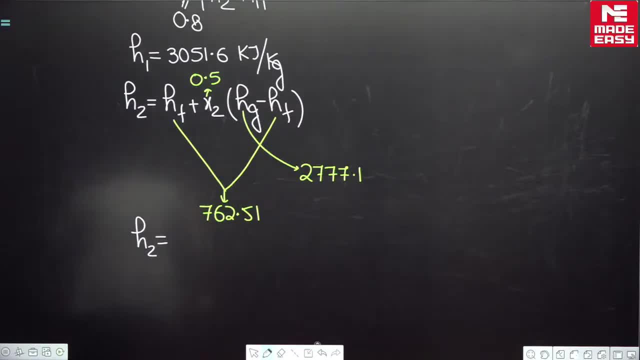 the value of H 2.. Saurav Chauhan, you are asking how to physically visualize reduction in volume When the vapor will reduce. same mass of vapor. same mass of vapor occupies more volume. So when the vapor will change into liquid the volume will reduce because same mass, if it is in the 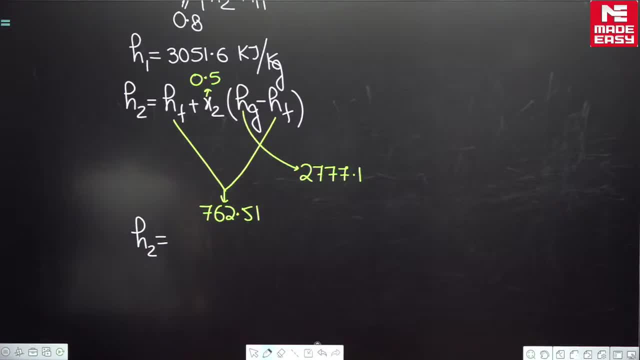 liquid state will have less volume. if it is in the vapor state will have more volume. So just let me know, Saurav Chauhan, you understood it or not? just let me know. So we have this nice. So H 2, let us calculate the value of H 2.. So H 2 is H F 762.51 plus this is 0.5. 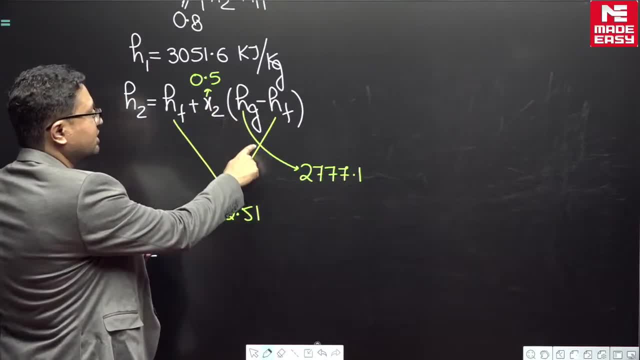 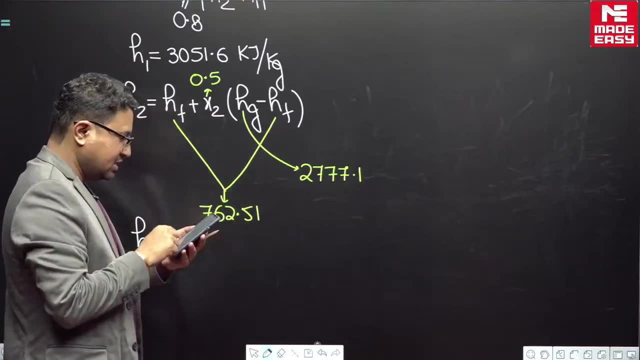 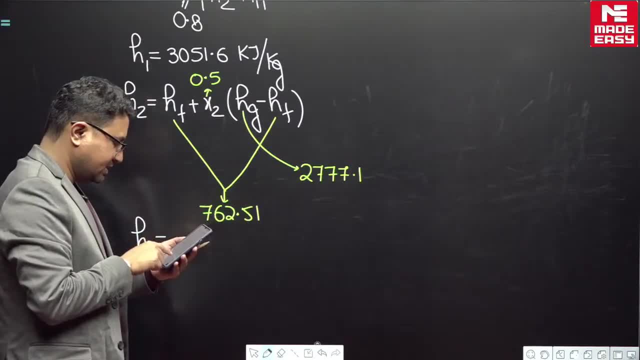 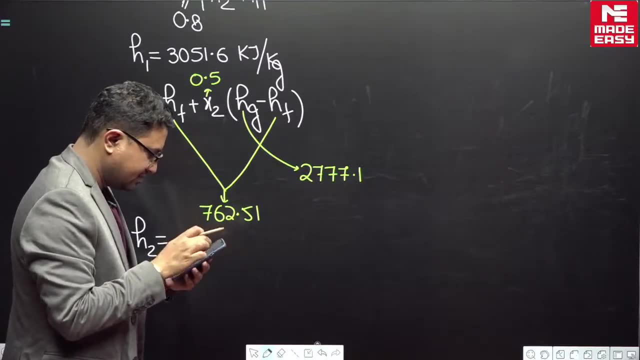 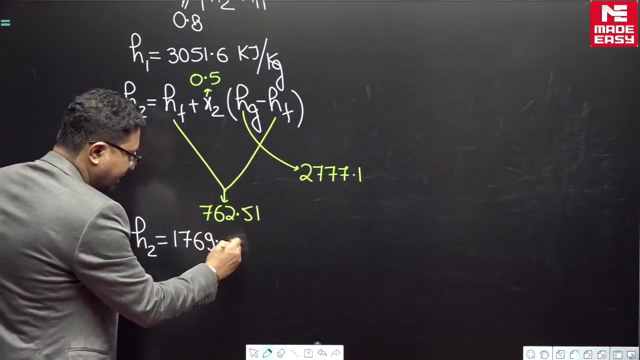 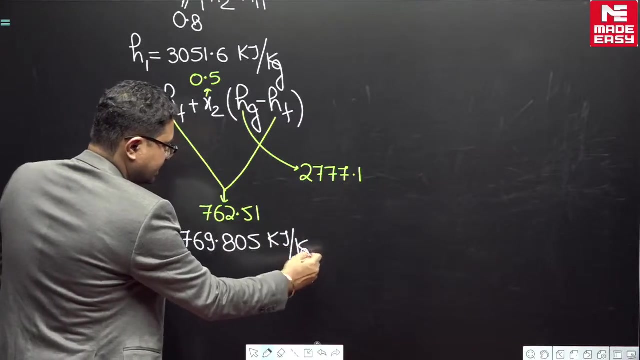 2777.1 minus H F. H F is 762, 762.51.. So we are getting. we are getting 171769.805, 1769.805 kilo joule. this is kilo joule per kg: 1769.805, 1769.805. very good. 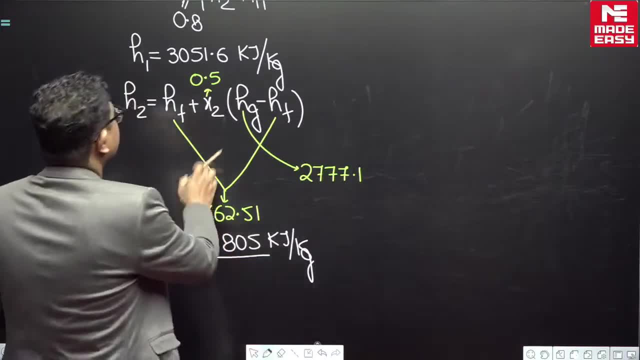 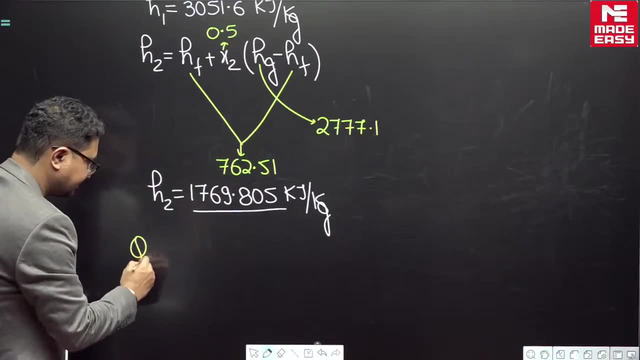 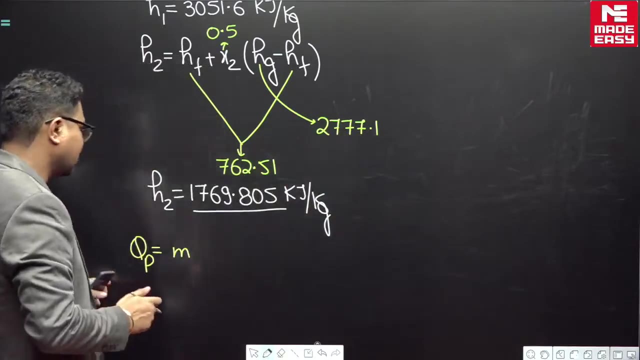 So this is the answer. fine, So now we have to calculate the heat supply. So heat supply is H 2 minus H 1 heat supply at constant pressure. It is actually heat removal, heat removal to heat rejection. this is the heat rejection because you are converting the steam into 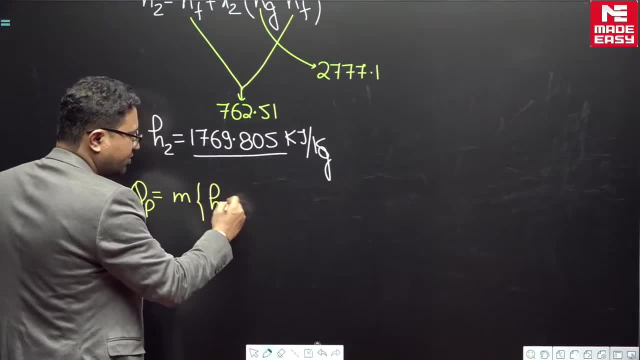 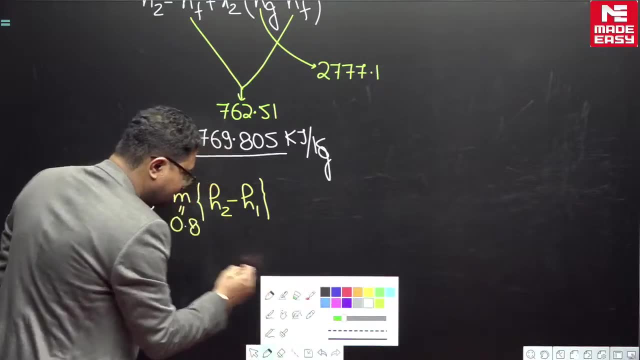 liquid. So this is H 2 minus H 1, and mass is 0.8, 0.8.. So find out negative, it will be negative, But tell me the answer. calculate this so: 1769 point 0.805 minus H 1, H 2 minus H 1.. So. 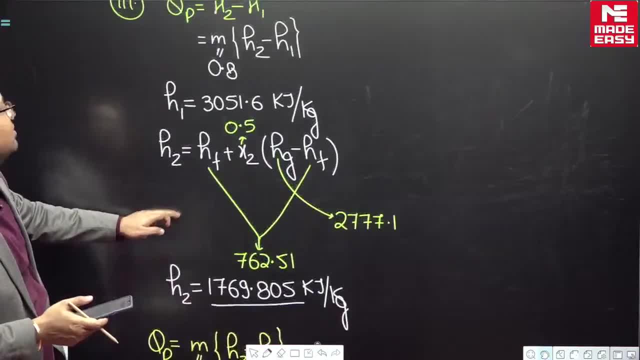 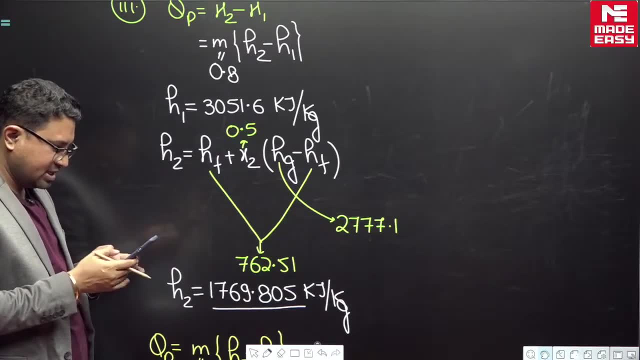 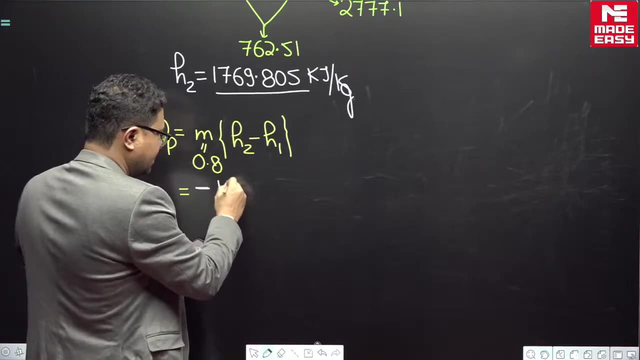 H: 1: we already know 3051, 3051.6. this is this into into 0.8, into 0.8.. So it is minus 1025, minus 1025.436.. E O: 0: 0, 0.8.. 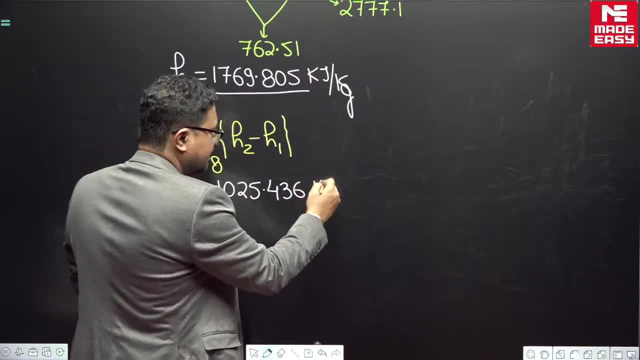 So so that is 0.8.. E O 0, 0, 0.2.. E O 0, 0.2.. E O 0, 0.2.. this much kilo joule is heat rejected, So heat rejected, so heat rejected will be heat. 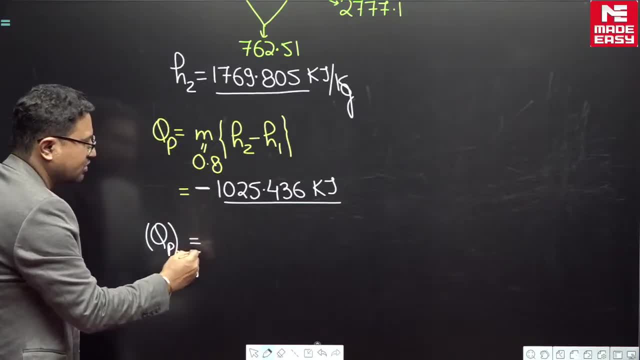 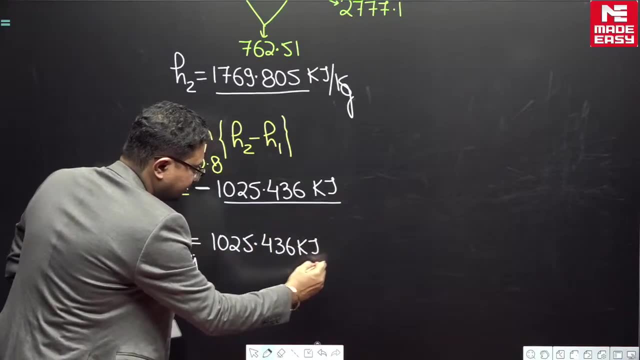 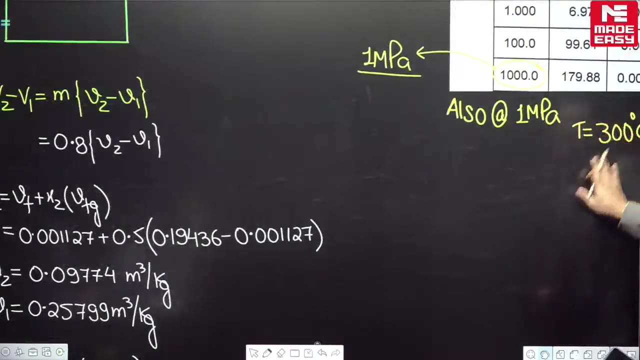 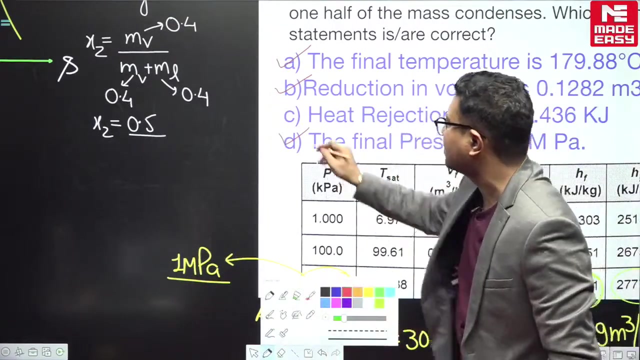 at constant pressure, which is being rejected. this is equals to 1025.436 kilo joule. 436 kilo joule- fine. So we can. we can here see 1025.436 kilo joule, So this is also correct. this is also. 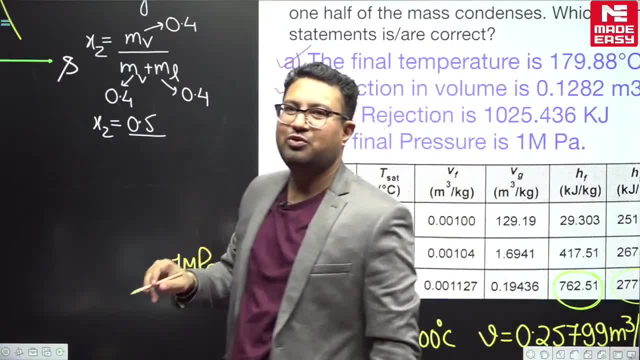 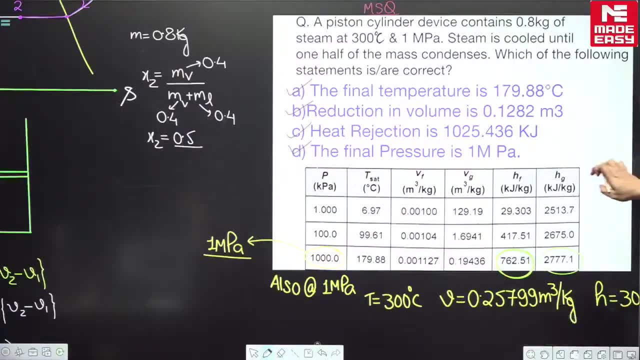 correct. this is also correct. So we have all the four options correct. all the four options are correct. So we have solved this. we have solved this. all the four options were correct. So just see the question here. question: see, if you want to note down, I will just show it on the screen and 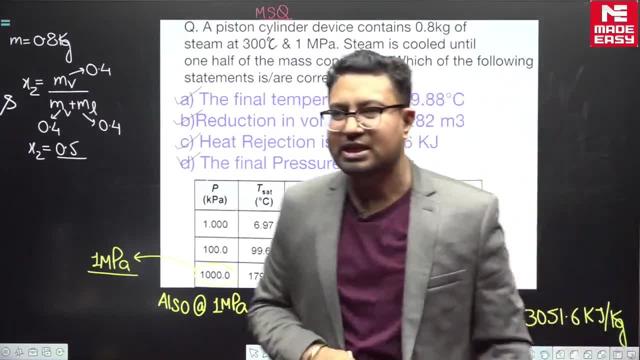 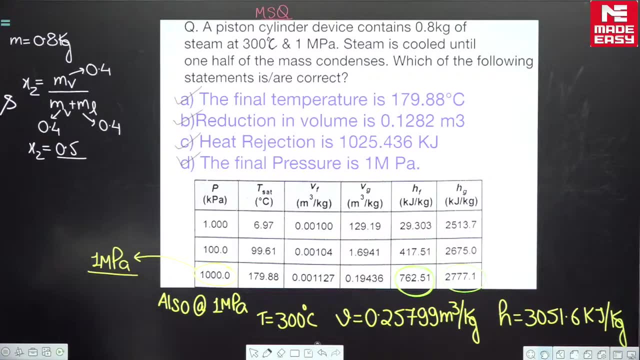 then I will show you this So solution. I will show you its solution also. just see the question here. question: see So Prabhat fine. Anuj Kumar Sai. Anupam Tomar correct. Shailesh Kumar Loni correct. Yogesh Rai correct. 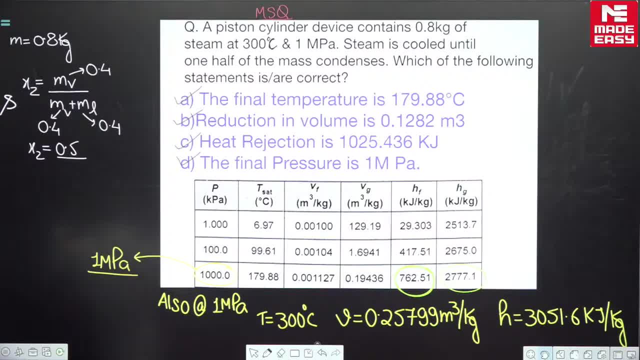 fine, Shashikant Gautam, you also calculated correctly. fine. So see, when the temperature changed, The never Hakana was, it is not change in sleep. replace face: edge of区 war. that is called as sensible heat, So sensible heat. and when the phase change is taking place, that is called 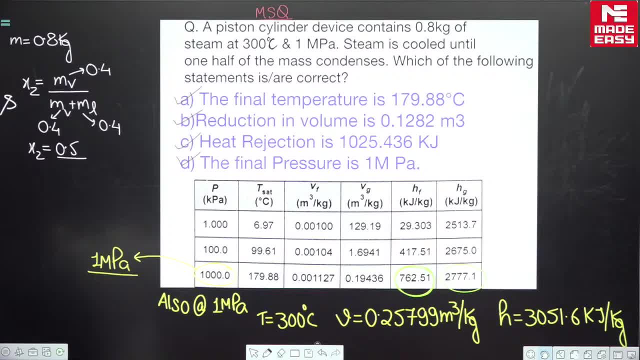 as latent heat. that latent heat that is called as latent heat, that is called as latent heat, sounds good. That is called as latent heat. heat rejected. whatever is the heat rejected, The heat rejected. there will be heat rejected. bring down the temperature from 300 degrees Celsius, 100 to 179.3°. 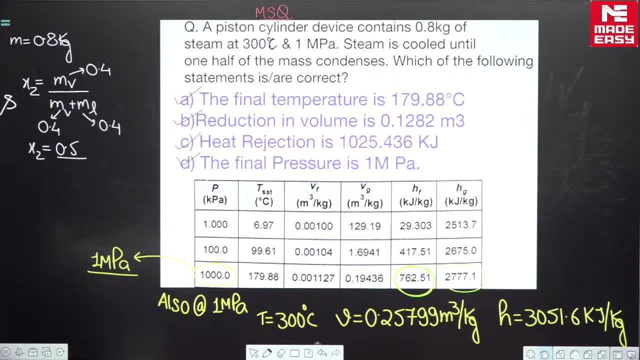 179.88 till 179.88, there will be heat rejected. that will be sensible heat. that will be sensible heat. after that, further heat rejection will happen. so that will be the phase change. phase change will happen, Nishant Singh. yes, both will happen. there will be both, there will. 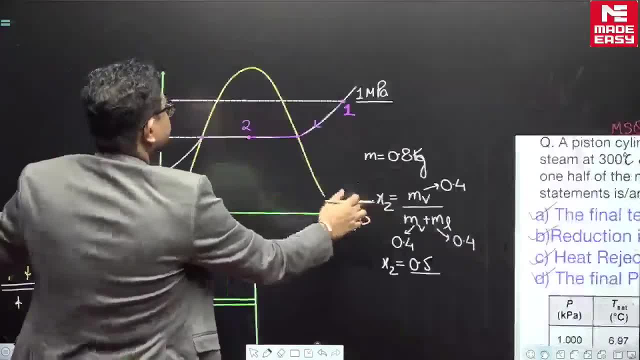 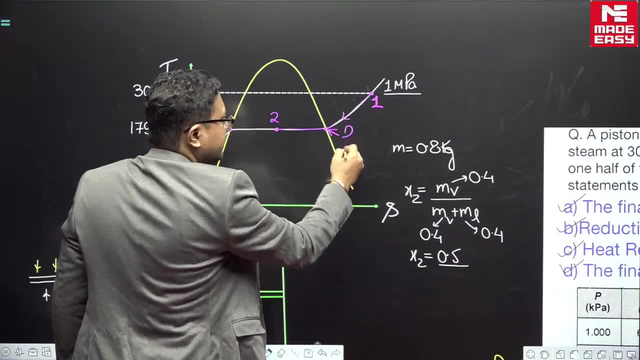 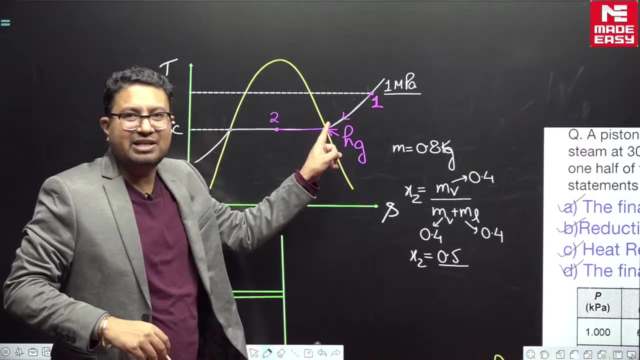 be both. both will happen. see, from here to here, if you are asked. if you are asked, suppose in this question this is Hg, this is Hg, Hg. so H1 minus Hg, H1 minus Hg is the heat rejected to bring down the temperature. suppose in this total heat is given. if we have to find 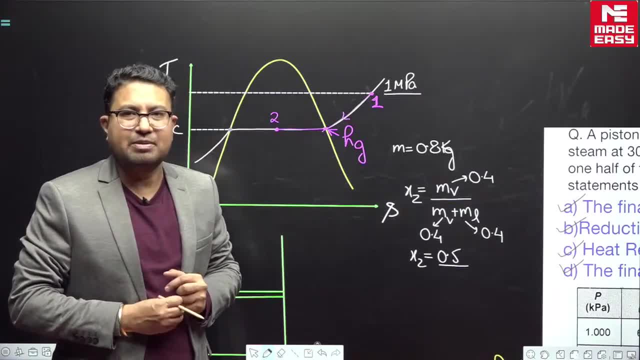 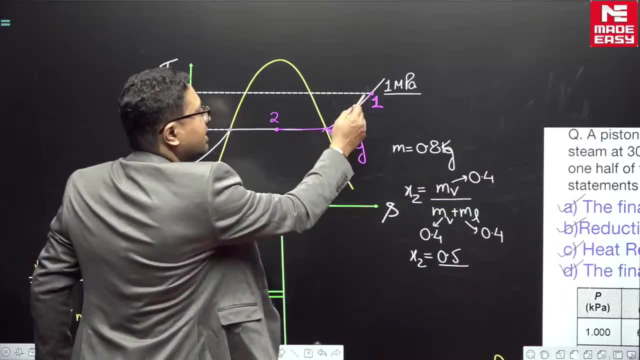 out the sensible heat. if you want to find out the sensible heat in this, if you are asked in the question that this is the amount of the sensible heat which is being rejected and this is the amount of the latent heat, so from one to this is the sensible heat and 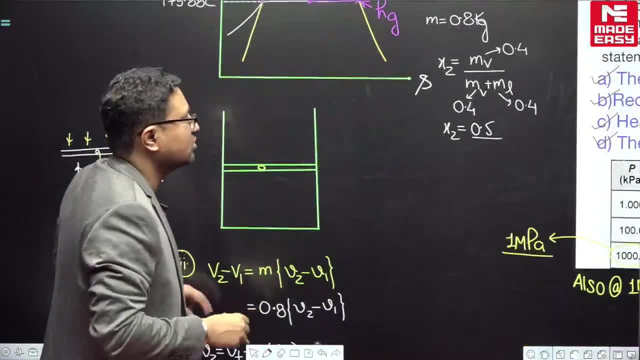 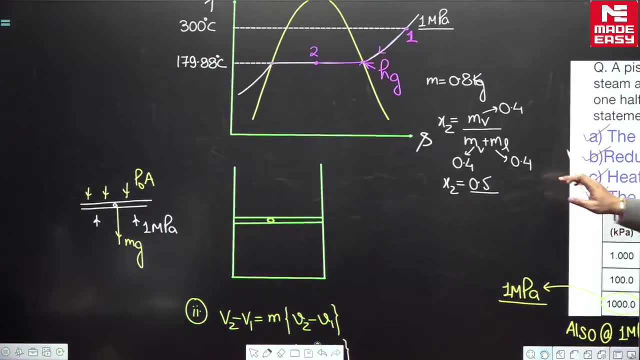 this to. this is the latent heat. let us calculate. so let me just show you. you take out and tell me quickly. i will just show you the solution, if somebody wants to note down this. so out of the total heat rejected, total heat rejected may say: tell me the sensible heat and the. 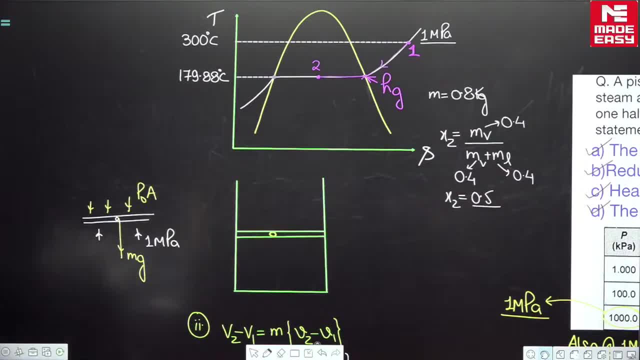 latent heat. i just told you how we can calculate it. how can we calculate? you can take it out quickly. tell me how we can calculate the sensible heat. Nishant, clear sir, thank you fine. So let us calculate also. Nishant Singh, let us calculate also, this is calculated. we calculate what is the total? 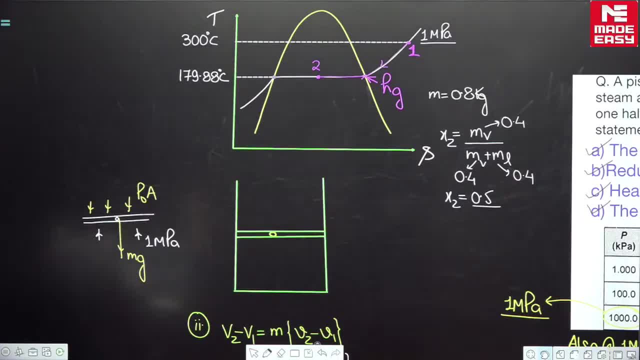 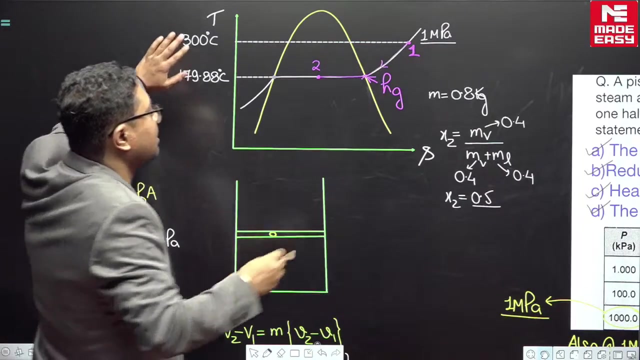 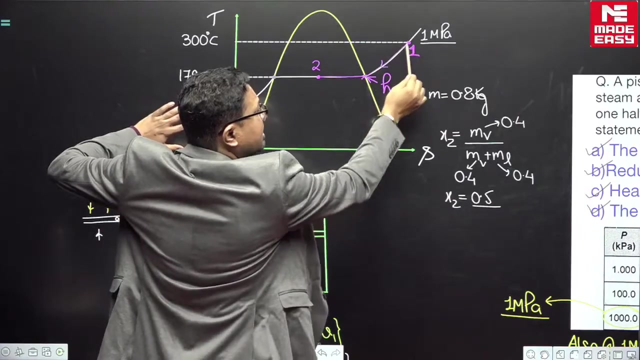 part which we have to. I mean write for the sensible heat as well as the latent heat, sensible heat or and the latent heat. So now see, now see, we will find out. we will write this: H 1 minus H g is the sensible heat. this is to reduce the temperature. we will reject H 1. 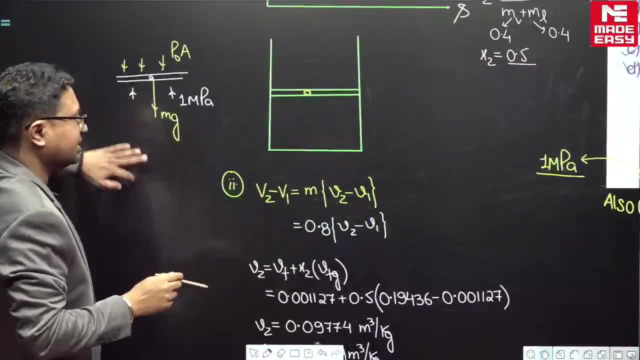 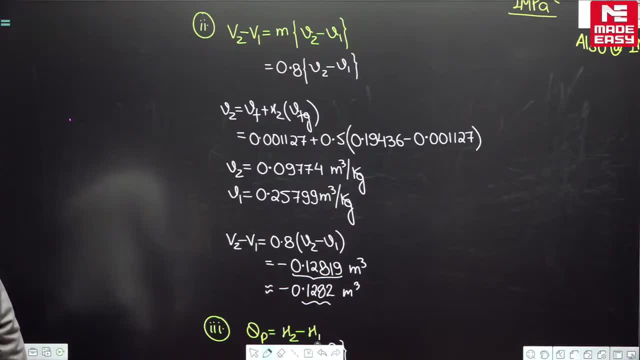 minus H, g. So sensible heat, look sensible heat. I will just show the solution if somebody wants to write, or the people Solving quickly. they tell me how much is the sensible heat? Rajgaving, you gave the answer, but tell me whether this is sensible heat or latent heat. you tell the value you have. 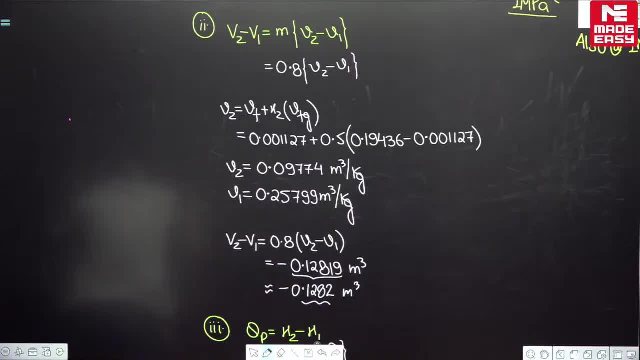 written the answer. 219.6. Aryan Kumar, you have also written the answer, but also parallely. you also tell the parallely that this is the sensible heat or latent heat. which answer you are telling parallely also mention this. mention this also parallely. 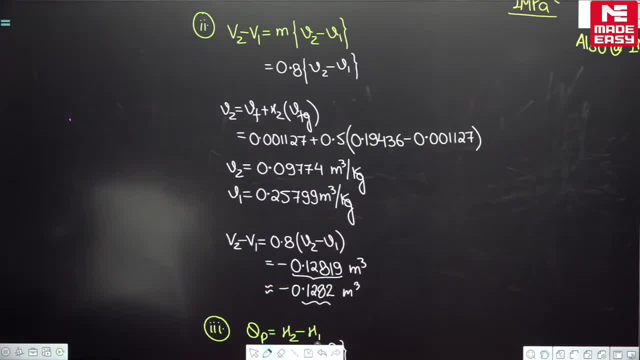 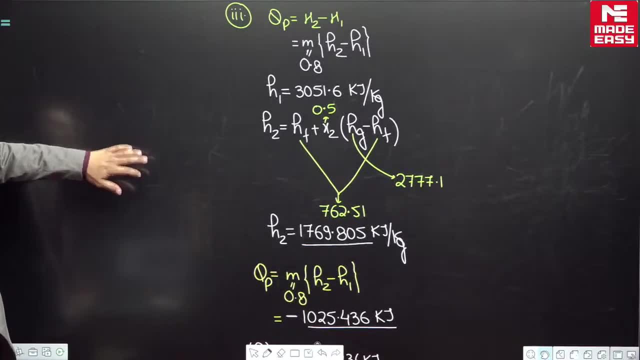 Sensible Aryan. sensible Rajgaving. sensible heat. sir, fine, I will also calculate. but just let me show this to the people who would want to write. we will calculate it. we will calculate 219.6.. Nishant Singh, you are also getting you also. you also got the answer: 219.6, sensible heat. 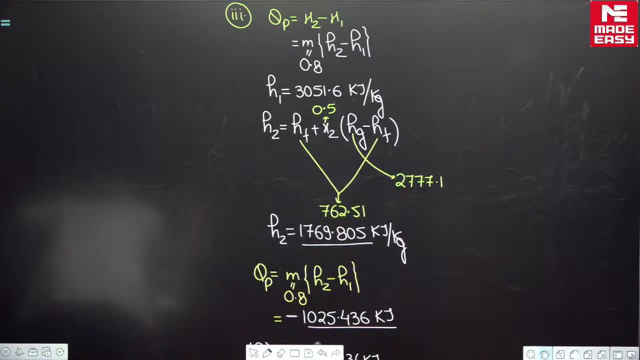 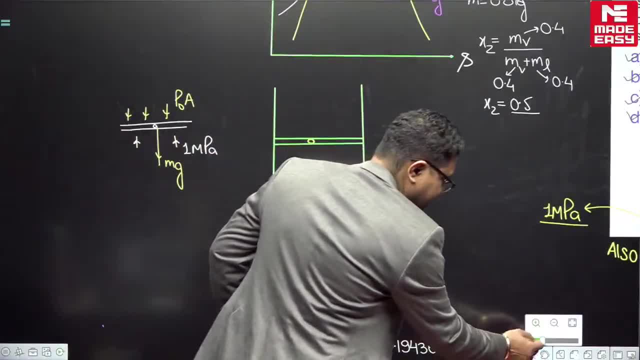 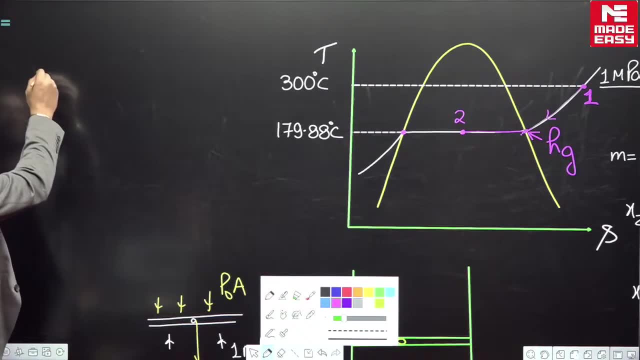 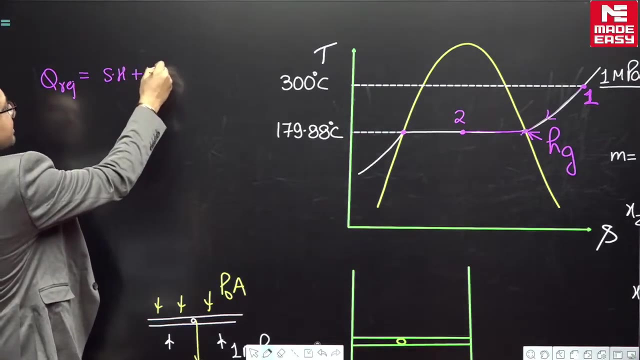 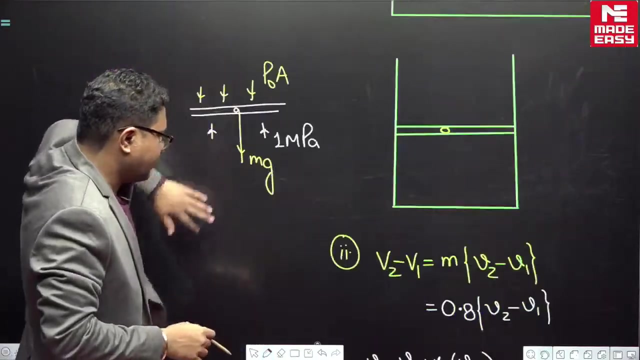 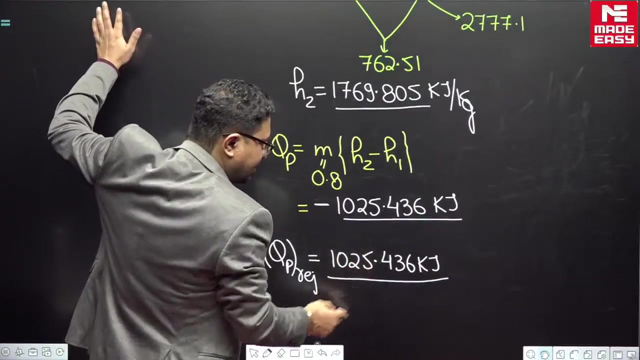 see, we will calculate, we will calculate. So let us calculate this. let me calculate So: sensible heat: out of the total heat rejection, the total heat rejection, the value will be equal to sensible heat Plus latent heat value. we have this value: total heat, total heat. this is the total heat: 1025.436, 1025.436. 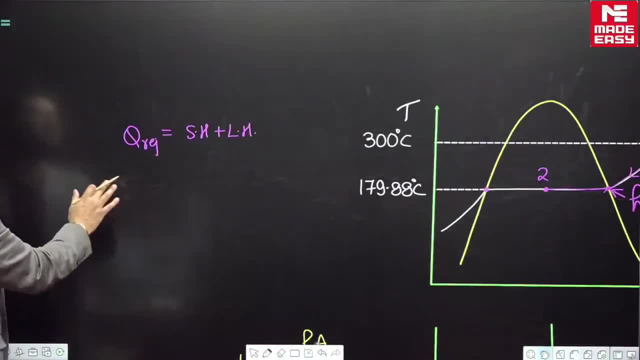 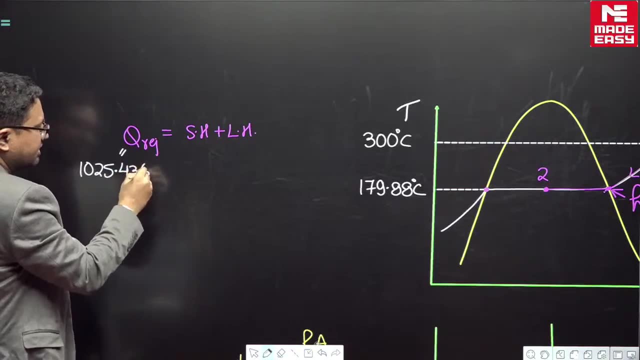 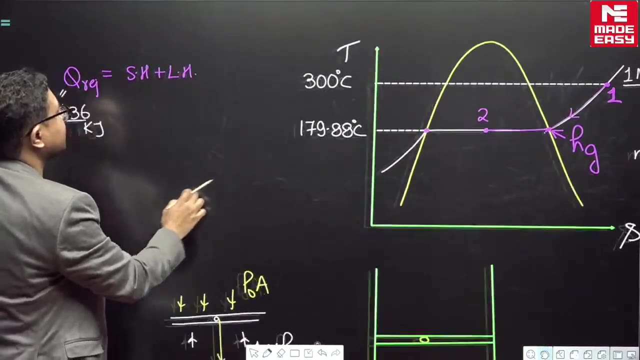 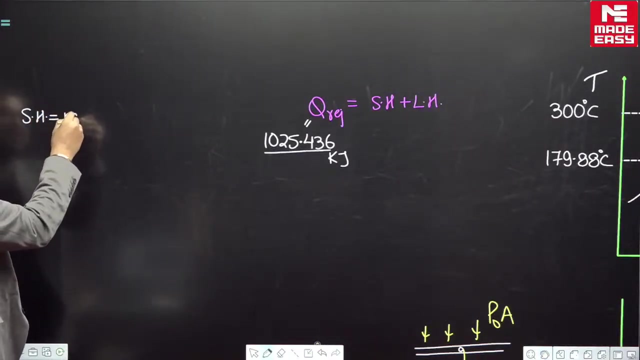 this is 1025.436, 1025, 1025.436, 0.436 kilo joule. this is the heat rejected. sensible heat. now sensible heat. sensible heat is h1 minus hg. h1 minus hg. calculate. let us calculate the sensible heat. so sensible heat will be equal to mass say. don't forget to multiply with mass. 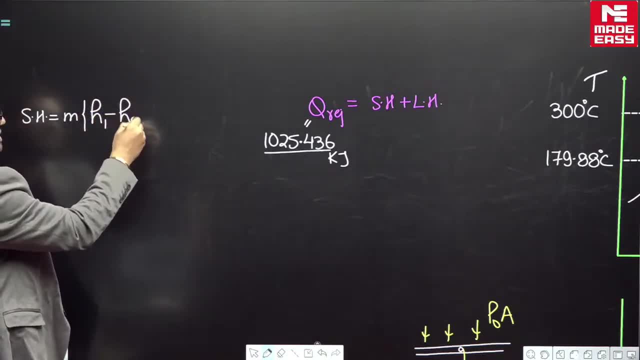 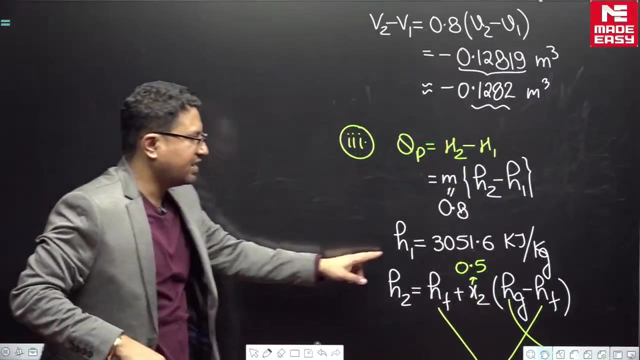 h1 minus hg. h1 minus hg. okay, so what is the mass? mass is 0.8. mass is 0.8. now, what is h1? h1? we have already written here h1 written here: h1. written here: 3051.4. 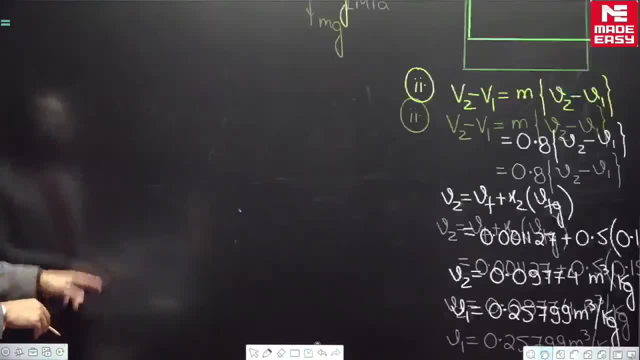 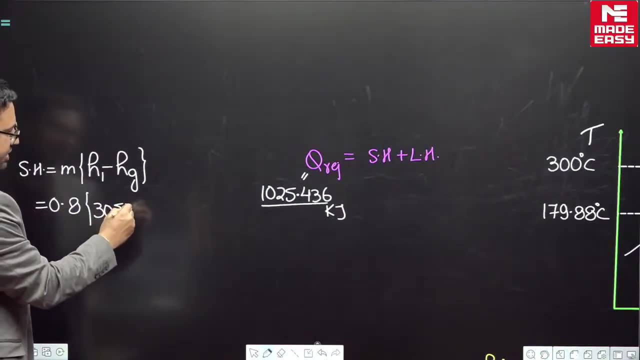 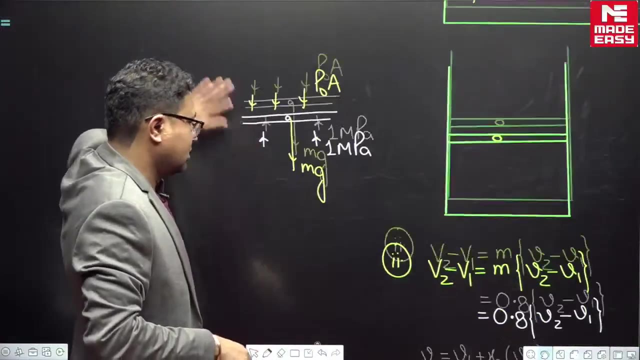 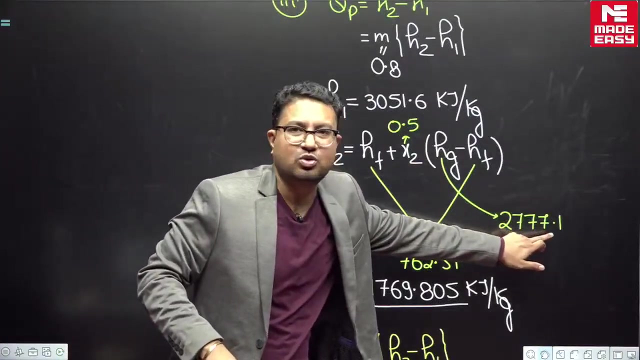 3051.6, 3051.6. we have already written 3051.6, 3051.6, 3051.6, minus hg, hg: see hg 1, mega pascal. what is hg here? so what is hg, hg? this hg is 2777.1, 2777.1. we have already written 2777.1. 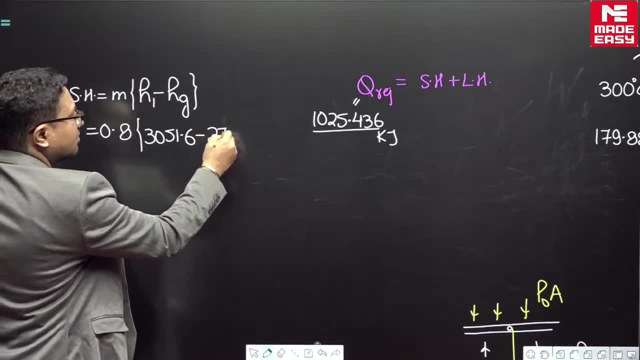 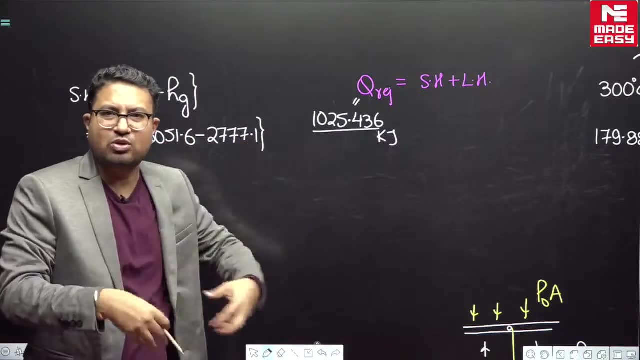 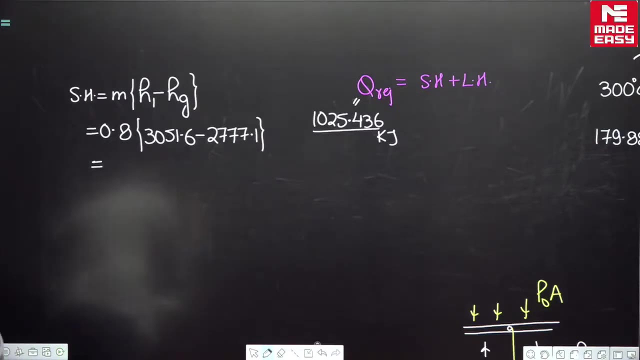 2777.1, 2777.1 when h1 higher, manifest lower karma, because I know it is rejection. it is rejection, so it will be a value. let me calculate this: there is 3051.6 minus 2777.1. and let me also check. there were few people who were giving the answer. 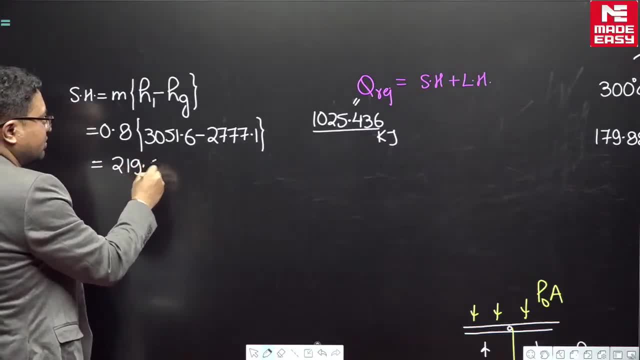 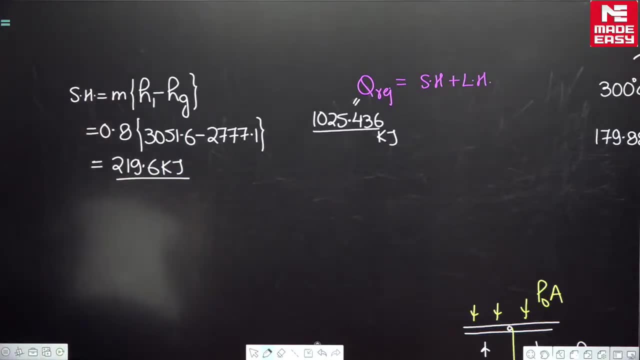 219.6 are at 219.6 kilo joule, So 219.6 kilo joule. I am getting, Yes, Yogesh Rai and Anuj Kumar. Shailesh Kumar Loni, you have given the correct answer. So you have given the correct. 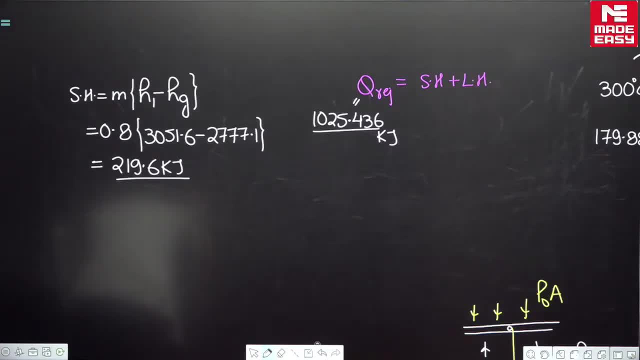 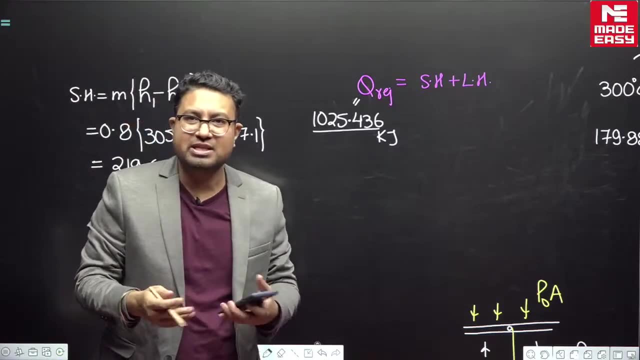 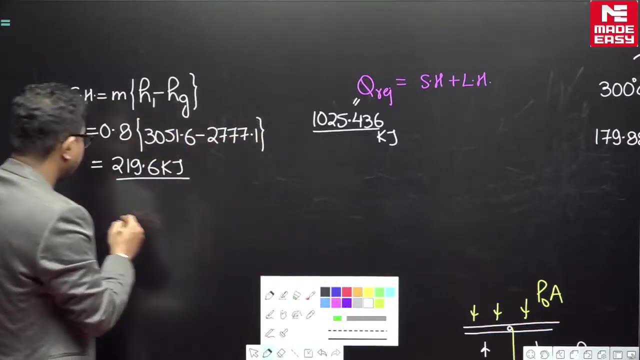 answer: 219.6. good, Now this is the 219.6 sensible heat. If you remove latent heat, how much is the energy which we removed? We removed heat, So how much we removed for the phase change, How much we removed So we can find out for the 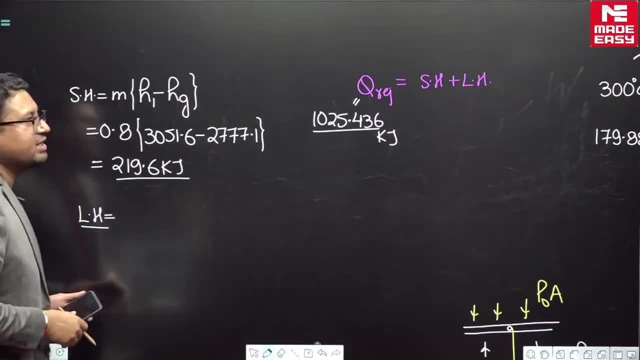 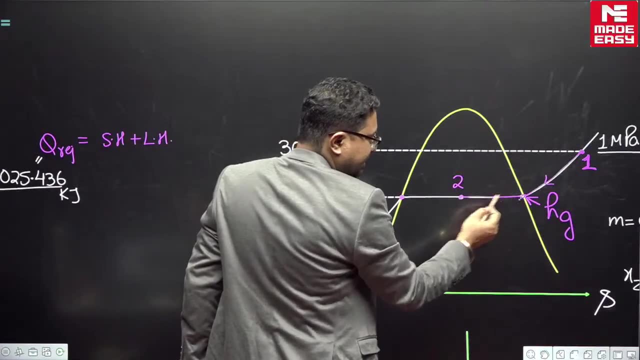 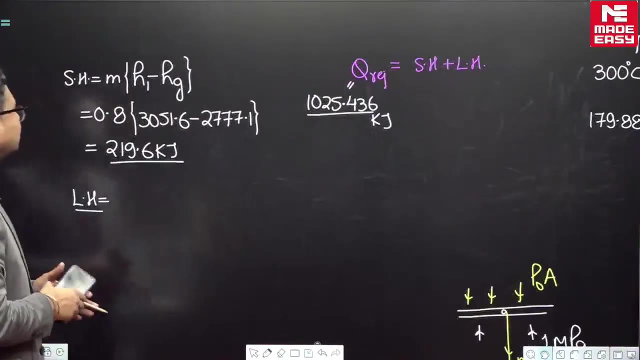 latent heat also. So latent heat. let us see this: Hg minus H2, H2, Hg minus H2.. This energy is for the phase change, for the phase change, Hg minus H2.. So we will have mass into Hg minus H2.. 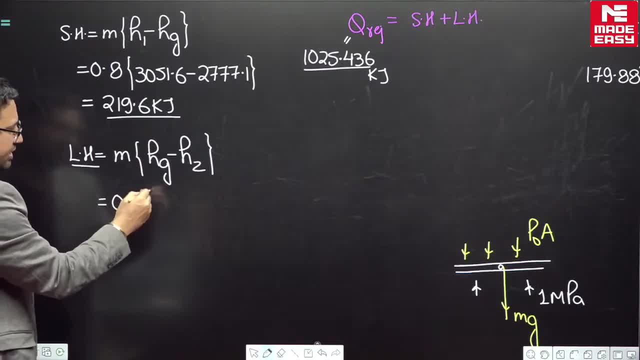 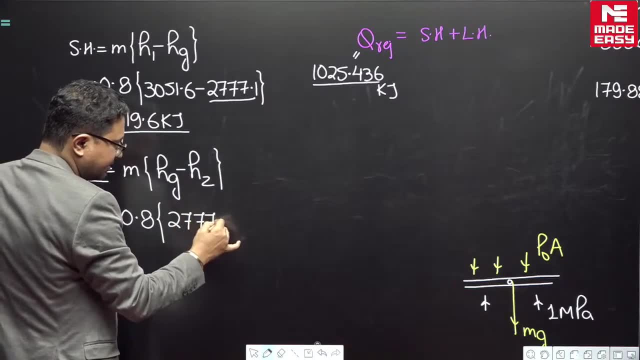 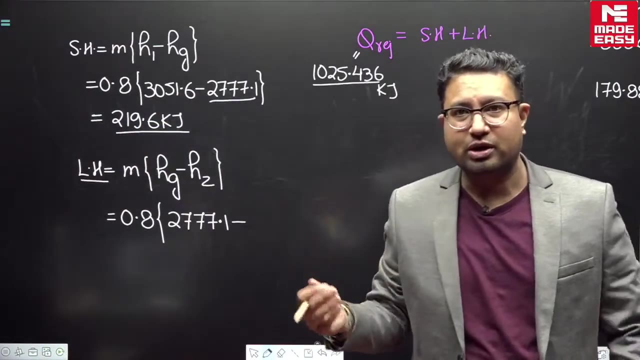 Hg minus H2.. So mass is 0.8.. Mass is 0.8.. Hg, Hg. we have already written 2777.1, 2777.1, this minus H2, H2.. So we will solve one more question after this. After this, we will solve. 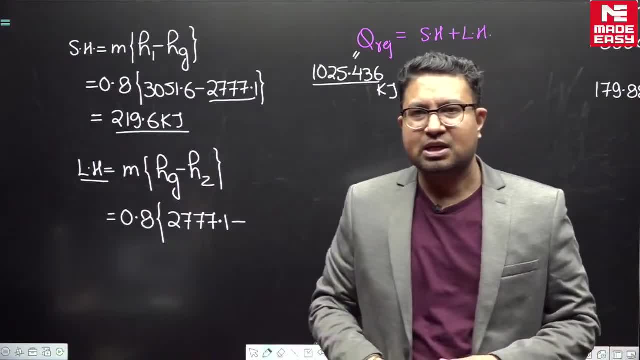 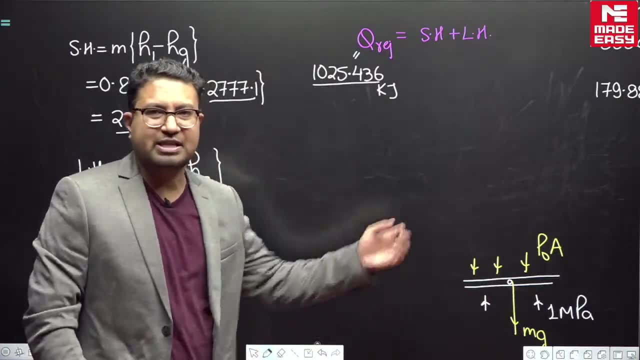 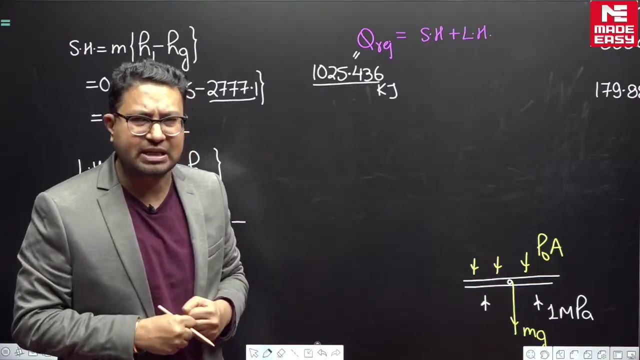 one more question and we will end the discussion. We will solve one more question after this and we will end the discussion. So we discussed the details of the TS diagram, We discussed the details of properties of pure substance and we discussed the details of the TS. 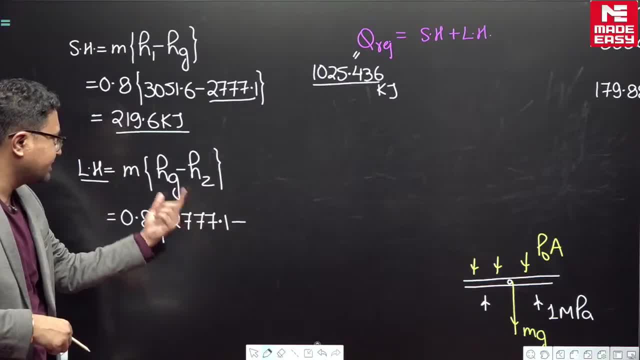 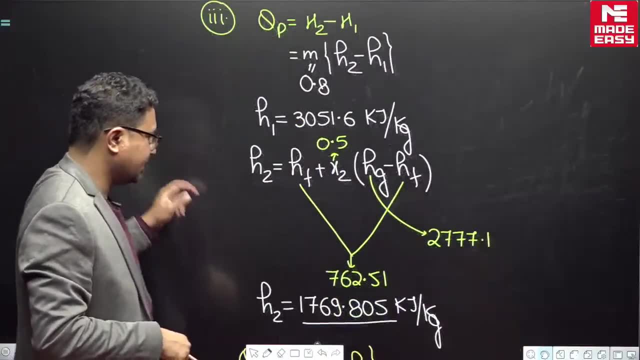 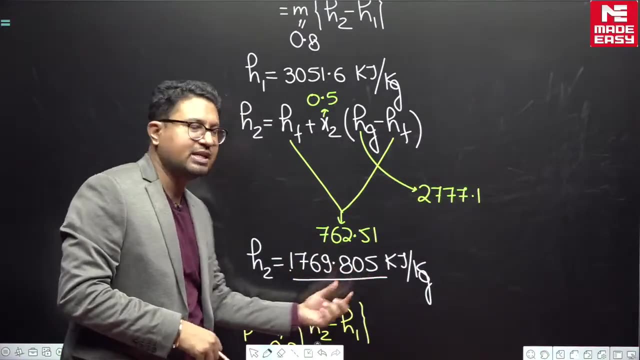 diagram. So Hg is this, Hg is this minus H2.. H2, see what is H2 here. What is H2?? H2 is 1769.805.. 1769.805,- this is H2.. 1769.805. 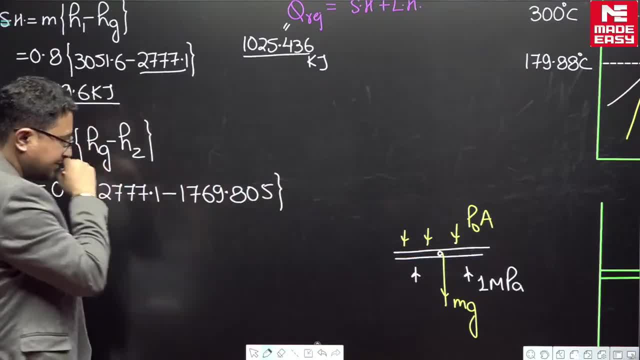 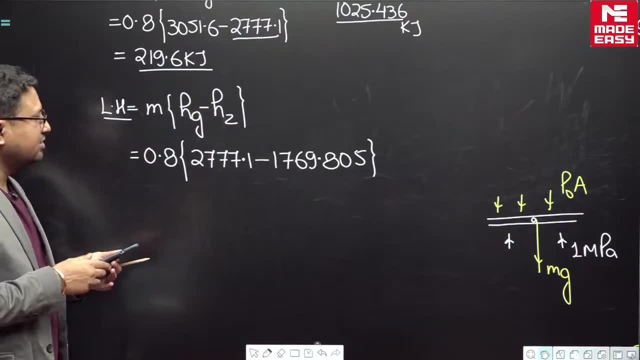 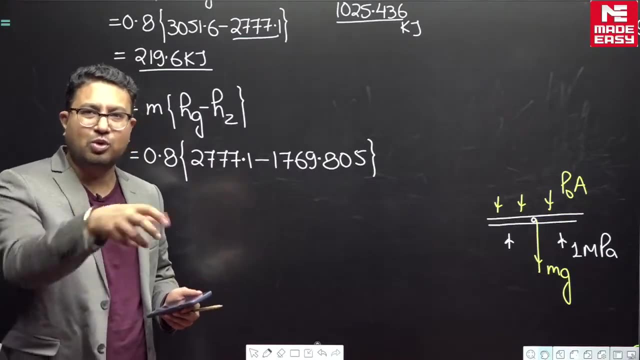 1769.805,. this is the value of H2.. Let us calculate this. So we have to calculate this, because Nishant raised a question. Nishant raised a question that it will be latent sensible, So we are trying to find out both. I mean there will be both, So we are also. 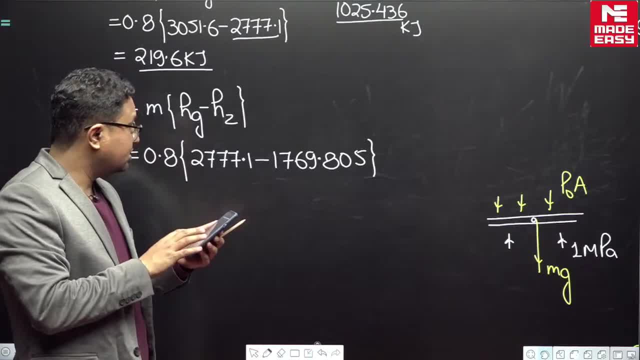 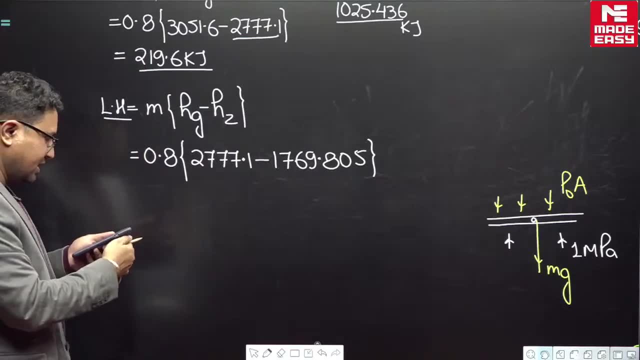 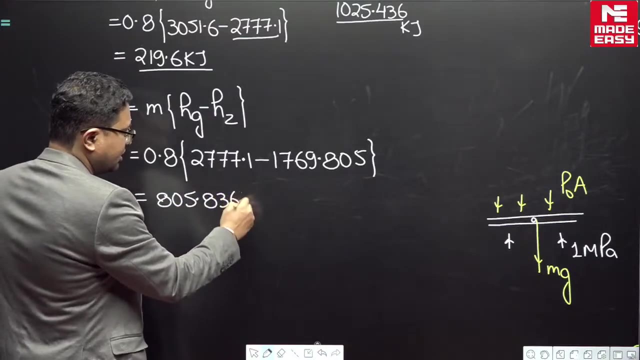 trying to find out the values. So for Nishant we have to find out the values. 805 into this is 0.8 into 0.8.. So we have 805.. This is 805.836.. So this is the latent heat. also, This is the latent. 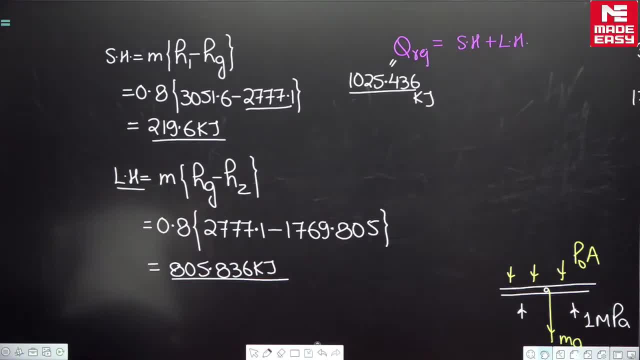 heat. This is the latent heat. Fine, Shashank Prasad, happy to see you. Thank you, Happy to see your comment. So, yes, this is the value. This is the value. So we have solved this. 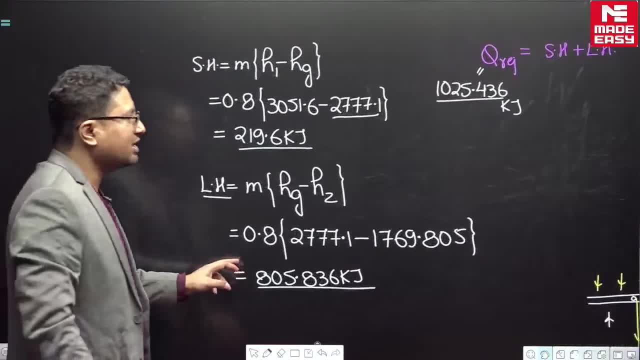 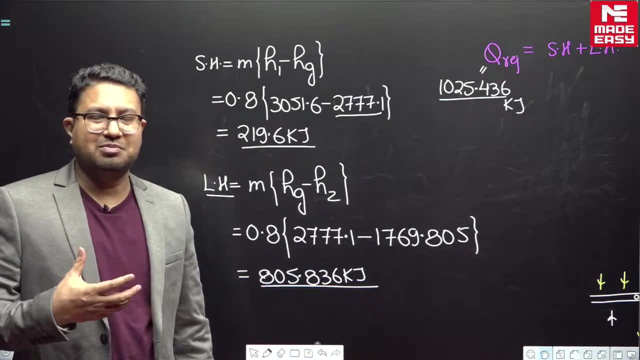 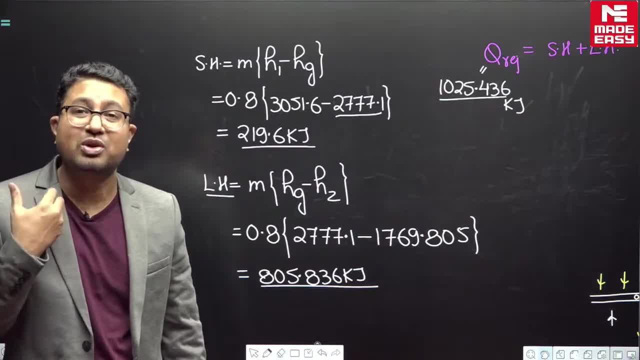 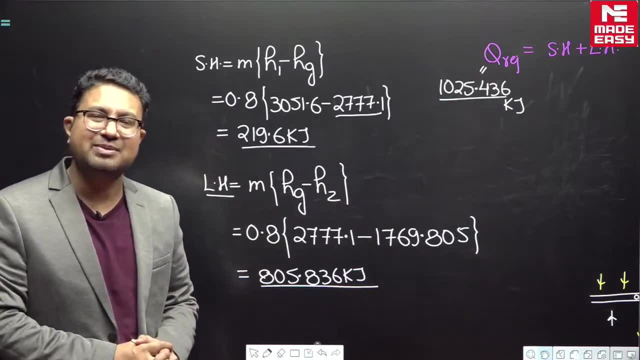 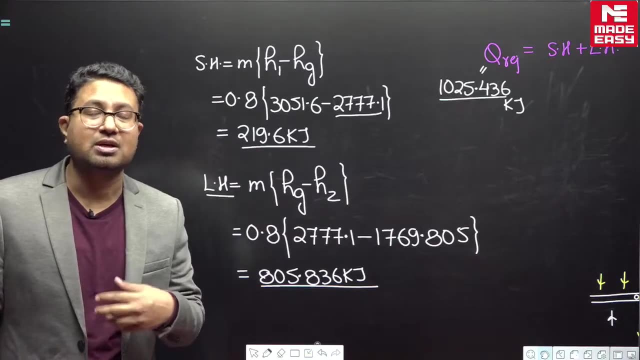 part, sometimes it is not. we are not able to visualize how to apply it. what type of questions can be asked? So for that we must understand- I mean, this should be understood- that we will be able to understand anything better if we try to solve problems on it. 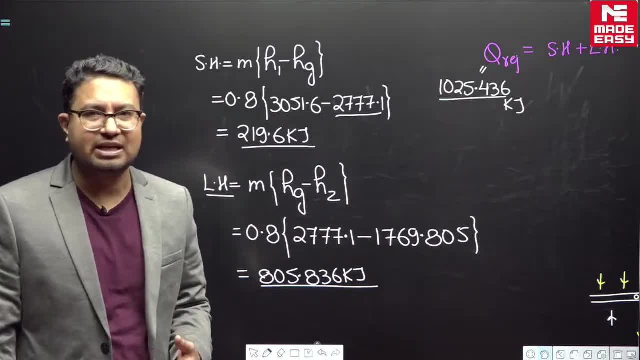 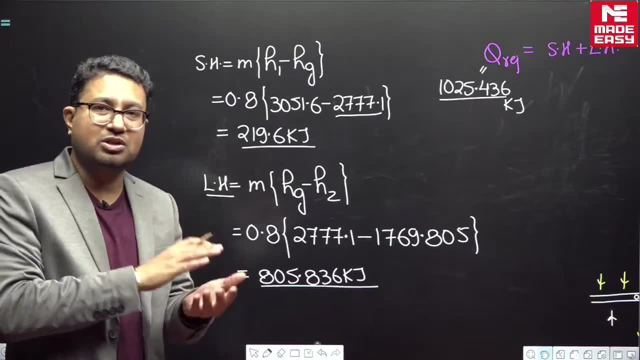 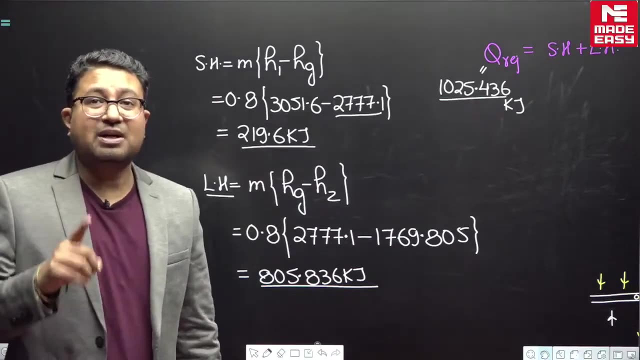 When we solve problems. when we solve problems, it is not that it is very smooth Because you are interacting. live with me, things will be more smoother. But when, suppose, you are on your own, you are trying to solve the problems, it becomes difficult. But but that difficulty. 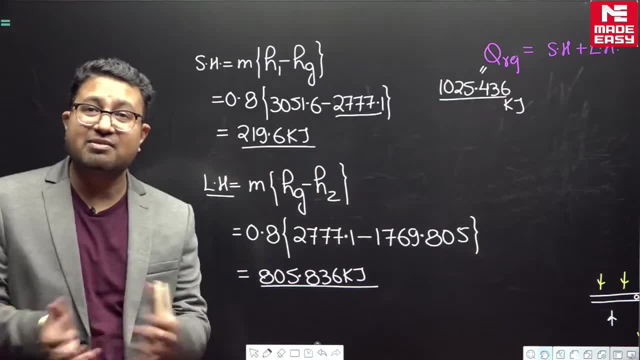 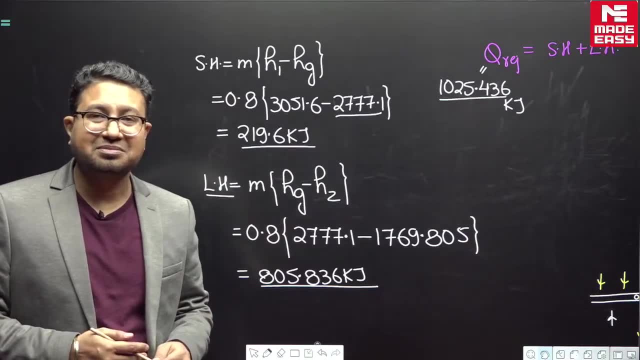 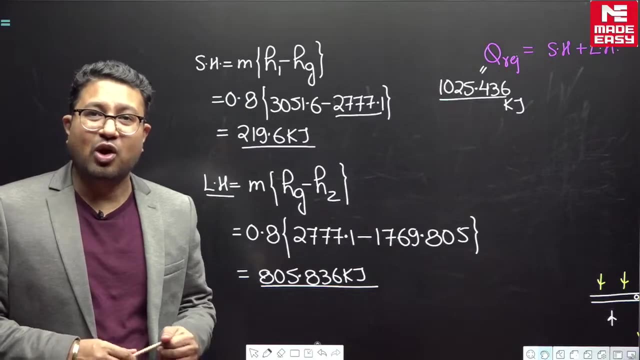 you have to face What the people do. What do people do? They run away. When they get frustrated, they run away. They stop studying at all. They stop studying. That is now. that is not how the things are done and things are achieved. If you want to move forward, 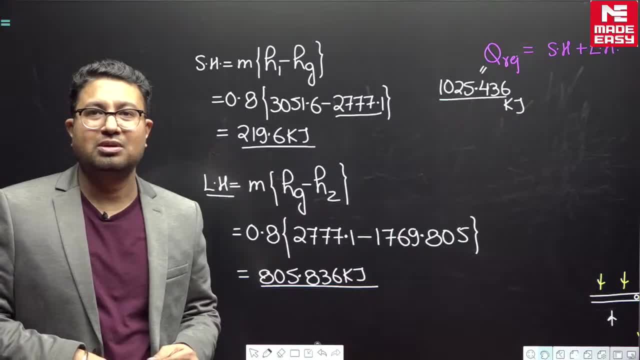 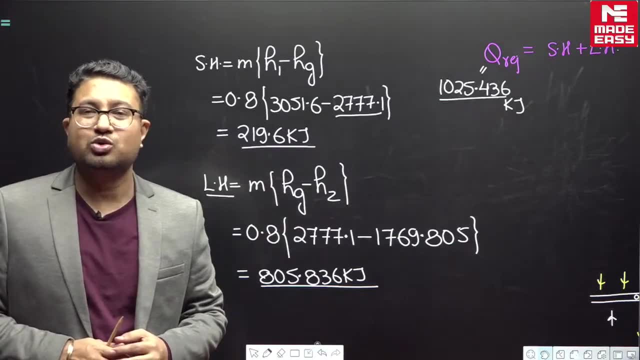 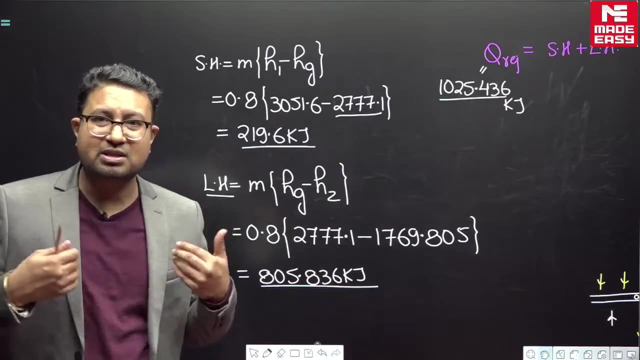 in a direction. you should be able to allow yourself to experience all the emotions that come in that path. The people get frustrated so they just back off When you are solving a question, when you are solving a question if it takes twenty minutes, twenty minutes. 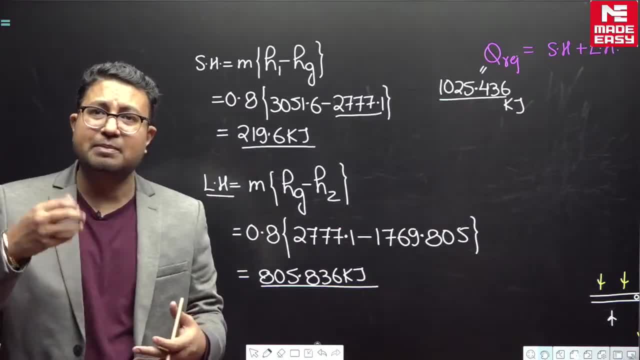 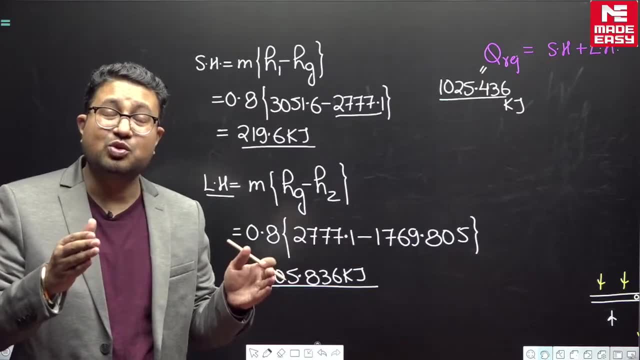 twenty five minutes and you are not able to solve the jo. frustration hota hai. The people stop studying that topic or that subject, But in that twenty minutes you would have thought so much about that subject or that topic that it would have churned your brain. 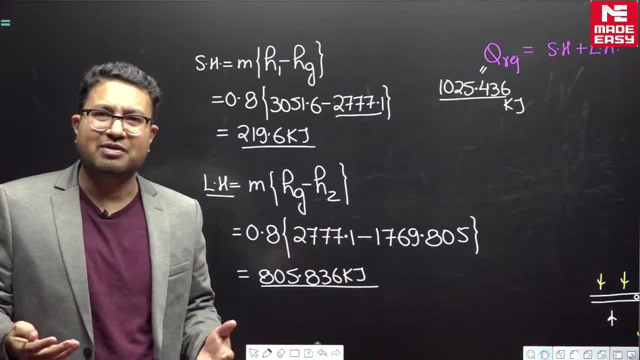 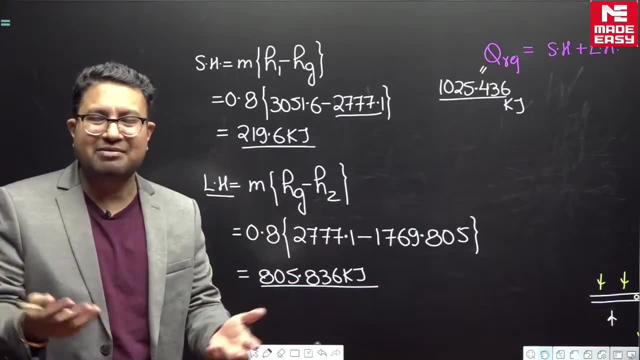 That is how the brain sharpens Aisi to sharp hota hai. When you would have learnt to ride a bicycle, Jip cycle, chalana shikaho ga to- nobody is here, I mean including me and everybody who is watching- nobody would have been able to solve menu. 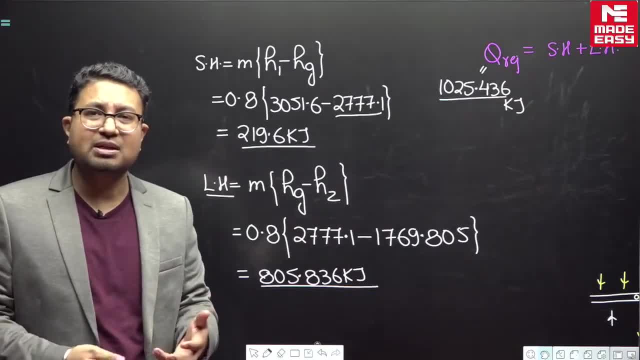 May be movie, may not be in blog, may not be in new maj- All these types of problems there. So that's, how are we able to solve our problems? So you leave a problem other than us. You know to ride a bicycle without falling. we fall, but we allow that experience to happen if you don't want. 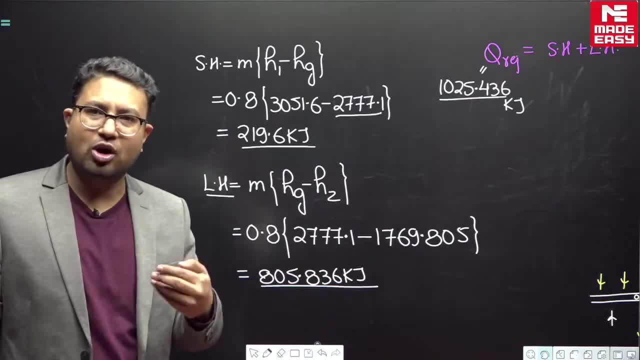 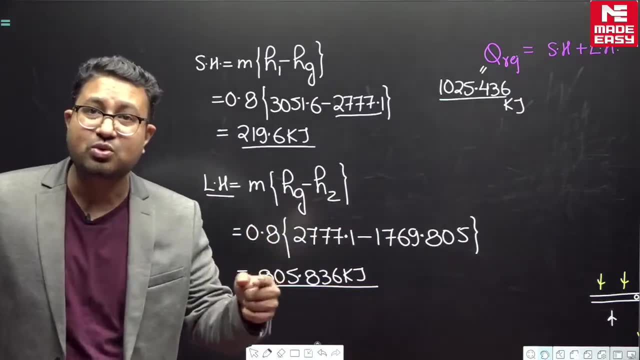 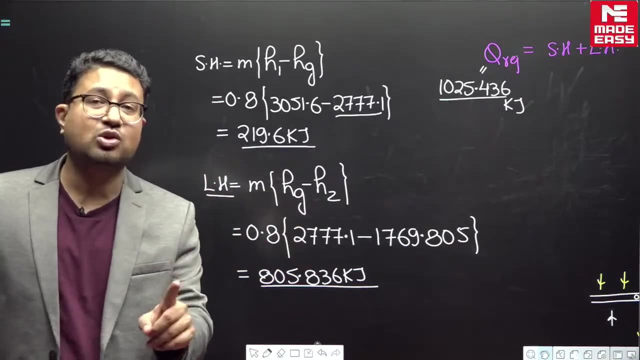 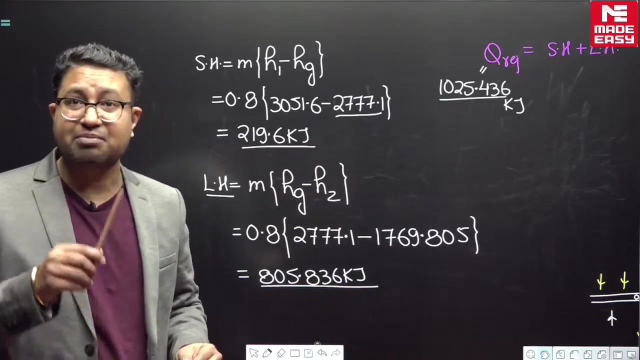 to get hurt or if you don't want to fall, you will not be able to know how to ride a bicycle. same is with these studies. you should not think ways of escaping the frustration. don't try to find out the reasons or the ways to escape frustration and fear. 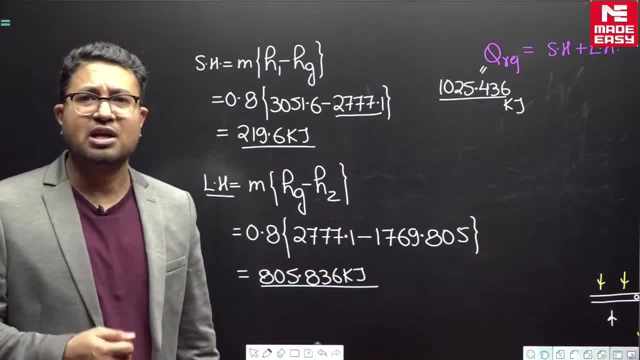 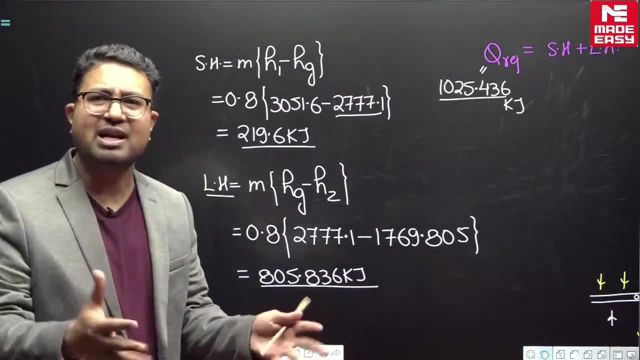 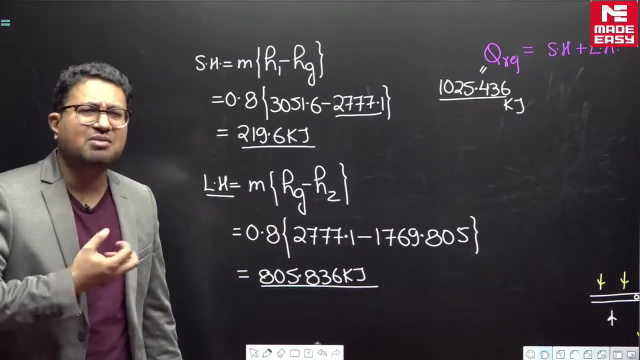 face that frustration and fear. live that fear. live that frustration and when you will live it and still keep on moving forward, that will go anyway. that is a temporary phase but you will have to allow yourself to bear that. when emotions come, we become very discomfortable. but if we allow, 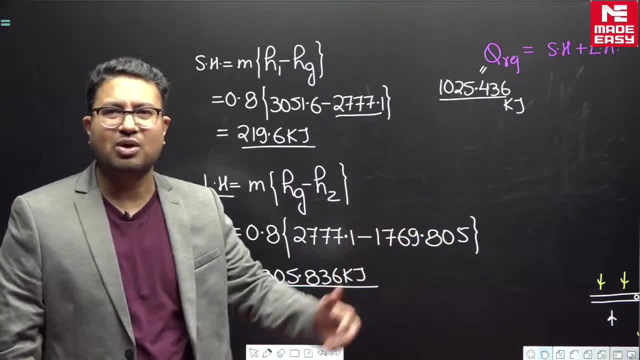 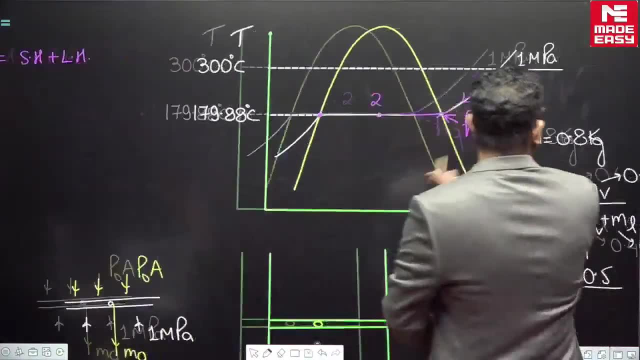 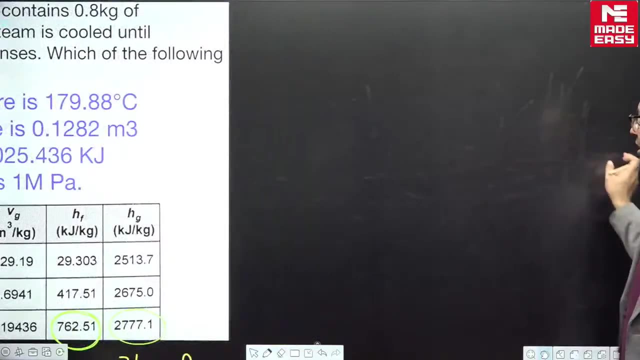 ourselves to go through those. we walk the path. so that is what we can do, that is what the best we can do, that is what i have been doing in my life. so i just said that now we have seen this problem. we have seen this problem. now there is one more problem. there is one more problem. that is the one. 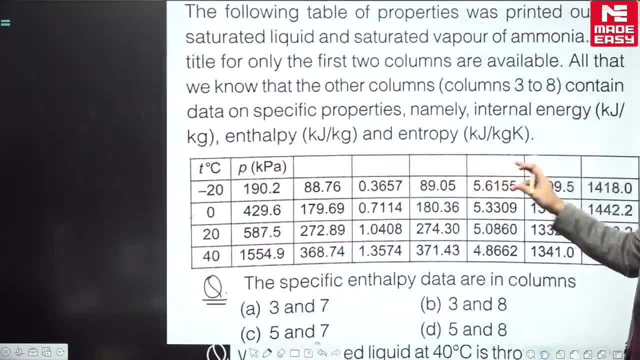 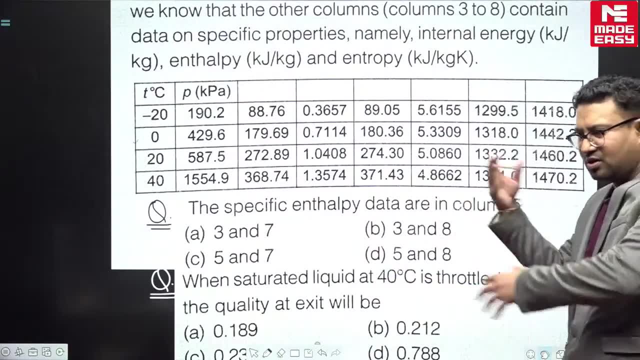 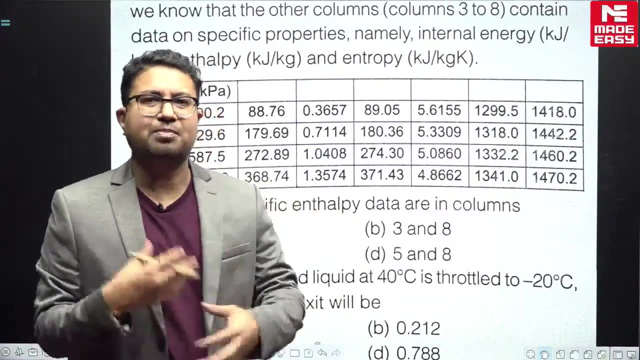 of the problem that was asked. that has been asked in the previous year 8 exam. why i have taken this problem is there are two things. so basically, there is one part which is based on whatever we are we have discussed, but there is one more thing which the people generally ask doubts to me, so i thought of taking this in my discussion. 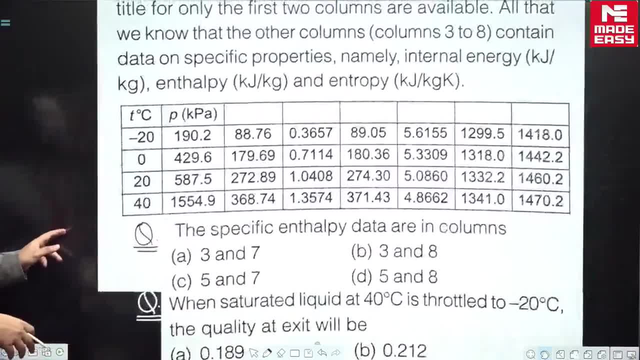 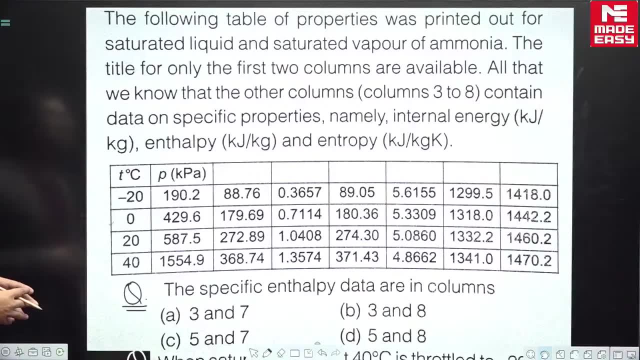 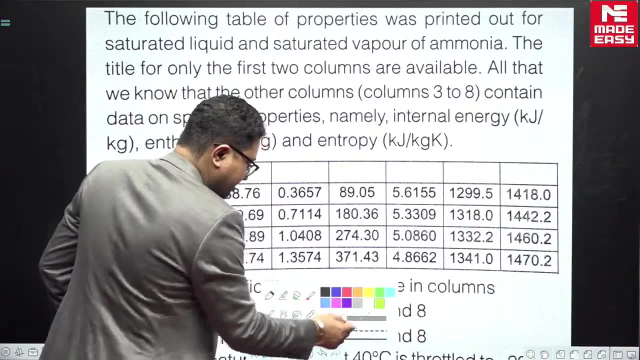 including this in my discussion. so let us see this question, this question. let us see this question, this question. the following table of properties was printed out for saturated liquid and saturated vapor of ammonia: previous year gate problem and through this we are going to discuss something. so the last problem which we saw, that is not a gate. 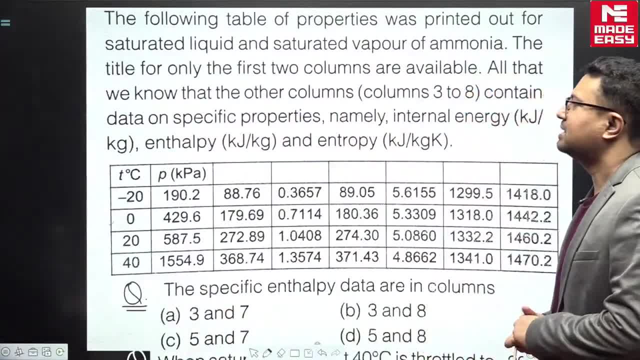 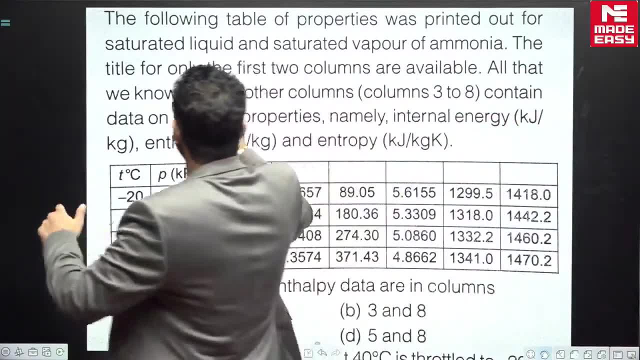 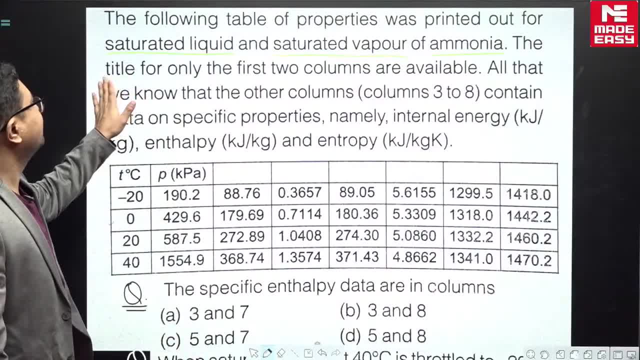 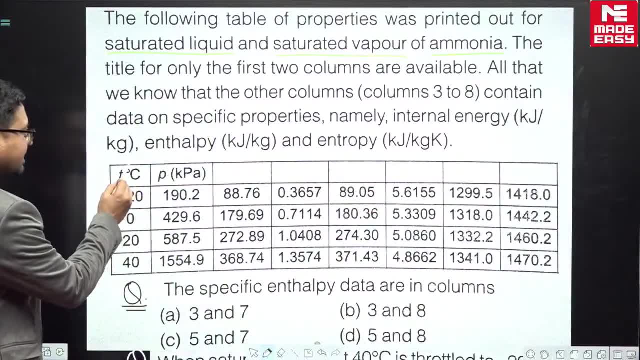 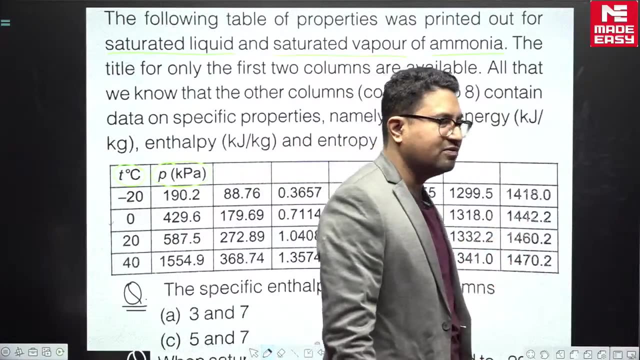 Okay For ammonia. The title for only the first two columns are available. Now somebody would have written these values, But the person has written here temperature and here pressure. Now all these, all this data is there, But you do not know which data is entropy, which data is enthalpy, which data is internal energy. 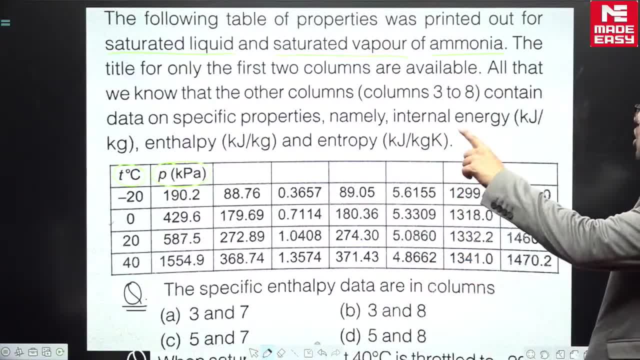 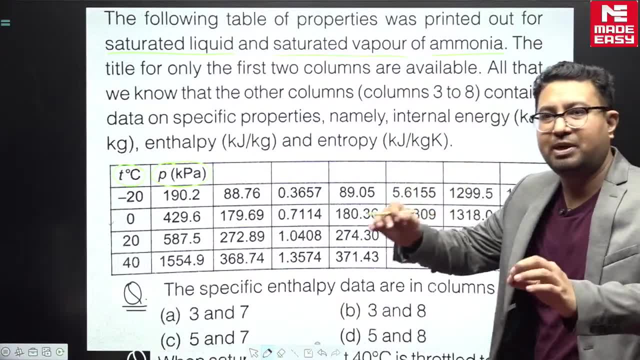 We do not know anything about it, All that. we know that the other columns, 3 to 8, contain. We know that. what are the properties the other column? So this is the column 1.. So this is the column 1.. 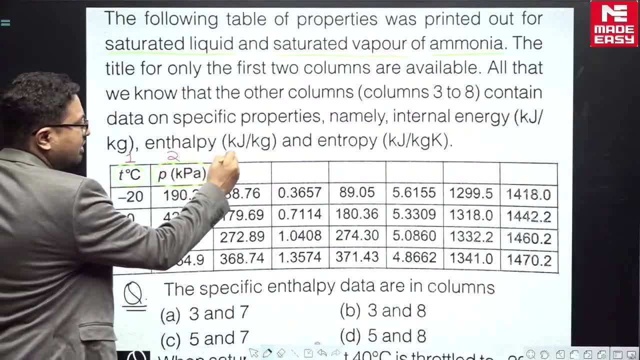 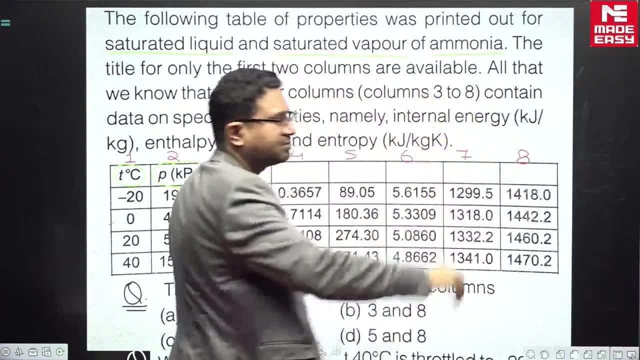 This is the column 1.. This is the column 2.. Now the column 3,, 4.. 5,, 6,, 7 and 8.. Now, all that, we know All that. we know that the other columns, 3 to 8, contain data on specific properties. 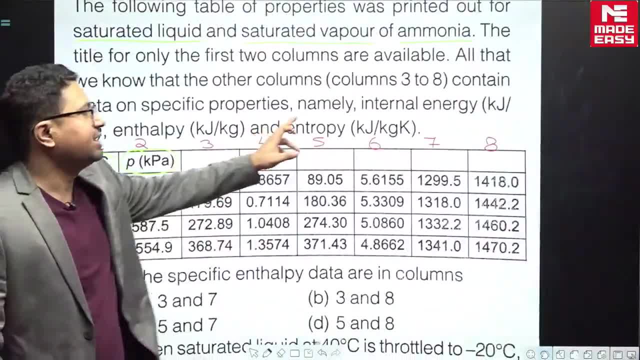 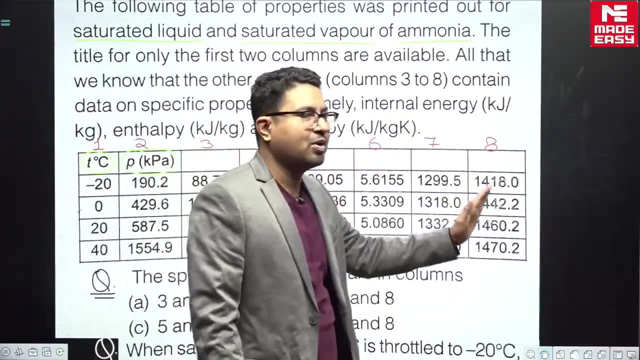 That is unit mass properties, Namely internal energy is also present, Enthalpy is present and entropy is present. We do not know the sequence. Which data is of which property. We do not know Also. also the data can be for saturated liquid. 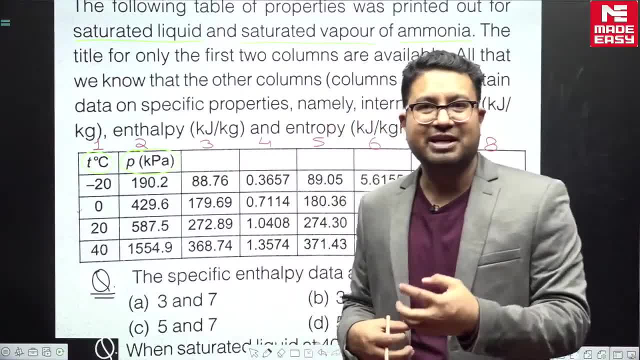 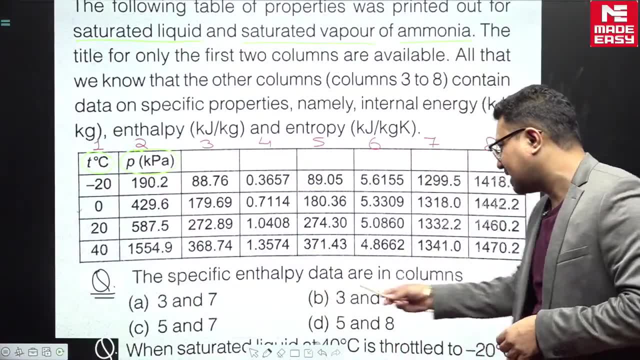 The data can be for saturated vapor also. We do not know Which data is UF and which data is UG, So let us first try to understand this. They have asked specific enthalpy data, But we will find out all. 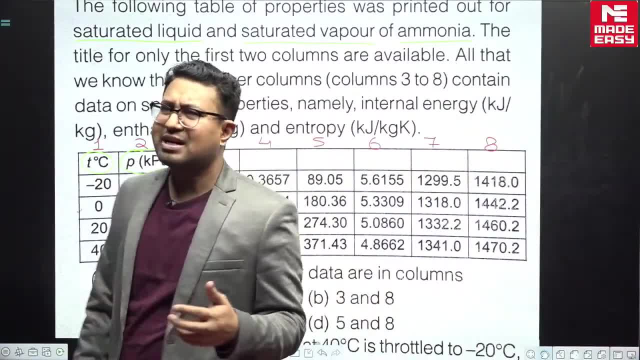 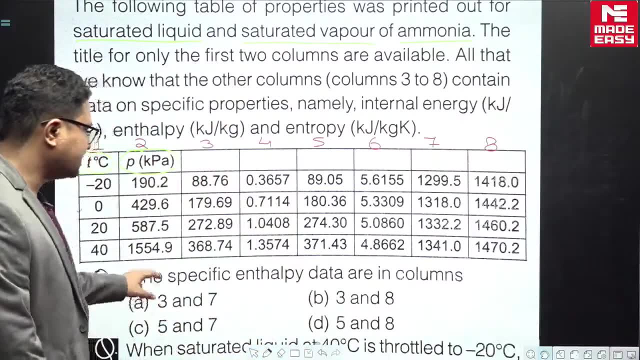 We will try to understand how we can identify. If we are given any question, how can we identify? That is what we will try to understand. And there is a second part that is a numerical. We will solve that also, But this is a frequently asked confusion. 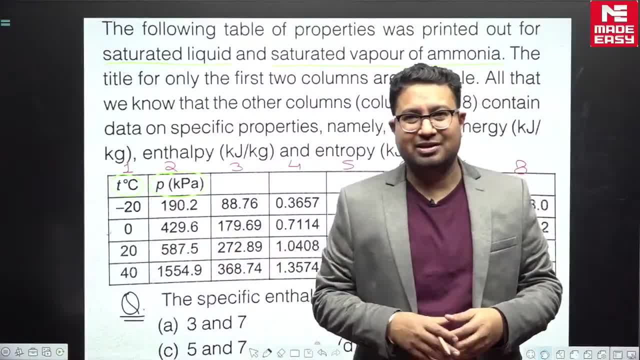 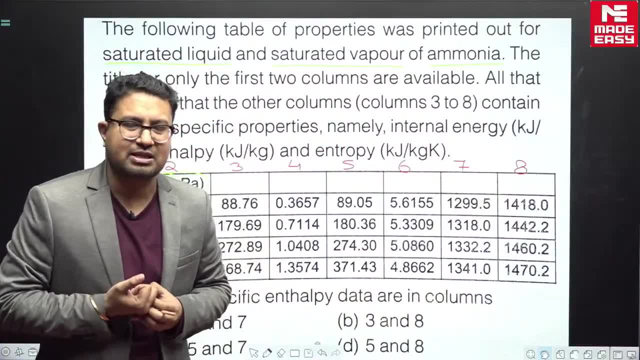 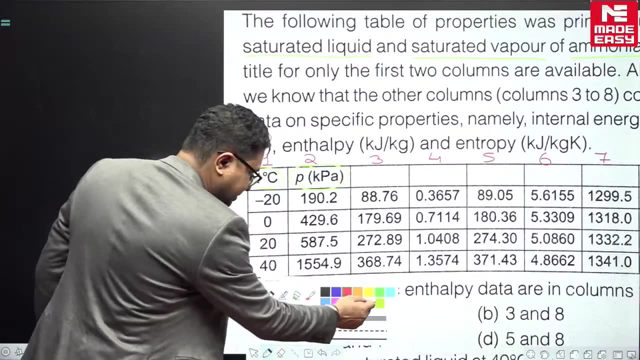 Because, see, there is no sure shot Thing here. we have to understand. We will have to understand. A little sense and experience is required to understand this. See, What are the properties? Which properties are there? Let us see. So what are the properties? 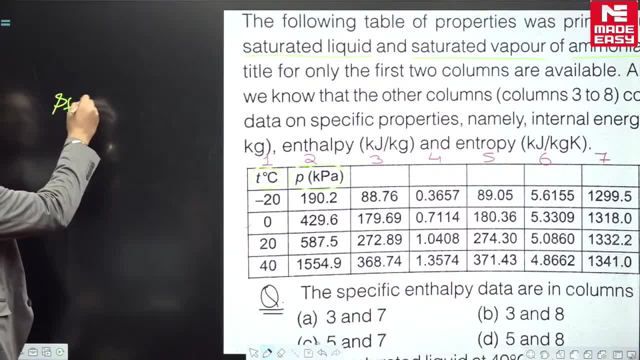 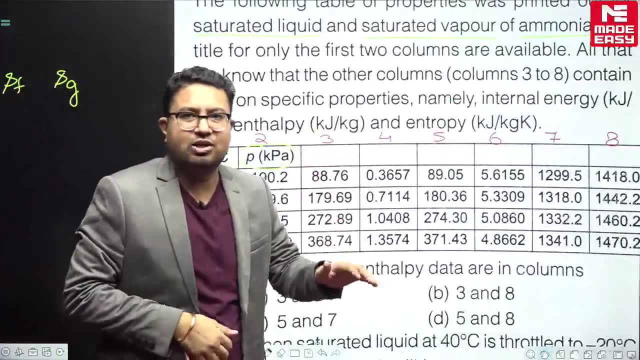 So properties are entropy, So SF and SG, Then internal energy, So there are total 8.. 2 are known, That is 6.. 6 columns are remaining 6,. 6 columns are remaining Right. 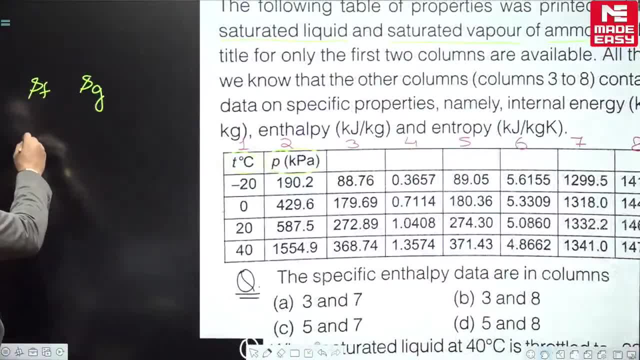 So 6 columns are remaining. So U, F, UG, HF and HG. These are the 6 properties. HF properties: These are the 6 properties. Now, if anybody is able to know, you can please let me know by messaging here. 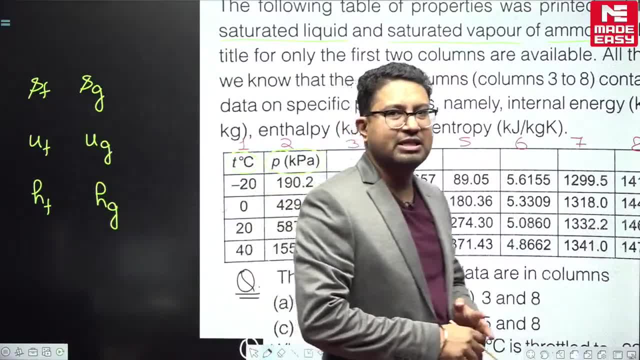 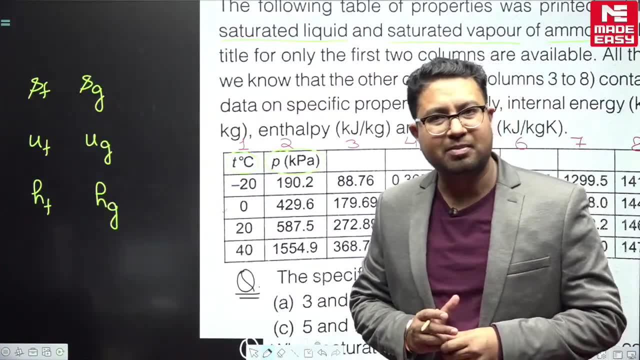 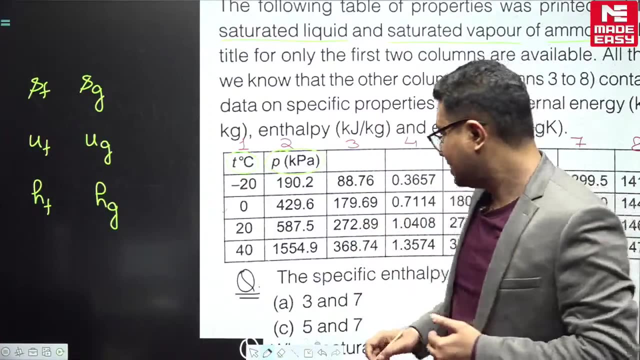 Now, now see How we can see, How we can see Entropy is obtained. The entropy which we get, that we obtain by dividing energy with temperature. Energy is obtained by dividing energy with temperature. The entropy values which we get, The entropy values we get. 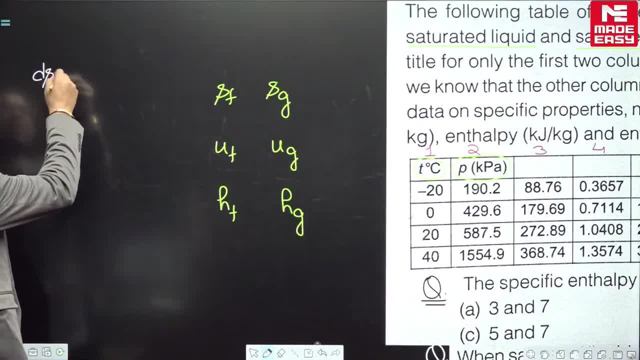 As you will see, DS is equal to del Q by T, Del Q by T Or del Q is. also, we can write HG minus HF. Just now, we obtained, we obtained a formula: Sg minus Sf is equals to Hg minus Hf upon. 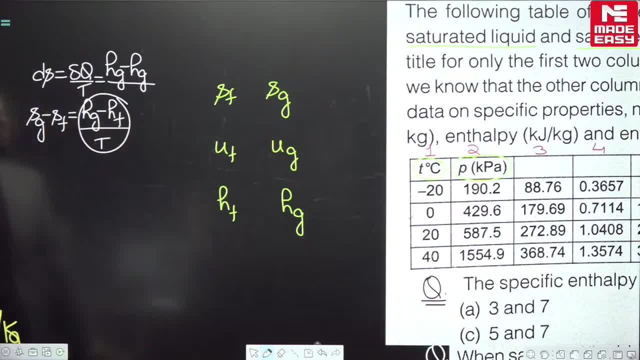 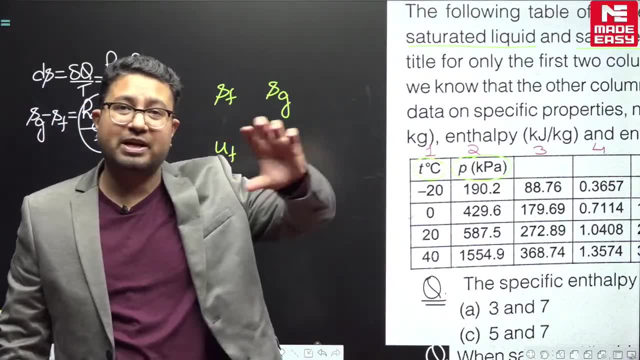 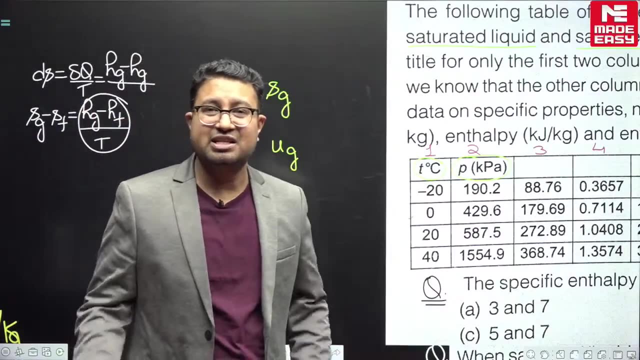 temperature. That means you divide energy values with temperature. Temperature is divided for the entropy values. So entropy values are obtained by dividing the energy value with temperature. So entropy value will be the minimum out of these, 6.. In 6, the lowest values will be the values of entropy. 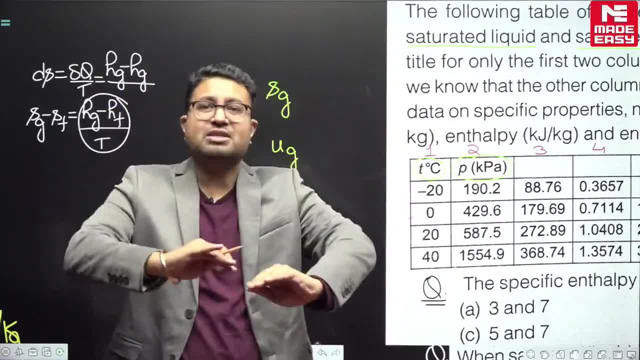 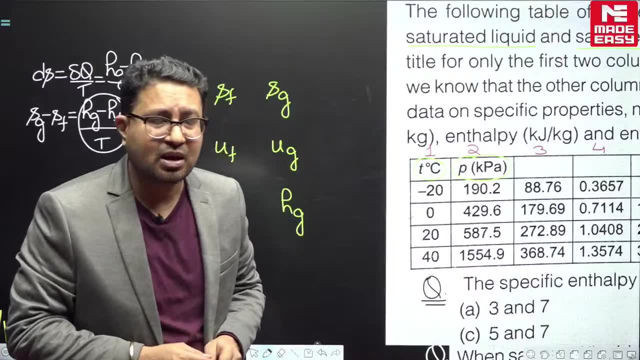 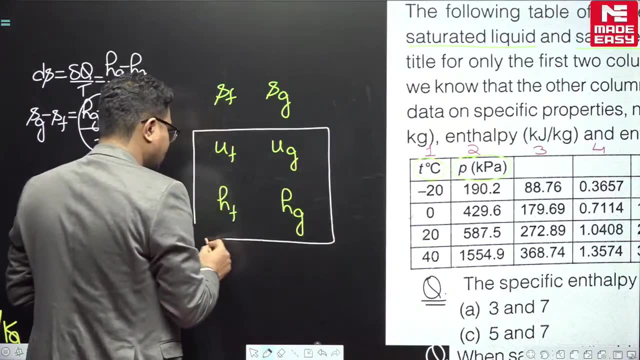 The lowest values of entropy will be there, because energy is also divided by temperature. 300,, 400, 500. you have divided with significant value, you have divided with a big value. So S the minimum minimum 2 are entropy value. 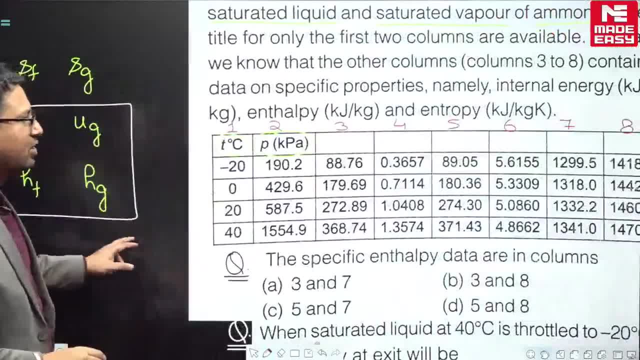 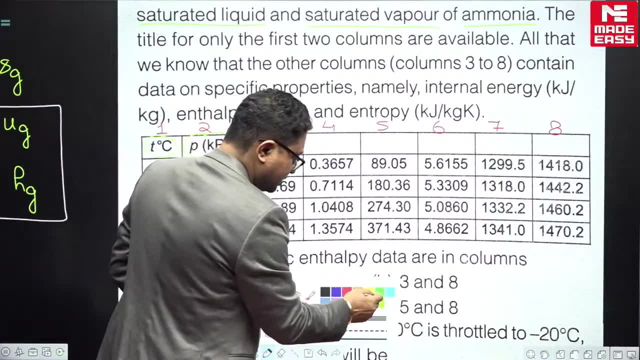 So separate the remaining 4 and look at the minimum 2.. So what is minimum 2?? What are the minimum 2 here? What are the minimum 2?? See, if you see here, if you look here, if we have to find out the minimum 2.. 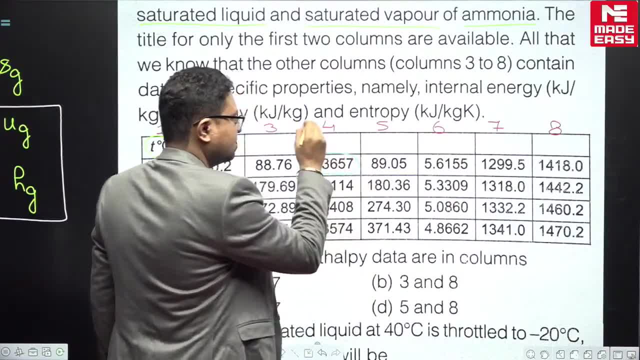 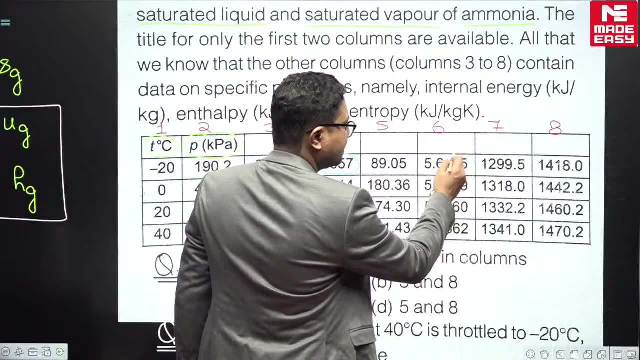 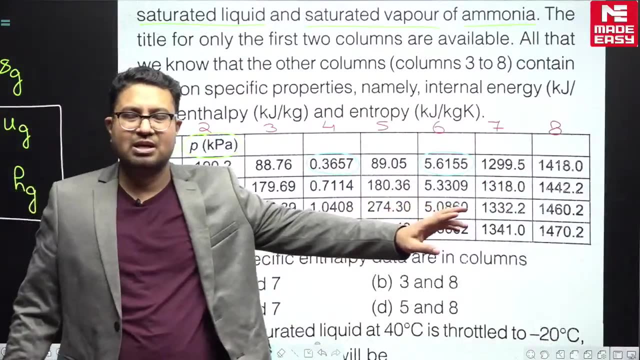 So this is a very small value. This is a very small value. Look at it: 88.76 and this 5.6155.. Rest all the values are more than these 2 values. Rest all the values are more than these 2 values. 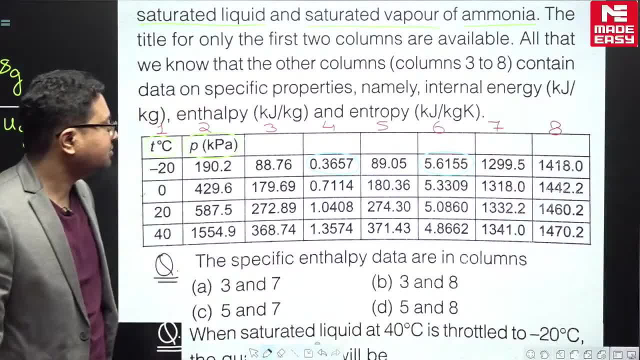 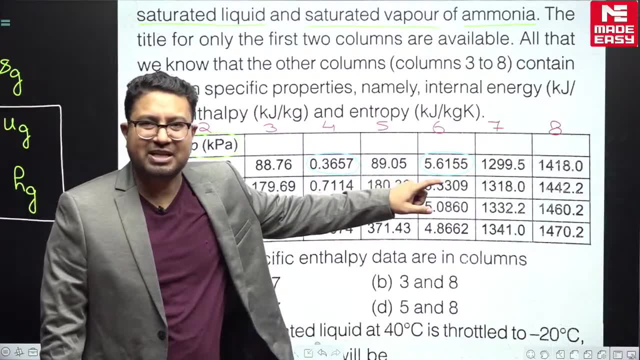 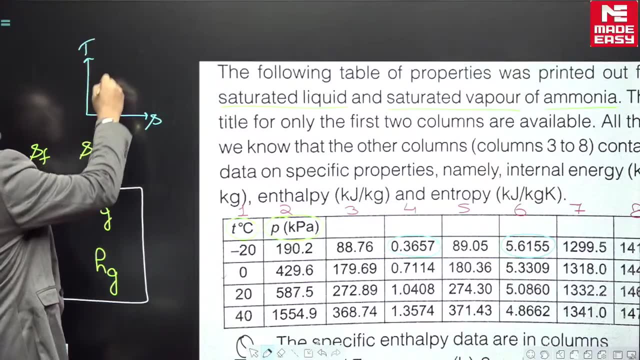 Rest, all the values are more than these 2 values. So one of them will be Sf And 2, as you have seen. one of them will be SG, Obviously, you will see. obviously, we see that entropy of vapor is more. 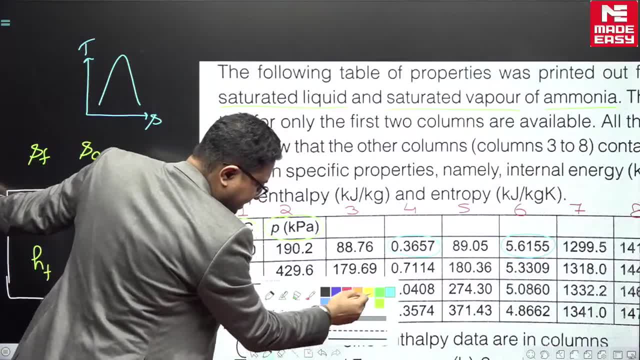 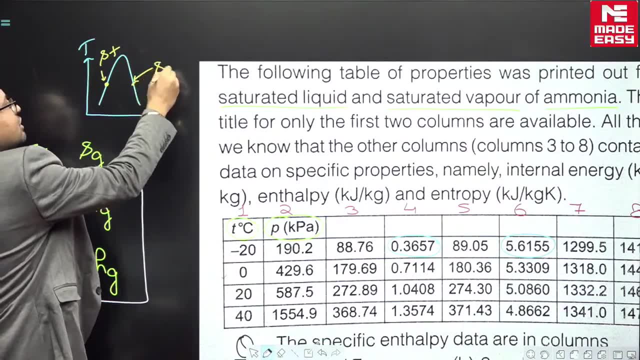 compared to entropy of vapor is more. If this is SF, this is SG, this is SF, this is SG. So, out of these two, the higher one will be SG. Out of these two, the higher one will be SG. 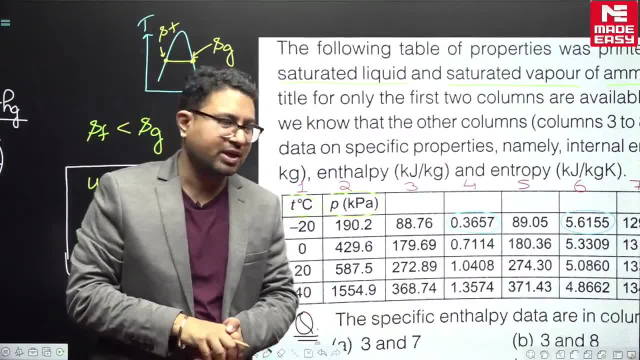 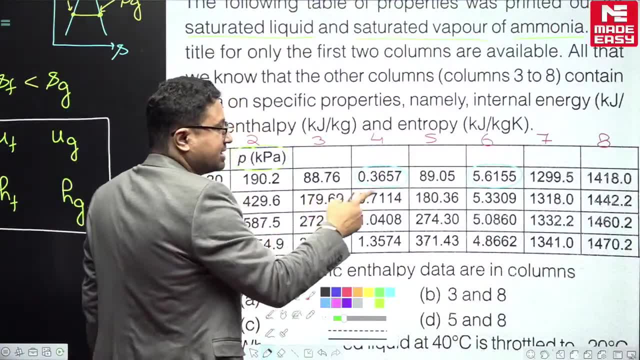 Obviously, the other will be SF, rest will be SF. So let us see this, let us see this here. So this is SG. this is SG because out of these two this is bigger. So this is SG. 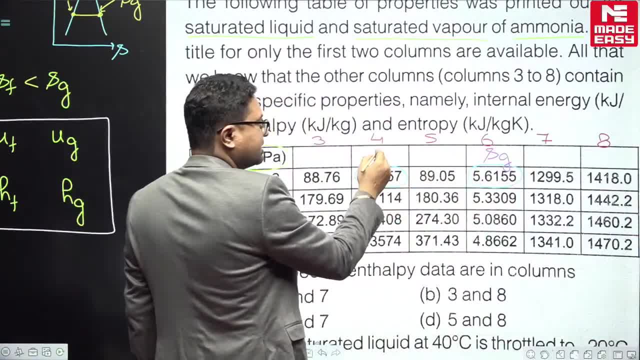 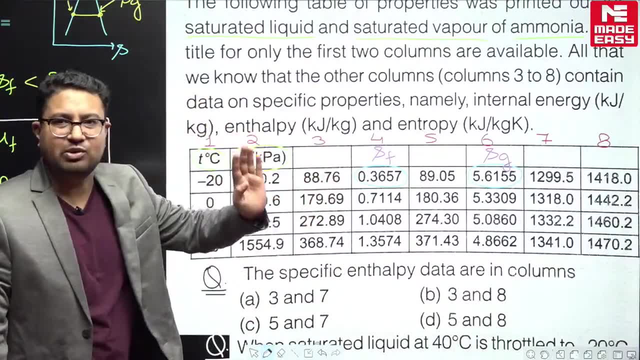 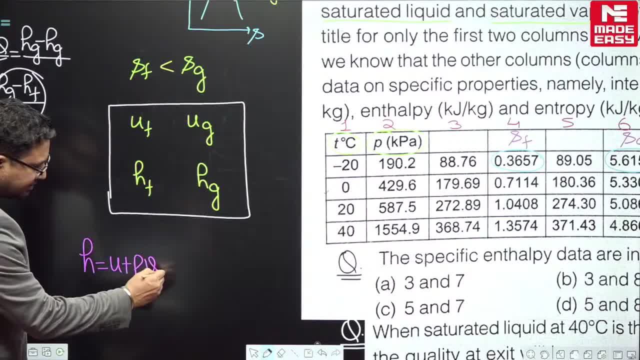 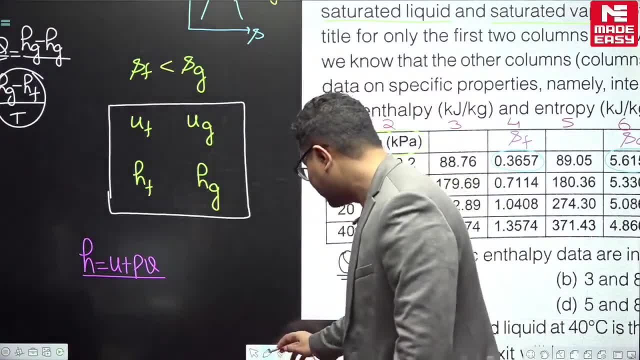 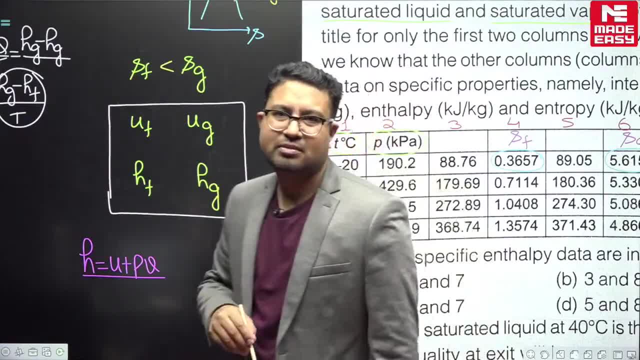 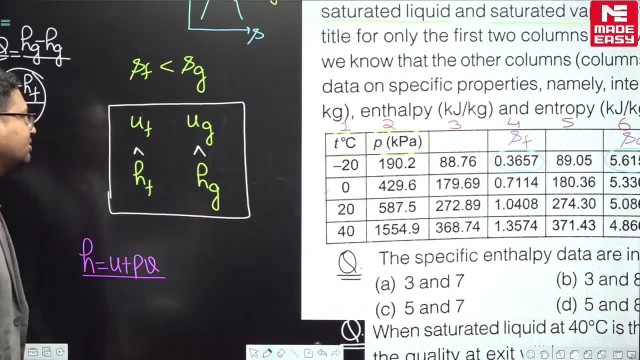 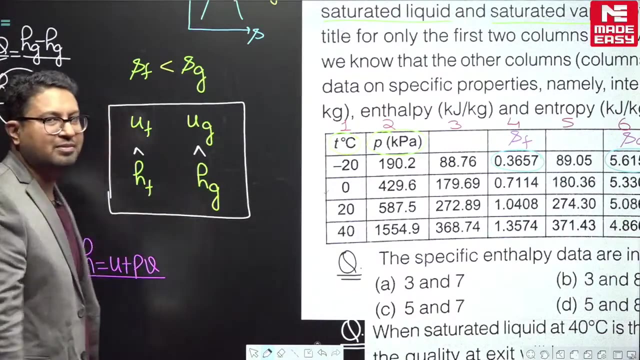 obviously, HG will be more than UG, HG will be higher than UG. so HG will be higher than UG and HF will be higher than UF. HG will be more than UG, UF will be less than HF, because, adding something, you get this, we get this by adding something in this. then, moreover, we can say the internal. energy of the enthalpy is very high for the liquid, for the vapor, compared to liquid liquid. may you add latent heat, then it becomes vapor. so enthalpy or internal energy for the vapor will be much higher compared to liquid. so if you want to compare, 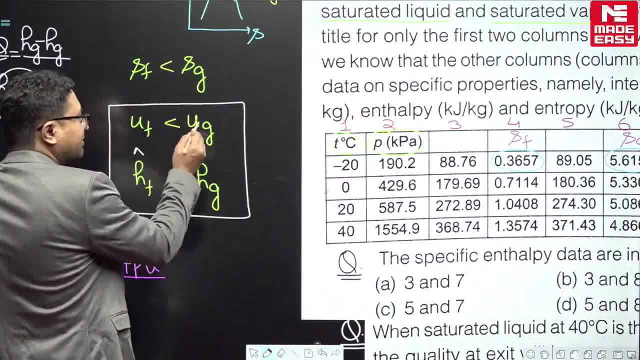 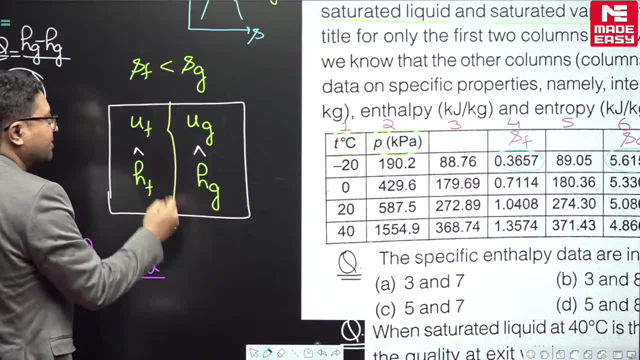 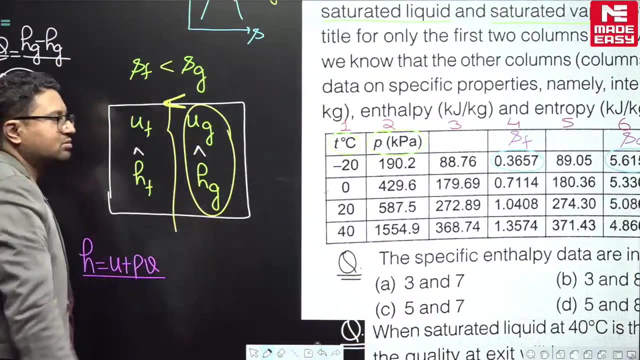 internal energy. it will be more for the very high values. so compared to liquid values, compared to liquid values, the vapor values will be very high. vapor ki value bahut jyada hogi to. out of the remaining four, the higher two, UG and HG. remaining four may say higher two, higher most two. so this is remaining. 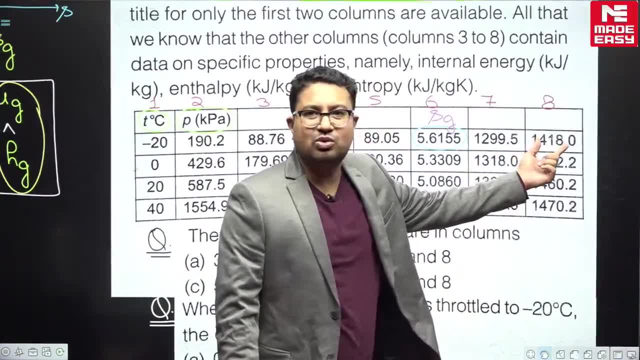 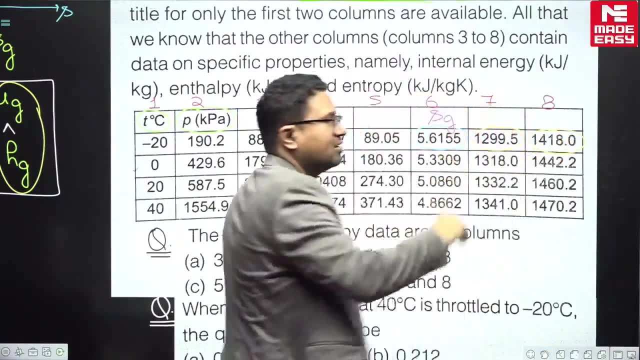 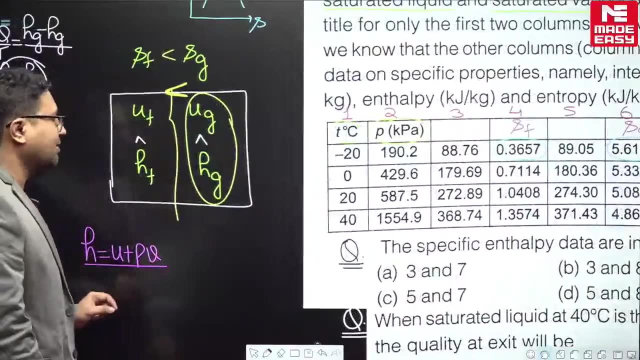 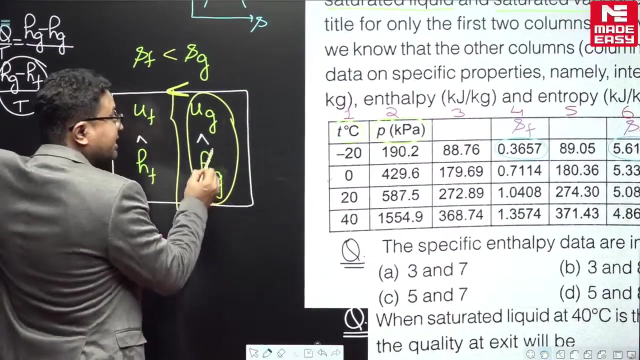 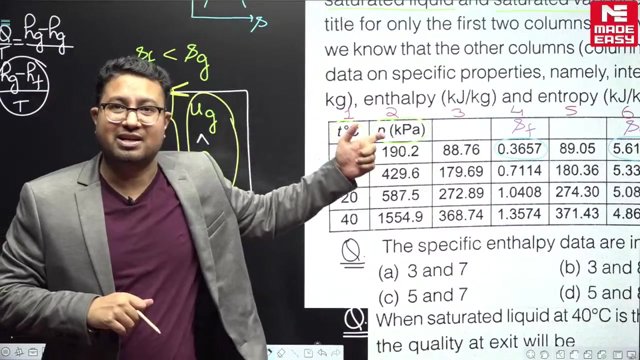 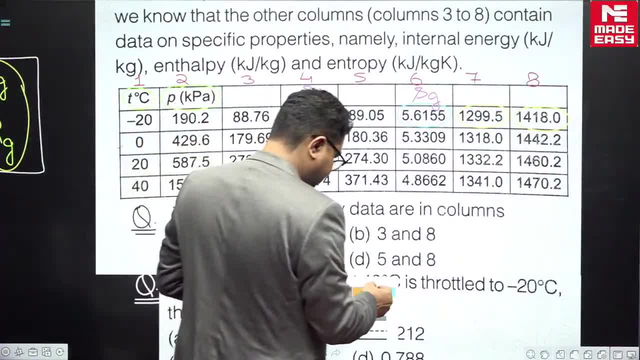 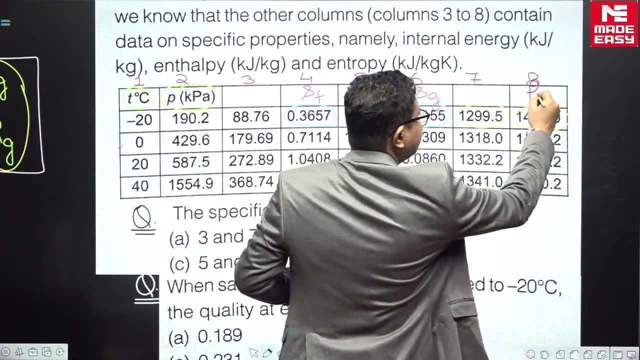 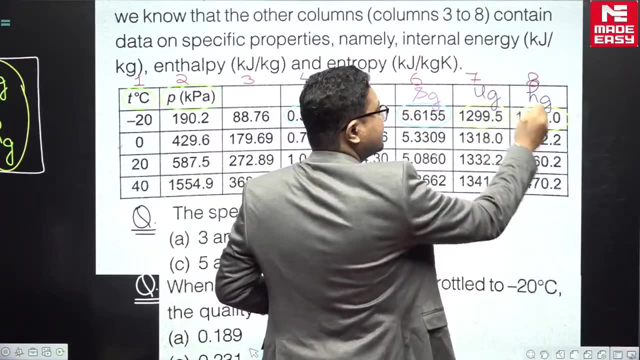 Out of these two, in these two, out of these two, out of these two, the higher one, higher one is HG. the smaller one is UG. Smaller one is UG. Higher one is HG. smaller one is UG. 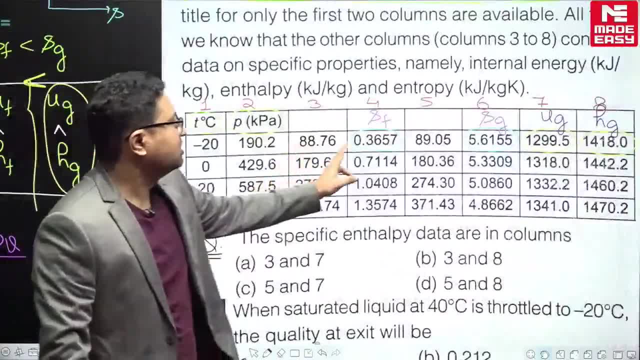 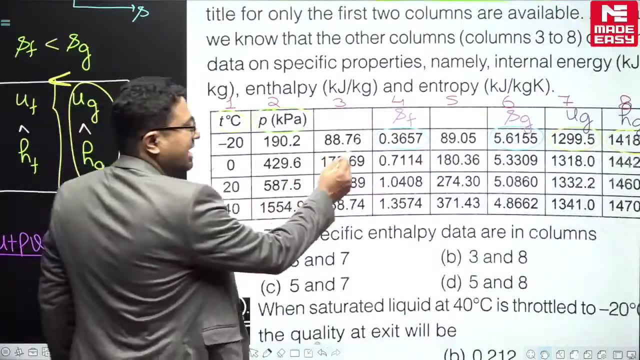 Smaller one is UG. Fine, Now remaining two: one will be UF, one will be HF. Same thing: HF will be more than UF. So this is slightly higher, slightly less. So this is UF and this is HF. 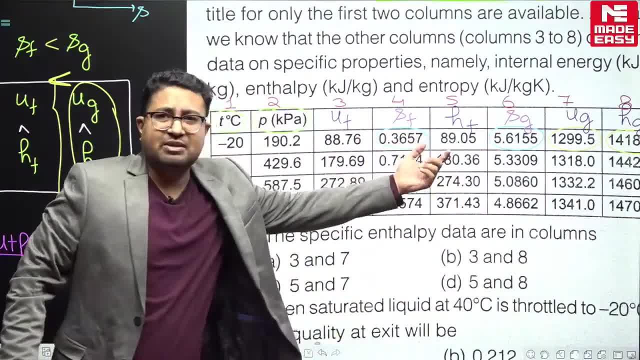 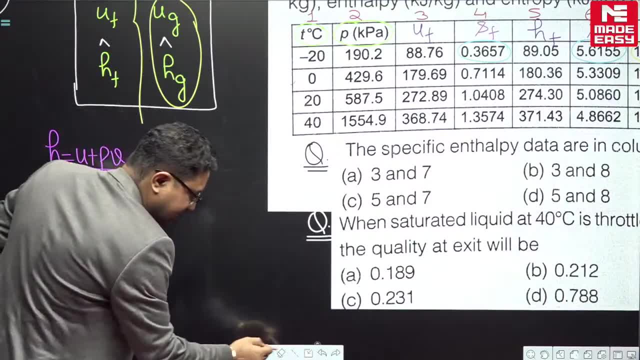 This is HF, UF and HF. the difference is very less. The difference between UF and HF is very less. The reason for that is: look enthalpy. let me write it here: enthalpy is almost equal to internal energy. 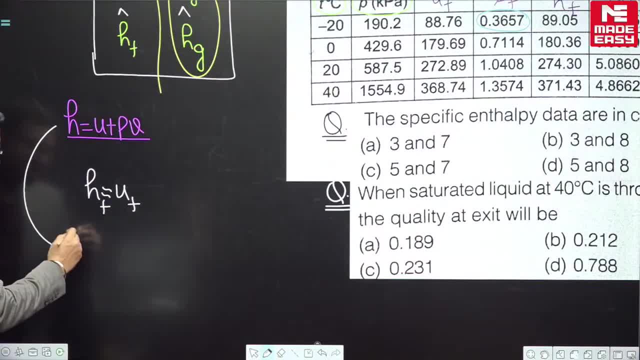 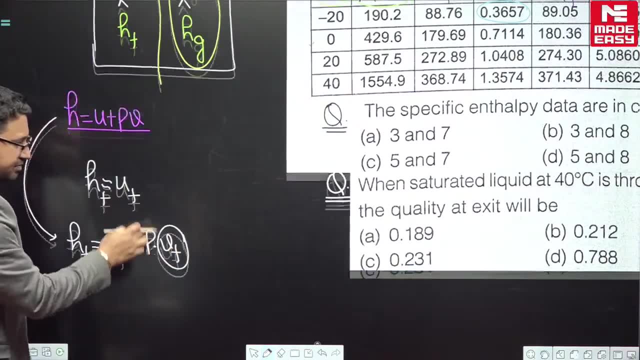 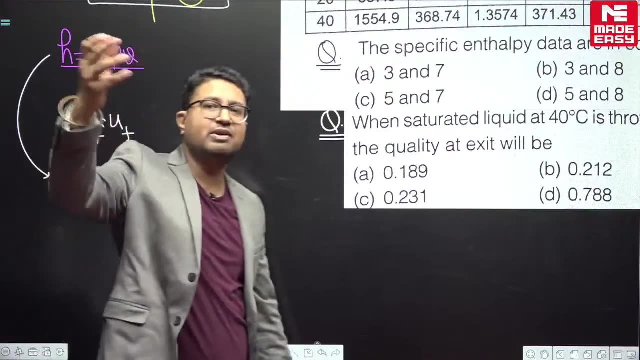 Why? The reason for that is: look- HF is equal to UF plus HF. P- into VF. VF is very less. VF is very less. Specific volume of liquid is very less. It is very less Because density of liquid is very high. 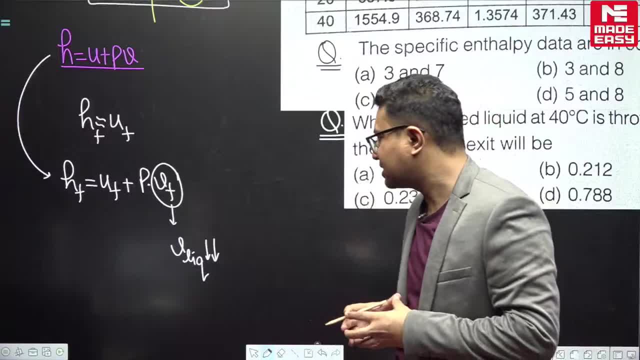 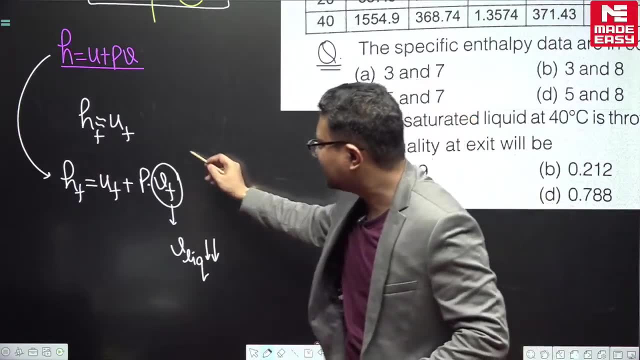 So when you multiply specific volume with the pressure, when you multiply the specific volume with the pressure, you do not get very significant higher value, You do not get very high value. So this expression is very less, The value is very less. 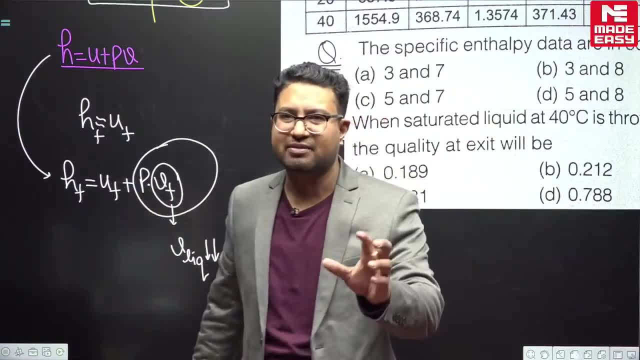 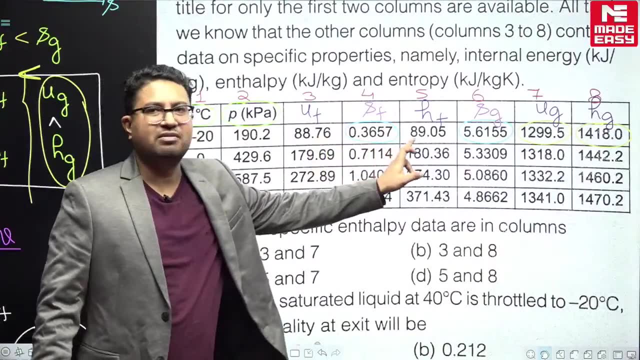 So even if, when you add in this, you add in this, you do not get a very high value. you will not get high value. So that is why it is coming out to be very close. You see very close values. Values are very close, Very close values. Then, so what was? 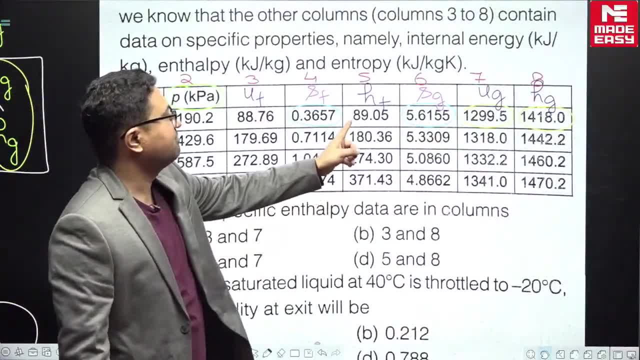 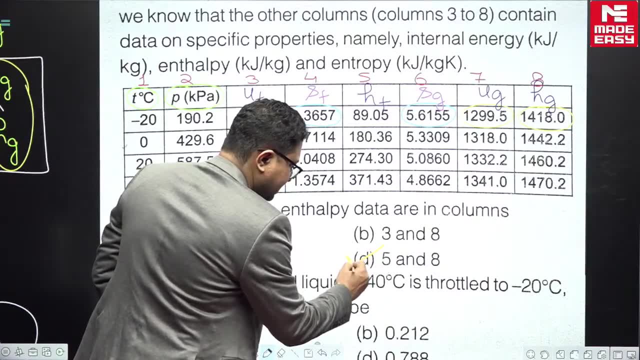 the question. The specific enthalpy data are in the columns. Specific enthalpy is 5 or 8.. So 5 and 8.. So what should be the answer? This? 5 and 8.. This is the answer: 5 and 8.. 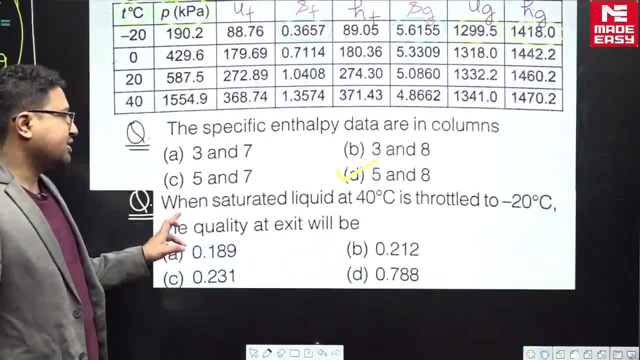 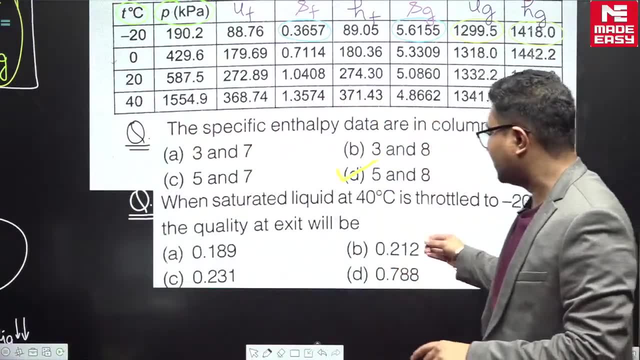 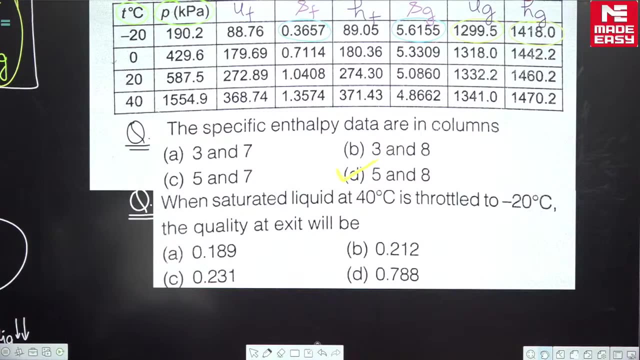 Now let us see this what they are saying. When saturated liquid at 40 degree is throttled, throttling is being done. So when saturated liquid at 40, let me see if somebody was able to give the right answer. Good Prabhat, Yes, Fine, You are. what you said is correct: Engineering. 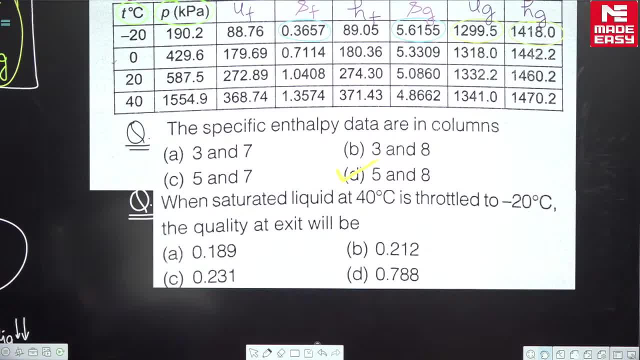 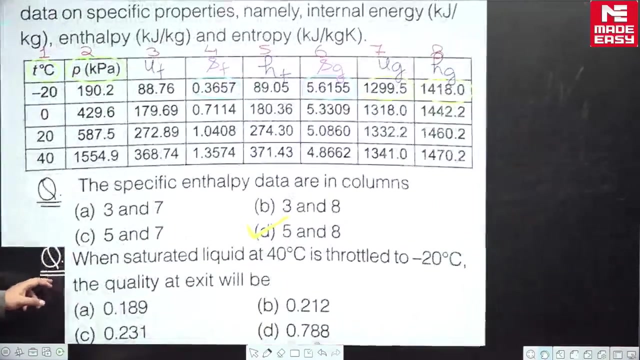 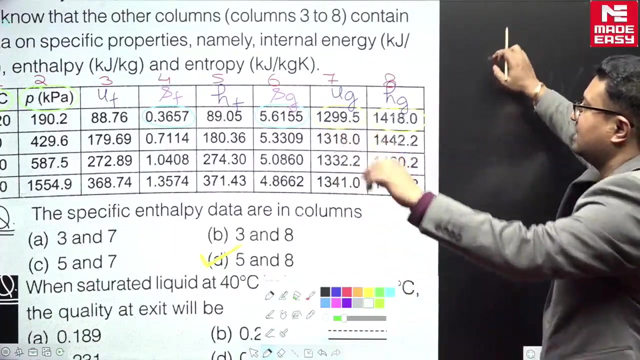 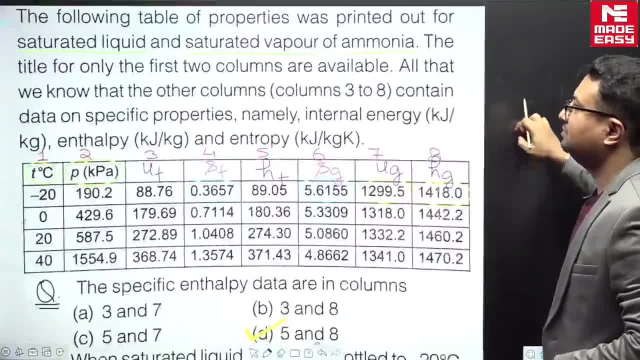 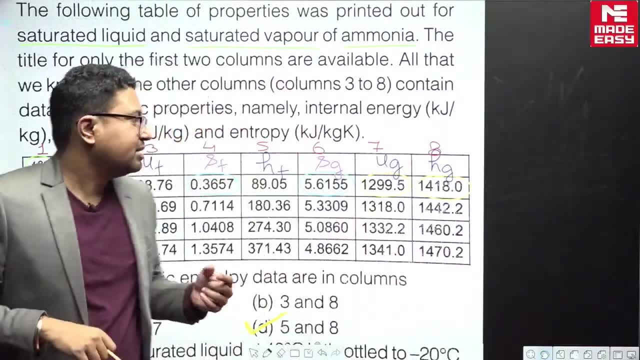 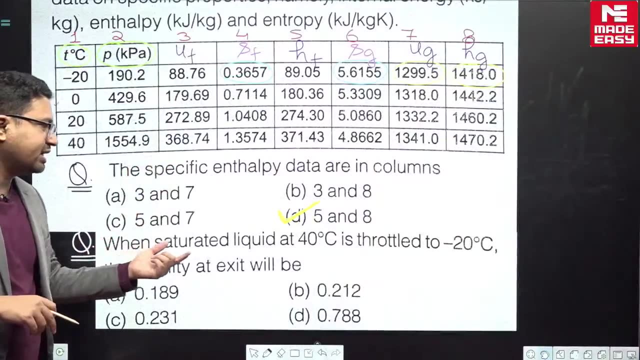 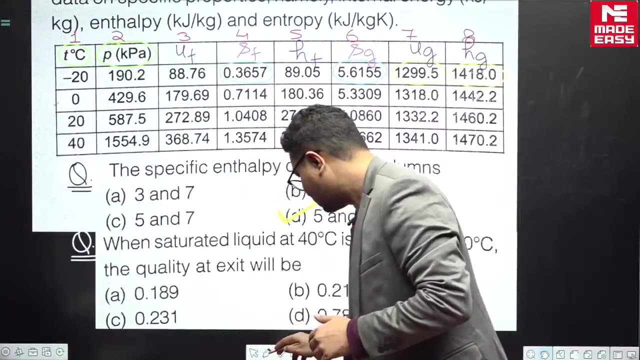 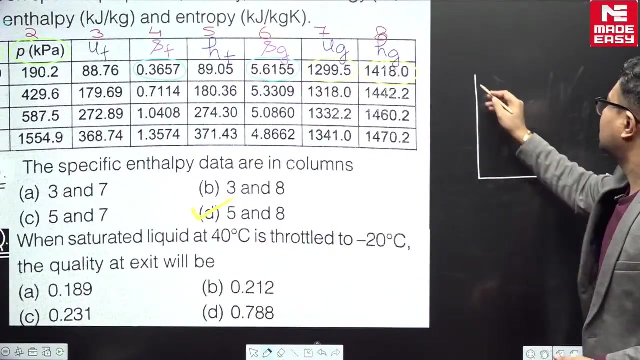 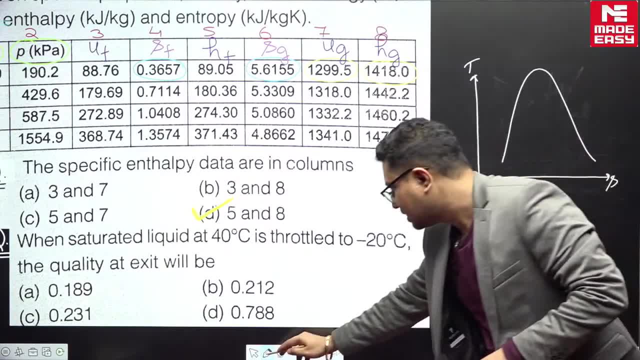 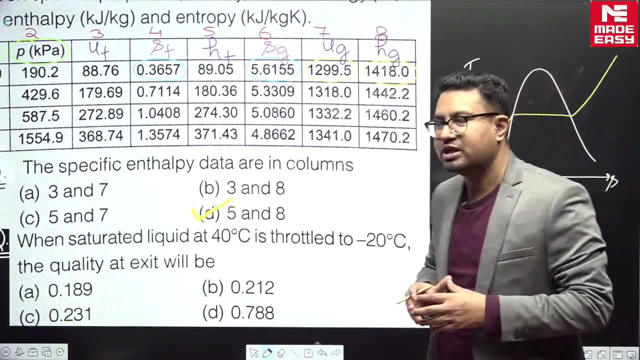 saya. we can say that suppose this is temperature and this is, let us say, the saturation curve. This is saturation curve Now for this and also this and also this, Here on here. Now, as you have seen there many such scenarios, this is the saturation constant pressure curve. Let us say: this is a higher pressure curve. 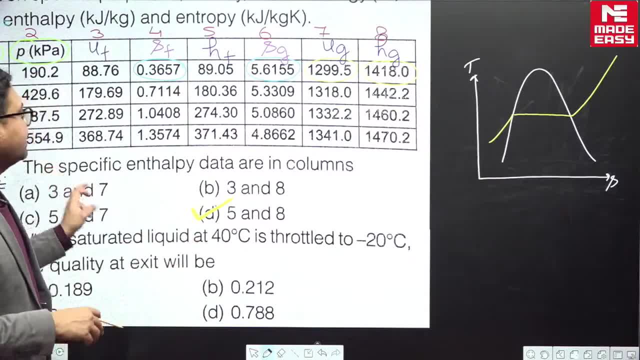 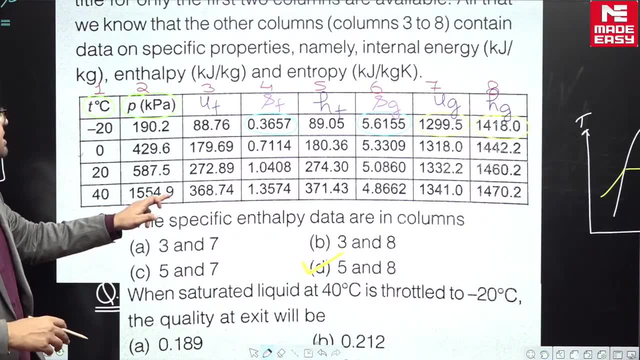 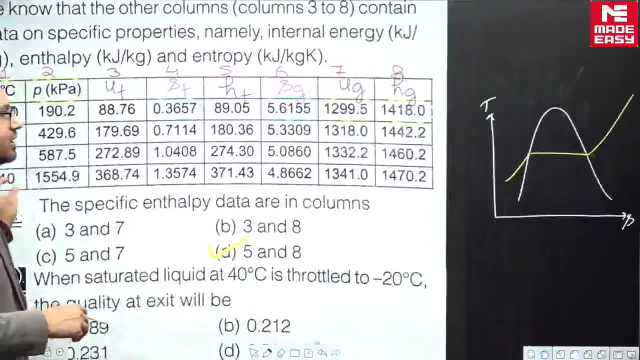 This is higher pressure curve. So 40 degree corresponding pressure is 1554.9.. This is the pressure corresponding to 40 degree Celsius and this is the pressure corresponding to minus 20.. This is corresponding to minus 20.. So suppose this is corresponding to plus. 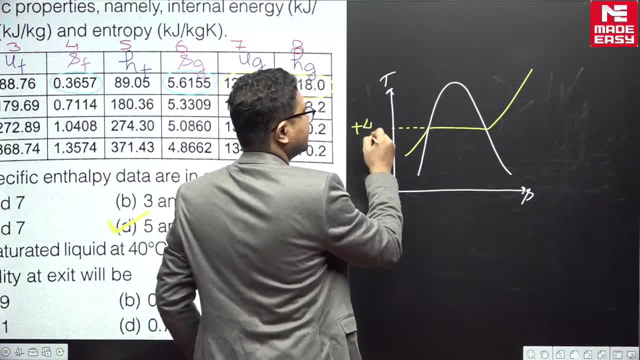 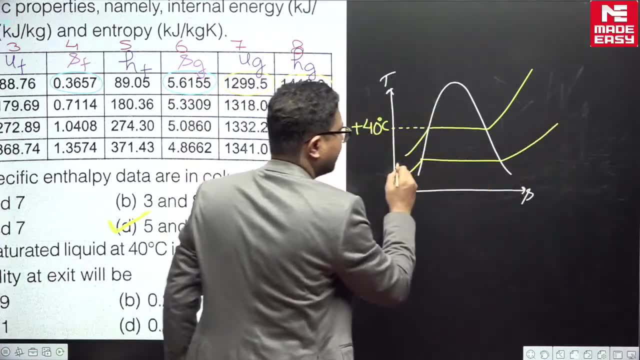 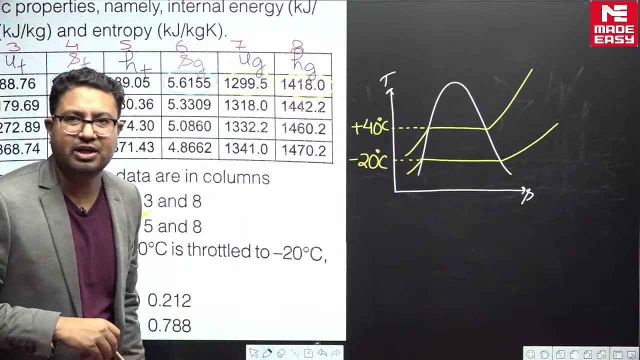 40 degree Celsius, This is corresponding to plus 40 degree Celsius. If 40 degree Celsius is corresponding, then this is corresponding to minus 20 degree Celsius. This is corresponding to minus 20 degree Celsius. This is corresponding to minus 20 degree Celsius. Now you see when. 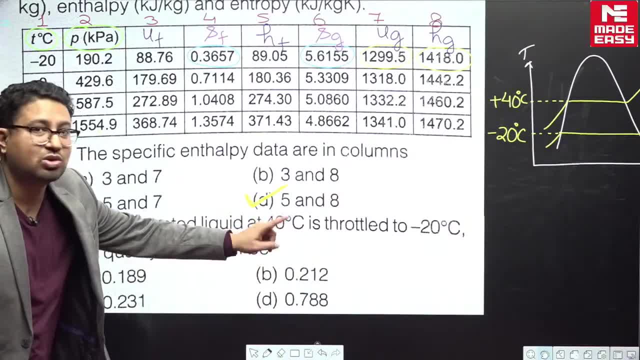 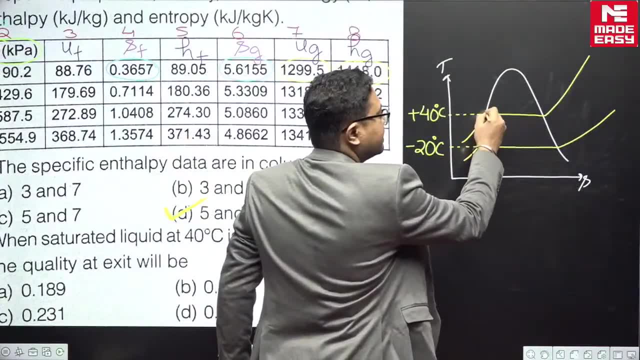 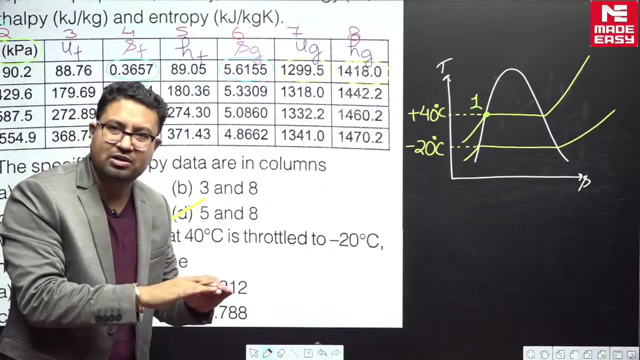 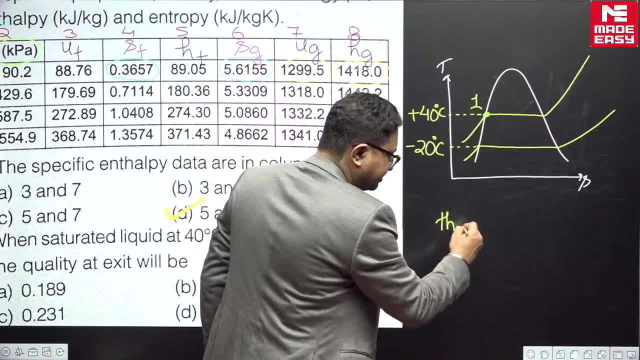 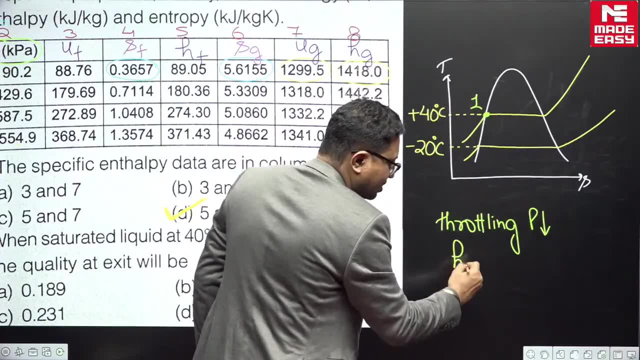 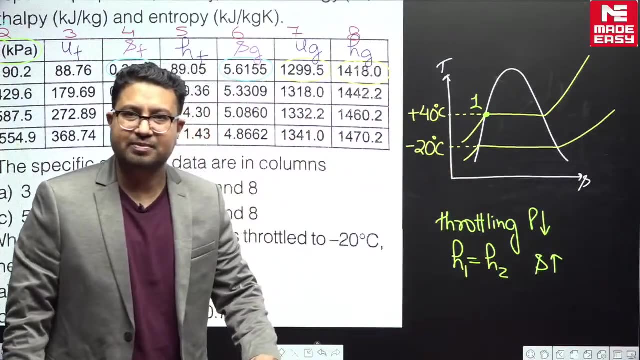 pressure. So what happens in throttling? In throttling, the pressure reduces, Pressure goes down, Pressure reduces, Enthalpy remains constant. H1 is equal to H2. But the entropy increases, Entropy increases, The entropy increases. So, in whatever situation, constant. 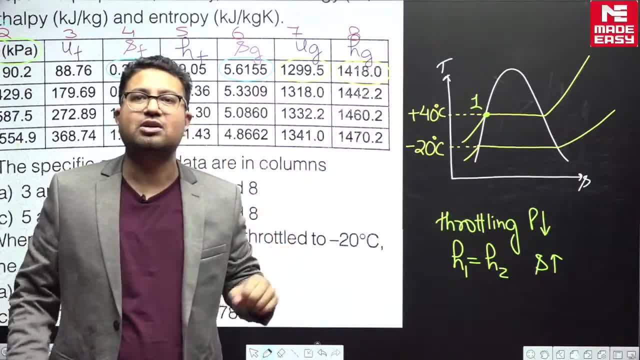 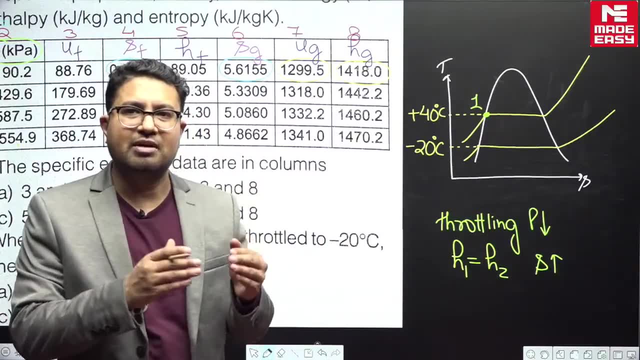 pressure processes may, or when the entropy is constant or it is increasing, TS diagram becomes very helpful. Actually, TS diagram is most widely used even for solving problem. That is why I have taken the TS diagram for discussion Discussion. so PT diagram ka bhi. 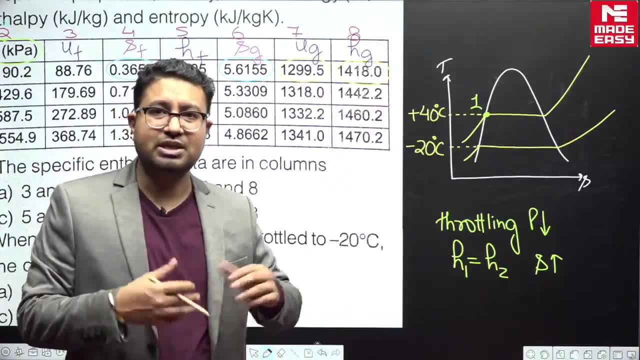 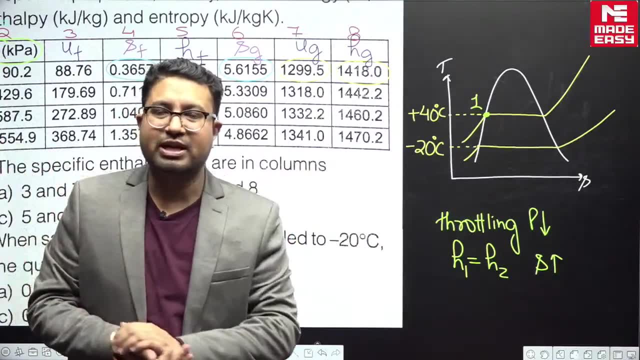 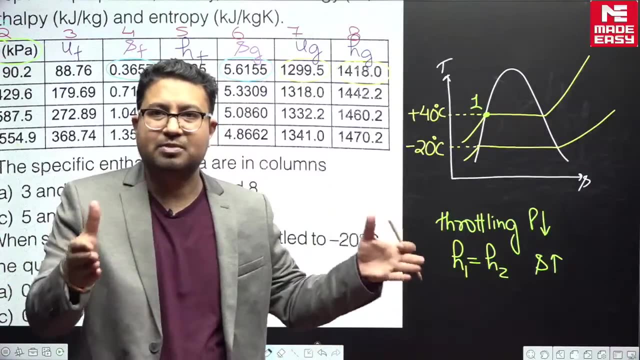 ho sakta hai. Discussion can be for PV diagram Generally, TS PV pressure specification volume, PT pressure temperature diagram and HS Moliere diagram. These are the diagrams which we discuss, jo hum discuss karte, But it is not possible to discuss all the diagrams. 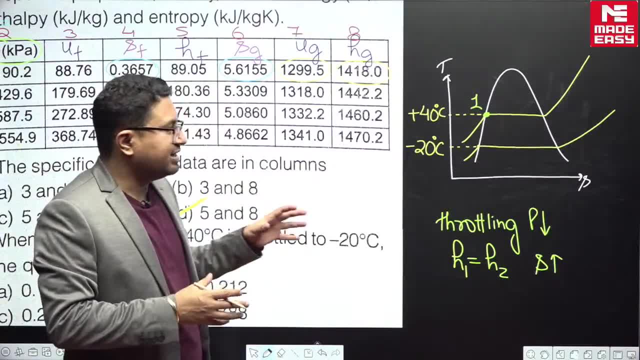 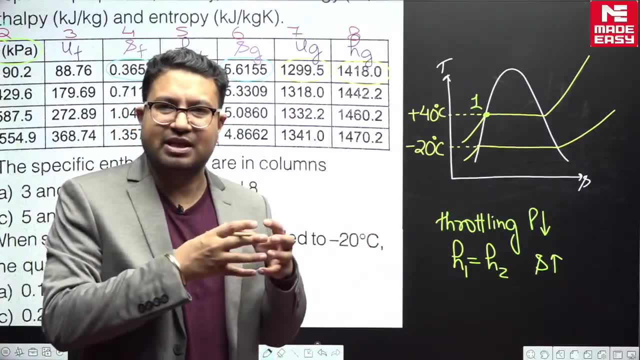 in a given time. So TS diagram: we have picked one diagram, Humne diagram, pick kiya TS diagram that we have discussed to the length, Humne sari baate uski discuss ki We discussed the entire length and breadth of whatever this TS diagram is. Other diagrams which can: 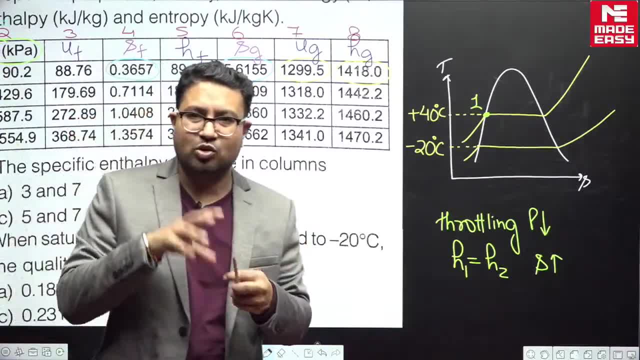 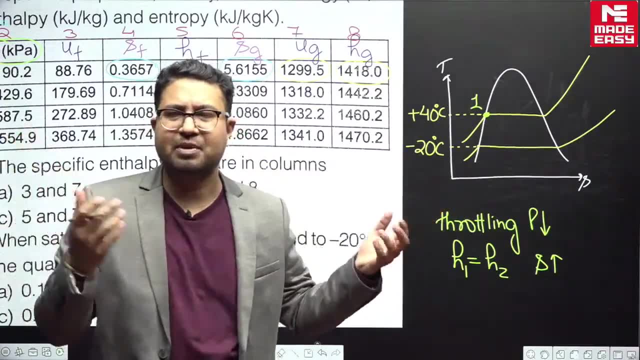 be discussed is PV can be discussed. Jo relevant hota hai, jo aapke question solving ke liye, jo relevant diagrams hota hai. They are TS. can be discussed, PV Otherwise diagram to bho saar hai: TS, PV, PT, pressure temperature. 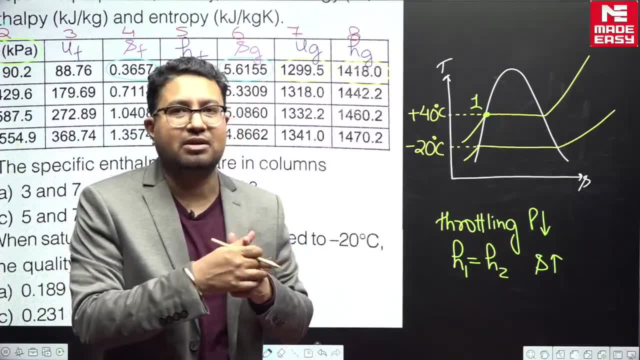 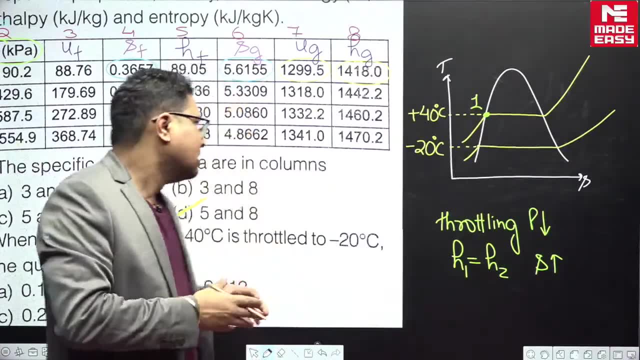 and HS Problem solving ke liye TS and PV. numerical solving ke liye TS and PV are more relevant. Theoretical questions bante PT se, HS diagram se bhi. But agar aap dekho, ke problem solving hai mostly RAC, power plant thermodynamics, we use the 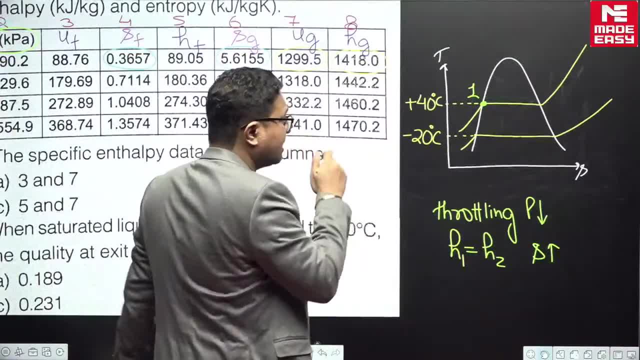 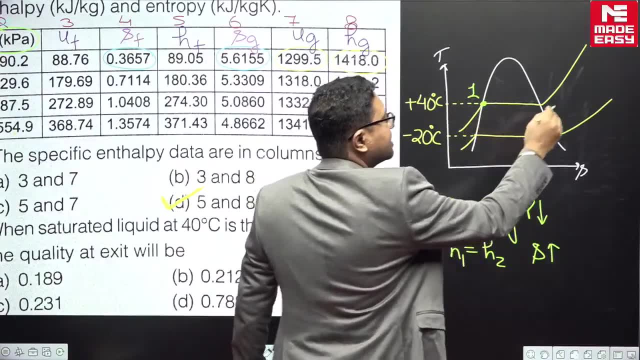 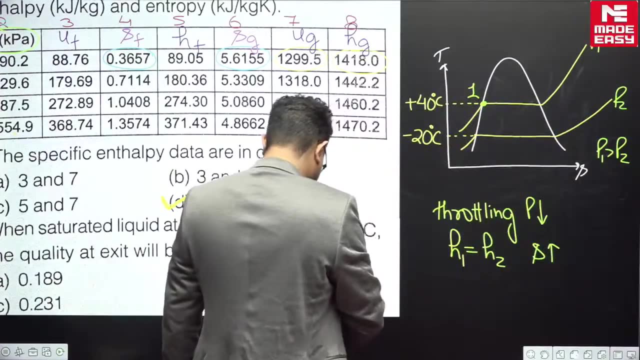 TS diagram. So if you see, agar aap dekho, this is the condition 1.. Ye condition 1 hai and throttling. So throttling for this lower pressure pressure, let us say P1 pressure, and this is P2.. P1 is higher than P2.. So throttling pe pressure kam hoga The point. 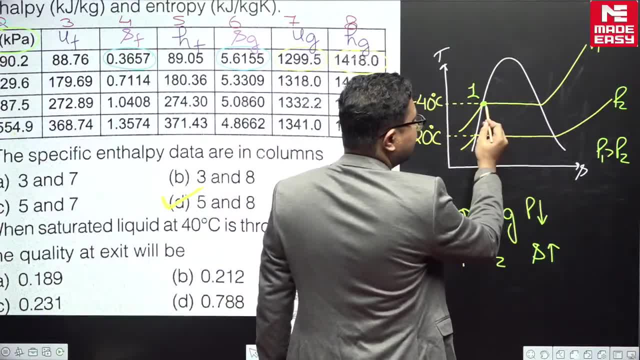 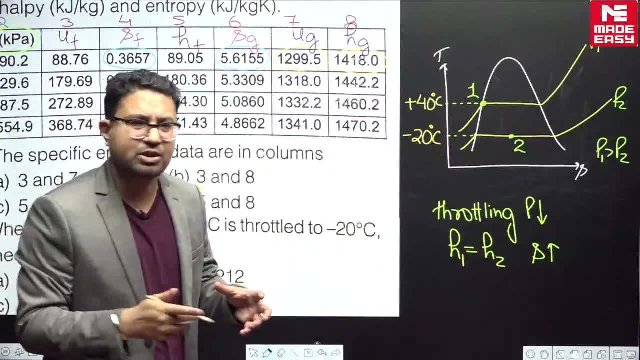 2, the point 2 will be on this, but at a higher entropy. Toh, let us say: yahan pe hai kai. Let us say: it is here somewhere. Okay, Throttling hai irreversible process hai. I will just show it with the dashed line. dashed line se show: karoon ga isko main I. 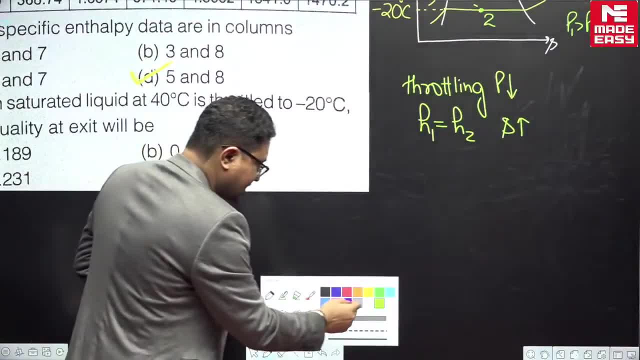 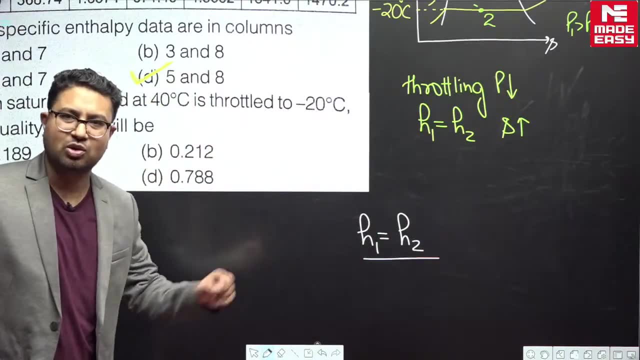 will just show it with the dashed line, So we can say: hame ye khai sakte hain ki H1 will be equal to H2, H1 H2 ke barabar hoga Throttling process hai. So what is H1? H1? 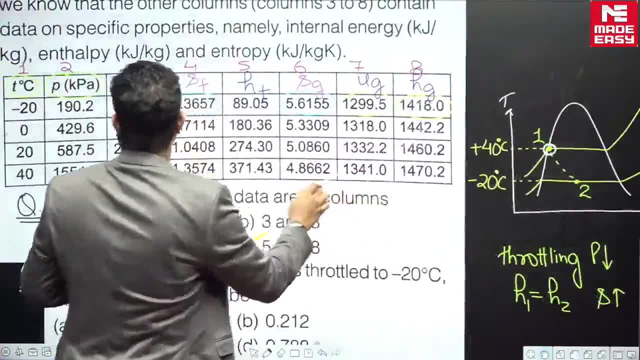 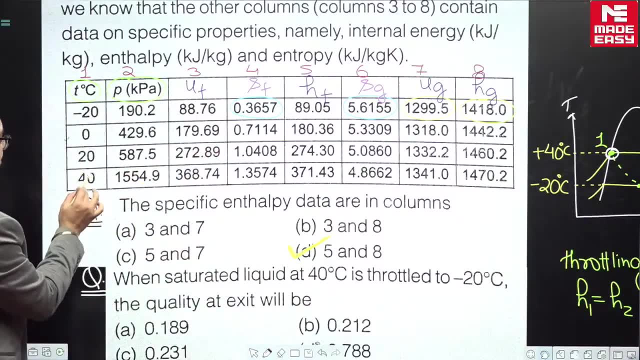 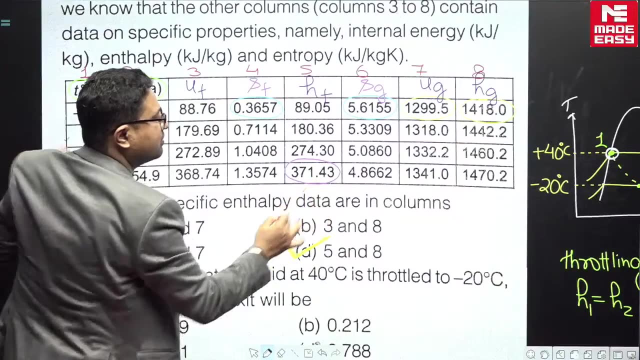 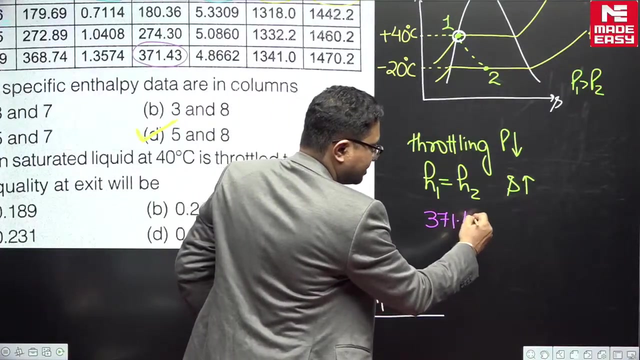 is HF. H1 is HF at plus 40.. H1, kya hai? HF hai plus 40 pe. So plus 40 pe, hF plus 40, this is hf. this is hf. so 371.43, 371.43 is hf. so this is equals to 371.43. this is h1 is hf. h1 is. 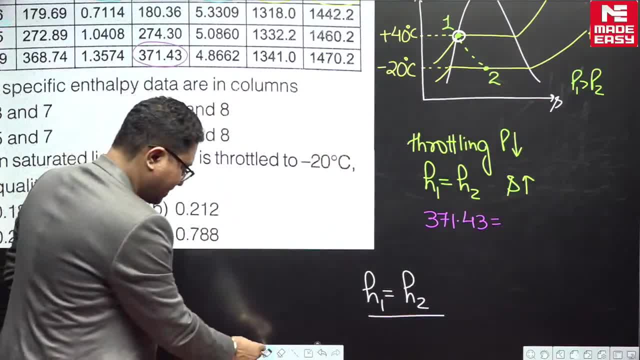 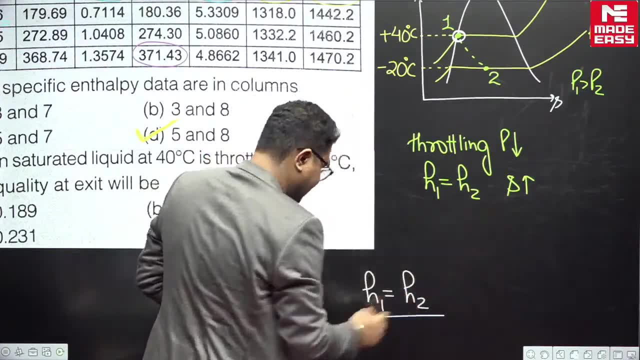 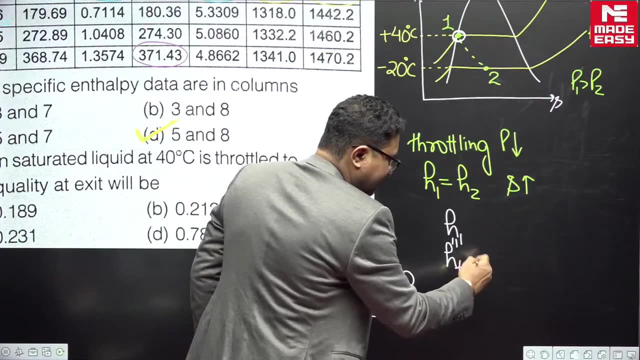 hf, h2 is hf. this is at higher pressure, so h1 is equals to h2. I will write it here: h1 is equals to h2, but h1 is hf. h1 is equal to hf, hf at pressure p1, and this is equals to hf plus x2. 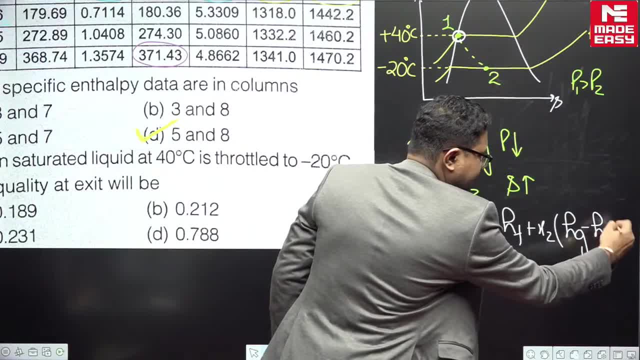 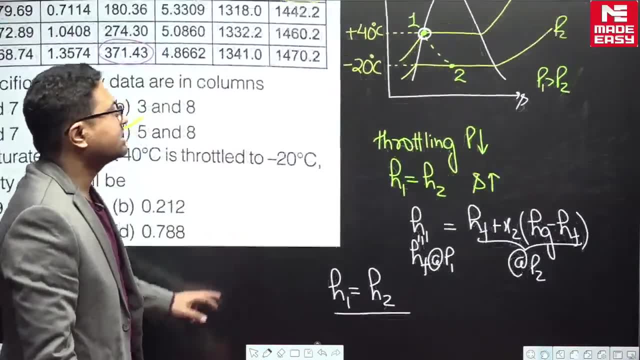 into: hg minus hf. hg minus hf. this is at pressure p2. this data is at p2 pressure. okay, so h1 is hf. this is equal to hf. we can see, we can write here: h1 is hf. this data: 371.43, 371.43. this data: 371.43. 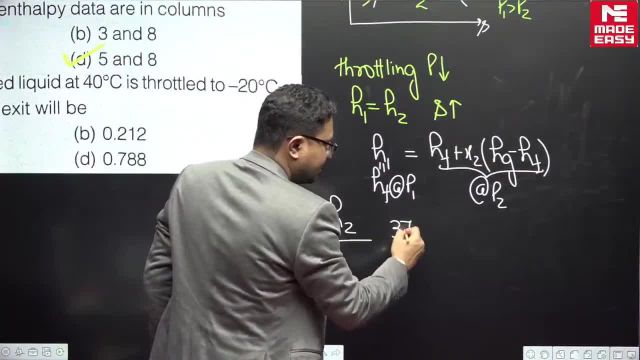 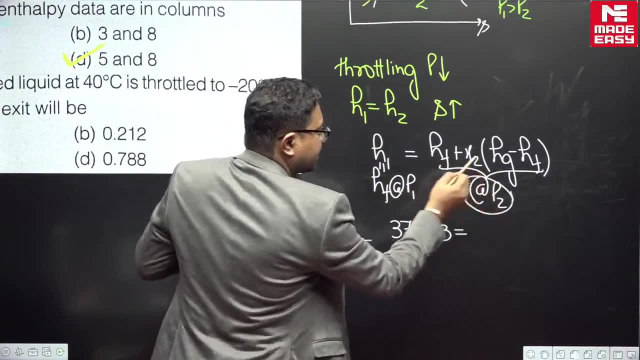 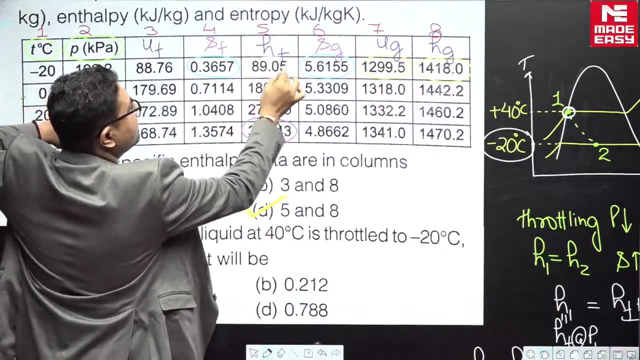 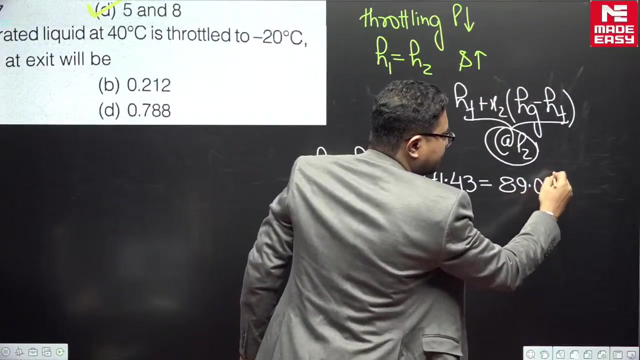 this is 371.43 and this is equals to this hf and this hf is not same. this is at p2 pressure, so p2 pressure is minus 20. temperature corresponding saturation temperature is minus 20. so this is hf 89.05- 89.05. this is hf 89.05.05 plus dryness fraction x2 into into hg, minus hf. 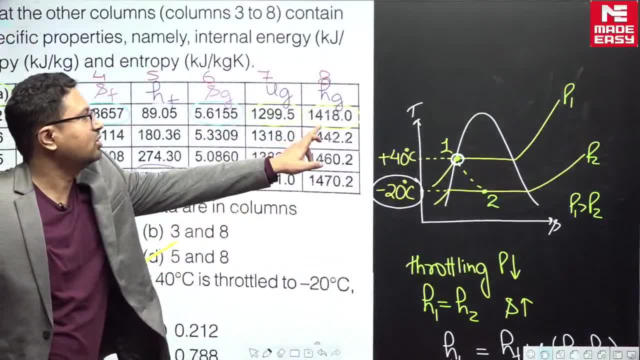 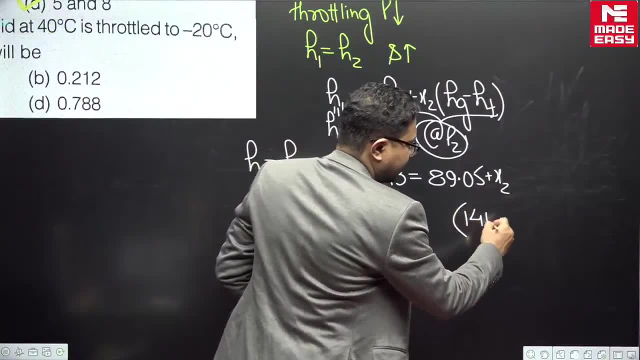 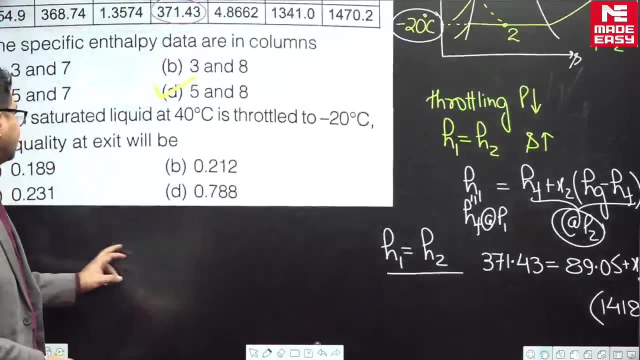 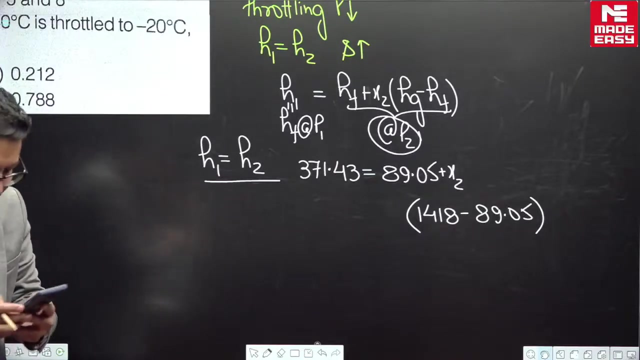 so hg minus 20, 1418, 1418. so 1418 minus hf is 89.05. dryness fraction x2. dryness fraction x2. what it will be x2 dryness fraction value. just let me know what will be the value of dryness. 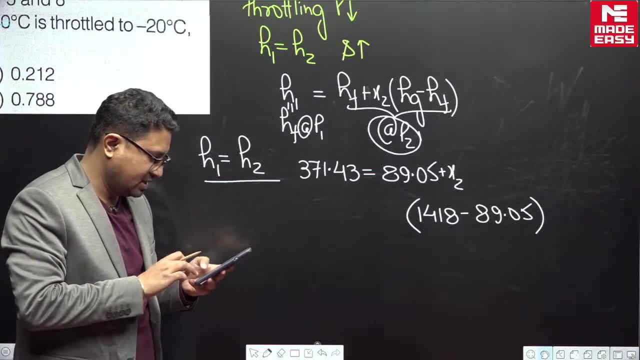 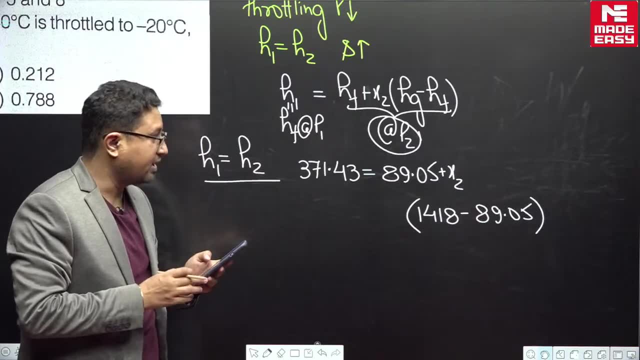 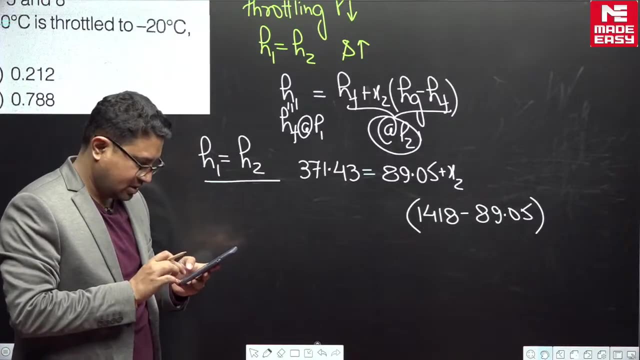 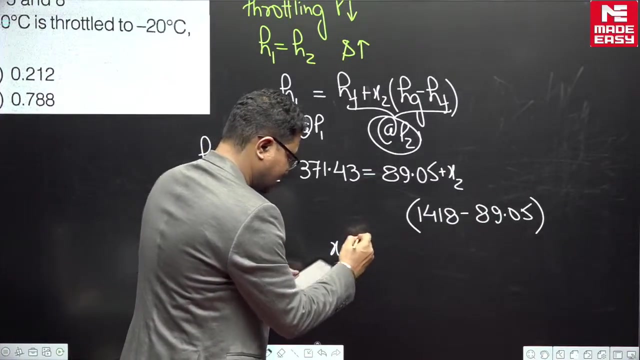 fraction. So we have 371.43.. 371.43.. So we have 371.43 minus 89.05 minus 89.05. this is divided with 1418 minus 89.05.. So dryness fraction x2. dryness fraction x2 will be x2. this will be 0.0.212. yeah, dryness. 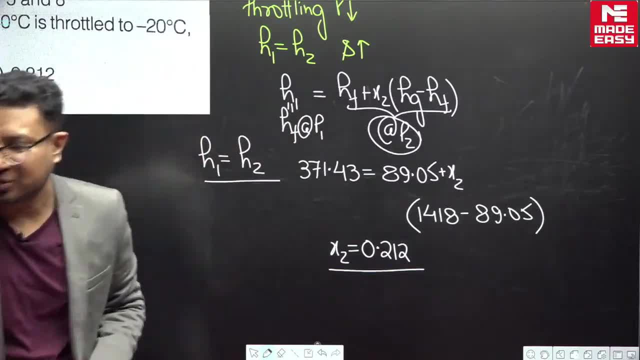 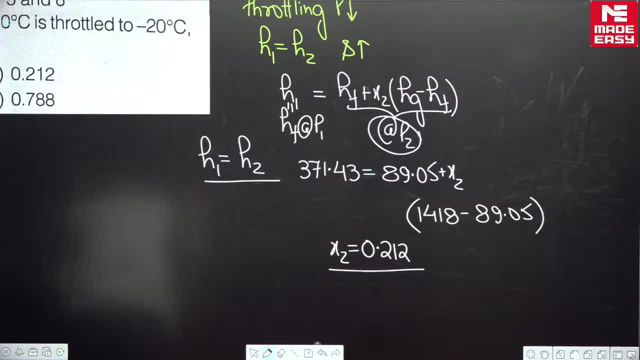 fraction x2 is 0.212.. x2 is 0.212.. So yes, Abhishek kumar, Raj keming, Mukesh kumar, Raju kumar, Mansoor Sharma, Shashikant Gautam. 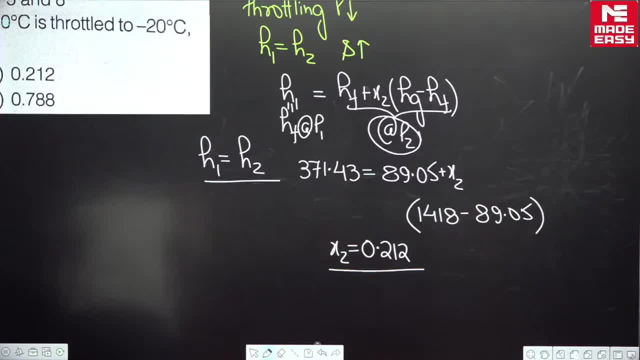 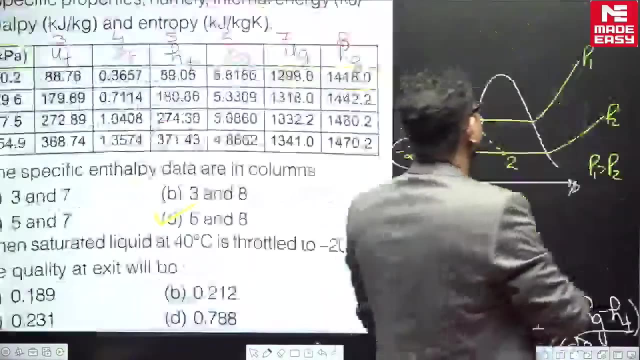 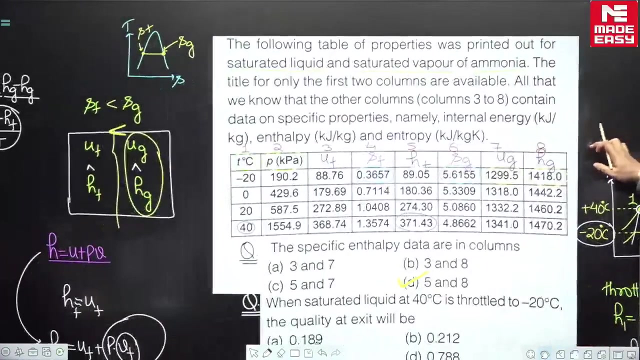 Shashikant Gautam. fine, So this is see. this is the. this is the discussion. a discussion hai for the. this is the discussion, discussion For the. this is the discussion here. ye question hai. just see the question. I will show you the discussion also. 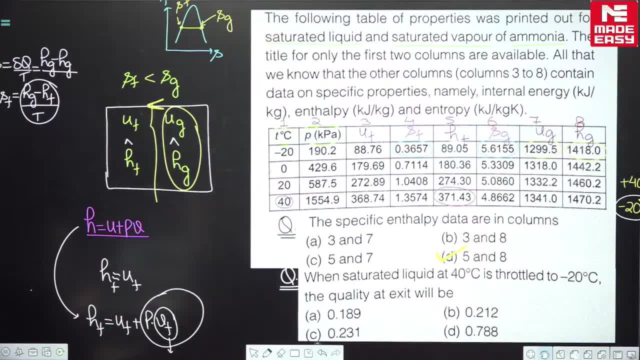 Discussion bhi dikhaunga aapko: yaha pe presents Hi ued 강 felt. they responding: ok, understand me. yeah, I Nadja. bye, bye, Mr Buhari. Name: Mansoor Sharma. Nama na nana 1948. 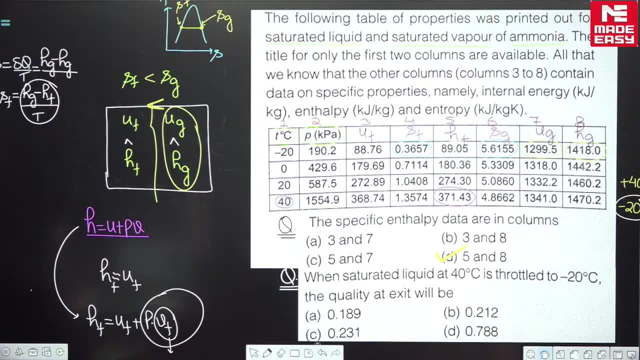 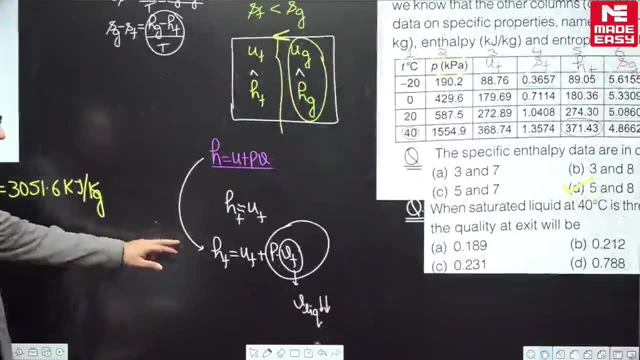 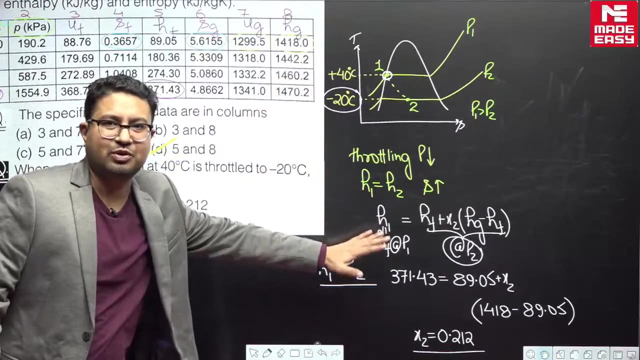 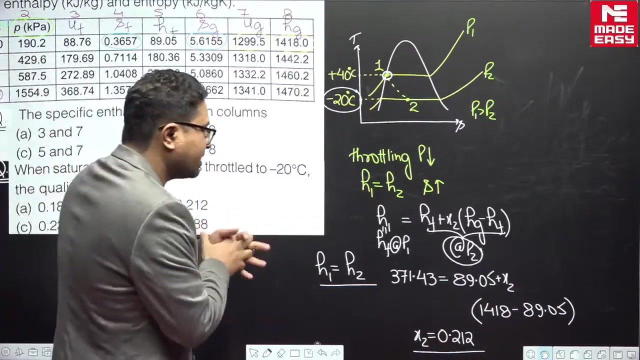 Yes, so this is here. this is here now. this is the discussion. just let me show you discussion we have done and this is this is the. this is the TS diagram and the second part of the discussion. So if you want, you can take the screenshot here, the entire solution I have. 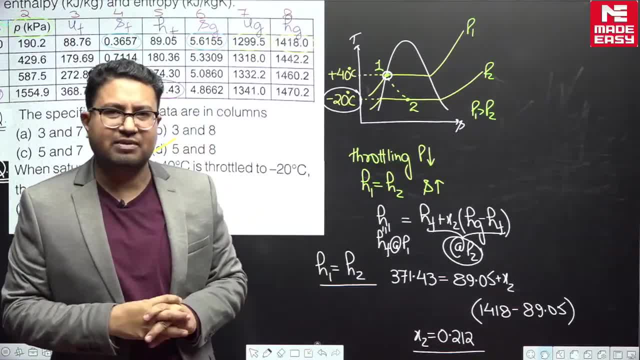 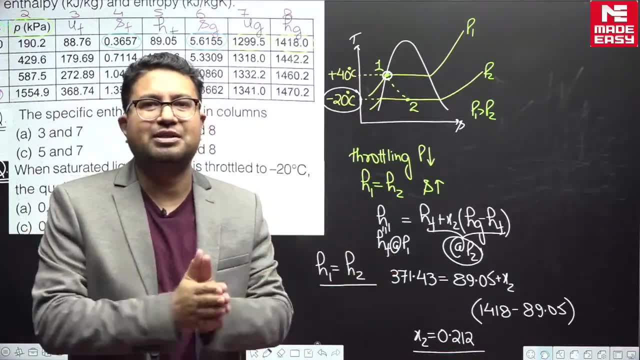 shown you. So see the TS diagram I have discussed. we were discussing the properties of pure substance. properties of pure substance ka discussion. hum kar rahe the and we have discussed the TS diagram. humne TS diagram ka discussion kiya and plus the basics of the properties. 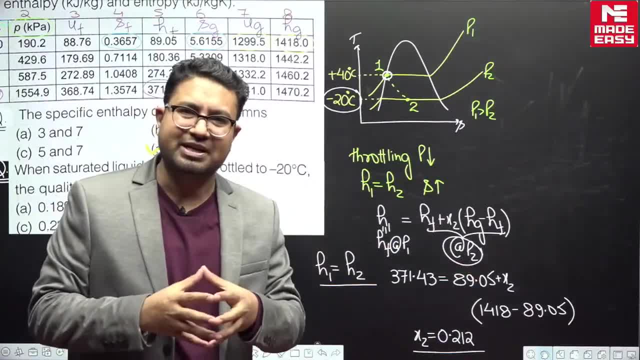 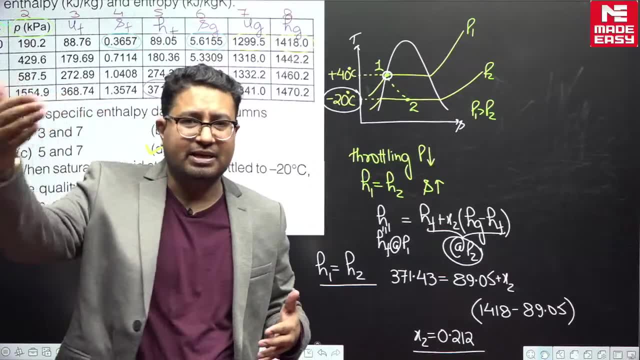 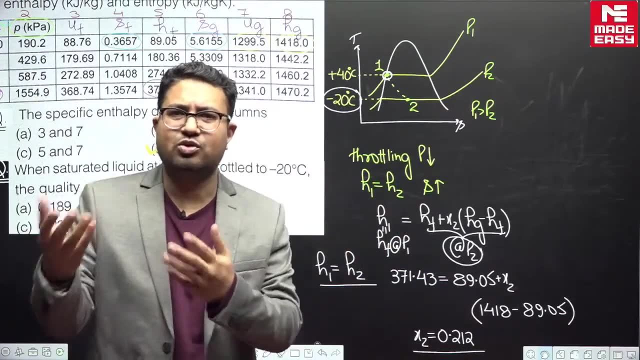 of pure substance and we picked up one diagram- ek diagram, humne pick kiya, TS diagram, and we discussed it to its entire length. And other diagrams- PV, PT, etcetera- that can also be discussed, but the session time will not allow that discussion. tomorrow you have your another session lined up, So this is 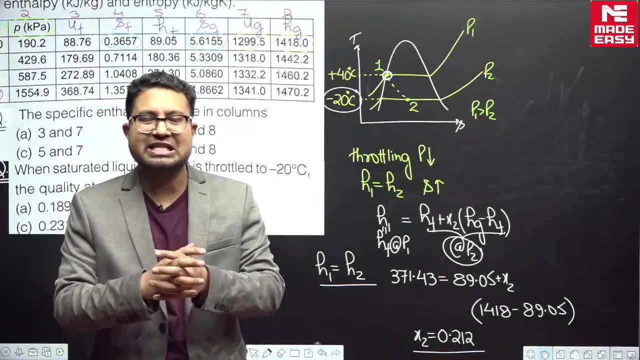 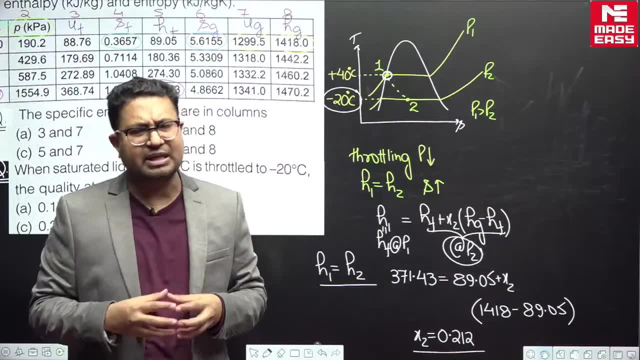 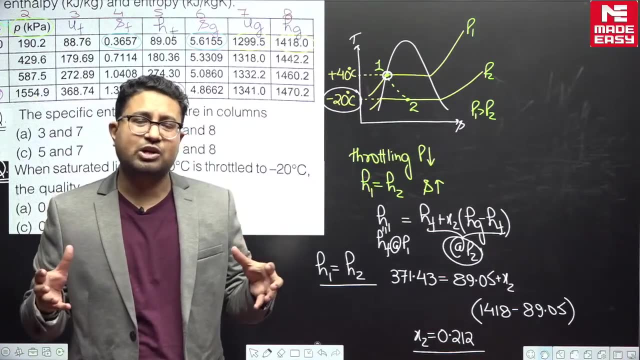 it for the discussion. ye humara discussion tha for the TS diagram as well as the basics of the properties of pure substance. we went into very details, for detail, humne baat ki iske baare mein, And So we have also tried to visualize some questions by solving some questions, by plotting the 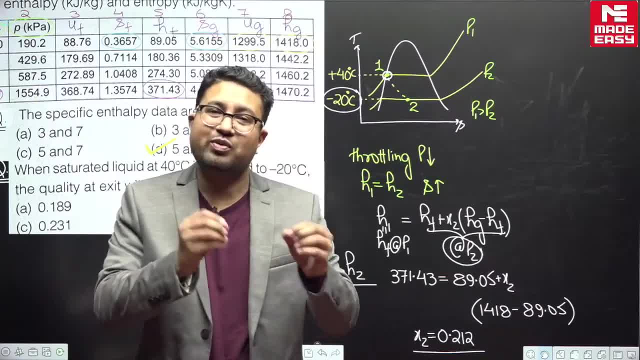 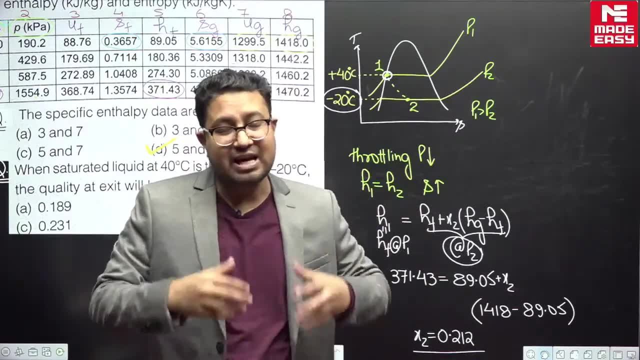 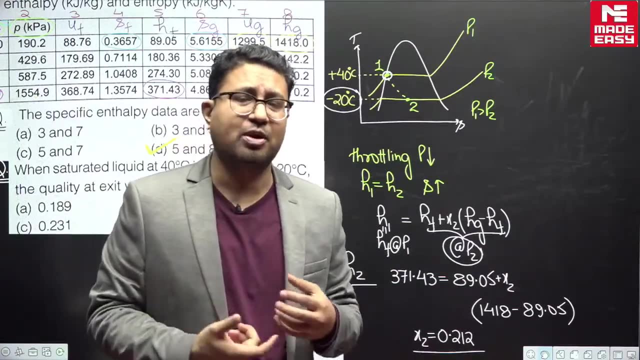 points we have tried to visualize ki how we can exactly understand a question and show it on a diagram, and then the visualization becomes very easy, Visualization bahut asaan ho jata hai, and then the reaching the solution to the problem becomes very, very easy. for 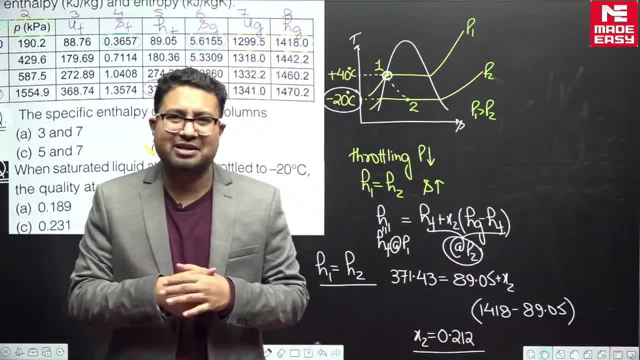 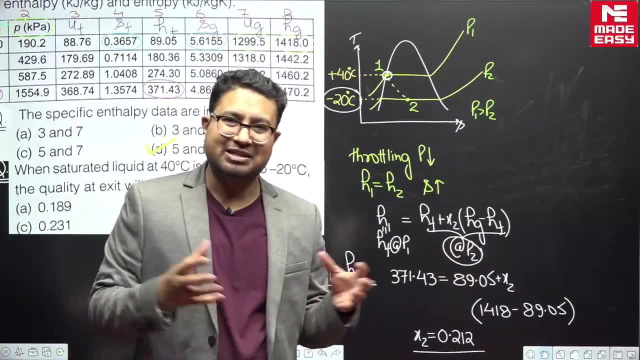 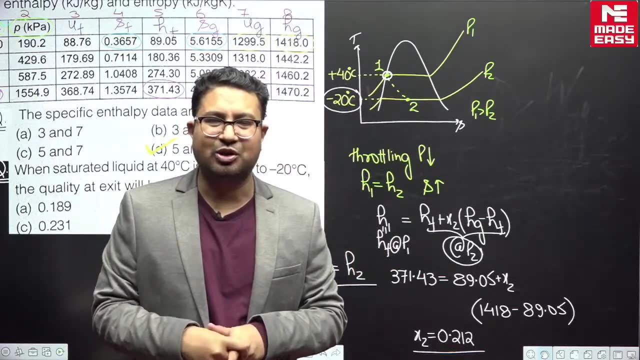 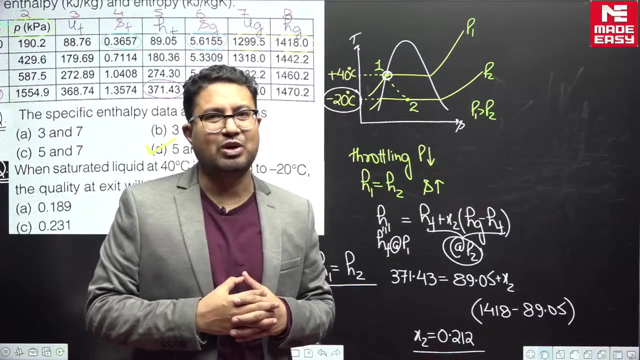 us. So thank you so much for watching aapne bahut saare log. there is a lot more to discuss, Thank you, So let us talk about little more. then also Here continuously, you are I mean interacting continuously. you are present in the entire. discussion. So thank you for watching and we will be completing this discussion here itself on the TS diagram. or the people who are preparing for the exams, the people who have to give the exam: zin ko gate exam, dena hai etza baar. So just continue your preparation. just continue your preparation day, one day at a time, ek din, ek baar ko you have to give the exam, zin ko gate exam dena hai as baar. So just continue your preparation. just continue your preparation day, 1 day at a time, ek din, ek baar k kperson is agrade that you attend. as I said, this is an 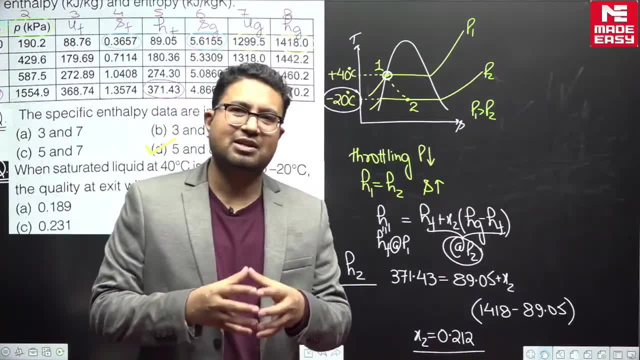 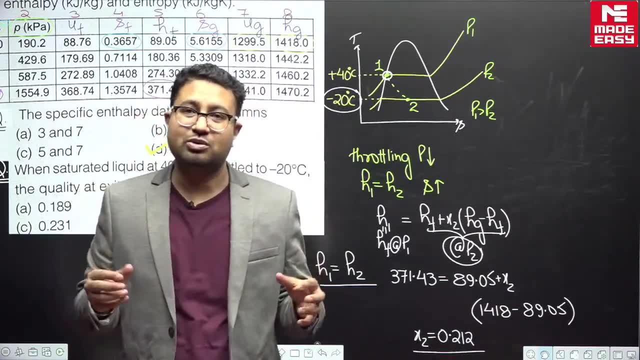 the other in the actual check of pert consulted to that doubt. the answers are important to every person. One day at a time, ek din, ek baar, mein just write down the time of your study. Aap apni padhai ka time likho, whatever study you are doing, jo bhi aap padh rahe ho, just. 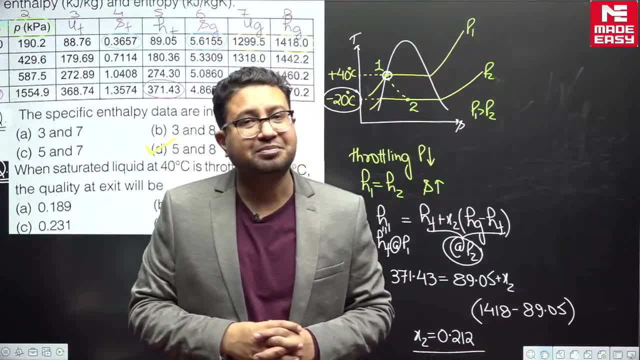 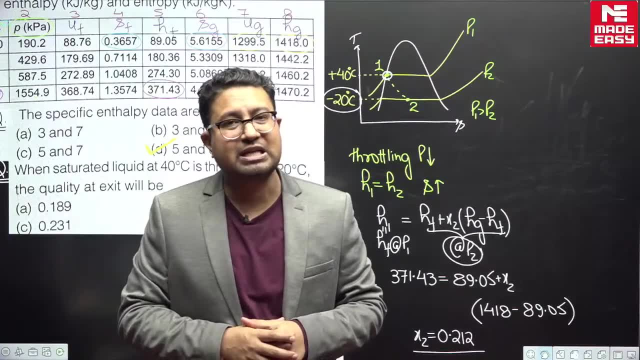 write down the time time likho uska and that will help you to analyze wo aapko help karega. analyze karne me to understand aapko samajhne me. aapko analyze karne me, help karega that. 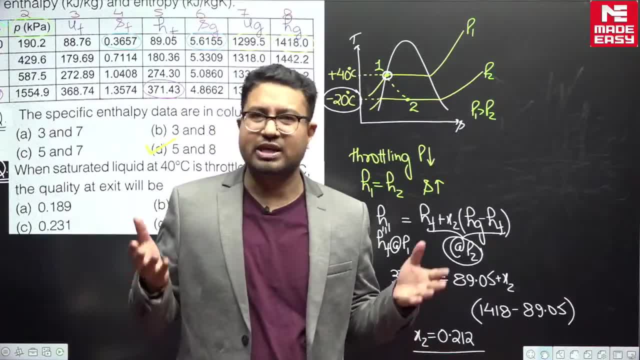 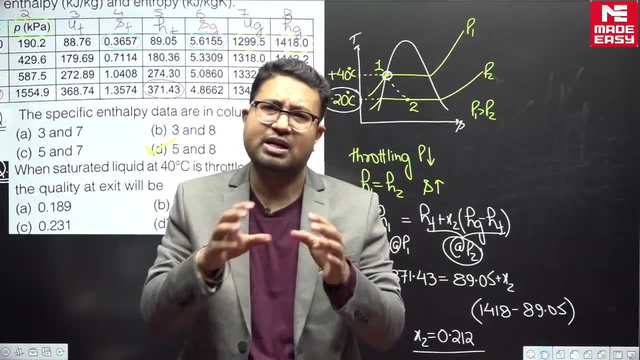 what is the track you are going on? that is the best we can do. yehi aap best kar sakte hai ki we take a day and we go through the entire day. jitna bhi humne us din padha hai. 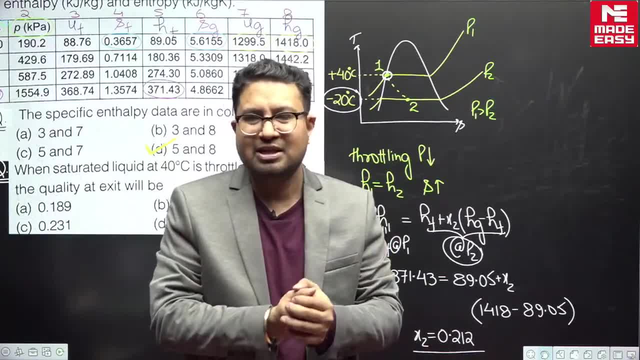 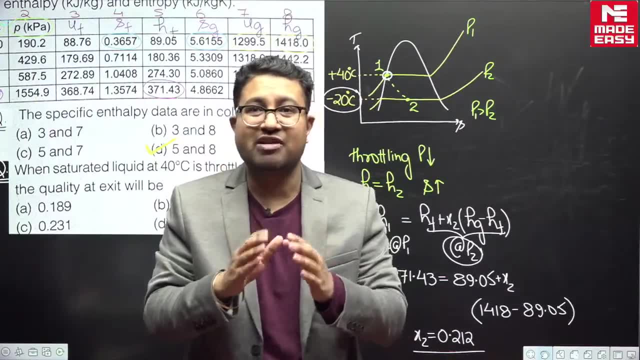 we just write down the time when I used to write down main yeh karta tha that before sleeping I used to write down the time that this is the number of hours which I have studied, and the time which I will note down will be minus everything else. suppose if I went for. 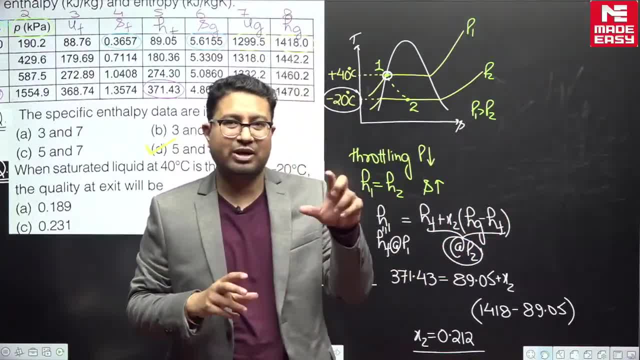 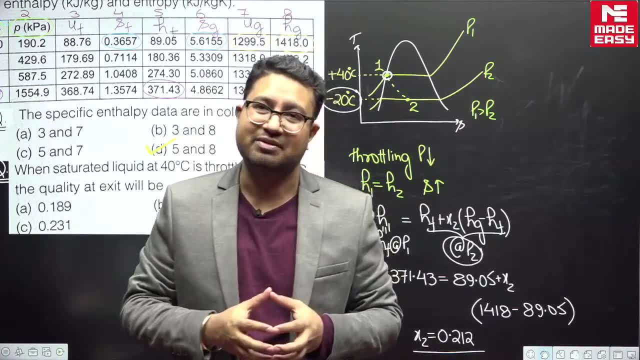 the washroom. that time also I will detect. so that is how I used to maintain time. so I used to have an idea. ki bhai, how much time I am devoting for the study Every day from here till the exam days are limited. each day you are studying or you. 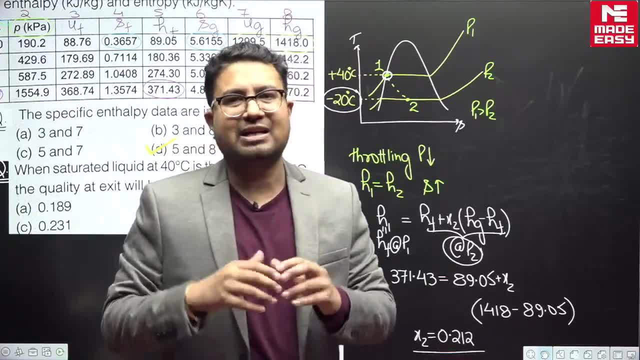 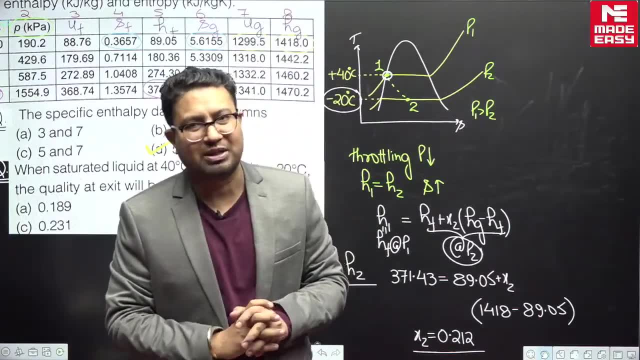 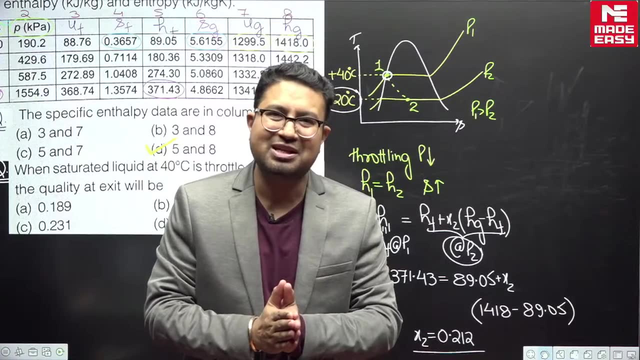 are giving your best. so if you do not study today, that cannot be compensated, wo compensate nahi ho sakta hai. so that is how you have to plan, that is how you have to move forward theek hai. So thank you so much and all the best for your exams. all the best for your exams. so. 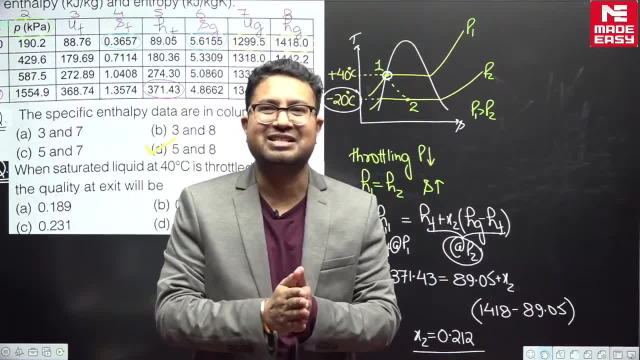 I am Amrinder Singh, signing off this discussion, ending this discussion here. Thank you so much for watching. Thank you, Thank you.